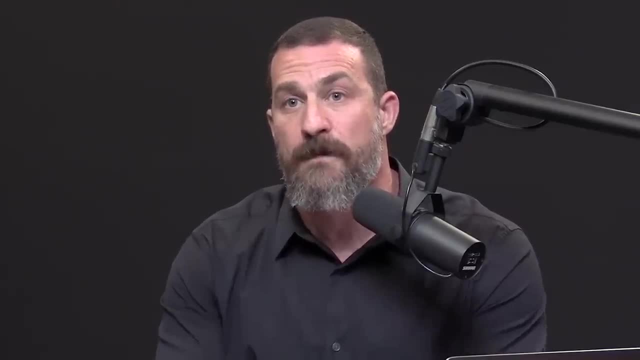 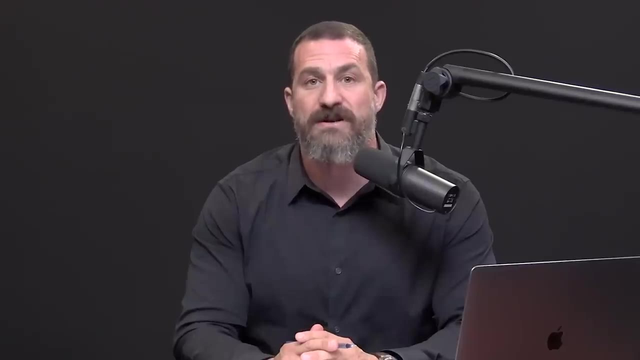 are critical for healthy weight maintenance, weight loss or directed muscle gain. We also talk about supplements, in particular, the supplements for which there is an immense amount of science pointing to their safety and efficacy for fitness and for health. We also discuss and for overall body composition. 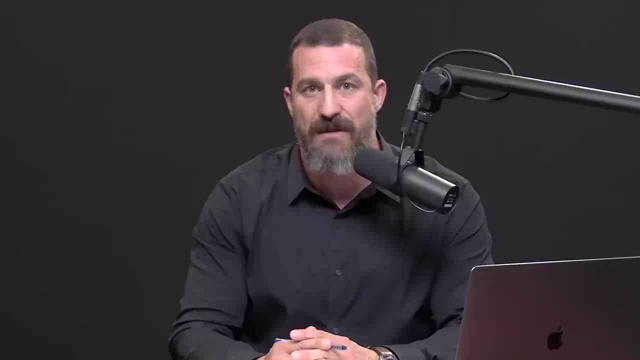 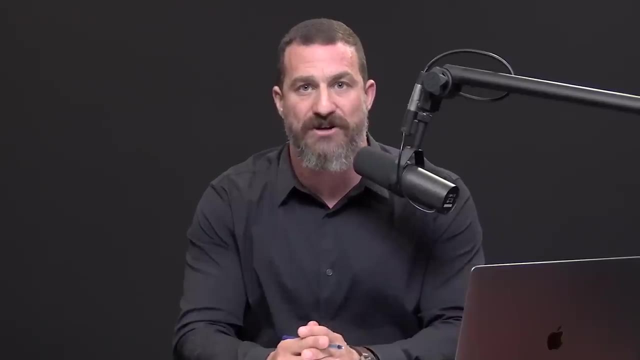 What I'm sure will become clear to you as you hear Lane talk about each and every one of these topics is that he has an incredible ability to both understand the mechanistic science but also the real world applications of the various discoveries that are made in particular papers. 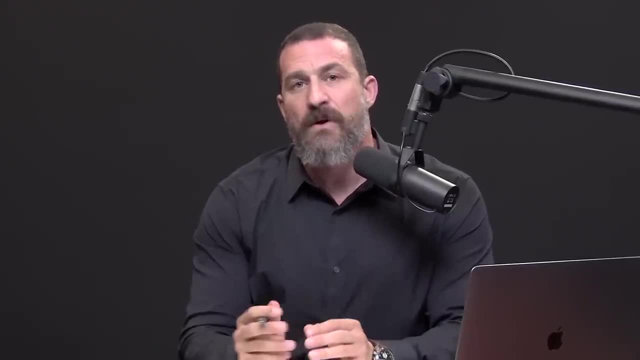 and in particular, in the randomized controlled trials, That is, when a given scientific hypothesis has been raised. he's extremely good at understanding why it was raised, but also at evaluating whether or not it works in the real world, which is what I believe most everybody out there. 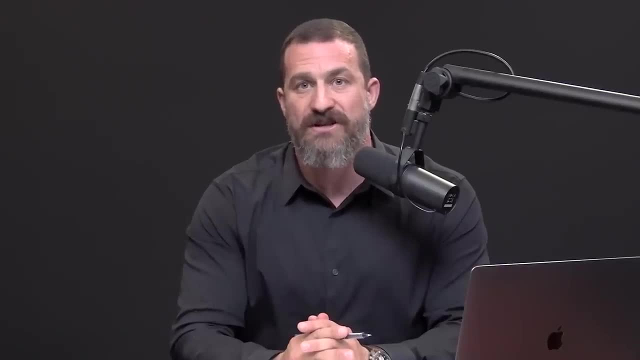 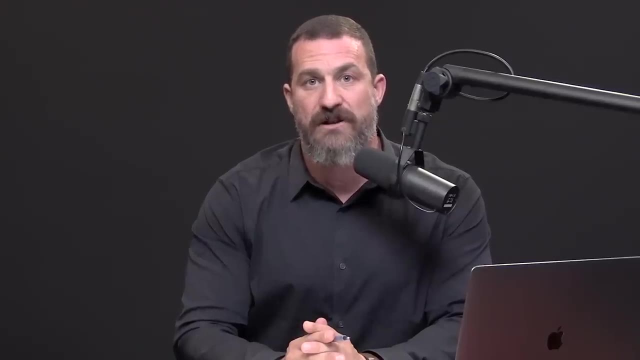 is concerned with. I think this is one of the things that really distinguishes him from the other voices in the nutritional landscape. I assure you that by the end of today's discussion, you will have a much clearer understanding about what the science says about nutrition. 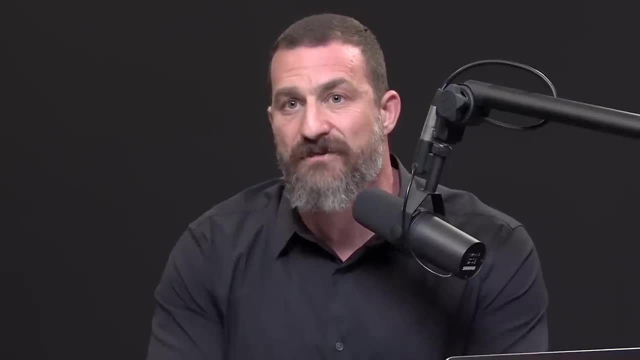 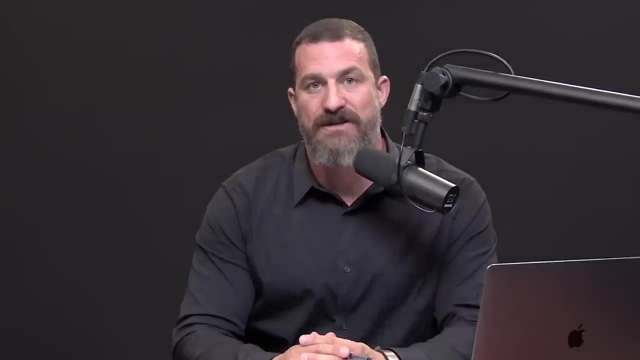 about fitness and about how different diets and fitness programs combine to achieve the results that you want. Before we begin, I'd like to emphasize that this podcast is brought to you by is separate from my teaching and research roles at Stanford. It is, however, part of my desire and effort. 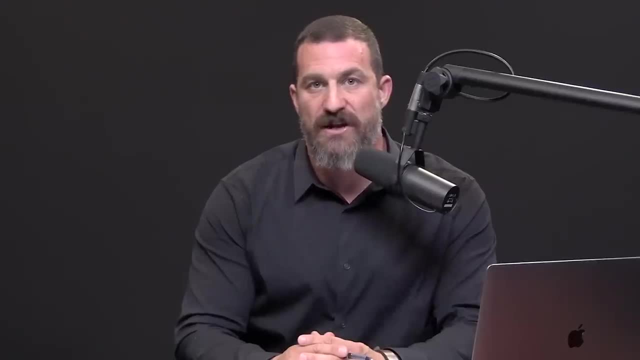 to bring zero cost to consumer information about science and science-related tools to the general public. In keeping with that theme, I'd like to thank the sponsors of today's podcast. Our first sponsor is Element. Element is an electrolyte drink with everything you need and nothing that you don't. 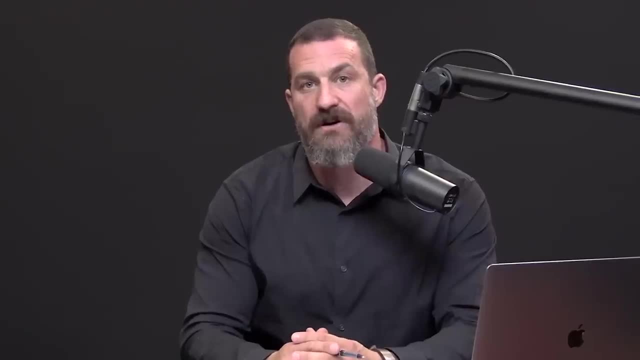 That means it contains sodium, potassium and magnesium- the so-called electrolytes, but no sugar, As you may have heard me discuss before on this podcast. every single day, every cell in our body and, in particular, cells within our brain. 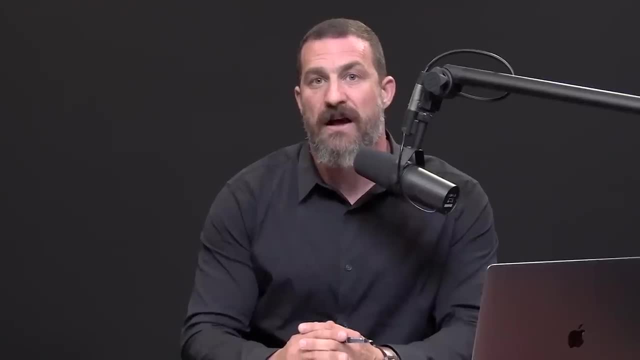 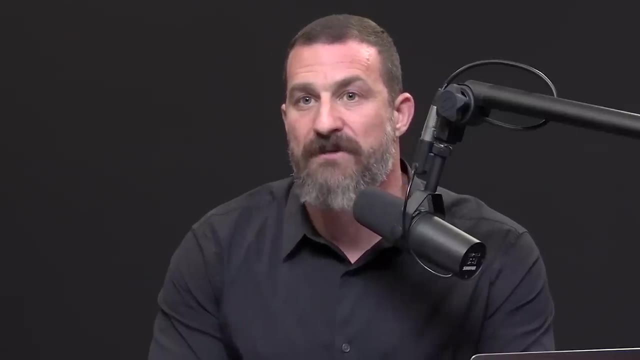 the so-called neurons, or nerve cells, critically rely on the presence of electrolytes- sodium, magnesium and potassium- in order to function properly. I myself am a big believer in consuming electrolytes anytime. I've been sweating a lot, So that could be after or during exercise. 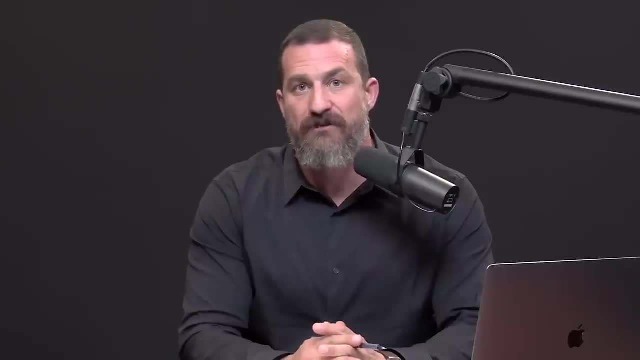 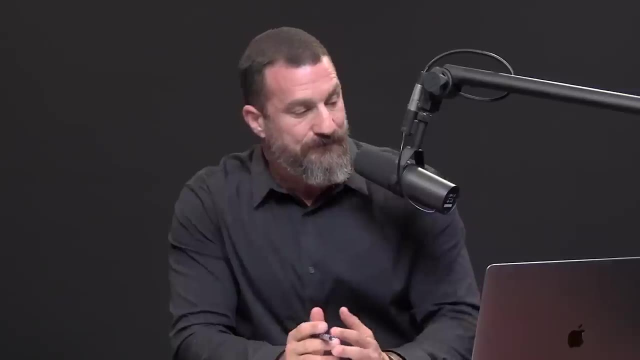 or after doing the sauna. So by drinking electrolytes in the form of Element electrolyte mix, I'm able to replenish those electrolytes and maintain mental clarity and energy throughout the day. Element contains a science-backed electrolyte ratio of 1,000 milligrams of sodium. 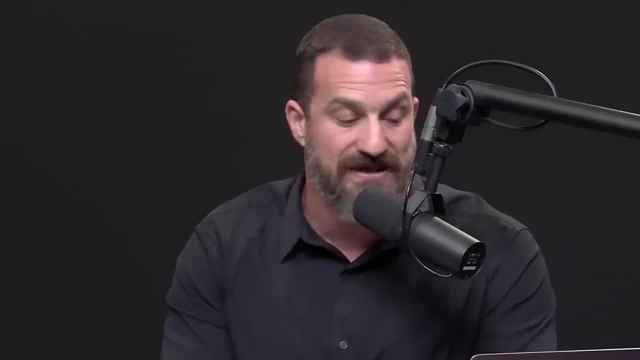 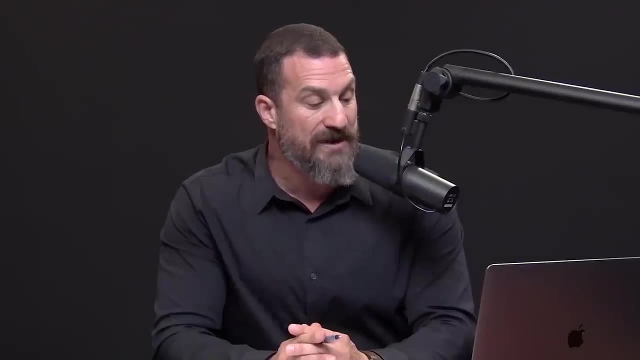 200 milligrams of potassium and 60 milligrams of magnesium. If you'd like to try Element, you can go to drinkelement spelled L-M-N-T dot com. slash Huberman to get a free sample pack with your purchase. 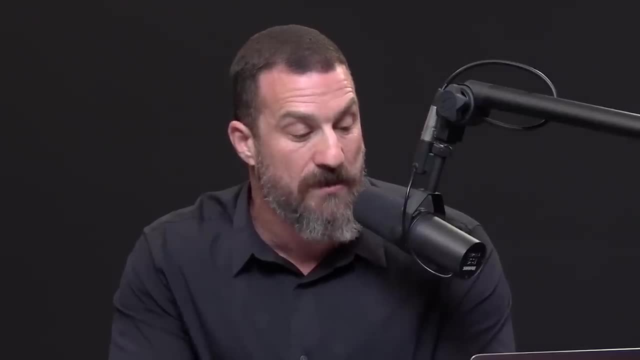 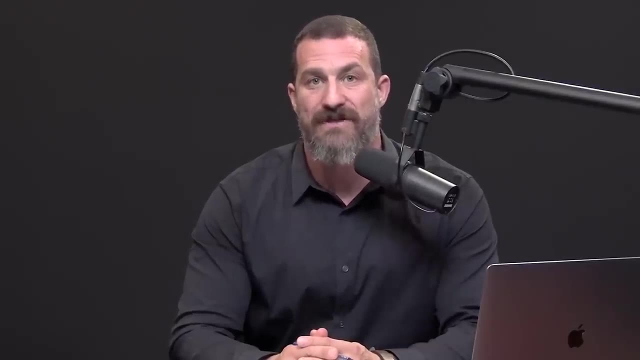 Again, that's drinkelementcom. slash Huberman to get the free sample pack. Today's episode is also brought to us by Roka. Roka makes eyeglasses and sunglasses that are the absolute highest quality. The company was founded by two all-American swimmers. 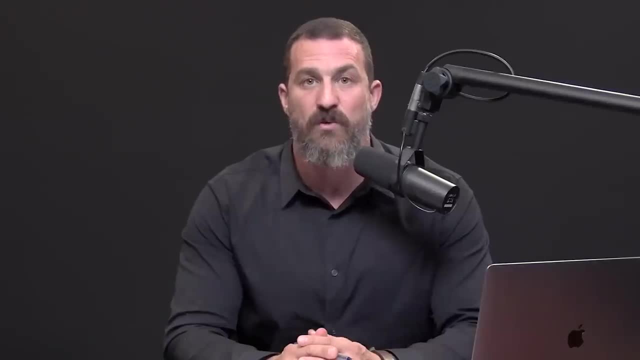 from Stanford, and everything about Roka eyeglasses and sunglasses were designed with performance in mind. I've spent a lifetime working on the biology, the visual system, and I can tell you that your visual system has to contend with an enormous number of challenges. 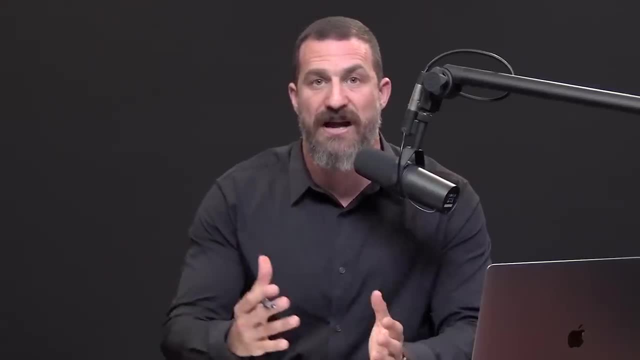 in order for you to see clearly, For instance when you move from a sunny area to a shady area and back again, whether or not you're looking at something up, close or off into the distance. Roka understands the biology of the visual system. 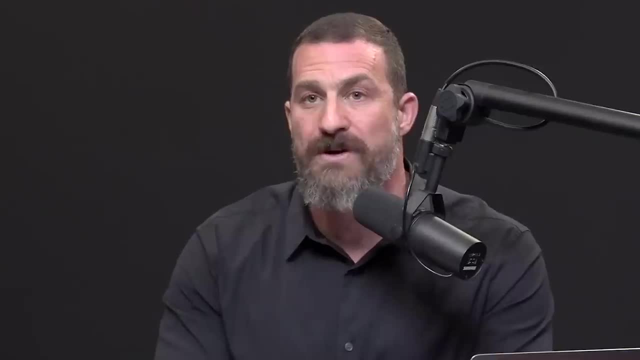 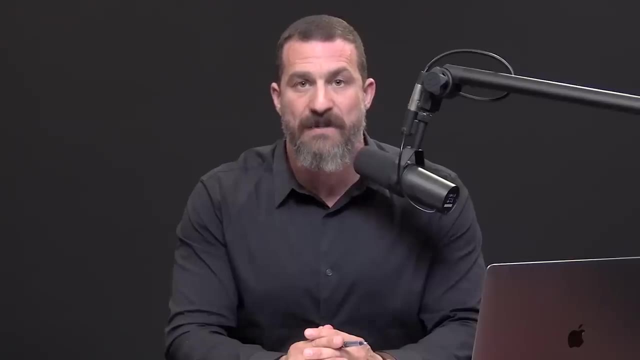 and has designed their eyeglasses and sunglasses accordingly, so that you always see with perfect clarity. Roka eyeglasses and sunglasses were initially designed for people with vision problems, for activities such as running and cycling, and indeed they are very lightweight. 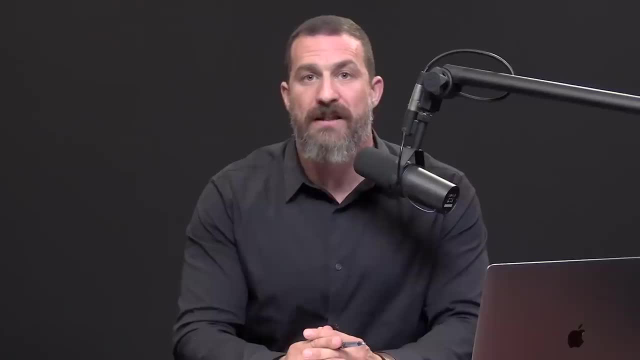 Most of the time I can't even remember that they're on my face. They're so lightweight. But the important thing to know about Roka eyeglasses and sunglasses is that, while they can be used during sports activities, they also have a terrific aesthetic. 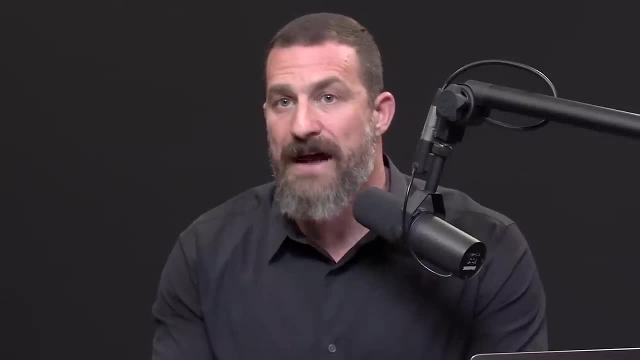 and they can be used just as well for wearing to work or out to dinner, et cetera. If you'd like to try Roka eyeglasses and sunglasses, you can go to Roka. that's R-O-K-Acom. 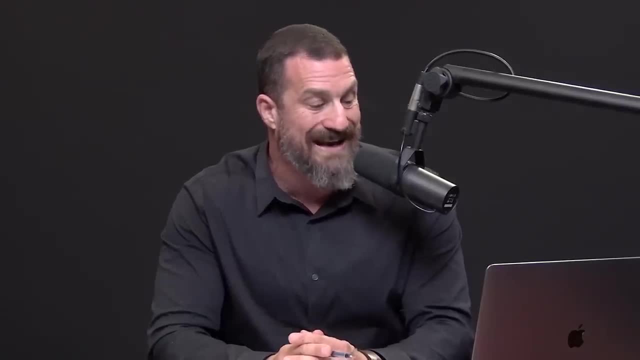 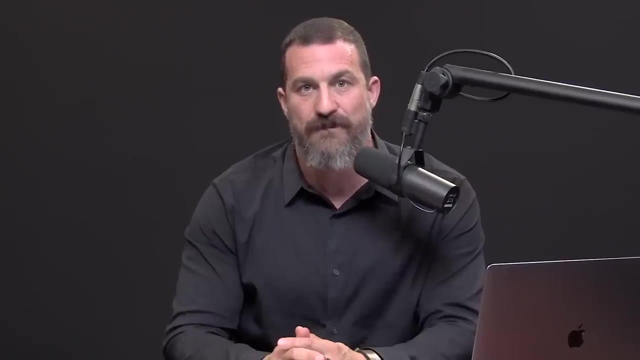 and enter the code Huberman to save 20% off on your first order. Again, that's R-O-K-Acom. Again, that's Roka, R-O-K-Acom. and enter the code Huberman at checkout. Today's episode is also brought to us by InsideTracker. 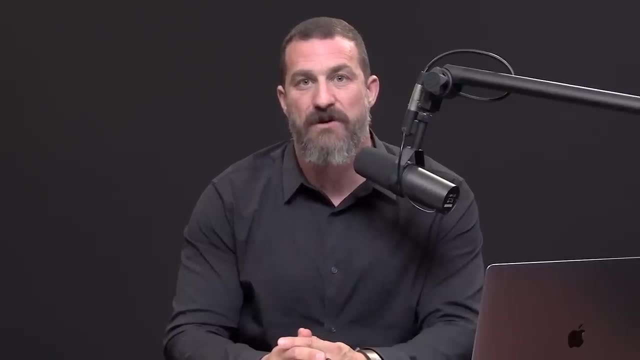 InsideTracker is a personalized nutrition program that analyzes data from your blood and DNA to help you better understand your body and help you reach your health goals. Now, I've long been a believer in getting regular blood work done, for the simple reason that many of the factors 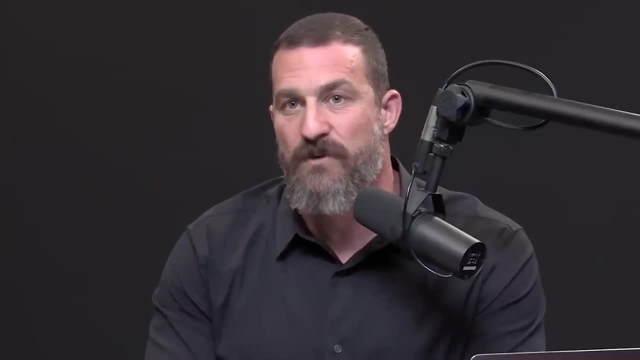 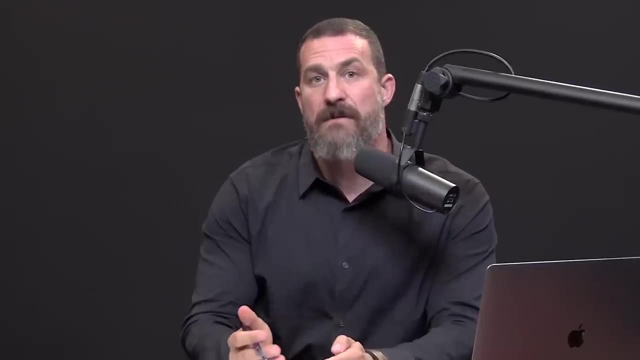 that impact your immediate and long-term health can only be analyzed with a quality blood test. One of the major issues with a lot of blood and DNA tests out there, however, is that you get information back about levels of hormones, levels of lipids. 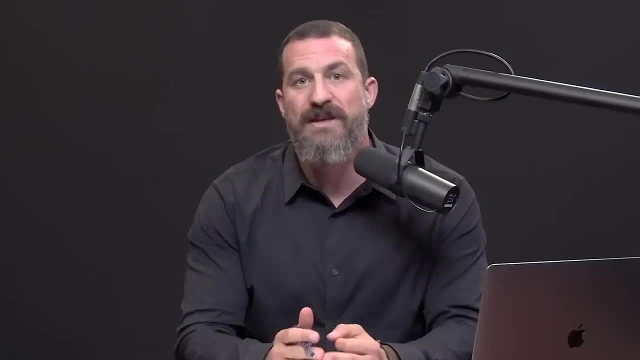 levels of metabolic factors, but you don't know what to do about that information. With InsideTracker, they have a easy-to-use platform that allows you to assess those levels and then determine what sorts of behavioral changes, nutritional changes, maybe even supplementation changes, you might want to make. 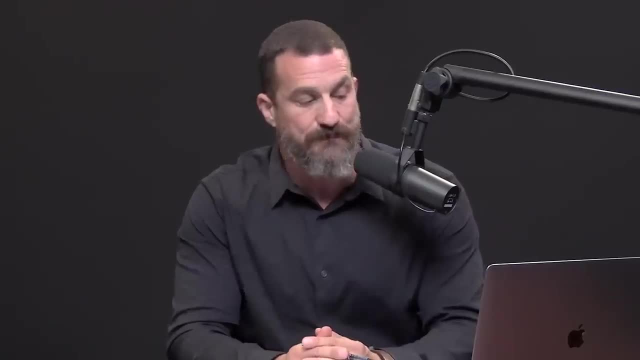 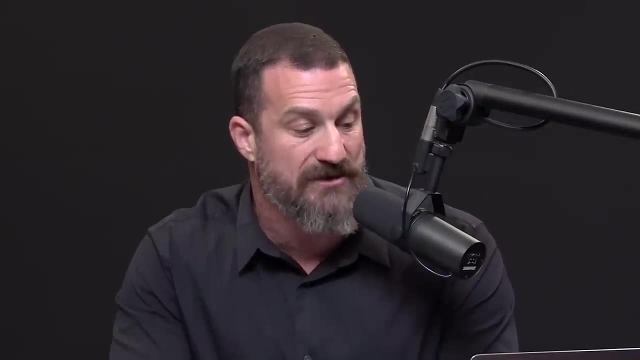 in order to bring those numbers into the ranges that are optimal for you. If you'd like to try InsideTracker, you can go to InsideTrackercom slash Huberman to get 20% off any of InsideTracker's products. Again, that's InsideTrackercom slash Huberman. 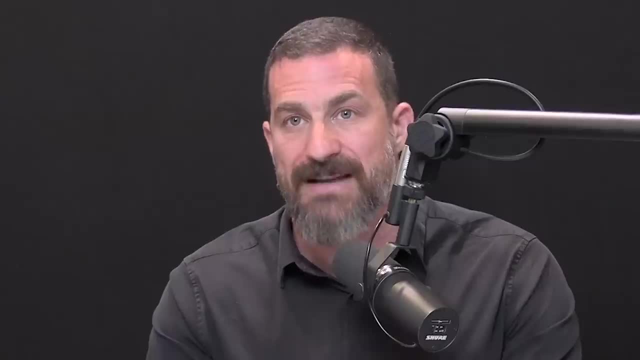 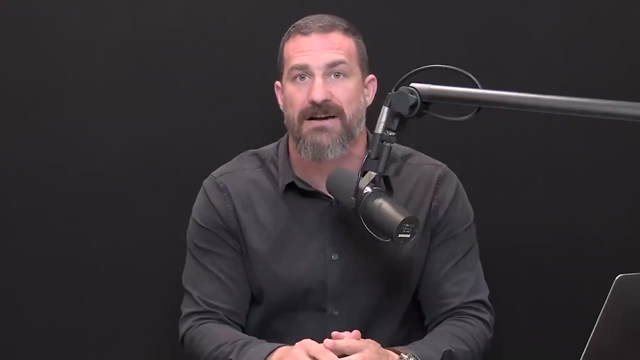 to get 20% off. The Huberman Lab Podcast is now partnered with Momentous Supplements. To find the supplements we discuss on the Huberman Lab Podcast, you can go to LiveMomentous spelled O-U-S: LiveMomentouscom- slash Huberman. 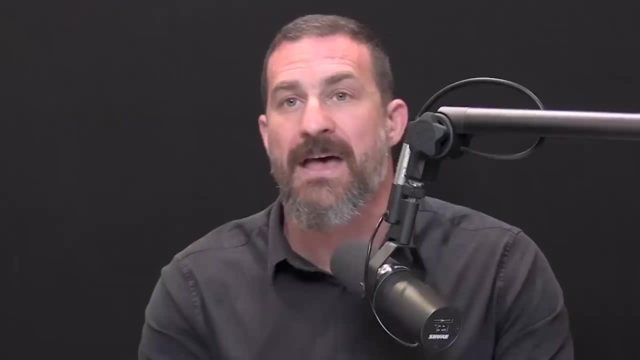 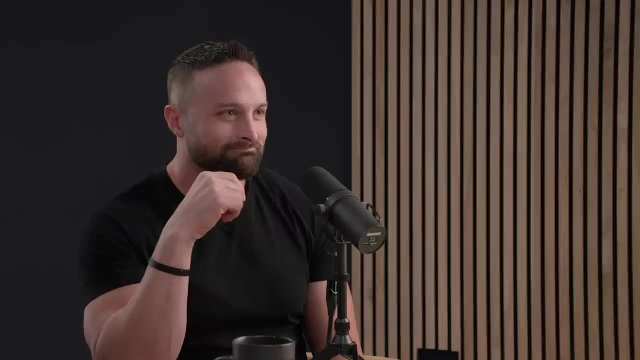 And I should just mention that the library of those supplements is constantly expanding. Again, that's LiveMomentouscom, slash Huberman. And now for my discussion with Dr Lane Norton. Lane, Dr Norton, thank you so much for being here. 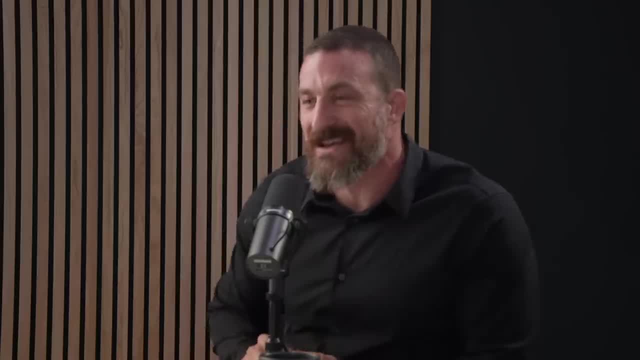 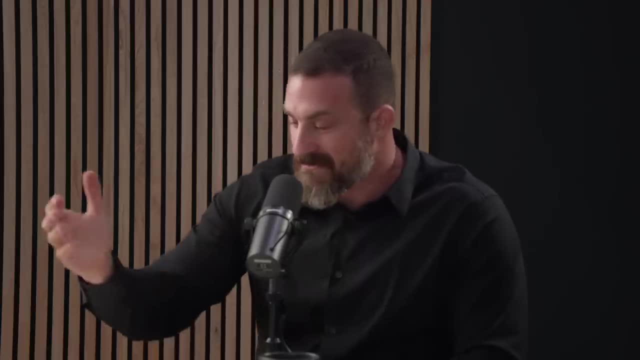 This is a long time coming and I have to say I'm really excited because I've seen you in the social media sphere. I've also listened to a number of your other podcasts And, as a fellow PhD scientist, I feel a great kinship with you. 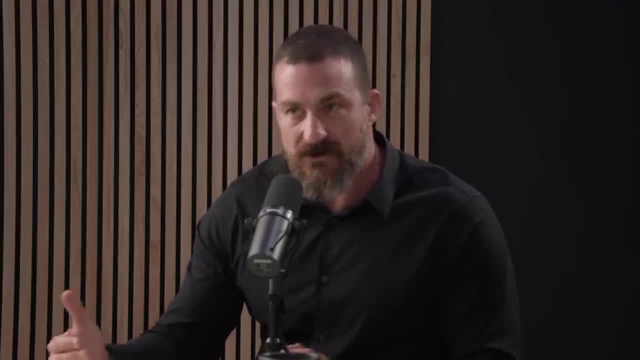 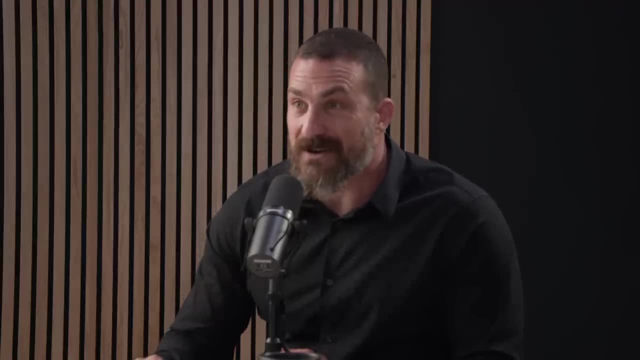 I know you have tremendous experience in fitness and nutrition- a number of areas. We also got a lot of questions from our audience and I'm really looking forward to talking with you today. Yeah, I'm excited too. I mean, like you said, 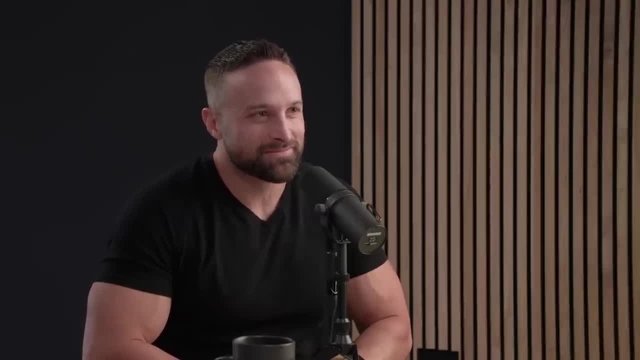 it's been something we've been talking about for a long time, so I was glad we were able to make it happen. Yeah, indeed Indeed, And I think some of the audience has requested a debate or a battle, and I can tell you right now. 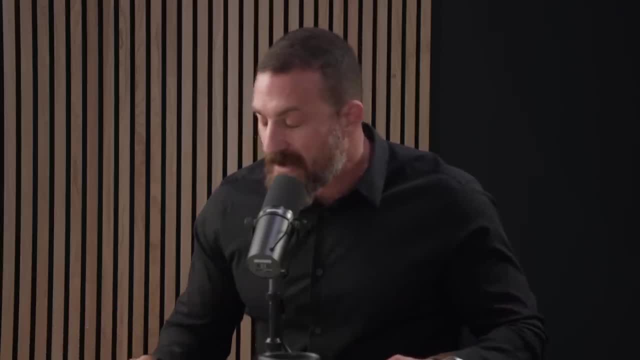 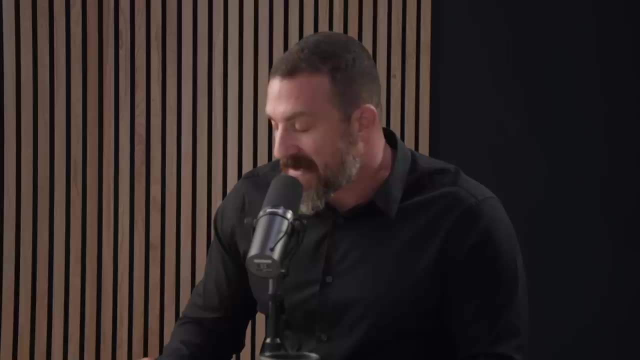 it's not going to happen. Actually, one of the things that brought Lane and I together in conversation online and then via text, et cetera, was the fact that I love to be corrected, And that's what happened. I did a post about artificial sweeteners. 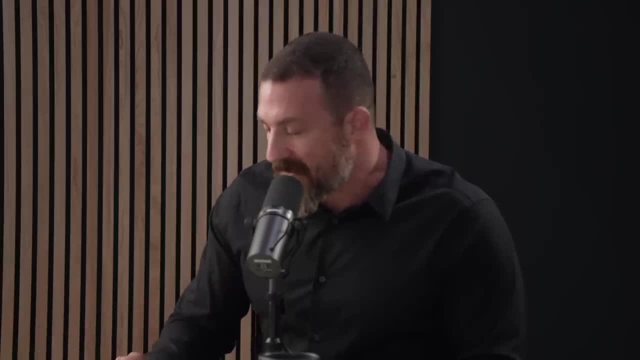 which we will talk about a little bit later in the episode, And Lane pointed out some areas of the study that I had missed out on. We did a post about artificial sweeteners, which we will talk about a little bit later in the episode. 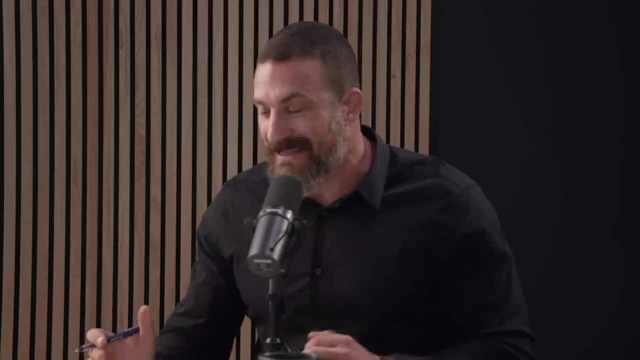 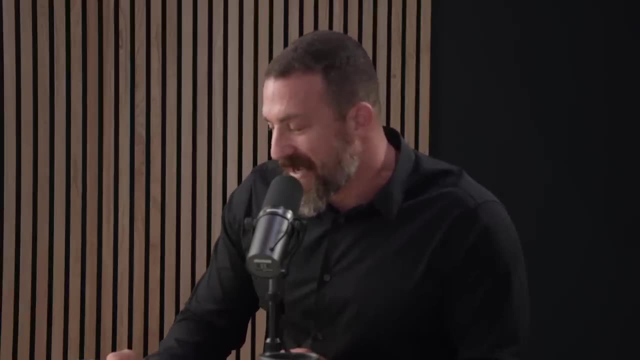 Or maybe even misunderstood, And I revised my opinions and I think it's wonderful, And other studies have come out since then, So hopefully our conversation will serve as a message of how science and actionable science can be perceived and that it doesn't always have to be a battle. 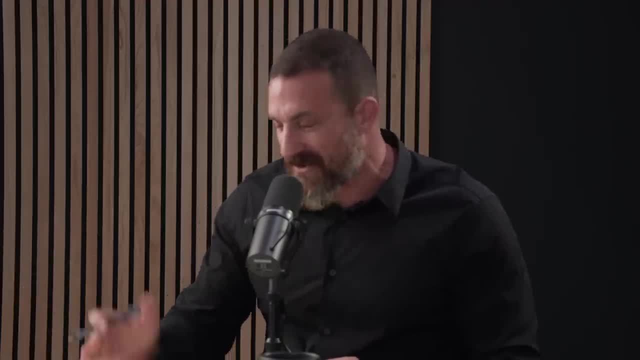 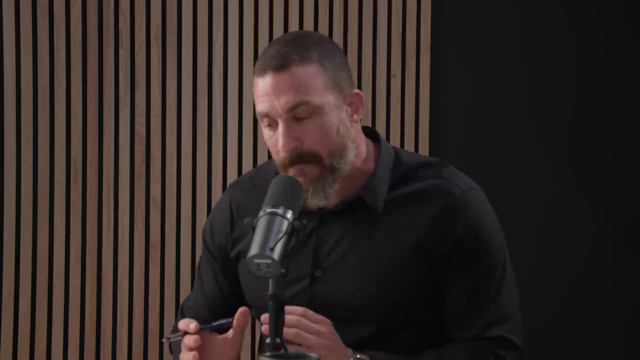 But hey, if we get into it, we get into it. It won't get physical because we know you would win In any case. I'd like to start with something that's rather basic and yet um can be pretty complex, um, and that's this issue of energy, balance and energy. 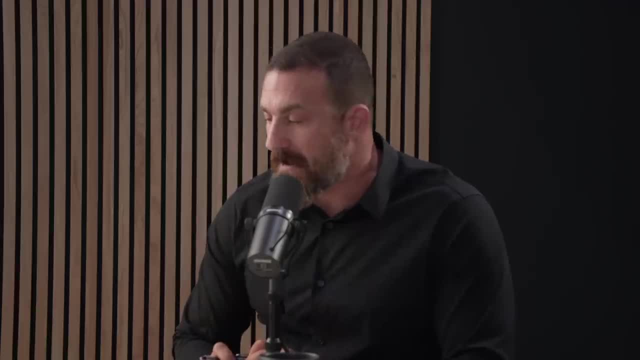 utilization. i think most people have heard of a calorie. um, i i'm assuming that most people don't actually know what that is in terms of how it works, what it represents, and so maybe you could just explain for people what happens when we eat food of any kind, and how is that actually converted? 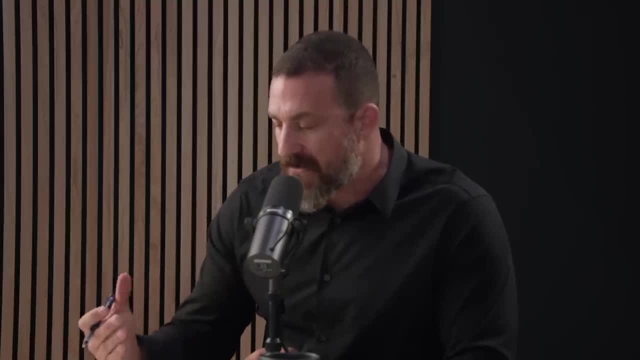 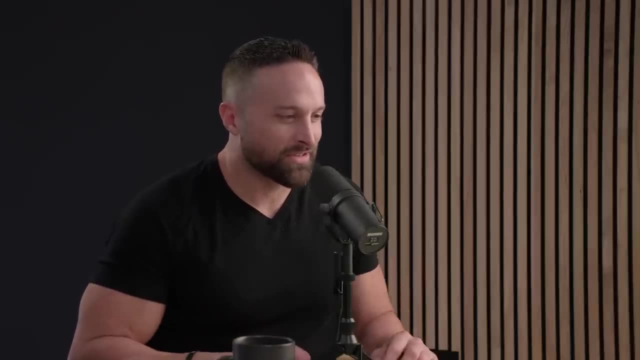 into energy as a way of framing up the discussion around weight loss, weight maintenance, weight gain and body composition. it's a great question and, like you said, this is one of those things where you know people use the term calories in, calories out and they say, well, that's way too simplistic. 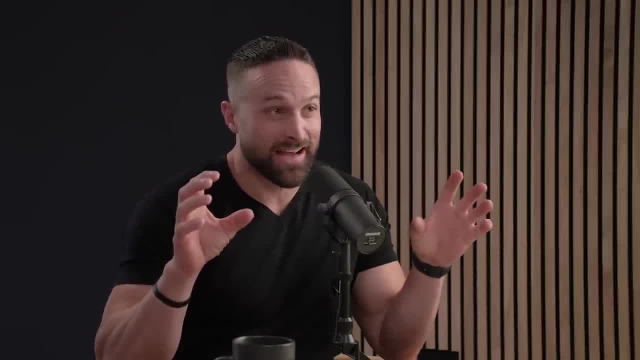 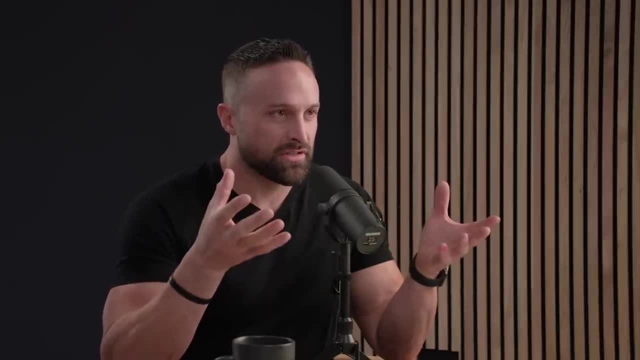 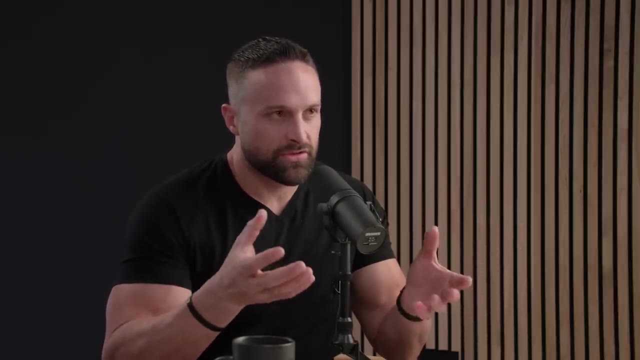 and i'm like, if you look at what actually makes up calories in calories out, it's actually very complicated, right? so let's deal with the uh, what you mentioned first. what is a calorie? because i think a lot of people don't quite understand this. so a calorie just refers to a unit of energy, of heat specifically. 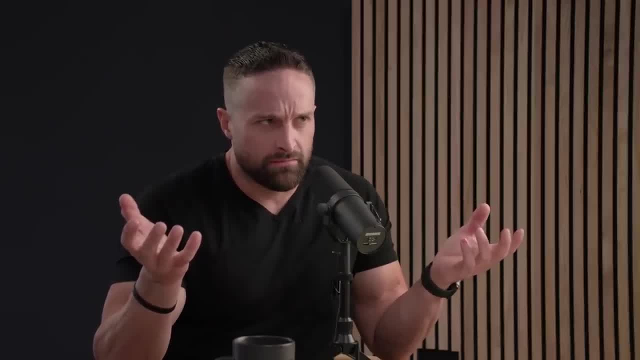 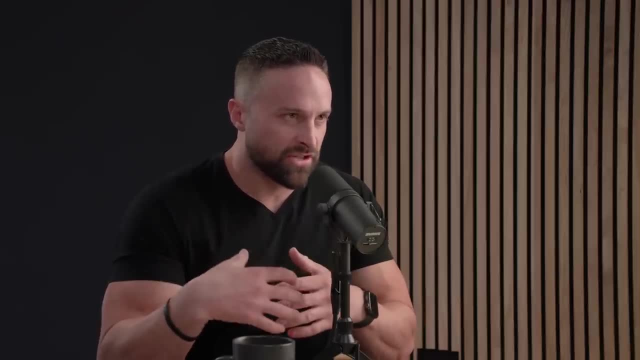 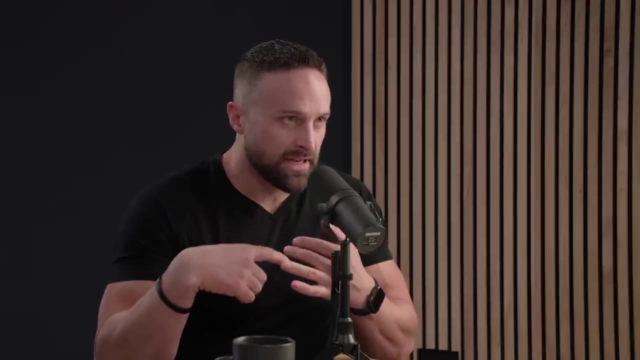 and so what does that have to do with food? what does that have to do with, like, what we digest and eat? really, what you're talking about is the potential chemical energy that is in the bonds of the macronutrients of food right and by digesting, assimilating and metabolizing those nutrients. 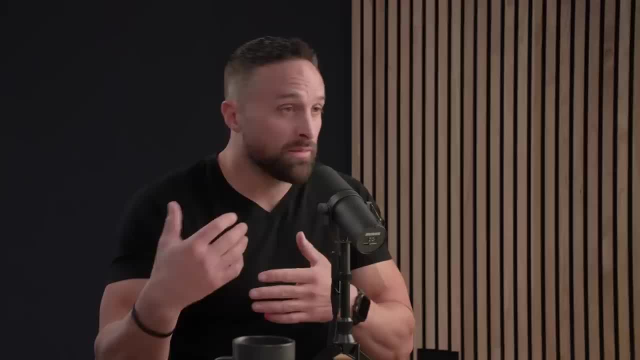 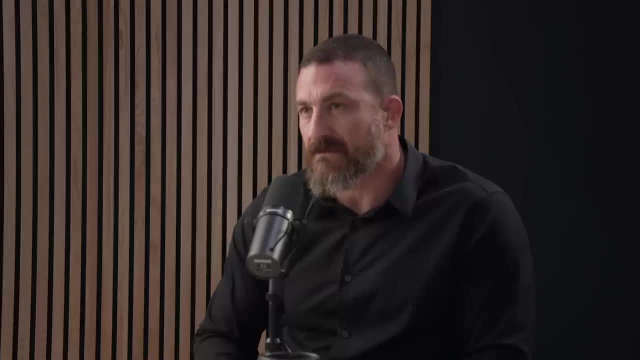 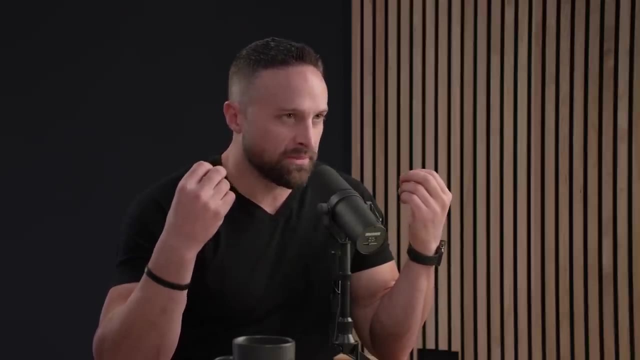 we are able to create energy and the end product of that mostly is atp, um, adenosine triphosphate, which is your body's energy currency. so, to understand atp, just try to think about if you're trying to power these various reactions in your body, and we're talking about tens of thousands of enzymes that require atp. 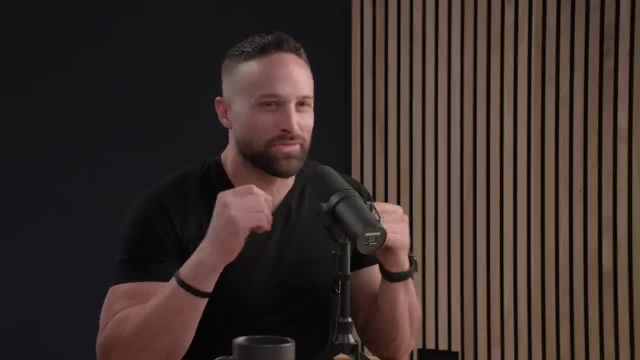 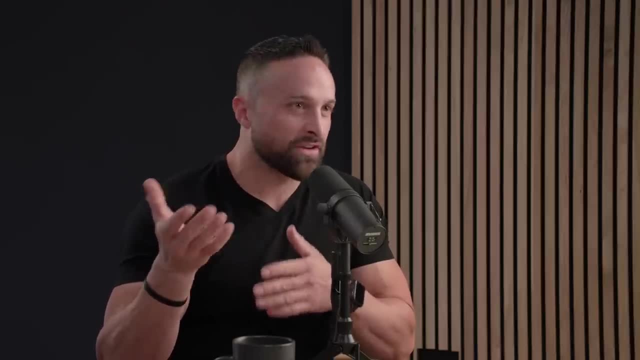 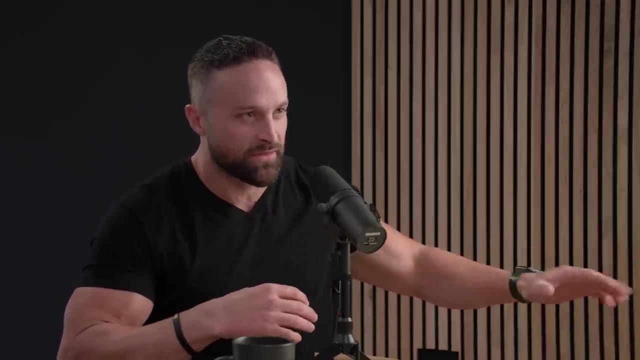 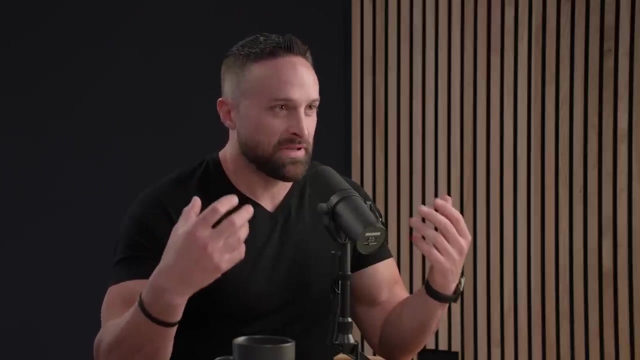 um, you know, it doesn't make sense that you would have to create a bunch of micro explosions, right? you want something that can transfer high energy phosphates to power these reactions, to give up essentially its energy, to power something that might otherwise be unfavorable. so a lot of metabolism is simply creating atp, which the end of the line of that i'm going to. 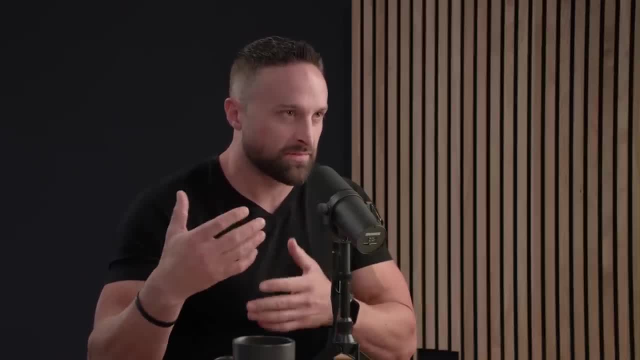 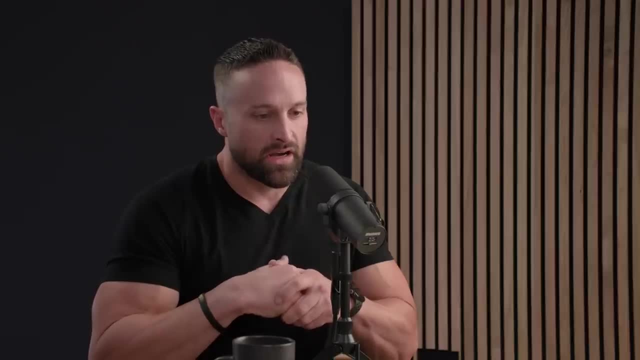 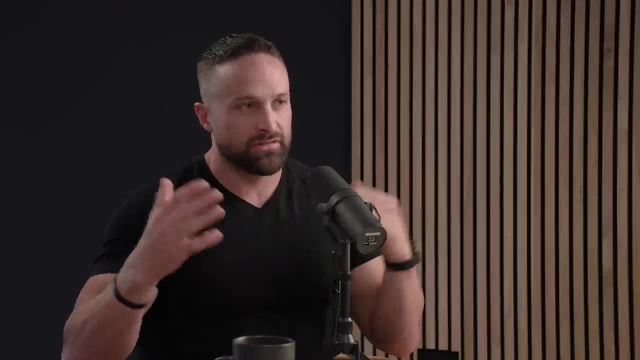 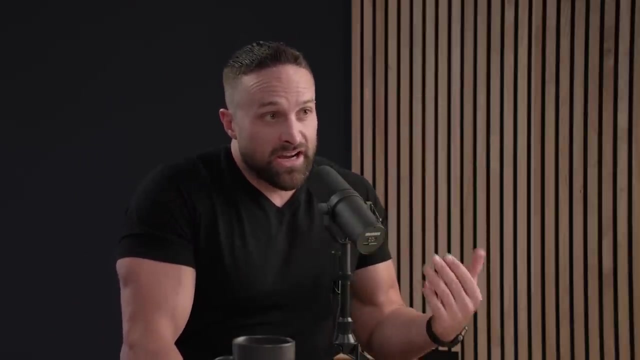 kind of work backwards is what's called oxidative respiration. so that happens in the mitochondria- everybody's heard mitochondria, powerhouse of the cell. and that is done, uh, through essentially creating a hydrogen ion gradient across the mitochondria which powers the production of atp, by converting free phosphate plus adp to atp. now the way that hydrogen ion gradient is created, is through- uh, you know, creating hydrogen, hydrogen ions that can be donated through the krebs cycle. now, the krebs cycle is linked to glycolysis, so if we talk about carbohydrate metabolism, carbohydrates basically other than fructose, get converted into glucose, which can go into glycolysis, and you can produce some atps through. glycolysis and then it boils down to pyruvate. then acetyl-coa, which goes through the krebs cycle, produces a lot more atps from that. if you talk about protein, protein's a little bit different because protein gets converted to amino acids which can be used for muscle protein synthesis. or protein synthesis and other tissues, but it also can be converted through gluconeogenesis to glucose, and there also are some ketogenic amino acids as well, and so you can have a few different ways to get to the krebs cycle, either being through acetyl-coa or through glucose going. through the glycolysis to pyruvate. then you have fatty acids which are able to create energy through what's called beta oxidation, where essentially you're taking these fatty acids and you're lopping them off two carbons at a time to produce acetyl-coa, which again can go into the 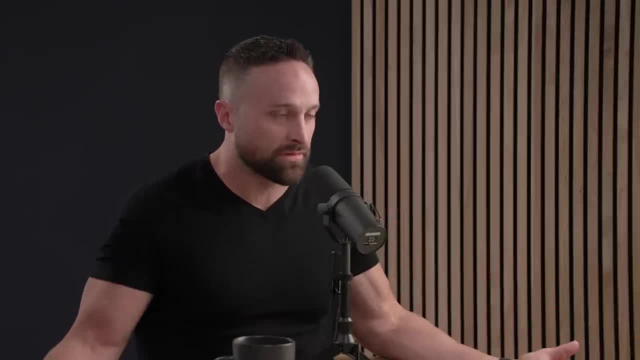 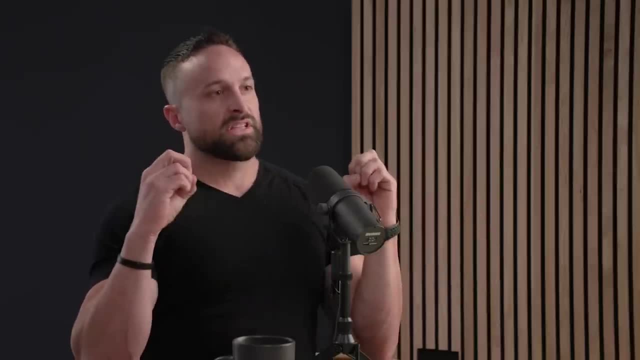 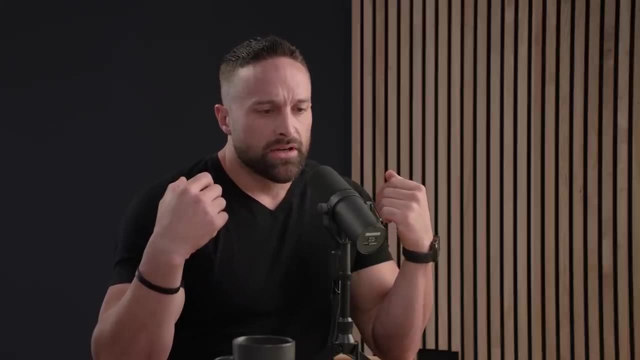 krebs cycle produce those hydrodynes that can then power the production of atp. so that's kind of like at the cellular level of how this stuff works. but stepping back and taking it back out like what does that have to do with weight loss or weight gain? right well, when you think about the balance, 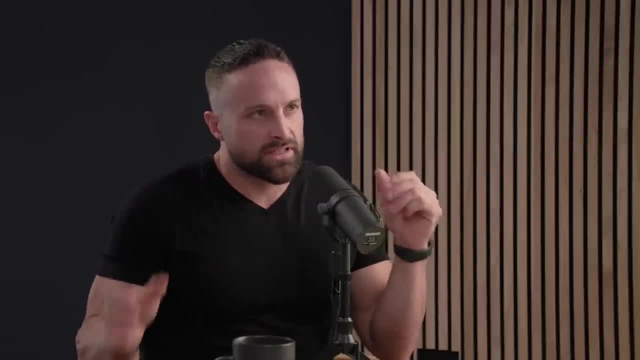 of energy in versus energy out. you're going to have to go through a lot of different things, so sounds very simple, but let's look at what actually makes up energy in versus energy out. first of all, you've got to realize that the energy inside of the equation 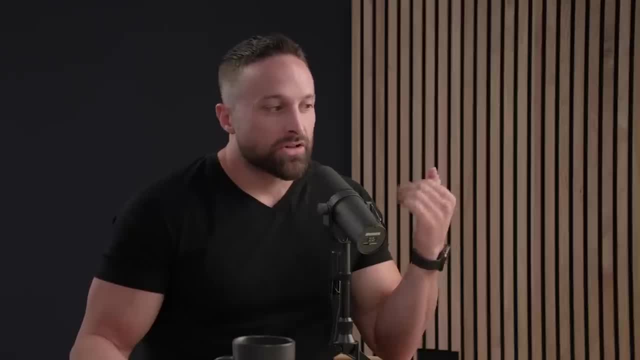 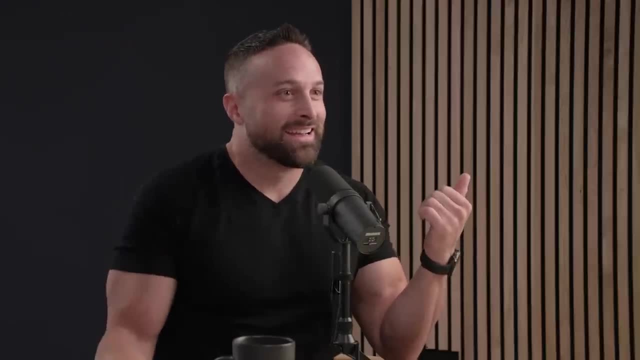 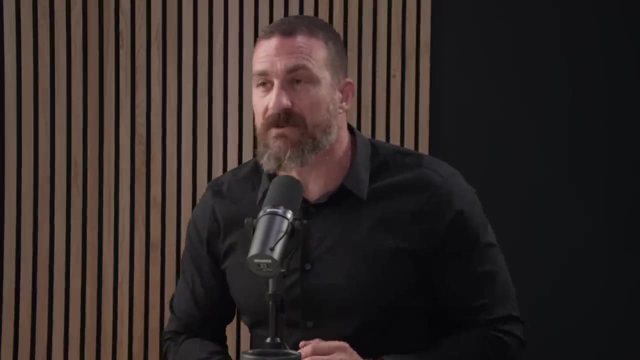 is more difficult to track than people think, right. so one uh food labels, which we like to think is being, you know, like from upon high uh can have up to a 20 error in them really. oh yeah, so 100 calorie is something listed as 100 calories per serving it could, what's actually in there, could be. 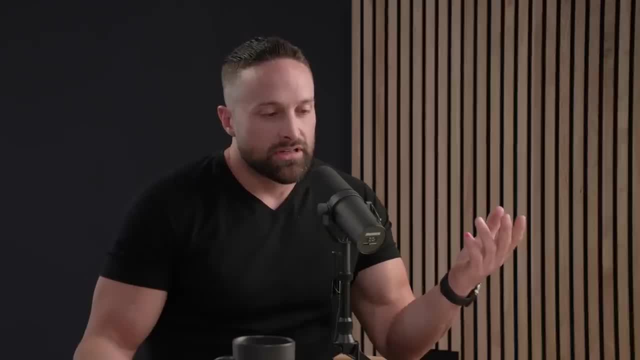 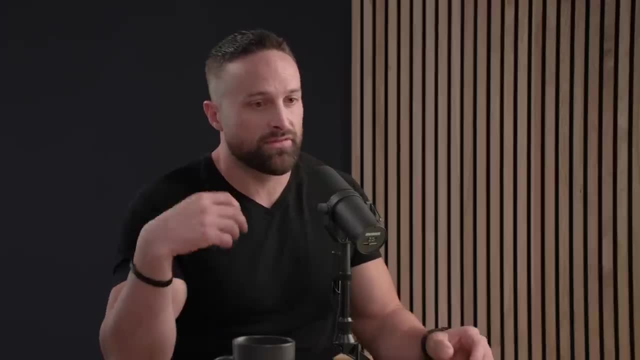 or 120.. right, exactly, so that's one aspect of it. the second aspect is there's what's called your energy, but then there's also metabolizable energy, right? so if you have uh food stuff with, say, a lot of insoluble fiber, typically insoluble fiber is not really digestible and 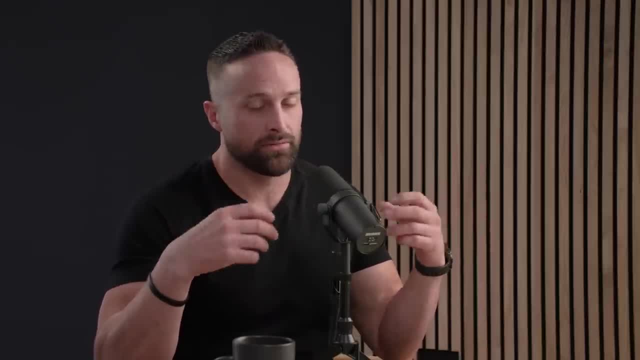 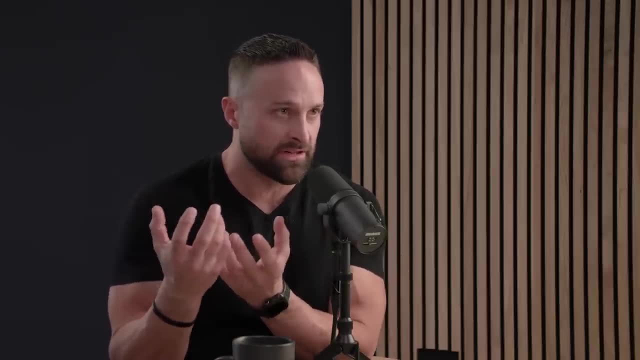 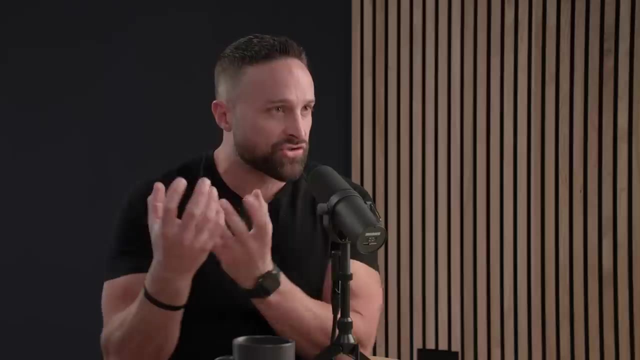 so you could have, you know, quite a bit of carbohydrate, you know, but if you can't extract the energy from it, and typically this is because insoluble fiber from like plant material, the carbohydrate or and even some of the protein, is bound up in the uh plant structure, which makes it inaccessible. 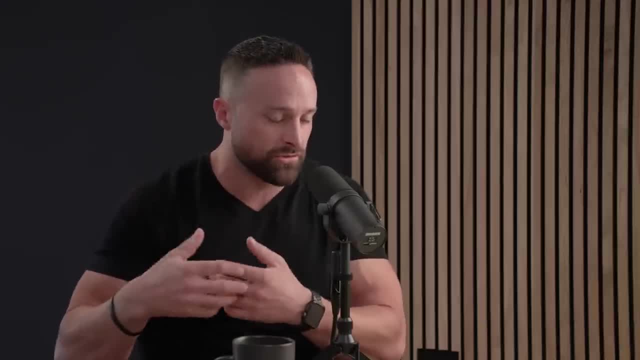 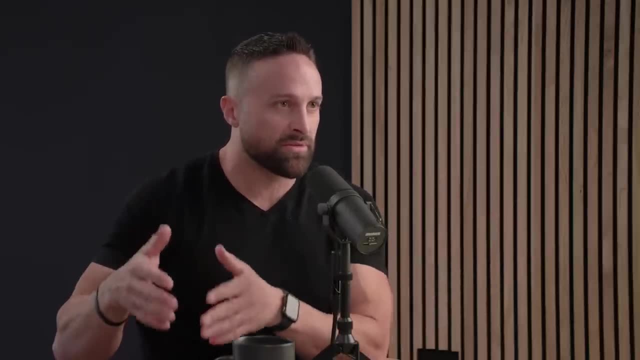 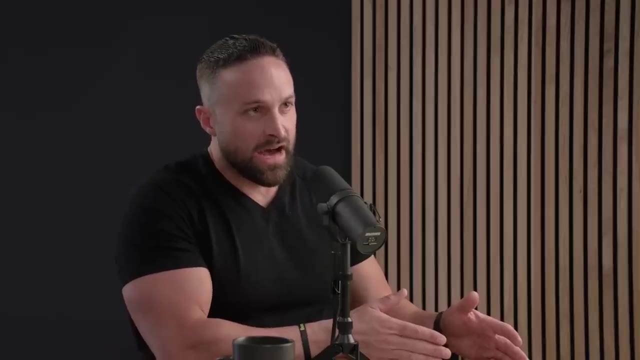 to digestive enzymes, and so this is what like adds bulk to your school stool and whatnot, but again reduces the metabolizable energy in there, and there's some evidence that, based on people's individual gut microbiome, that some people may actually be better at extracting energy out of fiber compared to other people. so just starting off right, 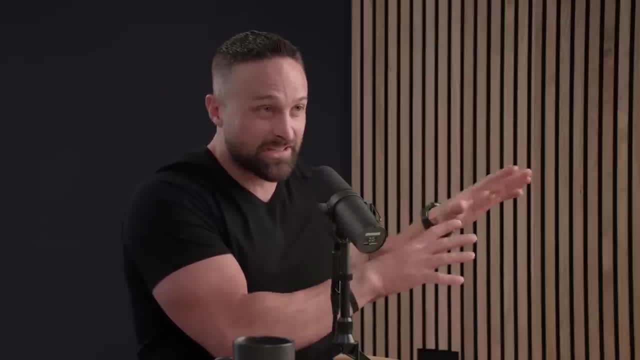 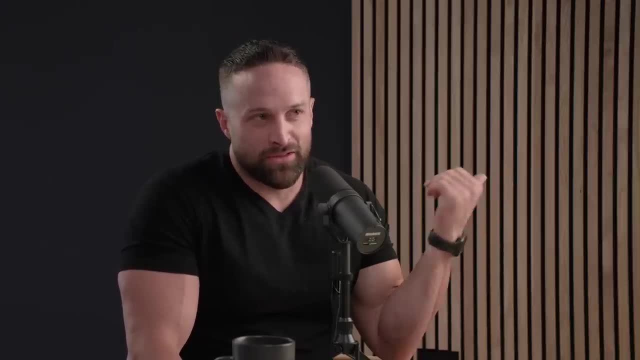 there. okay there's. there's quite a bit of play in the energy inside of things. now one of the things people will say is: well see, that's why you shouldn't worry about tracking calories, because you know if the food labels can be 20 off and what i'll say is: okay, that's a. 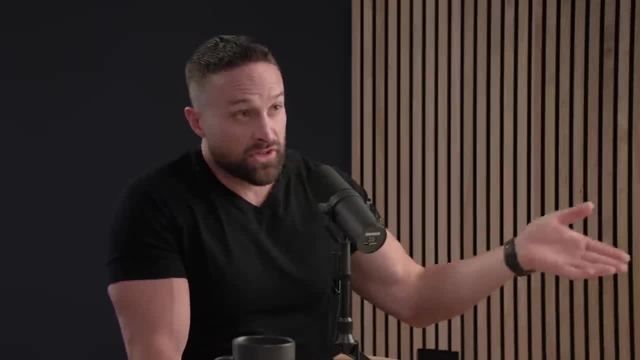 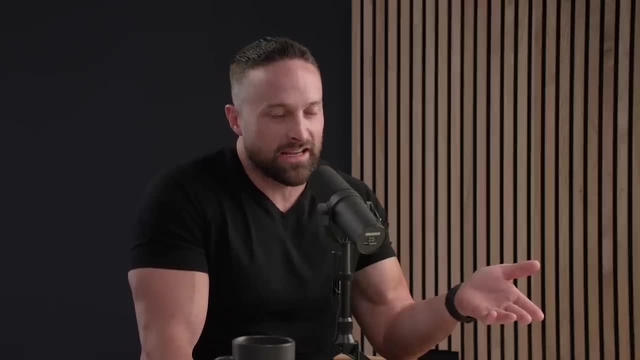 that's, i understand where you're coming from, but typically if it's off it's going to be consistently off and if you're consistent with how you track it, eventually you'll be able to know, kind of what you're taking in. and it's kind of that's kind of like saying, well, don't worry about. 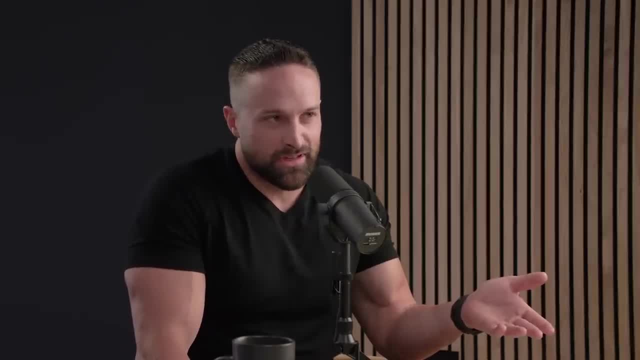 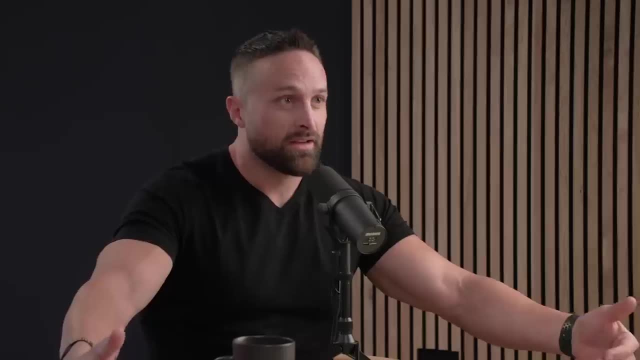 tracking. you know, if you're. i like to use financial um examples. you know, we know, that to save money or you have to earn more money than you spend. well, you can't exactly know how much money you're earning at a time. you know, because there's inflation and then there's uh, if you have. 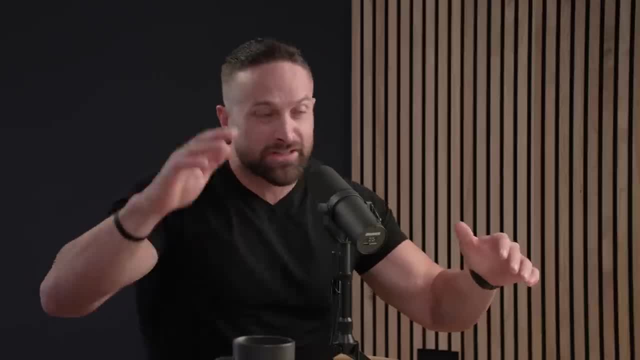 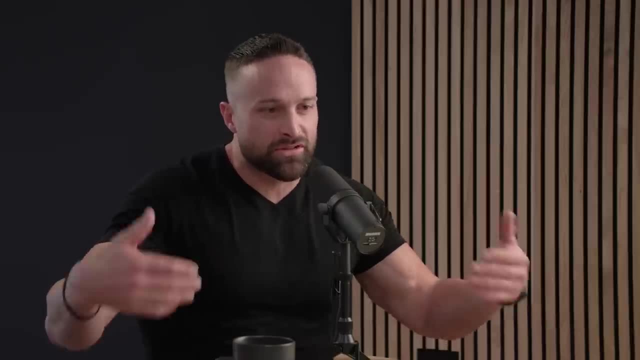 investments. those can be. you know different interest rates and whatnot- say okay, but you're, you know. if you have a budget, you have a reasonable idea of what it's going to be. you know and you make. you make certain assumptions, but you can relatively get a lot of money out of it and that's a good example, right. so now let's look at the energy. 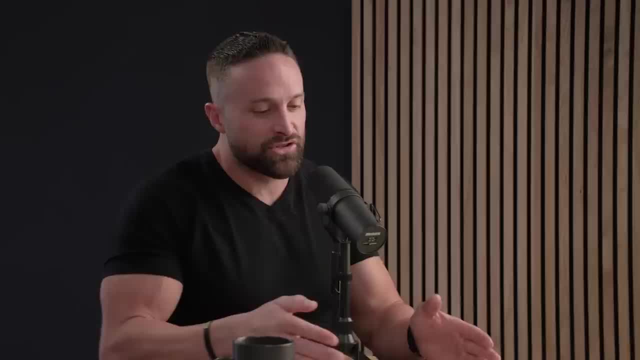 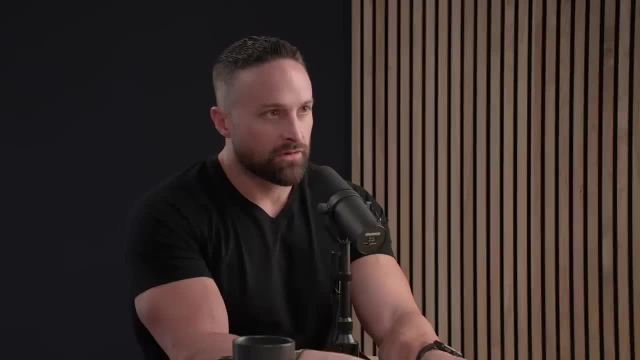 outside of the equation, which is actually way more complicated. right, and so your energy out is a few different uh buckets. the first one, and the biggest one, is your resting metabolic rate, so your rmr, and that, for most people, is anywhere from 50 to 70 percent of your. 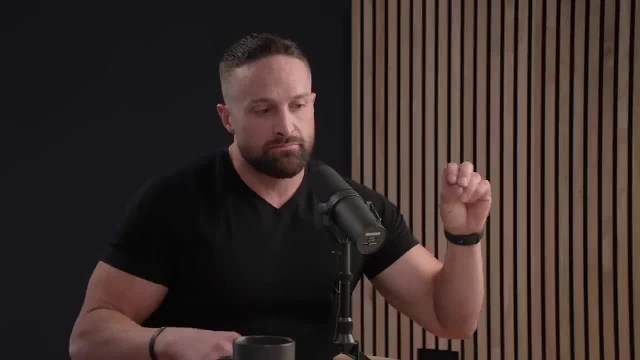 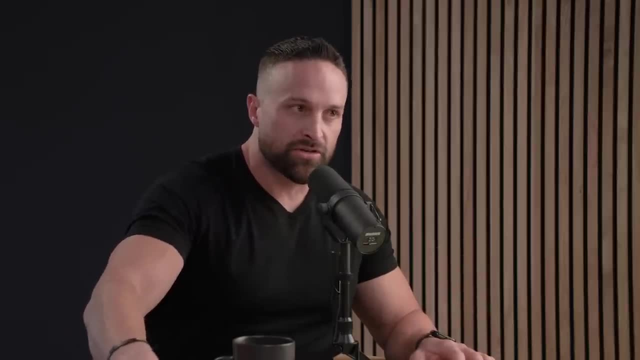 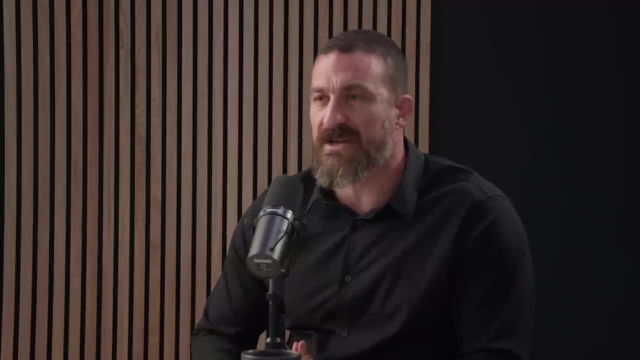 total daily energy expenditure. now people use the term metabolic rate and energy expenditure kind of interchangeably, but they're not the same thing. so your total daily energy expenditure is the summation of all the energy you expend in a day walking upstairs exercise- if you do it fidgeting, yeah, plus your resting metabolic rate, right. so resting metabolic rate is a big part of that, but it's not the only thing. so that's usually about 50 to 70 percent, and sedentary people will be on the higher end of that, so it'll be a bigger proportion, whereas people who are more active it'll be a little bit. 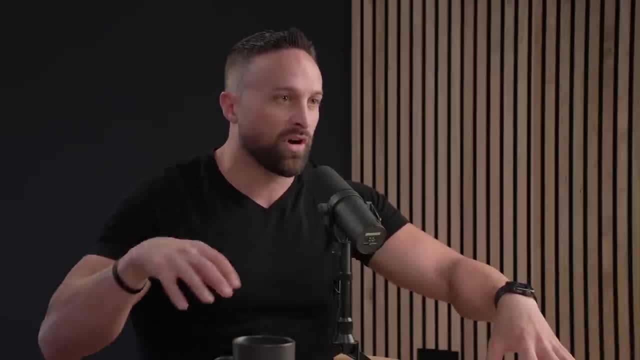 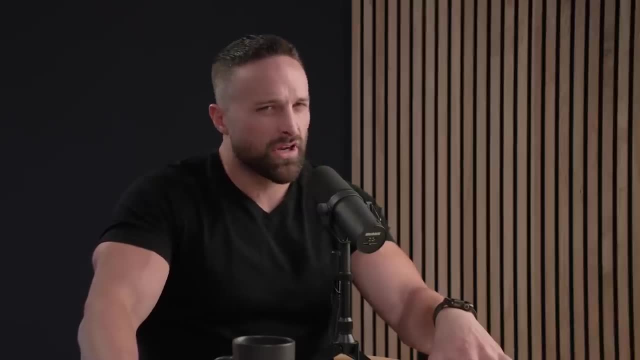 lower, not because their metabolic rate is lower, but because they're expending a greater percentage of their calories from physical activity. then you have something called the thermic effect of food, which is a relatively small percentage of your total daily energy expenditure. it's about five to ten percent, uh, and very difficult to measure, and usually what researchers do when they're. 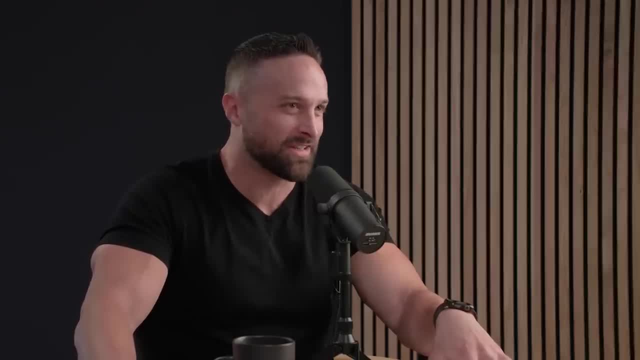 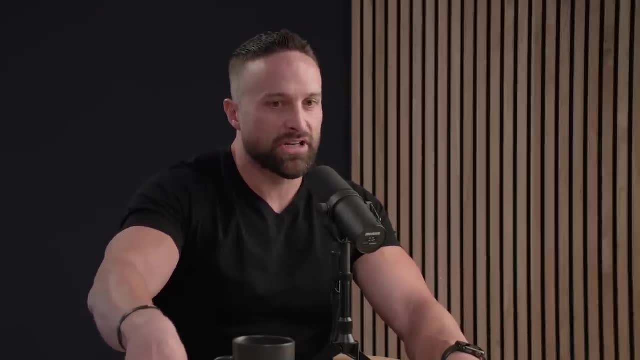 kind of looking at this stuff is. they just kind of make an assumption about it. they use a constant, but that's about five to ten percent of your daily energy expenditure and that refers to the amount of energy it takes to extract the energy out of food. so think about your body. 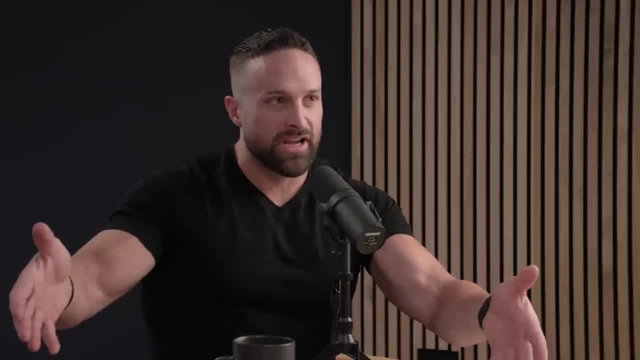 what's the amount of energy it takes to extract the energy out of food. so think about your body. you don't just have gas in your tank and it spontaneously starts up, right like you have to have a battery, so you put in energy so you can get the energy out of the petrol that you. 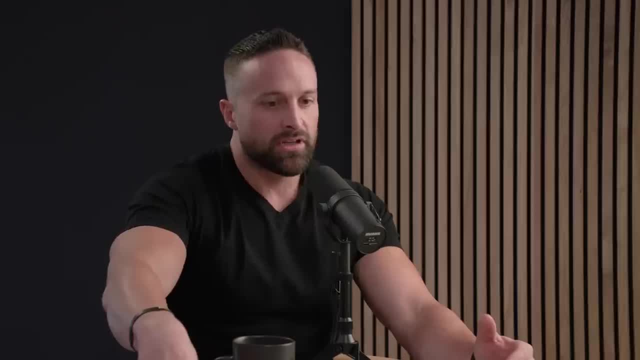 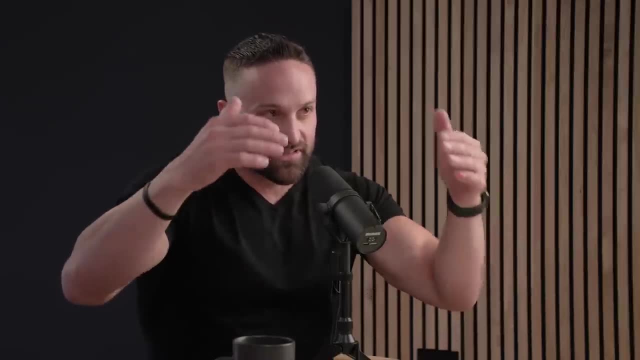 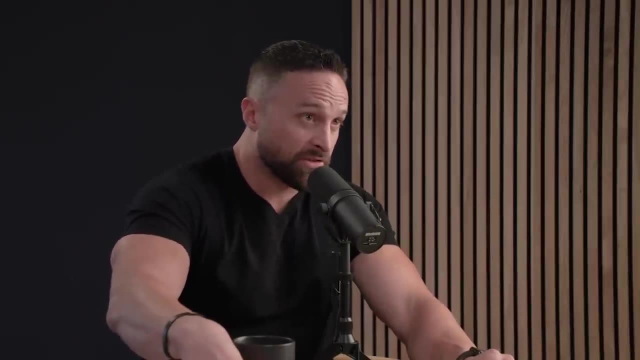 have in your car. similar with with food. you can't just eat food and then you know it just appears in your cells and you start doing stuff. it has to be systematically broken down and put into forms that can actually produce energy, and so you have to put some energy in to achieve that. and 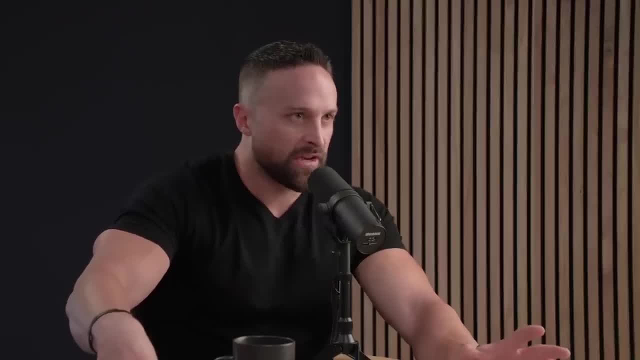 a lot of times people will say something like: well, not all calories are created equal. that's not true, because calories just a unit of measurement, right? that would be like saying not all seconds on a clock are created equal. yes, they are. all sources of calories may have differential 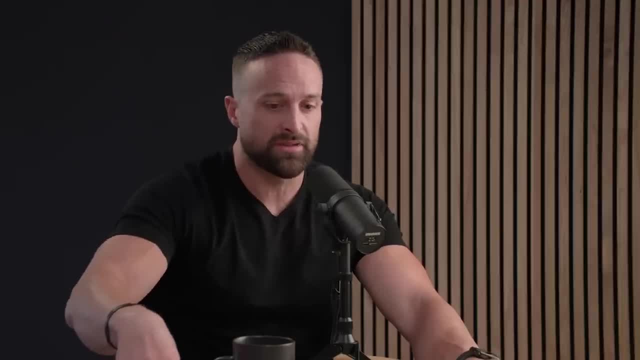 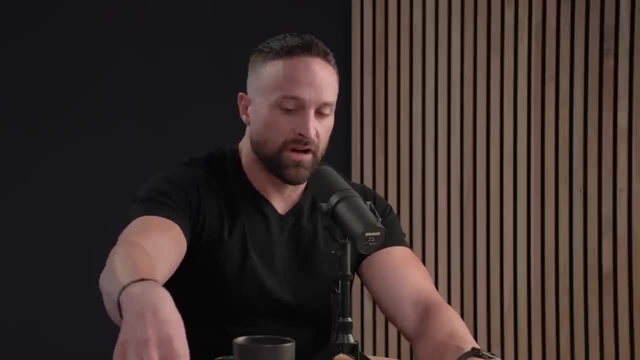 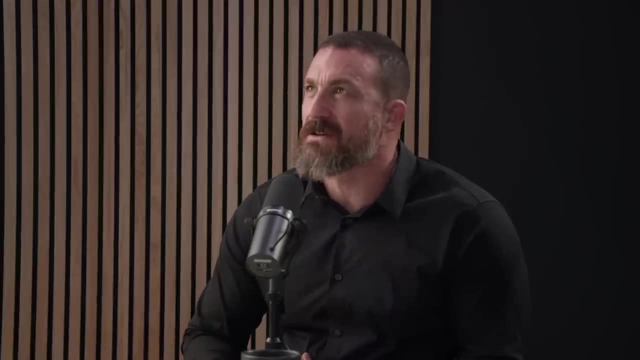 effects on energy expenditure and appetite. so if we look at something like um fat, for example, the tef of fat is about zero to three percent, meaning if you eat 100 calories from fat, your net is 100. so the process of breaking down that fat essentially subtracts some of the the calories. 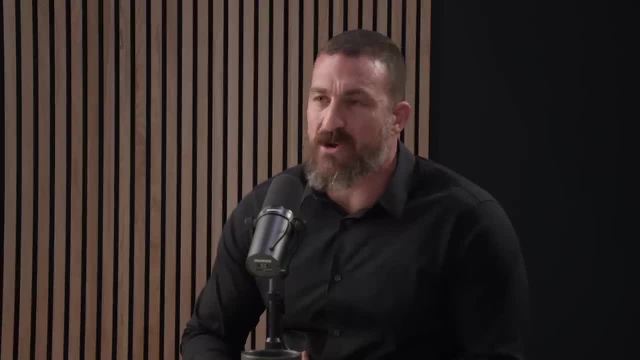 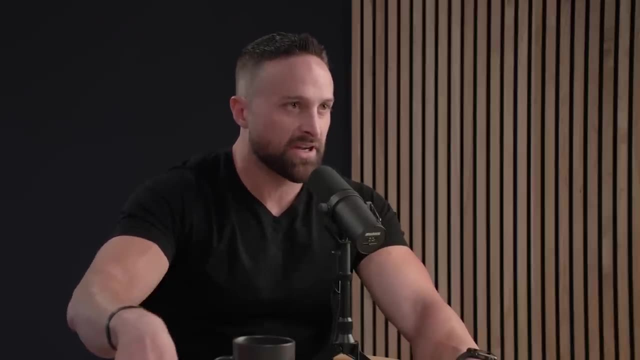 away because you used it in creating energy by breaking those chemical bonds to create atp, correct, okay, correct. so you have, like, for example, some enzymes that require atp to run these processes. now, fat is actually the easiest thing to convert into energy. then you have carbohydrate, which has a tf of like five to ten percent, so you eat 100 calories from. 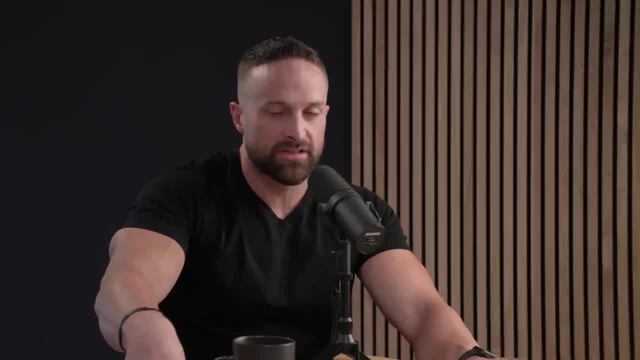 carbohydrate and obviously, like the fiber, content makes a big difference on this. you eat 100 calories, you'll net 90 to 95.. protein is about a 20 to 30 percent tef. so if you eat 100 calories from protein, you're only netting 70 to 80.. now you're still net. you know people say well. 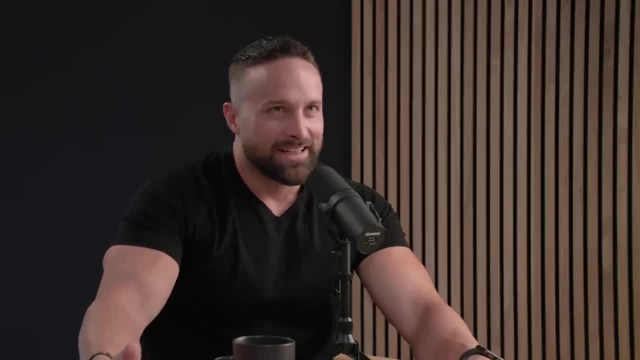 you can't eat too much protein. well, you know people will ask: well, can protein be stored as fat, the carbons from protein? it's unlikely. it's going to wind up in adipose tissue. but if you're eating a lot of protein overall as part of a lot of calories, it does. it has to be oxidized. 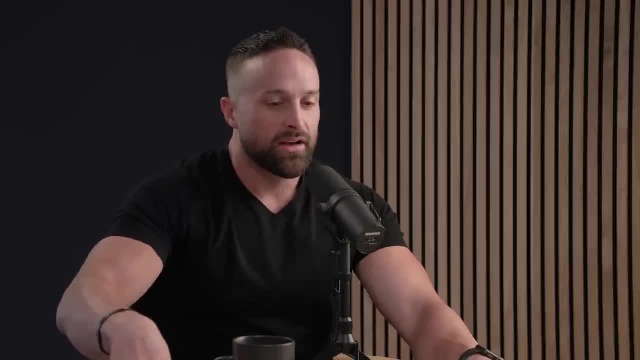 and it can provide a calorie cushion for other things to be stored in fat. but protein itself does provide, you know, a net positive for calories, but less so than carbohydrate or fat and tends to be more satiating. so again, when people talk about, you know, are all calories. 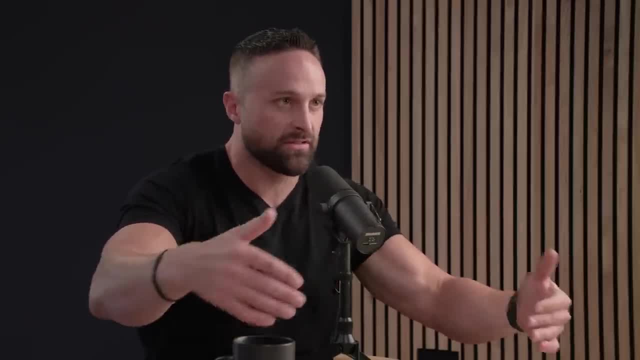 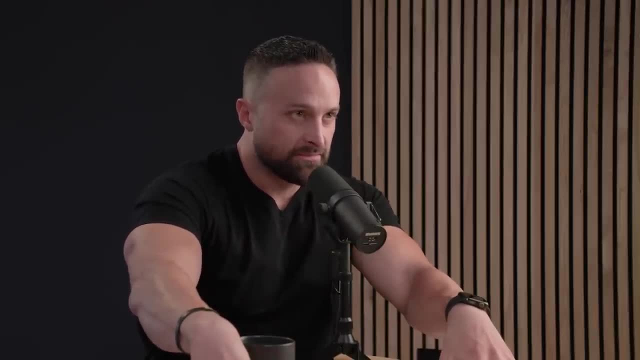 created equal, yes, but all sources of calories may have differential effects on energy expenditure and appetite. so that's the tef bucket and the bmr bucket. then we go to physical activity, and physical activity is essentially two parts. there's exercise, which is kind of your purposeful movements, like you. 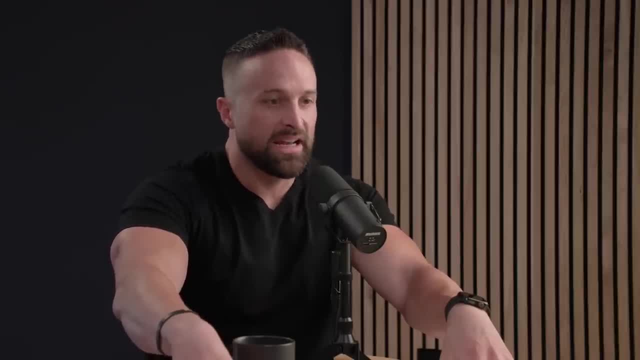 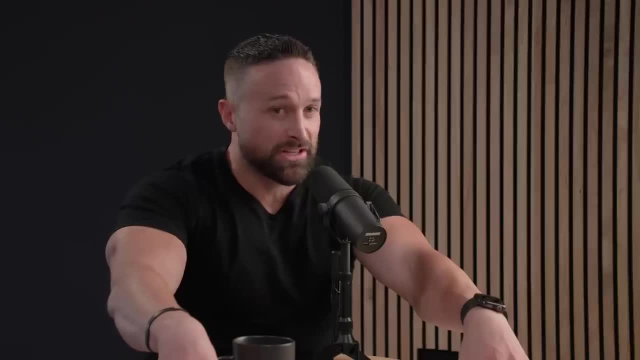 walk, you do a training session, i mean whatever, any purposeful activity, and then you have what's called neat, which is non-exercise activity, thermogenesis, which i think is actually really cool. it's fascinating. yeah, it is. so it's. i was actually hanging out with somebody last night and 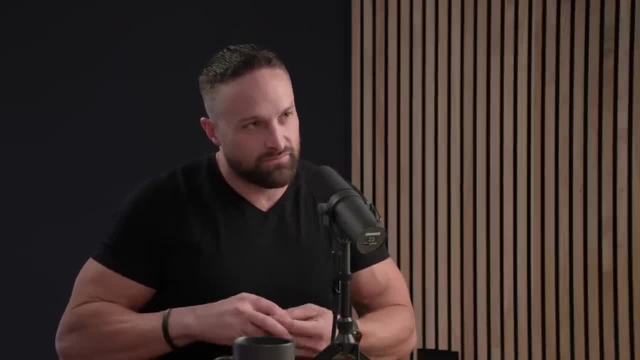 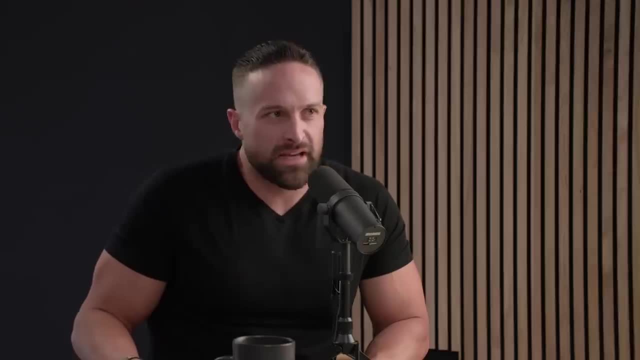 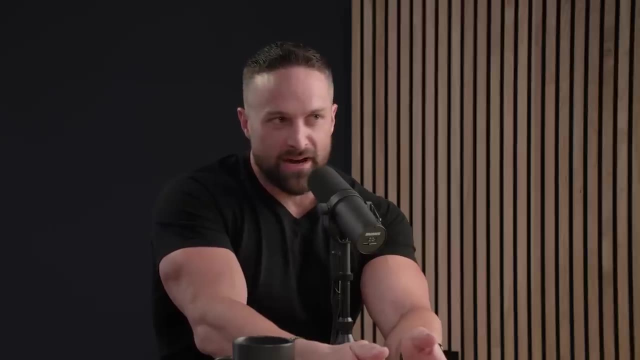 i was noticing them, they they were fidgeting their feet and their their fingers and i said: you know, have you always like been pretty lean? and they were like, yeah, i never really had a problem. and when you look at the obese resistant phenotype, people think they have high bmr or 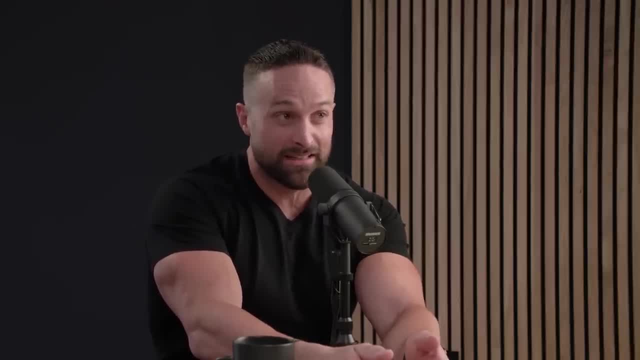 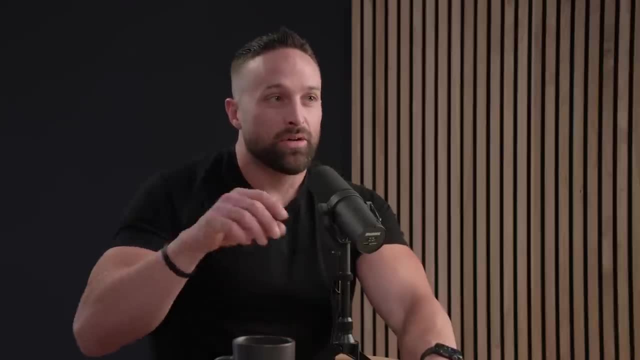 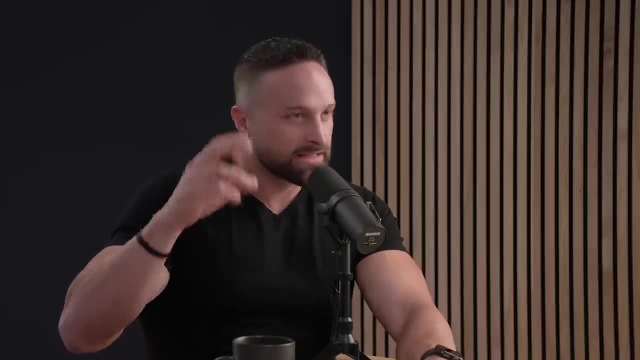 you know they exercise a lot and really what it seems to be is neat. they tend to. if they overeat, they just spontaneously increase their physical activity. now people get neat confused. i've heard people say: well, i'm going to go out for a walk to get my need up. that's not neat. neat is not. 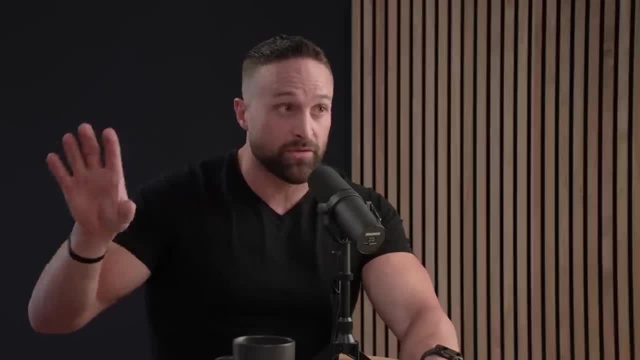 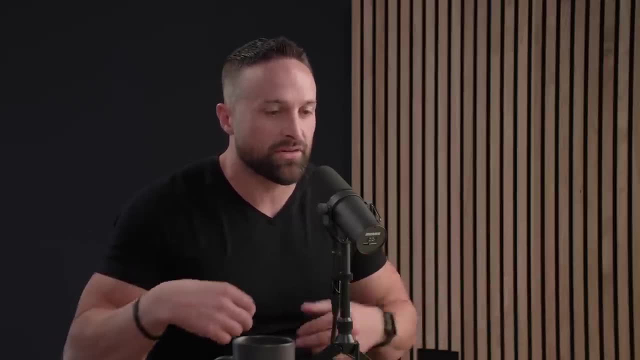 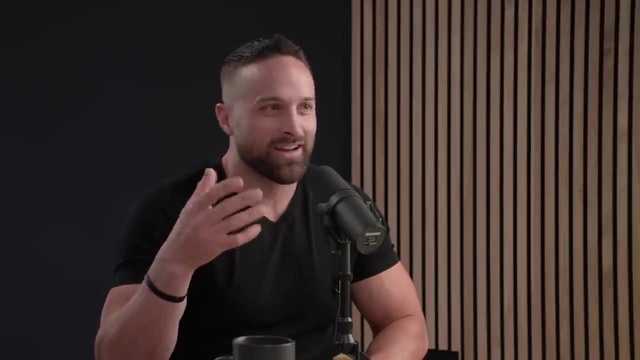 something you can consciously modify what you're doing there if it's purposeful, it's exercise. so for when i'm talking, if i'm waving around my hands, if i'm tapping my feet, if i'm whatever, that's neat. but you know, trying to like get yourself. well, i'm just going to tap my foot more. well, now, if i'm. 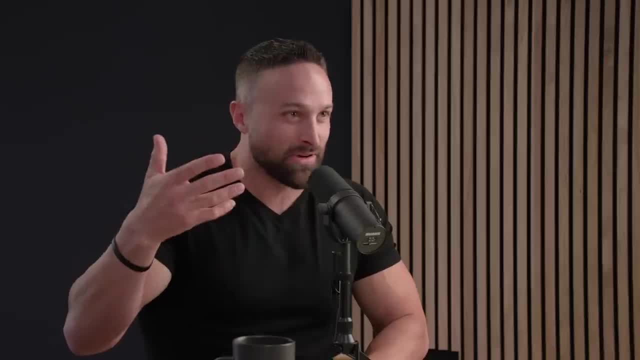 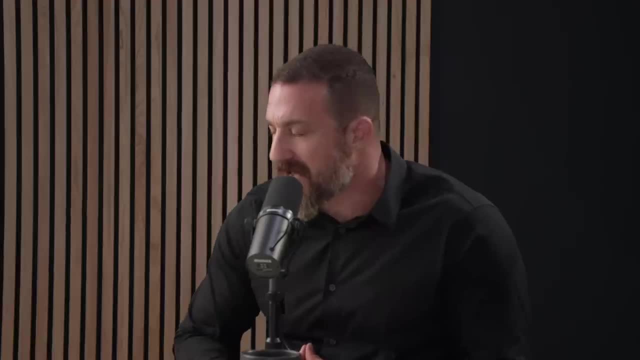 consciously having to do this, then my focus- i mean you. you know how the brain works very hard to do. you know you don't really do two things at once, right, you kind of switch quickly between tasks. absolutely, can i quickly ask: uh, was the person that you're referring to our friend? uh, ben bruno? 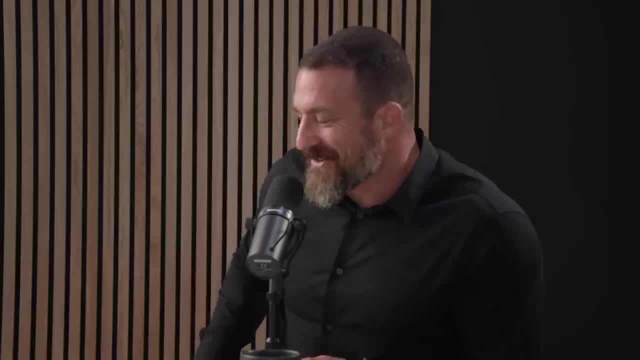 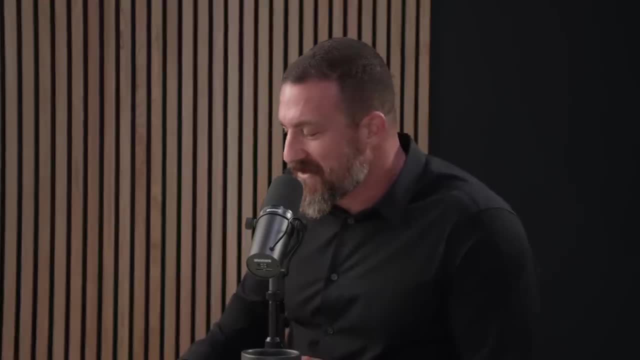 no, no, he was. he is fidgety. yeah, amazing online fitness channel. um, he's a freakishly strong individual, yeah, and uh, um, i can't remember whether or not ben you're a fidgeter or not, but anyway, i'll have to go go check and we'll measure. 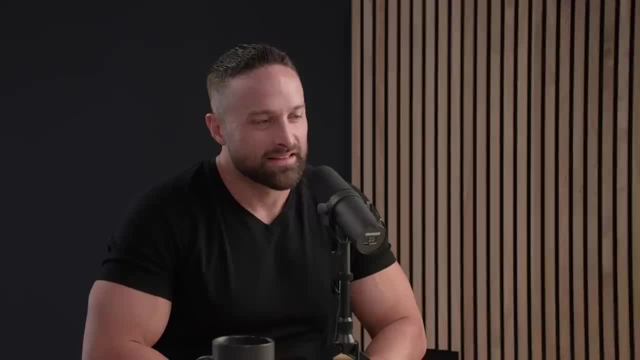 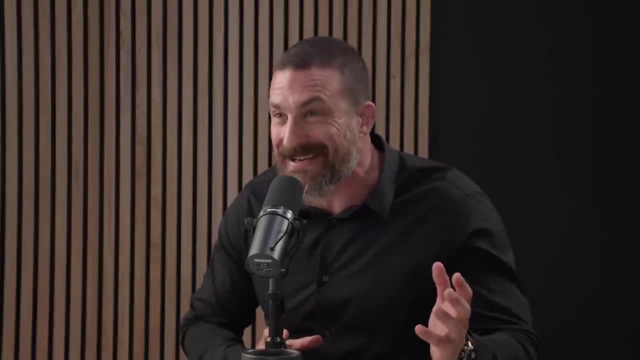 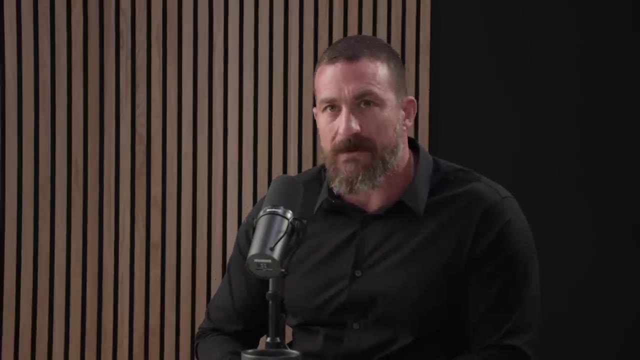 your fidgeting um about, uh, non-exercise induced thermogenesis, neat. my understanding of the old papers on this old being, i guess back to the mid 90s- is that the calorie burn from neat is actually pretty significant. we're not talking about 100 calories or 200 calories per day, we're talking 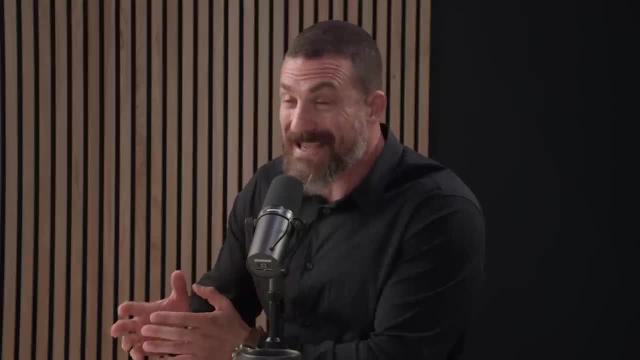 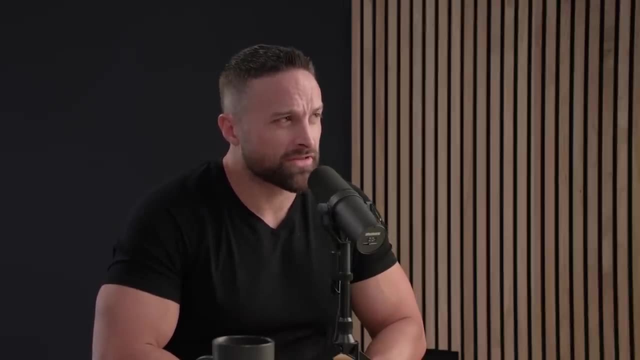 hundreds of thousand- excuse me, hundreds- to maybe even close to a thousand calories per day. could you elaborate on that? yeah, so there was actually a really classic study, i think from- i want to say it's from- levine in 1995. it was metabolic award study and hopefully i don't butcher the study. 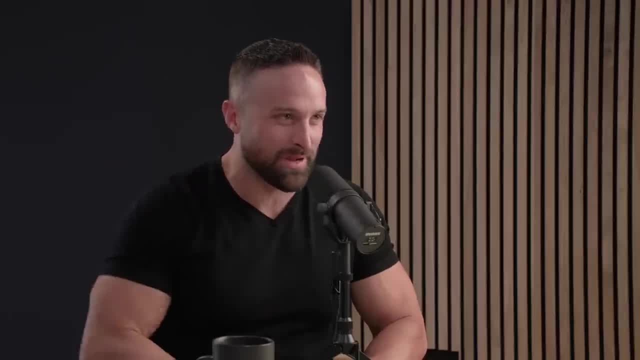 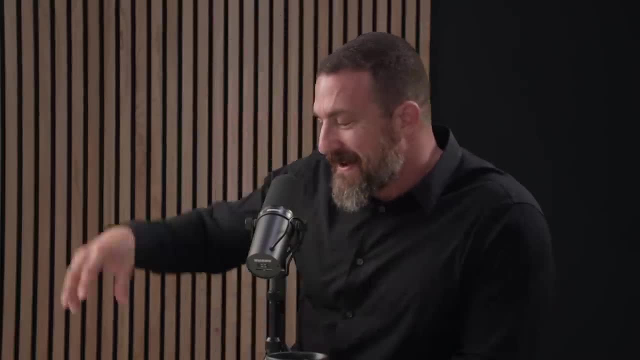 because i'm trying to, you know, pull it out of my brain. i don't expect you to have pubmed in your head, although i must say you have a quite extensive, uh pubmed id, um grab bag in there, so i try to bring the receipts. yeah, i try to bring the receipt we can put. we will put a link. 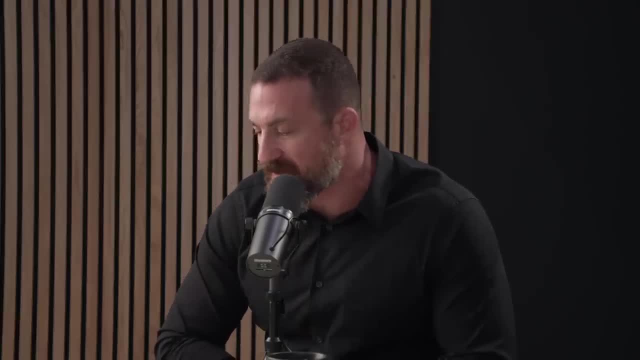 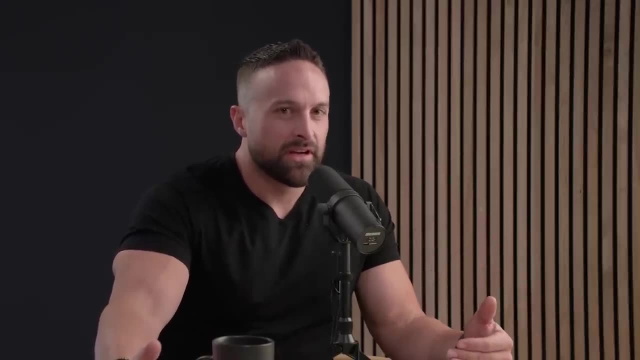 to this study in the show note captions. so, um, people can peruse it if they like. yeah, so i i believe they had people overeat and i think it was by like a thousand calories a day and i think for six weeks, and i mean, this is the metabolic ward. so they are. this is very tightly controlled, it's. 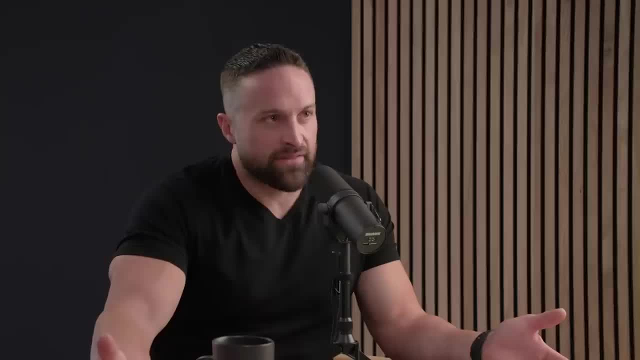 as tight as you get, and what was interesting is, of course, on average, people gained weight and gained fat mass, but some people gained more than expected, and there was one person in particular who only gained like just over half a kilo. right, they should have gained like, i think it was something like three to four kilos. it was was predicted and what they found. 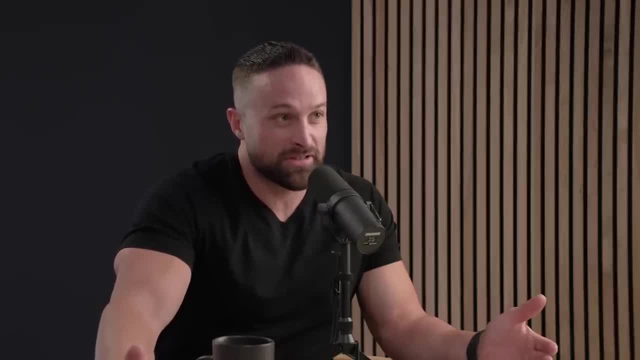 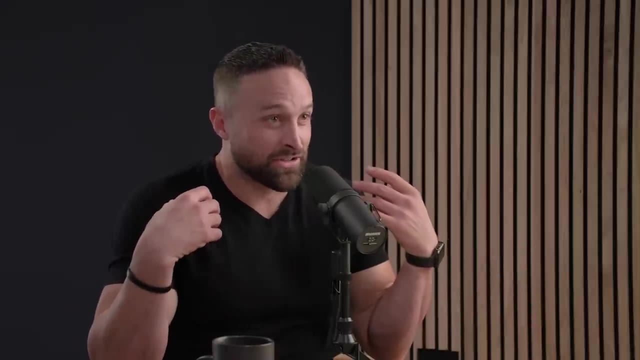 is this individual just spontaneously increased their physical activity, like he didn't purposely do it. it just happened. and i mean, you know, anecdotally, i've seen people who are- again, you know, very lean even eat a meal, sit down and start sweating, you know, and be very fidgety. there was a natural bodybuilder back in the day named jim cordova. 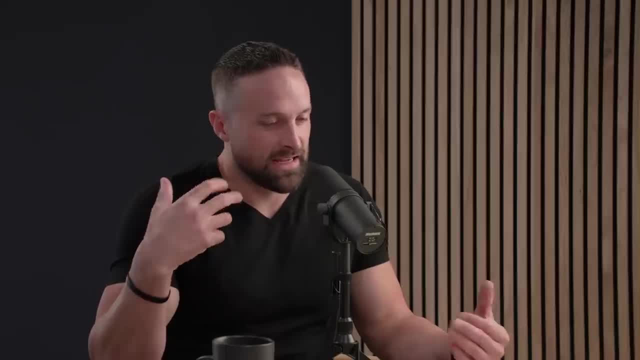 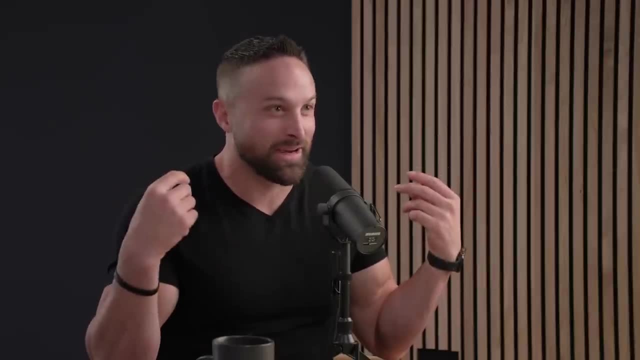 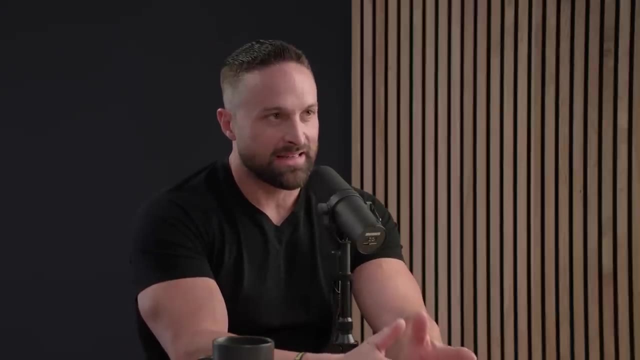 and this guy was just very lean all the time and he was exactly that phenotype. you know he would walk up a flight of stairs and all of a sudden he's sweating. sit down, eat a meal- he's sweating, you know he just he's a furnace just expending energy. and what's very interesting about neat is 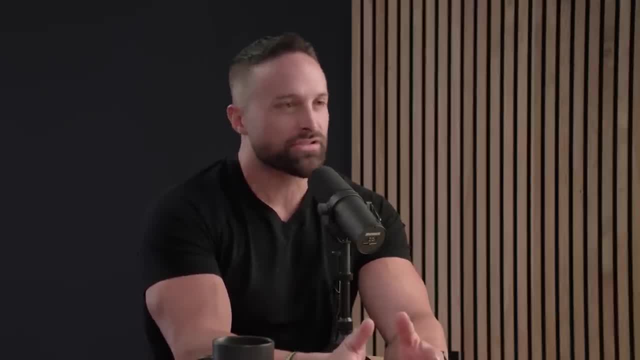 that seems to be the most modifiable. i mean, exercise is very modifiable because you can be intentional with that, but of you know, bmr, tef and neat, neat seems to be far more modifiable. so even a body weight reduction of 10. they've observed a decrease in neat of almost 500 calories a day. for for a 10 reduction in body weight. now, you also do get a decline in bmr when you lose weight. one, because you're just in a smaller body now, and so it takes less energy to locomote. but also there's what's called metabolic adaptation, which is a further reduction in your 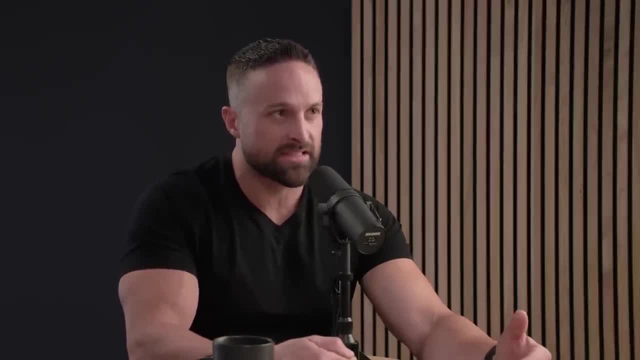 bmr than expected from the loss of body mass, and that's on average usually around like 15, but it does seem to be. there's new evidence coming out on the metabolic adaptation from bmr and it seems to be a little bit uh, kind of in the transition phases. so if you, if you start a diet, within the first few weeks you will have a reduction in bmr. that then kind of just after. thereafter, any further reduction is mostly from the amount of body mass you lose and then, if you like, for example, finish a diet and move your calories to maintenance. um, within a few weeks bmr kind of starts to come back up. there is still a small 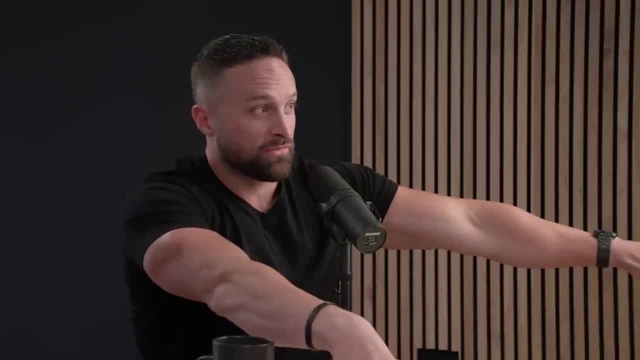 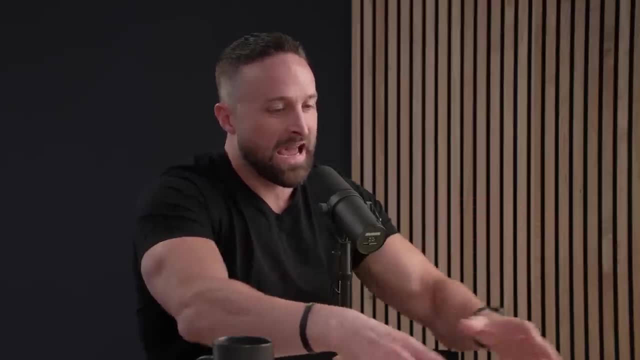 reduction, uh, but i used to be somebody who thought the bmr, you know, the metabolic adaptation, was a big reason why people stopped losing weight or plateaued. and now i think that's a little bit more. i think it's much more to do with neat, interesting, and you've said that it can't be conscious. um, 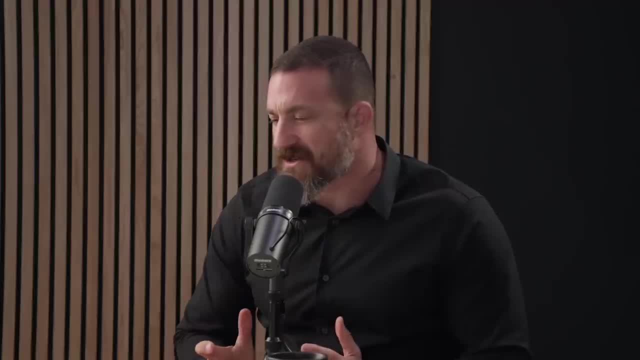 because that will distract us from other activities. i don't know if you've had a chance to look at this study and i'll send it to you. maybe it'd be fun to do a kind of an online journal club about this at some point soon. but there's a study that came out of university of 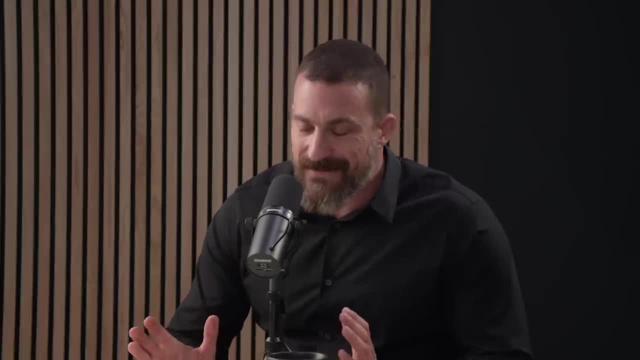 houston recently having people do. now this is a long period of time, four hours a day, of basically a soleus push-up which is basically a heel raise, kind of a seated calf raise, with one foot not weighted. and then they looked at a bunch of things about glucose metabolism. 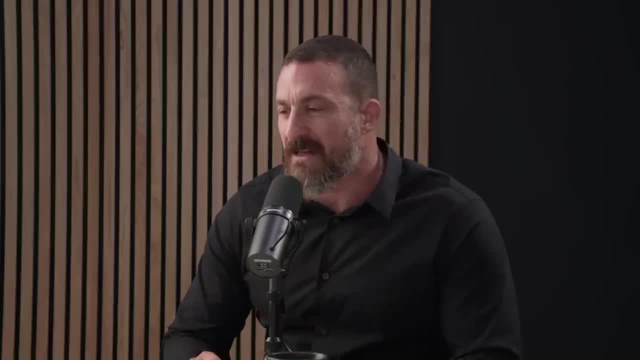 and glucose clearance and insulin levels, and they didn't conclude that people burned a ton of calories, but what they concluded was that um, blood sugar regulation improved greatly and i think you know there was a lot of excitement about this um at some level. but based on everything, 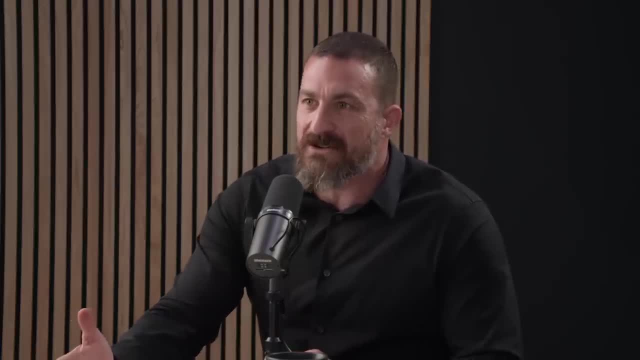 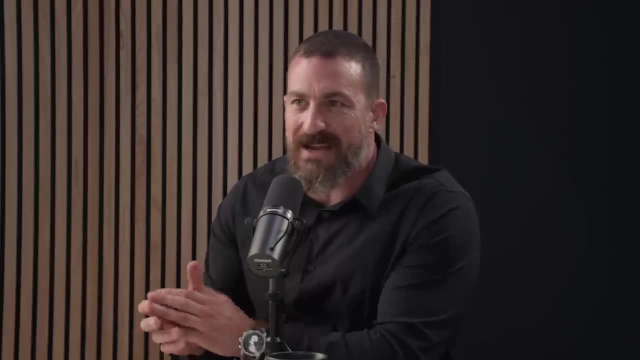 you're telling me this, it fits perfectly with what's known about neat. so this sort of fell somewhere in between with um in between, excuse me, uh, sort of deliberate exercise and spontaneous movement. i guess they've tried to make that sort of balance between what's known as neat and what's. 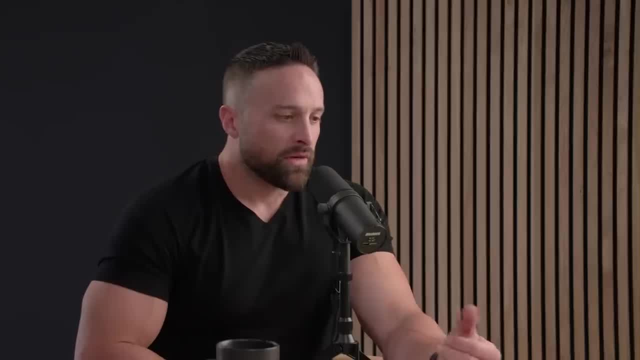 known as neat. i guess they've tried to make that sort of balance between what's known as neat and what's known as neat and what's known as neat. i guess they've tried to make that spontaneous movement, that spontaneous movement, a little bit more conscious. well, what i'll tell people is, if you're worried about neat, one thing you can do. 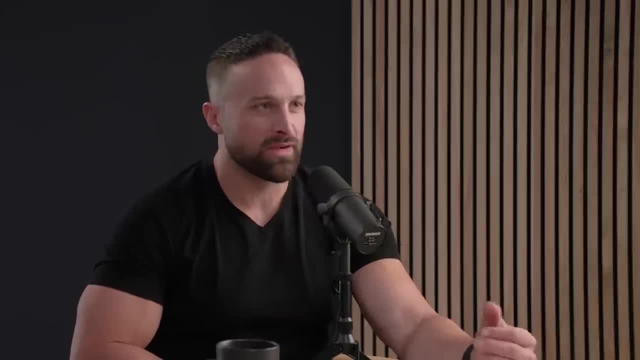 like these watches, for example, a lot of people like, oh, what told me? i burned this many calories. they are not accurate for energy expenditure. i mean, it is like there was a meta-analysis in 2018. i want to say between a 28 and 93 percent overestimation of energy expenditure by these. 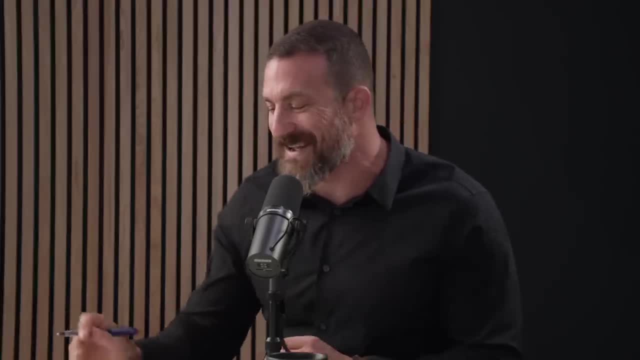 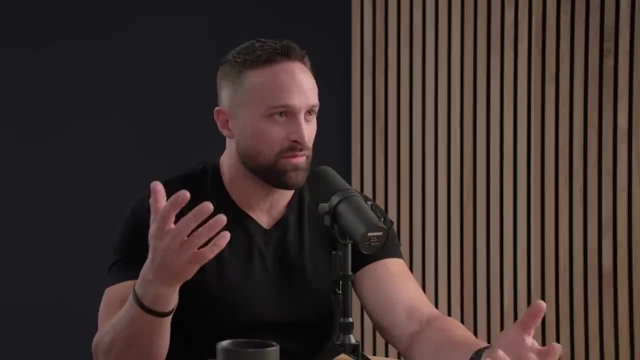 watches fitness track. so, for those of you listening, if you're listening, if you're listening, if you're listening, we're not going to name the brand, but, uh, fitness trackers, so wrist-worn fitness track and this, and this is across the board. um so like, depending on the brand, it could be you know more. 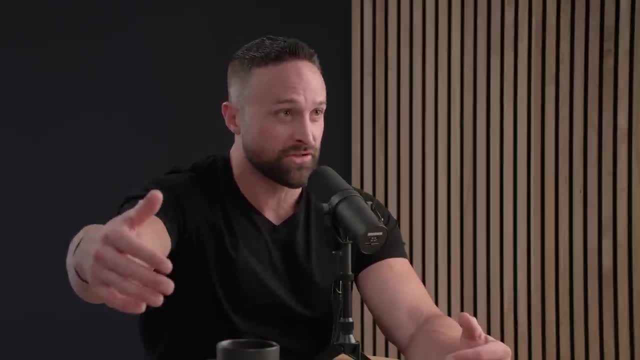 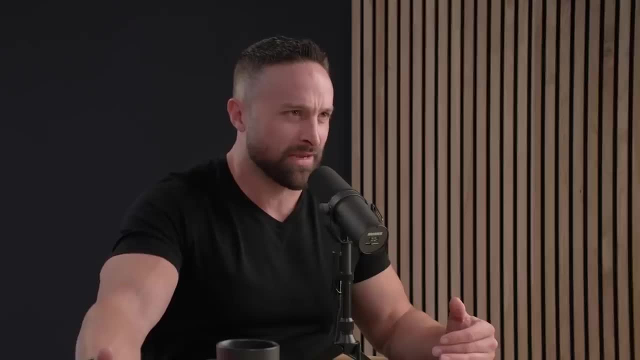 or less, but they all overestimated the amount of x, the calories you burn from exercise. so this is actually a great example where people go well, calories in, calories out doesn't work for me, because i ate in a calorie deficit. i didn't lose weight, you know, when i talked to them, usually it's 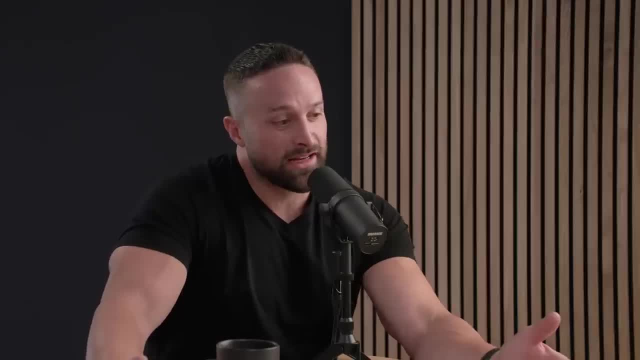 they went to an online calculator. it's one, it's a few things. they went to an online calculator, put in their information. it's spat out some calories to eat and they ate that and didn't lose weight and it's like, well, what do you think is more likely that you're defying the laws of? you know um, conservation of energy. 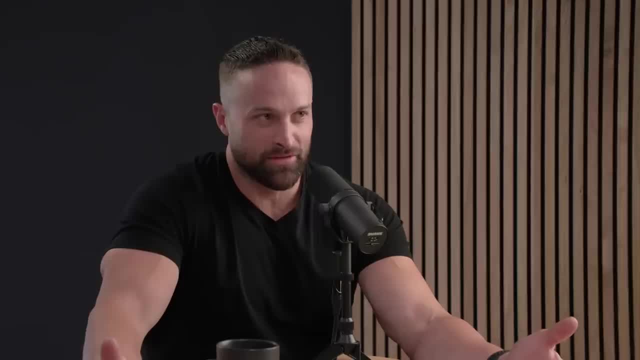 or that you're, you might have not gotten the right number for you. the rule: the measurement tool was off, yeah, the next thing is a lot of people weigh very sporadically and i'll tell people like, if you're going to make an intentional weight loss a goal, um and again, this can be. 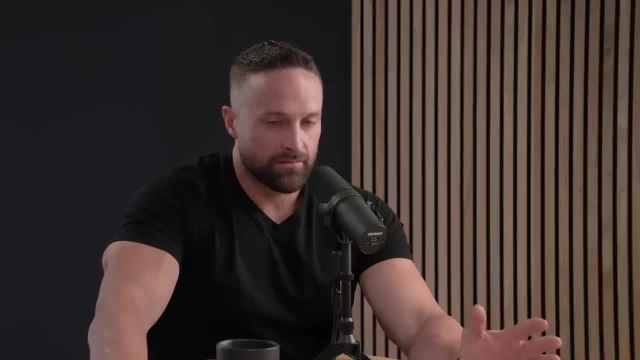 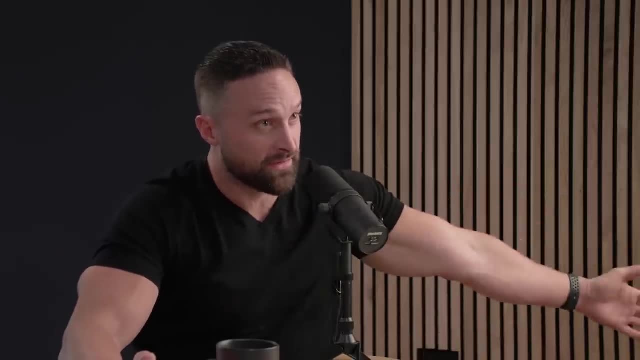 different for different people, but typically i tell people weigh in first thing in the morning, go to the bathroom, do it every day and take the average of that for the week and then compare that to the next week's average. can i ask one? sorry to interrupt but one quick question about that: when 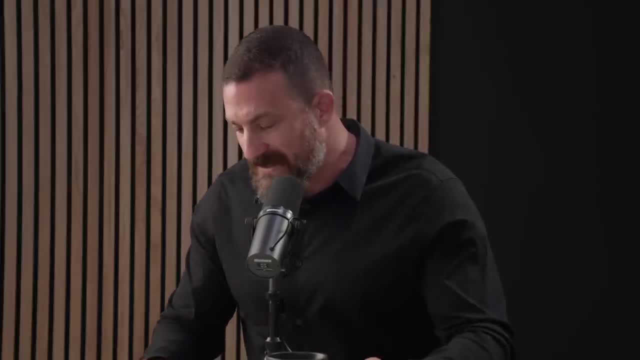 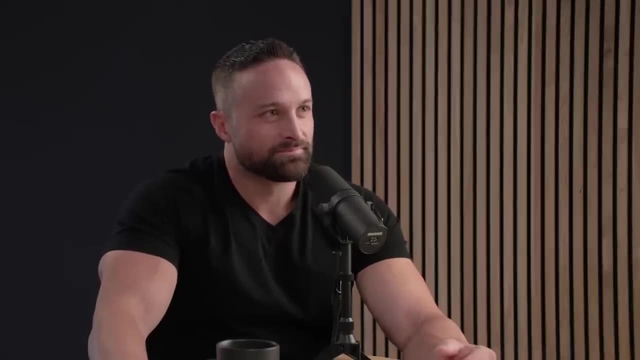 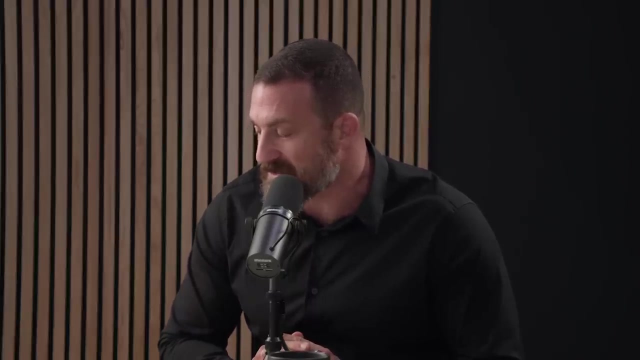 you say: go to the bathroom not to get um too detailed, uh, here for unnecessarily, but are you talking about urination and um emptying your bowels, ideally because you get a big meal the night before? yeah, yeah, got it. so wake up, uh, use the bathroom, um in all, all forms that you're ready, and then, and then get on the scale. take that. 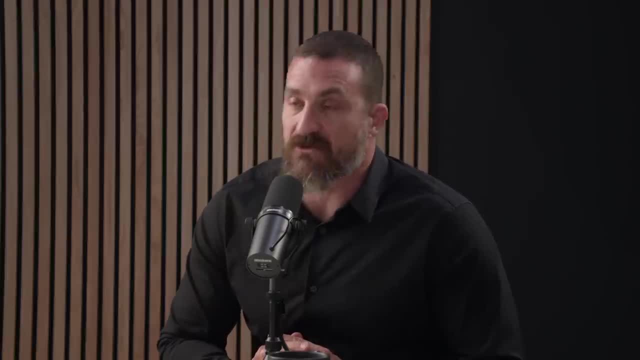 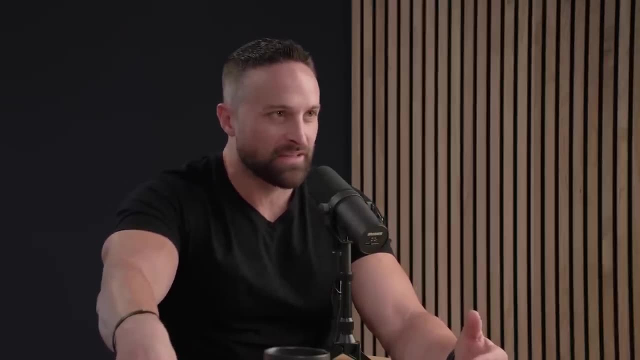 measurement, average that across the week and then maybe every monday you take that value and see. and the reason i i recommend doing that is if you're just kind of sporadically weighing in, as somebody who weighs themselves pretty, pretty regularly, i mean my weight will fluctuate you. 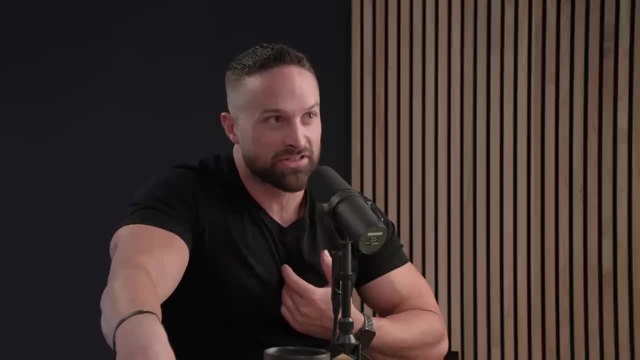 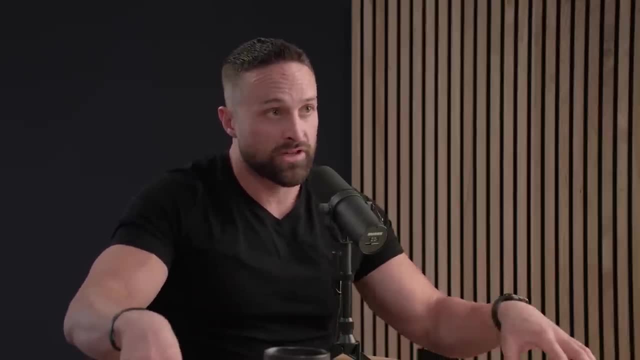 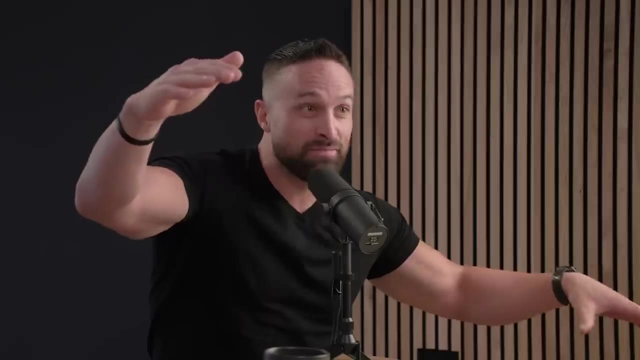 know five, six pounds and not seemingly changing much. you know, and that's just you know those short term changes are fluid. so i'm i've had it before where, week to week, my average didn't change but between the lowest weigh-in from a previous week and the highest weigh-in might have been like eight. 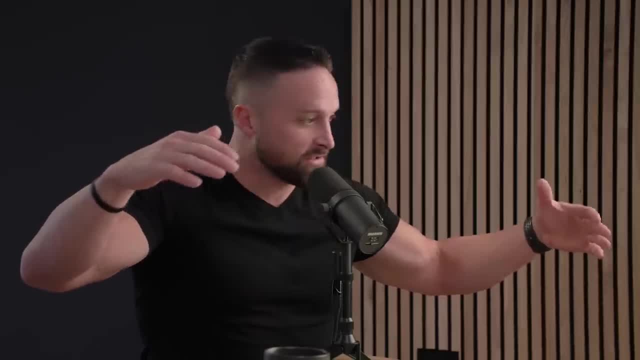 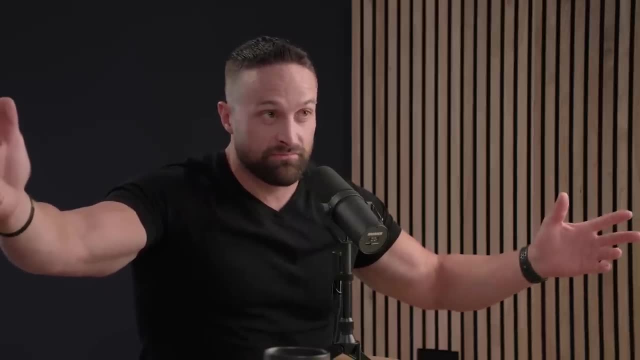 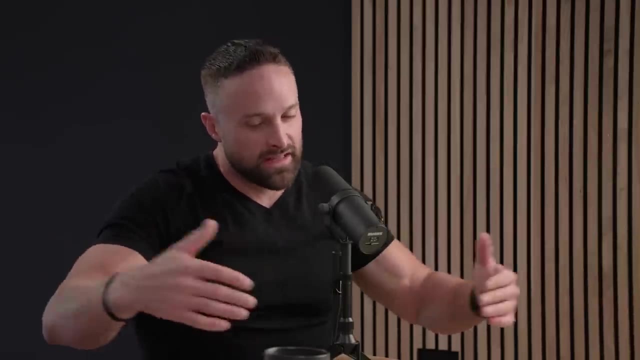 pounds, right. so if you're somebody who just randomly is weighing in and you're eating in a calorie deficit and you just weigh in one day where you just, whatever reason, holding some more fluid, then you oh see, this isn't working when in reality your average might be dropping. so that's. 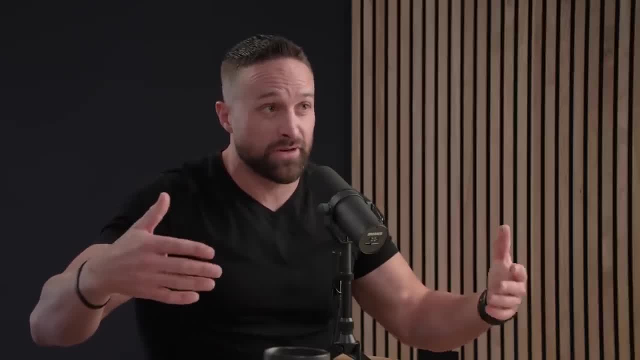 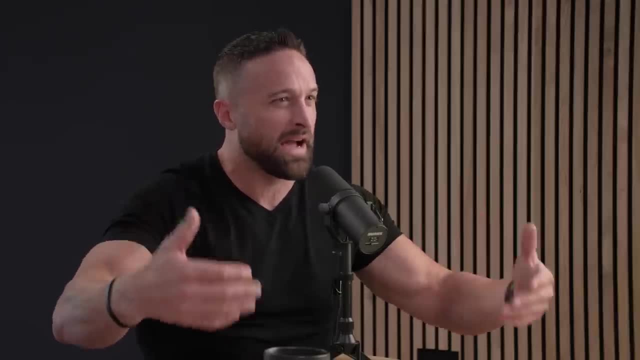 one of the reasons- and actually believe it or not, weight fluctuations are actually identified as a major reason why people get discouraged from weight loss. um, that it kind of stops the buy-in, you know, when they have a fluctuation up. so that's one of the reasons early. one of the reasons early on that low carb diets tend to 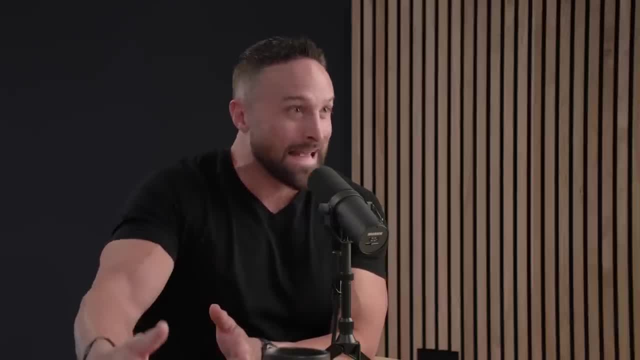 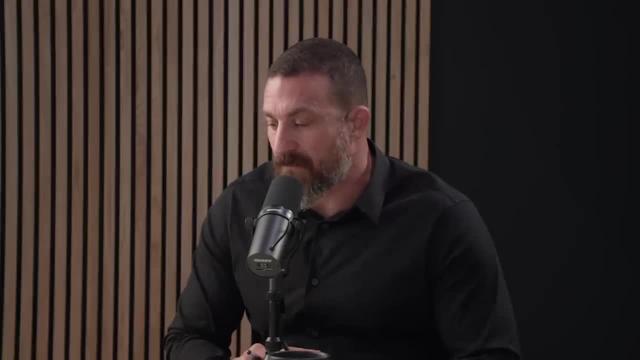 work really well is because people lose a lot of water weight really quickly and they get that buy-in right. so, oh, this is working. yeah, we can return to that in a little bit, because i have theories as to how that. um, you know, when people eat less carbohydrate, they scrape more water and 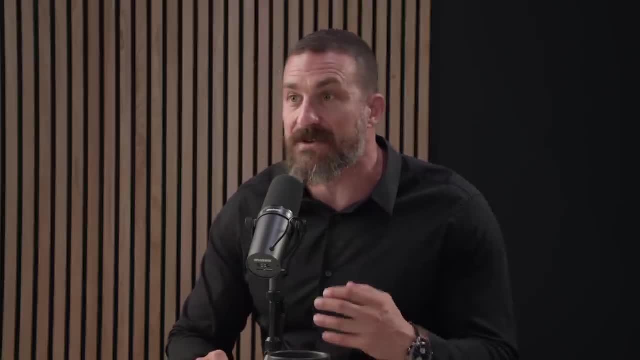 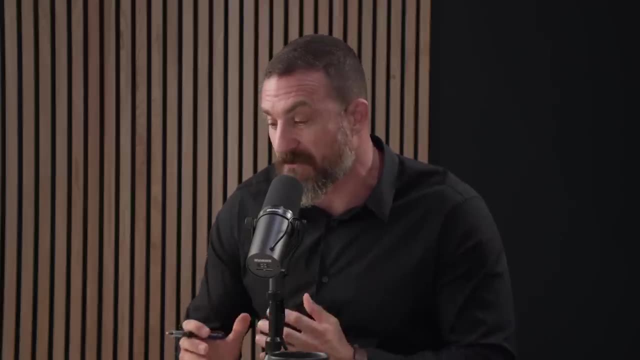 they'll see, you know, for the first time they'll see some definition in their abs and, oh my god, this diet's amazing. yeah, um, and the fluid loss does hold that promise. i think fluid loss can do some other things that might people make people literally feel lighter, although we have some negative effects. i do have one quick. 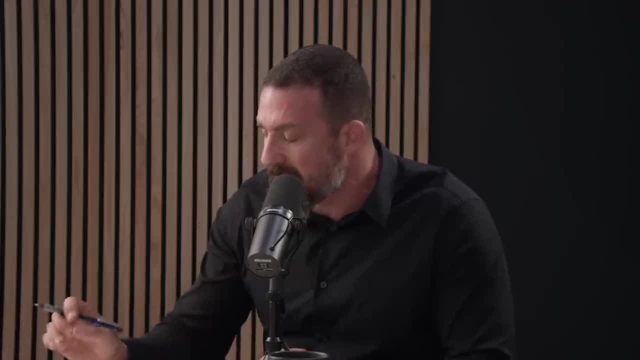 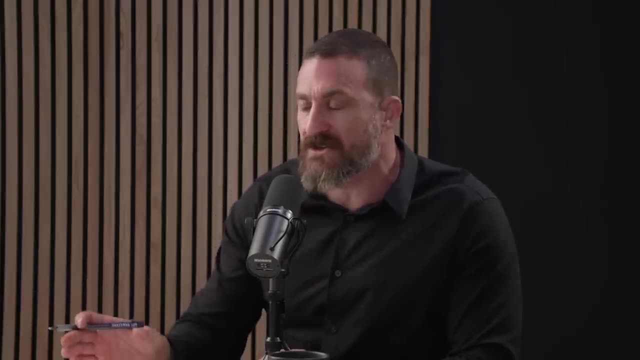 question and um, i do. we'll return to neat in a moment- but when you say the caloric burn as a consequence of exercise, i want to ask about the caloric burn during that exercise. so, for instance, somebody's on the treadmill and they'll see, okay, they burn, you know, 400 calories actually, i think. 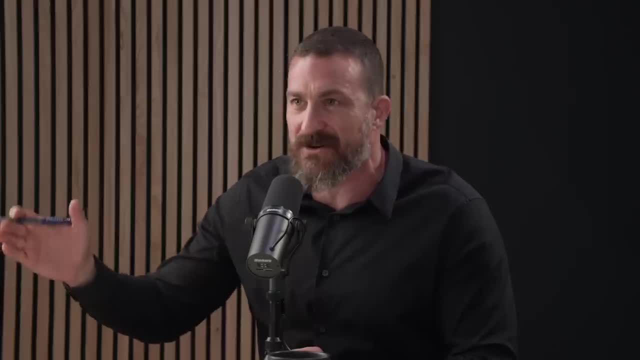 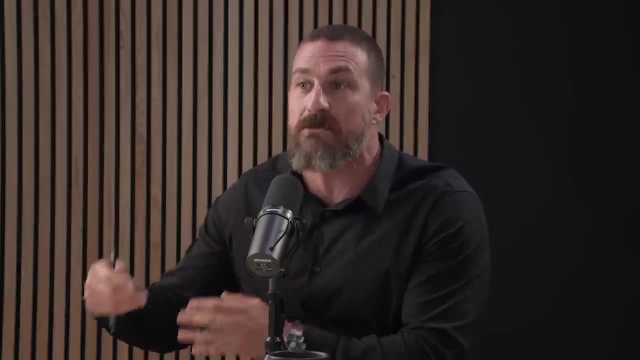 this is a month where a number of prominent podcasters like burke kreischer, tom segura, joe rogan, others, are doing. they call it sober and they're like, oh my god, they're burning 500 calories per day during the exercise. they're measuring it. a lot of people do this. they think they take track of whether, excuse me, take stock of. 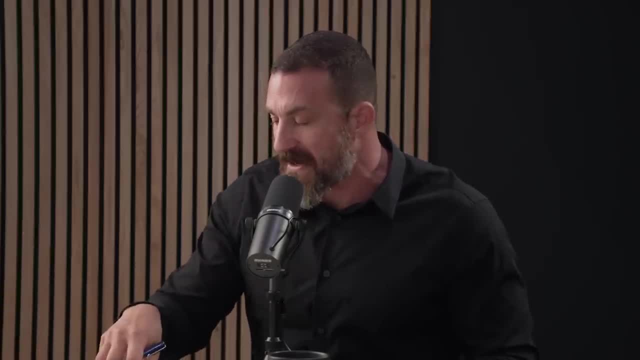 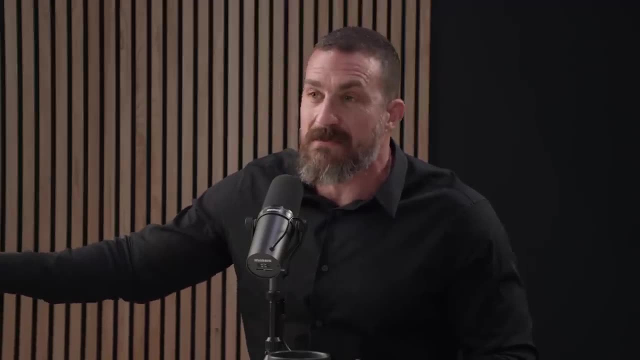 how many calories they burned. my understanding is that if that particular form of exercise is a muscle building form of exercise, that at some point later there might be an increase in muscle. if you did it everything right, do everything right and then you will burn more energy as 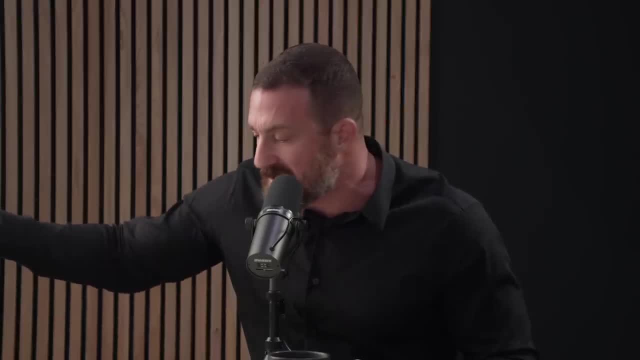 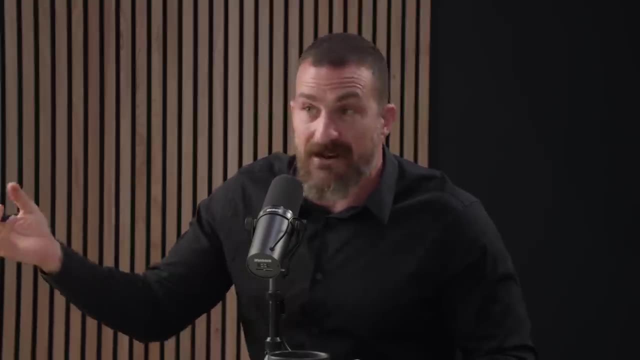 a consequence of adding that tissue. that's a lot of calories per day during the exercise long process, as as you know and we will discuss, but i have heard about this post-exercise induced increase in oxidative metabolism. i'm probably not using the right language in here. so if i were to go out, for instance, and sprint, do some sprints, run hard for a minute, jog for a minute, run hard for me and do that 10 times over, though let's assume i burn 400 calories during that exercise bout. but my understanding is that in the hours that follow, my basal metabolic 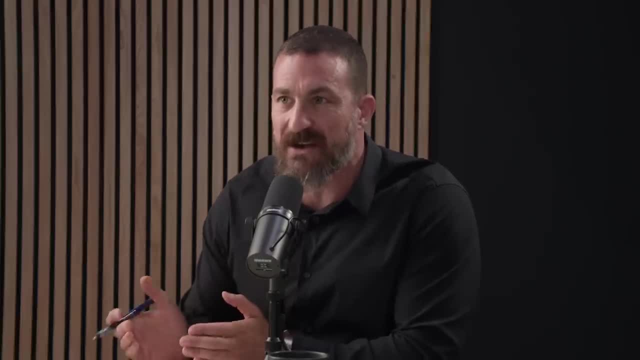 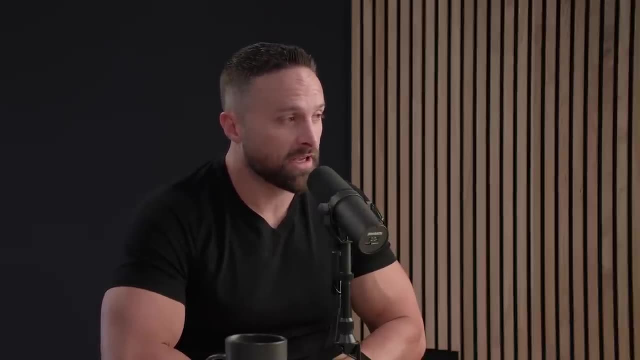 rate will have increased. is that true and is it significant enough to care about? so i answer both those questions. um, yes, there does seem to be a small increase in metabolic rate and no, it does not appear to be enough to actually make a difference. so when they look at- and again this, 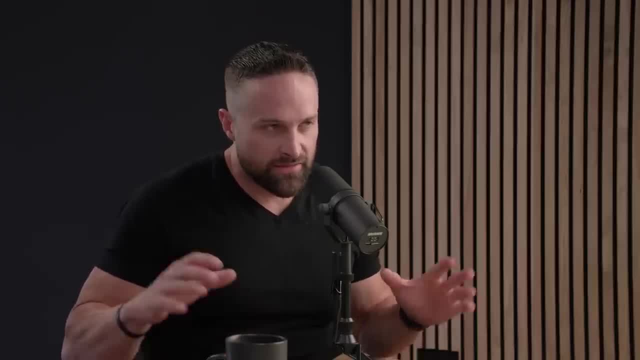 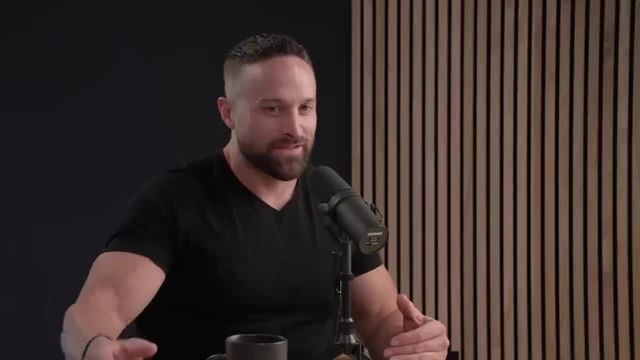 is where, um, i tell people i think i have a good perspective on this because i my undergraduate degree was a biochemistry degree, so i was very into mechanisms. you know what i mean. it was like if we just do this and this, we'll get this right. And then I did nutrition as a graduate. 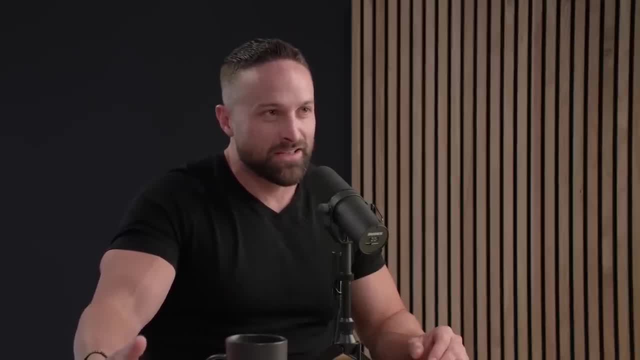 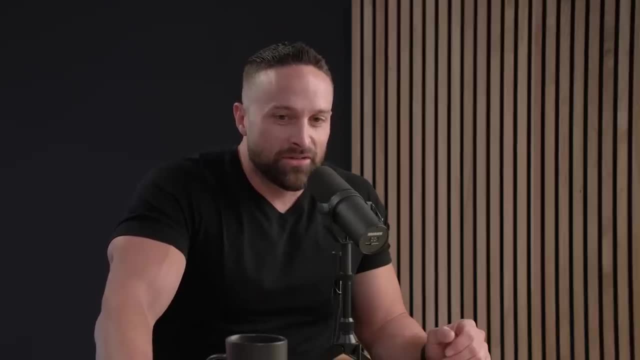 degree, And then my advisor was so great because you could do something over here and he could tell you how it would affect vitamin D metabolism over here. This is Don Lehman, Yeah, Don Lehman. So he would always kind of say, yeah, but what's the outcome? going to be right? So this is actually 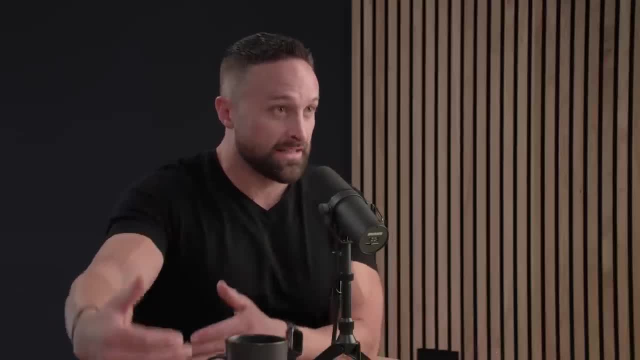 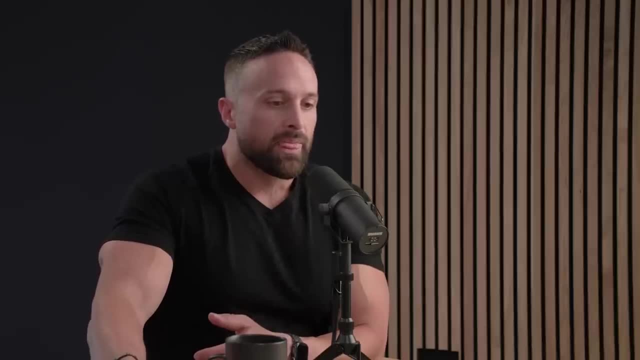 one of the things I changed my mind on was I used to be very much well, I think high intensity interval training is probably better because you get this post-exercise energy burn Which they do see in some of these studies but in the kind of meta-analyses and like more. tightly controlled studies where they equate work between high intensity intervals and moderate or low intensity cardio, so equating work, they don't see differences in the loss of body fat, And so to me, if I'm looking at that's the example of a mechanism which is okay. 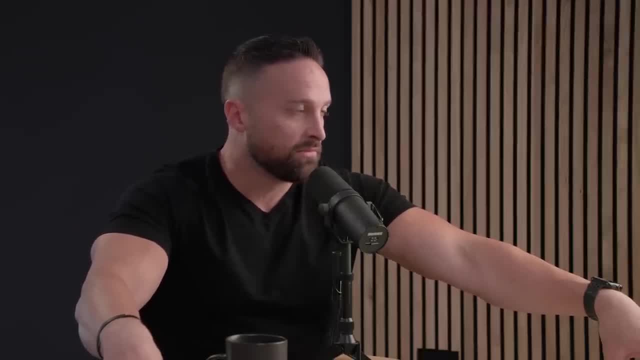 we're seeing this small increase in basal metabolic rate that should lead to increase loss of body fat. But again, remember, you're capturing a snapshot in time, right, But we don't see a difference in the loss of body fat. So what may be happening? and again, I'm just speculating. 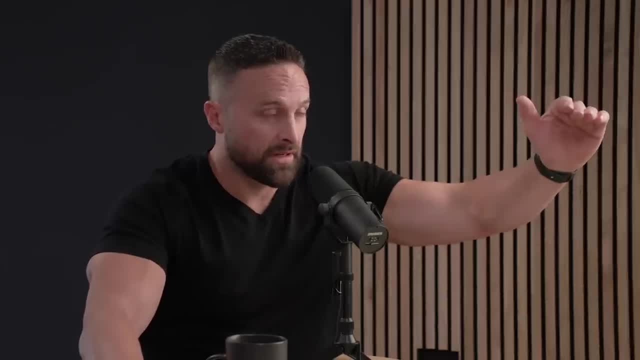 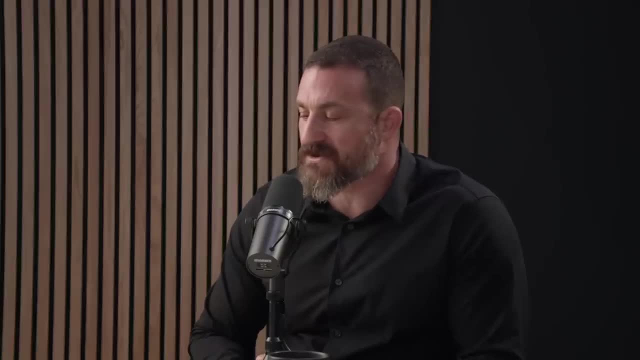 but a way to explain it could be you might have an increase and then you might actually have a decrease. that tends to just kind of wash it out, Right, I see, And I have to imagine some forms of exercise. this would be highly individual, but will spike appetite more than others. So, for instance, if I go out for a 45 minute jog or which I do a 45 to 60 minute hike or jog once a week, I just make it a point to do that or rock, or something like that: throw on a weight vest and hike. After that I find I very thirsty. I want to hydrate, but I'm not that hungry. That's true of most all cardiovascular exercise for me, But after I weight train, about 60 to 90 minutes later, I want to eat the refrigerator, And so 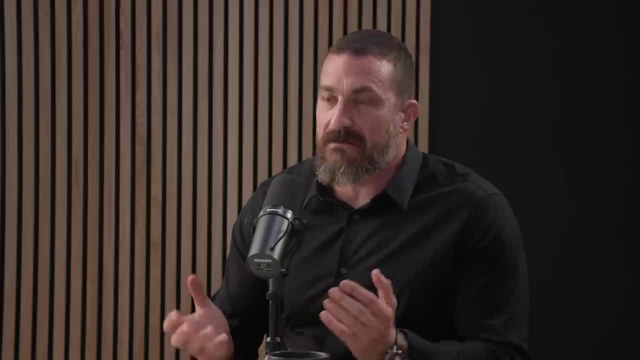 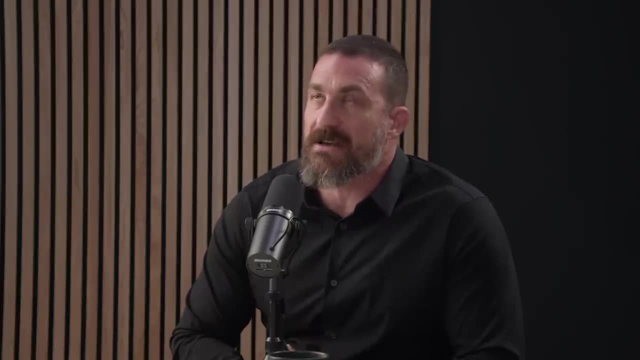 obviously, calories in calories out dictates that that will play an important role as to whether or not I gain or lose weight, etc. So is it safe to say that the specific form of exercise that people choose needs to be taken in consideration of calories in calories out? So how? 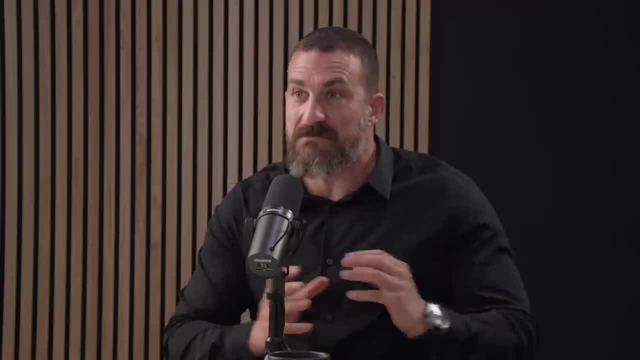 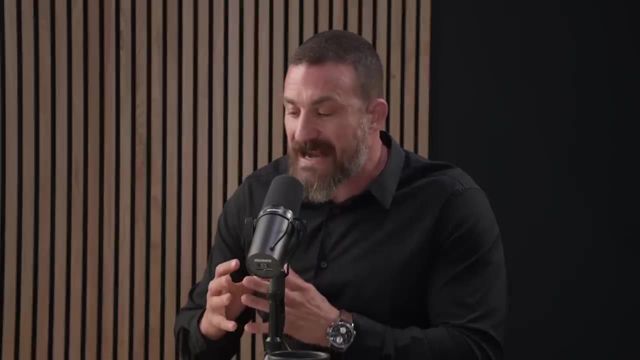 much is burned during the exercise. Also, how much that exercise tends to stimulate appetite. I don't know whether or not people explore this and the rigorous studies and whether or not that form of exercise actually increases lean muscle mass or not. So now we've taken exercise and split it into. 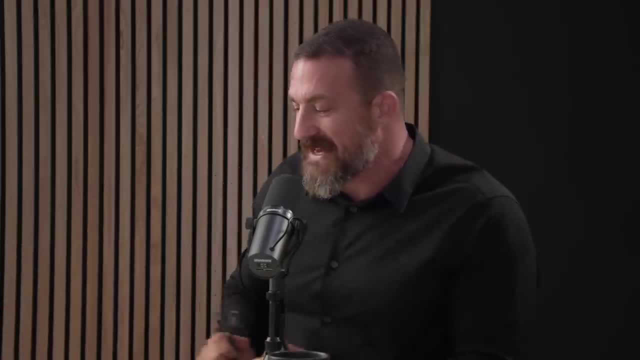 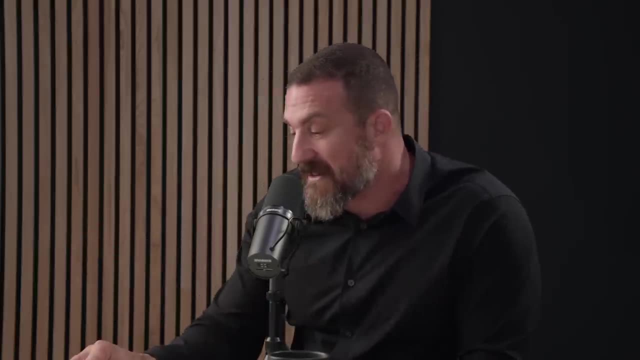 a number of different types mentions, but this is what you are so masterful at is really parsing how the different components work individually and together. So if you would just, you know, expand on that, I'd love to know what you're thinking. Yeah, So this is actually a really fascinating thing. So, first thing I want 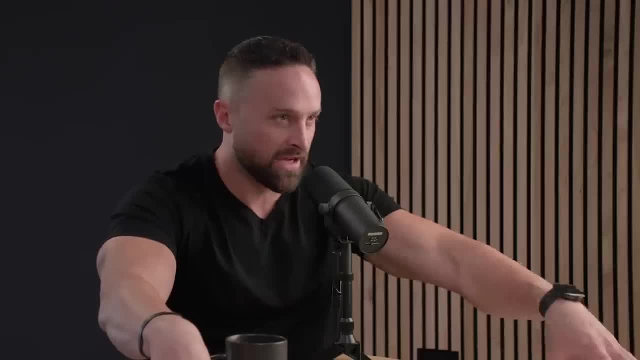 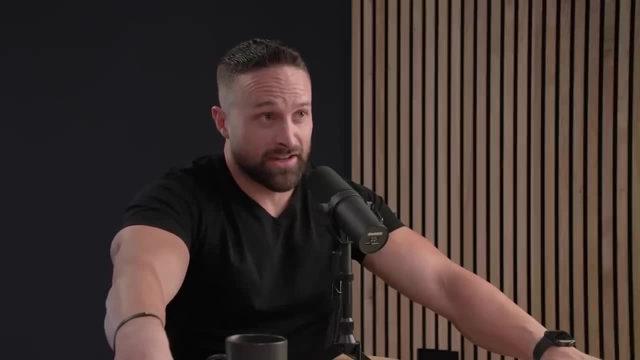 to. I want to just go back to talking about like, for example, Bert and Tom and Joe, we're gonna do 500 calories a day on whatever, So those apparatuses don't measure those things effectively either. right, Just like these watches. But the one thing I will say is: if you are like for example, if I do two hours of resistance training, typically this will say I burned about a thousand calories. right, That's a lot of resistance training. My weight workouts are like are warm up for 10 minutes and then one hour of work done. I just I love to train. Okay, And you can. recover from. my recovery quotient is pretty low. So I've been training for 30 plus years and I found that if I do more than an hour of hard work in the gym- meaning resistance training, 75 minutes, maybe I'm okay, But past. that I have to take two, maybe even three days off before I can train. My nervous system just doesn't tolerate it. well, So I limit it to an hour. you know, And part of that to remember is like I've kind of built up to that over a long period of time. right, You know? so you couldn't. 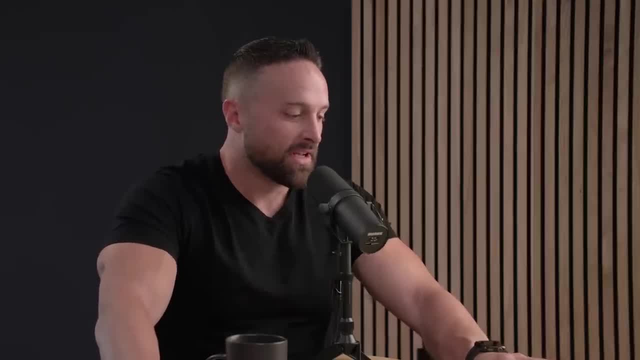 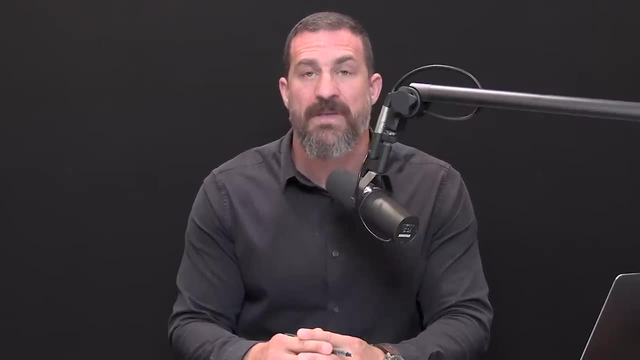 just throw somebody in and start having them do two hours a day. It's not going to go well for them. I'd like to take a quick break and acknowledge one of our sponsors, Athletic Greens. Athletic Greens, now called Athletic Greens- It's called AG1, is a vitamin, mineral, probiotic drink that covers all of your foundational nutritional needs. I've been taking Athletic Greens since 2012.. So I'm delighted that they're sponsoring the podcast. The reason I started taking Athletic Greens, and the reason I still take Athletic Greens once, or usually twice a day, is that it gets to be the probiotics that I need. 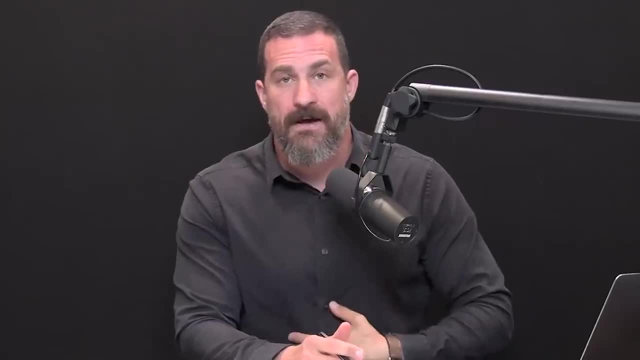 for gut health. Our gut is very important. It's populated by gut microbiota that communicate with the brain, the immune system and basically all the biological systems of our body to strongly impact our immune system. So I've been taking Athletic Greens since 2012.. So I'm delighted that. 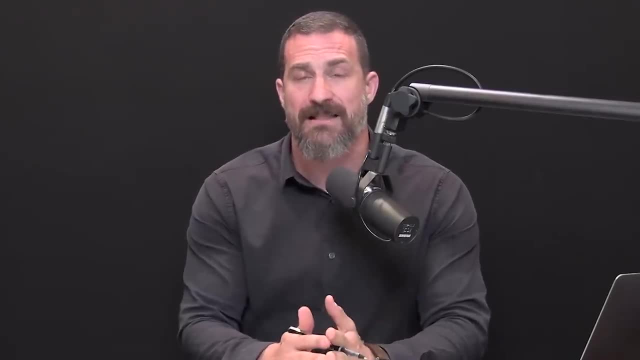 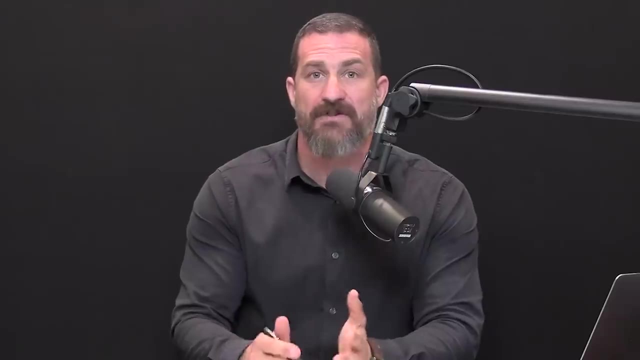 it's a good product for our immediate and long-term health, And those probiotics in Athletic Greens are optimal and vital for microbiotic health. In addition, Athletic Greens contains a number of adaptogens, vitamins and minerals that make sure that all of my foundational nutritional needs are. 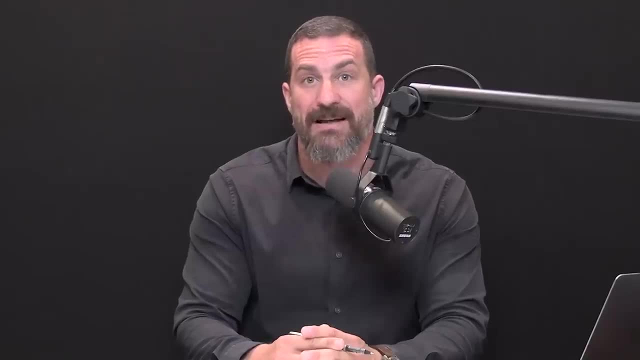 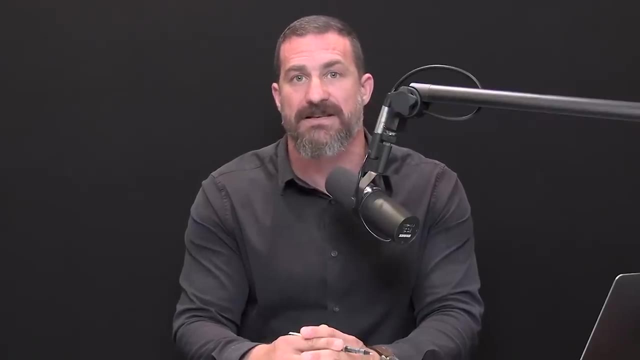 met And it tastes great. If you'd like to try Athletic Greens, you can go to athleticgreenscom- slash Huberman and they'll give you five free travel packs that make it really easy to mix up Athletic Greens while you're on the road, in the car, on the plane et cetera, And they'll give. 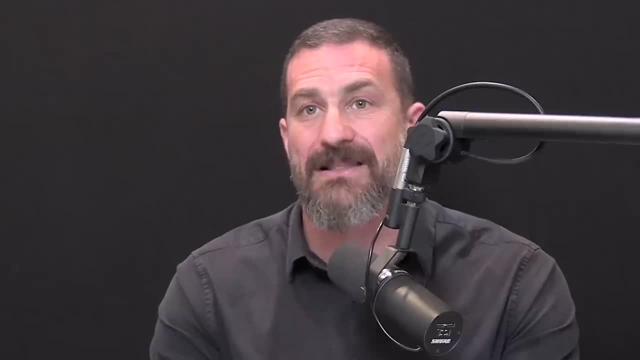 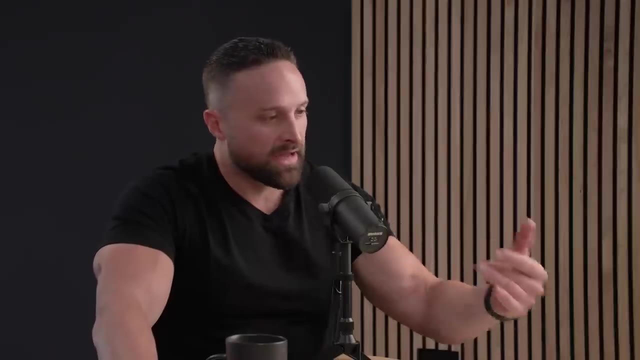 you a year's supply of Athletic Greens. So if you're a fan of Athletic Greens, you can go to of vitamin D3K2.. Again, that's athleticgreenscom. slash Huberman to get the five free travel packs and the year's supply of vitamin D3K2.. What I will say about the calorie trackers is: 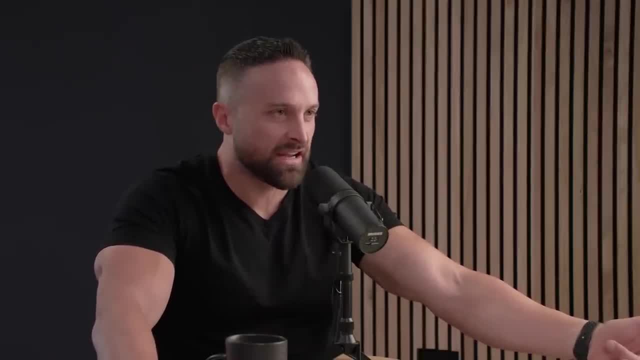 so if I'm used to okay, usually burn about a thousand calories according to this, it's not accurate. But if I go in tomorrow and I do 1300, it may not be accurate. I don't know what the exact number is, but I can be relatively confident that it's more than the previous session. 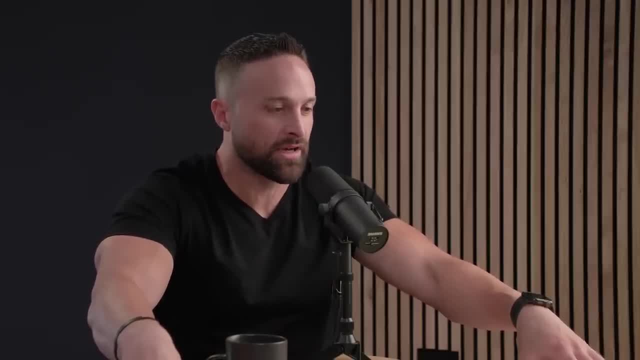 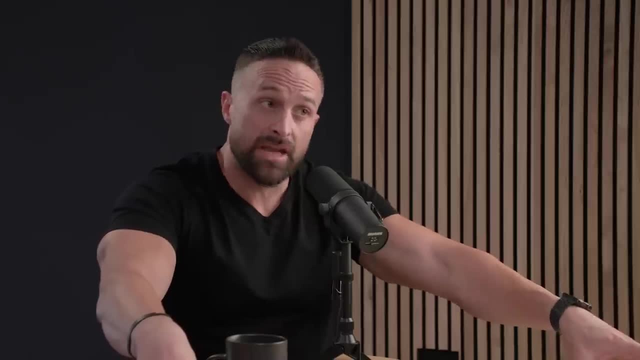 Right And so in terms of- and it might be okay, like you know, kind of within subject. And then the other thing I was kind of circling around on was if you're worried about NEAT tracking, your steps can be helpful. 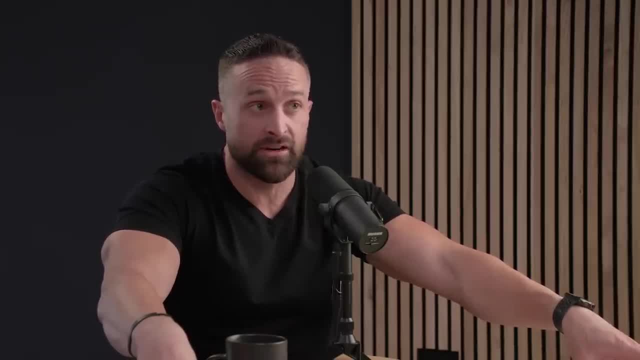 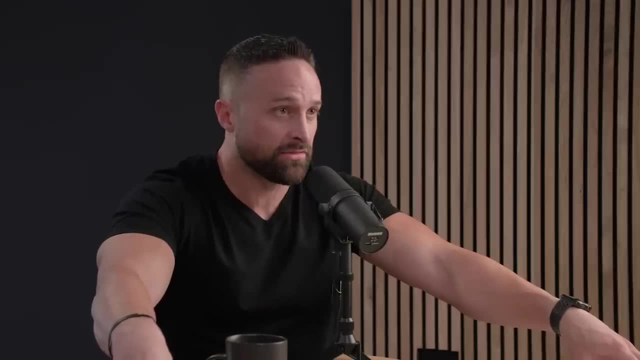 because people's step counts can spontaneously decrease when they're on a fat loss diet. They don't even realize it. So, and that again not a complete measure of NEAT, but what we've had some clients do with our team bioling coaches is they'll say: okay, you're at 8,000 steps right now. We're not going to add any purposeful cardio, but whatever you need to do to maintain that 8,000 steps do that And sometimes they have to add, you know, 15,, 20, 30 minutes of cardio because their spontaneous activity that they're not even. 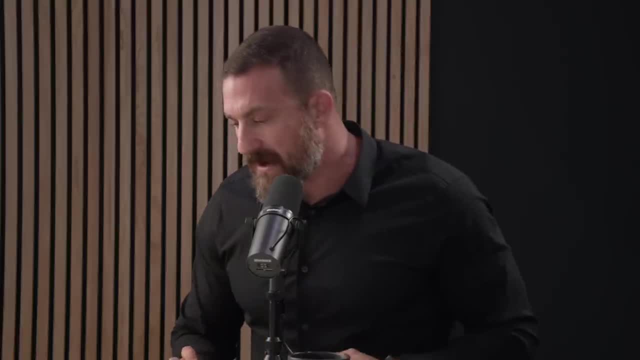 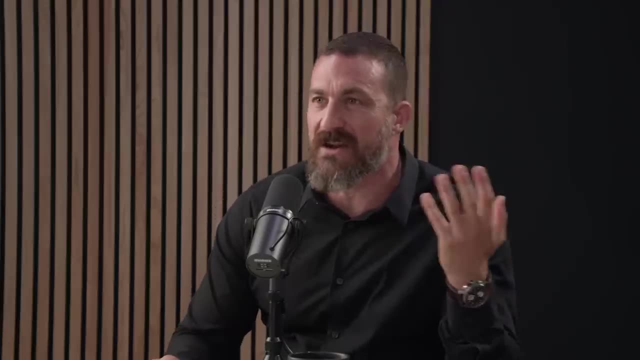 aware of goes down. That's a really excellent point. I've heard, you know, the 10,000 steps per day number was. we all heard that, And then I learned that 10,000 was just kind of thrown out as an arbitrary number. So we're like the eight hour intermittent fasting thing. There's a story. 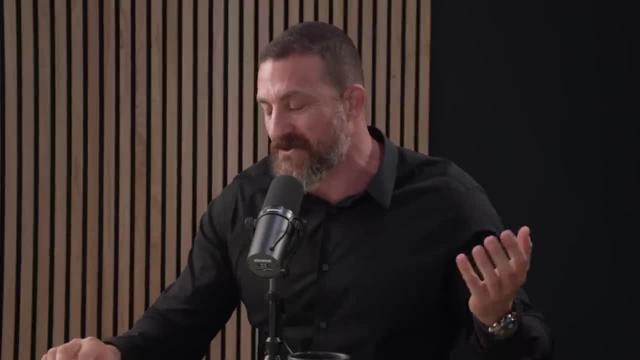 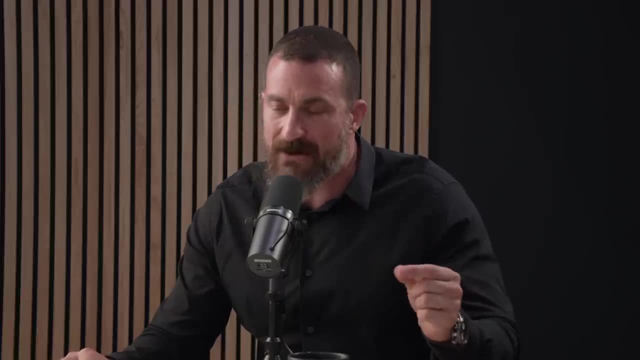 behind that, because I actually spoke to Sao Chin and it turns out that the graduate student in his lab that did that initial study- which was on mice, by the way- was limited to being in lab for about eight hours by their significant other. So the eight hour feeding window is actually the. 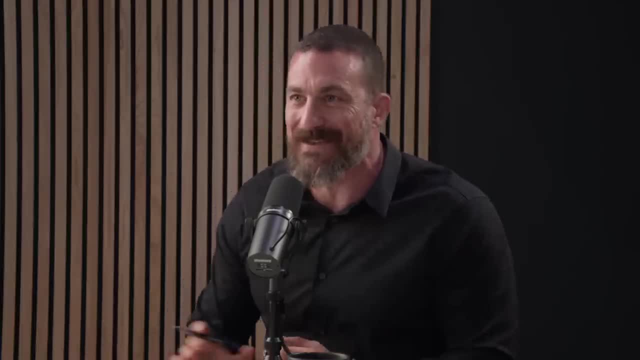 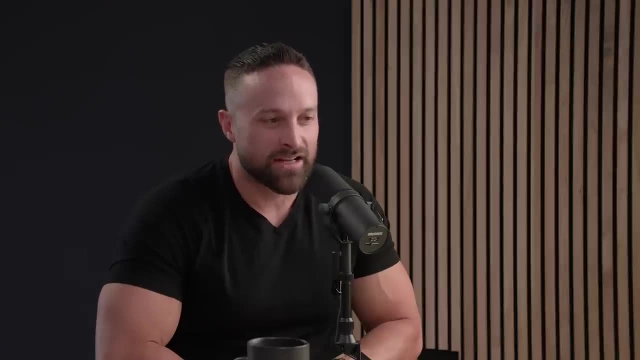 consequence of this person's relationship. That is a really great point that people don't realize when they. a lot of people will try to copy, like scientific studies, and I'll tell people like, listen, scientific studies are so confined You need to be very careful with how broadly you 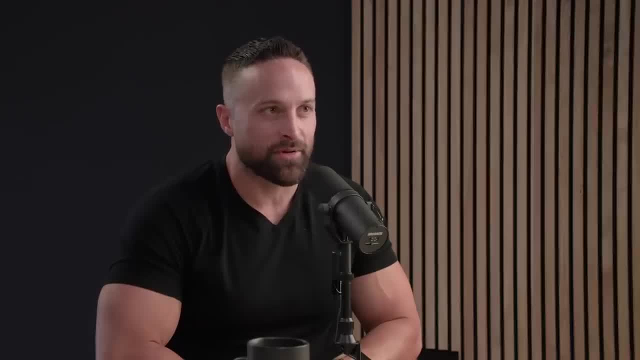 apply what's in there Right Like they're. they're a very big hammer- is the kind of the way I look at it. Okay, They're not a scalpel, They're a big hammer, And I think a lot of times in terms of coaching, scientific. 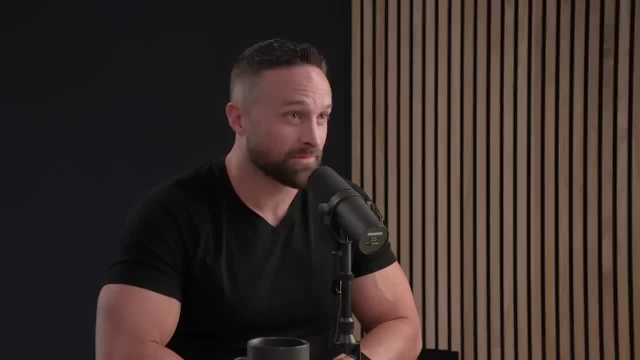 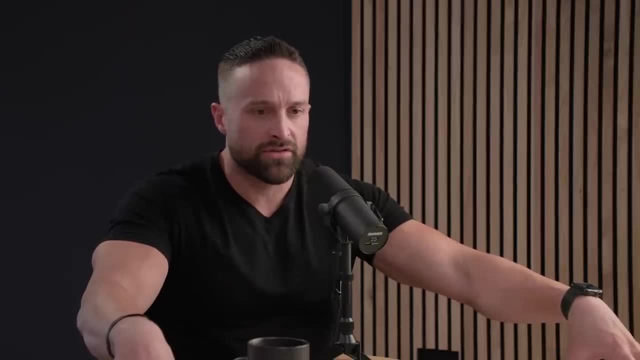 studies will tell you what not to do rather than what to do. Right, But getting back to your question about like exercise appetite. So, first off, I'm not really aware if there's evidence showing like differential effects of different forms of exercise on appetite. It's possible. 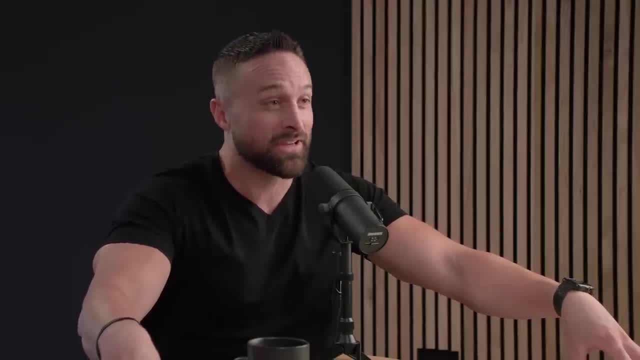 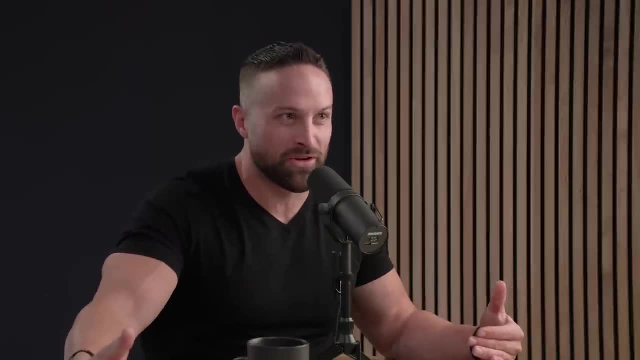 But again, look at a placebo effect, because we like, for example, you and I, grew up in an era where the muscle magazines it was like: well, as soon as you finish your workout, you can have your biggest meal of the day, Right, And you know, when I say placebo effect, I think people have the wrong idea. 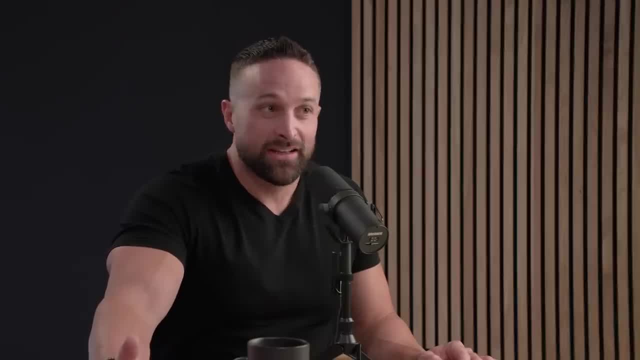 of what the placebo effect is. They think that's just a feeling. Placebo effect can actually change your physiology. People don't. people don't realize this. There's research showing that a placebo, or the power of suggestion, is basically as powerful as some pharmaceuticals, and one of the the great examples i like to use is actually: 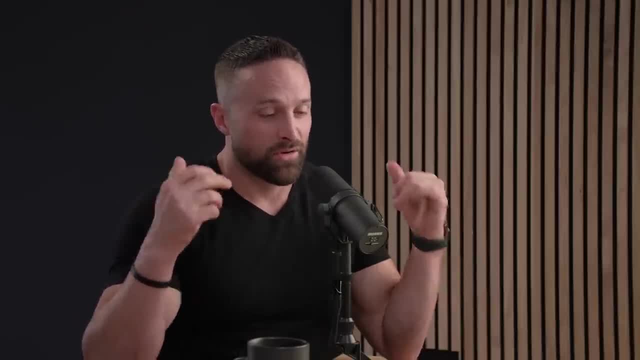 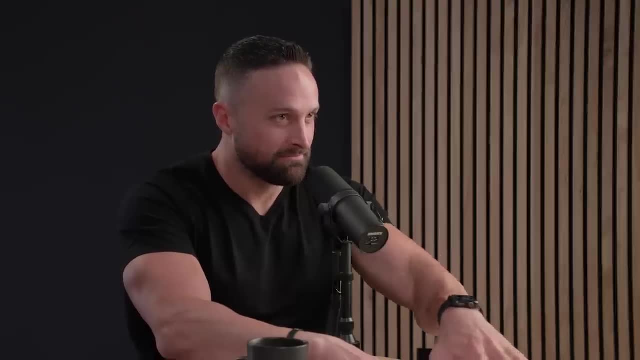 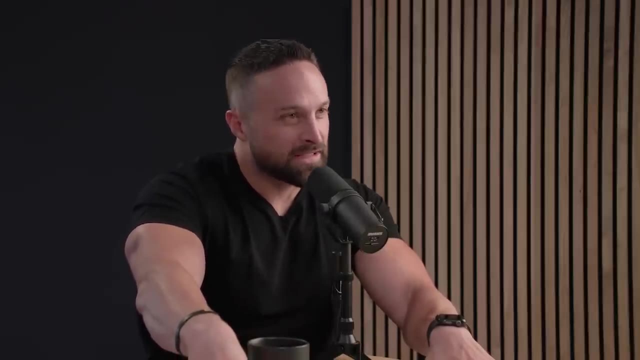 there was a study we just covered in our research review on creatine where they did um four groups: not supplemented with creatine: told they weren't supplemented with creatine. not supplemented: told they were supplemented. supplemented: told they weren't supplemented. told they were. basically, it just matters what they told them. really, oh yeah, this is incredible. 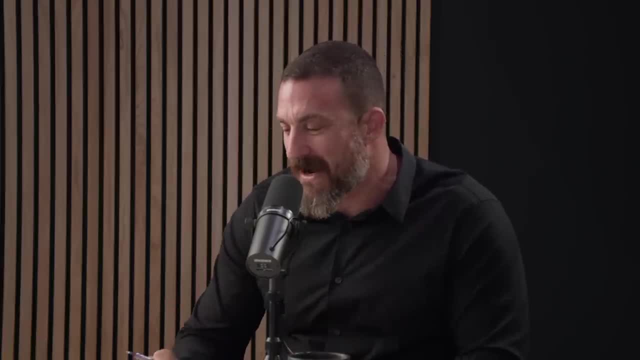 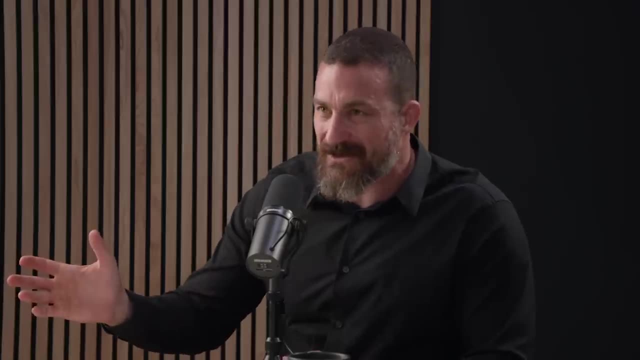 um, i have to get this study we'll so we can link to it. a colleague of mine at stanford- she's been on the podcast- i'd love to introduce you to because i think you guys, we could um really riff. first of all she was a former d1 athlete um, and then is a runs a lab at stanford in psychology. 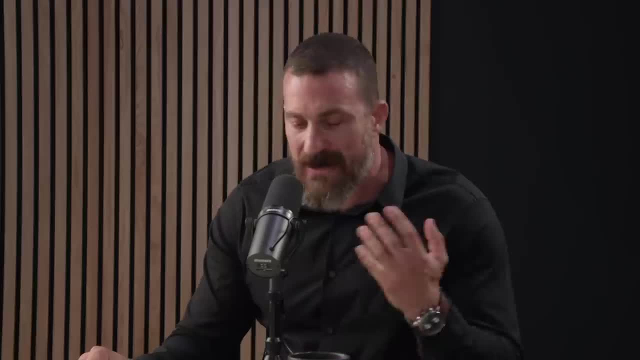 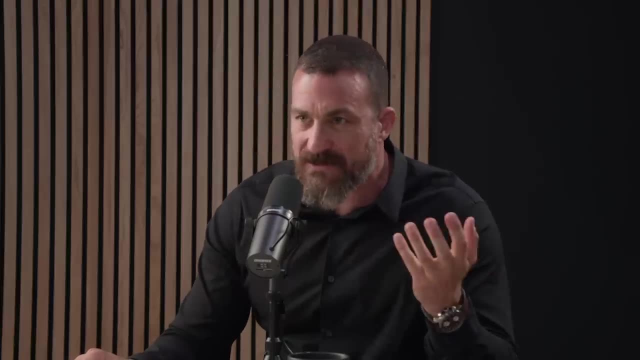 this is uh leah crumb and she's and grew up um in this, you know- very athletic, obviously, and very, very smart, and her laboratory focuses on these belief slash, placebo effects, where, if you tell people all the horrible things that stress do to you in terms of your memory and 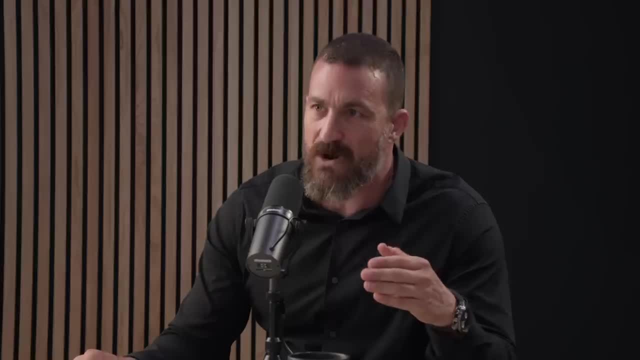 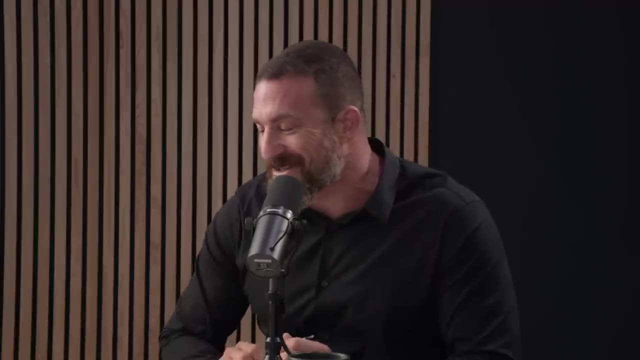 cognitive functioning and then you give them a memory test, they they perform well below baseline. if you tell them that stress sharpens them in the short term and that adrenaline is this powerful molecule that can, uh, really tune up a number of memory systems, memory improves, and it's remarkable. 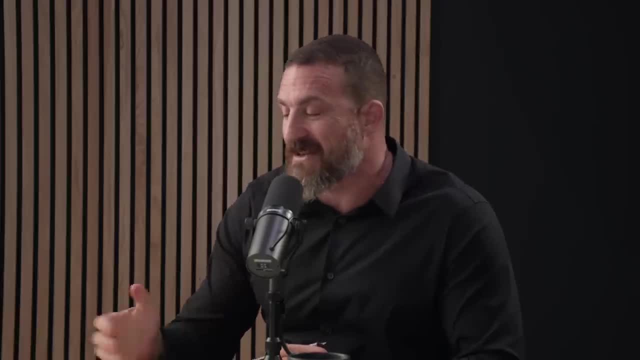 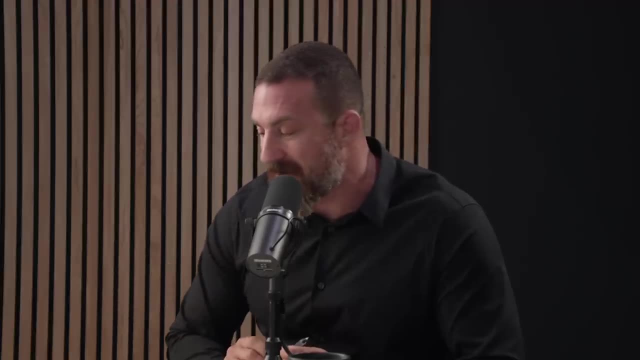 and it's consistent and uh and this, and they've done this for any number of different things, including food allergies, for instance. you know, incredible results. in any case, i i'm, i'm so glad you're bringing this up. um, i take creatine monohydrate. 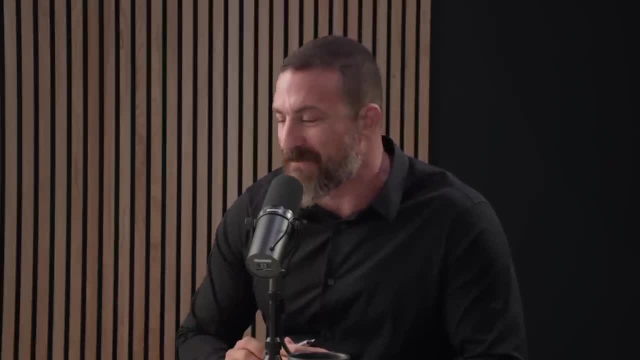 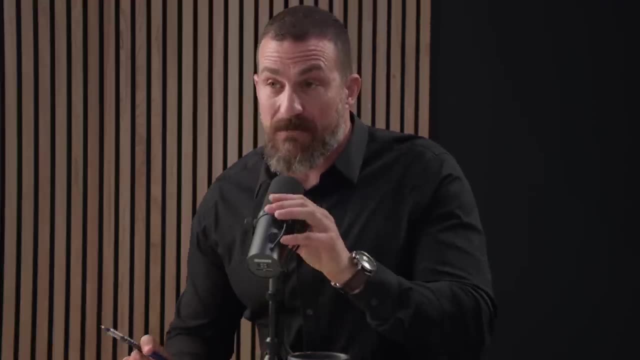 and i have for years five grams a day. i don't it's great and um and it's great and i believe it's great. so so is there a compound effect of believing it's great and it actually so? not not in this study, but so i think the thing to point out: people will misinterpret that as 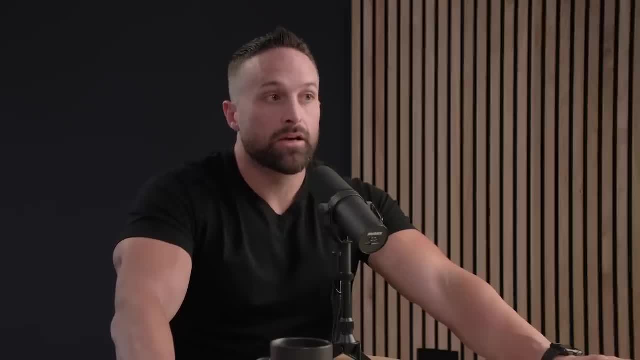 creatine doesn't work, and that's not what that says. what it says is: your beliefs about what it does are probably just as powerful as what it does, right? so, uh, they actually did a study, and i don't know if you're familiar with it, but it was, i think, within the last 10 years- where they told people 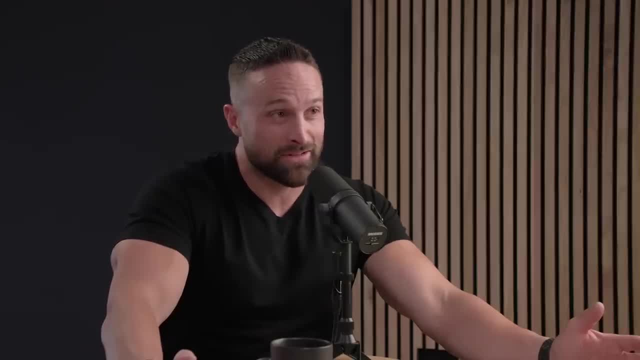 they were putting them on anabolic steroids and, wouldn't you know it, they had better gains even though they weren't actually on anabolic steroids. they had better gains than people that they didn't tell were anabolic steroids, and that's like hard outcomes: strength, lean body mass- you know those. 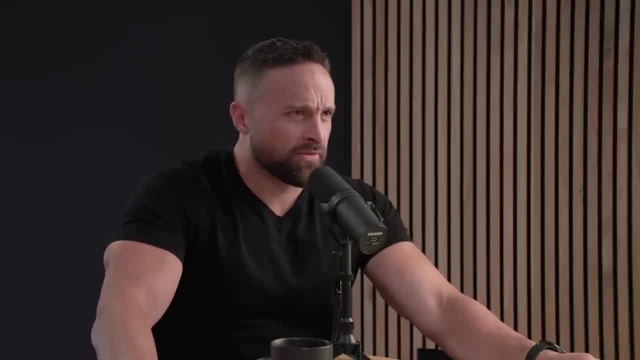 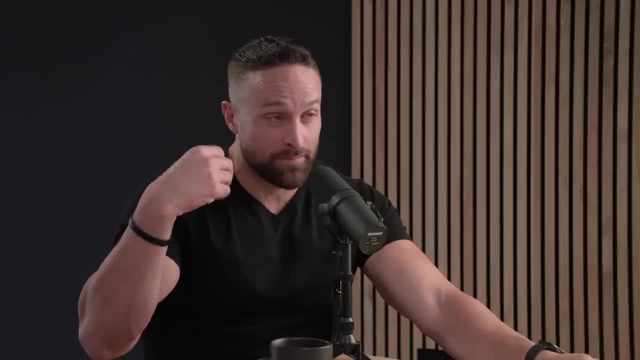 sorts of things. so when people say, well, i wouldn't fall for the placebo effect, it's like you don't have to fall for it if if you believe it to be true, the power of belief is very, very powerful. as a scientist, I wish sometimes I was ignorant so that I could subject myself to the placebo effect. 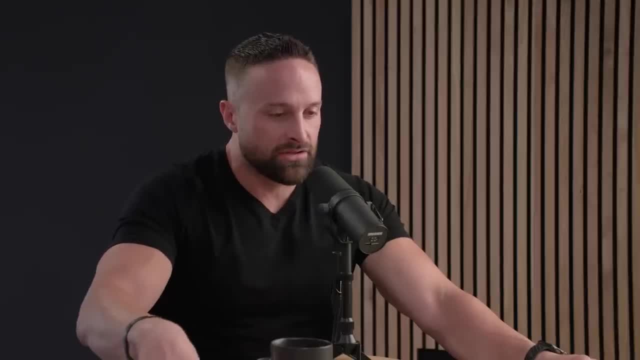 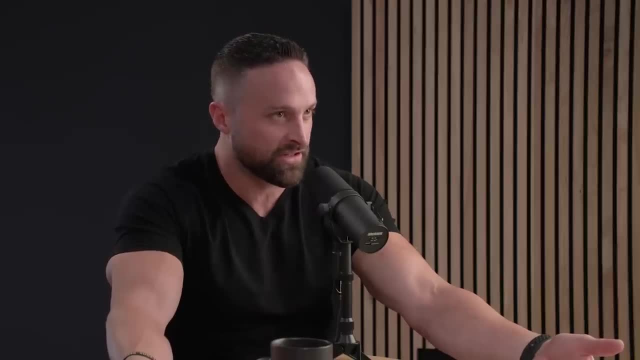 more often. yeah, absolutely, um. so kind of getting back to that's just a possible explanation of maybe why you know, and I'm the same way, like I get done with a workout, like a resistance training session, I'm like I'm ready to eat right now if you look at the literature overall on exercise. 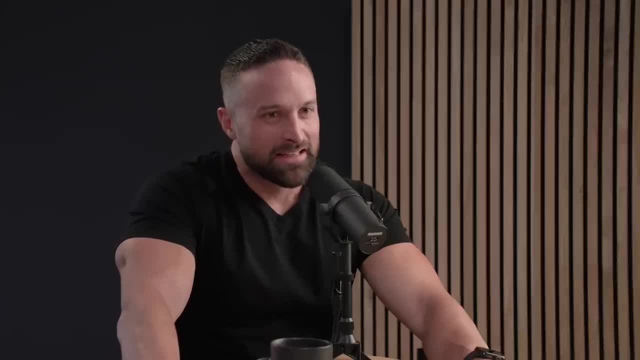 and appetite. it's not always what you'd expect. consistently, it seems to show that exercise actually has appetite suppressant effect. So people don't tend to compensate- at least fully, for the amount of movement they do, And there is some evidence that you've probably heard people say: well, 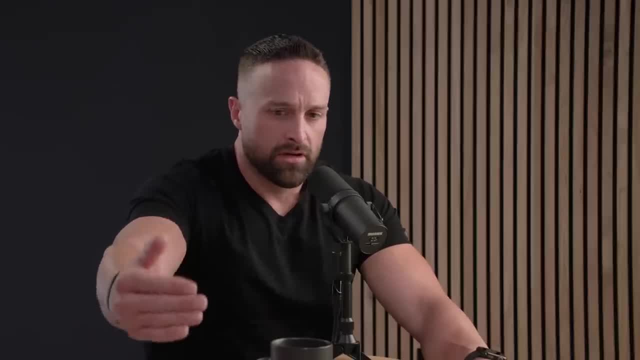 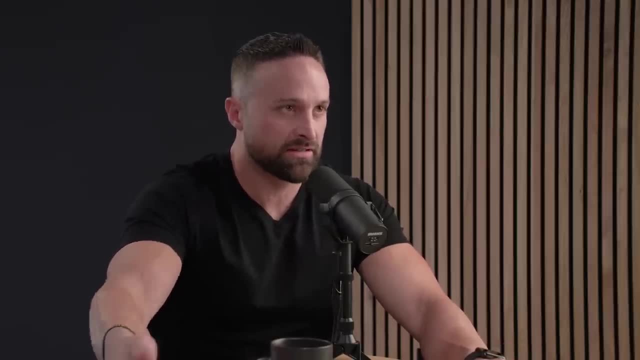 exercise is a really poor weight loss tool, right Like if you figure out how many calories you should be burning from it and you do that, you end up getting less weight loss than you would predict. I have a family member who is perfectly happy to eat less but doesn't loathe exercise. 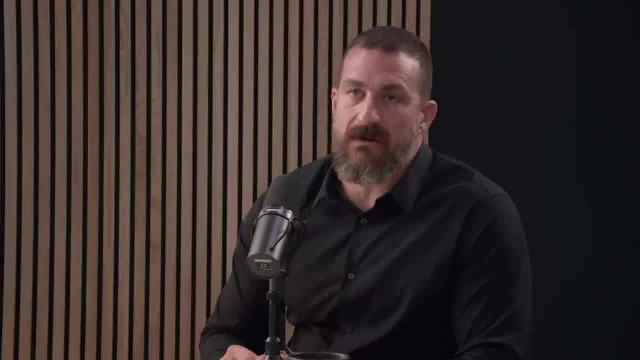 but dislikes exercise, And they're of healthy weight, but I'm always encouraging them to exercise more, And so this is an ongoing battle in our sibling relationship. Well, one thing I would say is that exercise, independent of anything that happens with your 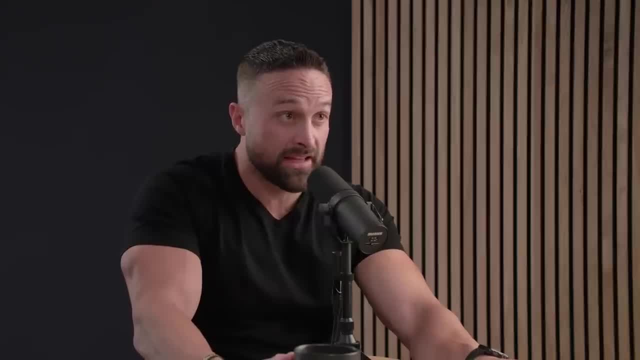 body weight, you will be healthier. So exercise is one of the only things that will actually improve your biomarkers of health without even losing weight. So there's like it'll improve your insulin sensitivity, inflammation, all that stuff. So everybody out there looking for a healthy weight loss tool. I would say exercise is one of the only things that will actually improve your biomarkers of health without even losing weight. So there's like it'll improve your insulin sensitivity, inflammation, all that stuff. So everybody out there looking for a healthy weight, 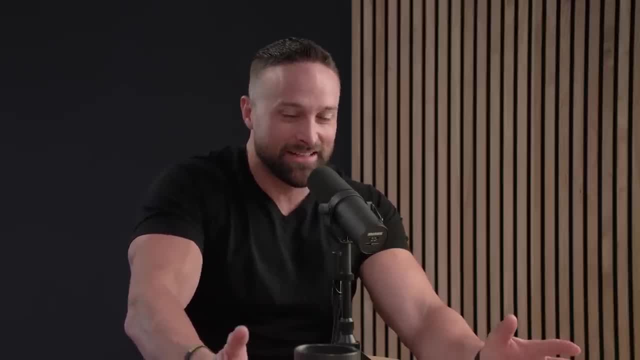 loss tool. I would say exercise is one of the only things that will actually improve your that. to be healthier, exercise is the hack, Yeah, Crucial point, And our mutual friend Dr Peter Attia, I think, has gone on record. 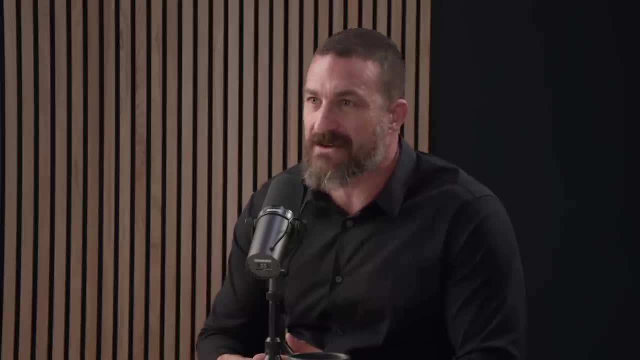 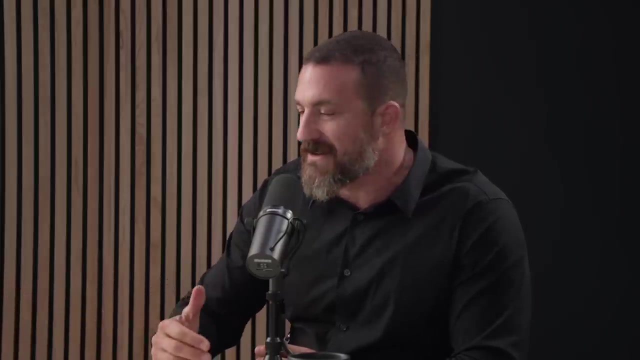 several times now saying that of all the things that one could take- NMN, et cetera, metformin of all, regardless of whether or not one takes those or doesn't take those- that the positive effects on longevity by way of biomarkers from regular exercise is far outweighs all of those. 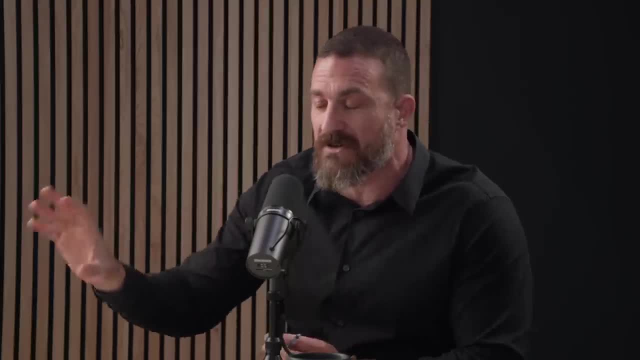 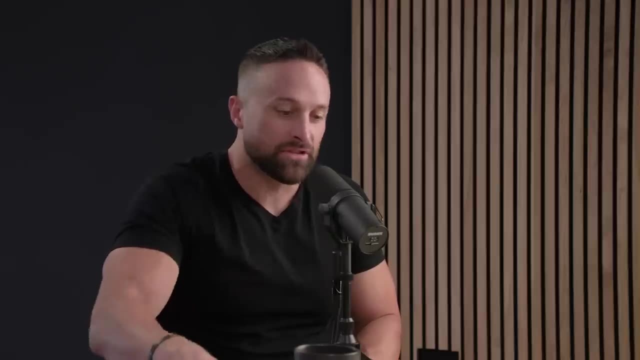 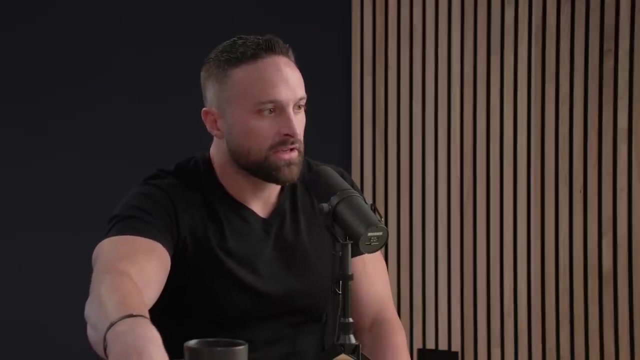 things combined. Not that those things don't necessarily work, but we're not going through them in detail now- but that exercise is by far the best thing we can do for our health span and lifespan. Yeah, absolutely, I 100% agree. And when you're talking about weight loss, people miss the point of exercise. I think there's some work that came out from Herman Ponser as well that basically showed like: well, if you do 100 calories from exercise, you have a like 28 calorie reduction in your basal metabolic rate in response to that. 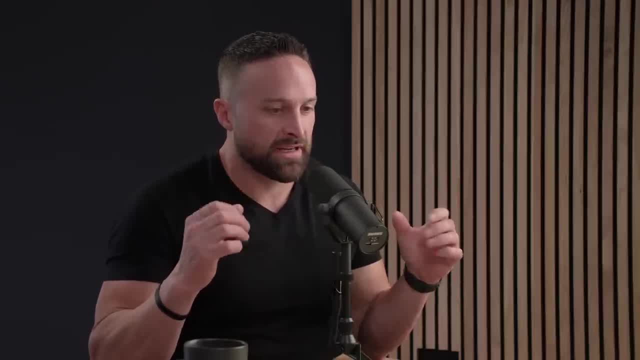 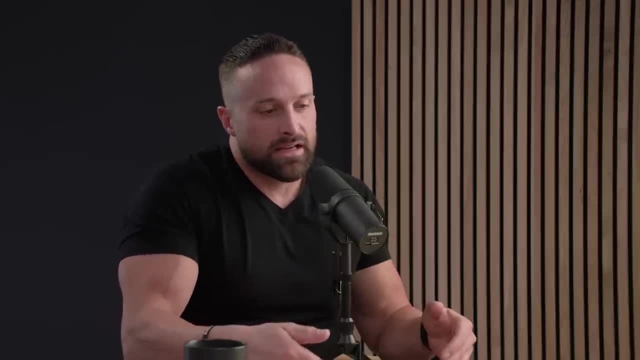 So it's kind of like this constrained energy expenditure model, right. But what I would say is okay. well, there's still a net of 72, right, So it's still okay. And the other thing is, I think the effects of exercise on weight loss are actually more due to what it does to appetite. 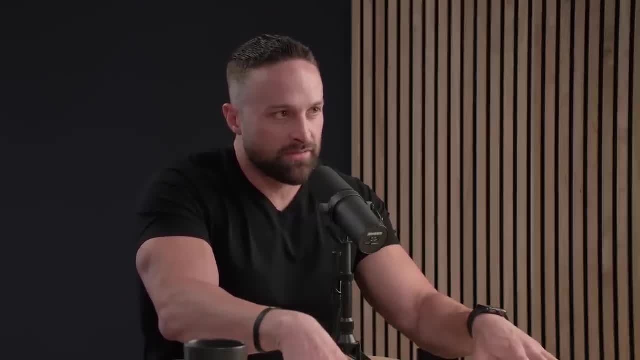 So if you look at people who lose weight and keep it off for a number of years- kind of outliers, because most people don't keep it off for years- over 70% of them engage in regular exercise- Of people who do not- Of people who do not keep weight loss like maintain weight loss less than 30% exercise regularly. So now that's just a correlation that doesn't necessarily prove causation, But there are some pretty compelling studies showing that exercise increases your sensitivity to satiety signals. 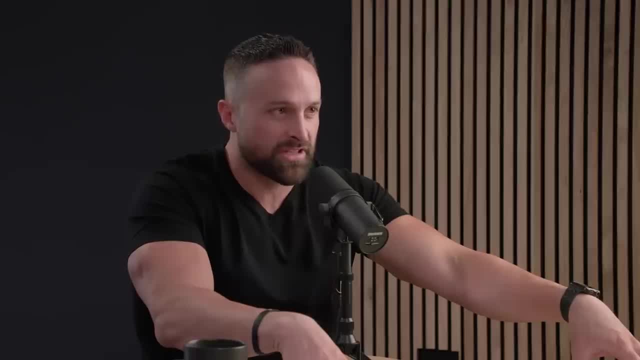 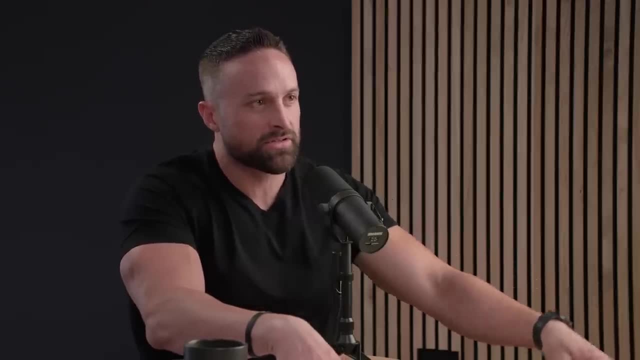 So basically, you can have the same satiety signals but you're more sensitive to them when you exercise. And there's actually a really classic study from the 1950s in Bengali workers where they looked at basically: So basically, you can have the same satiety signals but you're more sensitive to them when you exercise. And there's actually a really classic study from the 1950s in Bengali workers where they looked at basically: 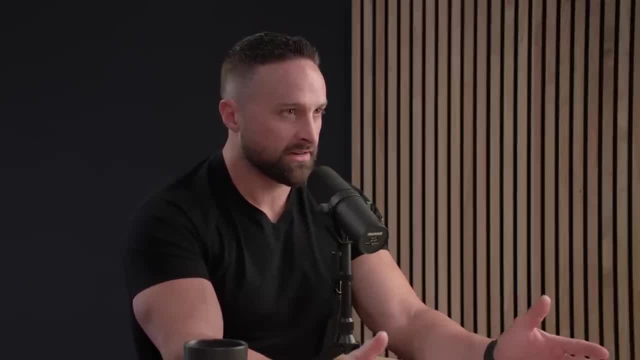 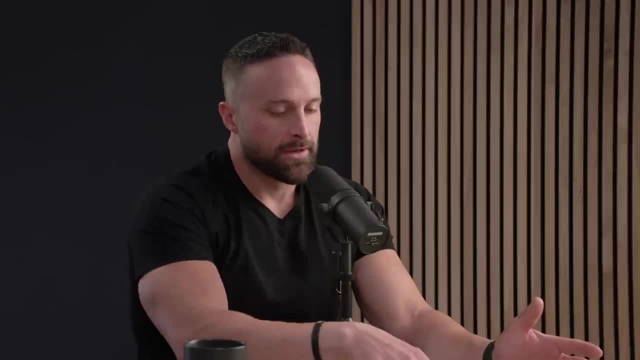 four different quadrants of activity. So you had sedentary, lightly active, moderately active, heavily active, basically based on their job choice, And they didn't have an intervention. They just wanted to track them and see how much, you know how many calories did they actually eat. So it was like a J-shaped curve. 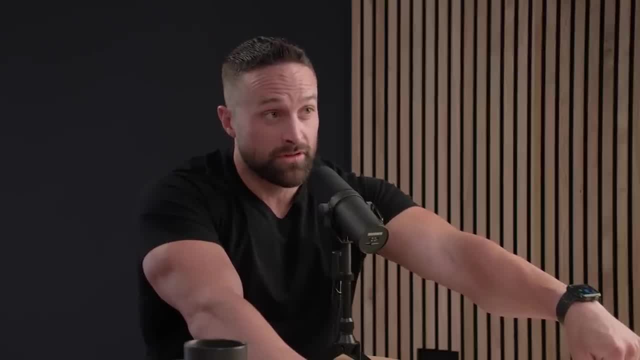 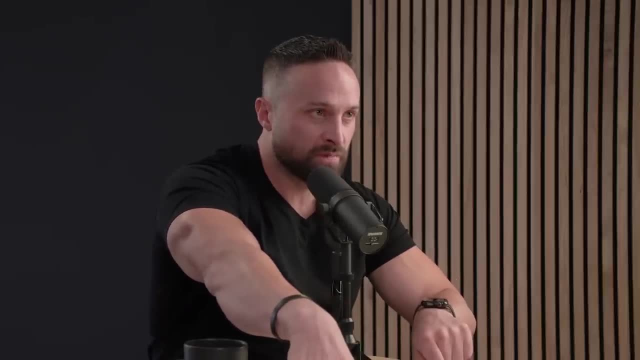 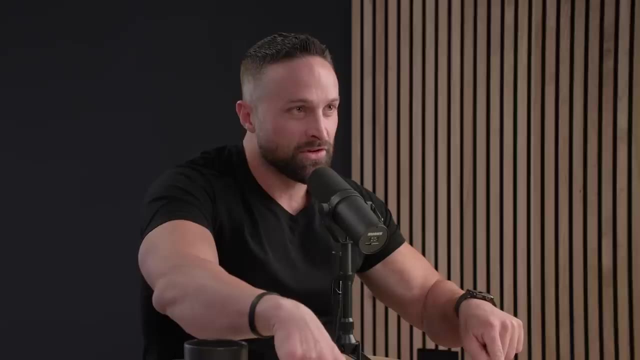 So the sedentary actually ate more food than the lightly active or moderately active. But from lightly active to heavily active they almost perfectly compensated how many calories they should be eating. So to me that suggests when you become active you can actually regulate your appetite appropriately, or much more appropriately than if you're sedentary. 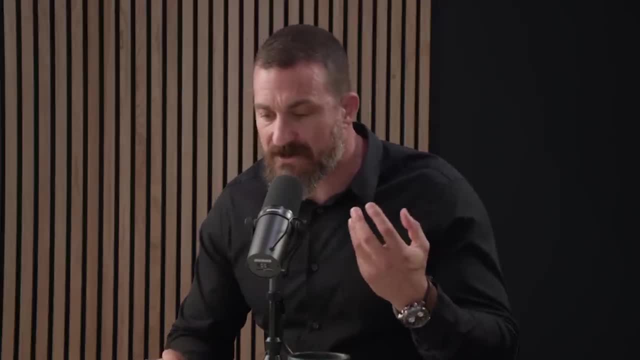 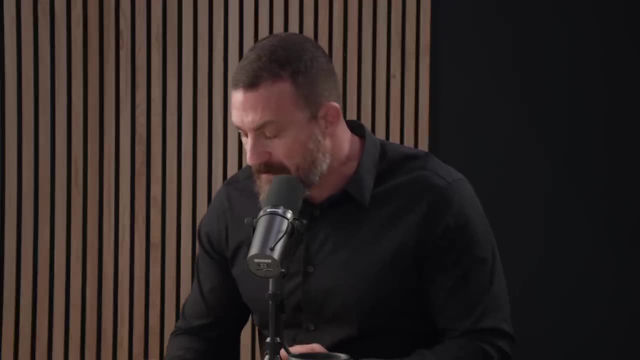 And do you think this has to do with changes in the brain brain centers that respond to satiety signals from the periphery, And or do you think it has to do with changes in blood sugar regulation? What I was taught- and I don't know if this is still considered true- is that you know spikes in blood. Sugar will trigger a desire to eat more, even though it's kind of exactly the opposite of what you need when you have a spike in blood sugar And there's this kind of- and we'll get into this when we talk about artificial sweeteners. 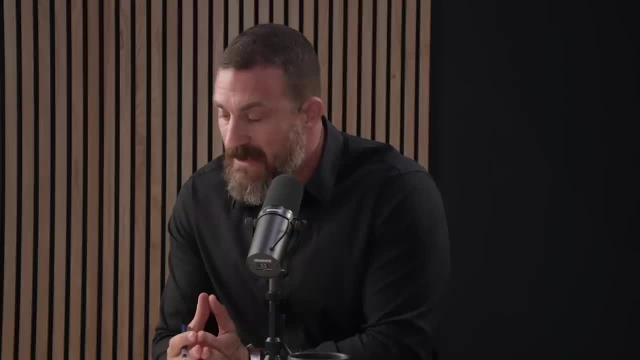 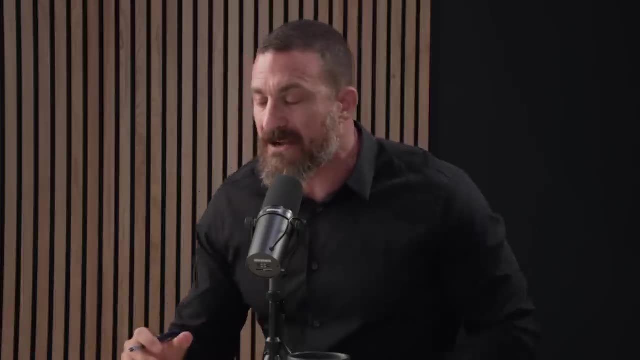 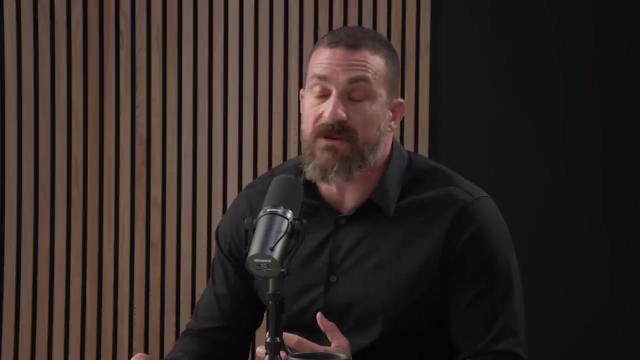 This is the idea in mind I think I adopted- perhaps falsely- that you know you eat something that's sweeter, that tastes really good, And you are suddenly on the train of wanting to eat more, And I could imagine how exercise, if it is increasing the satiety signals, could be working in a number of different ways. 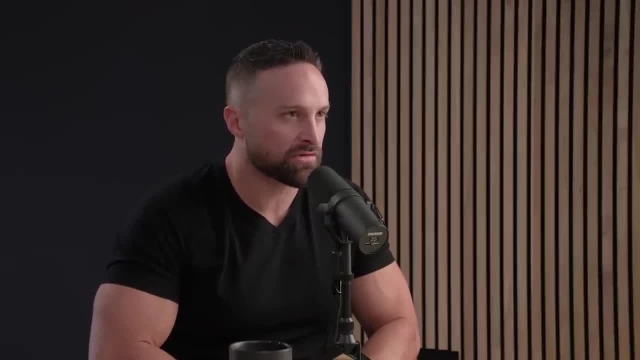 Yeah, I think it's a. I think The effect is probably mostly at the brain level. You know the effects on blood sugar. The research out there is not very compelling for blood sugar driving appetite. Now, if you become hypoglycemic, yes you'll, you'll get hungry, but it's a different kind of hunger than like your, normal. like I feel kind of empty and my stomach's growling. like those are, they can go together. But usually, like the hypoglycemia is like I am hot, I feel like I'm Going to pass out, like you want to eat something, not because your stomach's crawling, but because you know that you just need some fuel. 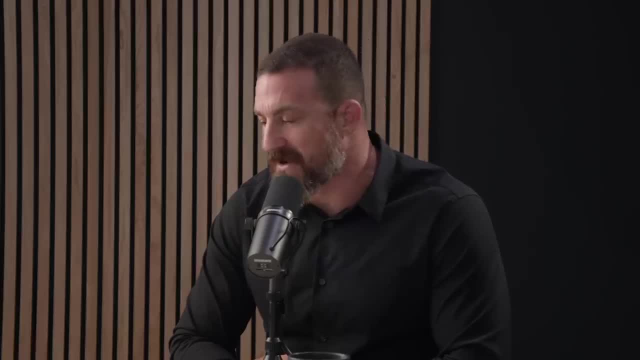 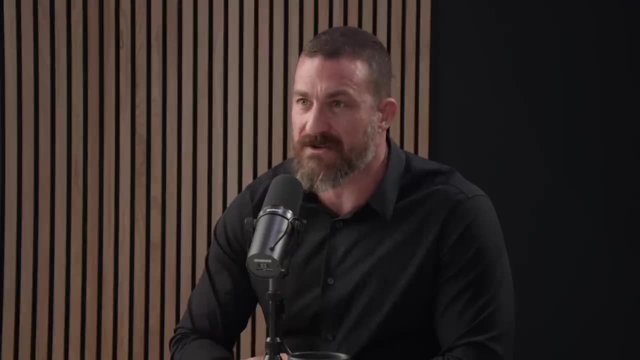 It's like you're getting pulled under. Oh yeah, I've been there. I've been there when I've done longer fast- something I don't do anymore- and drank a lot of black coffee. There was probably an electrolyte effect there, because coffee, as you, excrete sodium and other electrolytes and then just feeling like I needed something. 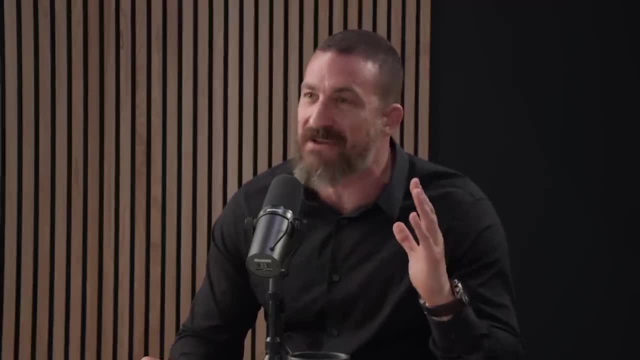 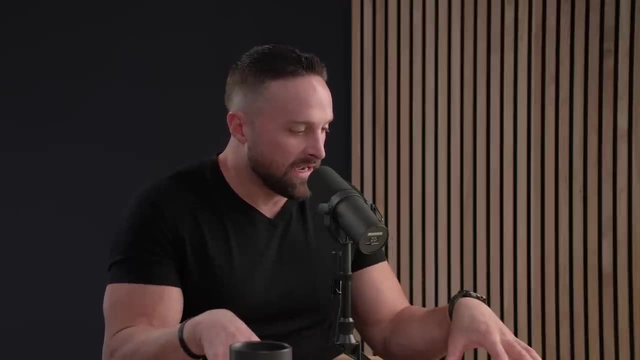 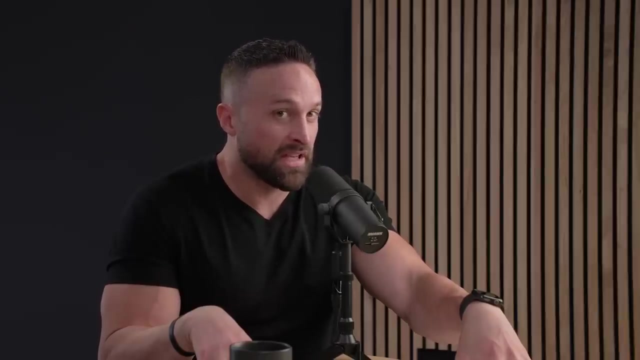 This whole thing like I need something. that's kind of desperation. I never want to be back here again. Hypoglycemia is very Uncomfortable, not fun. So you know again when they. and then when they look at you know actual randomized control trials of implementing some exercise where they're, you know pretty controlled environment. they typically see people if, if anything, they eat less as opposed to eating more. 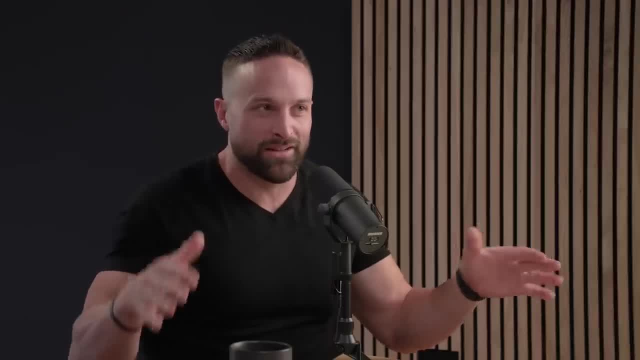 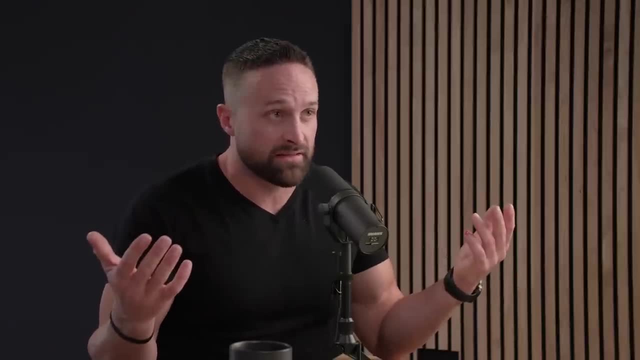 Now some people again, that's. you know, studies report averages, right, And there's individual data points. So there are some people who, at least anecdotally, report that exercise Makes them more hungry. That's completely valid. 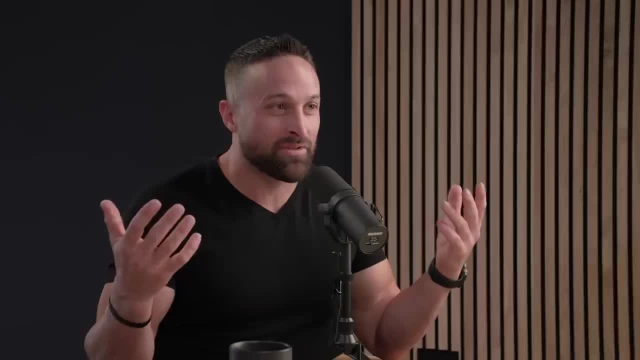 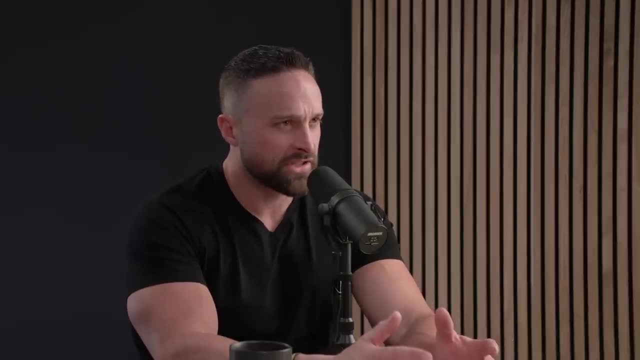 It's now. it could be their beliefs around it. It could be a number of different things, but it's important to understand that there is individual variability, And I think one of the things that I've learned to appreciate more is not trying to separate psychology and physiology. 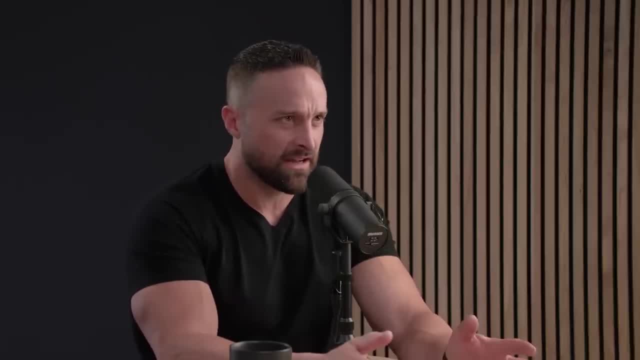 We do this a lot And so well, I want to know the physiology. I don't care about the psychology of it And now I'm kind of appreciating more. psychology is physiology. you know that, like with most things now, we have kind of. 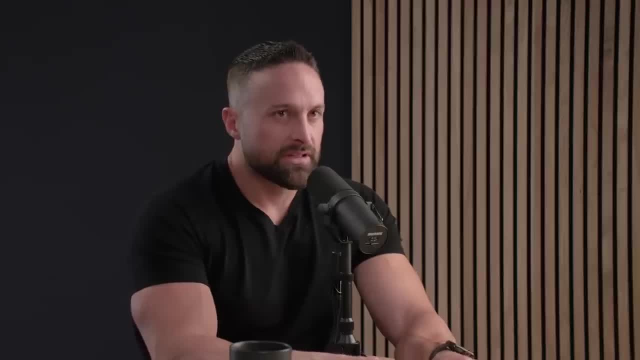 The biopsychosocial model, and I'll give you an example of this. A lot of people get really caught up with appetite, and if we could just suppress people's appetite, that's part of it. But people don't just eat because they're hungry. 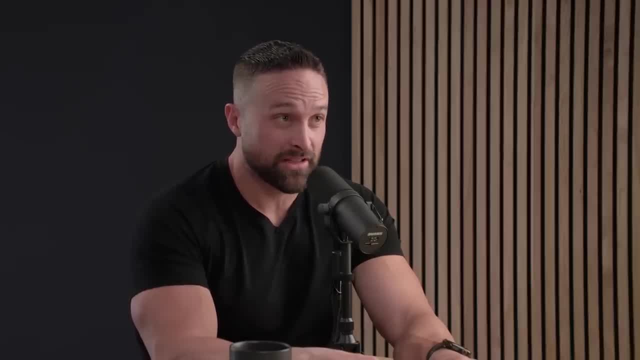 They eat for a lot of different reasons, social reasons especially So. can you remember the last social event you ever went to that didn't have food? No Right. If you look at dinner plates from the 1800s, they're about this big. 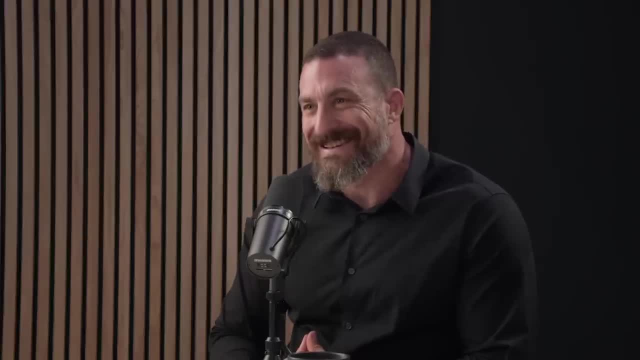 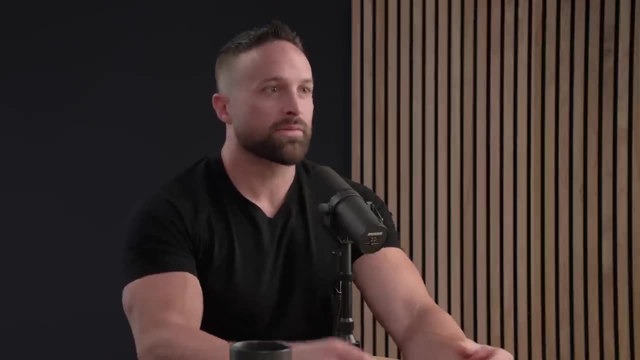 Yeah, Yeah, Yeah. How big are dinner plates? The whole buffet, Right, Right, Yeah, Um, if you there's situational cues, right, You're sitting down to watch TV. oh, grab some popcorn, grab some you know, snack, whatever. 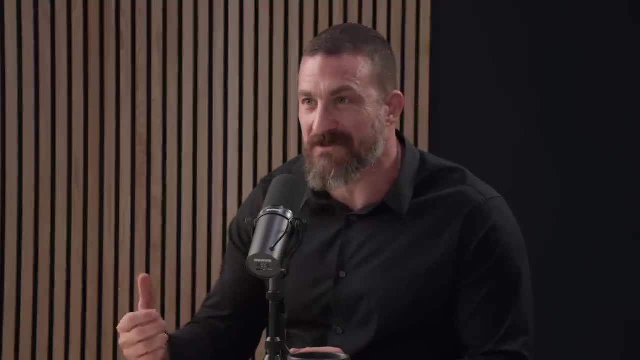 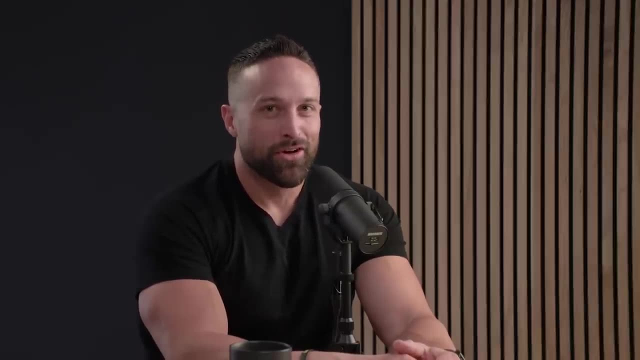 I even see this with you know how one person will pick up their phone and then everyone picks up their phone. I think there's a similar effect with food. Yeah And same thing, right, Like how many times have we either done it ourselves or been experienced people saying: oh, you should have some, you should have, like you know. 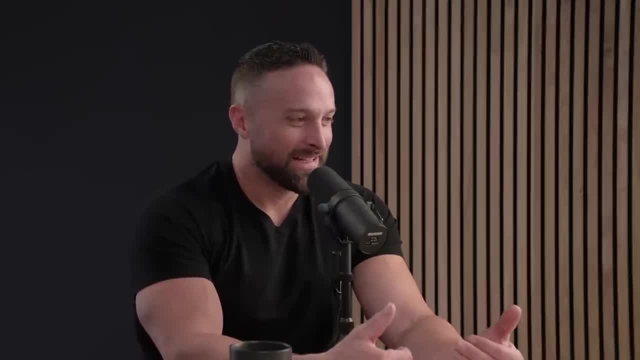 Alcohol especially right Like people will. um uh, I was hanging out with somebody last night and I had a beer and they just had, you know, a water and I'm like I feel no need to try and convince them to do that with me. 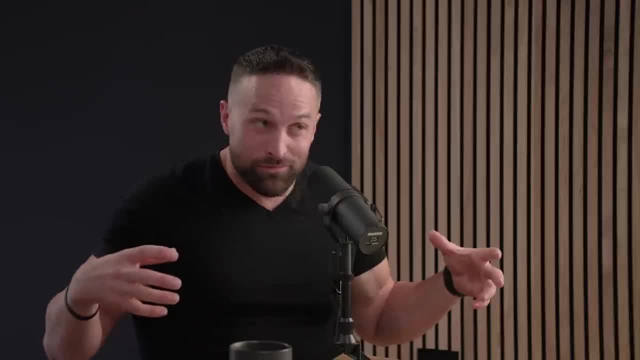 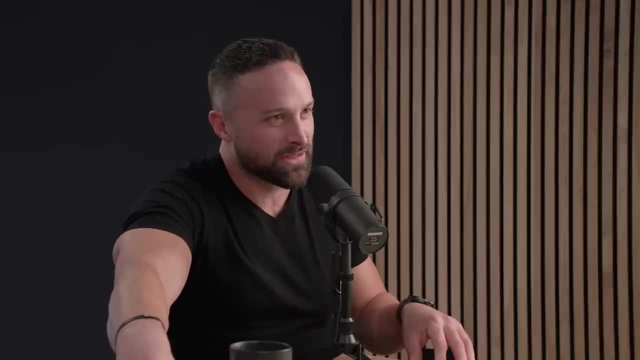 You know what I mean. But as humans, you know we're- we're kind of hurt animals, Like we don't want to be doing something out on isolation, on our own. Now I'm, I'm- this is a very tenuous, I guess, belief of mine, but you know- doing things alone. 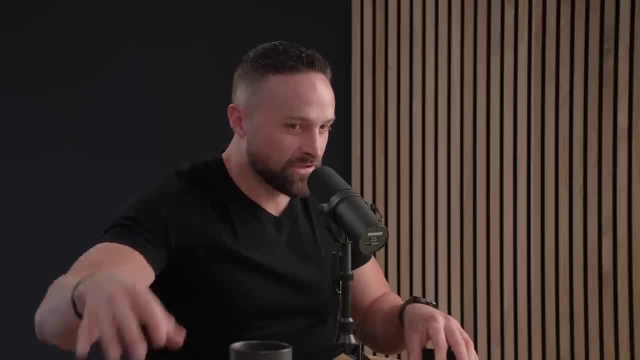 In isolation. you know, during kind of you know ancestral times that's going to set off your alarm system. you know, because if you don't have other people you can't protect yourself right. So typically things were done together in groups. 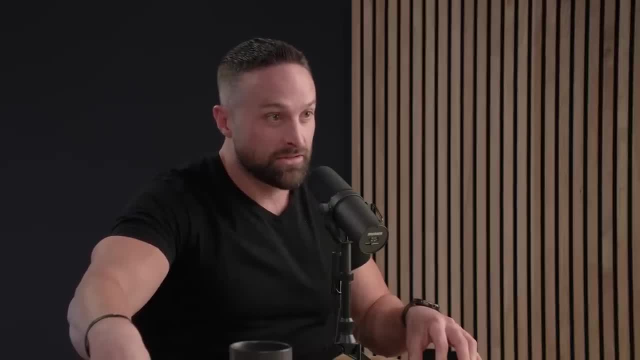 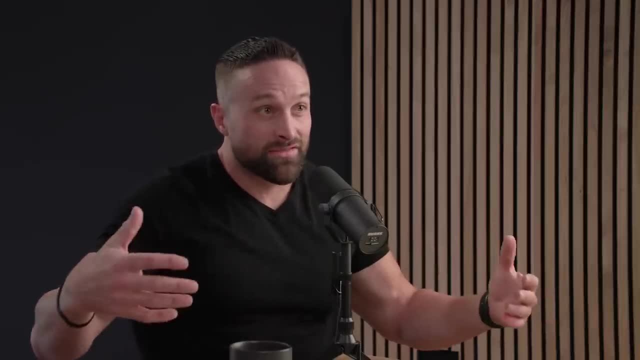 And I think that's a lot of the reason why we tend to be just tribal in nature about a lot of things, right? So the whole point to that is, you know, on the list of reasons why people eat, I mean, I've gotten better. 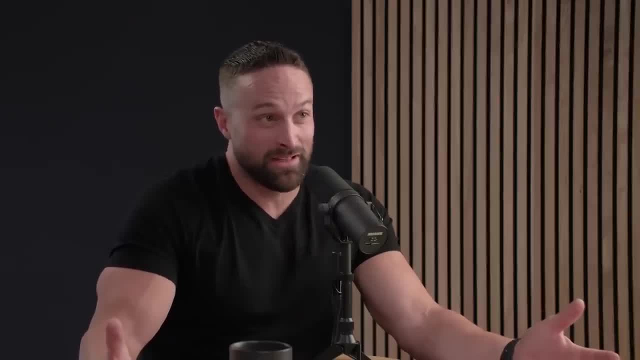 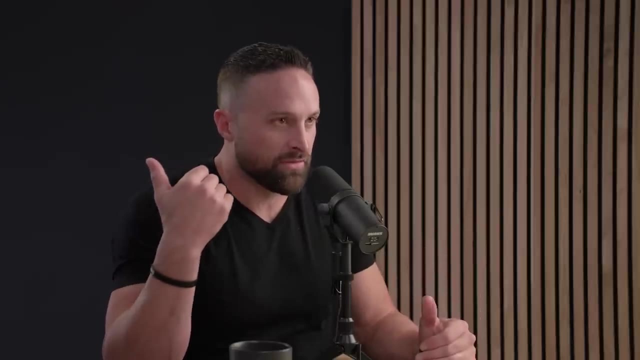 I've gotten better. I've gotten better The point where I think that hunger is actually not even the main reason people eat. uh, you know, stress, um lack of sleep, boredom, boredom, Yeah, absolutely So, unless you know we can do something that addresses all those things. um, there's a, there's a line from a review paper. 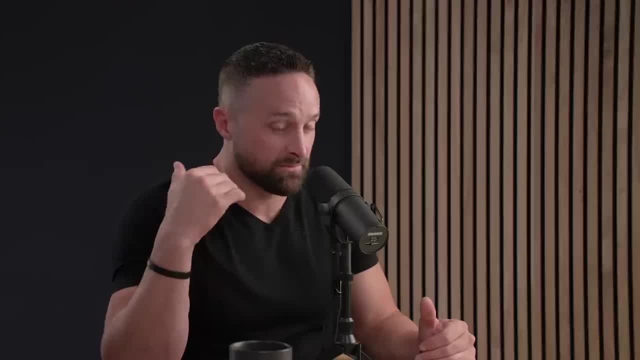 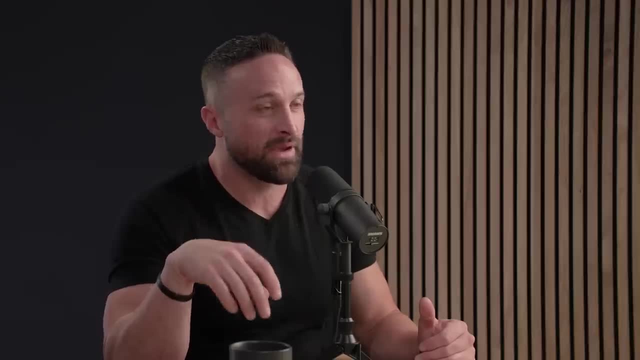 This review paper came out in 2011 by a researcher named McLean, And it's the best review paper I've ever read. It was called a biology's response to dieting, the impetus for weight regain and basically went through all the mechanisms. 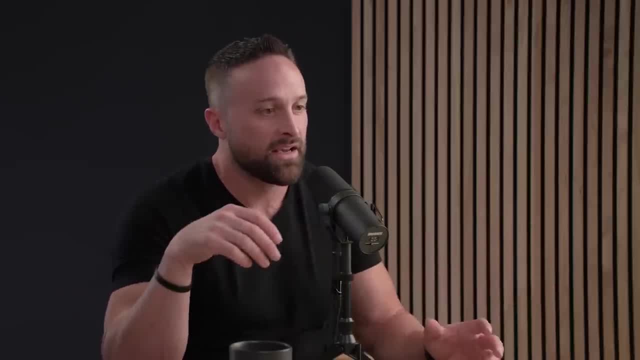 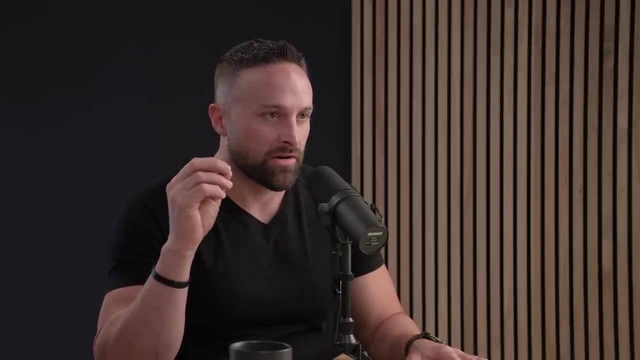 Of these adaptations that happen during fat loss diets and how biology's response is. to try to drive you back to your, your previous, and I'm going to butcher the quote, but at the end of the study he said: basically, the body's systems are comprehensive, redundant and well-focused on restoring depleted energy reserves. 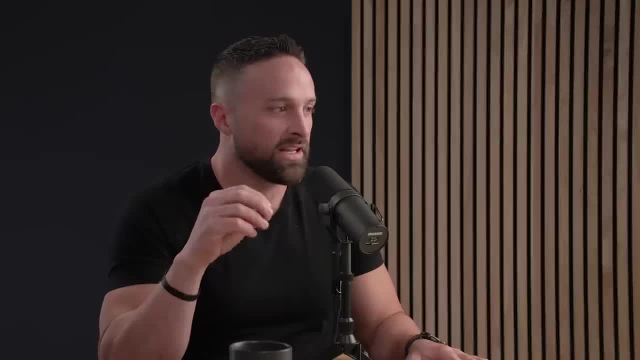 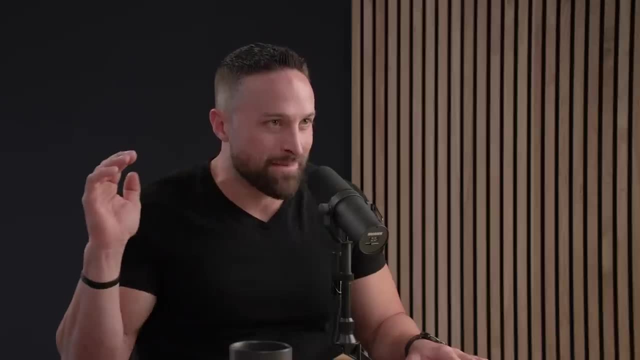 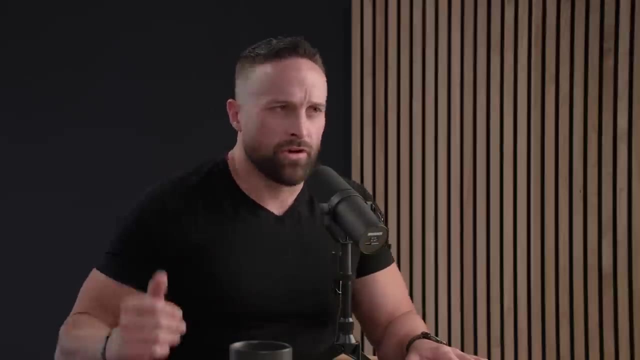 And any attempt or any kind of strategy for weight loss That doesn't attempt to address a broad spectrum of these things is going to fail, And so that's why when people say, well, just do low carb, you won't be hungry, 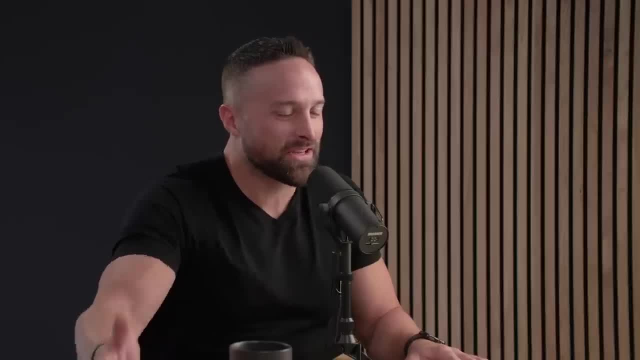 I'm like, yeah, but people don't just eat because they're hungry. So I think really like trying to get outside the box and think about these things, And especially when you read some of the literature. I recently read a systematic review of successful weight loss maintainers, which I thought was really interesting. 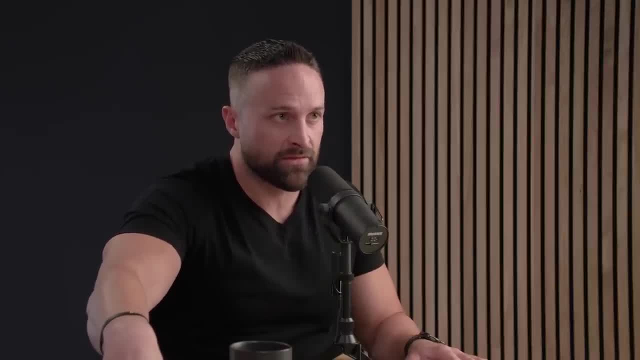 Um, so they took people who had lost a significant amount of body weight and kept it off for for I think it was three years, and they basically asked them questions and tried to identify commonalities, And there were some things that I expected, like cognitive restraint. 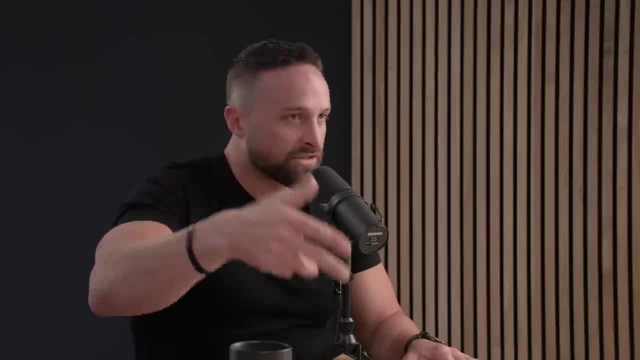 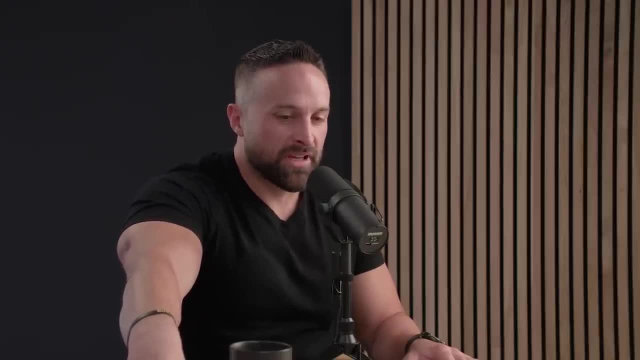 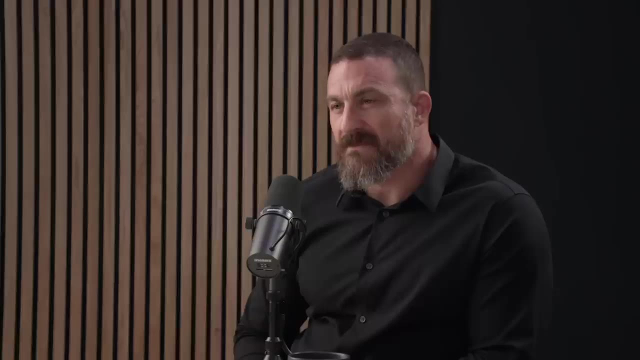 self-monitoring. um, you know exercise. And then one of the things they said that I found really fascinating was pretty ubiquitous between people. They said I had to develop a new identity. So are you familiar with Ethan Supley? No, 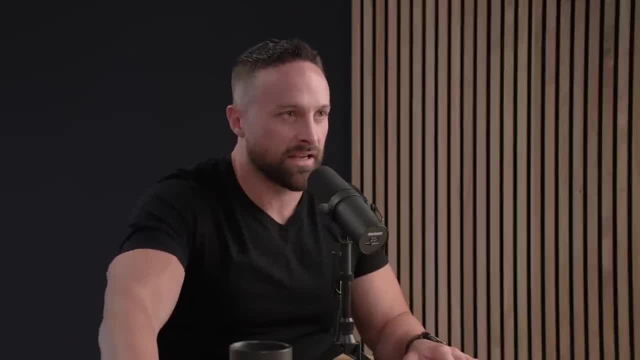 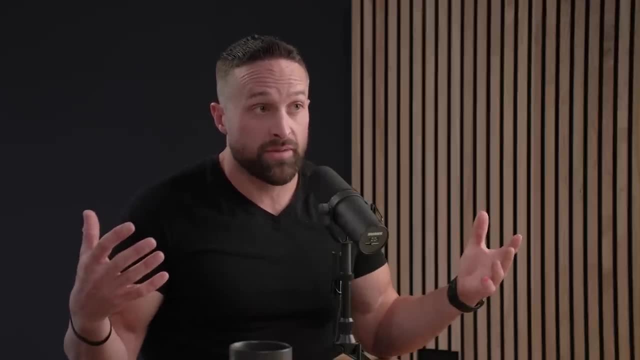 So Ethan is a actor. He's been in like remember the Titans and American history X? I certainly saw American history X. Yeah, So he was. he was very large, Like he was like 550 pounds and now he's like two, 30 and jacked. 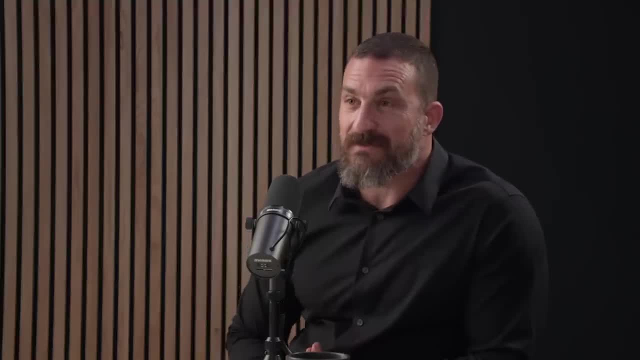 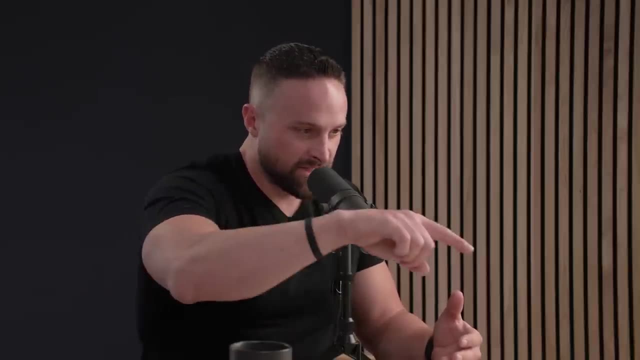 Wait, he was five. He was how? 550 pounds, Wow, Um, and he has it. whenever he puts up posts on his Instagram of him training, it'll say: I killed my clone today And I asked him like: is this what you're talking about? 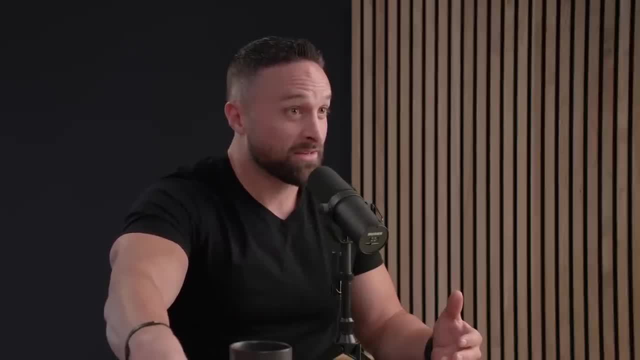 Like creating a new identity. And he said: this is exactly what I'm talking about, because I had to kill who I was, because there was no way I was going to be able to make longterm changes if I just didn't become a new person. because there's 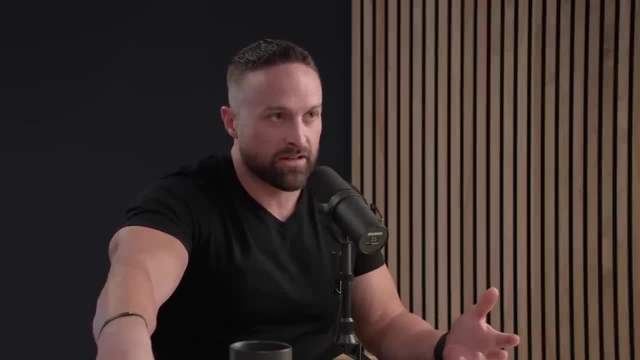 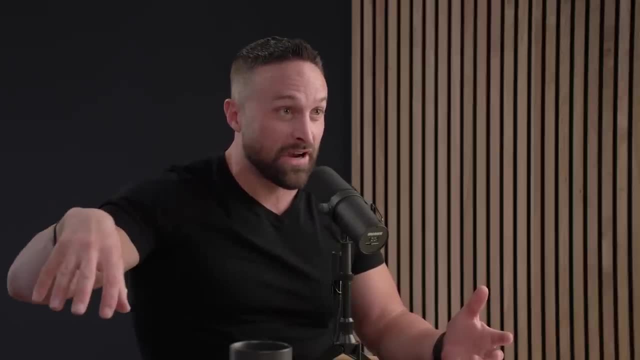 I mean an addicts talk about this right, Like um people who are alcoholics. they had to get new friends. They had to hang out at different places because their entire life had been set up around this lifestyle for alcohol, And I would actually argue that Yeah, Eating disorders or disordered eating patterns is much harder to break than other forms of addiction. And think about food addiction. Well, in some ways, bulimia and anorexia are still addictions. You can't stop eating Like if you're alcoholic. 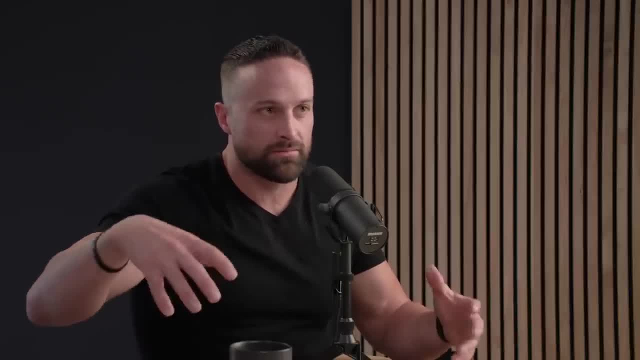 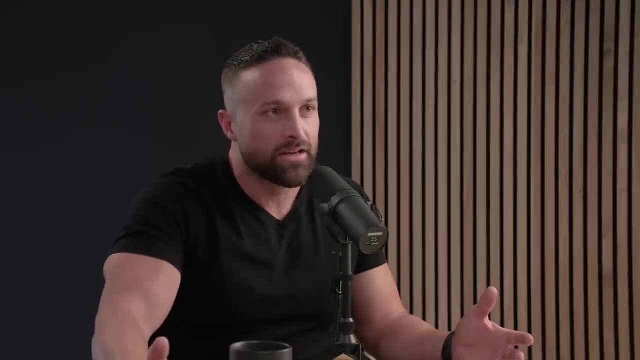 you can abstain from alcohol. If you become addicted to, say, cocaine, you can abstain from that. You can never abstain from food. And so now imagine telling a gambler, a gambling addict: well, you've got to play this slot. 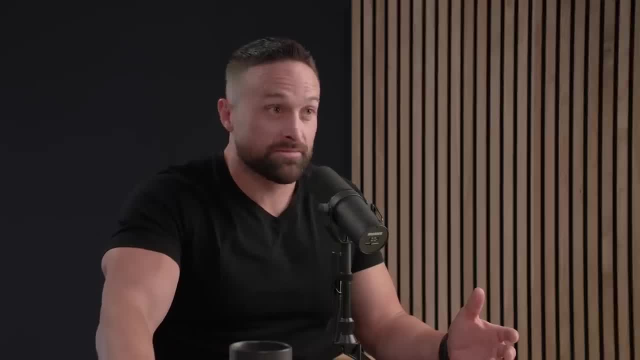 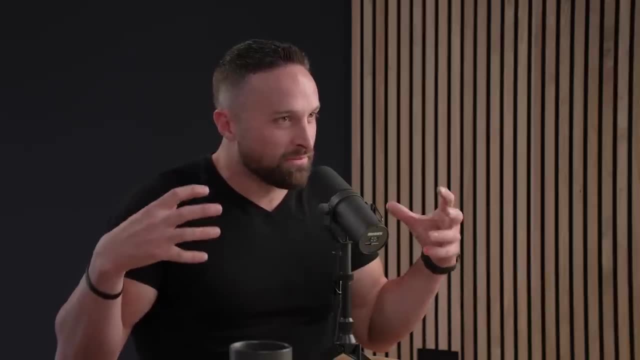 you know, a couple of times a day, but no more like that's. that's really challenging. So, um, yeah, I just like all this stuff. It's so important to be comprehensive with how we treat these things. These are incredibly important points. 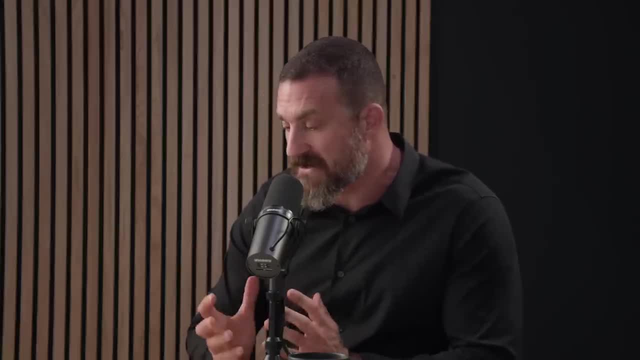 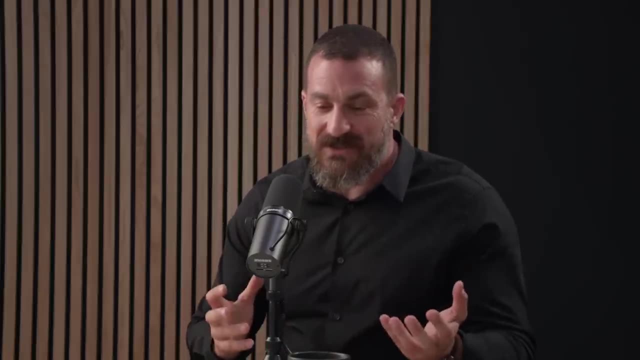 And, to my knowledge, I don't think anyone has really described it in a cohesive way the way that you're doing here. So important for people to understand this because obviously, as a neuroscientist, I think you know the nervous system is creating our thoughts. 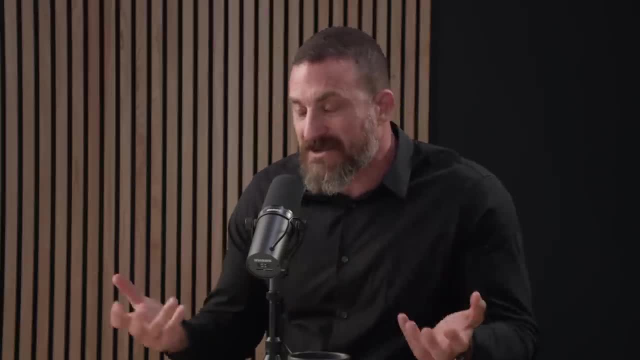 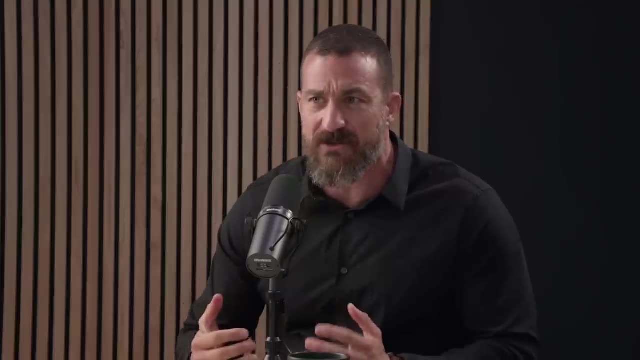 Our thoughts are and feelings are related to psychology And therefore, of course, our physiology and our psychology are one in the same. It's bi-directional. Now there's nowadays there's a lot of interest in brain, body, in particular gut, brain access. 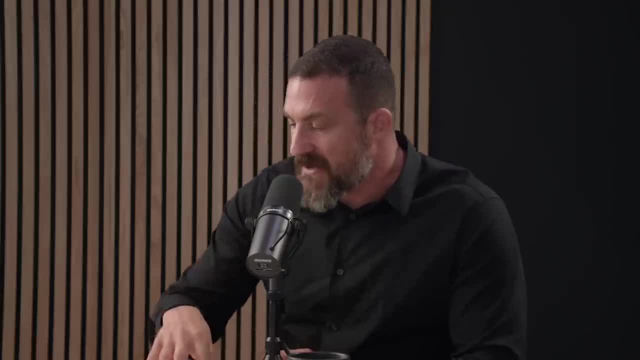 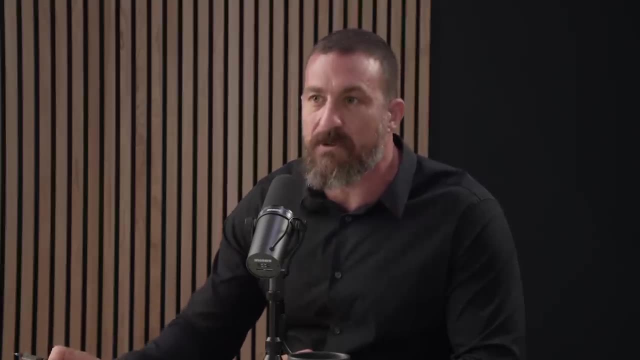 And we we can talk about that, but I I really appreciate that you're spelling out how there are these different variables. Each one can account for a number of different things. Exercise clearly has a remarkably potent defect, both during the exercise, in terms of caloric burn. 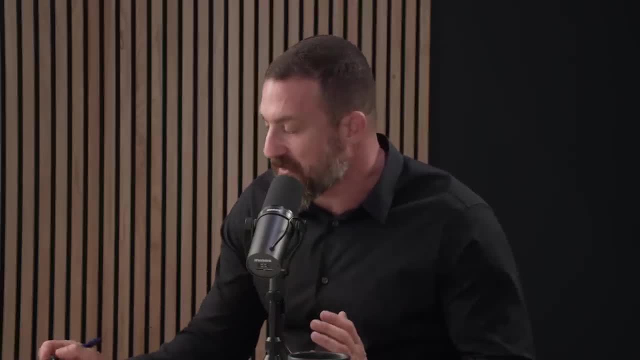 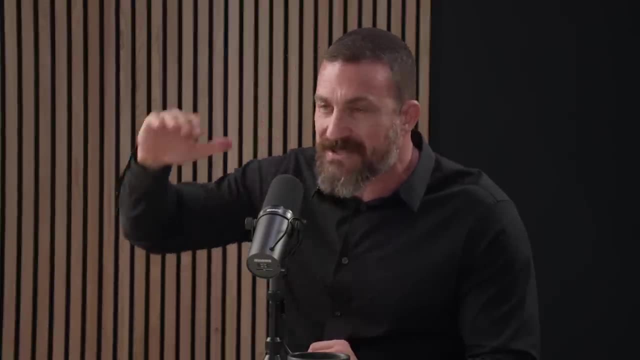 overall health and biomarkers. And then- this is wonderful to learn- that it can increase the sensitivity to satiety signals. I think that makes- at least my mind places very high on the list of things that people should absolutely do, but that there are other factors too. 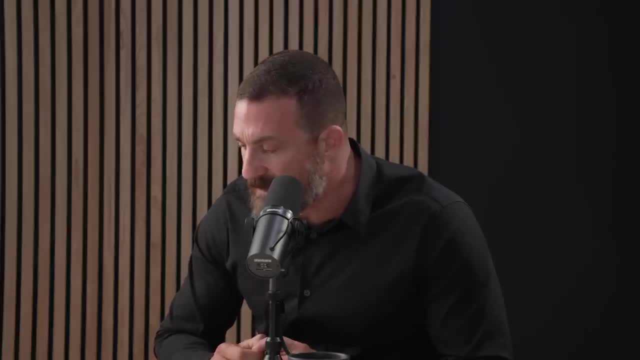 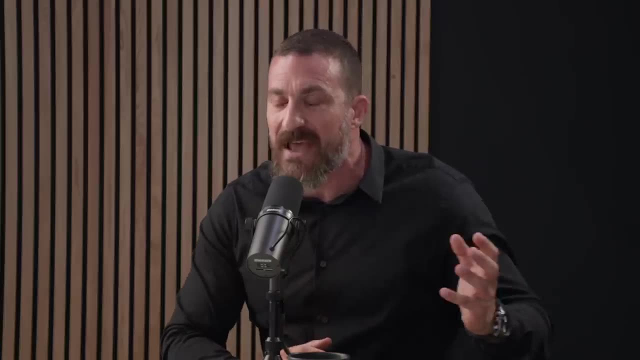 And the identity piece is fascinating. It reminds me also your story, reminds me also- of David Goggins, who is you know. he talks about his former, very overweight self almost as if it was a different person, And he uses language that I'm not going to use here. 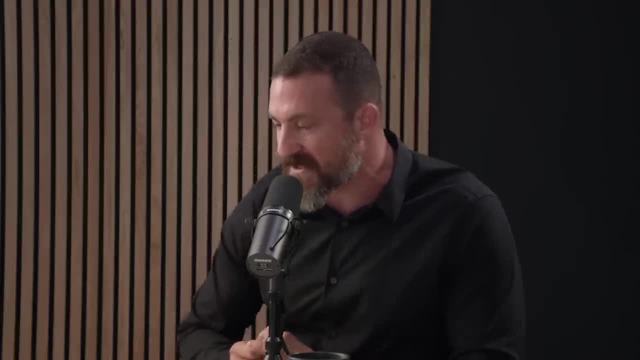 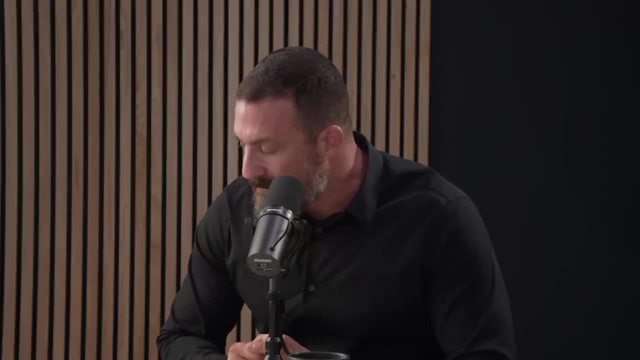 But you know, I've met David, know David a bit and he's he's every bit as intense and driven as, and a remarkable human being, as he appears to be online. He is that guy, But it does seem like he had to more or less kill. 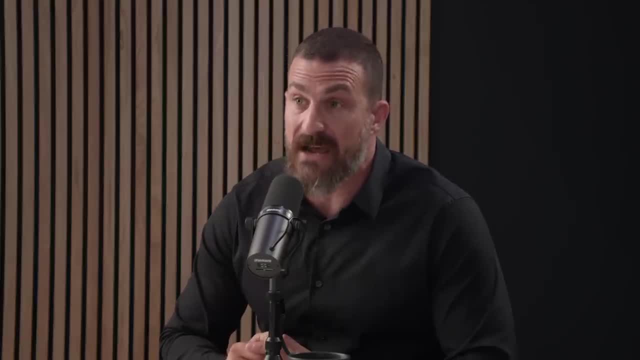 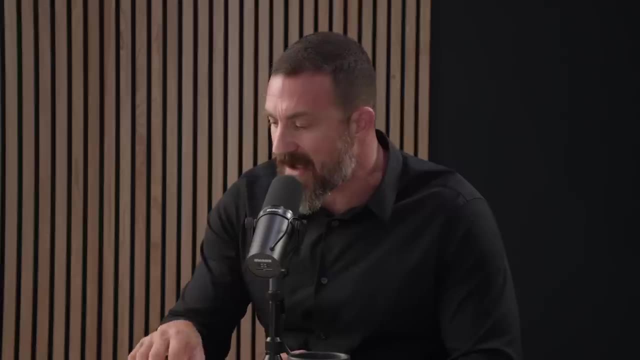 off of a former version of himself and and continues to do that every day. And I think what your point about that? this other fellow who did does it, does it through a similar process. I, the word today seems to really matter. It's not like you defeat this former version of yourself. 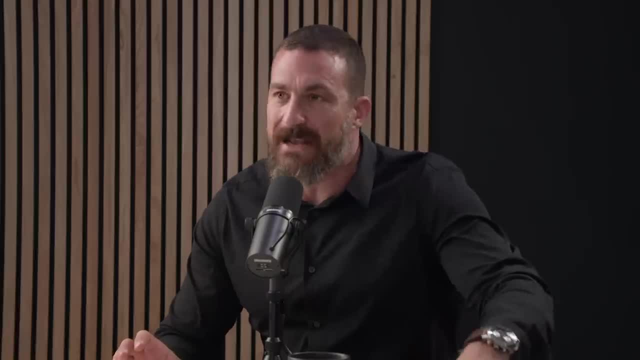 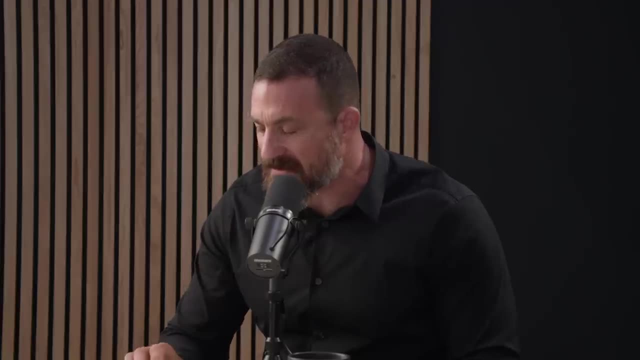 And then that that per that person is buried and gone. You said: you know, I killed my clone today, And that's the way that David talks about it also. So this is a daily process And I think this is not just a small detail in 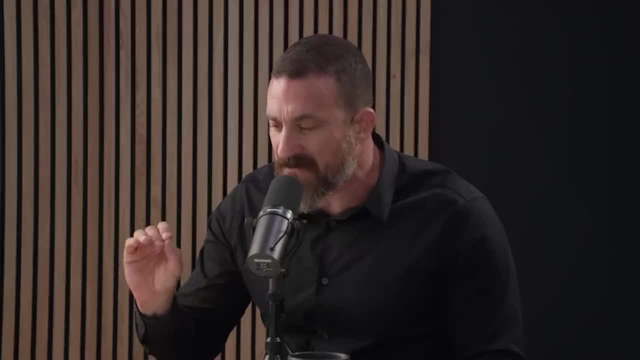 tying together all these things. I think that what you are describing is is fundamental, because we can pull on each one of these variables and talk about each one of them, But at the end of the day, we're a cohesive whole as a. 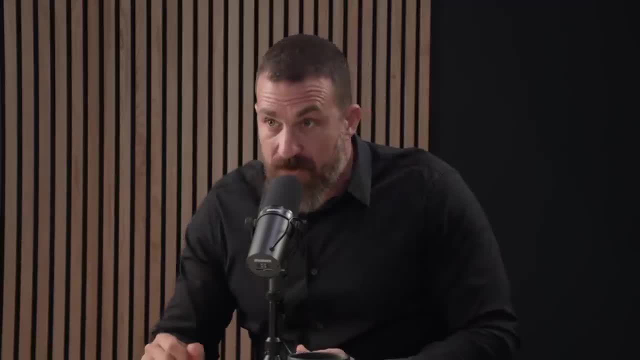 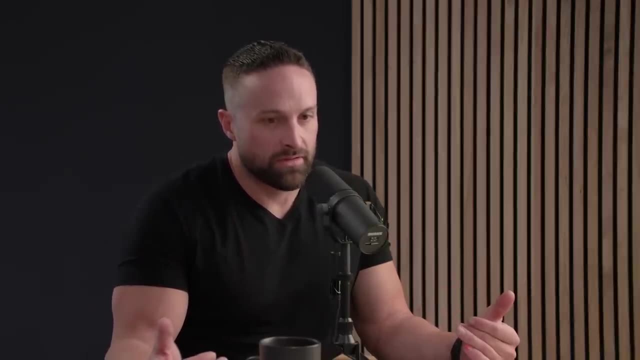 as an individual in. sorry, you were about to say that gets. that's good. Actually, I know one of my my favorite topics, which is: you know why do we have such a hard time with losing weight, but more so keeping it off? because of obese people. 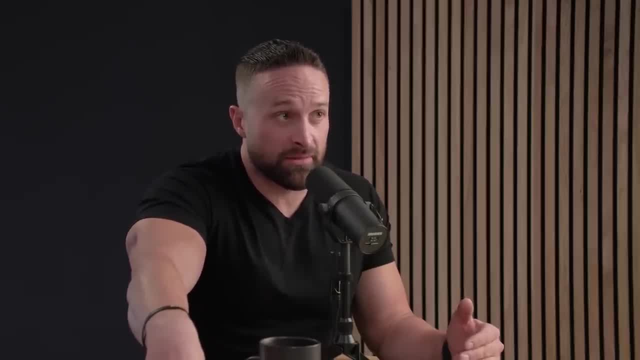 six out of every seven obese people will lose a significant amount of body weight in their life. So why do we still have an obesity problem? They don't keep it off. Why don't they keep it off When you look at the research? 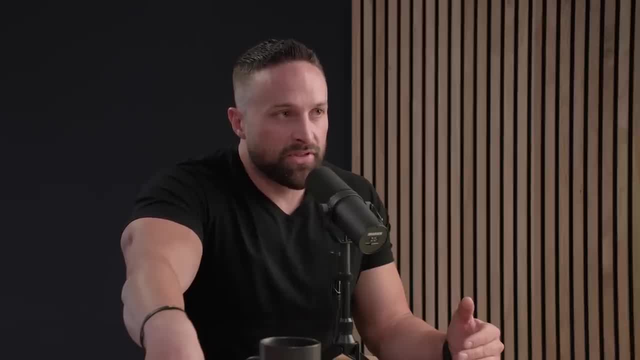 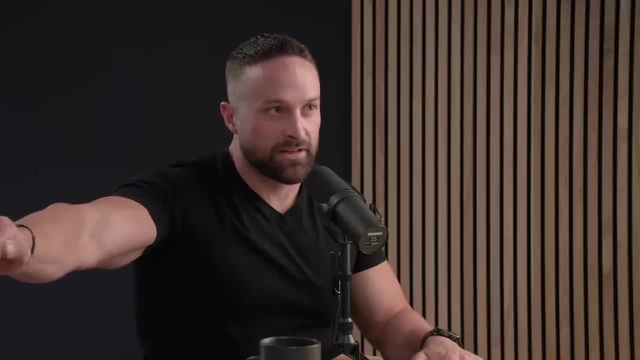 basically what it suggests is because people think about: I am going to do a diet, I'm going to lose This weight, And they do not give any thought to what happens afterwards. right, It's like think about if you have some kind of chronic disease or a. 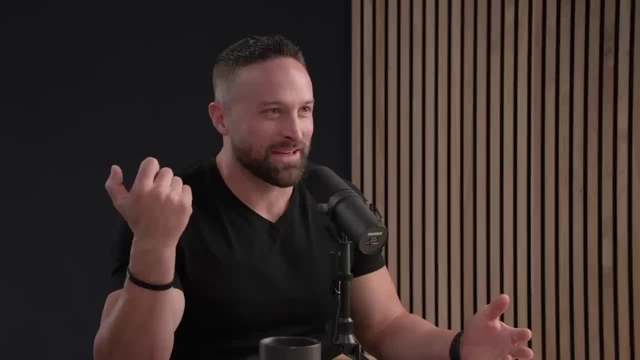 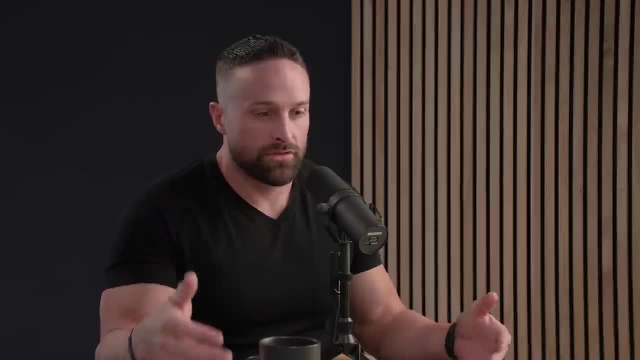 diabetic. right, You can't just take insulin once, and that's it. right, You got to take it continuously, Otherwise you're going to have problems If you do a diet and you lose, you know, 30 pounds. fantastic. But if you then just go back to all your old habits, you're going to go back to where you were, If not more. you can't. you can't create a new version of yourself while dragging your old habits and behaviors behind you. 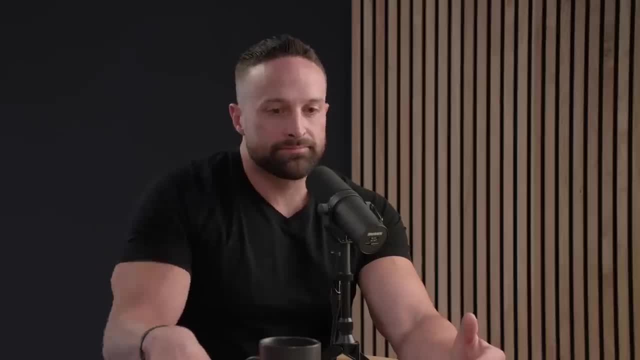 So what I'll tell people is because people say, well, I'm doing a carnivore diet, or I'm doing this diet or that diet, And I'll say, that's fine. Do you see yourself doing that for the rest of your life? 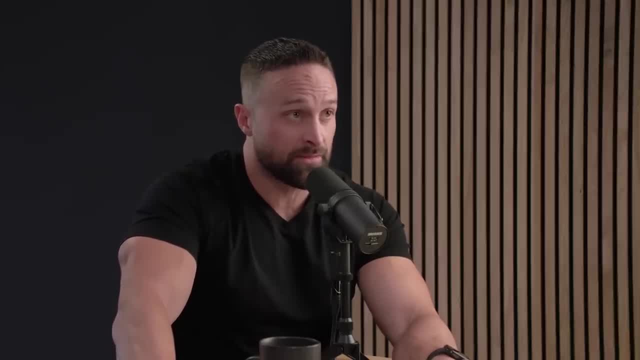 And if the answer is yes, if you, if you really believe that that's going to be sustainable for you and plenty of people- low carb intermittent fasting, whatever they say- felt easy. You know I could do this forever- Great. 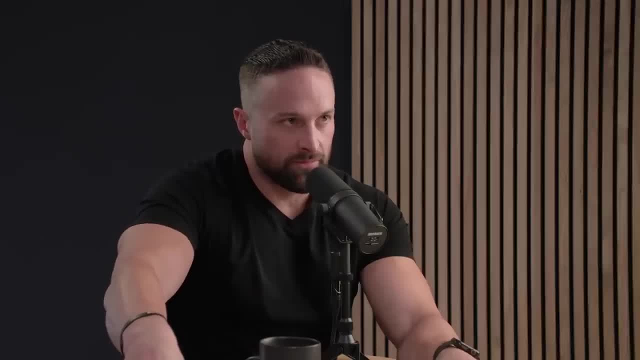 What? if you're going to lose weight, you have to invoke some form of restriction, whether it is a nutrient restriction like low carb, low fat, a time restriction, intermittent fasting, any form of time restricted eating or calorie restriction. tracking macros. 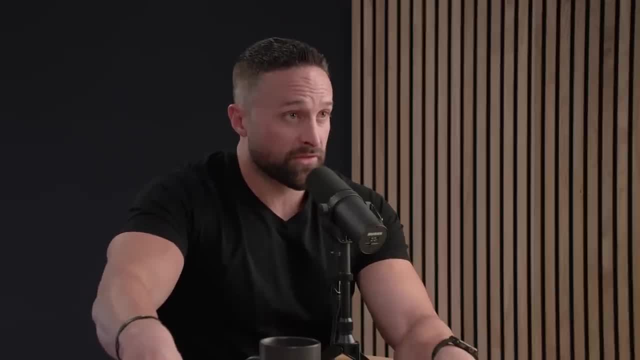 whatever. So you, you get. you get to pick the form of restriction. So pick the form of restriction that feels the least restrictive to you as an individual, And also do not assume that it will feel the same for everybody else, because I made this mistake where it's like I. 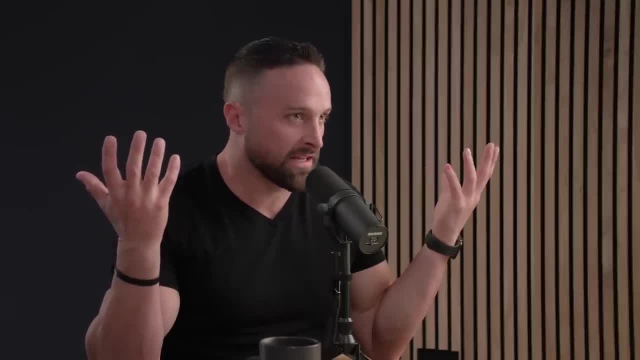 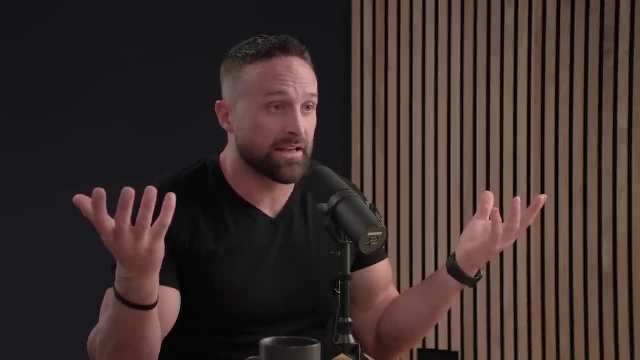 I track things, And so I allow myself to eat a variety of foods. I allow myself to eat some fun foods, Uh, but I track everything and I'm able to modify my body composition and be in good health. doing that Now, it doesn't feel hard for me. 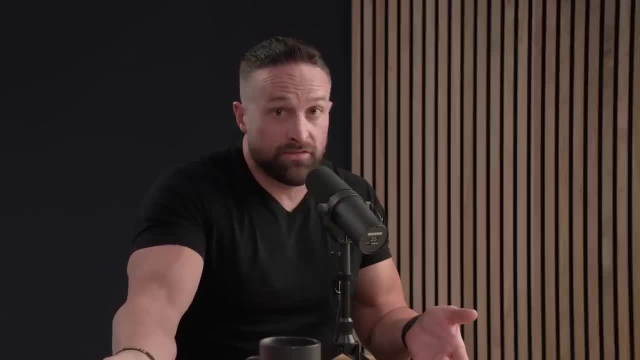 Like part of it's. I've just been doing it for so long. but the other people- that's very stressful, They don't want to do. they said: well, I'd rather just not eat for 16 hours If that feels easy for them. 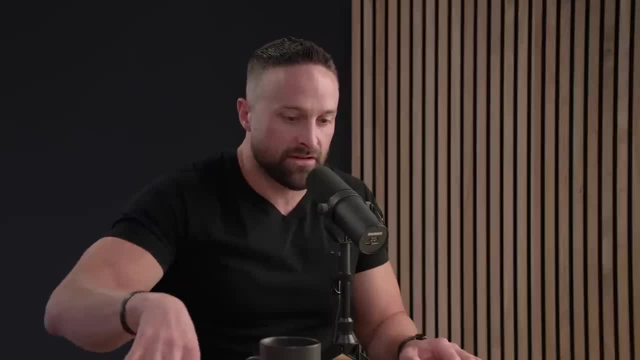 do that Because the one thing that there was- a couple of men analysis on a popular diets and basically what they showed was they were all equally terrible for for longterm weight loss, But when they stratified them by adherence and none of them were better for, 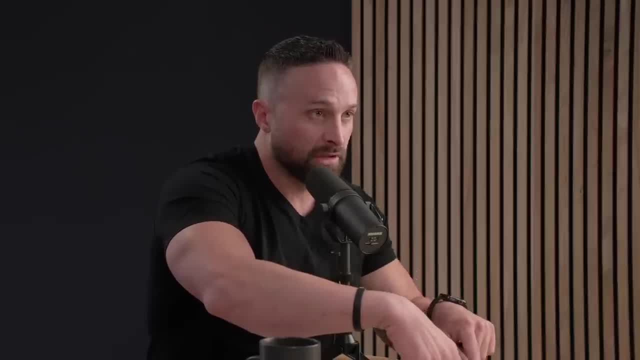 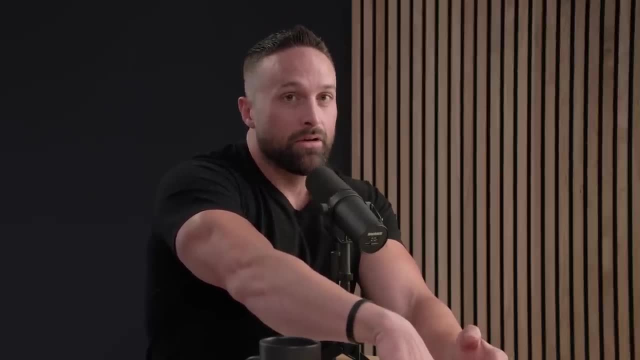 adherence overall, but when they stratified people just according from lowest adherence to best adherence, it was a linear effect on weight loss. So really what it says is: what is the diet that's going to be easiest for you to adhere to in the longterm? and you should probably do that. 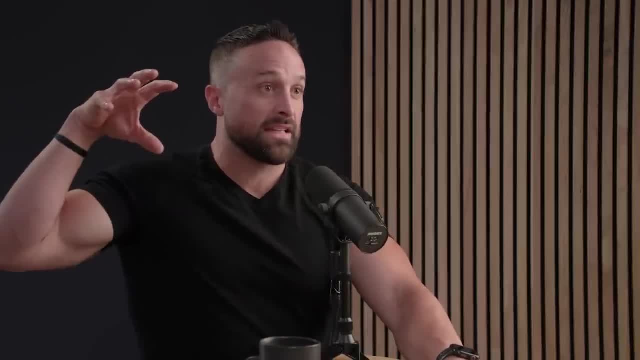 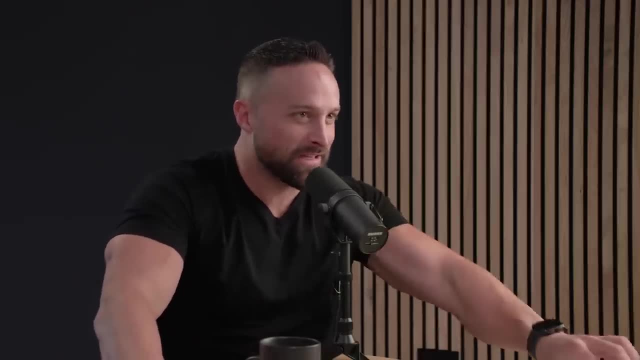 And people. again, this is where I step back and take the 10,000 foot view. Somebody will say, well, I'm going to do ketogenic because I want to increase my fat oxidation and I want to do this. And they're talking about all these mechanisms and everything. 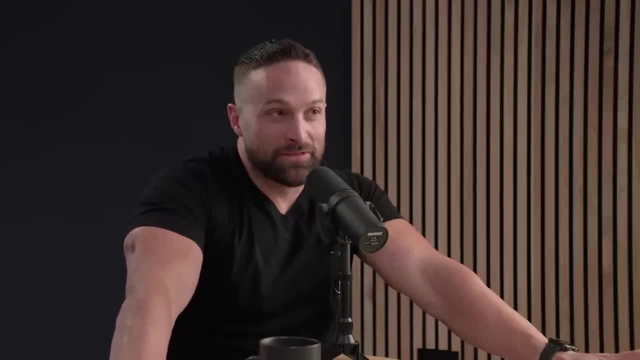 And that's great. Can you do it for the rest of your life, Right Is that? is this going to be something sustainable for you? And if the answer is no, you probably need to rethink what your approach is going to be. 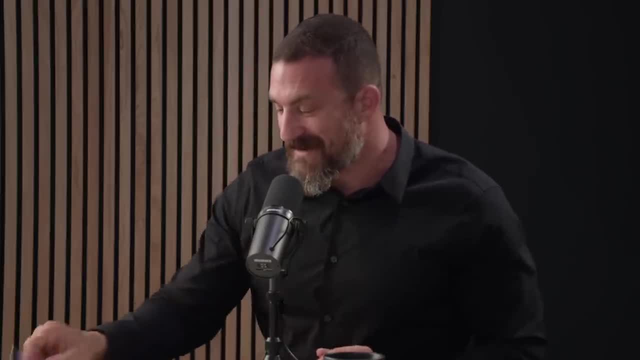 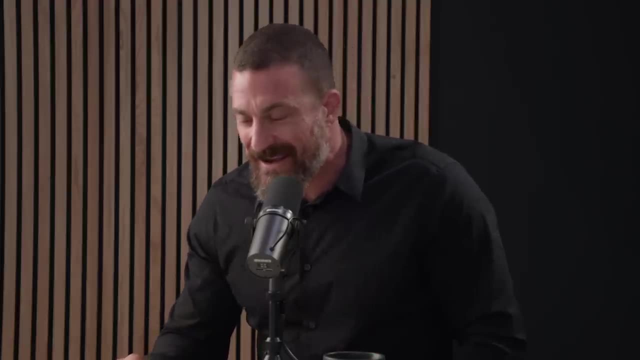 Yes, Incredibly important message Basically that you know if I can highlight, you know if there was a version of highlighter, boldface and underline in in the podcast space, I would highlight boldface and underline what you just said. 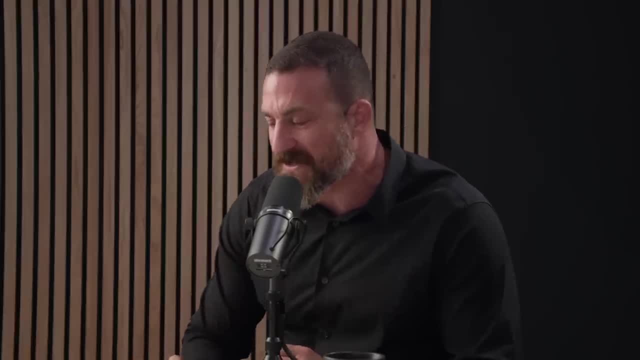 And for those of you that heard it, listen to it twice and then go forward, because it's absolutely key. I think it also explains a lot of the so-called controversy that exists out there. I think it also crosses over with the placebo effect. 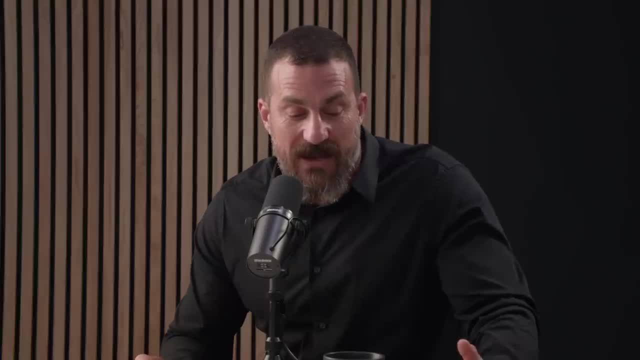 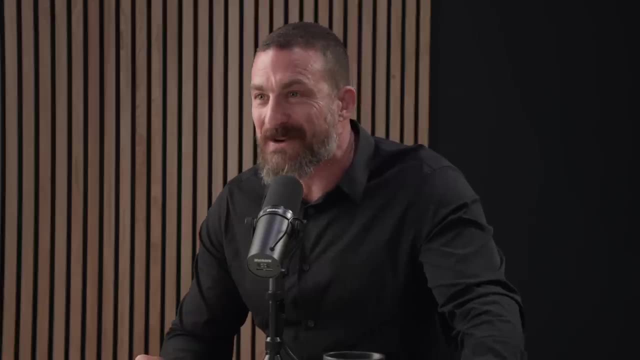 I almost want to say, um, pick the nutrition plan that you think you can stick to for for a long period of time, ideally forever. and pick your placebo too, because there's there is a lot of placebo woven into each and every one of these things. 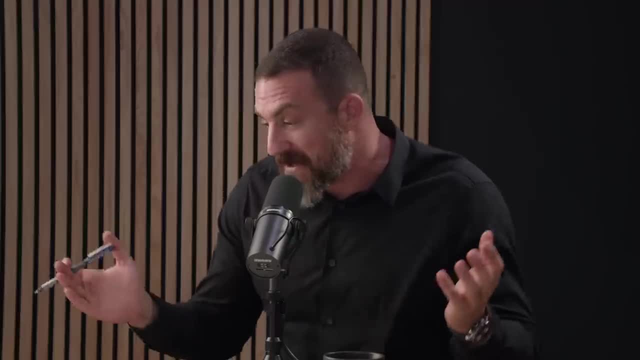 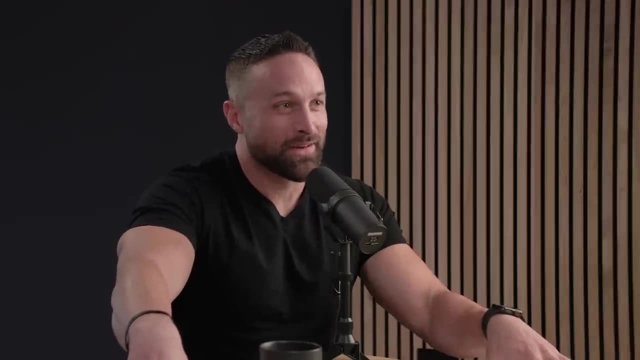 intermittent fasting, uh, keto, probably even um, vegan versus omnivore, versus carnivore. Well, they even talk about, um, you know, the diet honeymoon period, right, Where, like, you go into a diet and you're all fired up about it and like, 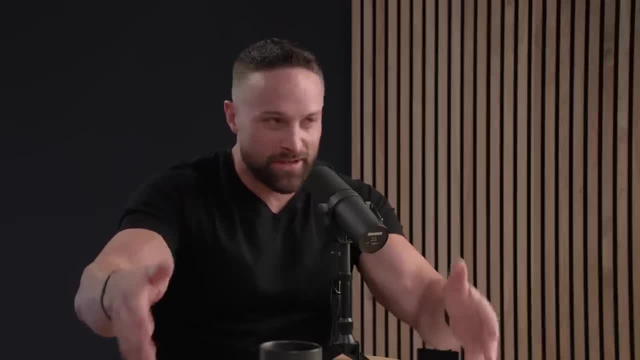 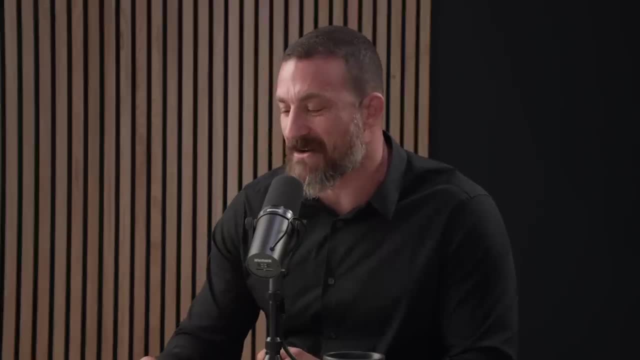 you're very adherent And then what happens with every single diet, without exception and research studies is, once you get past a few months, adherence just starts waiting and going off. here We are really talking about a form of relationship, You know. 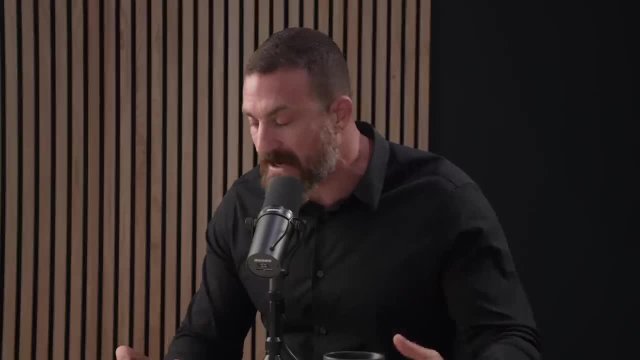 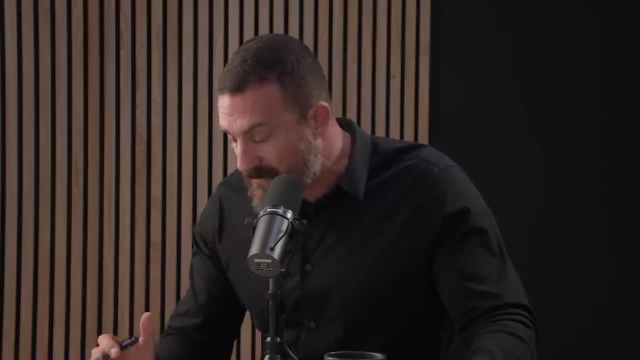 I'm not. I'm not saying that to be tongue in cheek. Actually, we had a guest early on in the podcast, Dr Carl Dice Roth. He's a psychiatrist and bio engineer at Stanford- Um tremendously successful Alaska award winner. 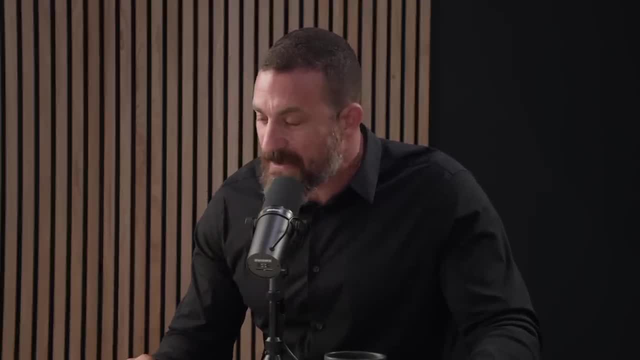 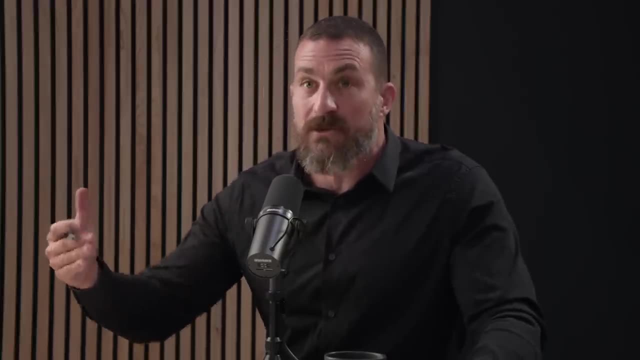 et cetera, And he talked about love as a sort of a, uh, an interesting aspect of our psychology, where it's a story that you co-create with somebody but that you live into the future of that story, You know, when you pair up with somebody that we use referring to romantic love. 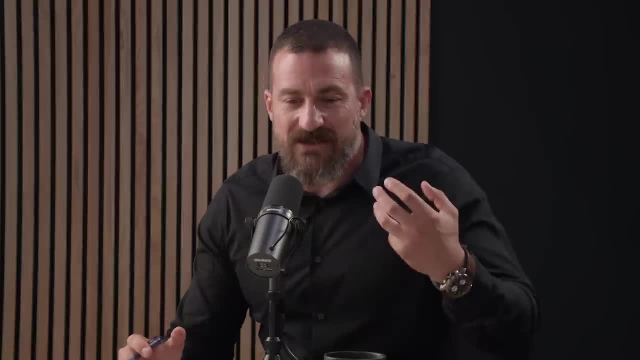 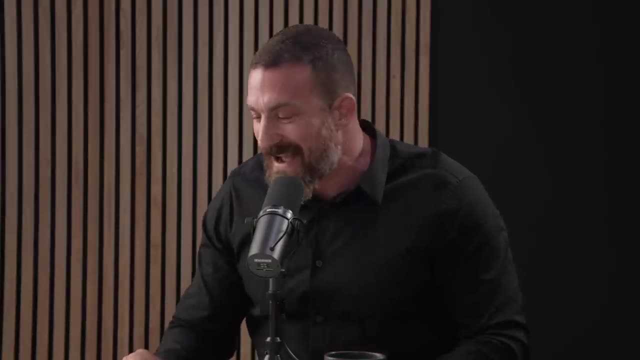 that there's this sort of mutual agreement to create this, this idea that you're going to live into. So it's not just about how you feel in the moment, It's also that you project into the future quite a lot. I'm seeing a lot of parallels with 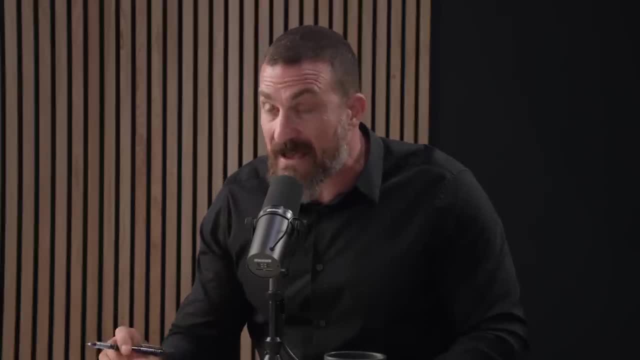 um, a highly functional and effective diet, And um, and I love it. I'm not setting this parallel up artificially. I'm setting up because I think that, ultimately, it boils down to what you said earlier, which is, which is that the brain and our decisions about what we are going to stick to. 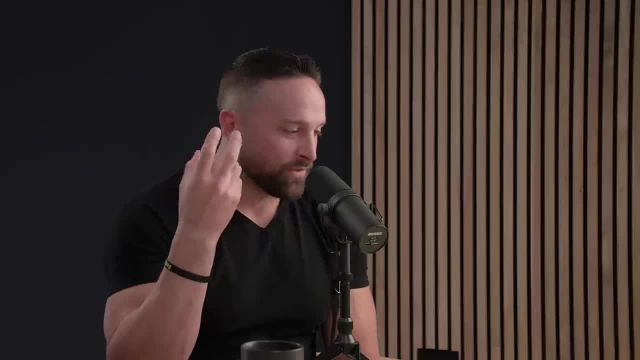 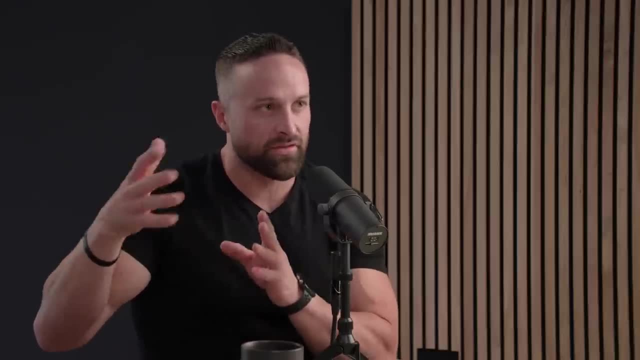 are tremendously powerful. I think one thing I will say is like: keep in mind, um, when you look at the research data, the meta-analyses on, say, time-restricted eating versus non, when calories are equated doesn't seem to be a difference in weight loss. 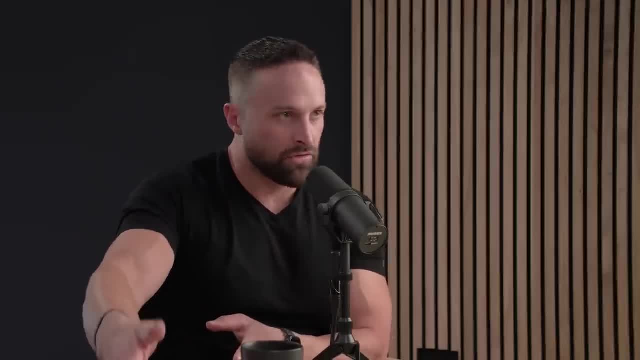 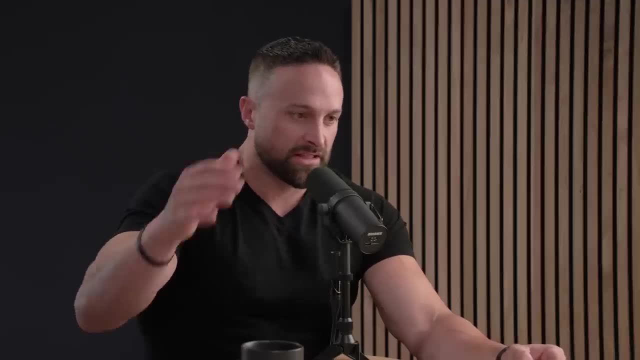 fat loss and most biomarkers of health. Same thing for low carb versus low fat. If you equate calories and protein. there was- there was- a meta-analysis done by Kevin hall back in 2017 where they looked at the and again. 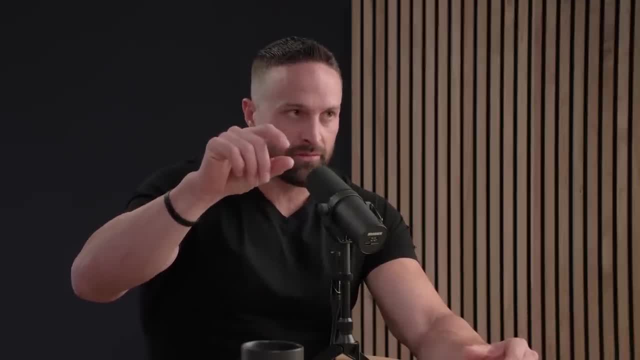 actual loss of body fat. And another important point was there was- I think there was 22 studies in this, but all of them provided food to the participants right. That's important because that makes ensures that adherence can be much higher in those studies. 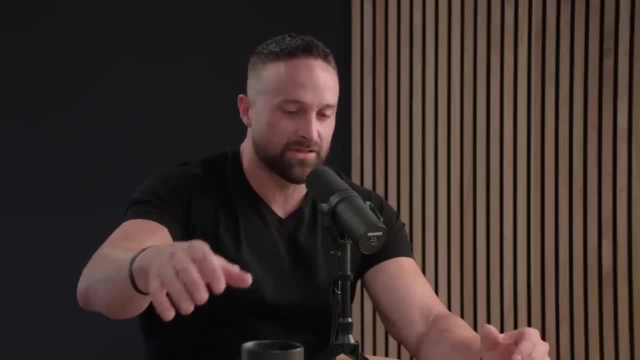 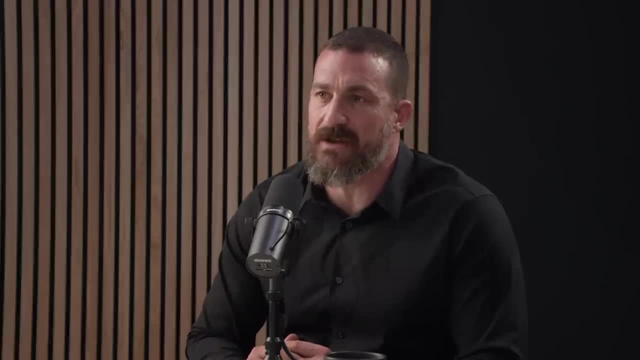 Whereas, like various free living studies, sometimes you can see funky results. People are sneaking food or or they're just not really eating the way that the study would ideally have them, Unless unless the person is getting like continuous support, like studies where they have a diet. 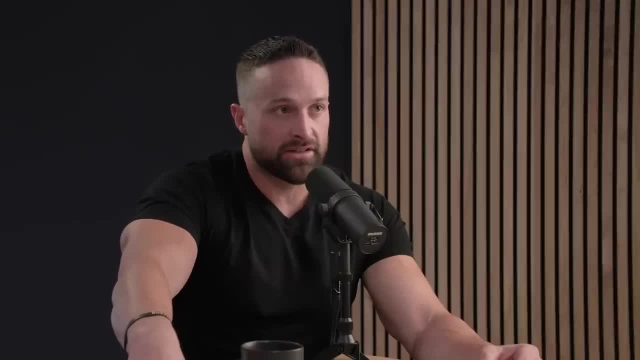 a dietitian talk to people like every week tend to actually have pretty good adherence. But I mean that's expensive to have done the study And again, like what limits studies, money, money and money, right, Um, but the low carb versus low fat and protein and calories are. 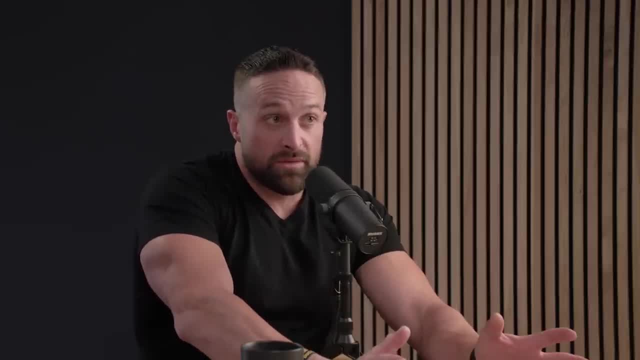 equated, basically no difference in fat loss. Now some people get upset about this, but it's like what? to me, that's like. this is great, because you get to pick the tool You want. the one tool, It doesn't seem to be that much better than another. 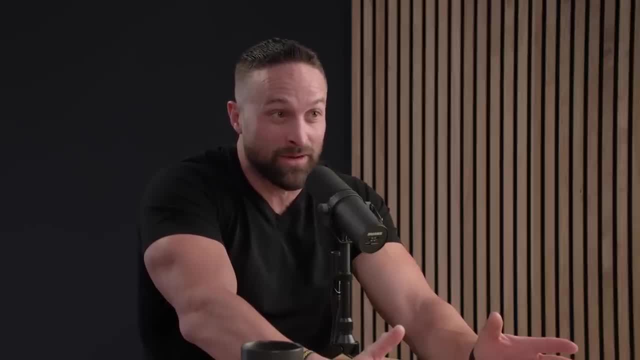 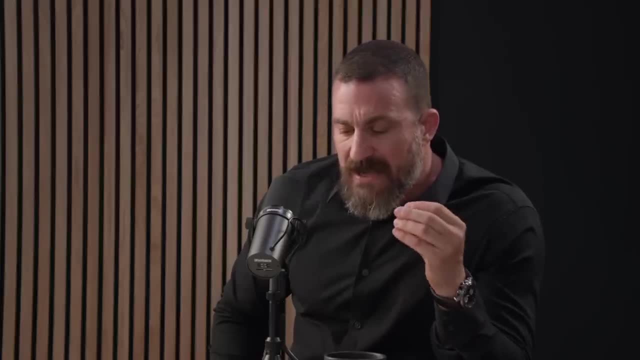 So pick the one that works for you, right? Whatever? you've got a pool, you've got a bunch of different options. You mentioned picking something that you can stick to for a period of time. Is there ever a case for someone saying: look, I like to eat low carb or even keto for six months and then switch to a more standard omnivore caloric maintenance type diet and then switch back. Is there any downside to doing that for sake of health or weight loss over time or weight maintenance over time? 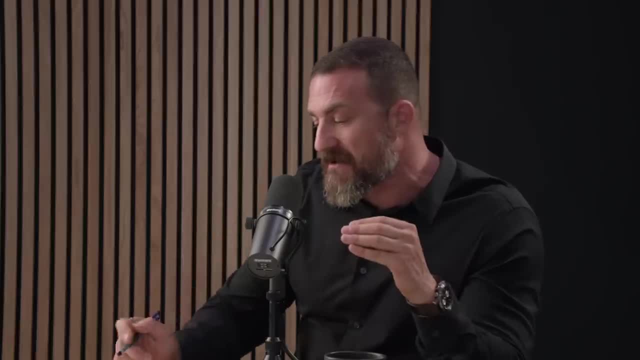 Cause I realized not everyone is trying to lose weight, And I definitely want to talk about at some point how to eat to maintain weight, Cause I think there are a significant fraction of people out there who are trying to do that, But yeah, 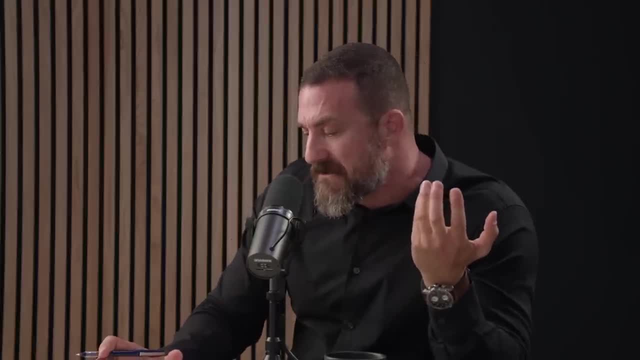 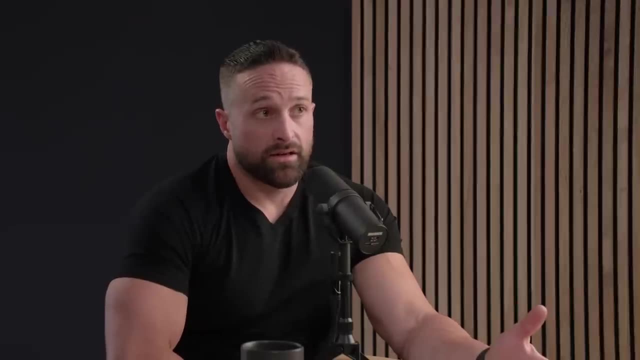 is there anything? is there any downside to being a dabbler? you know, keto for a few months and then omnivore for a few months, et cetera. I think that's actually a great thing, especially to like maybe find what you feel is easiest for you. 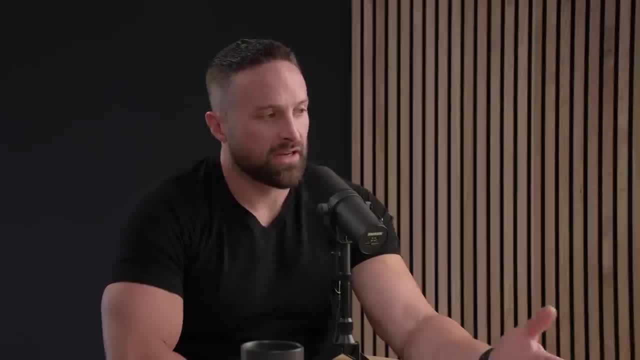 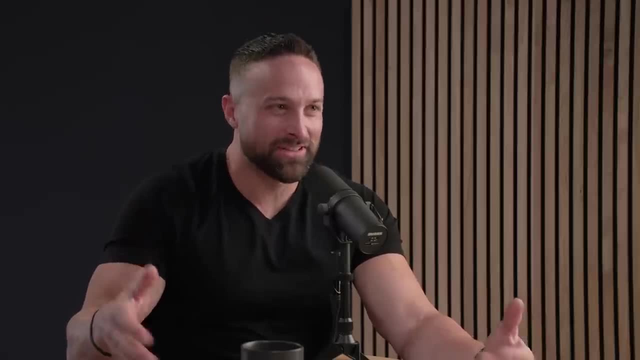 Right, But in terms of like as a strategy. I mean, I guess you know some people, this might get into dopamine, but like, Oh, change and get something new And, like you know, you feel a bit more positive about it. 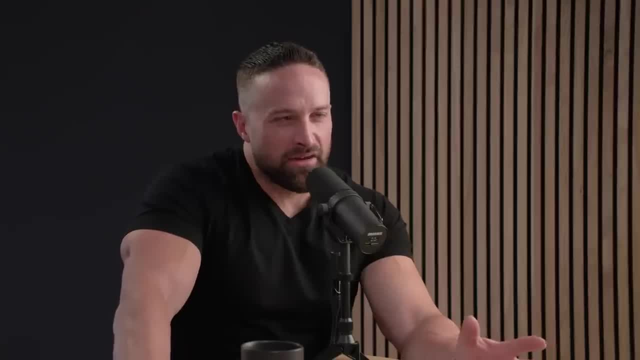 Partner model. Yeah, exactly. So I don't think it's how I would usually set things up initially for somebody, but if somebody said, Hey, I just like to have some variety and change it up, as long as they're still like. 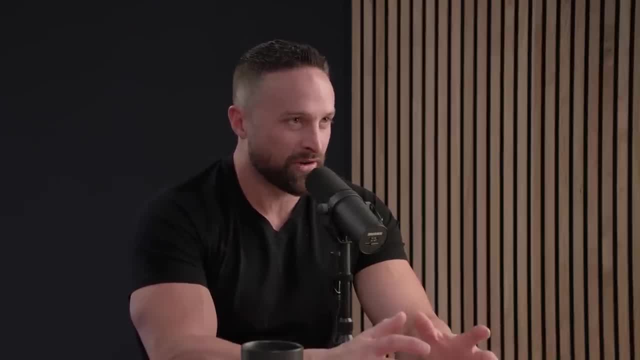 you know their behaviors and they're doing portion control or whatever it is, and they're able to sustain a calorie deficit or, you know, depending on whatever their goal is, I don't think there's really any downside to it. I do think the one thing to keep in mind is when you look at like going. 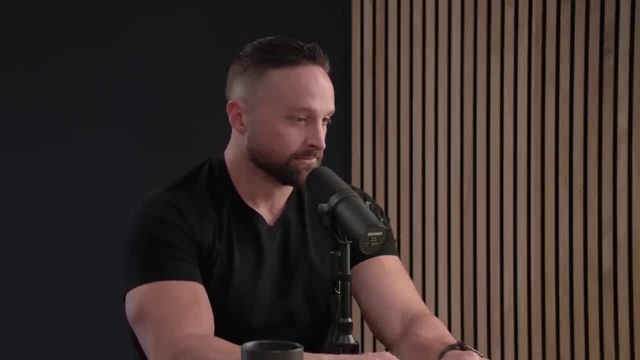 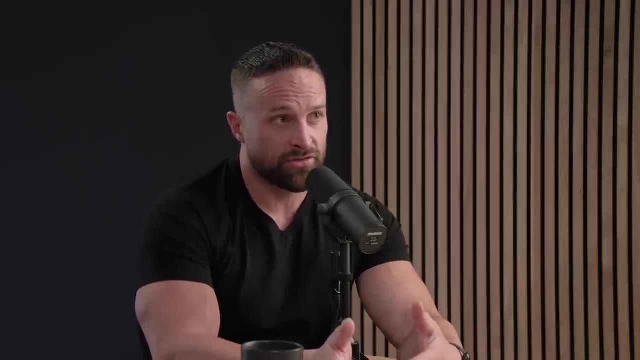 between, between extremes, So like low fat to low carb or or vice versa. there can be in that transition period a little bit of weirdness, for lack of better term- Like, for example, if you've been on a ketogenic diet and all of a sudden you move to. like a higher carb diet. you will be like basically insulin resistant for just a short period of time. Now, is that going to cause any health problems? Probably not in the longterm, especially if you're still controlling calories. But just because your body has kind of like upregulated these systems dealing. 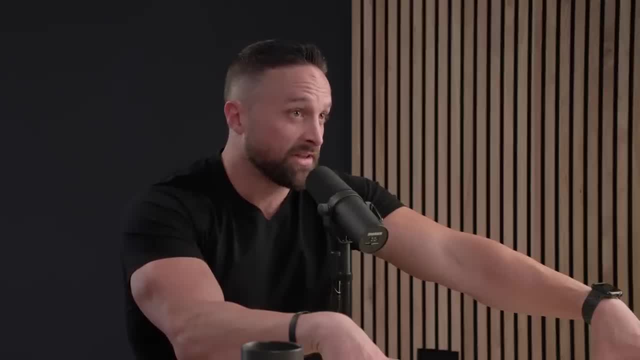 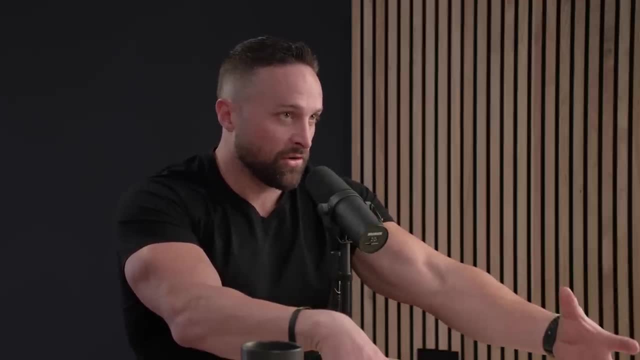 most with, mostly with fat and glucose production rather than glucose metabolism. So now if you start taking glucose or carbohydrate back in- like, for example, you get somebody in, or a glucose tolerance test after they've been on keto, the do pretty terribly at it. 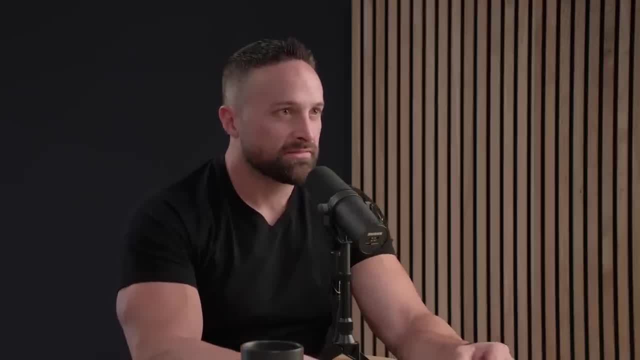 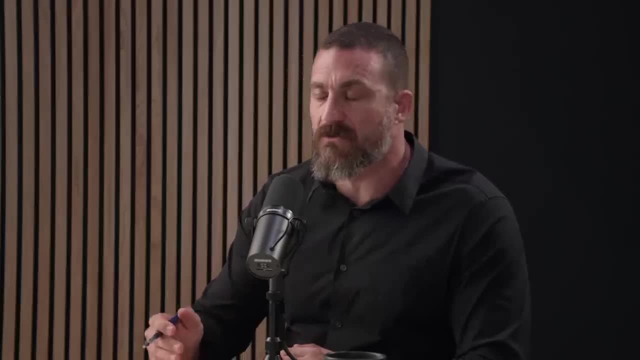 Uh, but that doesn't last that long. About how long Few weeks? I think that's important for people to know because I have a feeling during those first few weeks are the periods, A period of time when a lot of people go running back. 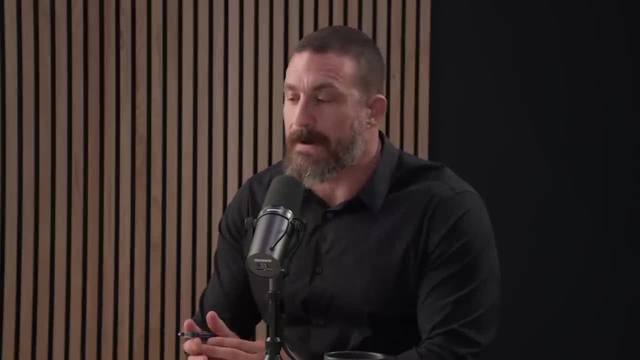 to what they were doing previously, which is not to say that they shouldn't, but um, I've certainly done that. I try, I've tried um very low carbohydrate diet and I would have assumed- and now I know I'm completely wrong- 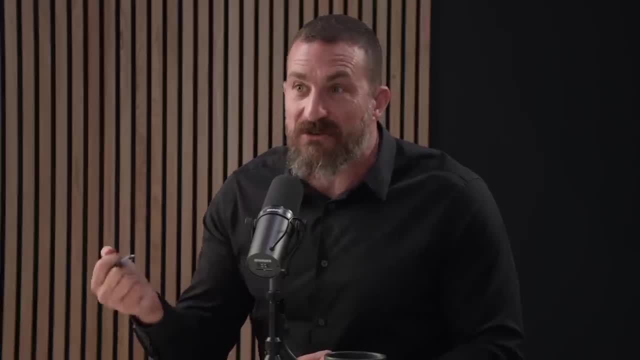 but I assumed that I was so carbohydrate starved for so long that my insulin sensitivity- which is a good thing, by the way folks- would have gone through the roof and I would be able to just sponge up every bit of glucose that I would have ingested through carbohydrate. 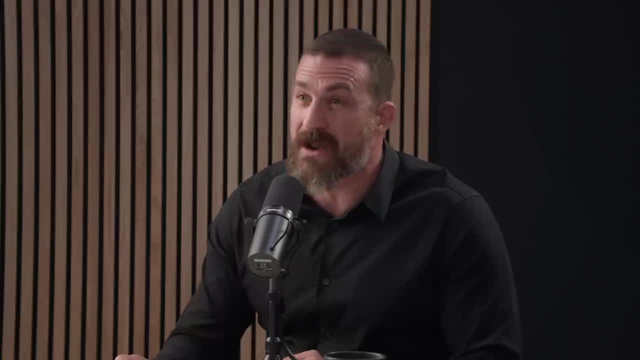 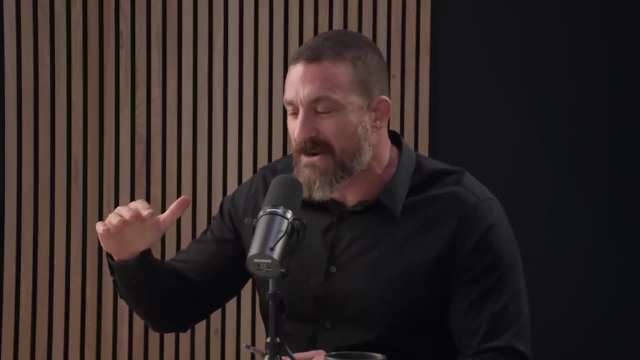 So I did indeed switch over And I felt like I had pretty terrible brain fog. I even got some jitters and I thought: wait, what is this? You know, my blood sugar was low before. Now my blood sugar should be in more moderate territory. 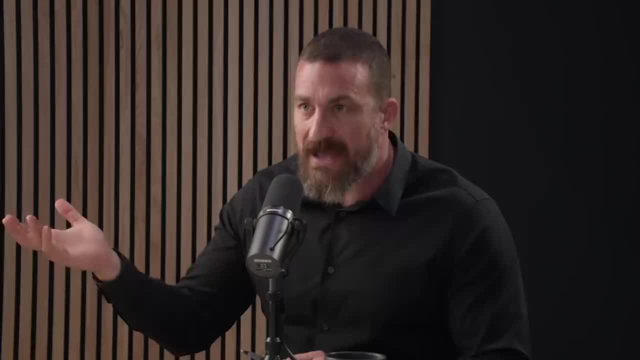 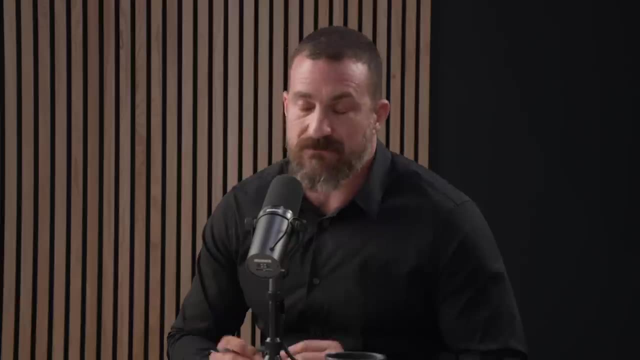 But, based on what you just said, I had upregulated the enzymes and systems in the body for fat metabolism on the keto diet And then, switching over um, there was a basically a ramping up of the of the the. the molecules involved in uh, presumably in glycol. So transition period, I mean, think about like if you haven't weight trained before and you start weight training, you're going to feel pretty terrible right, Like you're going to be sore and stiff and all that kind of stuff. 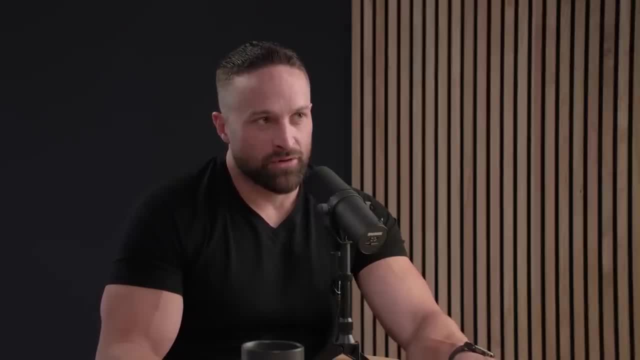 But I will say you aren't necessarily wrong in what you said about being more insulin sensitive, because it depends on how you measure insulin sensitivity. So if you measure with something like, um you know, fasting blood glucose or fasting insulin or even HOMA IR, 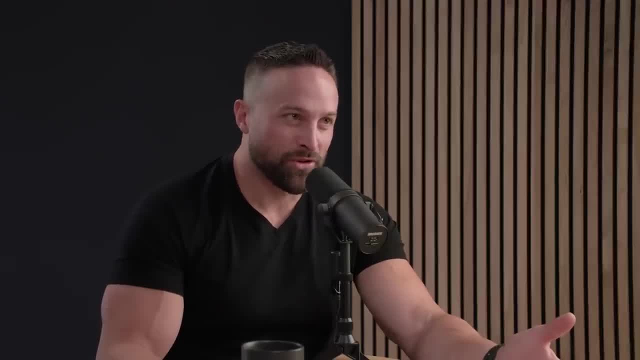 those tend to be pretty good on low carb, But then if you do an oral glucose tolerance test, it tends to be pretty bad, And so it depends on your specific measure, right? Um? so I I think that you know. 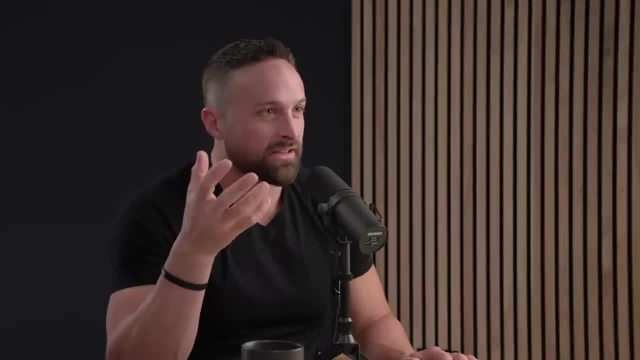 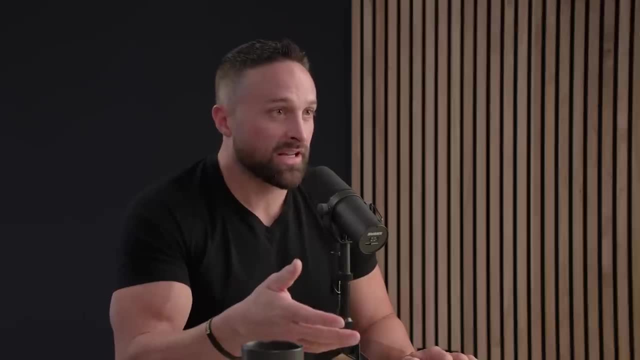 the idea that keto makes you- you know- glucose intolerant or insulin resistant. I think, again, it's just a transition period and I'm not too worried about it, but it is something important to keep in mind And one of the reasons like if somebody was to transition out of keto. typically if, like, I'm working with them or one of our coaches are working with them, we'll kind of instruct them to do it like slowly and kind of systematically over like a four to eight week period. 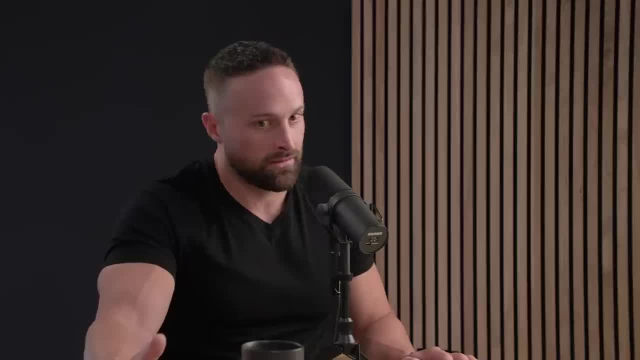 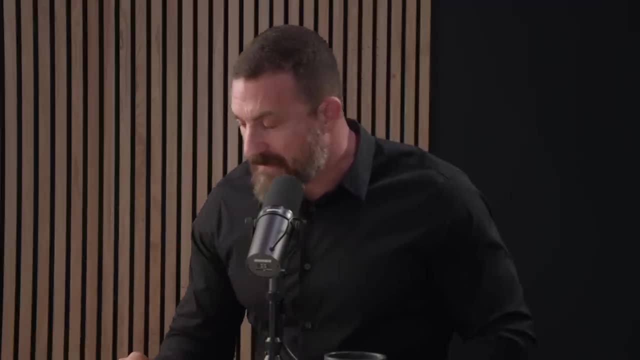 That way, hopefully, you know, they're not having that period of two weeks where they're like, Oh man, why, why do I feel so terrible? Very important point. I want to go to the other end, um, literally and figuratively, and talk about gut health, because 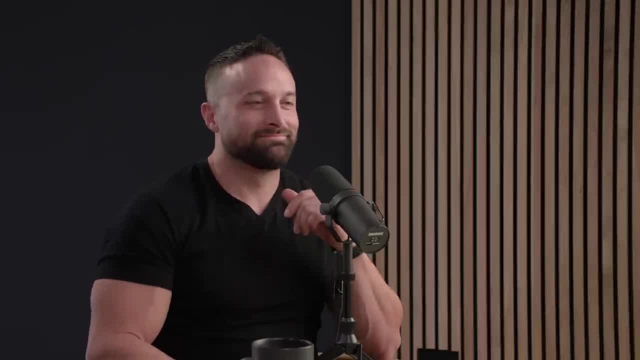 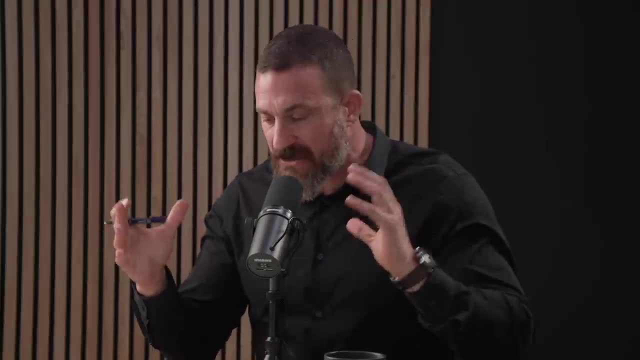 uh, up until now, and certainly what you did with that, and certainly in the last um few minutes, we've been talking a lot about sort of top down processes. you know that the brain, the psychology, placebo effects, but the very real aspects of those 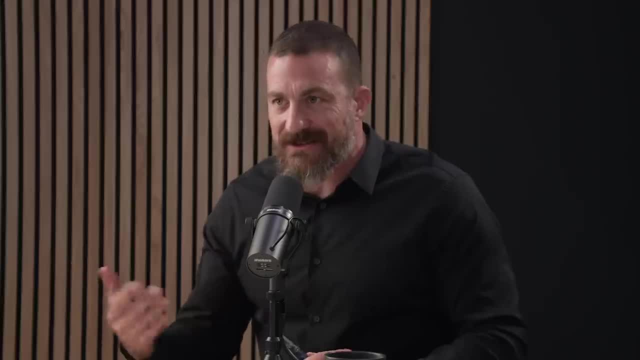 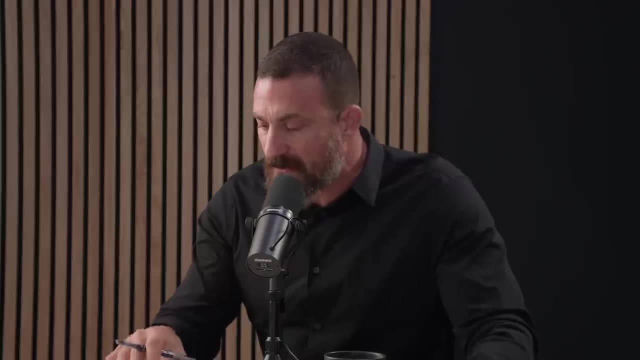 not that I can imagine 2,000 calories is a thousand calories and somehow change the law of thermodynamics. Can't do that. but we've been sort of top down and integrating a lot of different ideas into weight loss, maintenance and weight gain. 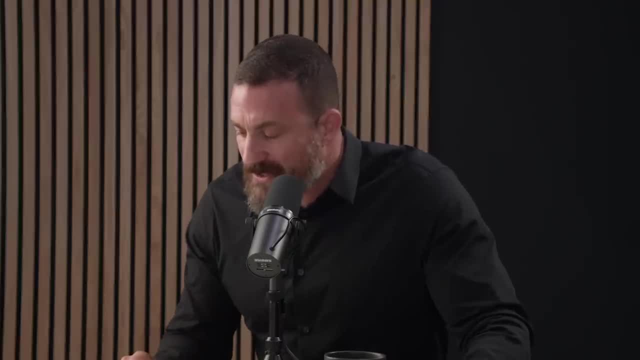 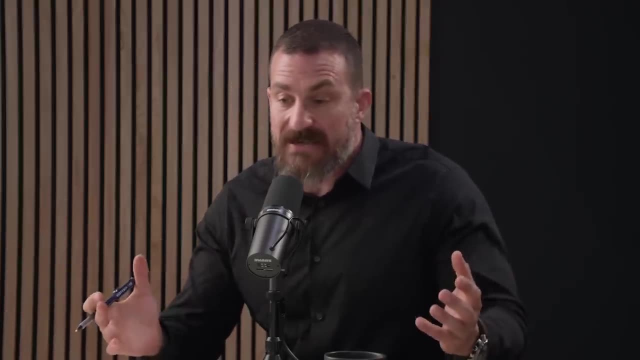 but gut health, at least the more popular studies on gut health, had blown a lot of things out of the water, For instance, this idea that you could take obese mice and literally give them fecal transplants from lean mice. And yes, that sounds like what it sounds like. 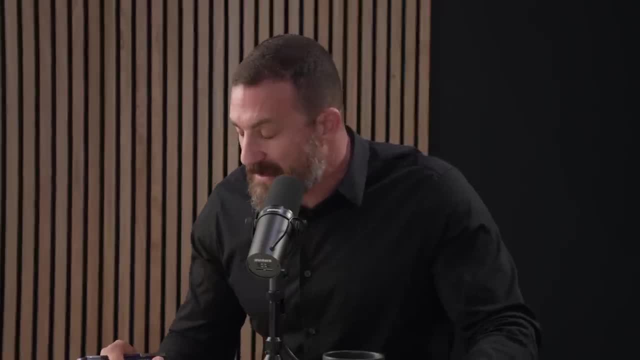 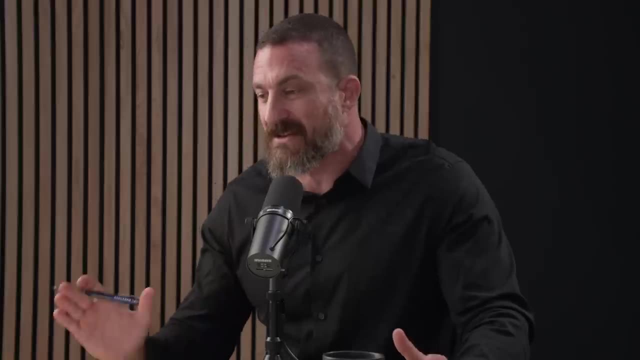 Um, fecal transplants, definitely inserted through the same end in which it comes out, And I point that out because a lot of people have asked me that they, you know it was kind of scary to me. I thought, yes, this is not about ingesting feces. 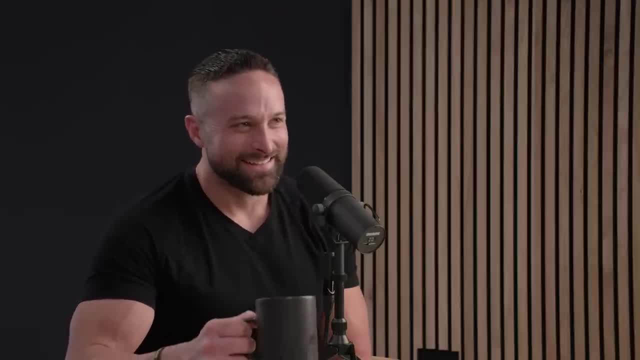 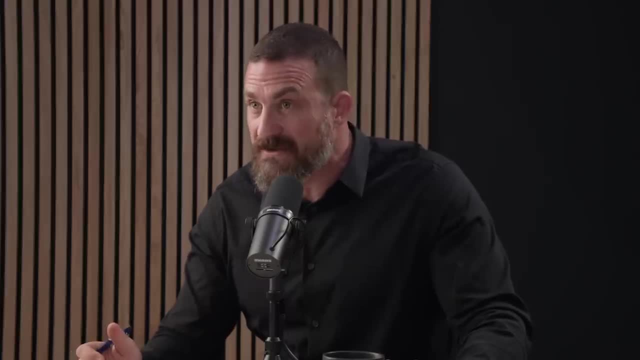 This is they. they, they literally do a transplant of feces from lean mice into obese mice and the obese mice get lean. And yes, this has been done in humans- limited number of studies- and observed some pretty impressive effects on weight loss that I have to assume could be related to. 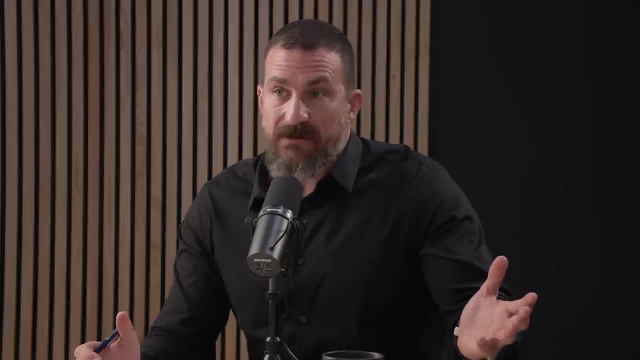 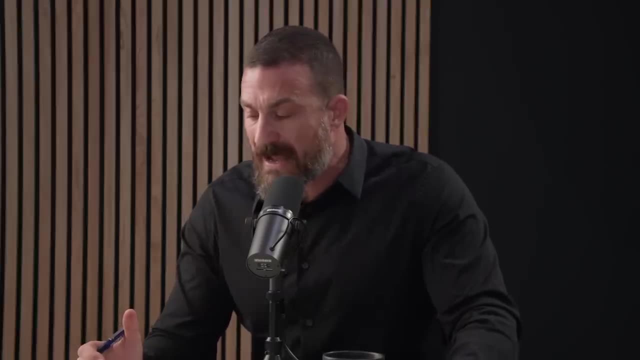 plant-based diet. So, um, I mean, I think it could be related to placebo effect. They might've told these obese people: Hey look, you're going to get lean through this fecal transplant from lean people. but more likely it had some effect on their core physiology. 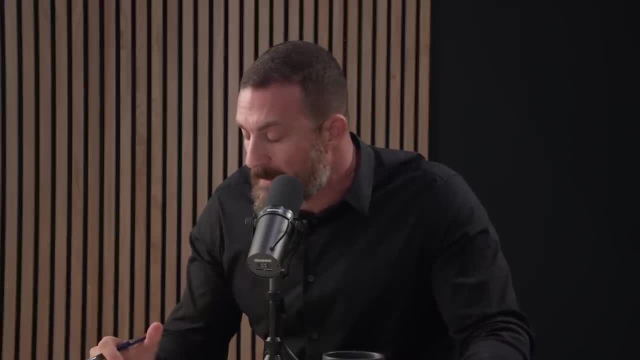 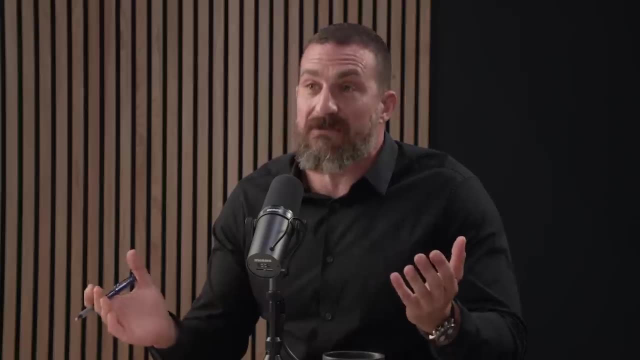 I don't know which aspects, although I can speculate which ones, and they became leaner, they lost weight And that is in some sense miraculous when you especially given the important role of psychology and exercise and satiety signals, because I'm going to assume that they controlled for a number of those. 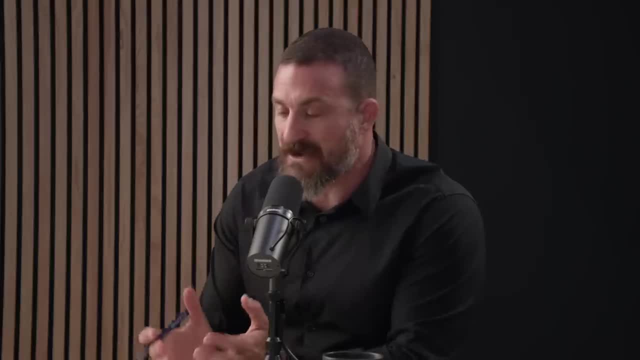 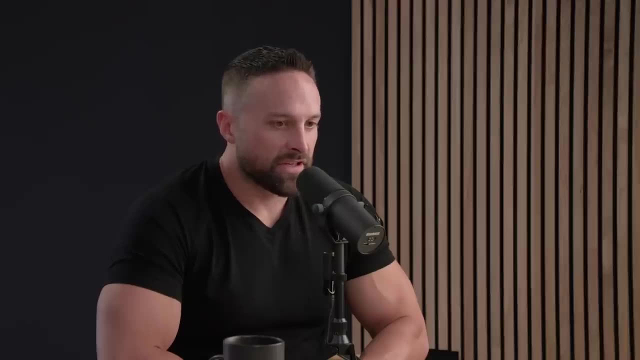 other variables, although no study is perfect. What are your thoughts about gut health as it relates to metabolism, energy utilization and balance? Yeah, So the first thing I'll say is I'm not a gut gut health expert, but I will. 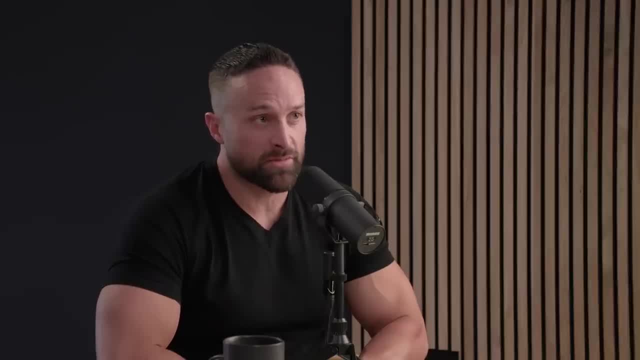 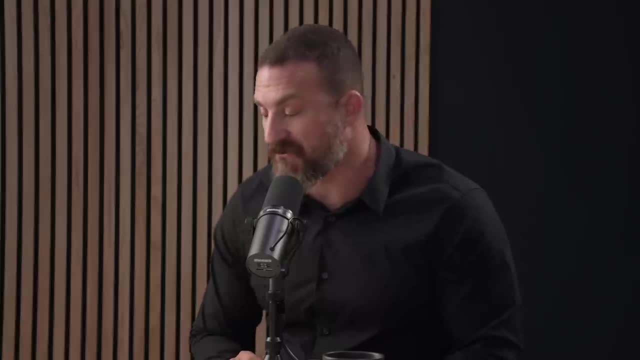 I feel relatively comfortable talking about it, based on conversations I've had with people who are experts, Uh, one being um Suzanne Devkota, who's um- uh, are you familiar with her? Well, she's sort of a phenom in this area, from what I understand. 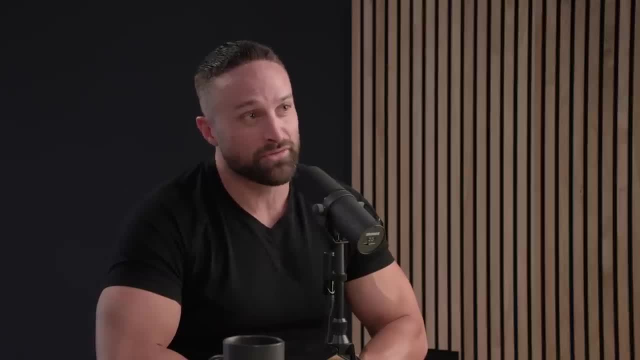 She was actually doing her masters when I was doing my PhD in layman's lab, So she was one of my one of my lab mates. Um, and you know, I the other thing to say- is even gut health experts, and Suzanne will tell you this. 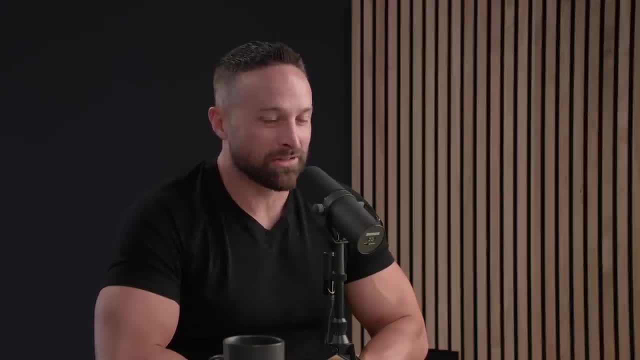 they're like you know, talk to me in 20 years. We just know so little. I think that's an overall thing. that people don't understand is the scientific consensus moves very, very slow, And probably for good reason, because if we just flipped our scientific consensus based on one study, 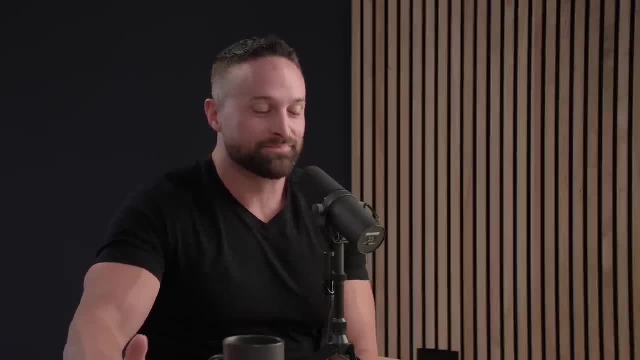 I mean you. it would be a mess, Right? So it's going to take time before you really understand the implications of the gut and what it means. So when it comes to weight loss, there probably is a role in there, I mean 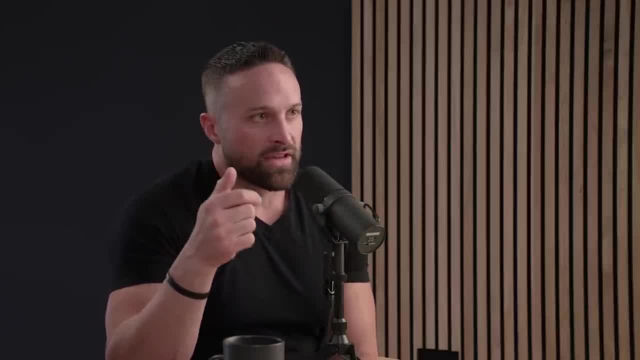 we've seen that there's something going on now, whether that's is it um something where a gut back microbiome makeup that's more obese resistant. uh, perhaps it extracts less calories out of the food you eat, right? 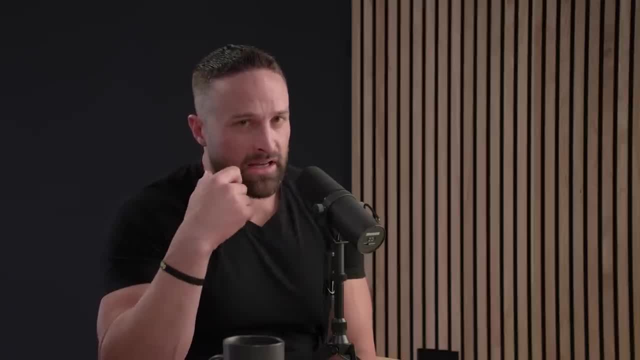 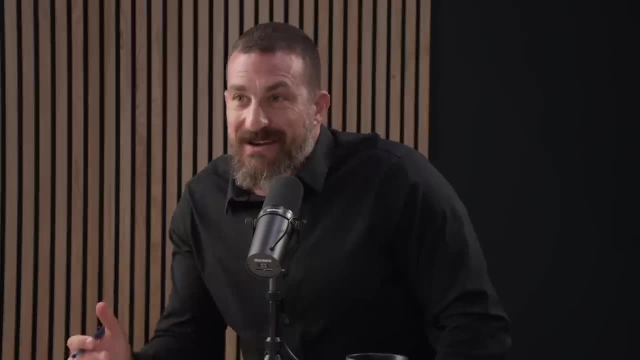 Uh, or perhaps it's elevating BMR, Although I I think that that's probably somewhat unlikely. Do you think it could impact the way satiety signals are? So that's? I mean back to the brain again, is so that's? 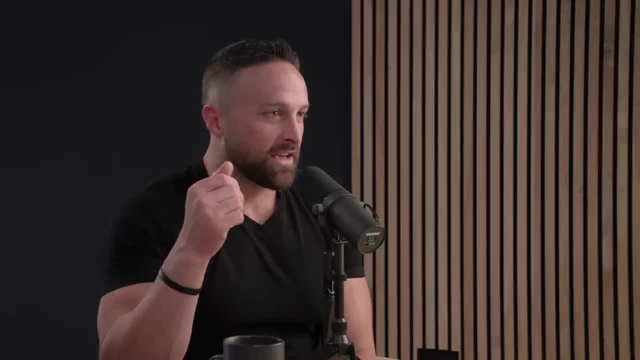 we know that there's a link in the gut brain access, And so my suspicion is that it probably is working via appetite regulation. So that I mean, if we look at um, if we look at the most effective um obesity treatments out there, 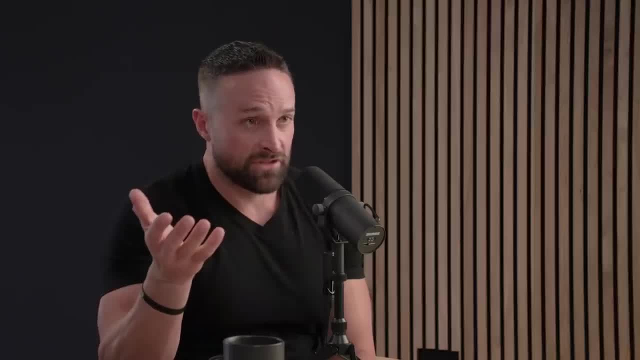 which is like semi-glutide. uh, I mean, you consistently see a, you know, 15%, you know, on average loss of body weight which is massive and people keep it off. Um, that is a GLP one, mimetic. 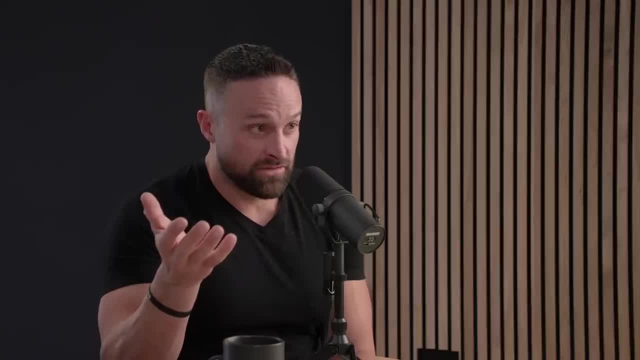 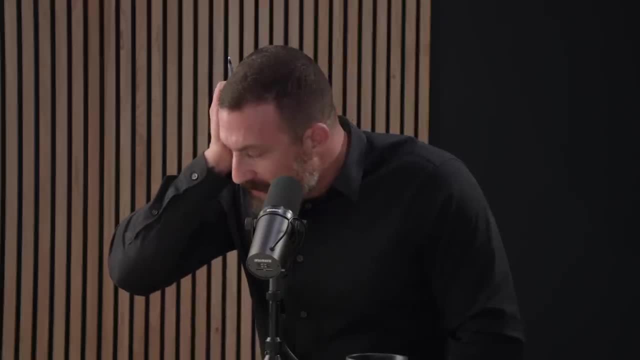 which is a gut hormone And it basically just is a very, very powerful appetite suppressant. Uh, not well, I guess I'm interrupting, but hopefully with a purpose. um, there's this really interesting study, and it's in mice, admittedly. 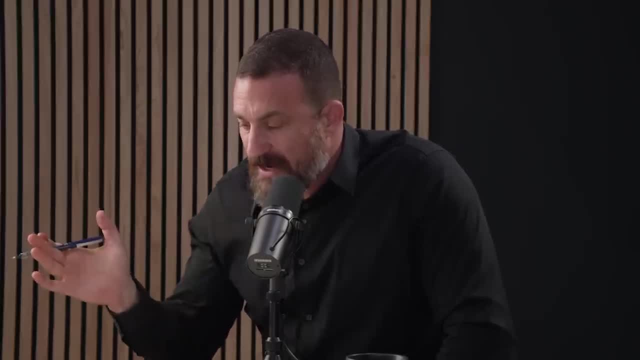 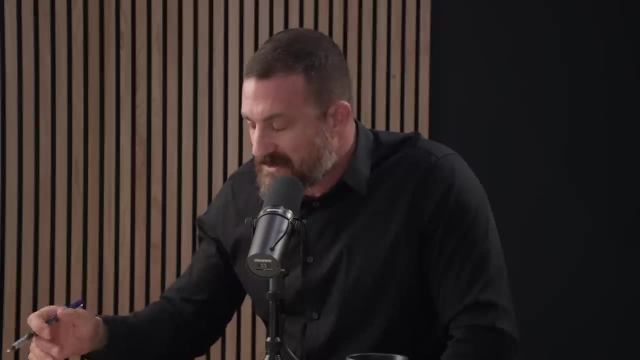 but uh, publishing it neuroscience journal recently And the basically the takeaway is that, like so many things in neuroscience it, the GLP one, works in two parallel pathways in the brain. It seems to impact neurons in the hypothalamus that control satiety. 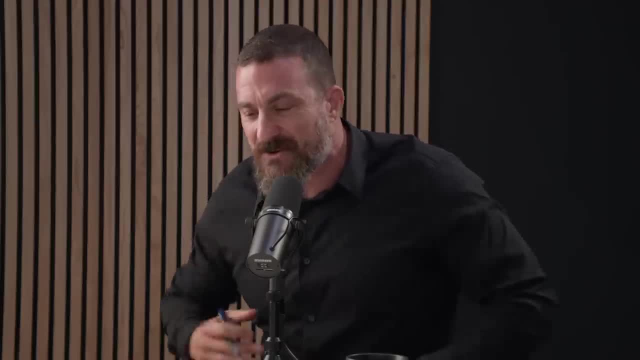 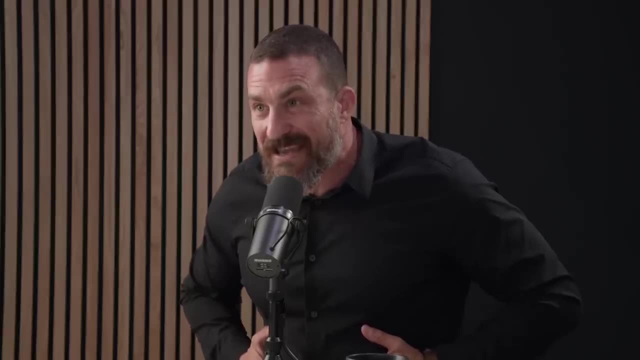 So exactly what you're saying. And in the gut it seems to create a um, the, an activation of the mechano sensors in the gut. So the perception is that the gut is full, even, or fuller, I should say, not full. 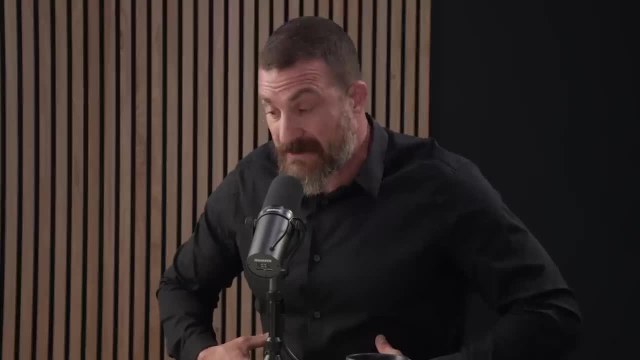 because I think people who take some of gluta don't feel bloated and that's. I don't know what they might, but but that one feels as if their gut is actually fuller because these mechano sensors, that sense stretch, are sending signals to the brain. 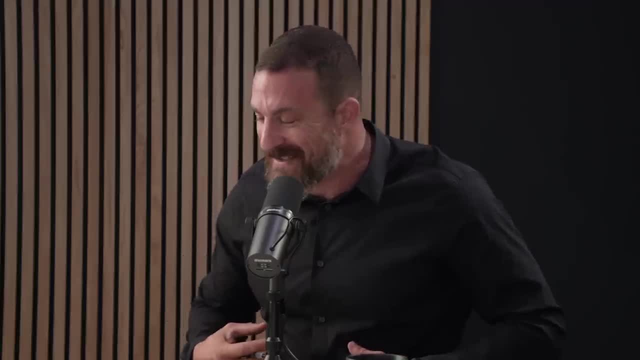 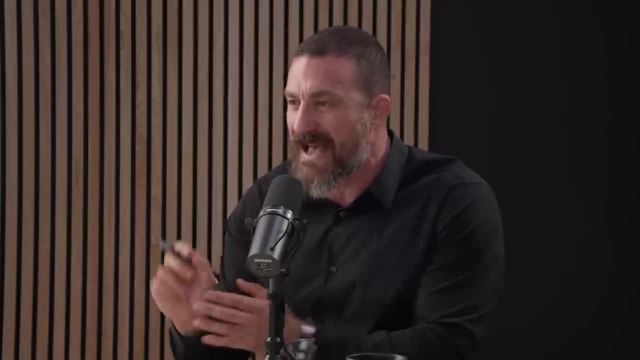 Oh, like I actually have some food, I'm not empty down there. Um, anyway, I I I'm tickled by this result, mostly because every time I hear about a drug or a or a molecule having effect, we think it has an effect at one location. 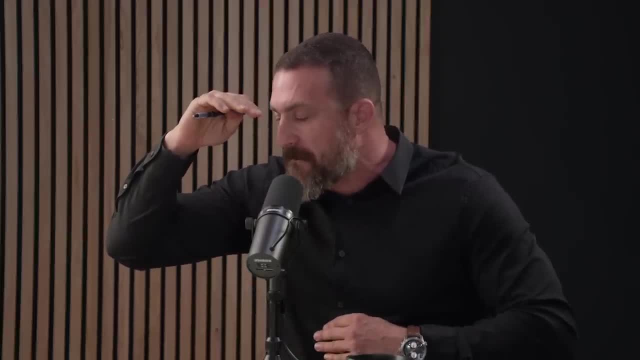 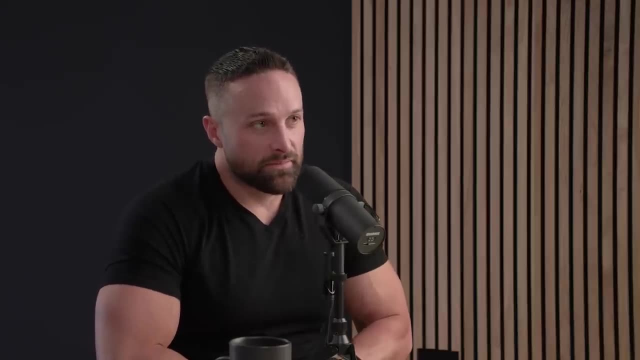 but it's kind of interesting that, especially for something like um appetite regulation, that it would be impacting body and brain in parallel. Anyway, forgive me, You can tell I'm I'm really really excited about this, And here you are telling a neuroscientist. 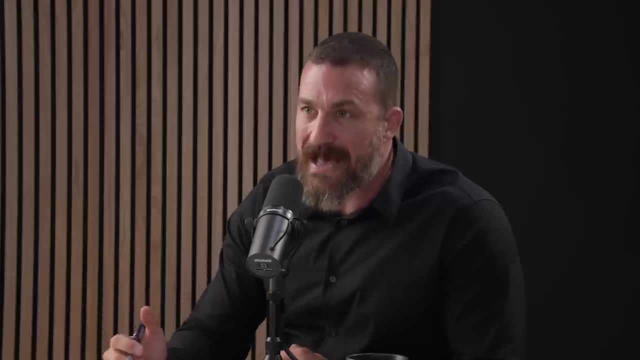 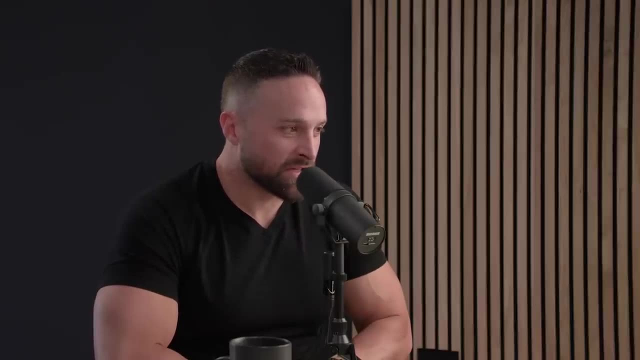 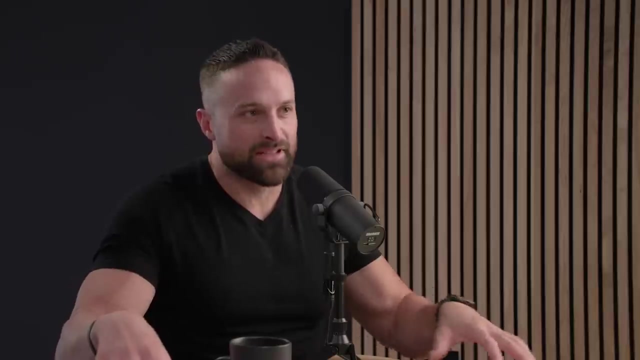 me that a lot perhaps circles back to these brain mechanisms of satiety. Yeah, I mean, I think that, and especially looking at the research on leptin, you know like we used to think: okay, metabolism is mostly like liver based. 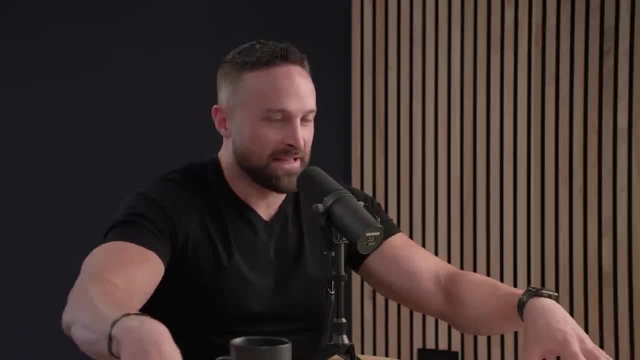 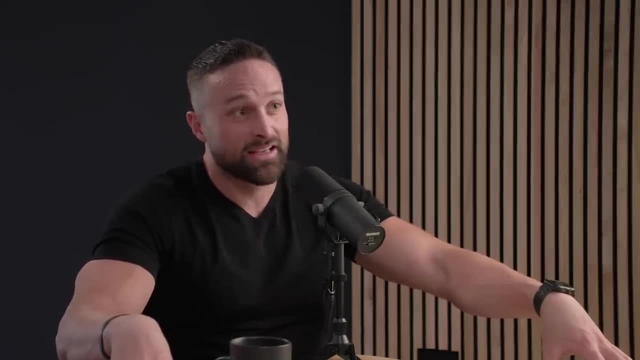 And then you know there's um, there's uh, you know metabolism and the adipocyte and skeletal muscle, but none of none of this stuff exists in isolation. There's so much crosstalk between these pathways and that's. 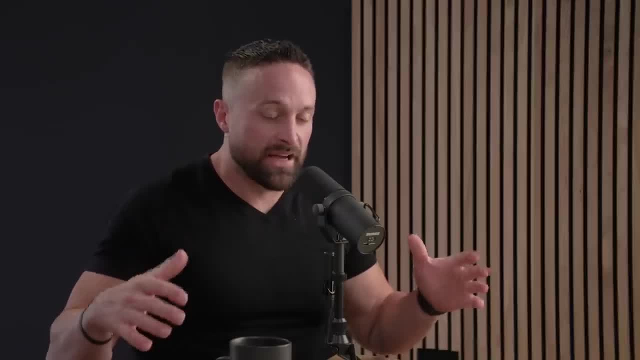 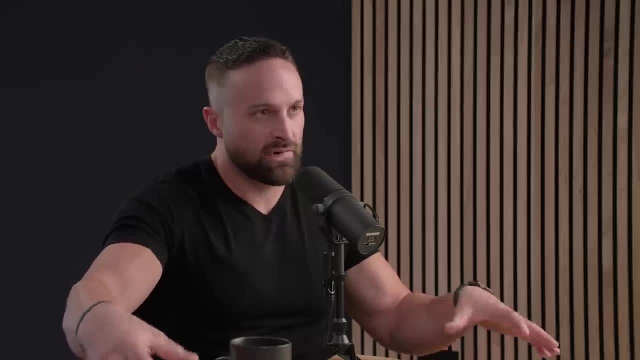 you know, when we get into mechanisms- the one of the things I love mechanisms but one of the things I tell people is: keep in mind that when you're dealing with an outcome right, So like when I say outcome based, we're talking about physical outcomes like weight loss. 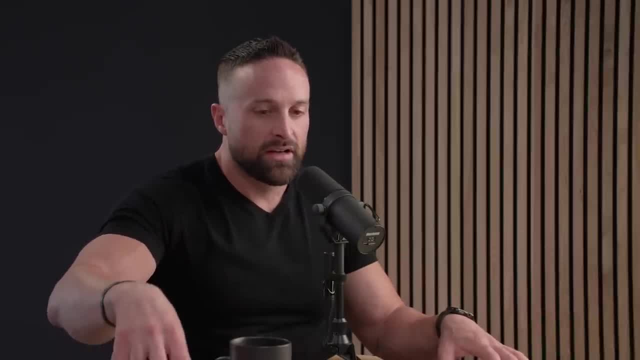 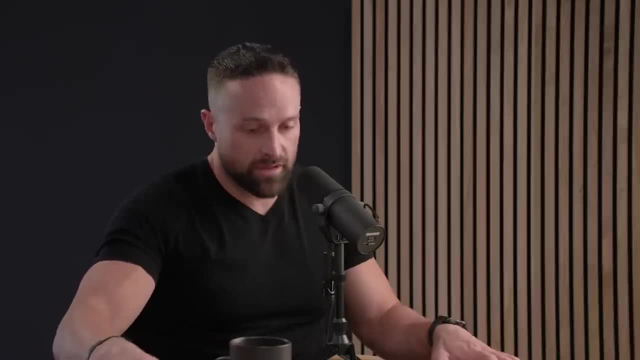 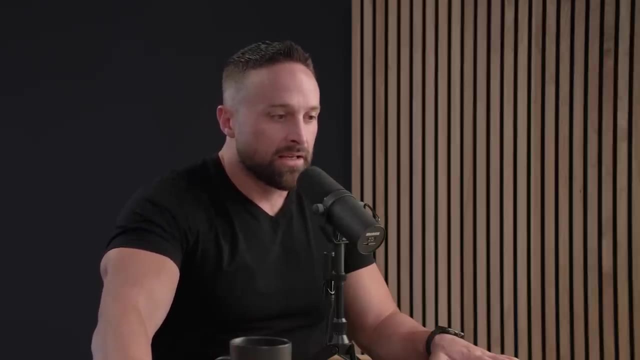 fat loss, changes in blood markers, whatever, though, that is the summation of thousands of different mechanisms. So sure, Sometimes you can affect a mechanistic pathway and you get kind of straight down the line outcome, but not always you know whenever you make a treatment or 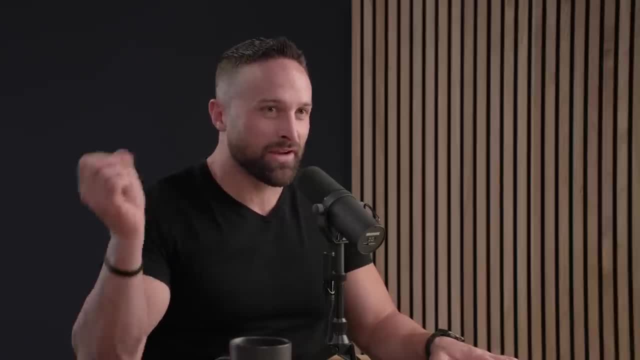 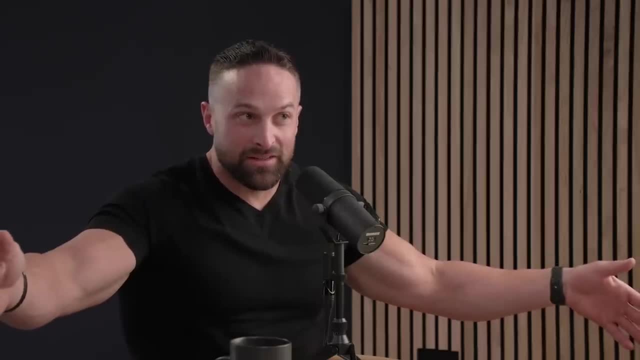 you know kind of anything into the system. it's like throwing a pebble in a lake. right, It creates ripples and we don't always know what those are going to be Right, Um, and that's why I mean. 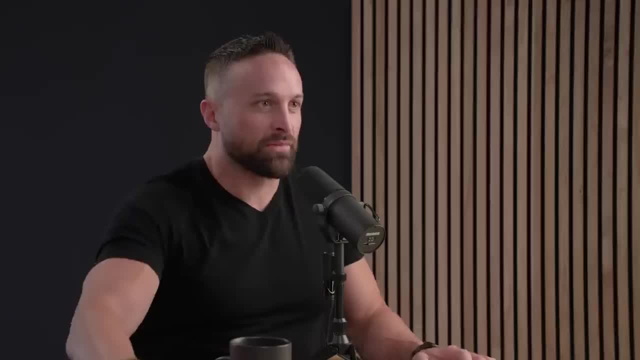 we've seen. you know certain drugs well, it works on this pathway, and then they list off all the side effects and you go. well, how would it create that many side effects? It's. it's because nothing, for the most part. 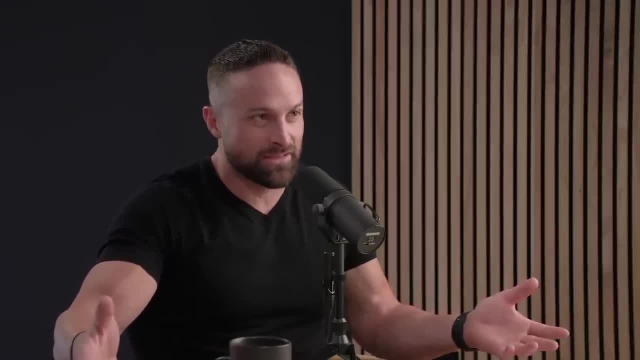 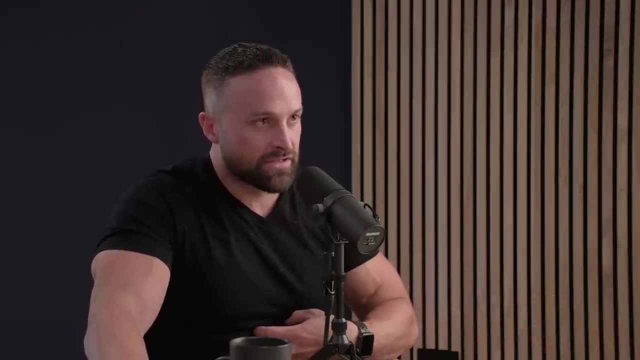 they don't just work in one place, There's multitude of places it works. Um and and to your point about um semi-glutide and the effects on uh mechanical sensors, it's probably why a lot of people report actually kind of like no, low grade. 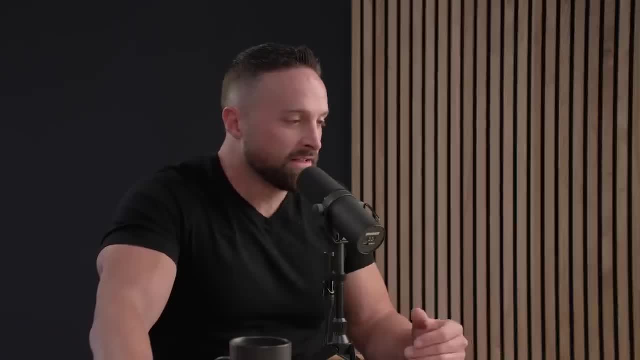 nausea, um, when they're using semi-glutide. uh, because of that, because if you're, you know that feeling is usually not like a real comfortable feeling, but I mean it will get you to not eat. So 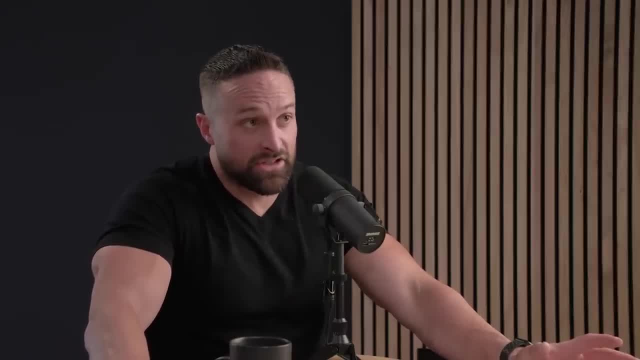 so I think there's absolutely likely a connection. Uh, but we haven't fully elucidated how that works. And when you think about how complicated the gut is, I think I heard something like: there's more, you know, there's more cells in our microbiome by far than there are in our body. 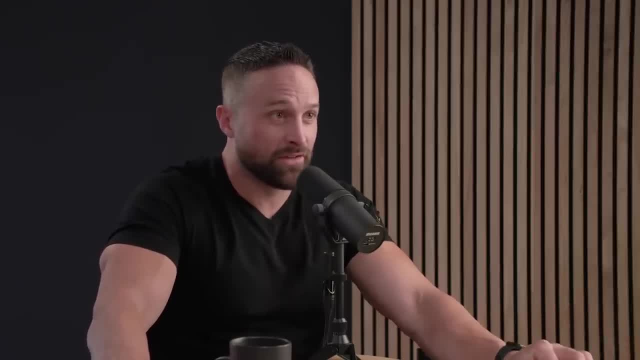 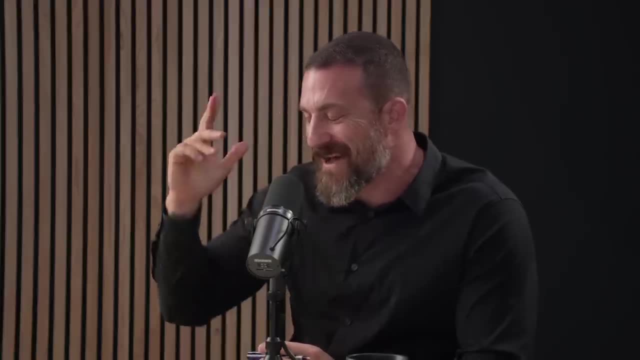 So we're actually more in terms of a cell per cell level. we're actually more bacteria than we are. You carry out right. There's a Justin Sonnenberg, who's one of the world experts on microbiome. He's in the lab upstairs from mine at Stanford. 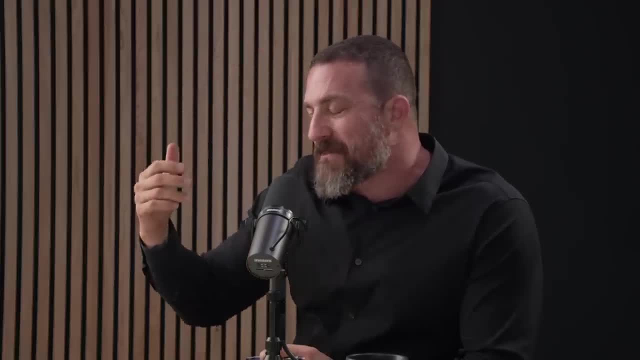 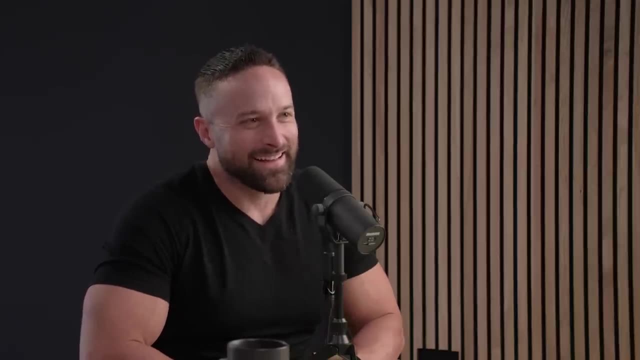 And, um, he has this idea. It's just an idea that, because we are indeed more bacteria than we are cells, the question is who's the host and who's the passenger? you know, like, maybe we are, just maybe they're exploiting us to take them around and interact because they 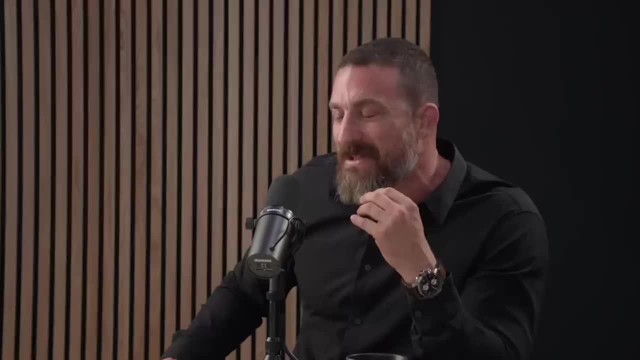 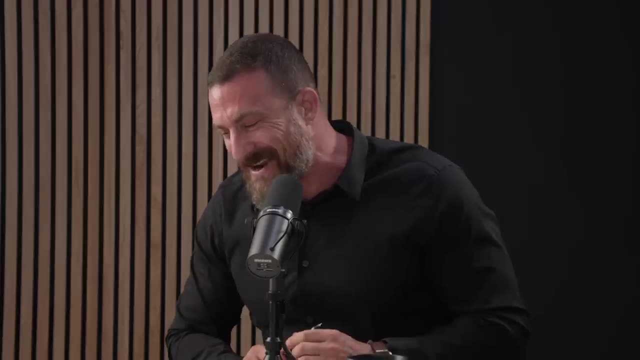 interact and grow on one another. And so this idea that this freaks people out- Lex Friedman will love this- that maybe human beings are just actually the vehicles for the microbiome and not the other way around. Anyway, kind of a um. 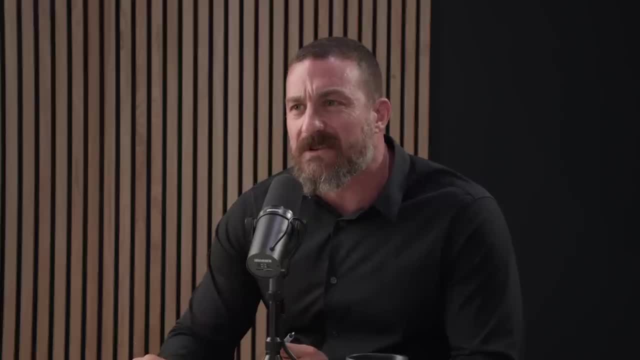 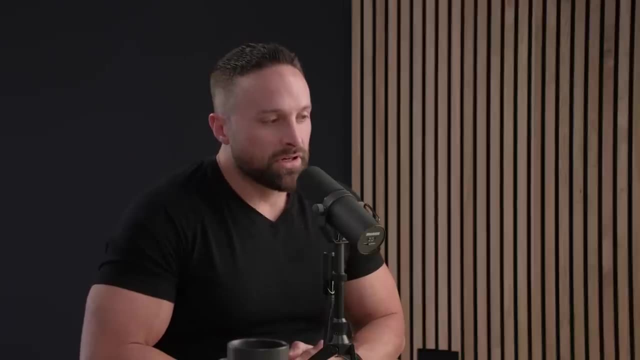 a scary thought: Um, do you do anything specific, Specifically, to support your gut microbiome? Are you a probiotic guy or a fermented foods guy or a fiber guy? So again, I'm going to kind of go straight down the line from: 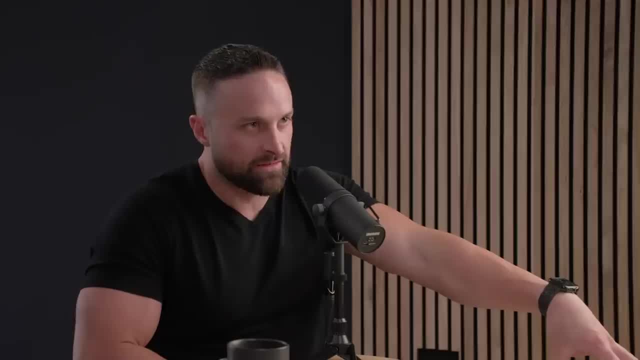 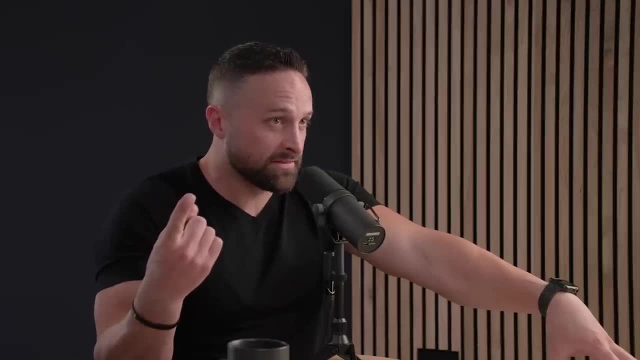 what I've heard from Suzanne and other experts. So if you want to improve gut health, one of the biggest levers- the three biggest levers you can pull- is not eating too many calories. exercising: There's a. there is a connection between exercise and the gut and fiber. 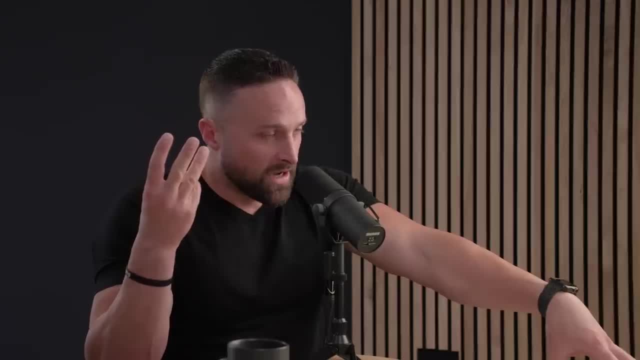 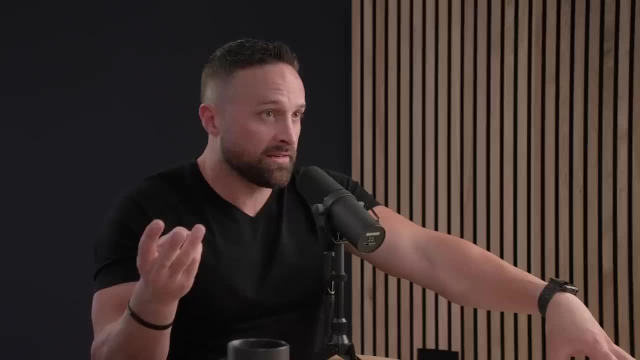 So we it is of the things we know. dietary fiber seems to positively impact the gut because it is a what's called a prebiotic, So your gut microbiota can take especially soluble fiber, Although there's actually some evidence. 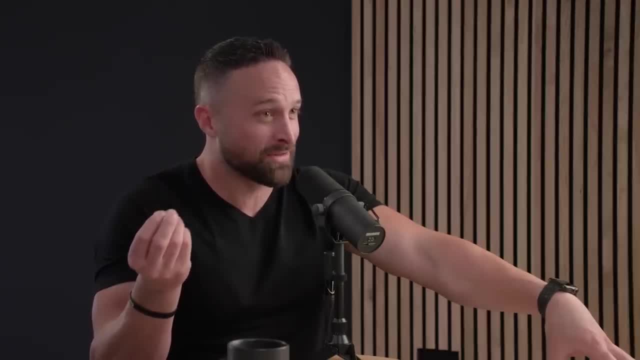 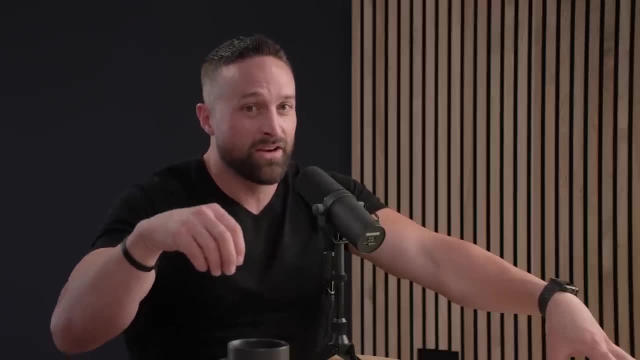 at least in mice, that they might be able to use some insoluble fiber as well. Uh, I think Suzanne was doing a study looking at hemicellulose and actually seeing that some like specific forms of microbiota flourish with hemicellulose. 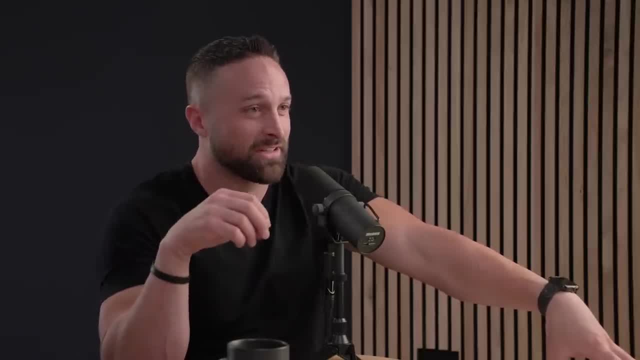 suggesting that they may actually be getting some kind of fuel out of it, which is really interesting. Um, but again in mice. so you know, just huge caveat. So your gut microbiome can produce these short chain fatty acids from uh. 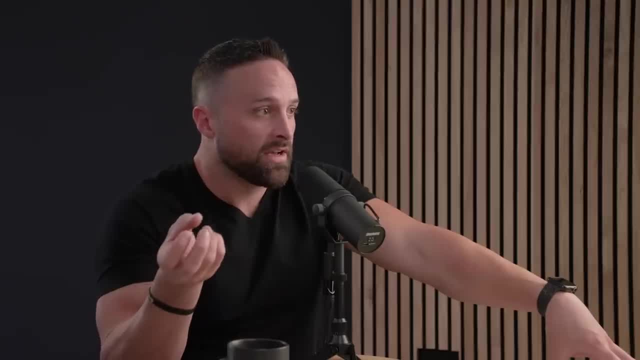 by fermenting, uh, this, this, this soluble fiber, And there's quite a bit of evidence that these volatile fatty acids, which can be then actually reabsorbed and, through the liver, that they have some positive effects. Um, like, for example, 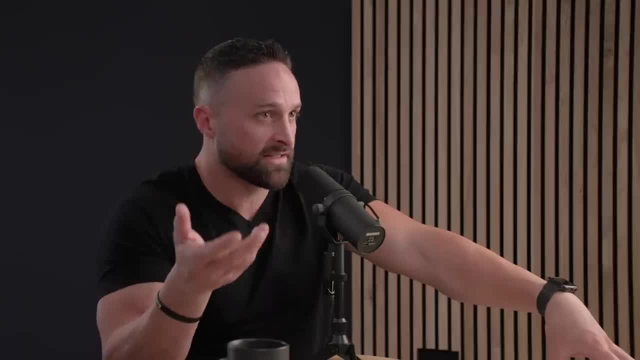 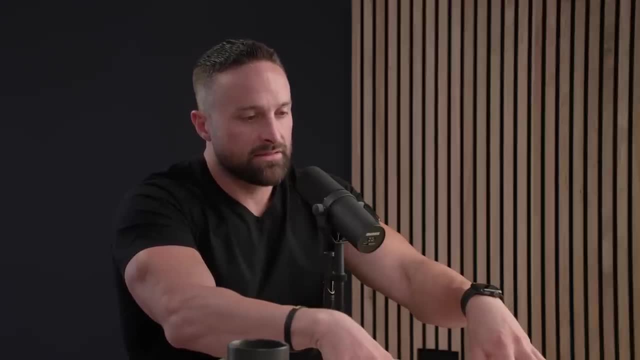 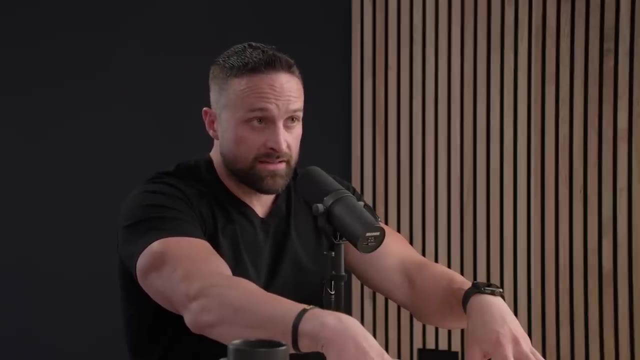 butyrate. when they've done butyrate supplementation, they've actually- they've actually- seen positive effects on insulin sensitivity. So what we seem to understand is that more diversity seems to be better. Fiber seems to be positive. Prebiotics seem to work much better than probiotics- supplemented prebiotics. 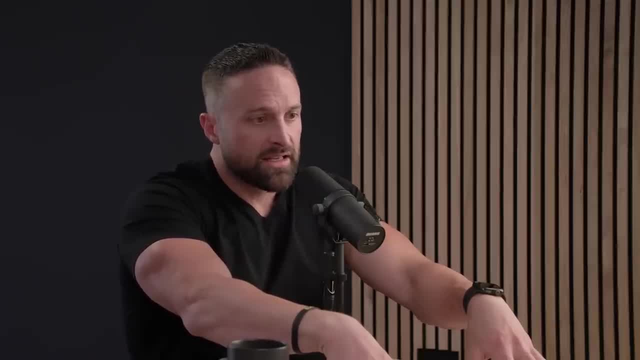 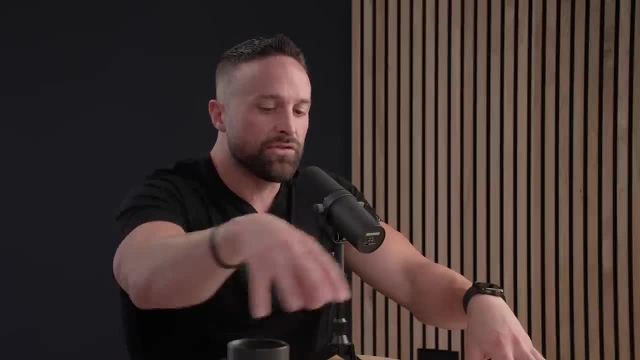 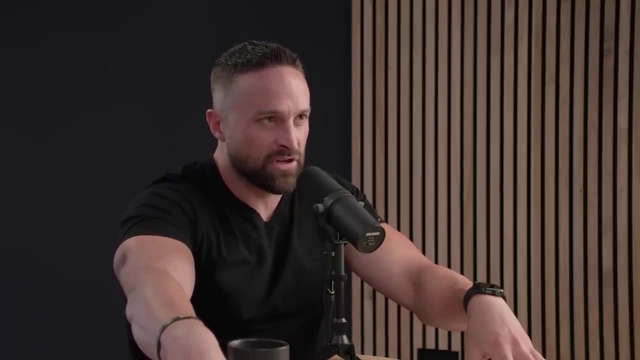 Yes. So the problem with most of the probiotics is they're typically not concentrated enough to actually colonize. And even if you do colonize, what happens is like, let's say, you colonize some microbiota that you didn't really have much of. 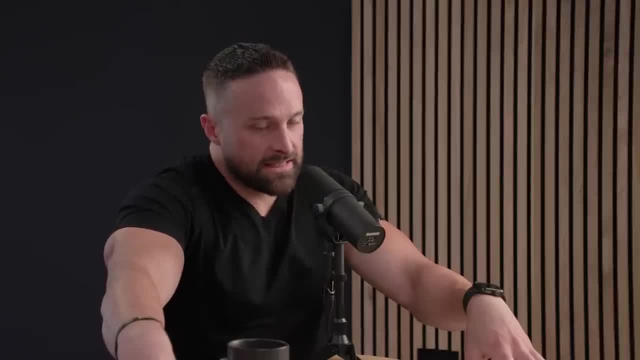 If you're not fueling it with the appropriate fiber, it's not going to stay anyway, because it's essentially going to starve. So the research seems to really clearly suggest that eating in a fiber, which is again a prebiotic- 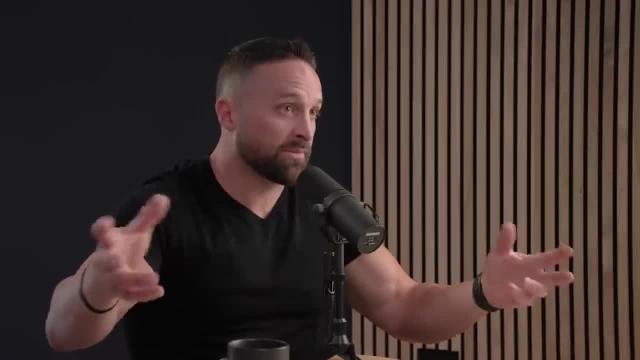 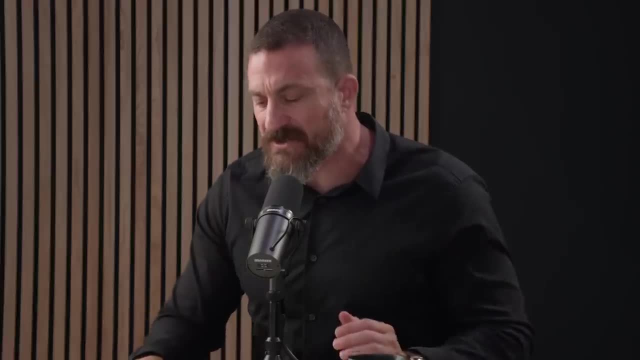 that that is a better way to get a healthier gut per se than probiotic. What fiber sources do you use? And I think I realize there's a huge array of choices out there, but people will want to have some ideas as to how they could perhaps mimic what. 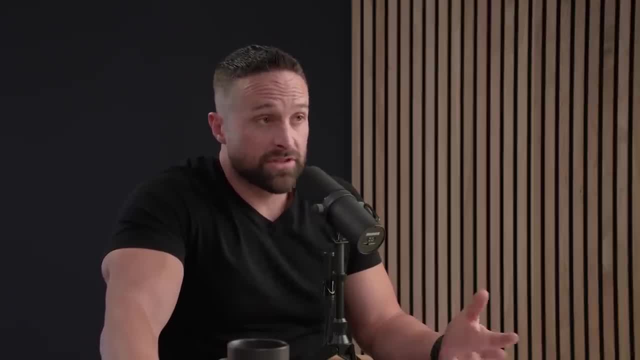 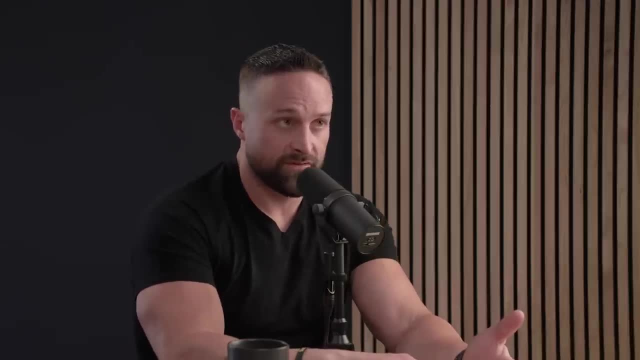 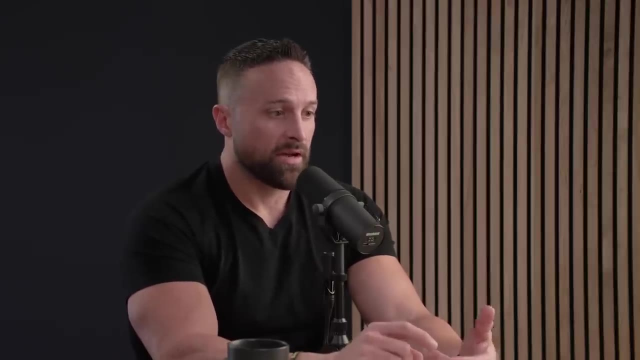 you're doing, Yeah, And I would just say diversity, right, So you know some there's. there's various evidence from various different fiber sources: fruits and vegetables. obviously you know grains, some whole grains, some cereals and then various other sources. 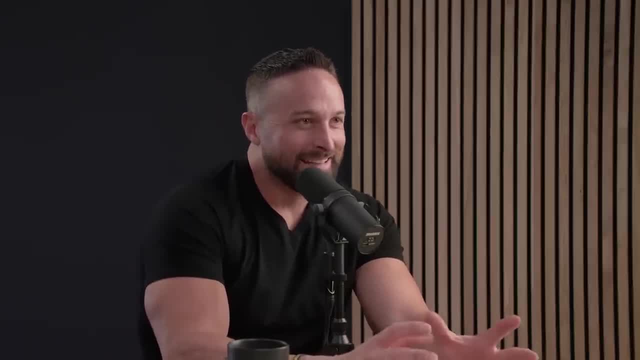 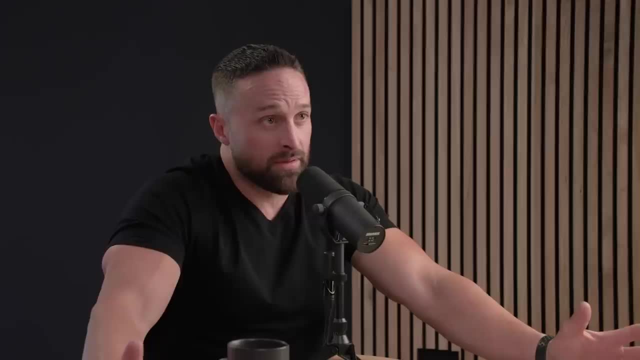 So this is one of the things where we don't really have a good idea. If you know this, one source of fiber is better than another source of fiber. We just know that fiber overall is pretty good. And one thing I'll tell people is like: 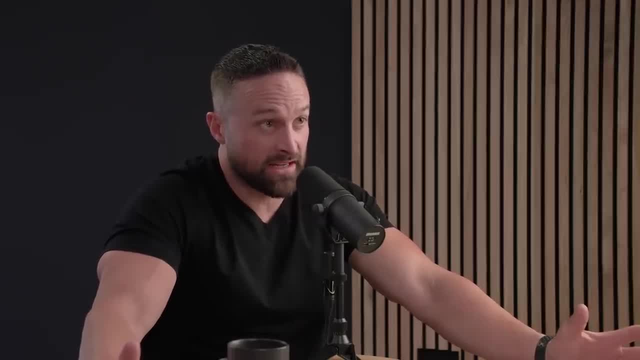 if you want a longevity hack. I mean fiber is kind of the longevity hack. If you look at some of these cohort studies, there was actually a recent really large meta analysis of over a million subjects And basically what it showed was that for every 10 gram increase in 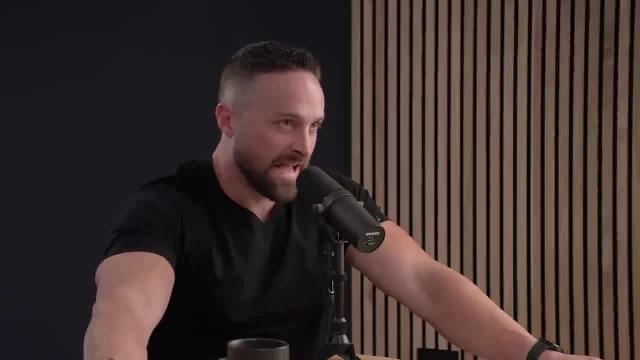 fiber. there was a 10% reduction in the risk of mortality And that extended specifically also to cardiovascular disease and cancer. So one of the things I'll tell people when they get like really into you know whether it's intermittent fasting or 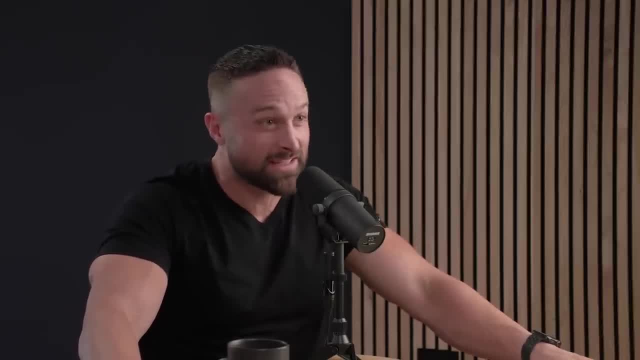 you know all these other things. so that's great. That's great. Are you eating like over 50, 60 grams of fiber a day? And I just conceptualize 50 to 60 grams. So if I already like a, 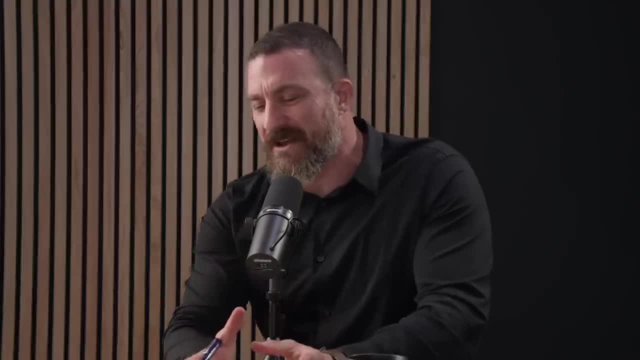 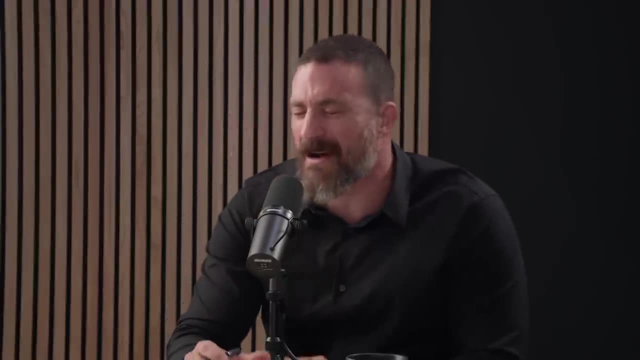 a bolt like a, let's just say, a quarter plate of broccoli and the broccoli isn't stacked to the ceiling, The broccoli is just reasonably stacked on there. I, I, I, approximately. how many grams of fiber is that If it's like a two? like two cups of broccoli is a lot, Yeah, So if you like, 200 grams of broccoli per se would probably be like five, six grams of fiber And I need to get how much per day. Well, I would say I would typically what the recommended dose is. is 15 grams per thousand calories intake, because if you're eating you know low calories it's it's difficult to get enough fiber in. But based on- and again, these are cohort studies. so but you can't do 20 year long randomized human control trials on. 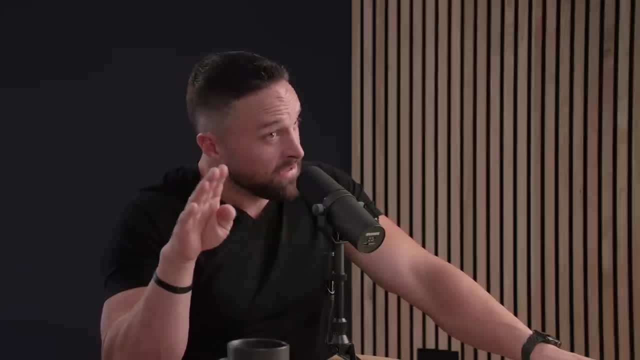 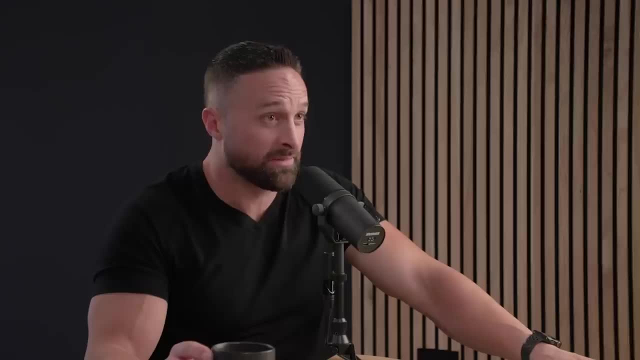 unfortunately, that doesn't really appear to be a top end, at least for the benefits of fiber, The. it probably boils down to like how much you can tolerate without feeling uncomfortable, Right, Because if you're eating like a ton of fiber, I mean. 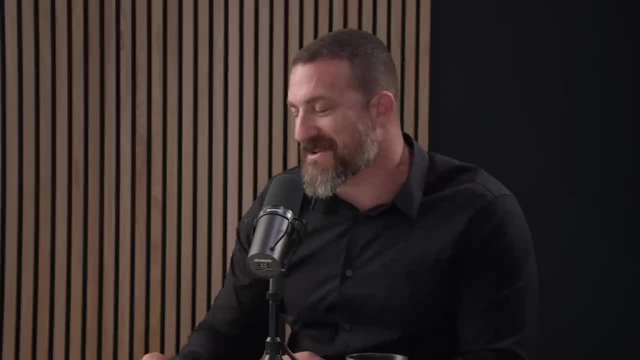 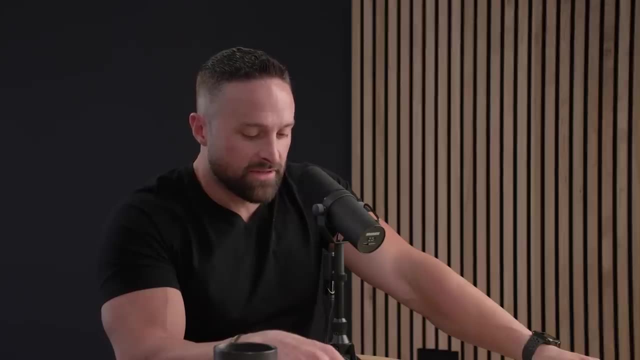 at some point it's not going to be very comfortable. Exercise becomes uncomfortable or hazardous. Yeah, And I see a kind of touching on that because I think it is important. You know, a lot of people have, kind of in the carnivore community, said 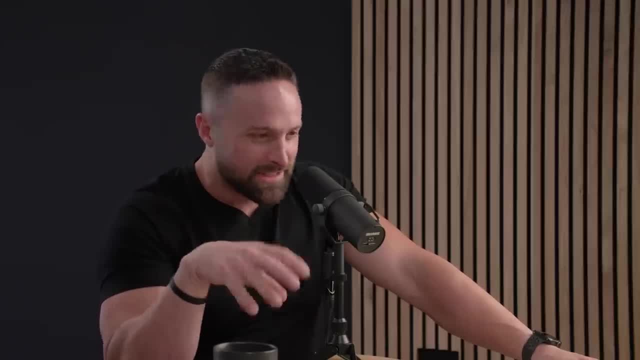 well, you don't need fiber, You poop just fine without it. And I'll always say: well, pooping is the last reason to have fiber. Like, yes, it does help. It does seem to make elimination easier. You can do it more frequently. adds bulk to stool. 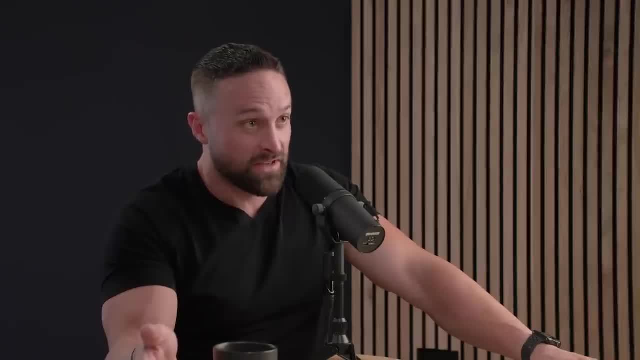 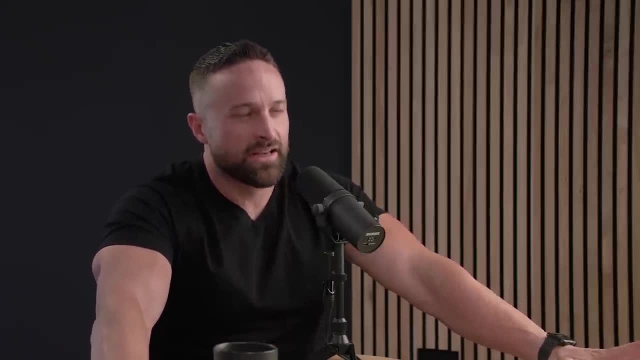 but that's not why you should eat fiber. Why should eat fiber is because of the effects of mortality, And you know some of the pushback will be well, this is healthy user bias And what I'll say is meaning: healthy people do this and 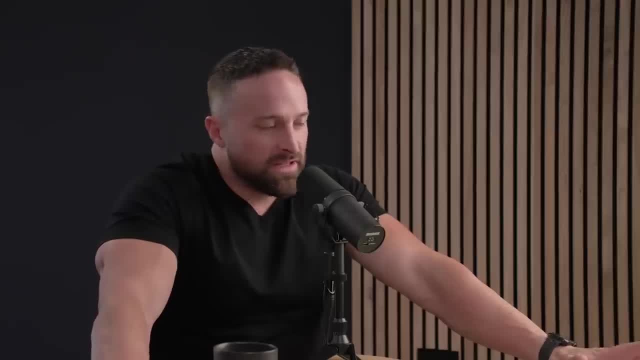 therefore, it's healthy. people eat more fiber and therefore, and I mean, yeah, there's there's something to that, but if it was just healthy user bias, typically you would see some disagreement between the studies, And the great example of that is like red meat. 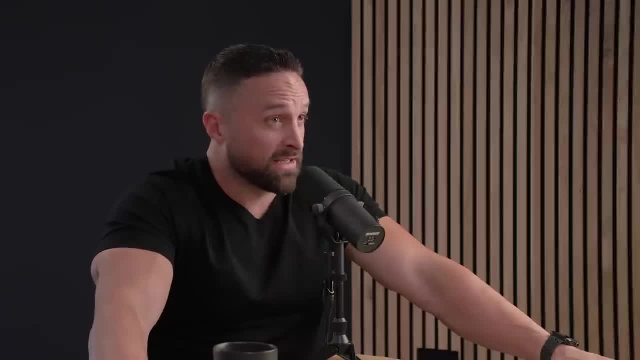 So not every study shows red meat has an association with cancer and mortality. There's there's differences depending on the population use, depending on, like what they define as high red meat, low red meat, whether it's processed, unprocessed. But I have not found a study on fiber and cardiovascular disease. 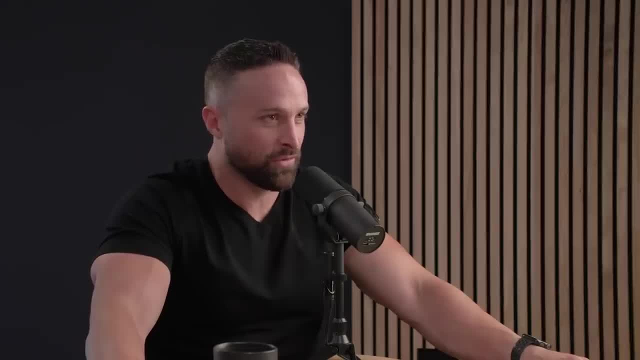 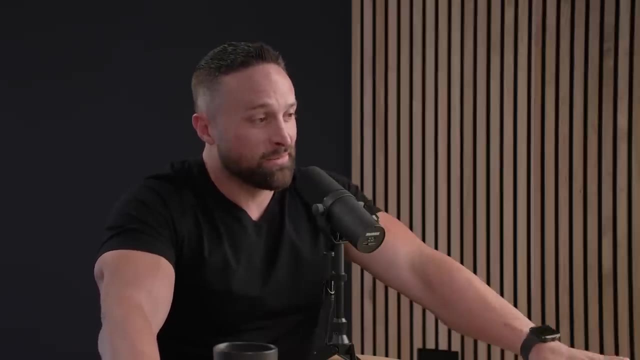 and cancer and mortality, where it did not show Improvements from higher fiber. So to me that suggests that that that effect is real. And so again, you know, as much fiber as you can get in comfortably. I would try to do it because it seems to have. 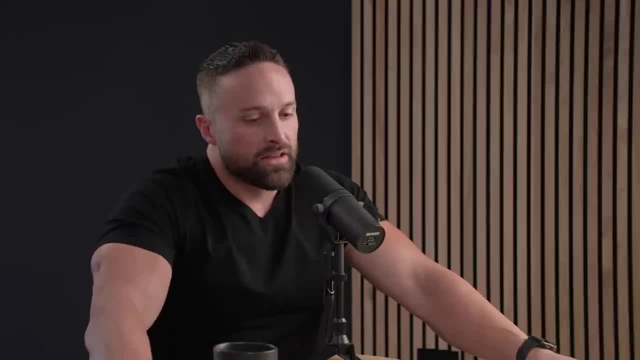 some really powerful effects and is good for the gut microbiome. The other thing that may be a consideration for the microbiome is there's some evidence that saturated fat may not be great for the microbiome, that it reduces the the prevalence of some. 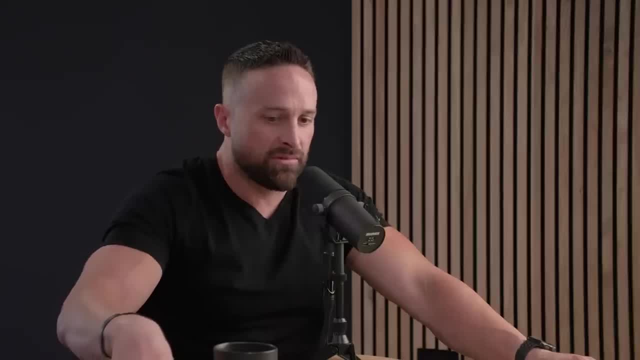 some of the more positive strains of bacteria, And that appears to be not so much from the saturated fat itself but from the bile in products that combine with saturated fat seems to have a negative effect on some of these more healthier forms of gut microbiota. 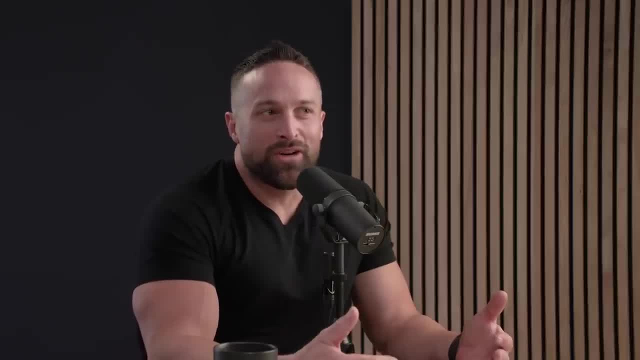 But again, this is really difficult because we don't even know necessarily yet which species of gut microbiota are positive or negative, And that's I mean this gets into some of these studies where they may. they call it dysbiosis. sounds scary. 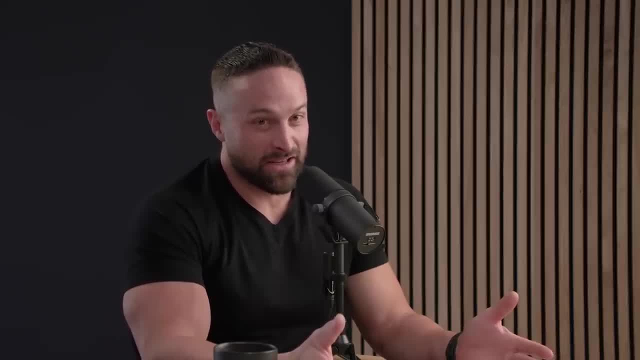 but dysbiosis just means that the gut changed. it doesn't necessarily- I mean, it doesn't- tell you anything qualitative about whether the change was bad or good, And so these are just things I think we need to keep in mind when we talk about this stuff. 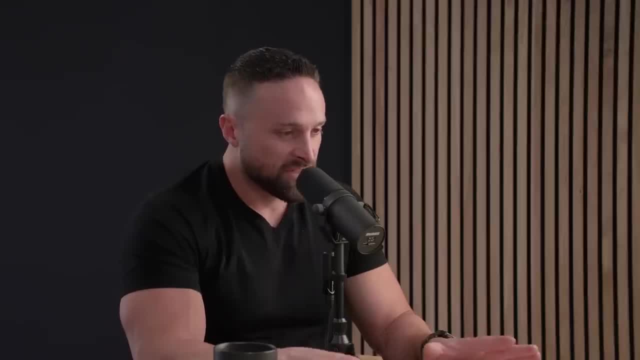 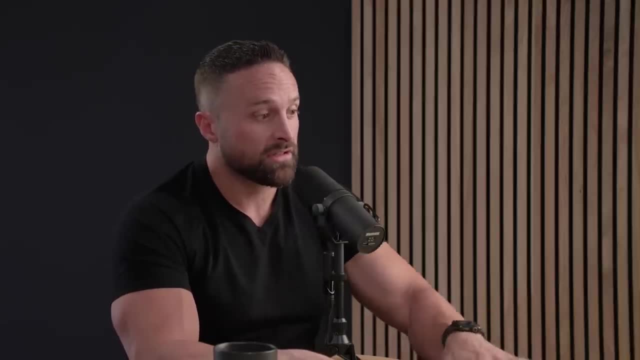 that this stuff is still very much in its infancy, but in terms of the big lever levers, I mean, it's pretty much fits with what we know about a healthy lifestyle: exercise Don't eat too much, consume a good amount of fiber from different diverse sources. 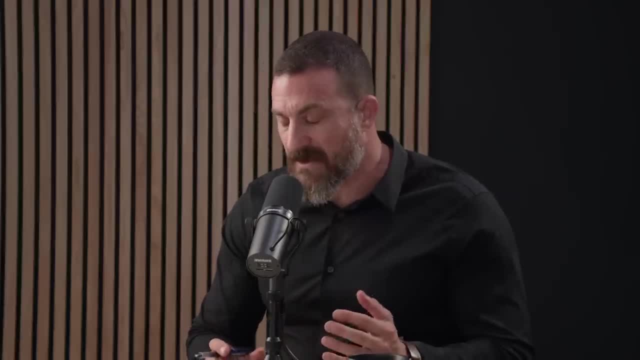 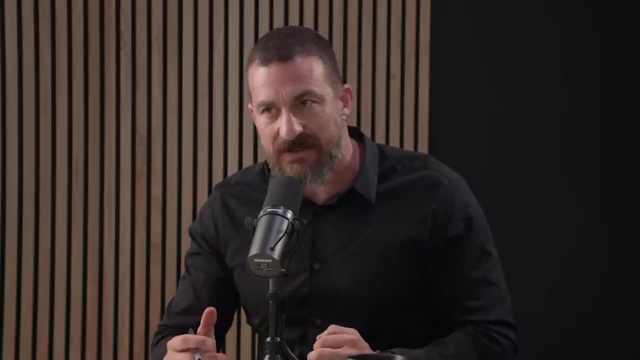 Fantastic. fantastic because it fits with what I like to think of as kind of the center of mass of evidence. Right, And I I'm starting to get some window into what your process is around: selection of studies and no one study being holy. 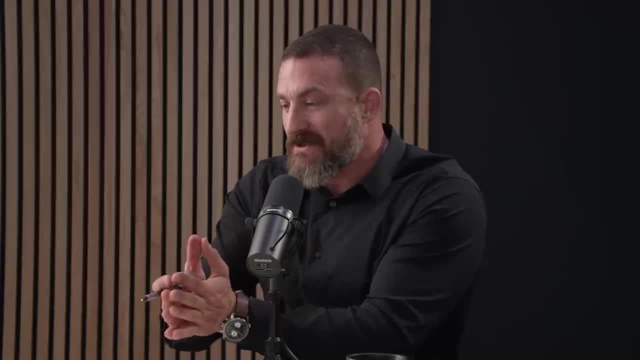 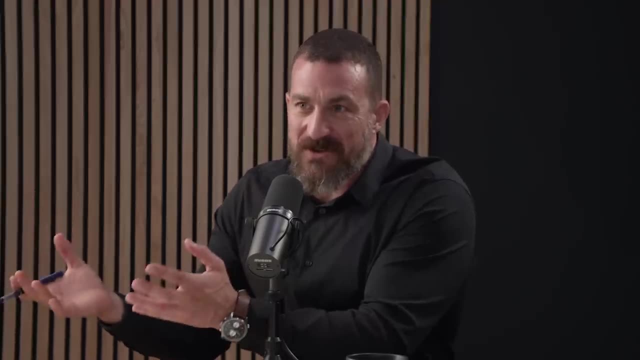 But when you look at, as you mentioned, all the studies on fiber having a positive effect to some degree or another, it's pretty hard to refute that there isn't something really interesting there. And one thing I'll tell people is: like you know, 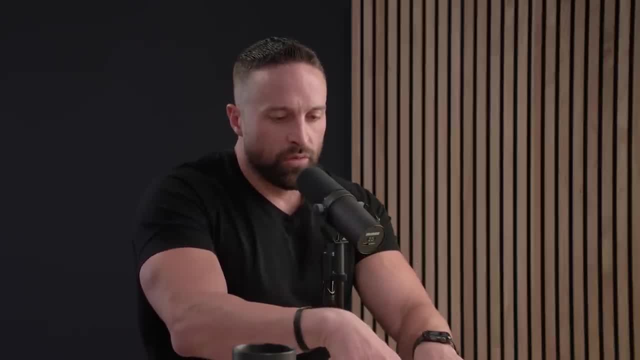 one study. I mean I don't know if you've ever heard of it, but I've heard of it. but I don't know if you've ever heard of it, but I don't know if you've ever heard of it. 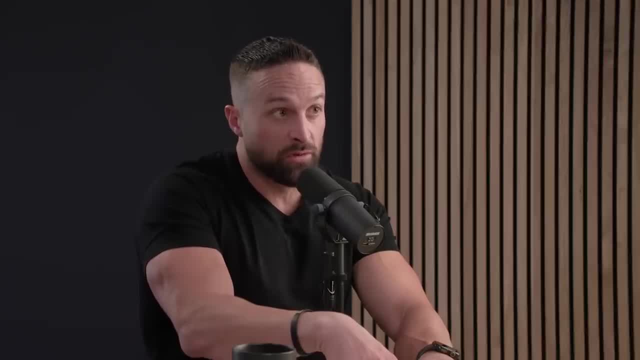 but I don't know if you've ever heard of it. but sometimes I'll change my opinion based on a single study when it's really well done and very powerful. but usually like one study is just going to move me just a little bit. 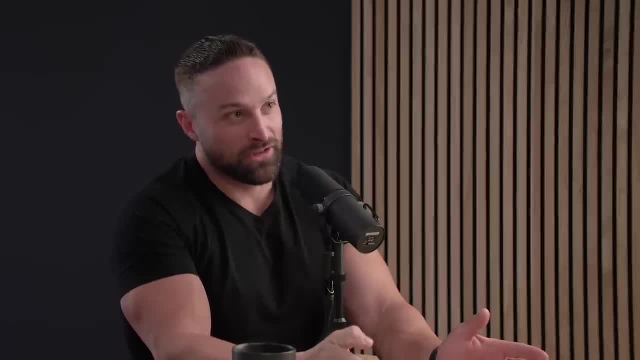 All right. And then maybe if another one comes out and move me a little bit more right And then like, very slowly I'm going to get some- I mean my my experience with LDL cholesterol is something I changed my mind on a. 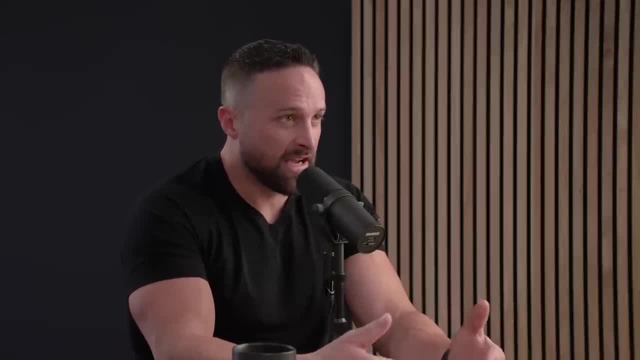 while back when I was younger- like circa 2005,, getting into grad school kind of- the prevailing thought was: well, it's not so much the LDL, it's the ratio of LDL to HDL, That's what matters. And probably about five years ago. 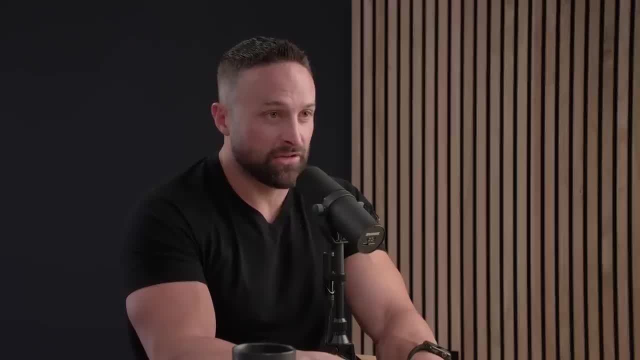 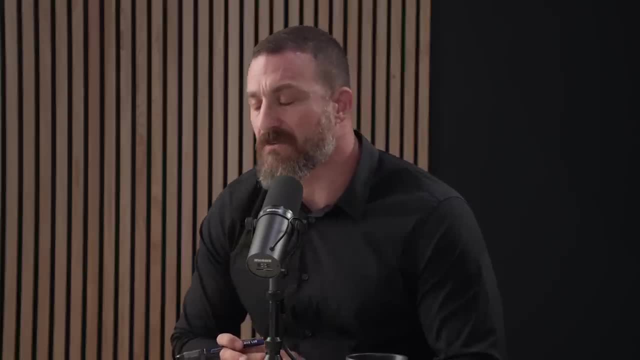 And I was. I was pretty strong about that opinion And then, five years ago, looking at these Mendelian randomization studies, I kind of went: I can't hold this position anymore. What's your new? what is your revised position on LDL? 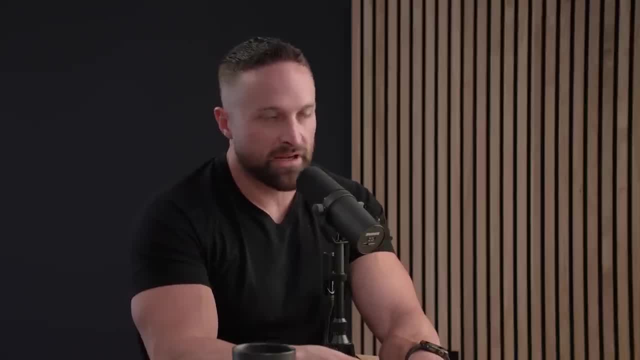 So if you look at the research, HDL is important because it's a marker of metabolic health. If you have high HDL it suggests that you are metabolically quite healthy. You very rarely will you have high HDL and like high CRP. 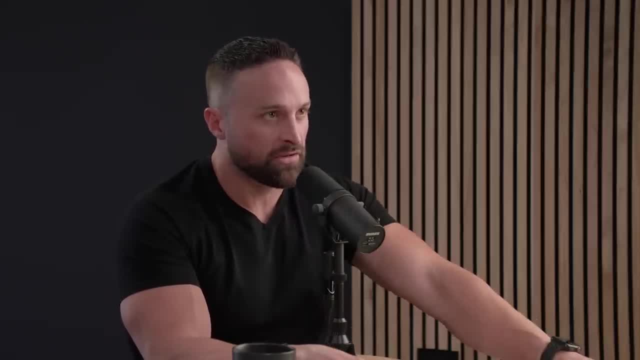 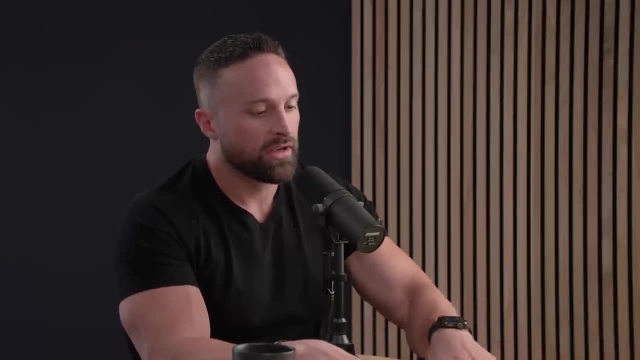 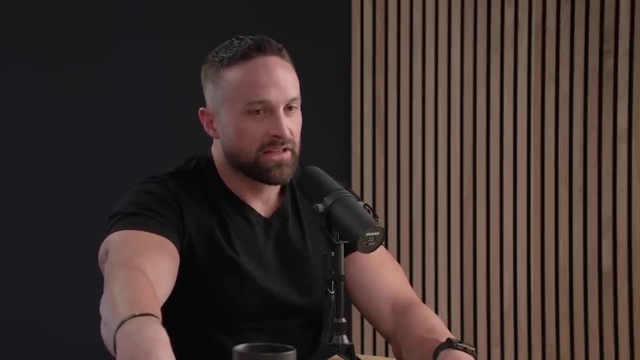 which is inflammatory marker or dysregulated blood glucose. almost exclusively people who have high HDL will have good biomarkers of metabolic health. But if you take drugs that raise HDL it doesn't reduce your risk. cardiovascular disease in Mendel and Mendelian. 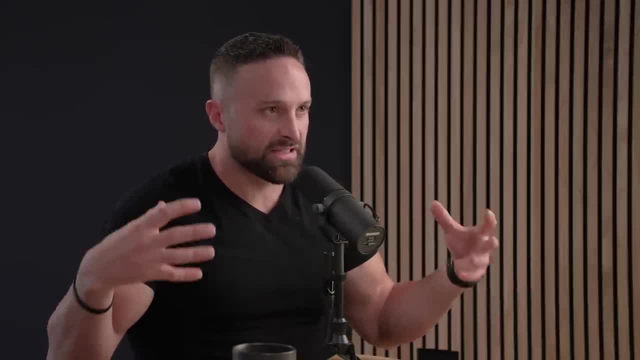 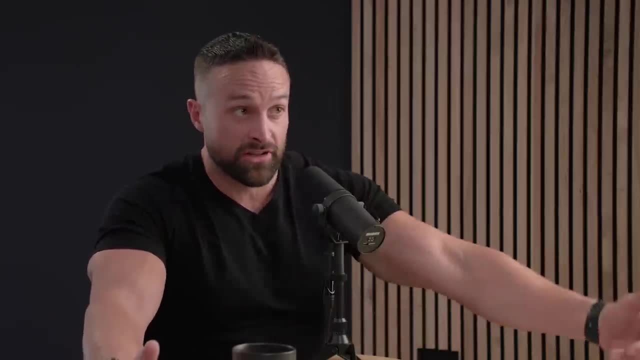 randomization studies, which Mendelian randomization, basically uses natural randomization. So some people are, in the case of HDL, naturally higher secretors or naturally lower secretors of HDL, And you know we talked about how you can't really do a 20 year human. 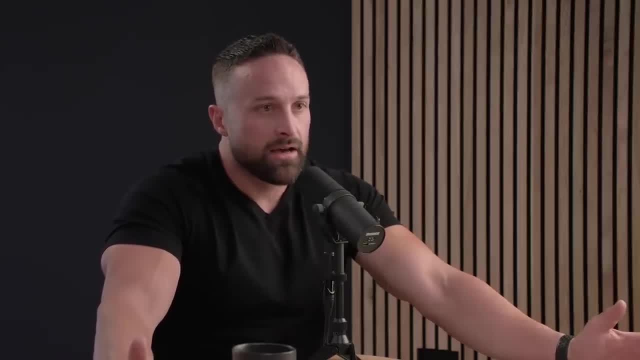 randomized control trial And when you're trying to examine something like heart disease, I mean that is a lifetime exposure issue. It's very unlikely that you're going to pick out differences between treatments in two years or even five years, I mean. 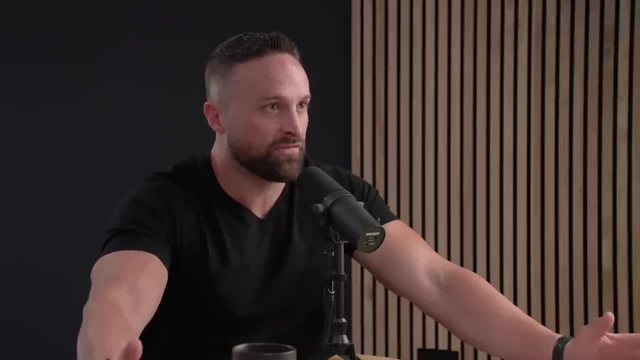 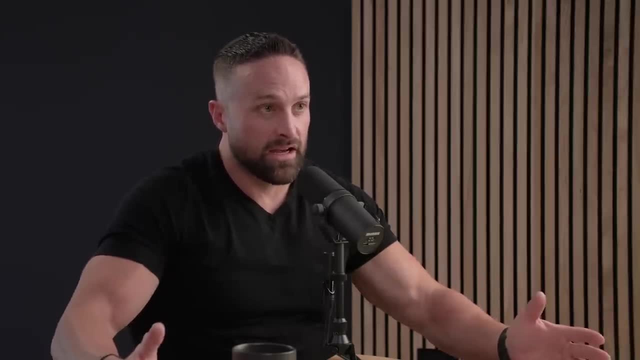 people don't develop- typically don't develop- heart disease until they're in their fifties, sixties and seventies. What Mendelian randomization allows is to say: okay, we have these people who naturally secrete more or less, so we can stratify those and look at what is their risk. 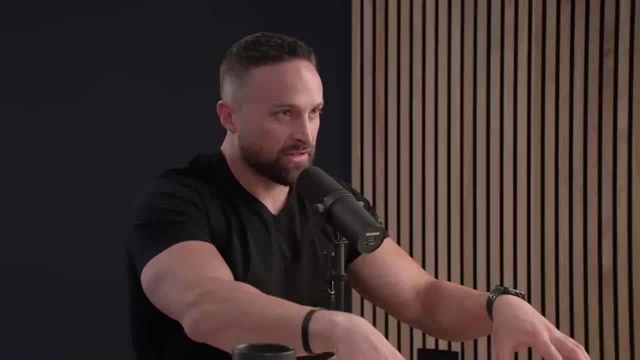 So if you look at people who are low secretors of HDL versus high secretors of HDL with holding some of the other key variables consistent, like LDL, you don't see an effect on heart disease really of LDL, of HDL, Got it. 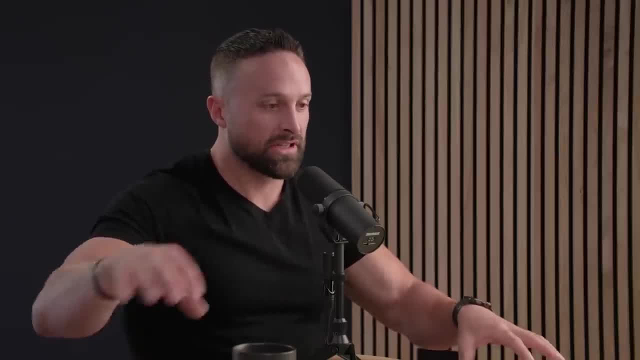 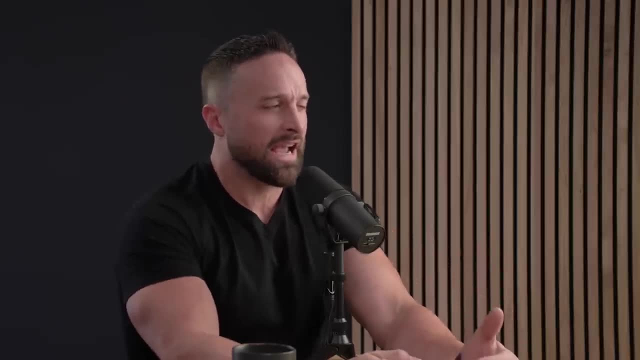 Okay, But when you look at LDL and you look at the lifetime exposure to LDL, it is like a linear effect on heart disease And we we know that it's. it's actually not so much LDL, but it's more apolipoprotein B. 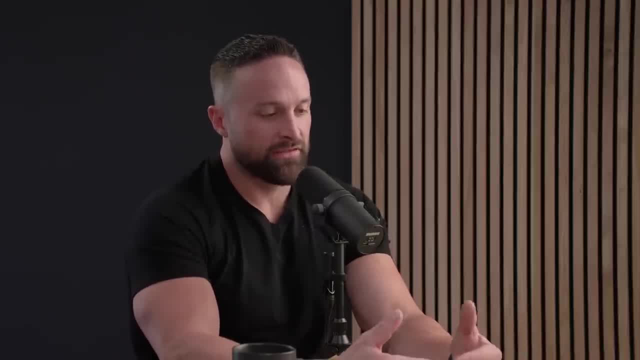 but that tends to track with LDL, just in general. And if you look at the mechanism, I mean we know that LDL can penetrate the endothelium. So there's, the mechanism is present. If we look at the epidemiology, it supports that. it's a. 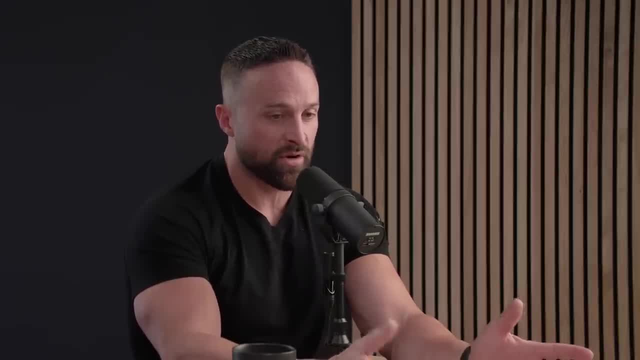 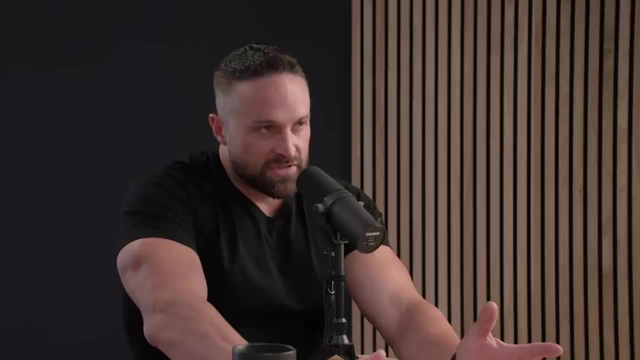 an independent risk factor, And then again these Mendelian randomization studies where we can kind of look at people's exposure over a lifetime And then we see that linear kind of dose dependent effect. To me that was convincing And I think that's a really good example of how we can look at that. 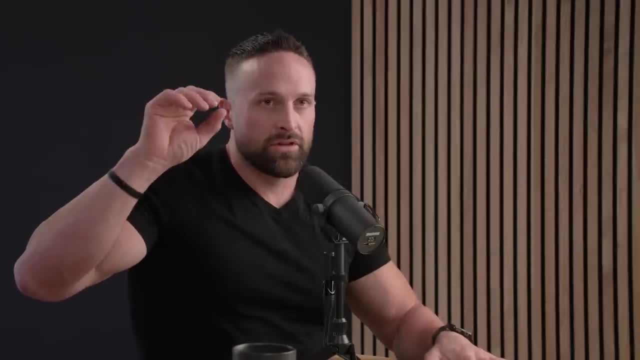 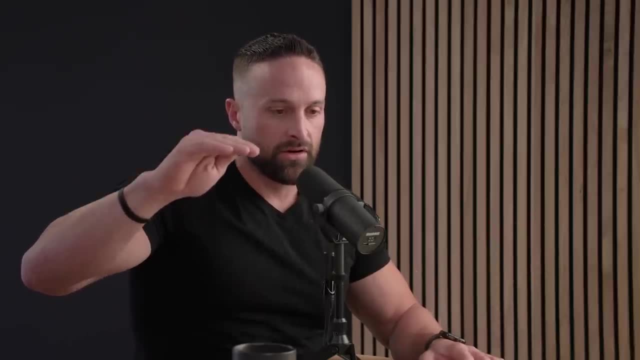 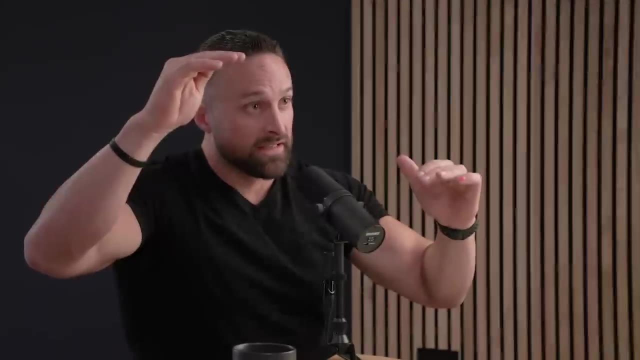 And then if you look at like some of the Framingham data, look at high. if you like stratify like high HDL versus low HDL, both groups looking at high LDL and low LDL. So if you have high HDL, low LDL. 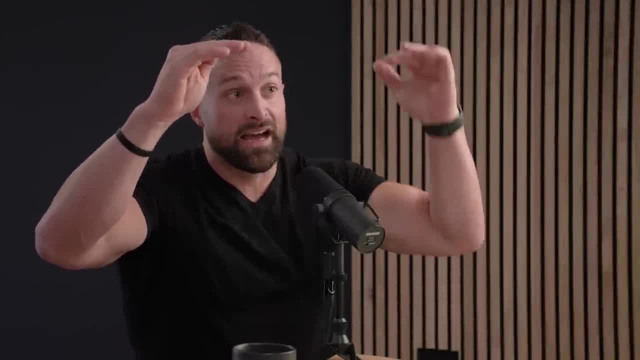 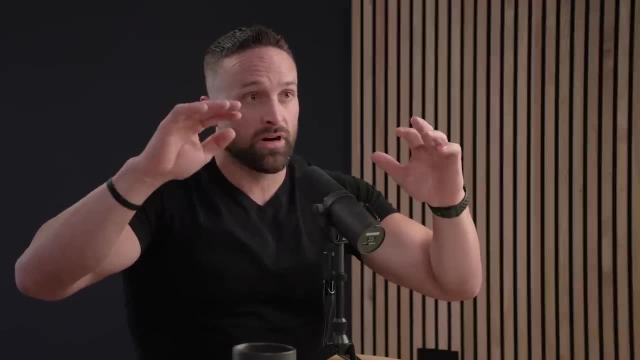 you will still be lower risk factor than somebody who has high HDL and high LDL, right, So the ratio does matter. So the ratio does matter. Same thing with it with inflammation, If you look at people who are low inflammation, low LDL. 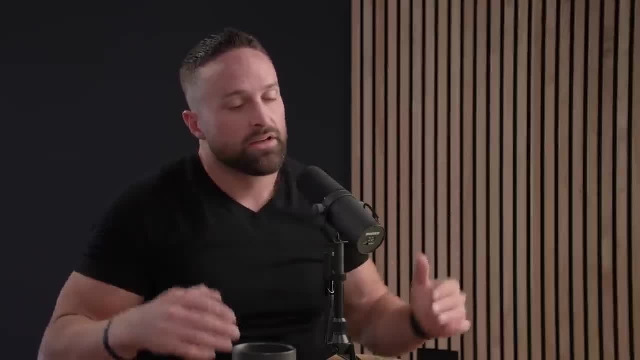 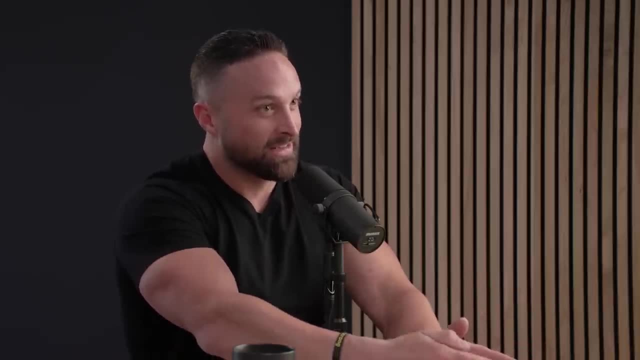 they'll have a lower risk than people who are low inflammation, high LDL. So again, that was kind of sufficient for me to change my mind, but it took. it was like not just one study came out, It was okay. Then there was another study, and then another study, and then another study. 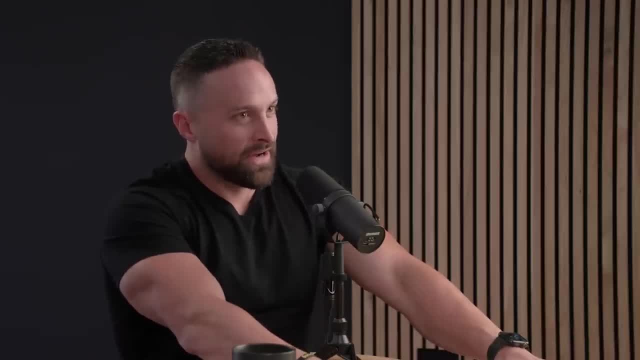 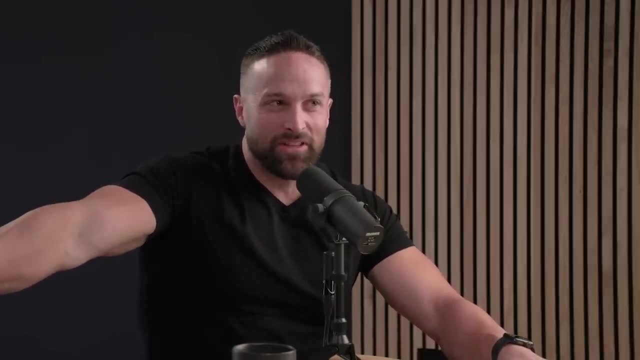 And at a certain point I go okay, well, now I either have to change my mind or I'm basically just going to be cognitively dissonant and say, nope, I don't believe all that, You know, And so I think that's one of the things to keep in. 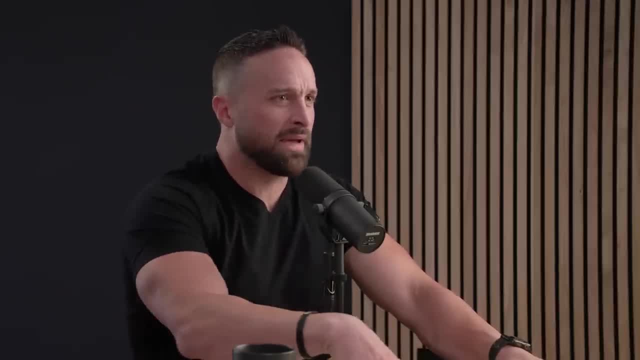 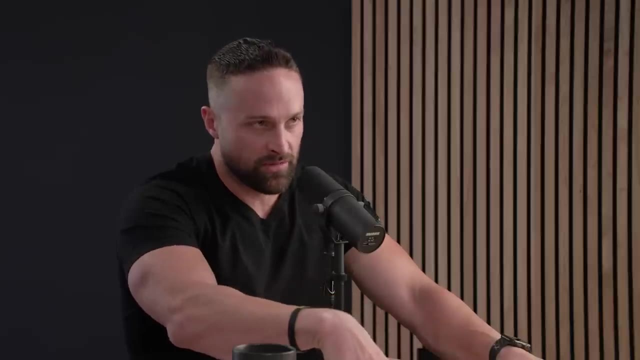 mind. People will say: oh you are, you're saying this is a bad study? Very rarely. why I call something a bad study? because data is just data. but the issue becomes how it is presented and how broadly it's applied in the mainstream media or by people on fitness influencers. 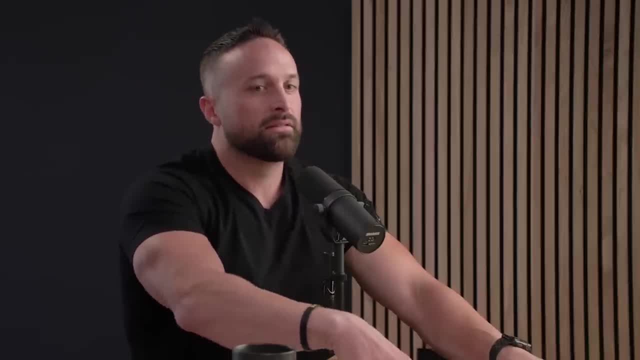 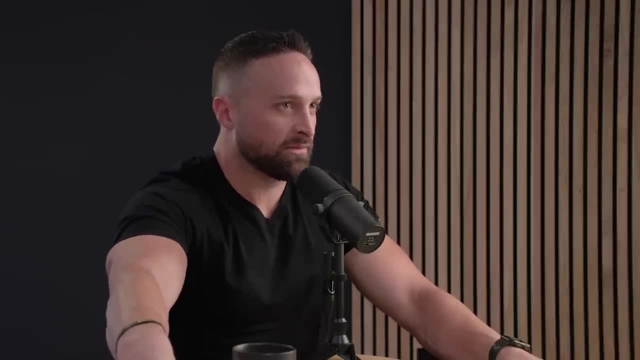 And what I'll do is try to step in and say, okay, let's consider X, Y and Z as well, And then it's not a bad study, but let's just be careful about how broadly we imply the interpretation. Yeah. 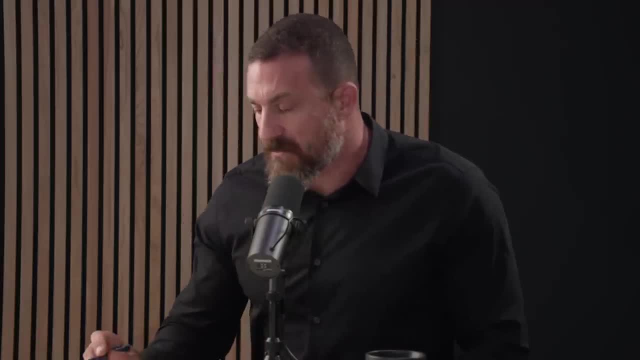 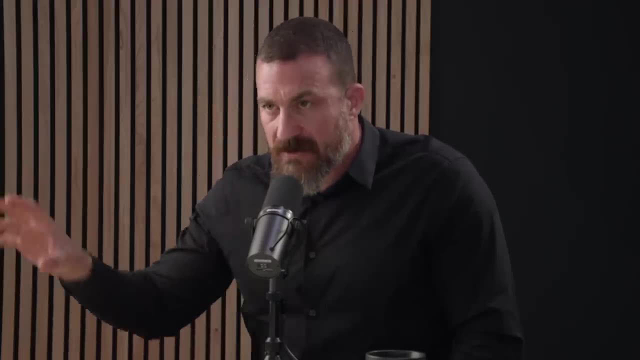 Well, and I I think you are in a very unique and important position to be able to place things into their proper context because of this- for lack of a better word- holistic view of how the psychology placebo effects also core uh core physiology. 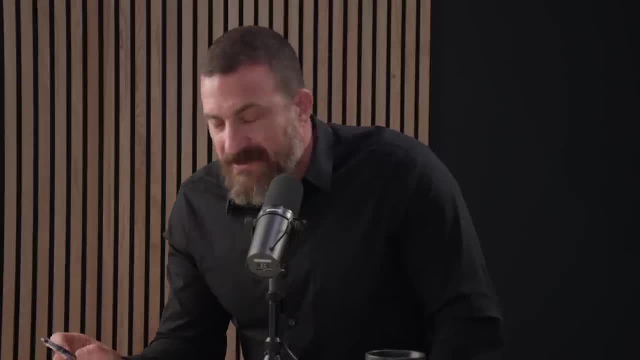 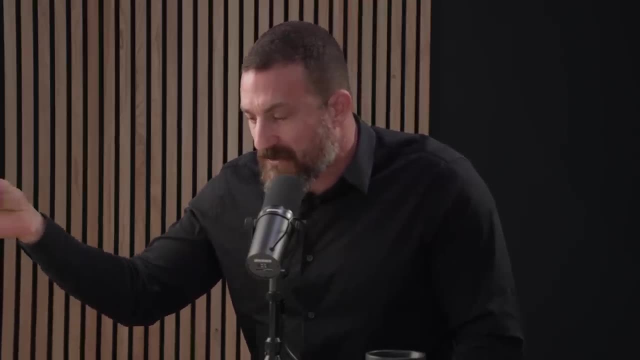 um relate to one another and so on. In fact, I think that you're training as a biochemist and then training as a new um in nutrition, with somebody who Don layman, who was pushing you to focus on outcomes. I think that's a beautiful 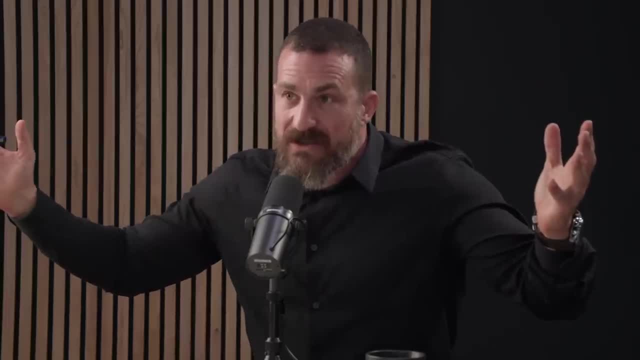 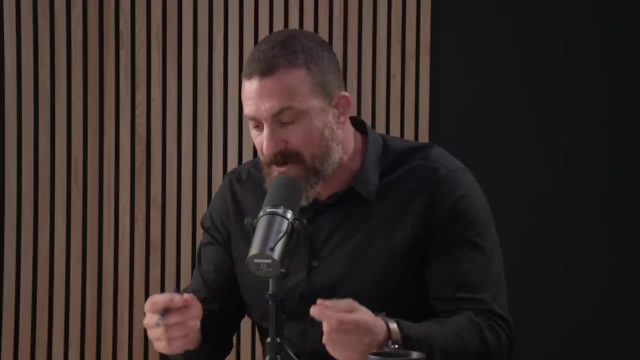 um capture of the continuum at which one can look at something, because for those of you that don't know, out there you know a lot of laboratory studies on mice and humans, for instance in the realm of biochemistry or in vitro studies. 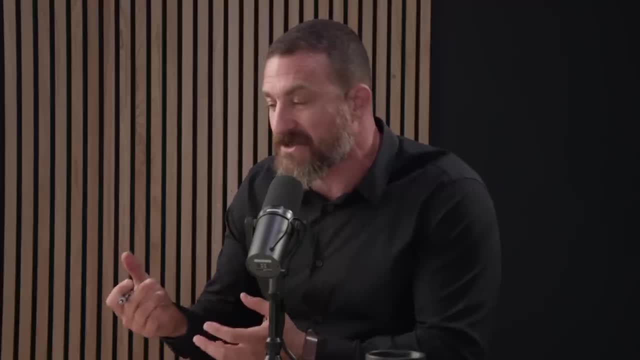 you'll see, a change in some molecule can be quite traumatic. And then the assumption is: oh, you just take. you take the drug that will change that molecule in a particular direction And then you'll get the effect you want at the 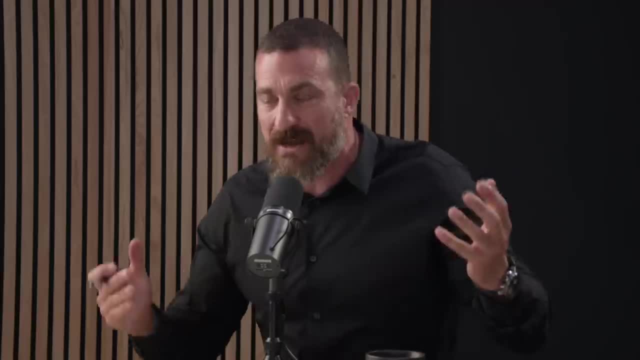 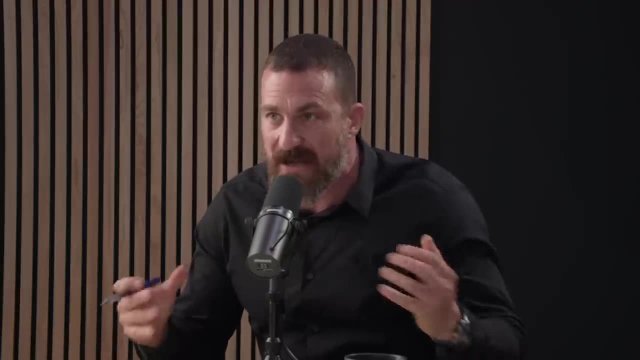 at the whole organ, organism level: the person will lose weight, The person will gain muscle, The animal will, um, not uh, have Alzheimer's, et cetera. but it just doesn't work that way because of the redundancy and this interplay. 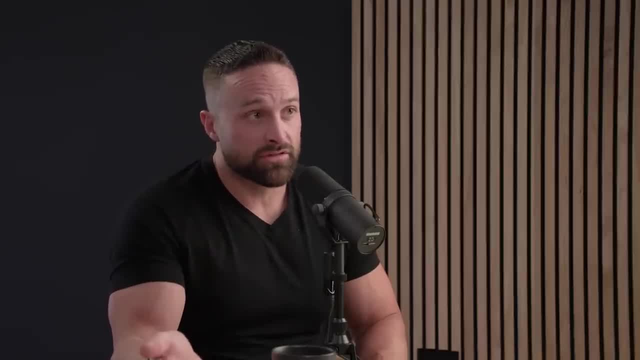 Well, a great example of that is. so my research was actually in rodents. all my, all my studies on protein metabolism, and leucine in particular, is what we were studying. Well, we know, if you give leucine, increases muscle protein synthesis. 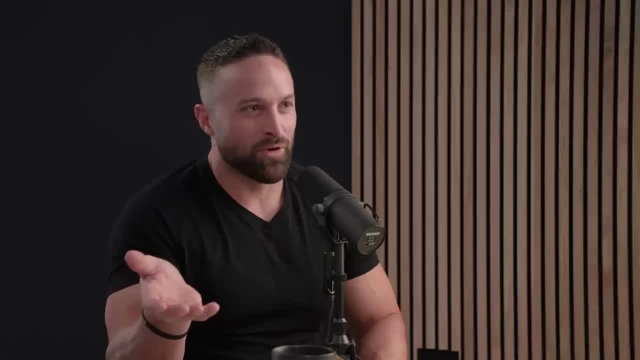 but we also know: if you supplement with leucine, people don't get more muscular. I was about to say so. all you have to do is supplement with leucine, Right, right, right. And so how is that possible? 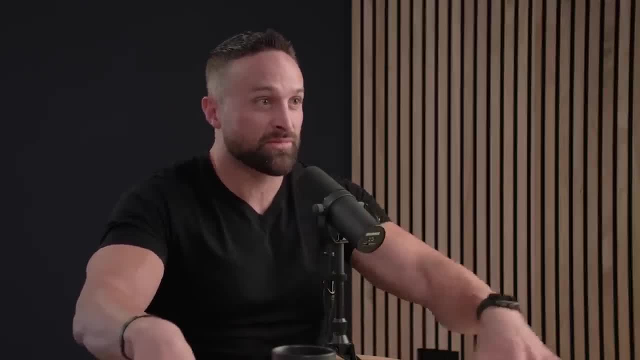 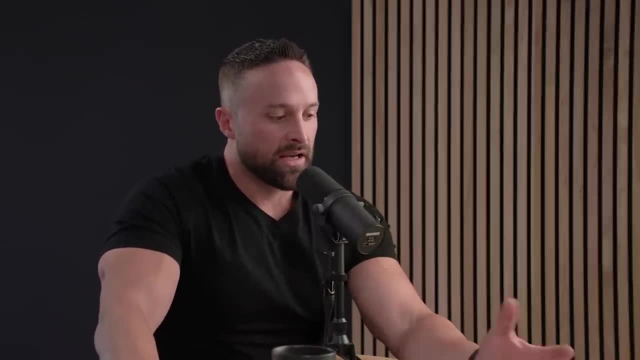 Where you know, muscle building is not just protein synthesis, It's also the balance between synthesis and degradation. So, um, and degradation just happens to be very, very difficult to measure. But, uh, a great example. And again, 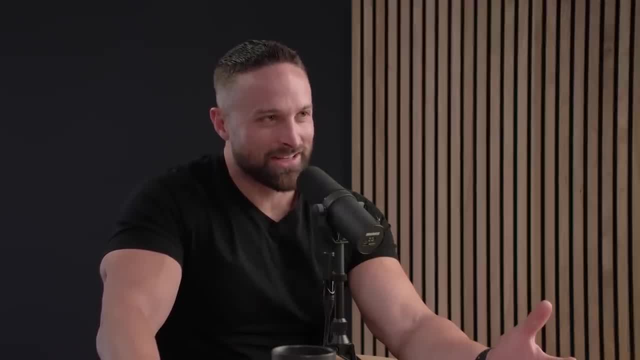 one of the cool things about my PhD was actually changed the way I ate, um, which I think is interesting. So before I had been like: uh, I eat eight meals a day, eat every two hours, try to keep meals a day. 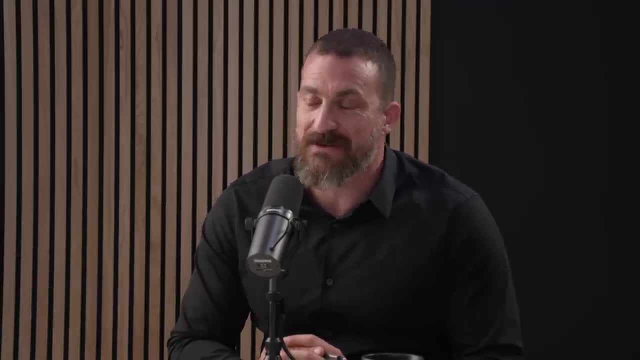 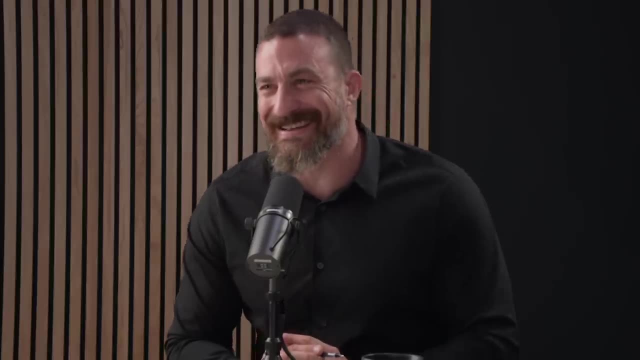 Yeah, When I got to grad school, that 30 grams of protein, get that, get that amino drip going in, was the idea right Like just have an IV hooked up of amino acids. Not really folks, Not really Yeah. 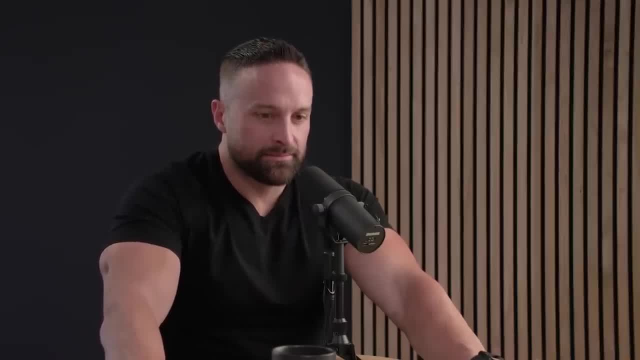 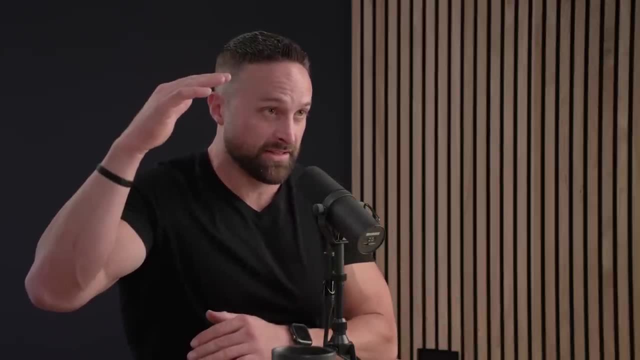 But that that was kind of the concept. But the first study I did we basically looked at: okay, a lot of people had measured the amplitude of protein synthesis in response to a meal. We wanted to see how long does this last and where does. 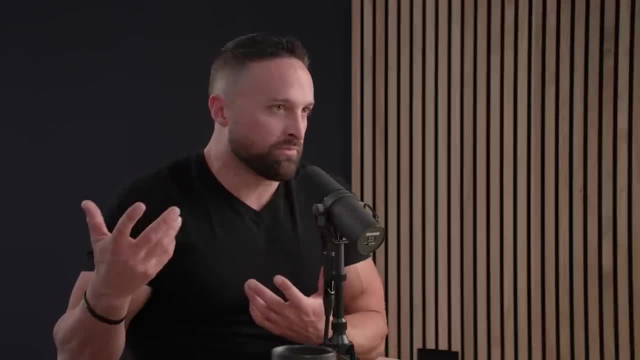 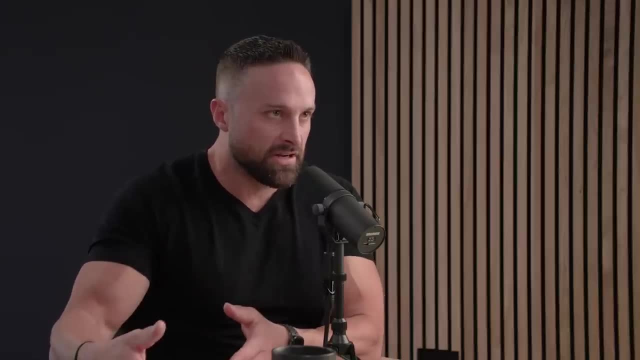 it peak Right, And so my thought was: okay. well, it'll probably track with plasma leucine You give. for those that are not familiar, leucine is the amino acid that is almost exclusively responsible for increasing muscle protein synthesis when you eat protein. 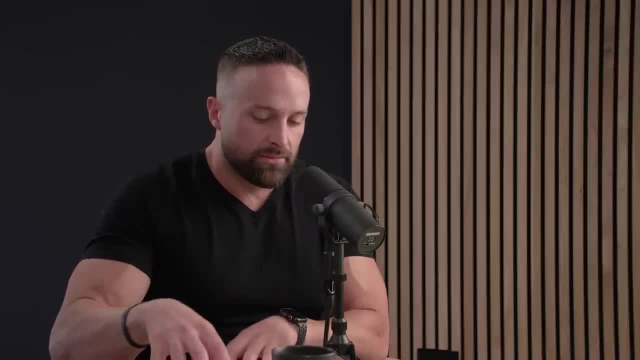 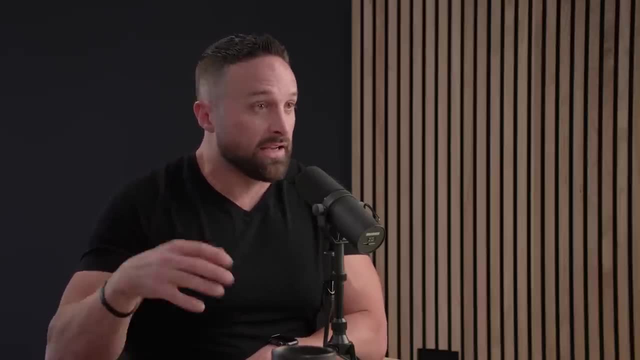 So it's. it's one of the branch chain amino acids, So we wanted to see, okay, how long does this effect last? So we, we fed these animals, uh, whey protein. And again I thought, okay. 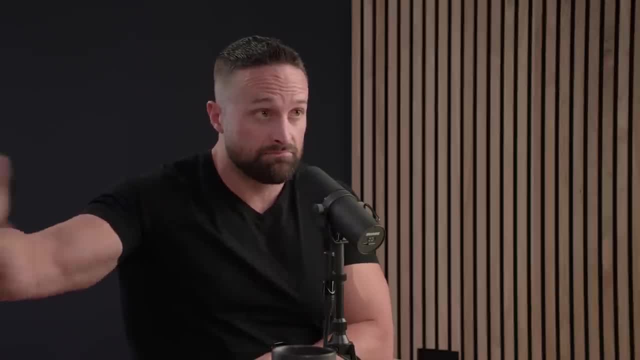 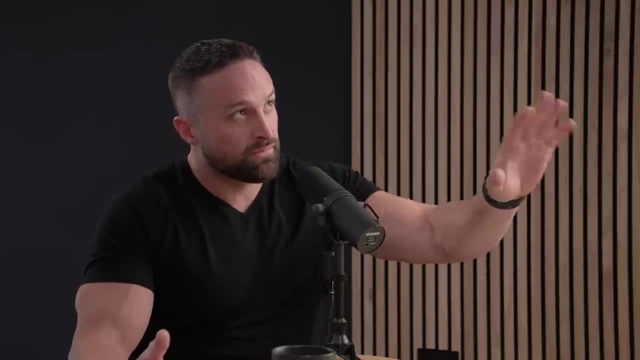 well, however long plasma leucine stays up, that will be how long uh protein synthesis stays up. And so we got the protein synthesis data back and it was peaked at 90 minutes, or sorry, peaked from 45 to 90 minutes, and then was back. 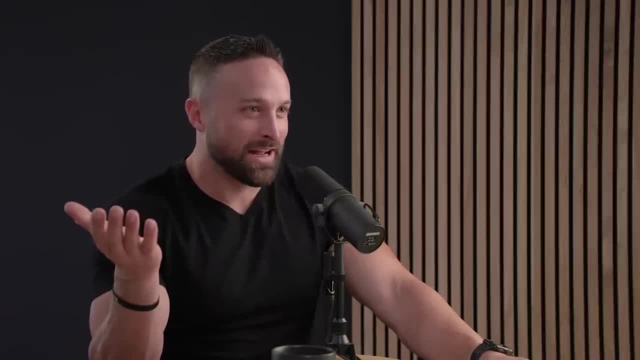 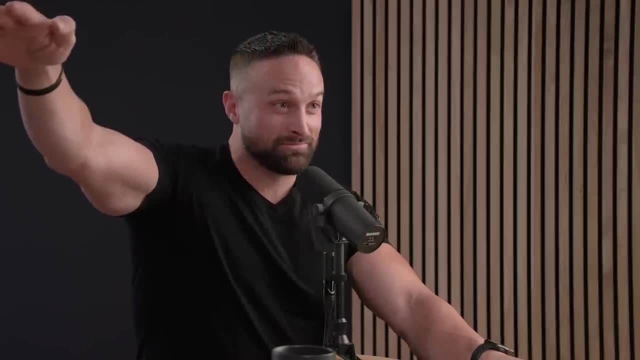 down to baseline by 180 minutes, And so when I went to do the plasma leucine analysis, my shock was, at three hours, plasma leucine was still plateaued out And I said, okay. well, when I look at the initiation factors, that will show. 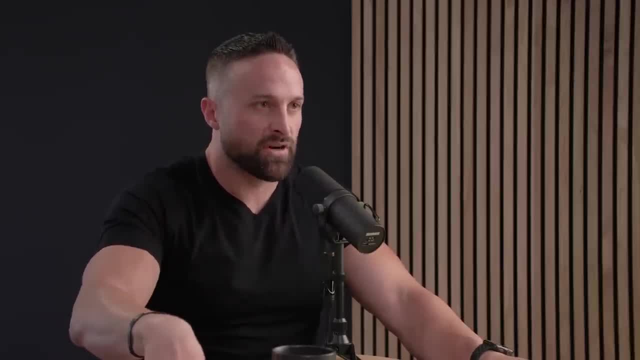 me something. So, um, for those not familiar, um, this is part of the mTOR signaling pathway, So one of the two of the targets of mTOR. when it's stimulated, leucine stimulates mTOR. two of the targets of mTOR are a protein compound called 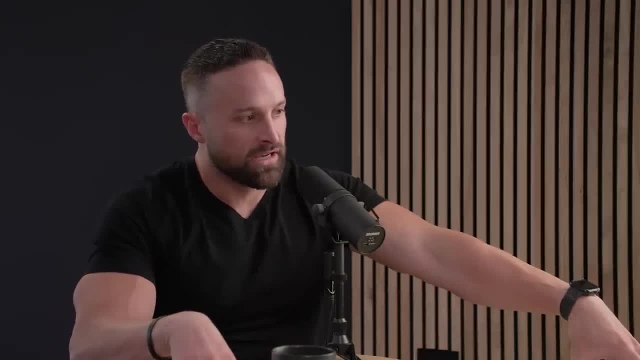 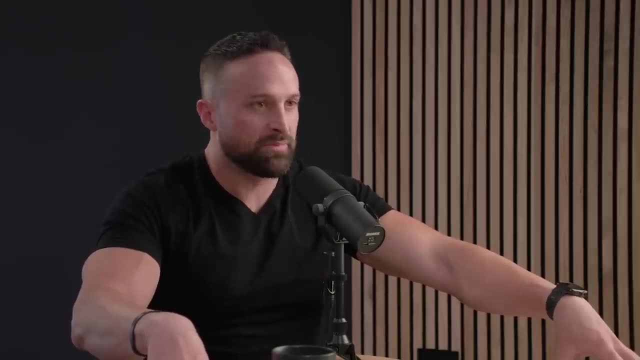 4-EBP1.. And then another one is called a ribosomal protein, S6K. So I don't want to get into the specifics about it because it's kind of beyond the scope, but basically when these things are phosphorylated by mTOR, 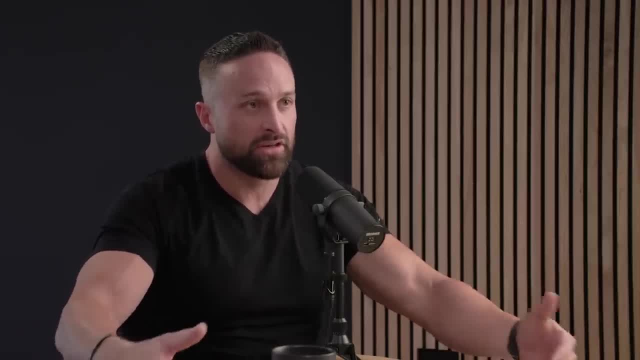 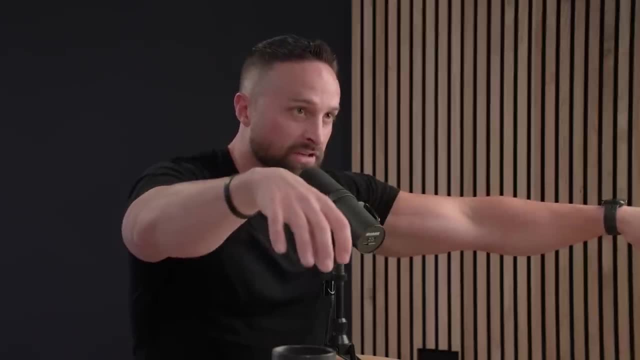 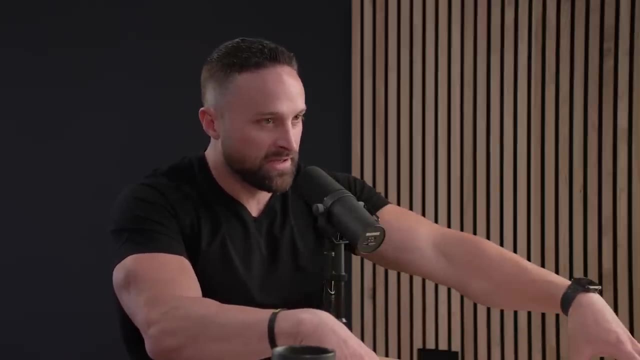 it increases the rate of translation initiation, which translation initiation is basically the process of the ribosome hooking onto the mRNA and then starting protein synthesis. So I was looking at the phosphorylation of 4-EBP1 and RPS6.. I was like 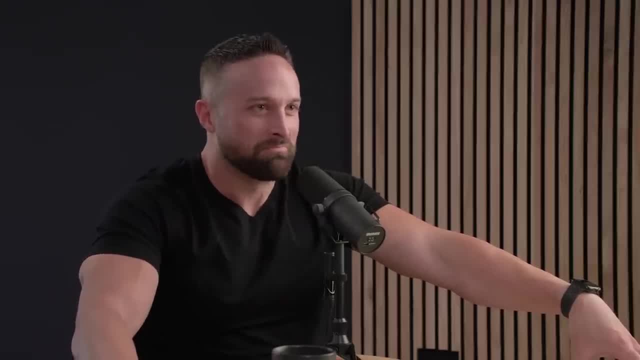 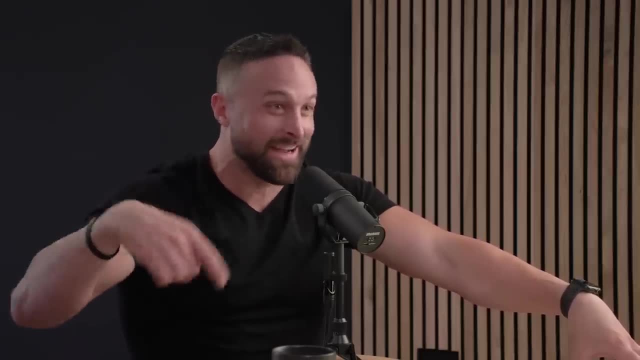 okay, well, I'll probably see these things come down at three hours still plateaued, And so then it was like: what is what's going on here? So I kept, actually kept, rerunning the data and rerunning the data, and rerunning the data. 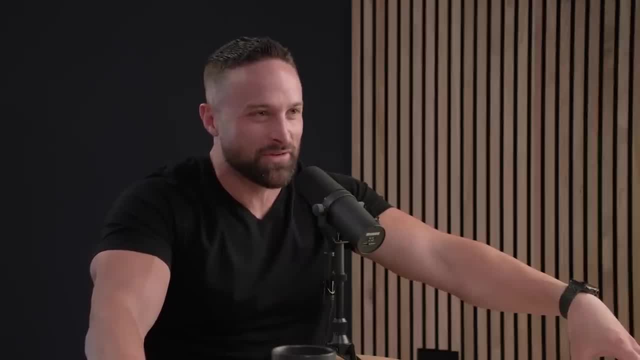 And I'll never forget. I went into the layman's office and this is, like you know, six months after we've done this study, because this analysis takes time, He's like. so where are we with this duration study? I said 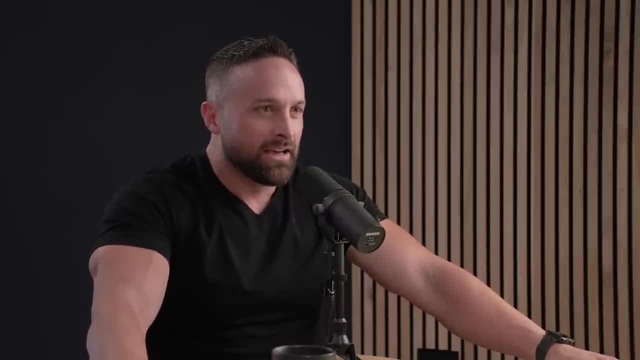 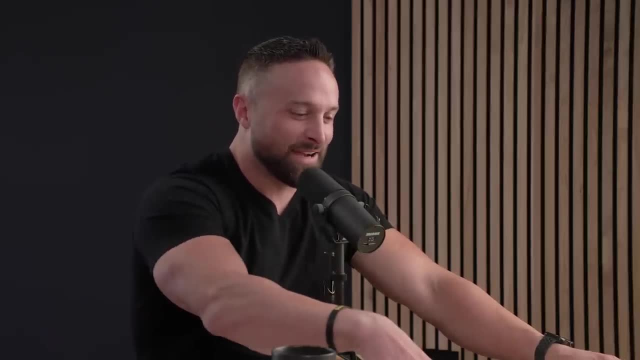 well, I just got to run the plasma data again because it's not right. And he's like, well, why is it not right? And I said, well, it just doesn't make any sense, you know, And I kind of went through. 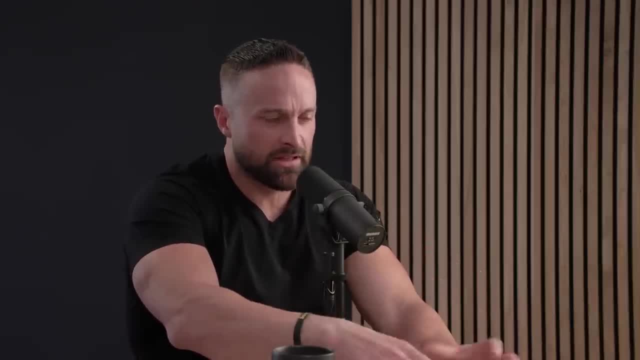 he's like: well, like, describe to me your technique, Like, how are you doing this? And I described it and he said: well, what, how's your standard error? And I told him what the numbers were, He said: 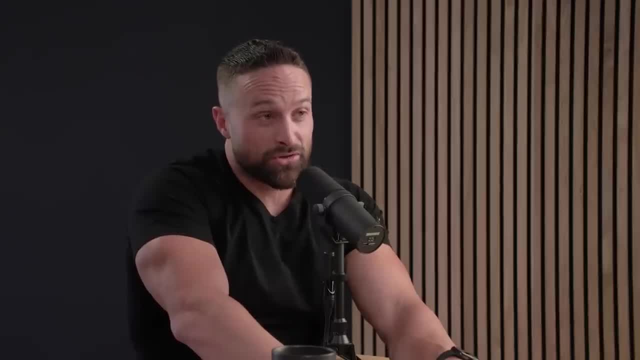 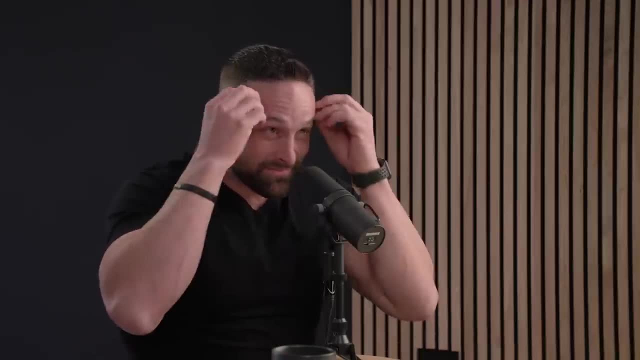 it sounds like it's good data. He said it sounds like you are trying to get the data to fit your conclusion And you need to change your conclusion to fit the data And that statement. this is why we do PhDs, Yeah. 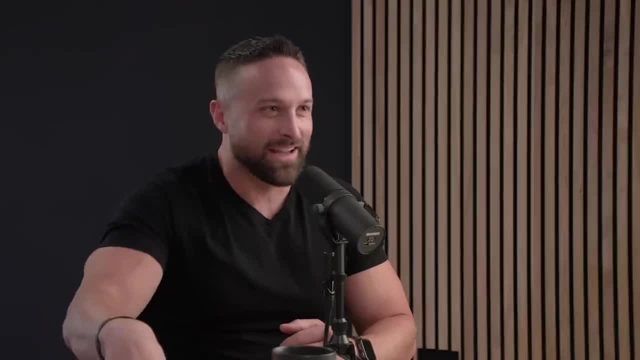 You need an advisor. This is why I'm so skeptical of everything, because I have had so many of my ideas crushed by my own data Right. So we actually ended up this, this, this kind of effect, this phenomenon, is called a muscle protein. 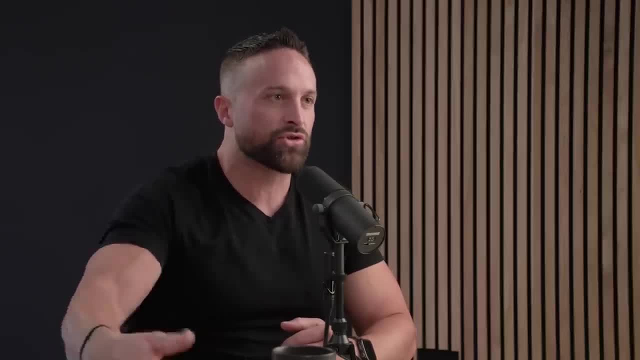 synthetic refractory period. So basically like once you trigger, the system kind of runs for for a defined period of time and then it takes time to essentially like reset, for lack of a better term. It's also been referred to as the muscle full effect. But so I looked at that and said, why am I eating every two hours? then you know, and there was even a study out of Wolf's lab, like back in 99, I think, where they infused amino, essential amino acids for six hours. protein synthesis went up, peaked at 60 minutes, came back down at 120 and never went back up again. Maybe I'm being naive, but I would have thought, thought that if protein synthesis goes up and then comes back down, that eating more often would be exactly the thing you would. 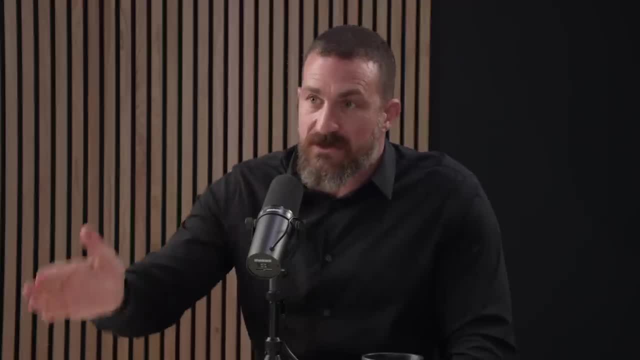 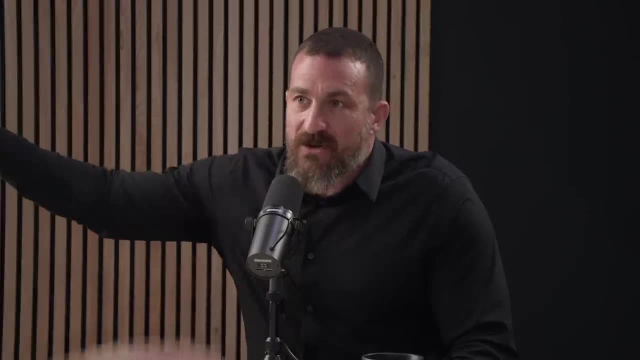 want to do if your goal was to get increased protein synthesis, because you'd be pinging the system periodically. But the but, the problem is the plasma amino acids are still elevated, So it's essentially like eating the whole way through from the perspective of Lucy, from the cells. 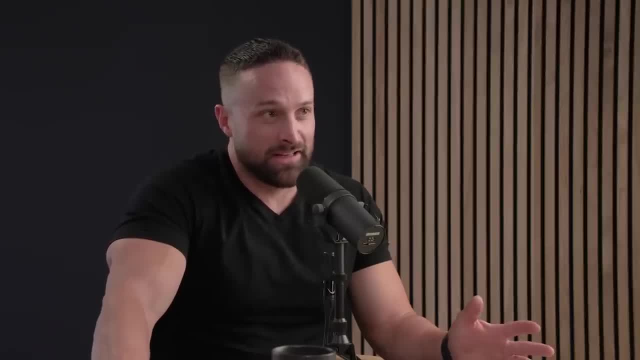 Yeah, So that was one of those things where I said: you know what I'm actually going to eat less often because, like, if I'm eating in three hours later, I've still got, you know, capped out plasma amino acids. 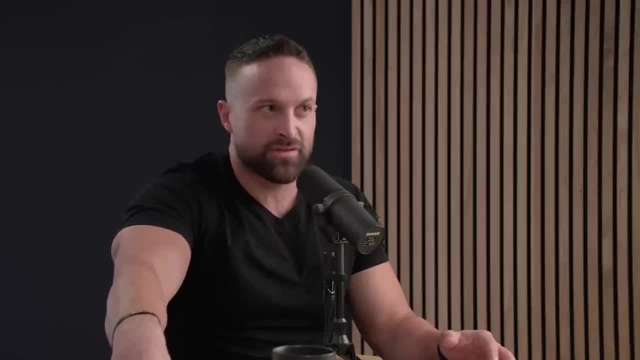 you know, and we looked at all kinds of stuff, Like we looked at intracellular Lucene, just to make sure that you know that wasn't falling off, It wasn't. we looked at all the plasma essential amino acids because we were 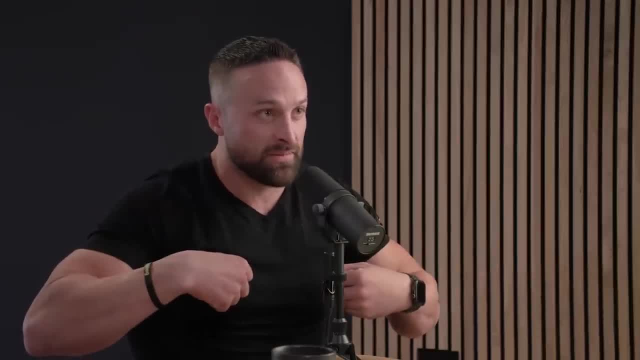 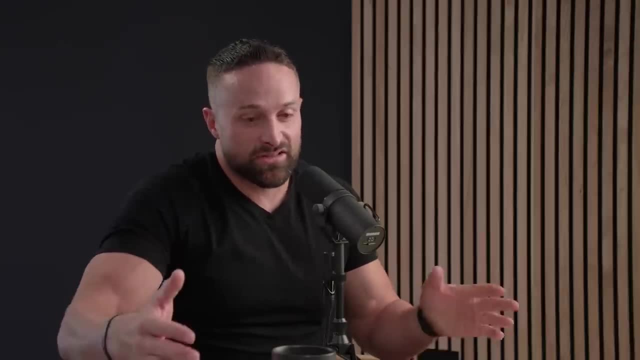 thinking: well, maybe protein synthesis is, you know, sucking some of these amino acids out of the plasma and they're dropping and that's causing it to kind of short circuit the system. That wasn't the case, It just essentially what the evidence suggests. 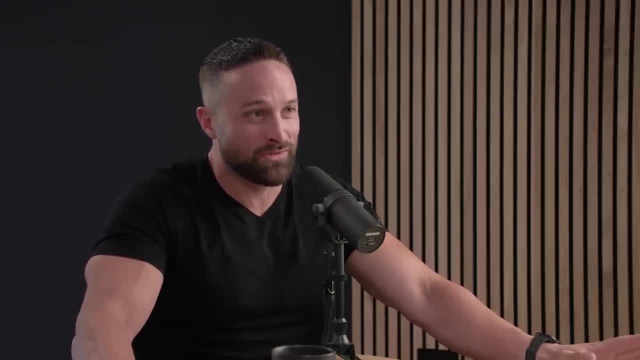 I think we're the only ones to show this so far. So I'm not ready to say that This is a real effect, because I hold out the idea that data artifacts do exist and you can't be totally sure. but we saw an increase in AMP, kinase kind of around. 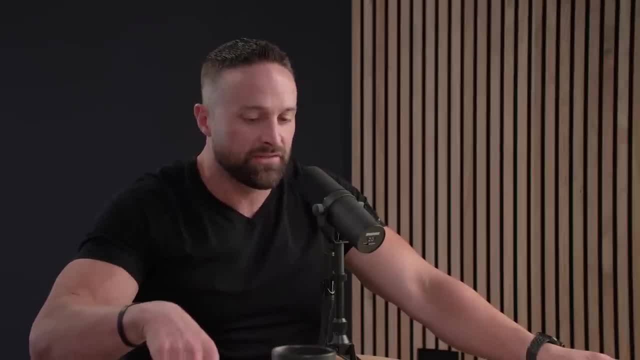 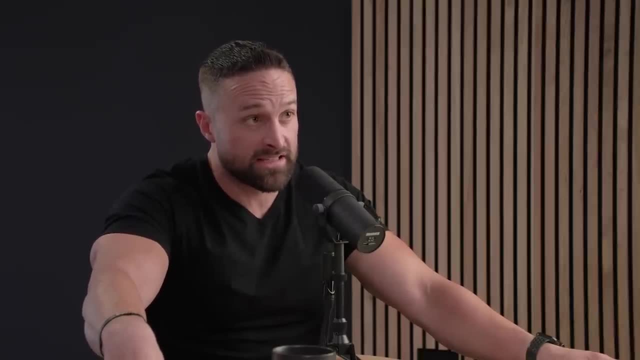 this mark where a protein synthesis started falling off And we also saw a decrease in intracellular ATP, and protein synthesis is an ATP dependent process, And so what we think might be happening is: you're, you know, consuming. you're consuming muscle protein and you're up for your increasing muscle. 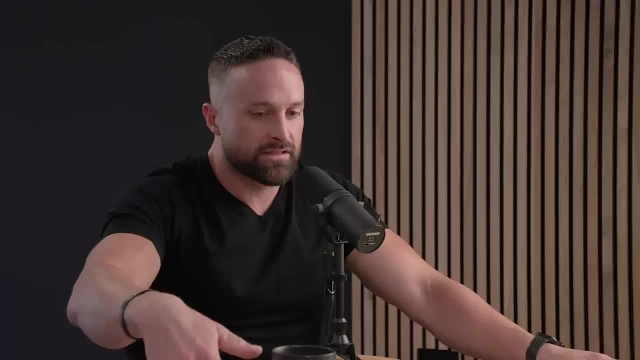 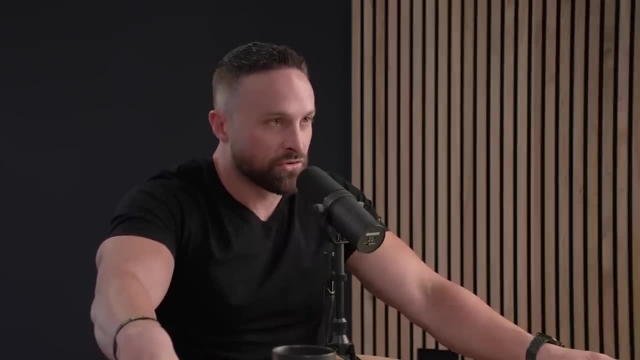 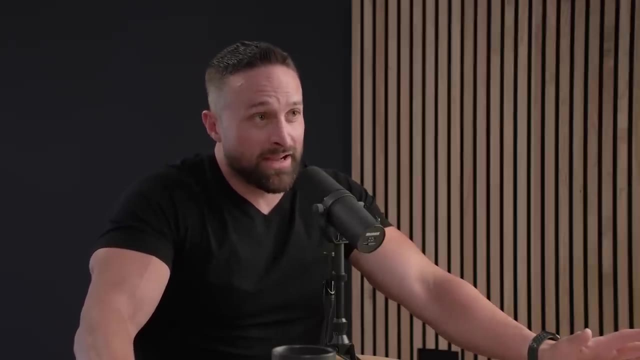 protein synthesis And then at a certain point it's has enough effect on your- you know- energy metabolism in your cells that it kind of short- not short circuits it, but it kind of cuts it off Right. So again, we're the only ones to show that. 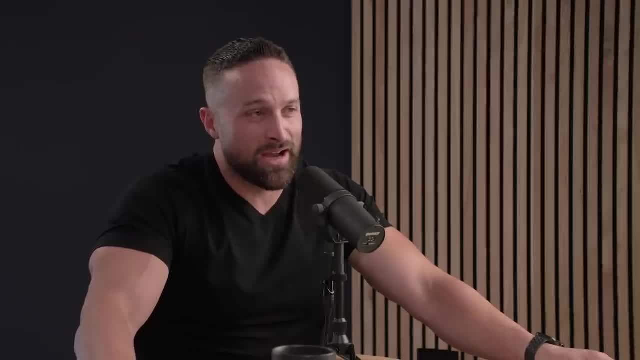 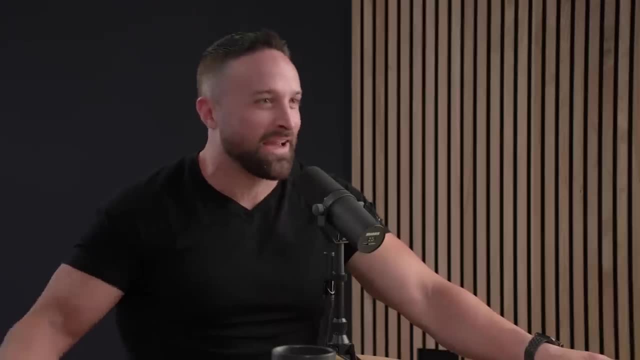 that I'm aware of. So, and that was again in rats, So I, I I always talk about data like there's data. I'm willing to bet my my toe on my foot on my leg on and my life on. 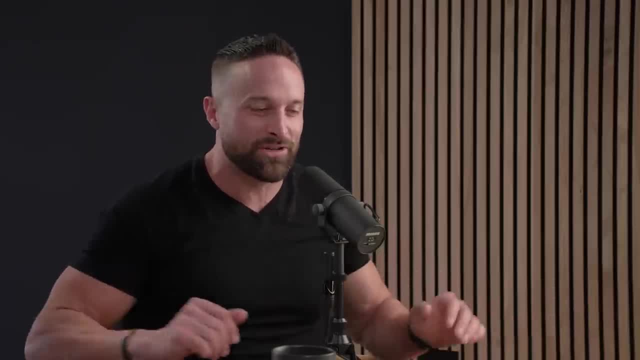 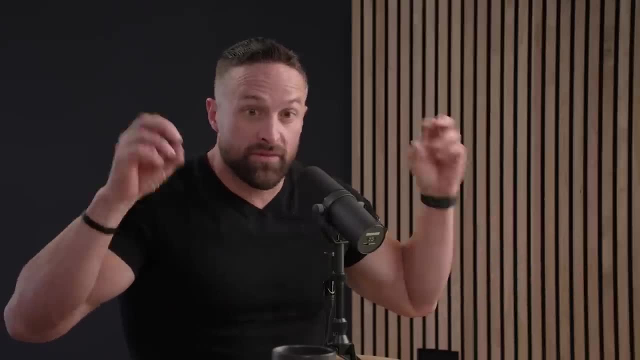 I'd probably barely bet the end of my little toe on that one. I'm not quite sure, but it's interesting nonetheless. So that's a that's a great example of, okay, we're looking at this mechanism of mTOR signaling. 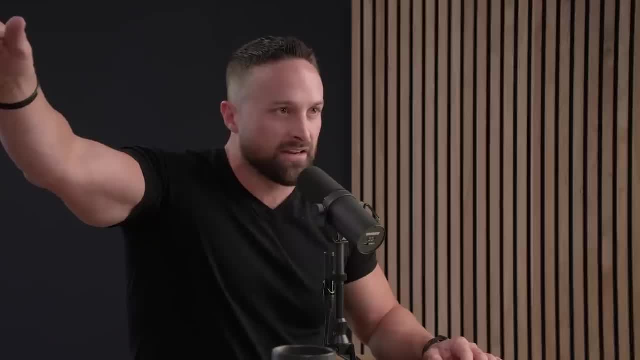 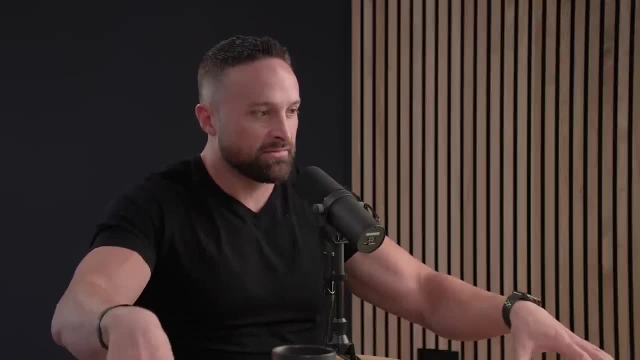 And if we just looked at that, we'd say, oh well, protein synthesis is going to stay elevated, for you know past three hours, but that's not what we saw. So yeah, I think it's again. that's why I really try to. 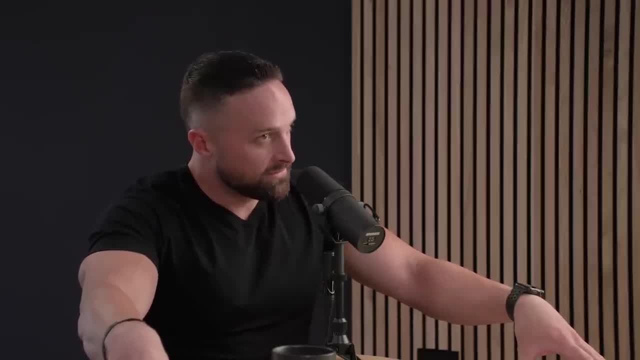 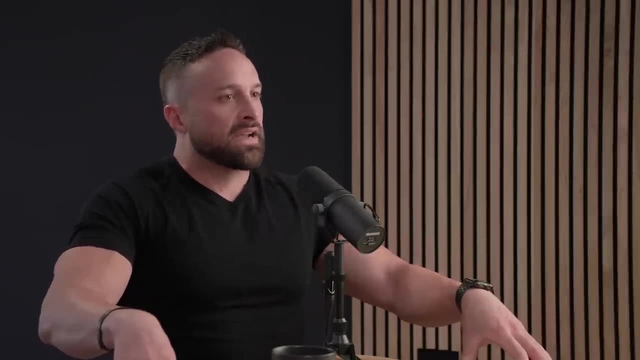 you know, get people to say: well, let's mechanisms are important. It's especially if you're seeing an outcome. it's important to identify mechanisms that may explain that. but let's step back from the mechanisms, from trying to chase mechanisms. 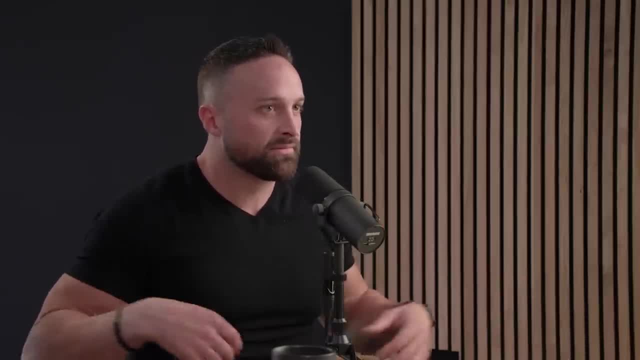 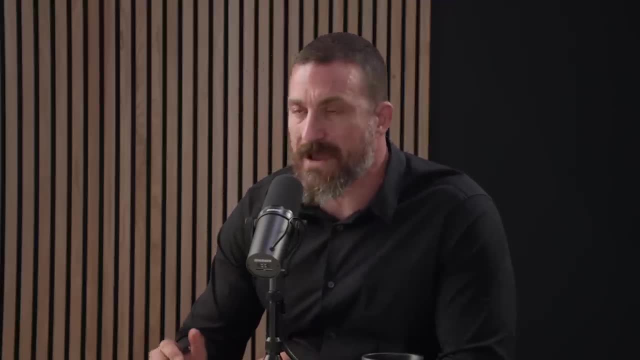 And let's look at like chasing outcomes in terms of what we recommend to people. Excellent point in terms of chasing outcomes. a number of people I know are interested in weight loss or weight maintenance And several times throughout today's conversation we've come back to this issue of satiety signals. 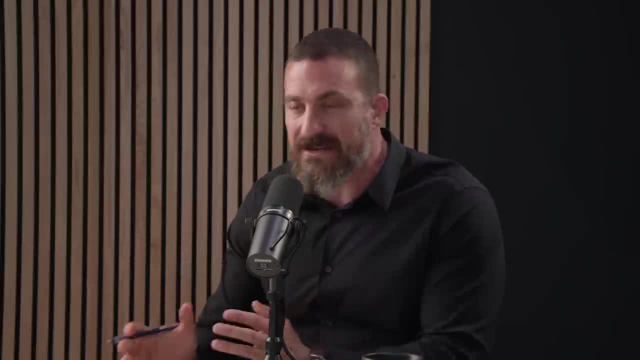 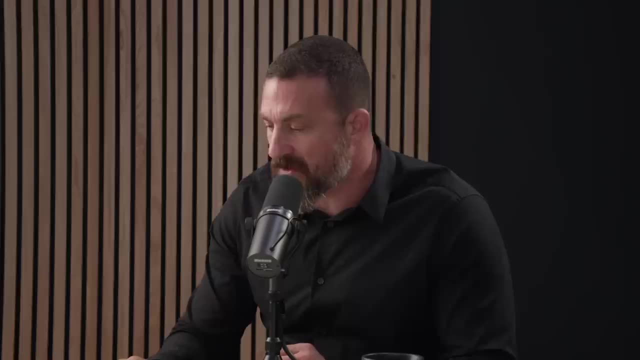 whether or not they're brain-based, body-based or both. you know, not wanting to, not wanting to eat more, is a great way to maintain or lose weight, because you simply don't want to. I heard you mentioned earlier that protein and maybe specific types. 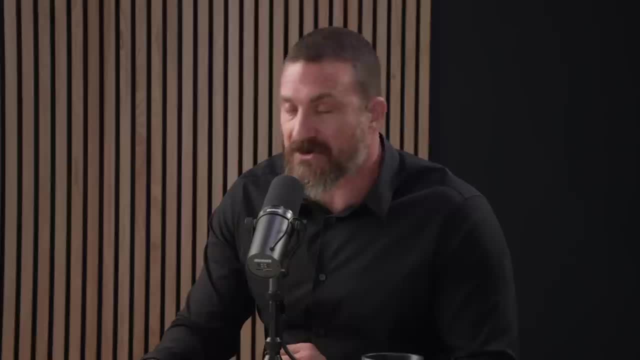 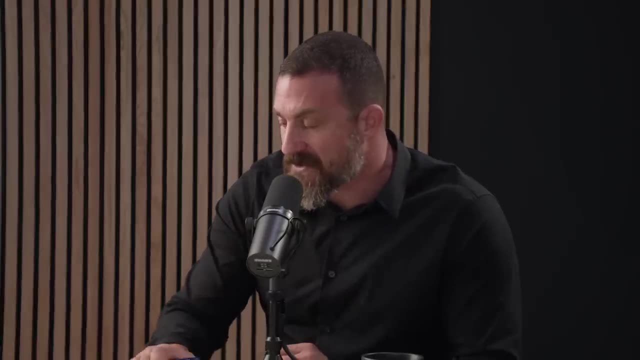 of protein or sources of protein may provide better satiety signals than other macronutrients. Could you briefly talk about how macronutrients, including protein, but also carbohydrates and fats, impact satiety, And from the standpoint of somebody who 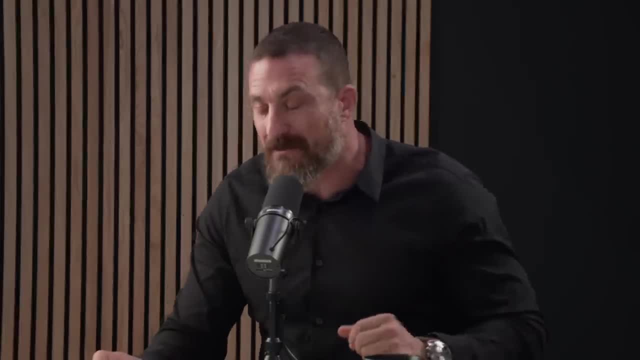 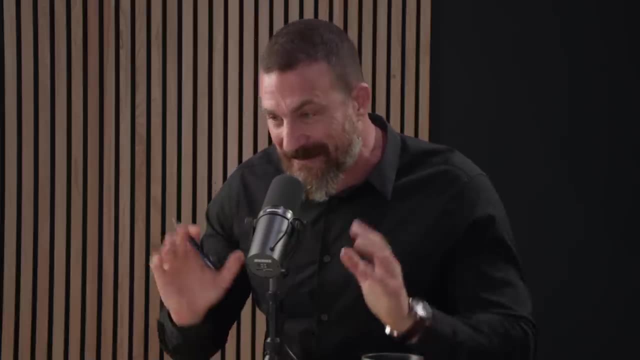 for instance, would like to quote unquote: lose a few pounds, right. Probably would be happy to gain a little bit of lean body mass, provided it was in a particular location on their body. That seems to be a thing now directed hypertrophy. 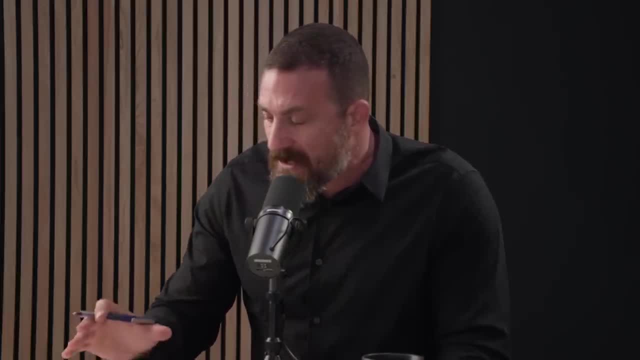 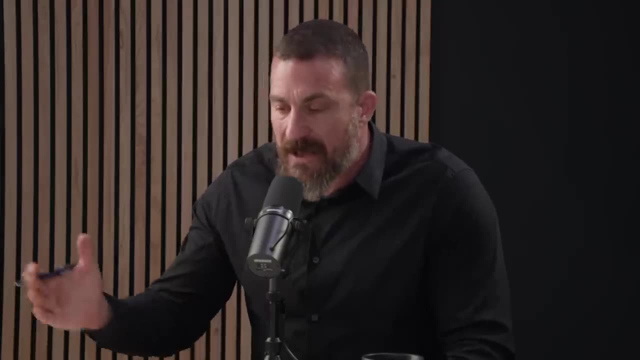 if you will, and how much they should focus on protein as a core component of creating this diet. you know, assuming everything else has been done correctly, they're going to hit the right number of calories relative to their, their output neat. 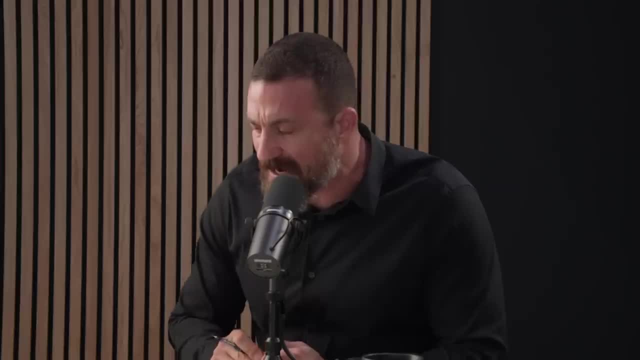 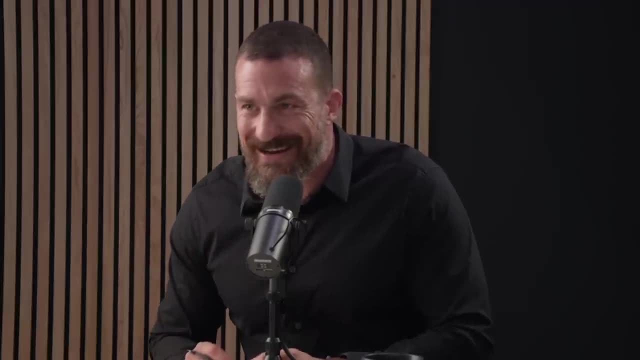 et cetera. How should we think about protein And satiety signals and our animal sources of protein, indeed more bioavailable? That's a tricky word for sake of muscle building, but also for sake of somebody who just would like to lose. 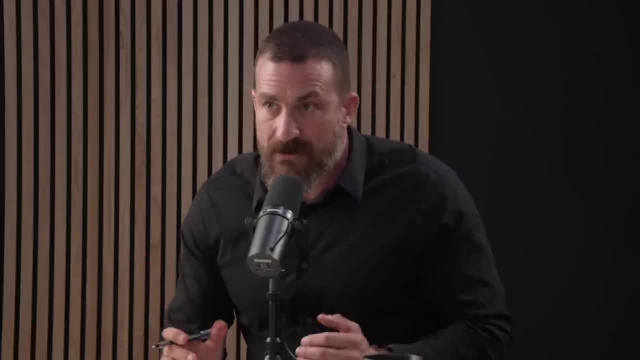 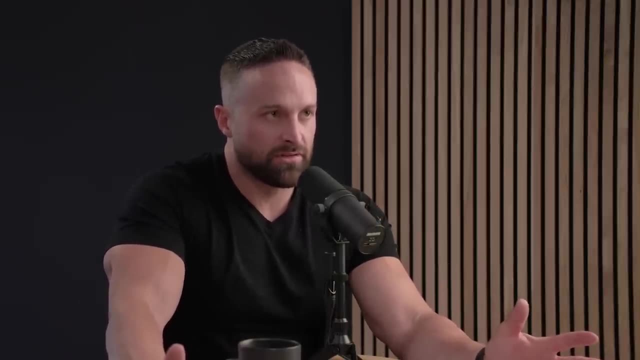 body fat, They don't want to lose muscle and they'd like to bring their weight down a few pounds. So a lot of things are more, Yeah, A lot of things to unpack there. of the macronutrients, Protein is definitely the biggest lever that you can pull, because even 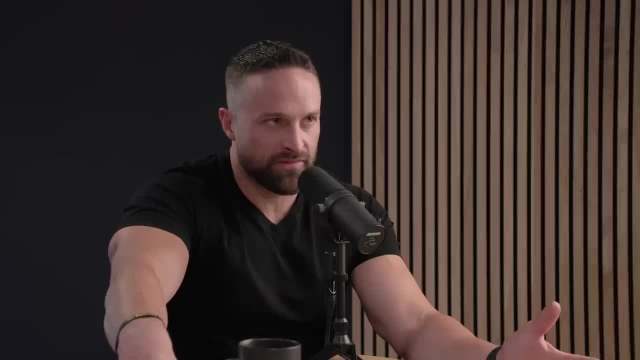 if you know it doesn't take a ton of protein to get a lot of the muscle building benefits. I mean, I think the benefits really, they start to plateau out around 1.6 grams per kilogram of body weight. There's some evidence that maybe even up to like 2.4 or 2.8 grams per kilo may give like a little bit more benefit. I think it probably looks something like an asymptote in terms of a curve where as you put more into the system you always get a little bit more, but it just gets to the point where it's so infinitesimally small. 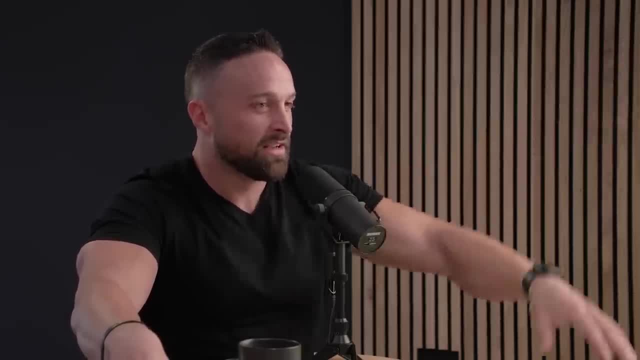 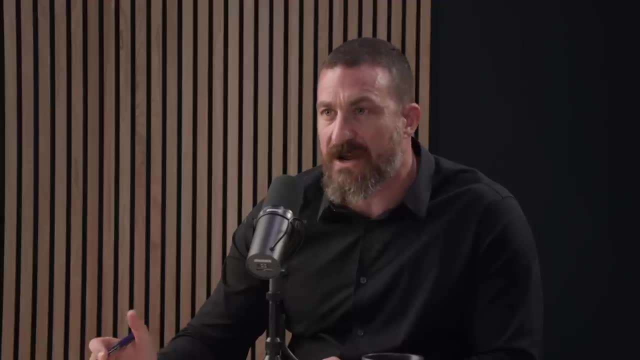 benefit that it's for all intensive purposes, no benefit. But you mentioned 1.6 grams of protein per kilogram of body weight. Is that? would you consider that a threshold that most people should try and achieve daily? I think I see very few downsides to hitting that. 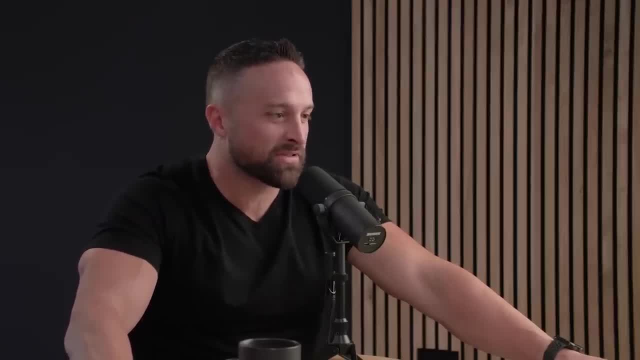 I mean, I know some people- and this is going to get into a separate conversation- but I know some people will say: well, I don't want to stimulate mTOR because that's going to make me die early. And I think one of the things to keep in mind is: 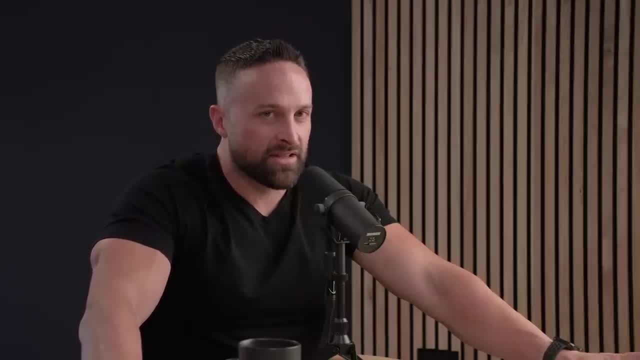 if you look at, there's kind of this thought process out there that if you're stimulating mTOR, that protein is going to make you die early. And, first off, we have very little human outcome data to support that claim. And the second thing is, if you look at any macronutrient isolation, 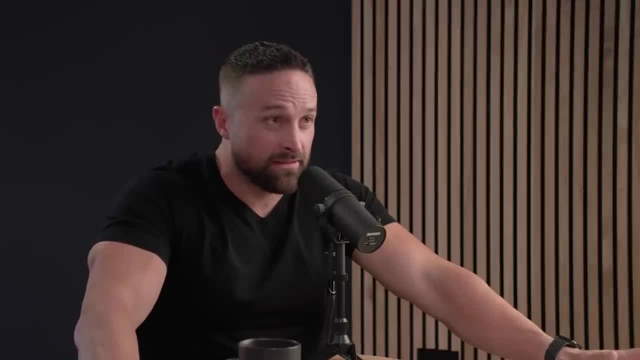 I can make a mechanistic argument that it's going to kill you, So fat if you take in fat, and it decreases flow mediated dilation. flow mediated dilation is important for heart health in the short term. Carbohydrates stimulate insulin- insulin. 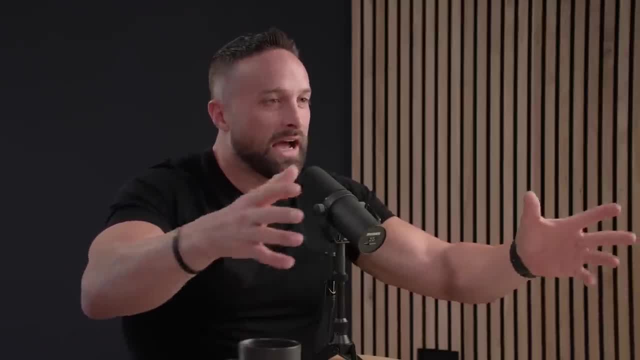 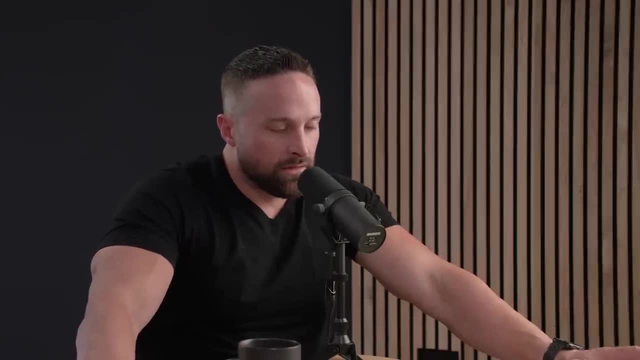 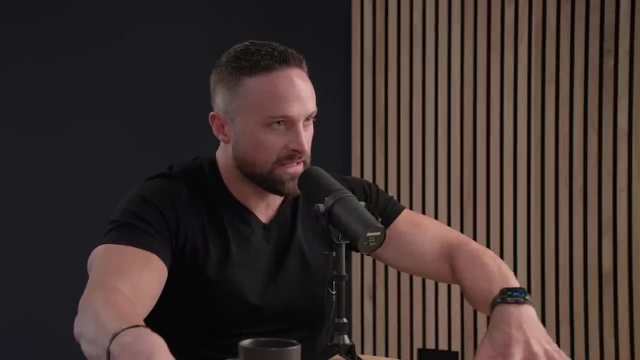 you know pro-inflammatory and you know all these other things, And so I can make an argument for any single macronutrient to be negative for longevity. I really want people. this is something that even scientists get wrong. They look at an acute response of something and assume that that. 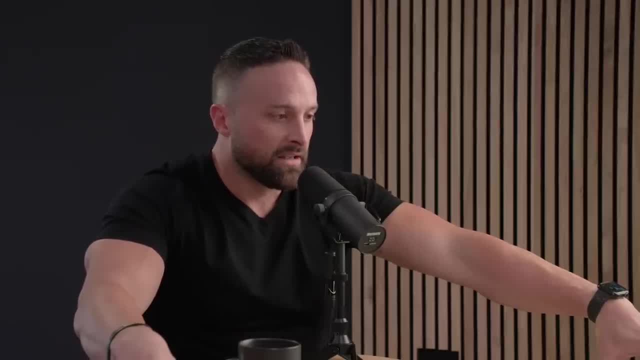 is going to relate to long-term outcomes and signaling. So let's just take exercise, For example. if I, if you didn't know anything about exercise and I said to you, Andrew, I'm going to do something that's going to make you. 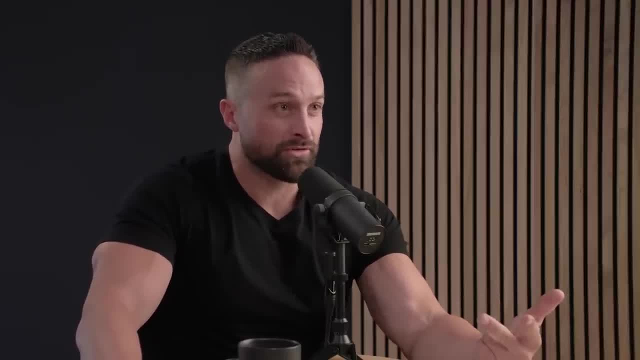 your heart rate go up, your blood pressure go up, your inflammatory markers go up, your reactive oxygen species increase. You're going to say, Andrew, and it's going to damage your muscles. You're going to say: I'm not doing that. 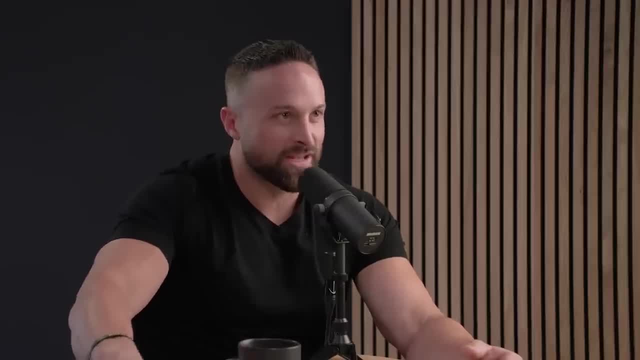 That sounds horrible, you know, but it does all those things in the short term. But what is the long-term effect of exercise? You actually get healthier. All those things improve. Now, I'm not saying that, you know, protein is a longevity hack or anything like that. 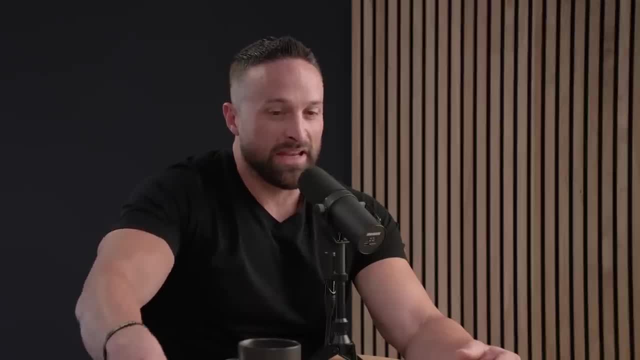 But what I'm saying is, I think some of the arguments out there based on mechanistic. you know, this increases mTOR. therefore we don't want to do it. I think it is a much more complicated argument, Then, than just that. 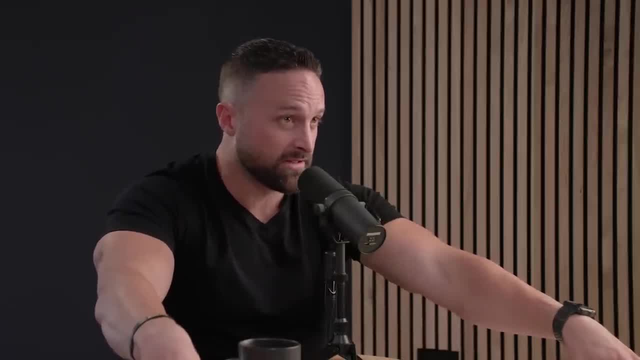 So there's that. So protein is the biggest lever. I would shoot for 1.6,, you know, grams per kilogram. If you can do more great, there doesn't seem to be really downsides to it, Even like up to very high levels of protein. A Jose Antonio did a study that was a year long randomized control trial, And again it's just one year, but they were looking at all sorts of different biomarkers And basically even up to like four grams per kilogram of protein. 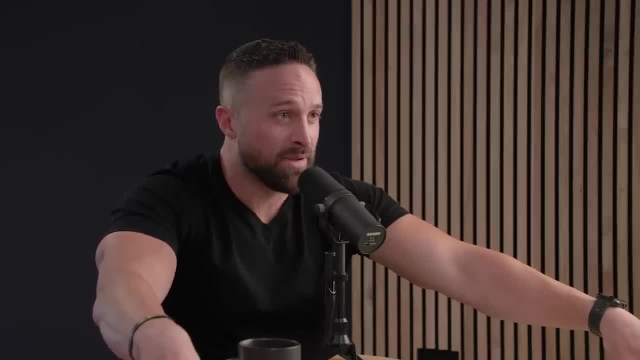 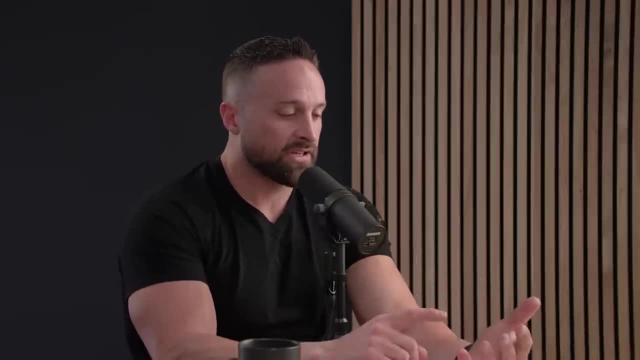 they couldn't really find any negative health outcomes from it, Other than people were just so satiated they ended up eating less calories. So protein is a big lever. lever because one it has a higher thermic effect of food, So you're getting a little bit more calorie burn per day. 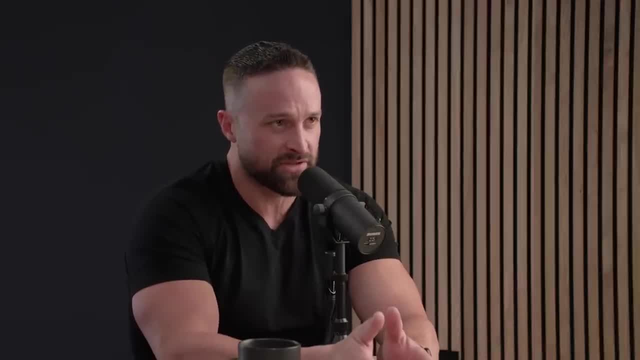 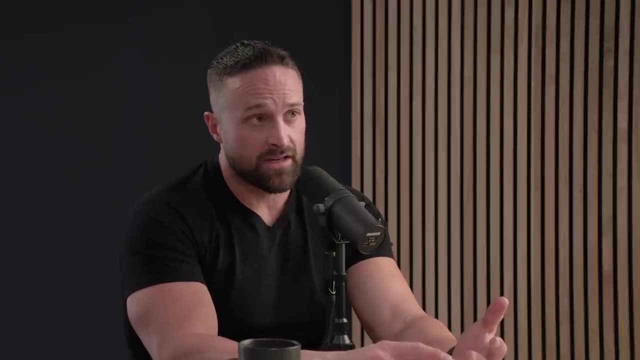 even though it's not a ton, because TEF is a pretty small percentage of your overall energy expenditure, but still a benefit. You're getting the effects on lean body mass It's going to. if you're in a diet, it's going to help preserve lean body mass. 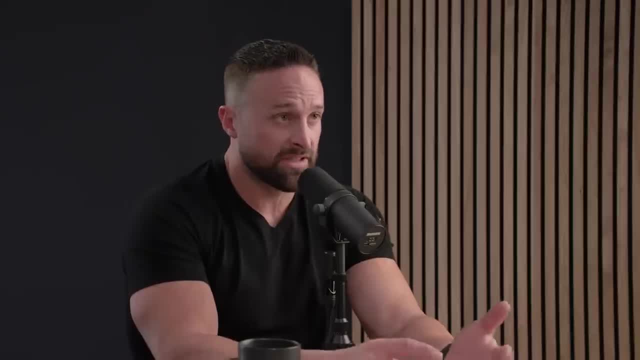 If you're at maintenance, it's going to help build a preserve lean body mass, And if you're in a surplus, it's going to help build a preserve lean body mass. So, and then you get the effects on appetite. So now I want to be careful, because appetite effects tend to 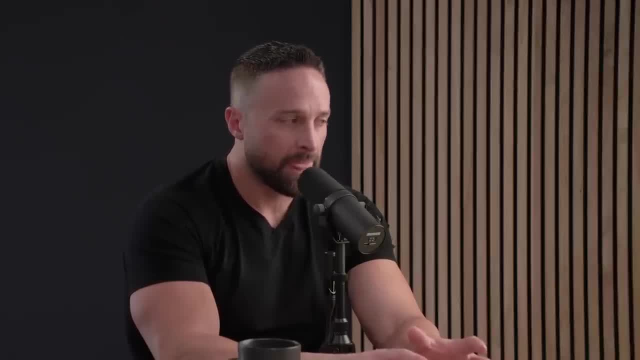 be very specific to individual foods, right, So you can take a high protein food and make it not very, not very, satiating. So take, for example, like a really tasty protein bar which you know back when we were getting into this. 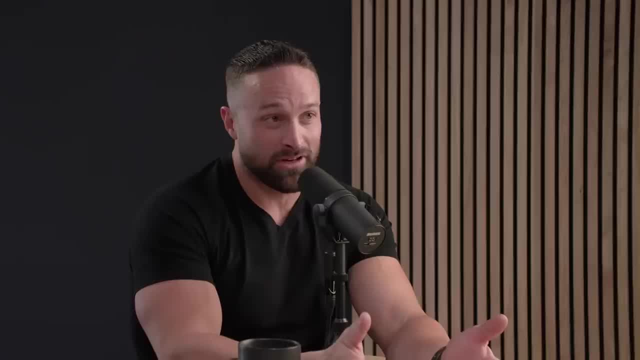 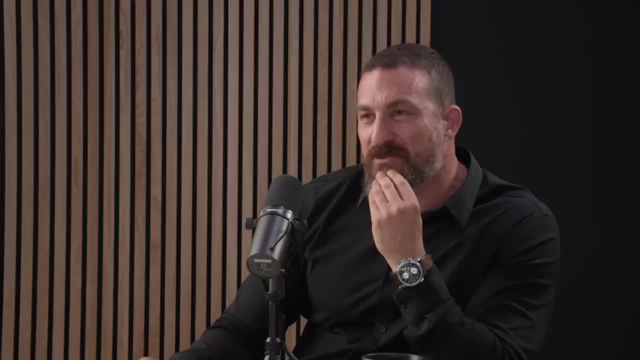 there, no such thing existed. Now you have protein bars. actually take pretty darn good, but if you eat one of them, I mean, are you really satiated? I don't really feel satiated. That's my protein bar. That's my pre meal snack. 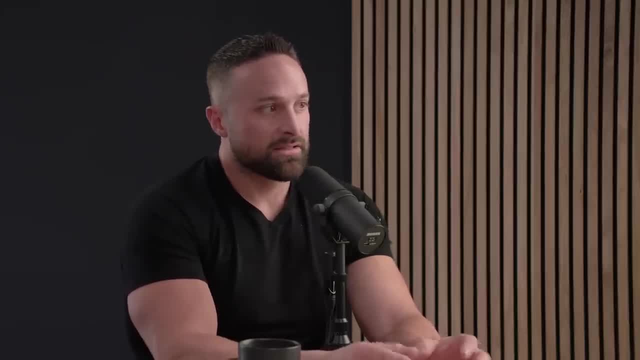 Right, right. So why? Because I mean it's processed, refined and made to be very palatable, Okay, But take something like a 200 gram chicken breast. very satiating, right. And that's why, when people say 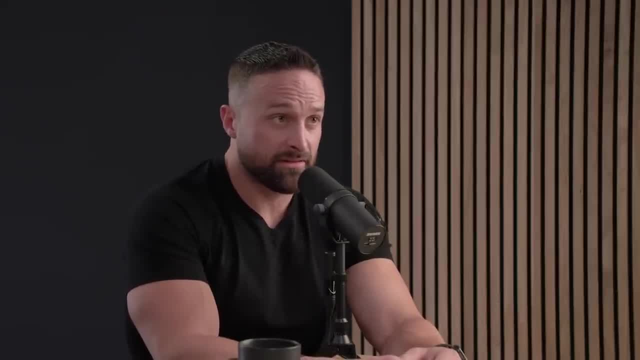 well, carbohydrates aren't very satiating. depends on the carbohydrate I mean. when you look at the like the satiety index, a plain baked potato is about as satiating as it gets If I eat a bowl of oatmeal. 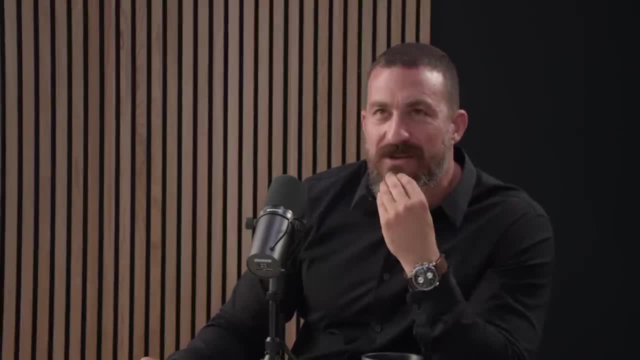 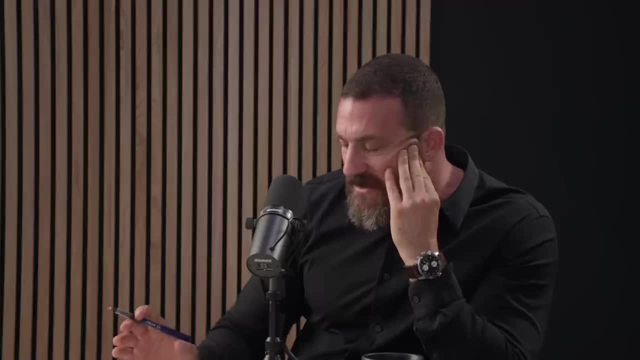 I feel pretty good afterward for a while, Right, I mean, I usually I'll eat that along with some other things. but I completely agree The. so you're saying that the form that it comes in, maybe even how much chewing is required? 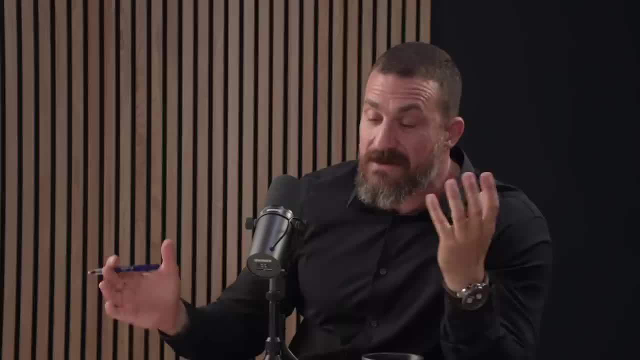 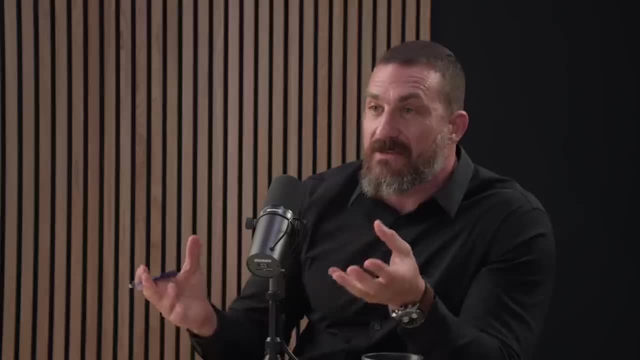 how good it smells that your psychological associations, because to me a steak is an incredible meal, Like I mean, if I had to pick one food that I could eat- even though I'm not pure carnivore- for the rest of my life. 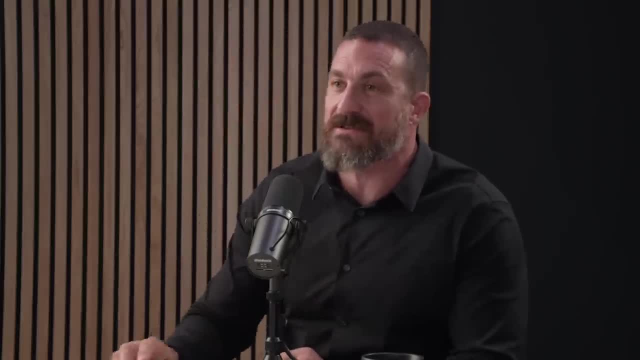 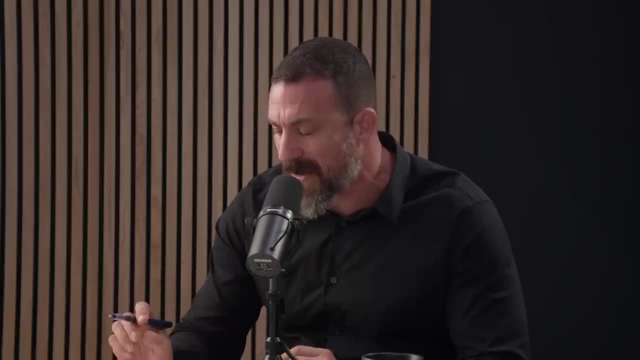 it would be that, because I think it would get me where I need to go, And then I'd probably have to sneak some fiber, you know. but it's an excellent point. I have a question that I don't want to take us off track. 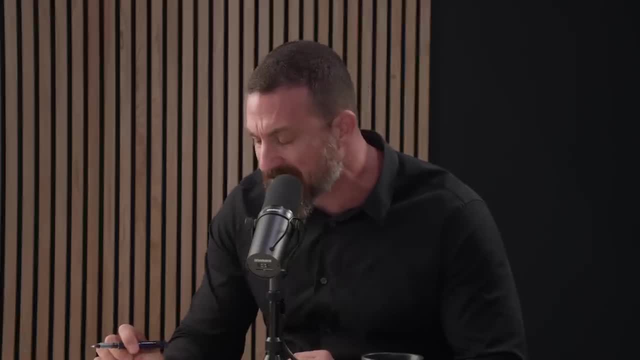 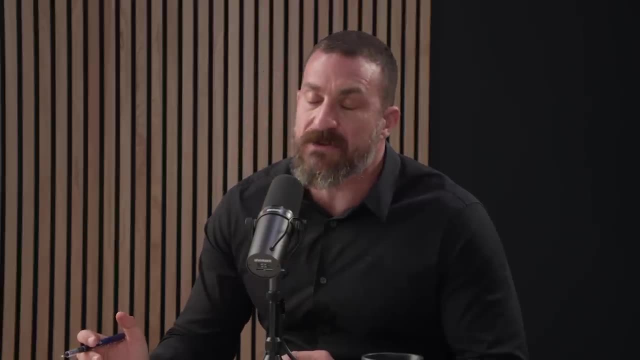 but I'm hoping it relates enough that you could answer it Now in the context of this. if I'm going to eat, let's say, two grams per kilogram of body weight protein and I'm not eating multiple meals, but maybe I'm eating two or three meals per day, 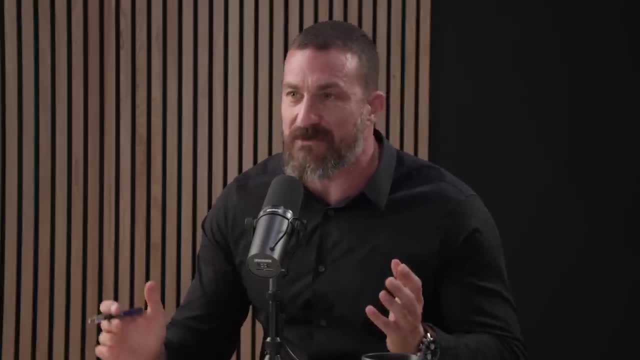 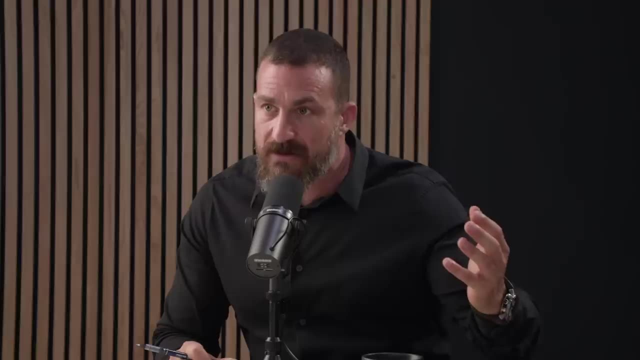 I'm certainly going to be eating more- more than the 30 gram threshold that was thrown around for a long time, that we can only assimilate 30 grams of protein per meal. Should I just not worry about that? Some of it is going to go towards the thermic effect of. food. Some of that might be converted into glucose, of all things, through gluconeogenesis. So should I worry about this 30 gram cutoff? Because I think balancing the 1.6 gram per kilogram body weight threshold with number of meals, with the need to exercise and work and live my life and sleep, et cetera. pretty soon you run into bottlenecks where you just can't do it all Or you're spending so much time trying to focus on it. You can't optimize all the things at the same time. You'd lose your mind and your body. 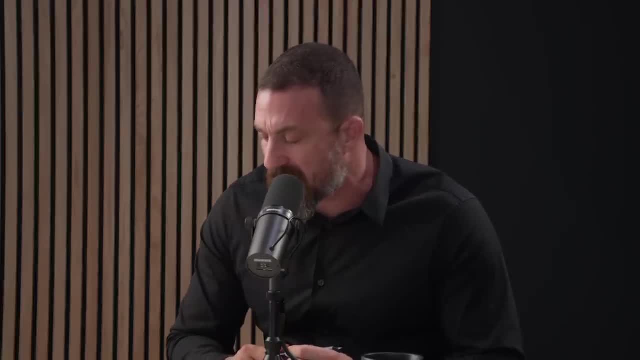 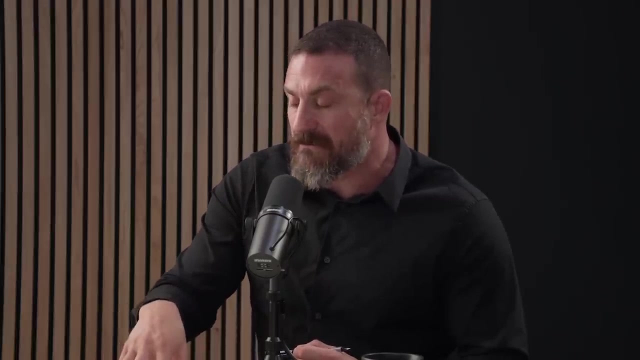 So what is necessary in terms of frequency if one is getting enough protein? And then, tied into that question, is there any reality to this idea that if you eat one meal per day or you're fasting and then you eat, you know, let's say, 200 grams of protein in a single feeding, that you can assimilate more because you were protein starved. Is that, is that a real thing? So most of the studies with protein are after a fast like, because to assess it with stable isotope you have to be in a steady state. So we haven't observed that. it doesn't appear that fasting really kind of allows you to assimilate more protein after a fast. So this gets into a core of one of the things I looked at my PhD, which is: does protein distribution matter? Because most Americans get about 65 to 70% of their protein? 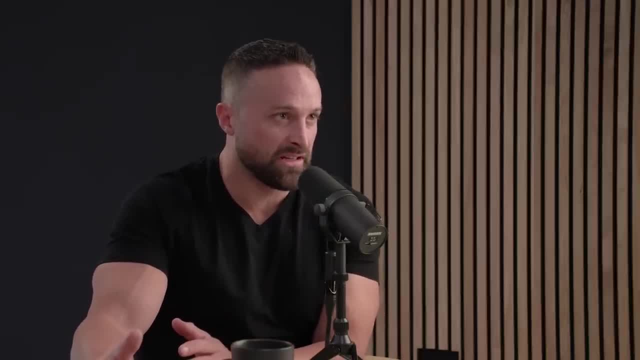 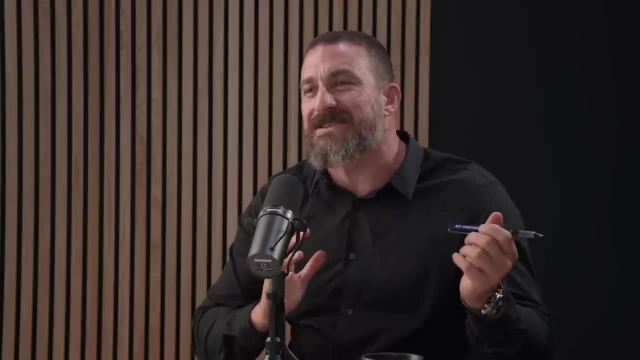 at dinner right? Breakfast tends to be pretty minimal protein foods. Do any cultures actually a big breakfast and not a big lunch and dinner? I get you know we all heard that that was ideal. We'll get into circadian timing and a little bit. 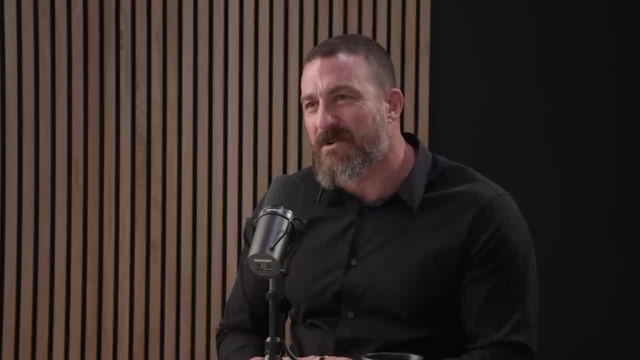 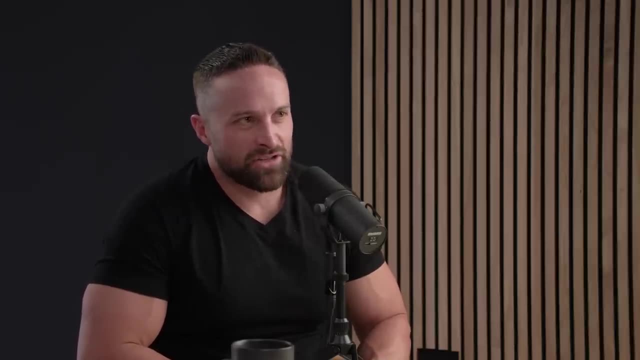 but does anyone actually do that Steak and eggs for breakfast and then taper off the rest of the day? I know German culture tends to have a big breakfast, but it also tends to be like sugary foods and whatnot, As far as like teleologically. 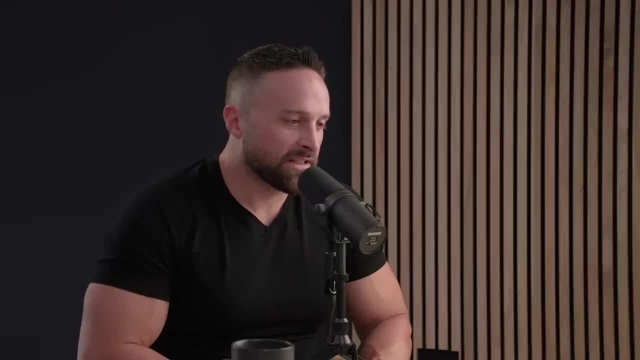 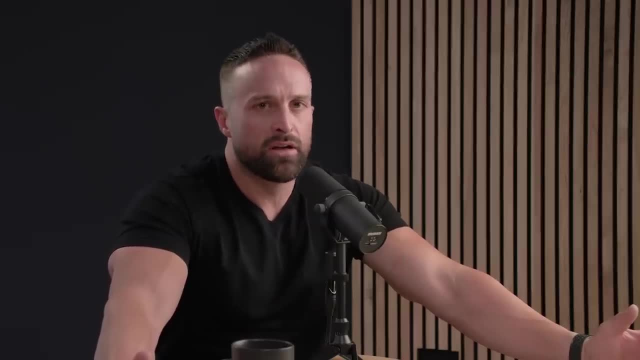 I'm not. I'm actually not sure about that. So if you look at that and then you consider that protein doesn't really have a storage mechanism, right, Like people will say- well, you know, lean tissue is a storage mechanism. 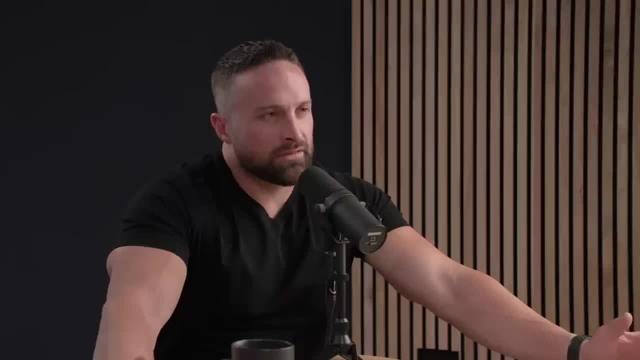 That's like saying a house is a storage facility for wood. You know, Yeah, If you're, the house has been out of wood. you could get wood out of it, but that's not why you build the house right, Like you're building the house out of a demand. 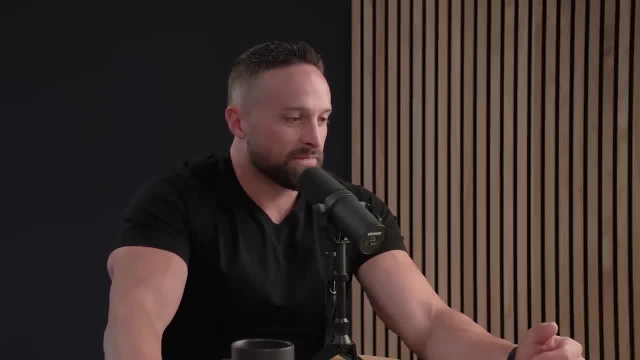 Same thing for muscle tissue. There is a free pool of amino acids, but it's very, very small. So when you think about that, you know you consider things like fat, which basically has unlimited storage capacity. carbohydrate, a relatively large storage capacity. 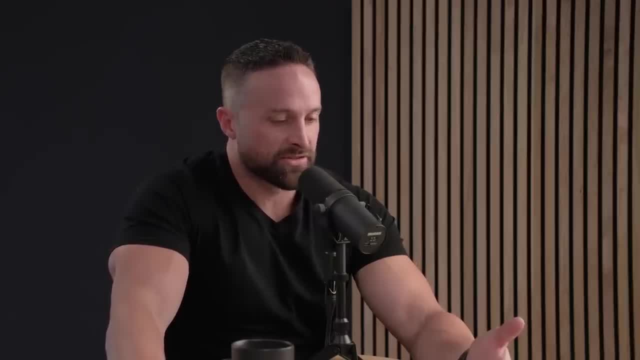 You can store, you know, four or 500 grams of carbohydrate between your liver and muscles, and then protein which almost has no storage capacity. The idea that, okay, you could make up for a low protein at one meal by over-consuming another meal. 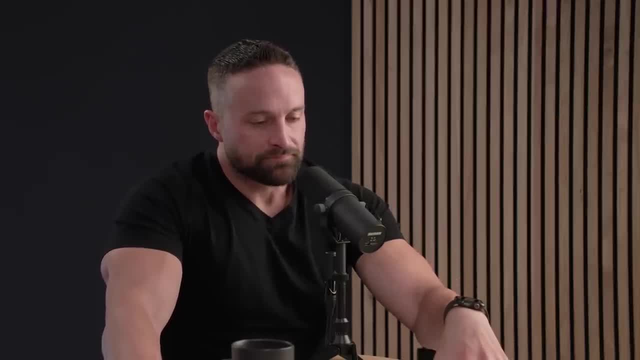 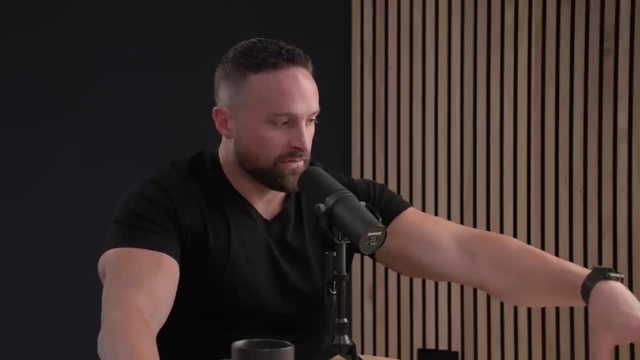 Didn't make sense to me. So one of the studies we did and again in rats we took, both groups were getting whey protein, So high quality protein. they were getting the exact same amount of calories, exact same amount of. 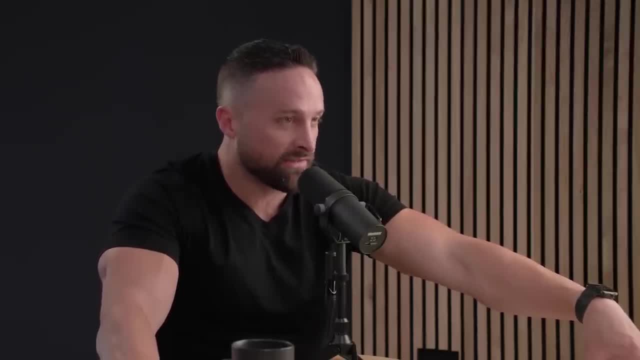 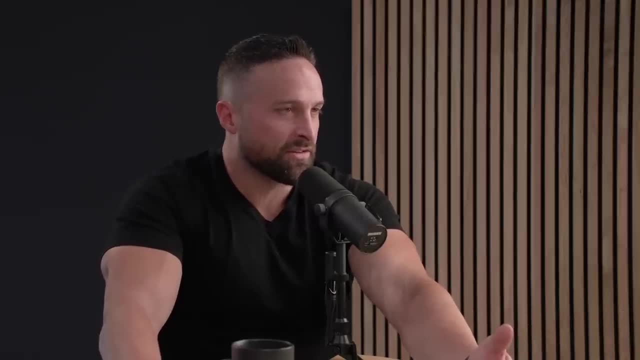 you know, nitrogen- exact same macros. Everything was the same. The only difference was one group basically got kind of three meals of similar amounts of protein. Like dinner was a little bit bigger because we wanted to keep it somewhat similar to how people eat. but each meal was going to be over the threshold to stimulate muscle protein synthesis, Whereas the other group- I- constructed it. So the first two meals of the day should not stimulate muscle protein synthesis, It should be under that threshold. And then the last meal was about 70% of their total daily. protein, And so we had them eat those for 11 weeks and I'll never forget this. This is how like obsessive I became about it is. there was 110 animals in the study and I made all the diets and I weighed out exactly every single meal for every single animal. 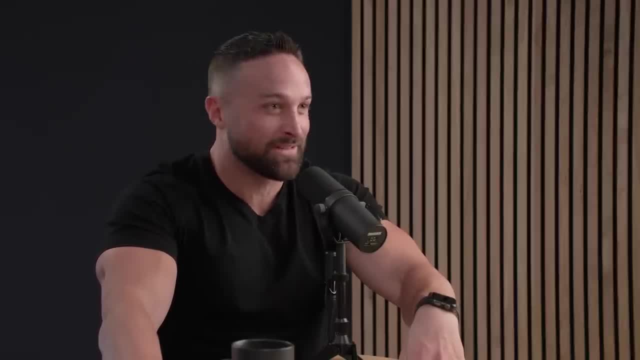 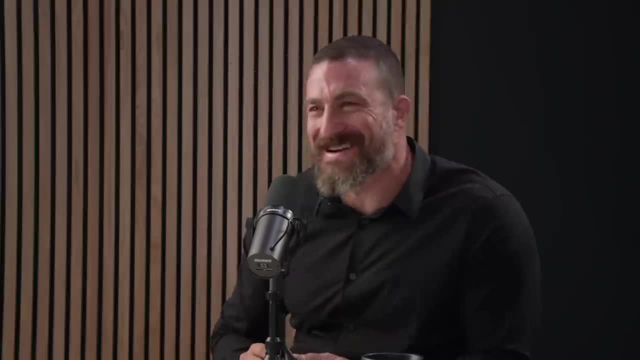 for 11 weeks. So I was in there at 6: 00 AM, I was in there at noon and now I was in there at 6: 00 PM. You know I love it. So kind of PhD student that professors dream of you guys in a. 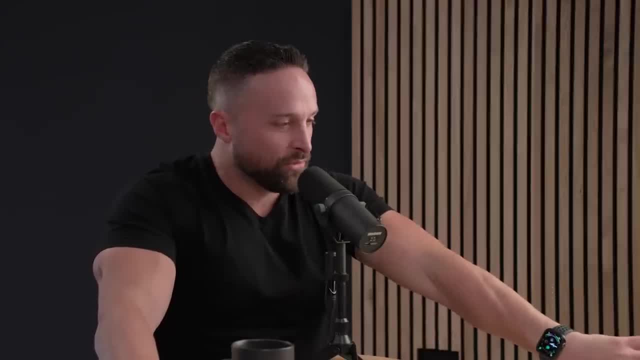 dream student. So at the end of 11 weeks we looked at like lean body mass, We looked at body fat, We looked at hind limb weights. We didn't really see differences in lean body mass, but what we did see was a difference in hind limb weights. 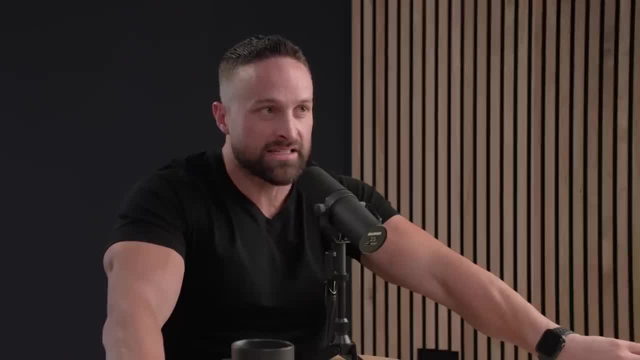 It wasn't massive, but there was a significant difference In the size of the muscles of the hind limbs of these animals, And so it was interesting that there wasn't a difference in lean body mass And what we found, at least, with the liver. 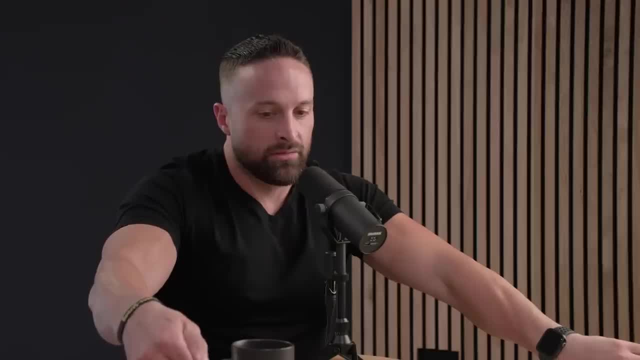 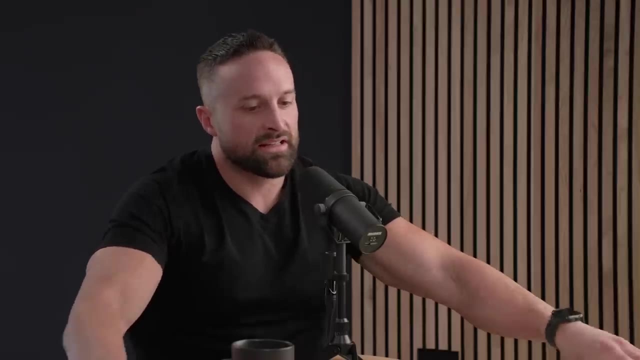 the animals that were eating the like one meal with really high protein actually had bigger livers, not like a huge amount and not something that I would consider unsafe, but they it was a statistically significant difference And so to me at least, like- if I'm trying to explain- like no different. 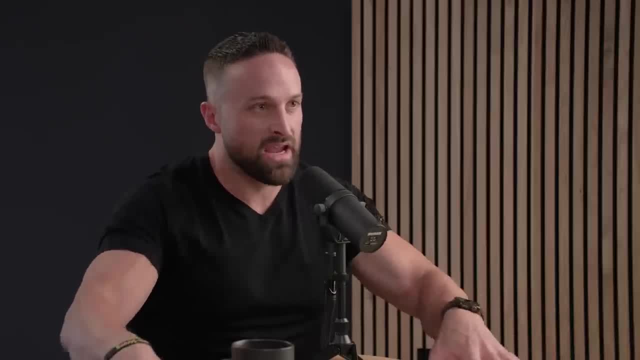 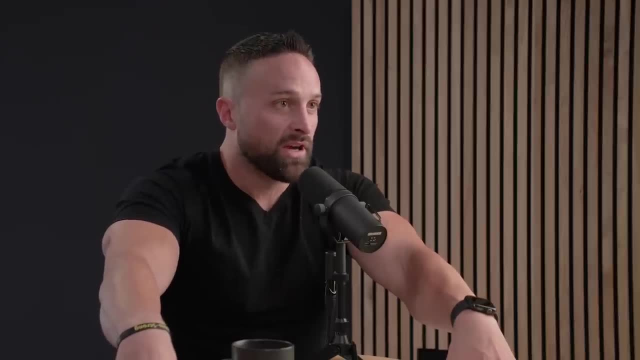 no difference in lean body mass but a difference in these hind limb weights. maybe there's some like sequestering of you know, like that that that's fueling a little bit more protein synthesis of the splint neck tissues, rather than you know. 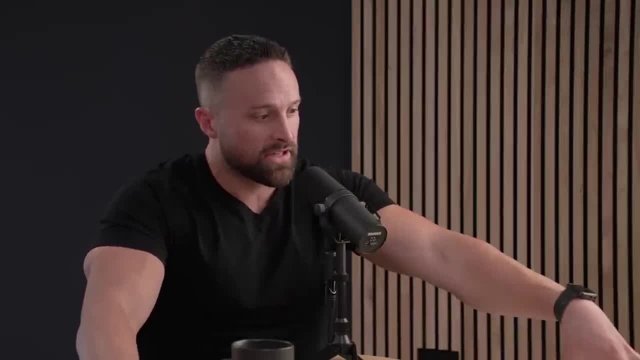 cause you're capping out skeletal muscle protein synthesis And we do know that the splint neck tissues are more sensitive or have a greater rate of protein synthesis per day, Like the rate of skeletal muscle protein synthesis in humans is about like 1% per day. So it takes like a hundred days to turn over, You know, skeletal muscle, whereas, like your entire gut, your entire GI will turn itself over in like two to three days, Right. So really, in the liver also has a very high amount of protein synthesis. 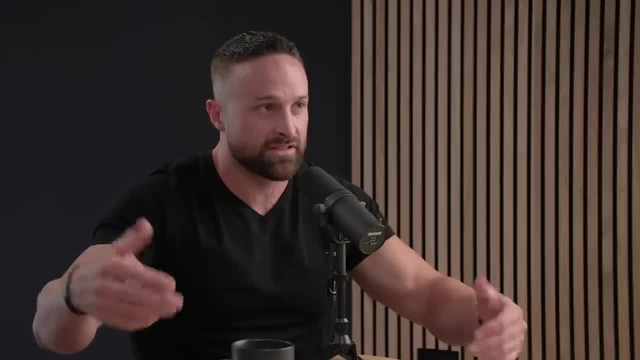 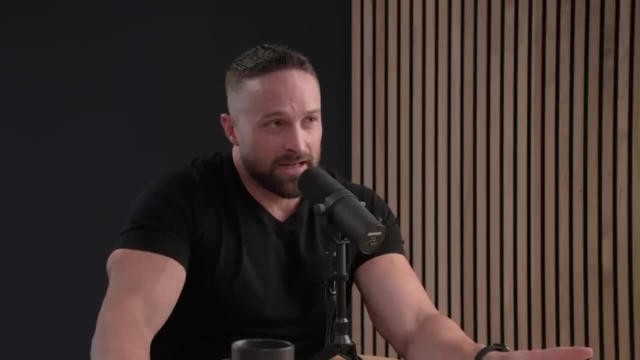 which is one of the reasons it's actually one of the most metabolically active organs. So all that to say, it has not it's been. there's been one human study that showed something similar, And then there's been a couple of others that didn't. 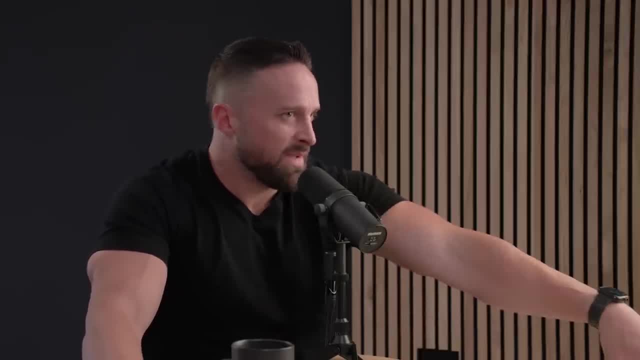 And then in the intermittent fasting studies, which is maybe a good tool to look at compared to compared to continuous feeding it. One thing I will say is it looks like the 16, eight intermittent fasting style. There's been a couple of studies with grant Tinsley. 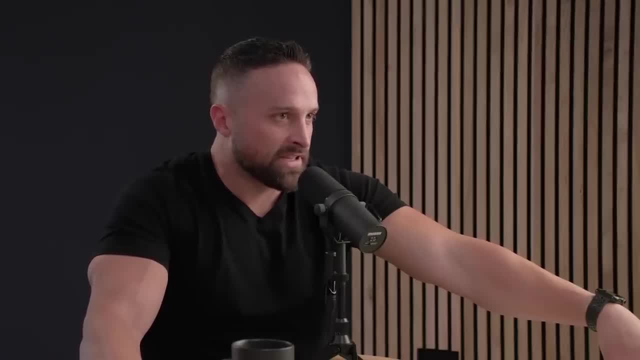 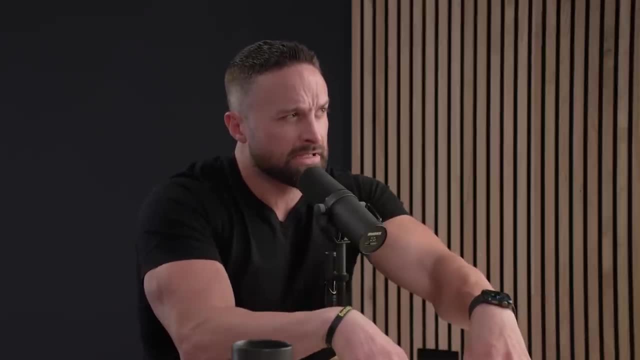 And this is something I've changed my mind on as well. Grant Tinsley has done a couple of studies where they did use the 16, eight protocol. They had them train during their feeding window and they had them eat- I think it was at least three protein containing meals- during that eight. 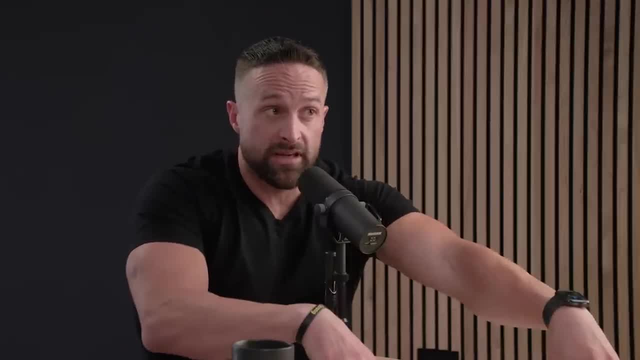 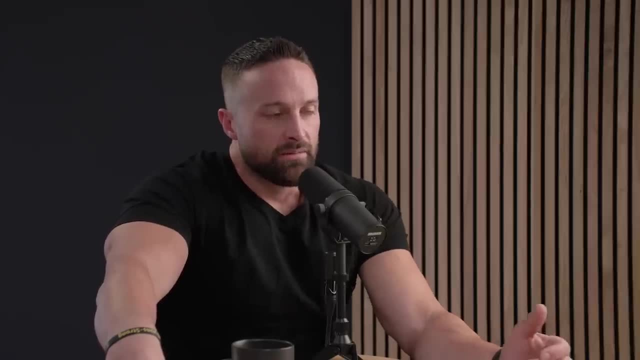 hours. These are humans. These are humans And they saw no difference in lean body mass at the end of the day. And then they did a study compared to people who were eating, like you know, as many times as they wanted throughout the day. Now, if you look at some of the more extreme forms of fasting- like alternate day fasting or like 22,, two or 24, there are some studies where you do start to see differences in lean body mass. So my suspicion is, and I'm 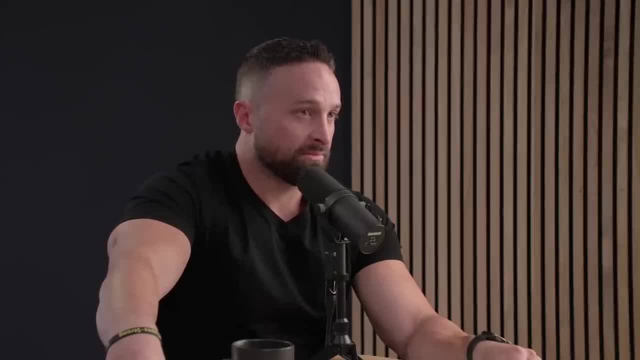 I'm I'm just guessing, So this is tenuous. My suspicion is, probably, if you're getting like you know, like a three to five, you know, probably if you're getting like two to three like high quality protein meals in a day, 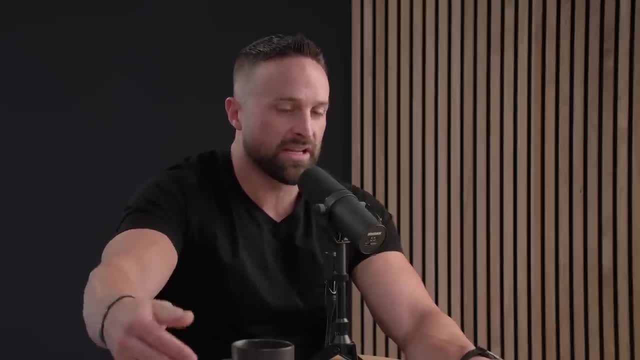 you're getting the vast majority of the benefits of protein, that the most important thing is getting enough total And then secondarily trying to get you know at least two or three meals with high quality protein in. But if you're going like pretty extreme with like alternate day fasting or you know, maybe only one meal a day, then I think there may be some effects on lean body mass. But again, these can be mitigated. mitigated as well If you're doing, you know, hard resistance training. typically that is the biggest lever in terms of lean body mass. 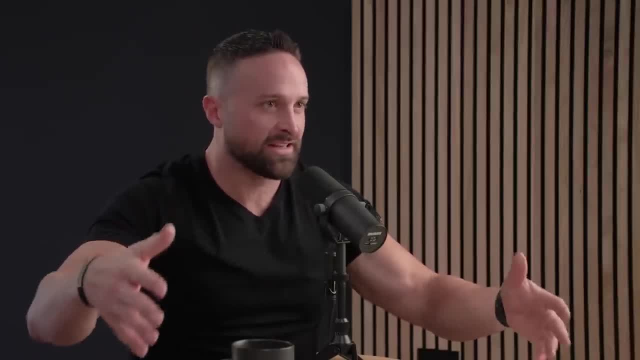 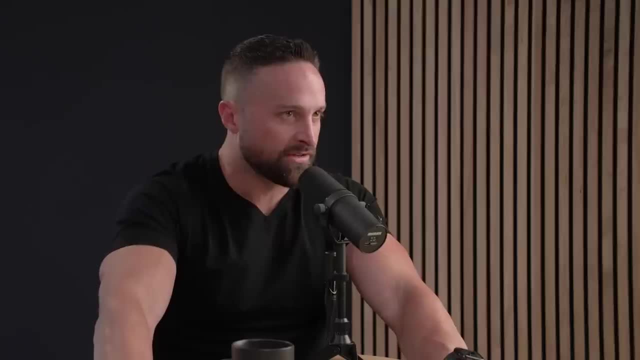 Yes, You know, protein distribution may make a difference, but I'm trying to put it in context. So people don't feel like they need to go out and eat. you know four meals a day, But again. so what I would say is, like some of the more milder forms, 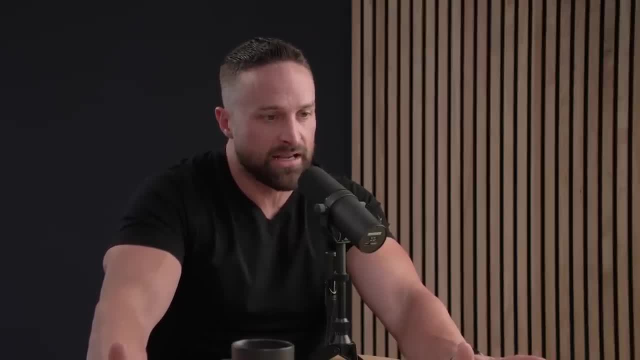 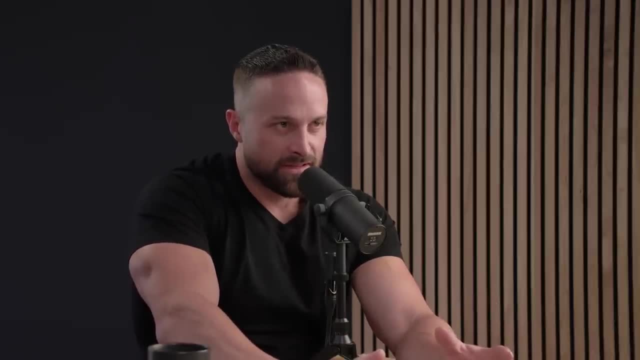 of you know, time-restricted eating appear to be fine for lean body mass. Now, the caveat is the following: One of the nice things about animal studies is um is when you consider if you want to have a high subject number. 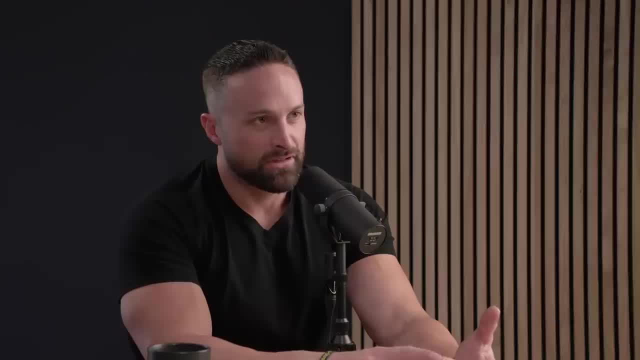 high level of control and a long duration. it's pretty much your only option, right? So I I've, uh in our research review, uh, reps, I created a Venn diagram which basically is like three um. 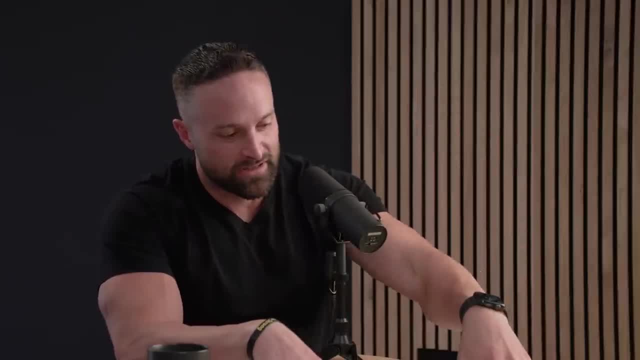 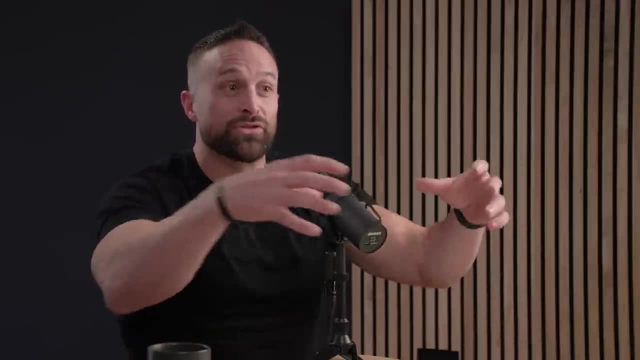 you know circles crossing over. One is study duration, One is um level of control and the other one is subject number. And to get all three of those circles to cross over it almost has to be in animals, Right? 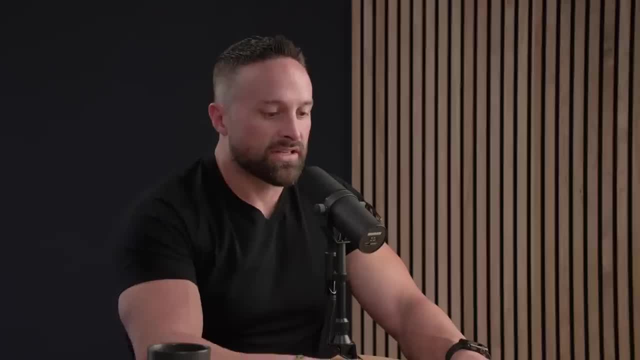 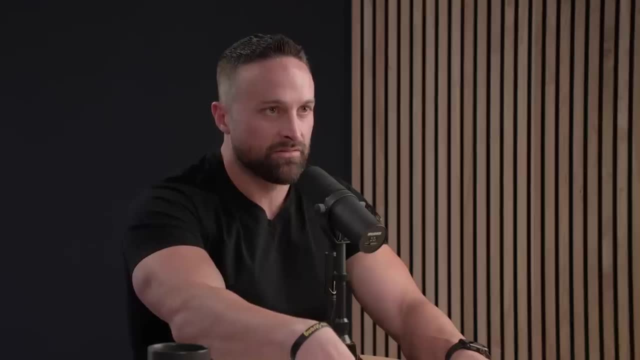 So in this in reps is it's a newsletter or a book, So it's a. it's our monthly research review. Great. So every month we review like five um studies that come out in fitness and nutrition, Like we'll usually do, at least one nutrition. 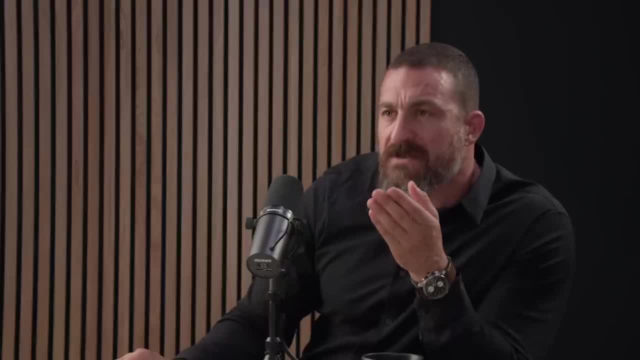 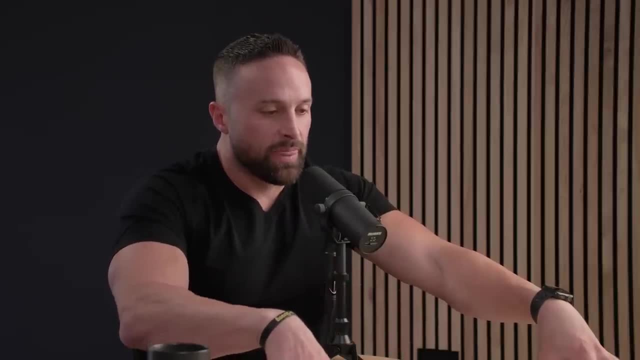 one training and one supplement per per month. We will put a link to where people can sign up. This is a sign up format: Great Yep, Yep. So it's a script subscription based service. So So, basically, when people might look at like my study, well, why did you see a difference in muscle weights, Whereas some of these other studies don't see a difference? I weighed out every single meal for 11 weeks, and keep in mind that 11 weeks in a rodent's lifespan is a really long time. 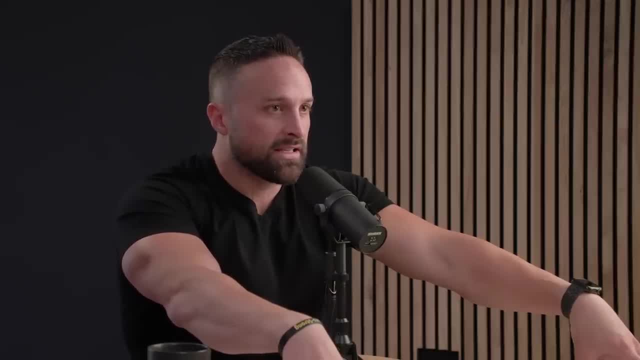 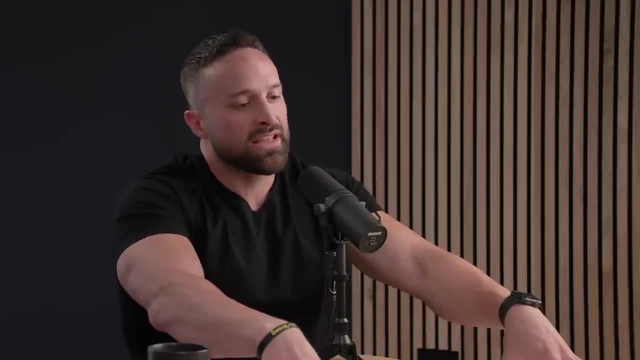 That's about an eighth of their total lifespan. So is it that there's no effect, or is it that the effect is relatively small and would take a really long time and very high level of control to see in humans? I don't know, but I think what I would say relatively confidently is: if you're 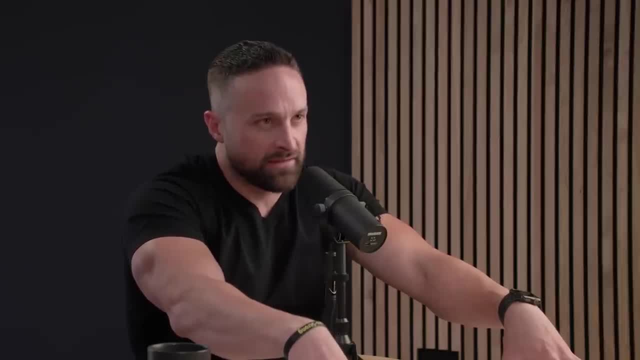 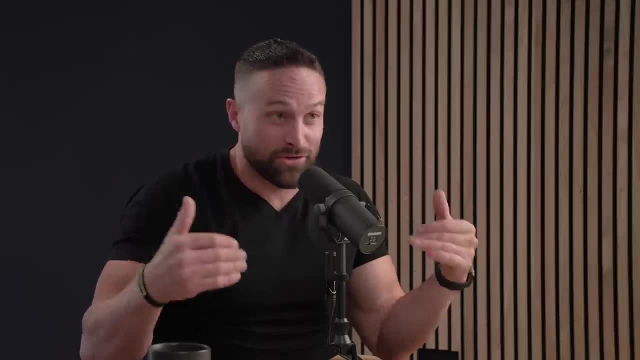 going to do like a 16, eight intermittent fasting. you're probably fine, especially And again, what is the goal right, Like if you're a bodybuilder looking to be the most massive person you possibly can, or you're a football player. 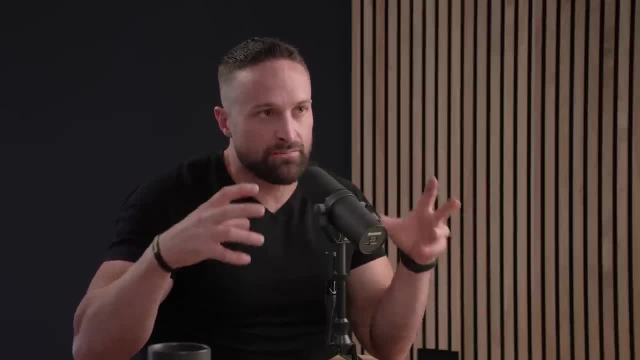 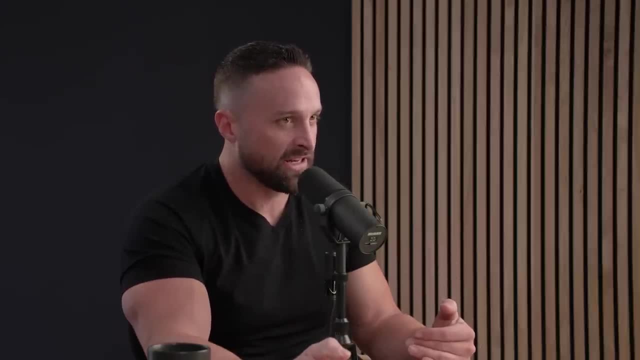 you're some in some field that that having as much lean body mass as possible is really important for you, Then I would say: well, you're not really gaining a whole lot by doing some form of time-restricted eating. I think most of the people listening to this don't do. 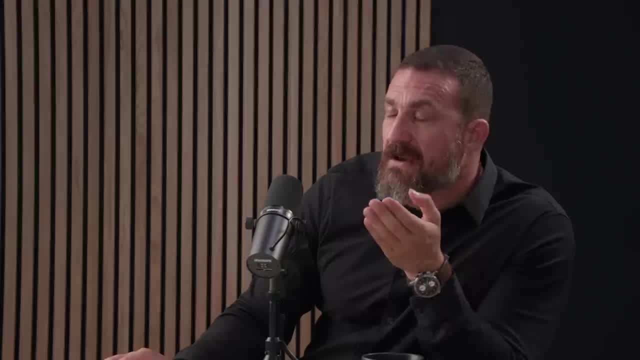 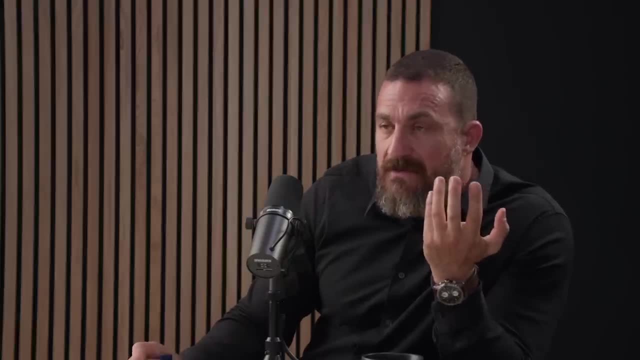 not fall into that category. I think most people want to maintain or lose weight. They'd like to perhaps add a bit of quote, unquote, shape or muscle to specific areas of their body and lose body fat. Right And, I think, your normal forms of time-restricted eating. 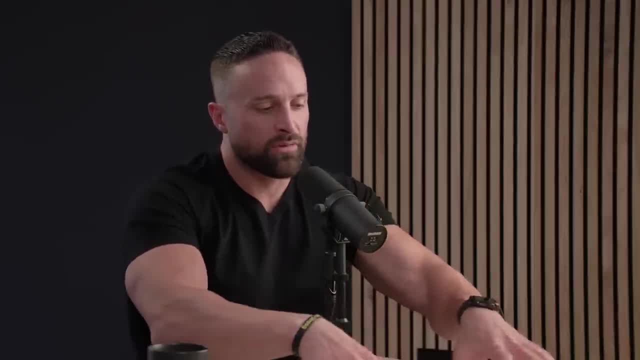 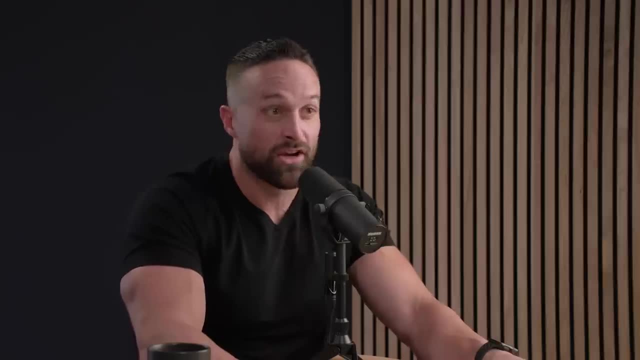 you're probably perfectly fine for that Right. And again, if I don't want somebody to think, well, I do. you know, I'm alternate day fasting and there's no point to me resistance training because I'm going to lose muscle mass. 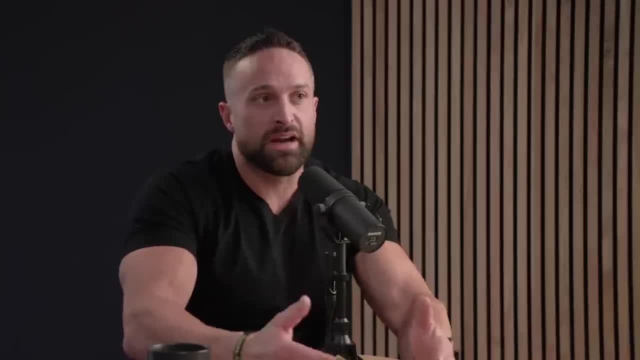 No, no, no, no, no, no, no. You can still build muscle doing that. You just might not build as much muscle as you would if you were eating in a more traditional format, But if that's something that works for you and your, 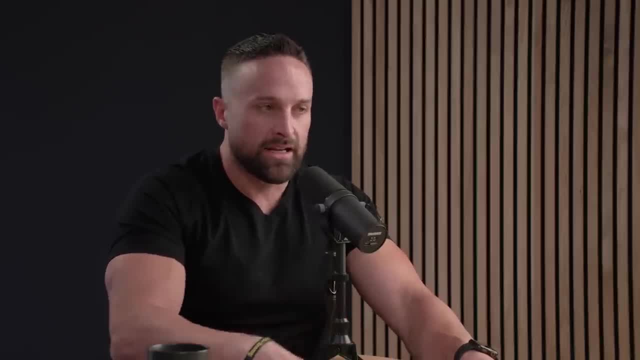 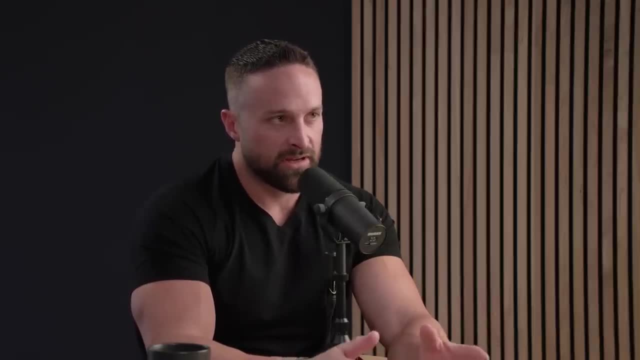 goals and especially if it's fat loss or, you know, controlling your calories, then again it's. it's about the hierarchy of what's important, right? So, to answer your question, I do think that timing and frequency matters a little. 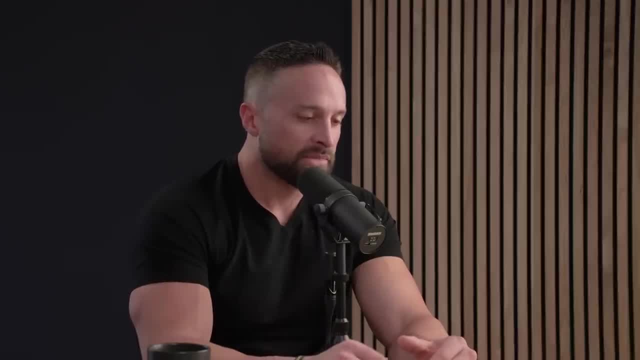 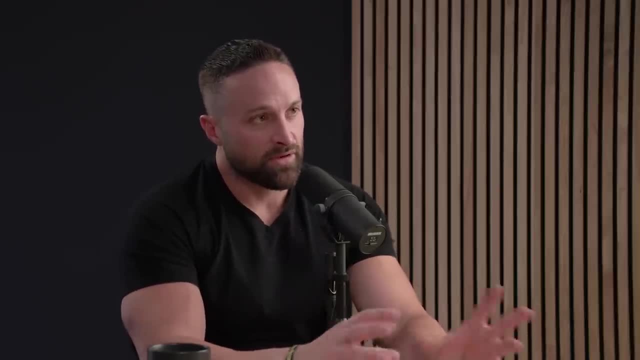 not so much frequency but distribution more so. Um. so I think the distribution matters, but it's a. it's a much smaller lever than just getting enough total protein in. And then, as far as like animal versus plant, I used to be in the camp of: there's no way. 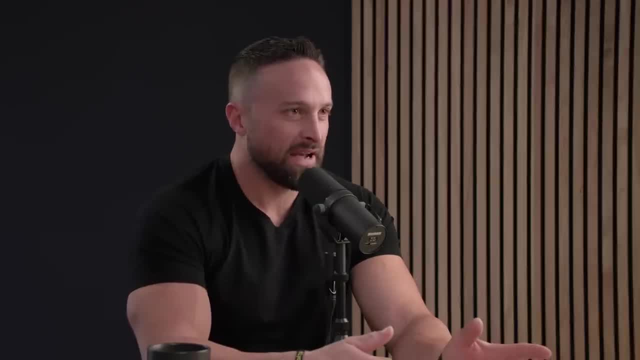 somebody can build as much muscle on a plant based diet- And now I think I've come back to you- can? it just requires a little bit more planning. Um, and I don't want to say always, but it's very difficult to do without an isolated source of protein. So unless you're going to supplement with an isolated plant source of protein, it's very difficult to get enough without going over on total calories, because you can figure that especially like take somebody who may be calorically restricted trying to get enough protein from whole intact plant sources. 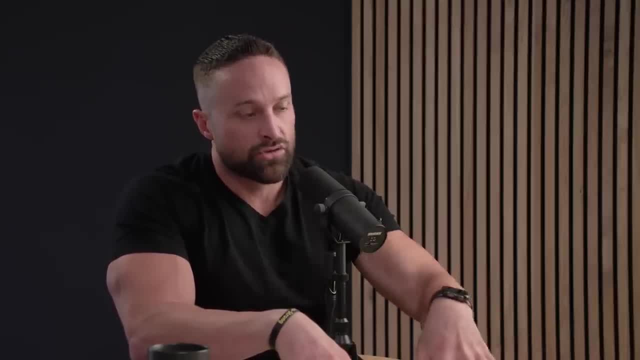 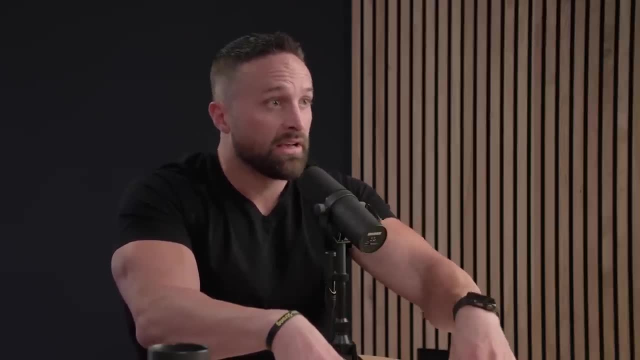 So you've got a few different things working against you. One, the sources of protein you're consuming also have carbohydrate and or fat Um. two, it's a less bioavailable form of protein. and three, it's a lower quality of protein in terms of it has typically less leucine. 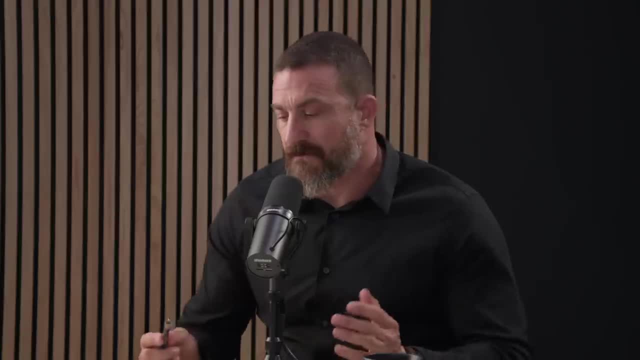 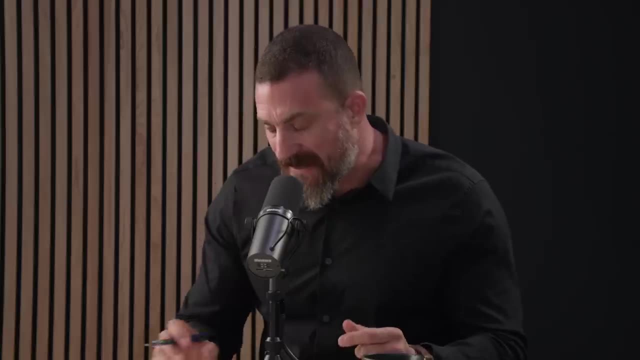 less branched amino acids and less essential amino acids. Um, you answered the question that I almost interrupted you to ask, which was: does it boil down to the leucine content? And um, it sounds like that is one of the components and that. 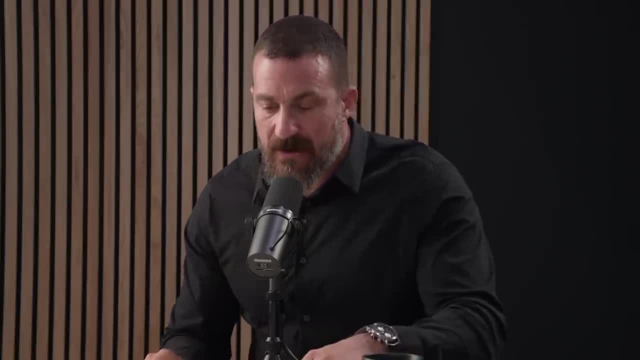 uh, a lot of the vegan and vegetarian sources of excellent protein. um, that excellent protein vegetarian or vegan source is co-packaged with calories from carbohydrates and or fat that make it hard to stay. stay under the clerk threshold, Whereas a steak is. I'm not. 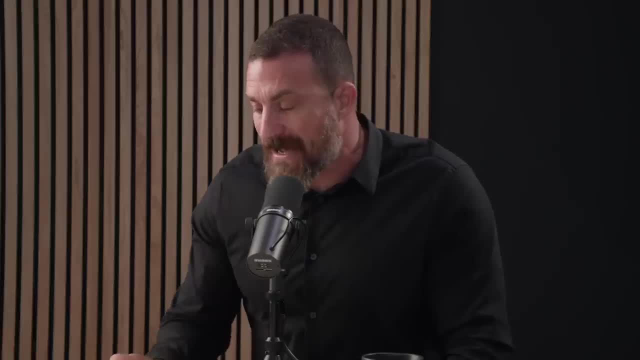 and obviously people might want to avoid that for ethical reasons, but that's a different matter entirely. but a steak or a piece of chicken or an egg is well, an egg, you know, has a yoke, which is there's fat there. 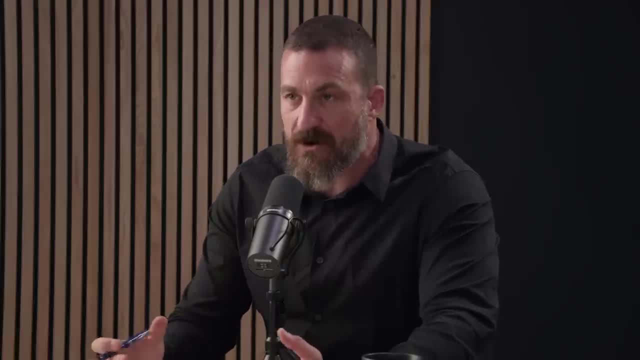 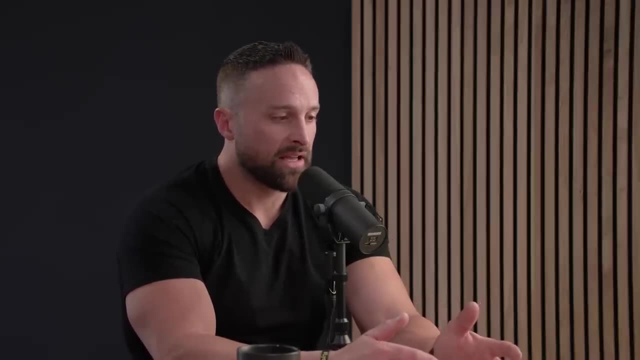 but is almost a pure protein fat source. There's no carbohydrate along for the ride, Right. So I think what I would say is that you know you can do. it takes a little more planning, Um, and you're almost always. 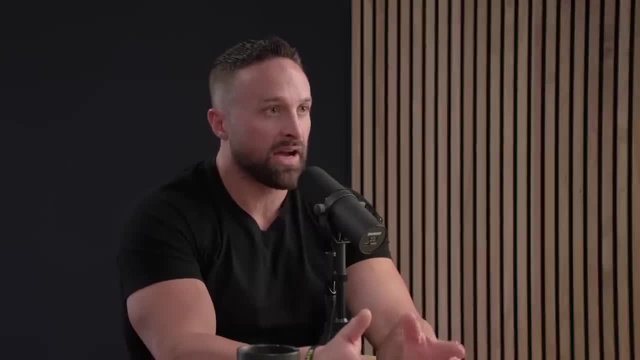 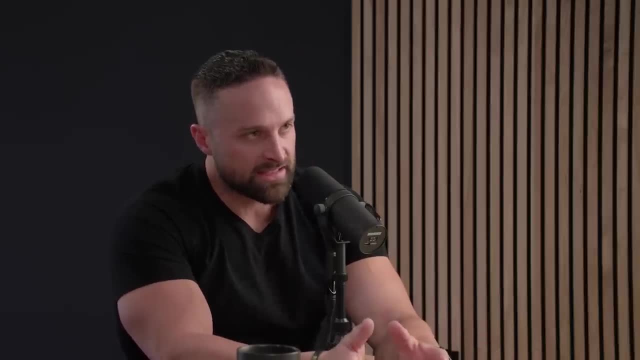 if you're a vegan especially, you're going to be better off like something with some isolated form of protein, uh, or vegan form of protein. Now, this is where it gets into. people say, well, what about the limiting amino acids and those sorts of things? 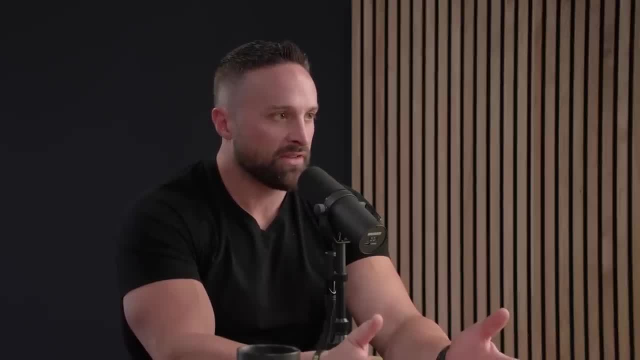 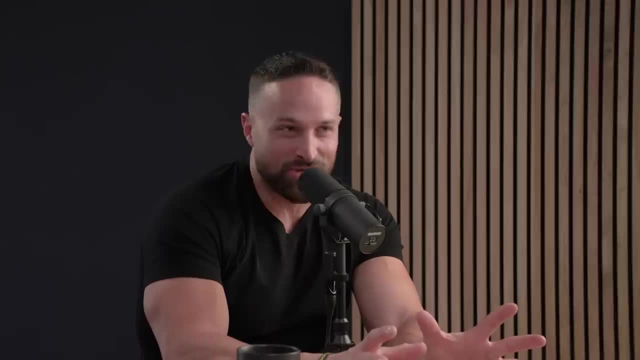 It's a consideration. Um, some of the better forms of uh vegan protein in terms of amino acid content are like soy. Now I can- everybody here- everybody's screaming online about their testosterone levels. in terms of actual outcomes and looking at testosterone, 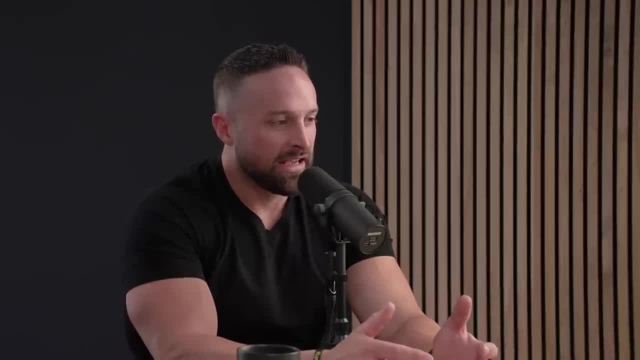 There was a recent meta-analysis looking at soy, And I think if it's your only source of protein, then maybe the dosage is high enough to cause some weird, weird effects. Um, but if you're just using it like once or twice a day, 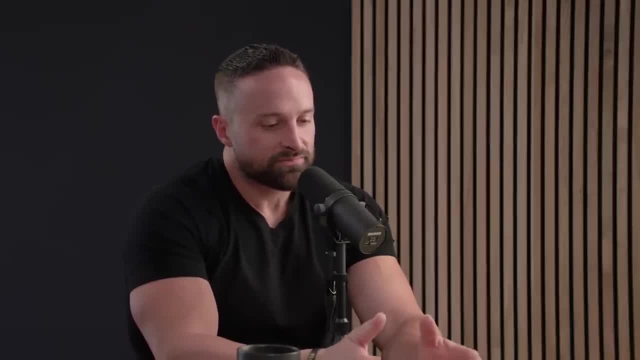 it doesn't seem to have an effect on testosterone or estrogen, So that can be a decent source of protein, because it is a complete protein source. Um, it does have a PD cause of one, which PD cause is basically a- uh, a measure of protein quality based on does it provide enough of all the amino? 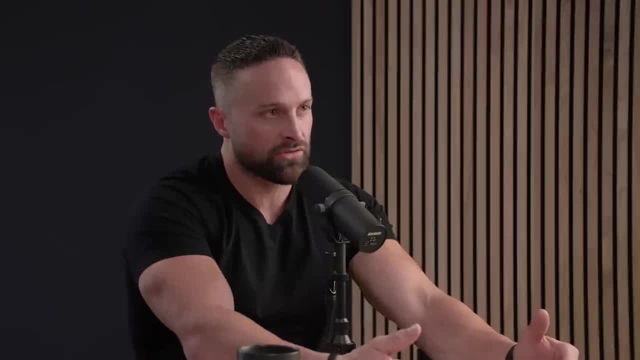 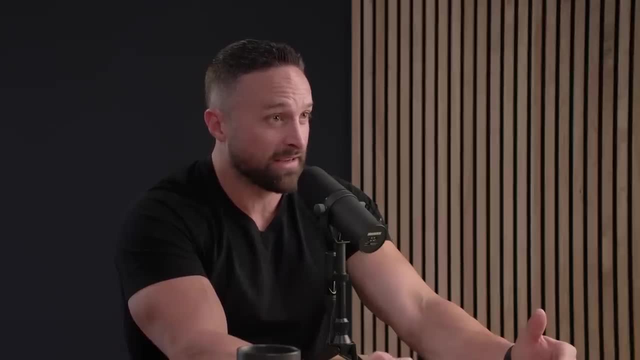 acids so that none are limiting, And so soy is one of the only vegan sources that does that. Interestingly, potato protein isolate- uh, that actually has a similar essential amino acid content to whey. So isolated potato protein it's just really hard to find. 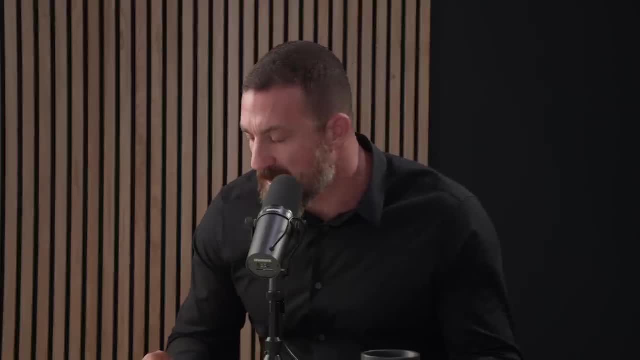 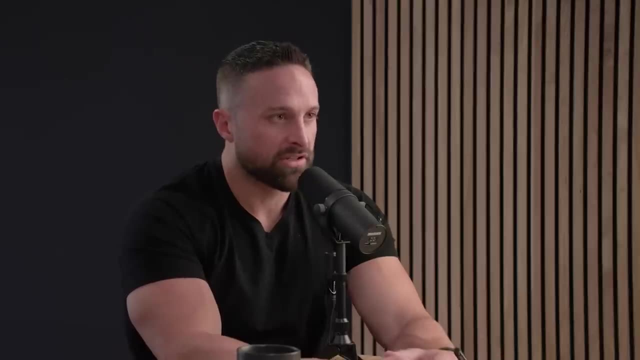 I've been. I've been trying to take note. Vegetarians take note because our vegans rather cause whey is vegetarian Um, and whey is a very high quality protein protein source and actually they're actually um creating whey now out of. 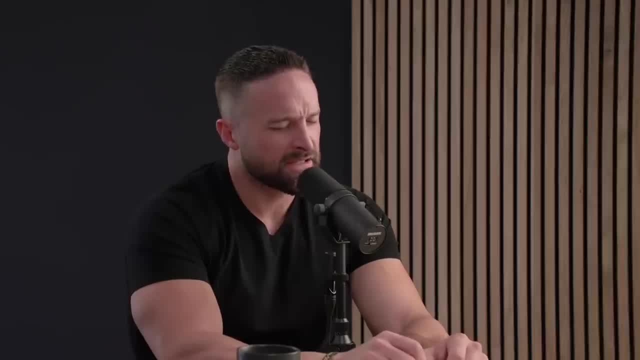 um, I think it's. I may mischaracterize this, but I believe they're able to produce an out of like yeast or something like that. Amazing that, um, you know. so for vegans, now, this is a great option, because you can have whey that's not animal based. 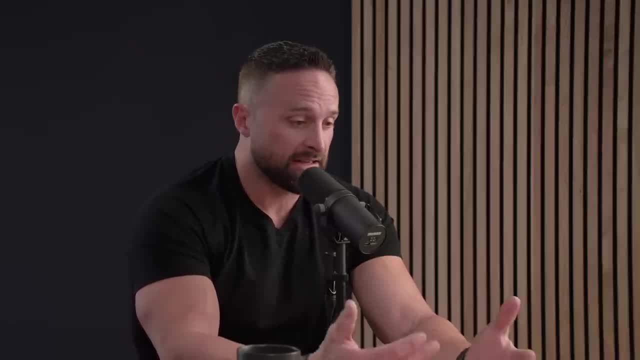 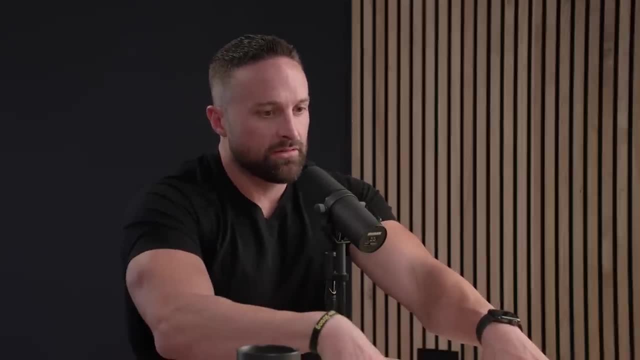 That is going to be every bit as good as an animal based whey, So I think that's great. Um, getting to the leucine, let me go back Sorry. So another reason that the using an isolated protein can be helpful is: 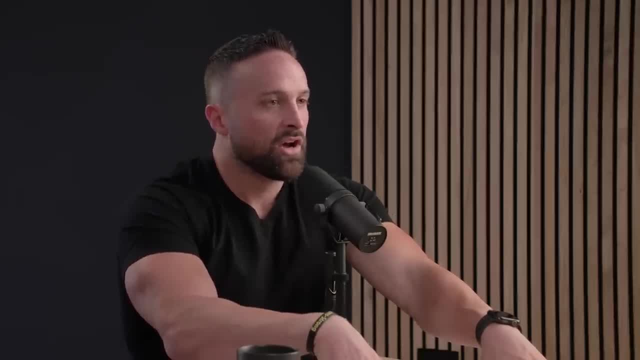 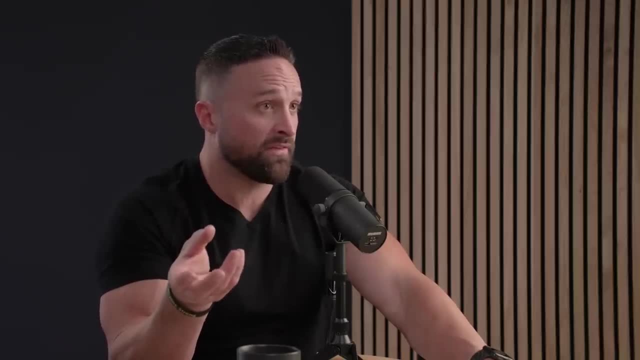 um, because it's more bioavailable as well. when it's been isolated out, when it's the protein bound up in the actual plant material, it tends to be less bioavailable. Now, cooking can help increase the bioavailability- bioavailability because it breaks some of those bonds and whatnot. but it still seems to be lower. and you don't? it's really interesting. There was a recent study where they did a corn, wheat and pea blend of protein versus whey And basically the outcome was, uh, 30 grams of each similar stimulated protein synthesis to a similar degree. but the plasma amino acids in the um- plant-based protein- still did not get as high as with whey. Now it may be that that's just. it doesn't matter, because once you get to a certain level you get all the benefits. 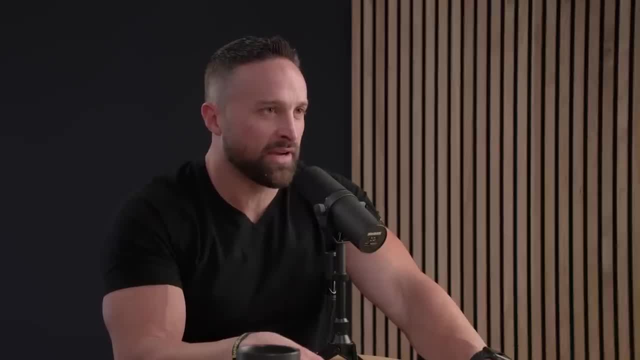 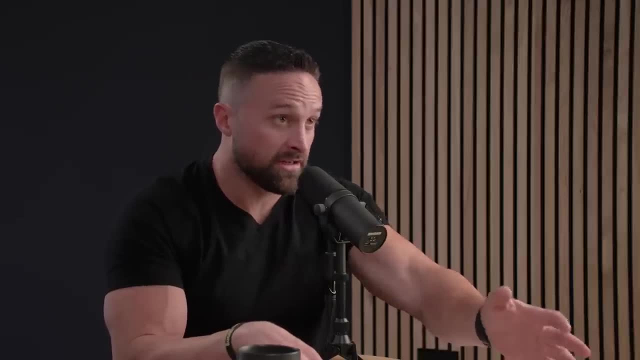 So, um, but I still found it interesting nonetheless that they didn't quite get as high. Um, the other thing to consider with the vegan sources of protein is the leucine content. So one of the studies we did was we looked at wheat. 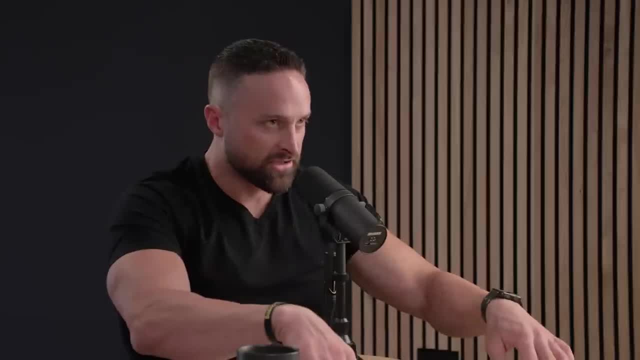 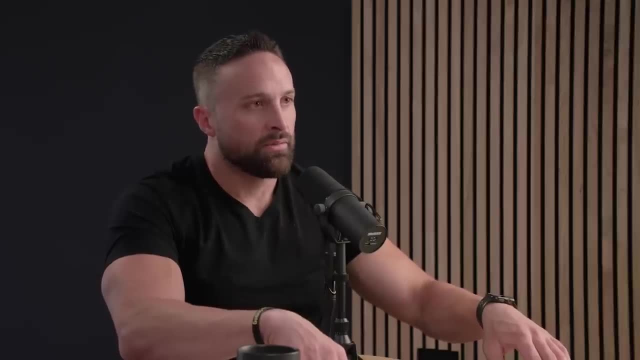 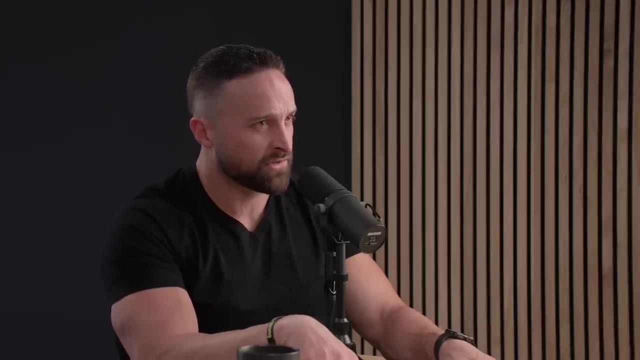 soy, egg and whey. isonitrogenous meaning, meaning we equated protein between the groups isocaloric, We had created cl, we equated calories and we looked at muscle protein synthesis And I think this was the meals were 15% of total energy from. 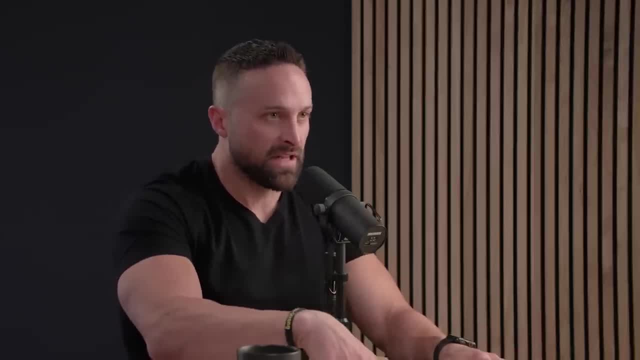 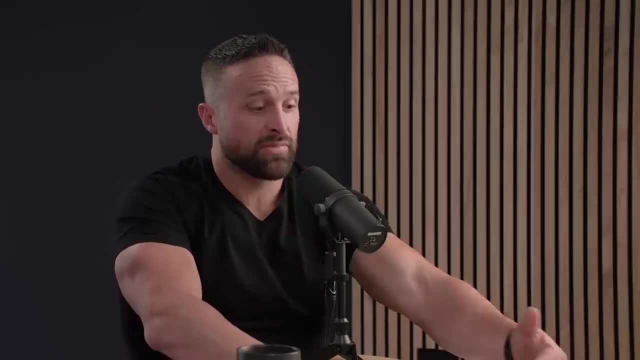 protein. So, like a like your food guide pyramid level of protein. Uh, and we saw that in the wheat and soy group. uh, they did not increase muscle protein synthesis, but the egg and whey group increased muscle protein synthesis. Now, 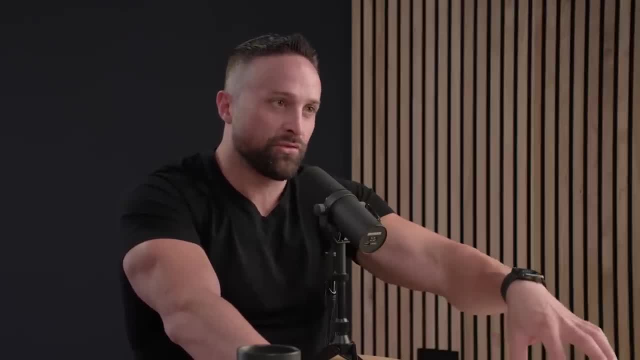 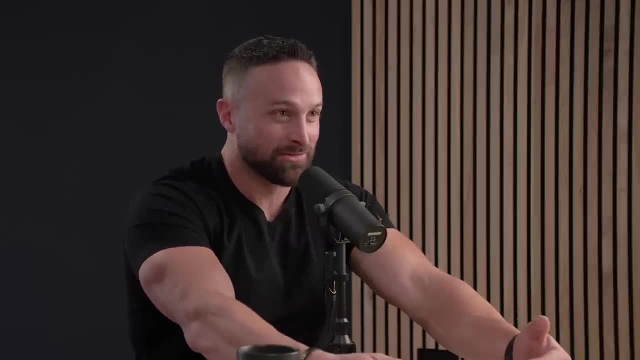 what's really interesting is we went back and we took wheat and added free leucine to it to match the leucine content of whey, And the protein synthetic response was identical. So again, I don't like to simplify things too much. 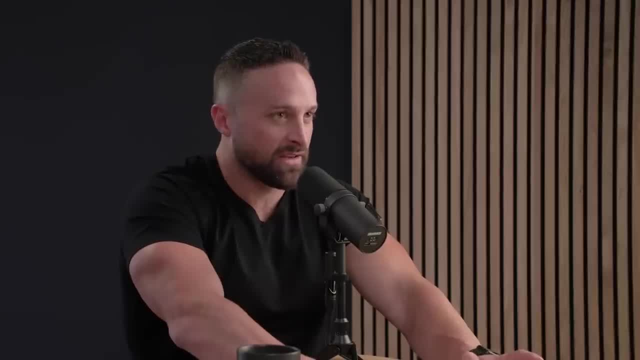 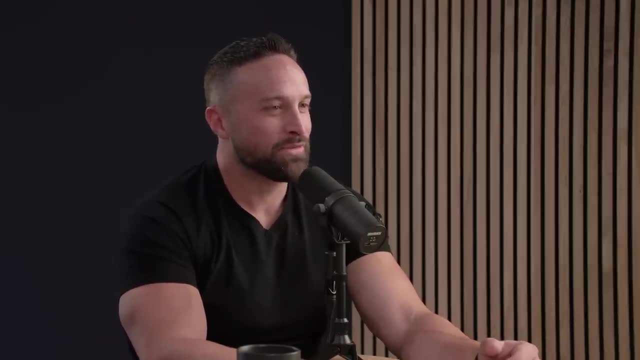 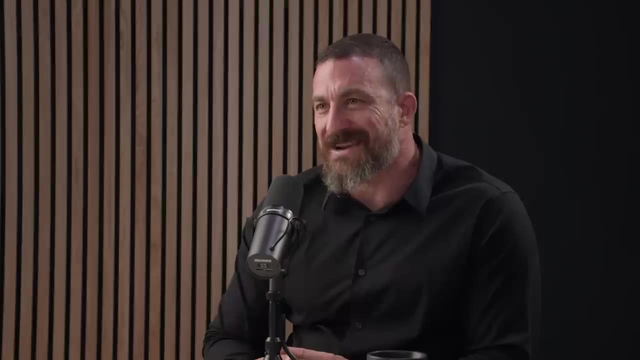 but leucine appears to really be driving this ship. And uh, I I'll never forget. a layman called me into his office one day and he would always do these like thought experiments of he. he liked to think about why, why something occurs the way it does, dangerous. 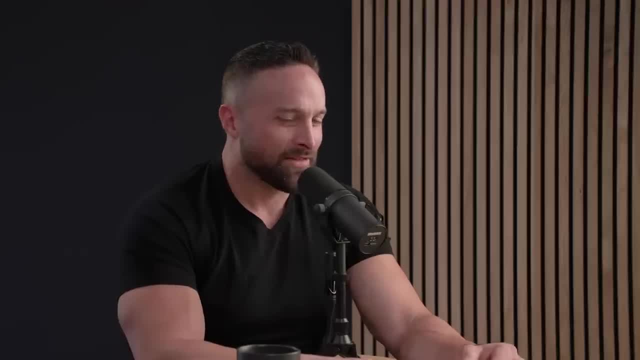 dangerous territory. Yeah, So he would say one day, I'll never forget He's like lane. Why do you think the body evolved to just sense leucine for muscle protein synthesis? And of course I'm like, uh, I don't know. 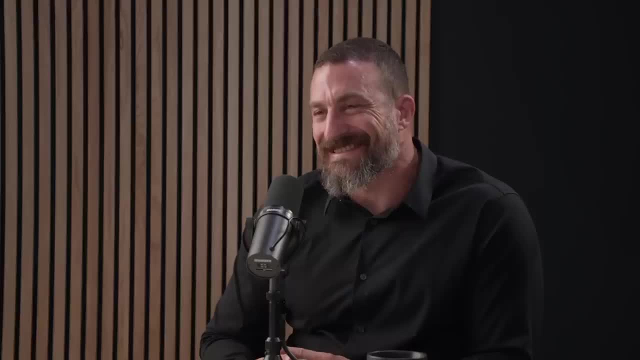 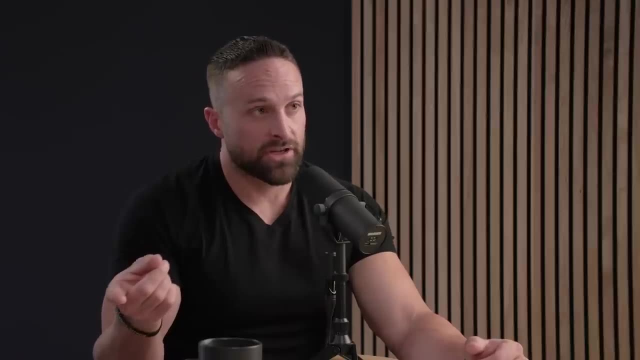 man, I just work here, Like I'm just trying to get my PhD, Um. and he said: well, think about it. You would want something that really wasn't extensively metabolized by the gut and liver, because you would want it to show up in the blood in values that reflect what. 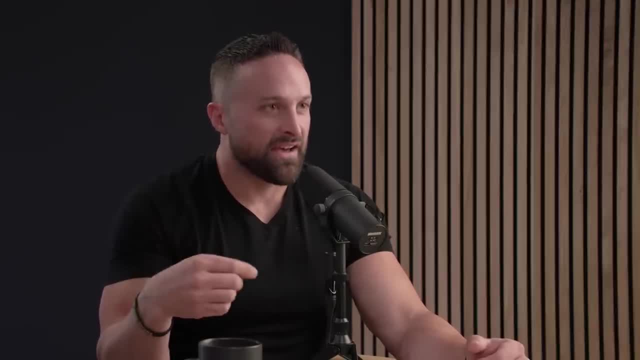 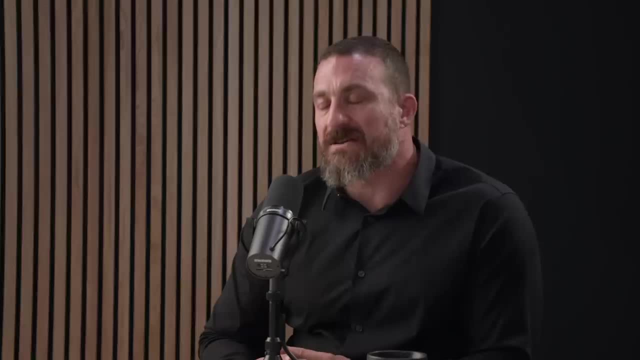 you just ate Makes sense, And you would want it to have passive diffusion across the muscle cell because you'd want to be concentration dependent, which it is. So get into the tissues and cells that need it most, Right So? but you know. 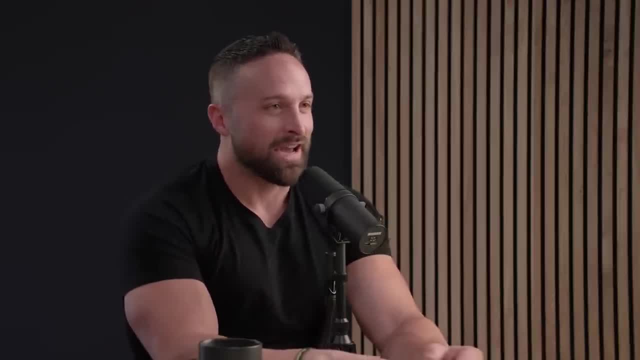 not having active transport but rather passive transport. Uh, so yeah, I thought that that was really interesting the way you broke that down. So few few different options for the vegan folks out there. You can use an isolated source of protein. 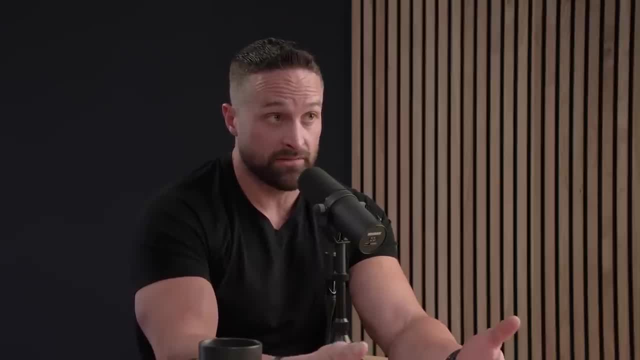 And again like there's going to be good options coming because this plant based way is going to be a great option for folks. Um, you can add free leucine to it, to whatever your source of protein is, just by supplemented leucine. 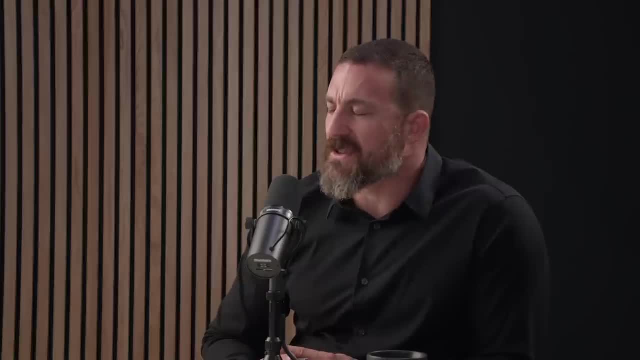 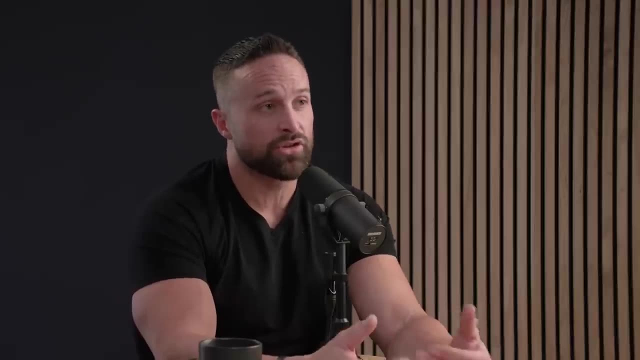 Now it tastes horrible. Yeah, I think I've heard that. Maybe I've even tried it. It's completely non-polar, does not dissolve in anything And it is a capsule rose. It can't be put into capsules. Yeah, So you could take a capsule. 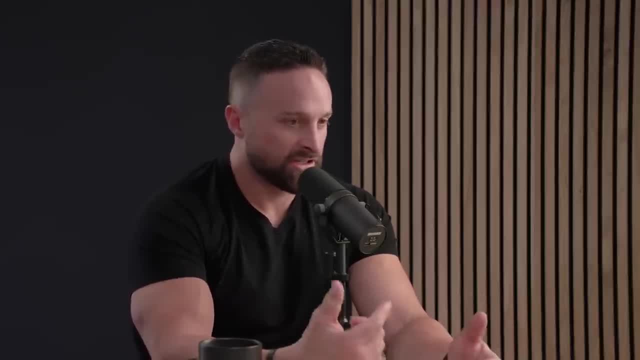 like, for example, if you're eating your normal meal, you could just take a capsule of like one gram of leucine. It's probably going to bump you off, bump you up enough that you're going to be good to go Um. 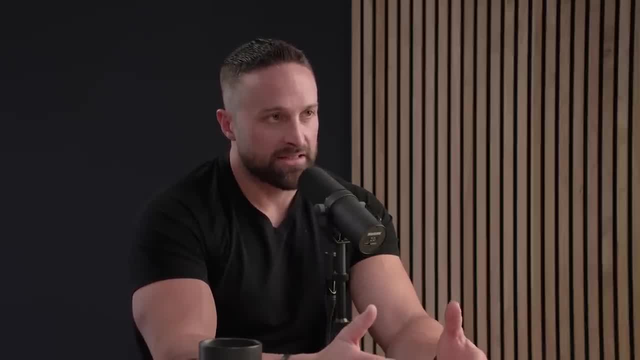 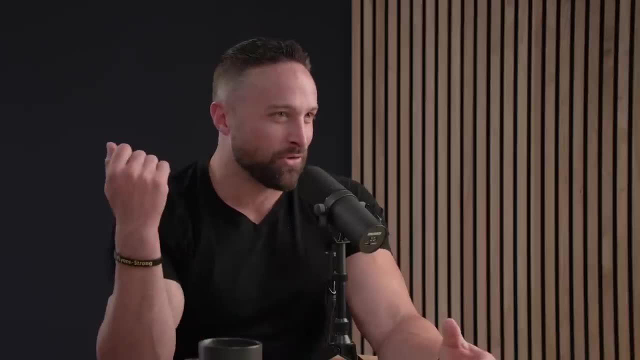 and then there's there's options like um blends, especially with corn. Corn is actually very high in leucine as a percentage of its protein. Now you got to remember like you go eat corn on a cob and you're getting like two grams of total. 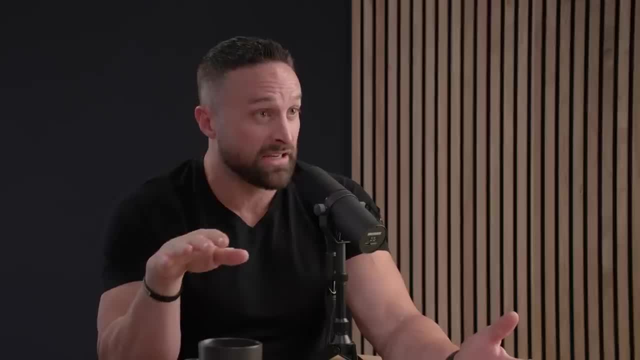 protein. So it's not that much leucine. but if you isolate out the protein, put it into a powder. Well, now you know when you're getting like 80, 90% of the weight is now protein. 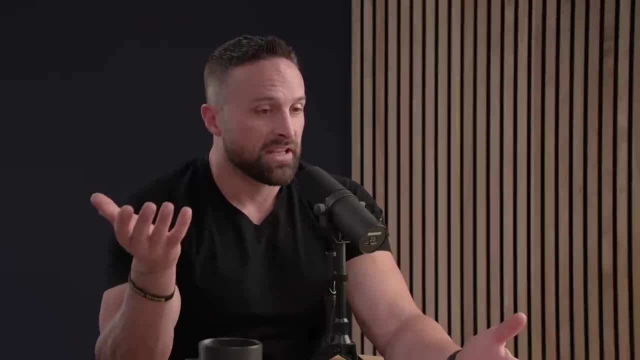 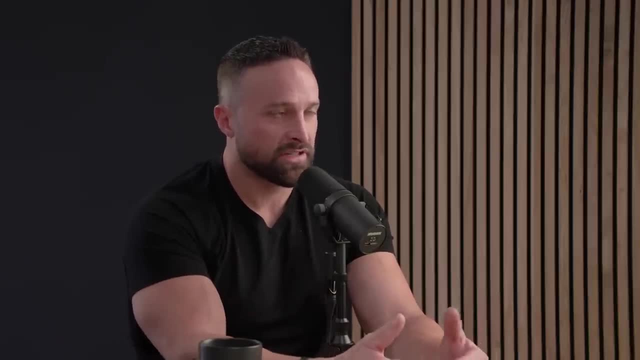 Corn is actually about 12% leucine in terms of the protein, So a great source of leucine. It is like almost Frank, deficient in some other amino acids, but you can blend it with a few other sources of protein, Like you could blend it with a soy. 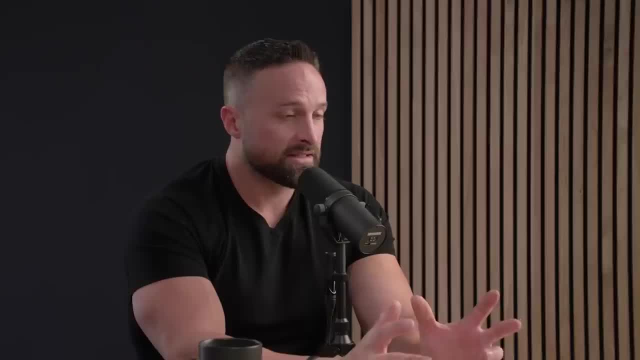 uh, a P, and you can create these complimentary blends that would actually have quite a bit of leucine but also some of the other essential amino acids. So there are options out there for plant-based folks, And I mean we have seen people who are plant-based. 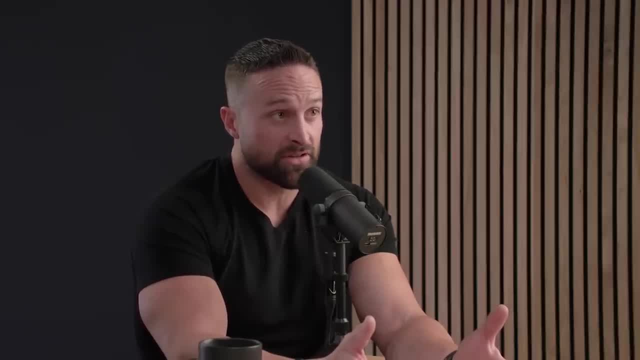 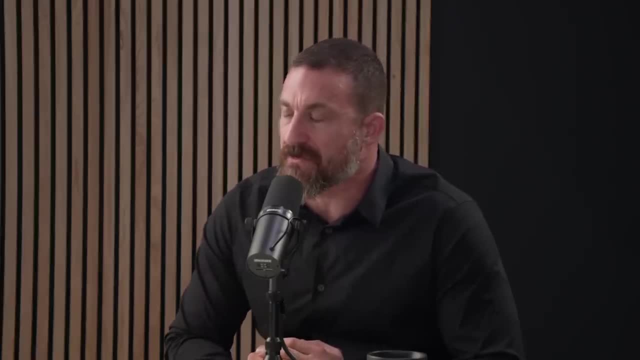 um, you know, build impressive amounts of muscle. There's quite a few bodybuilders that are plant-based and a lot of the endurance athletes like it, And even though, um, when we talk about muscle, we think about muscle building often. 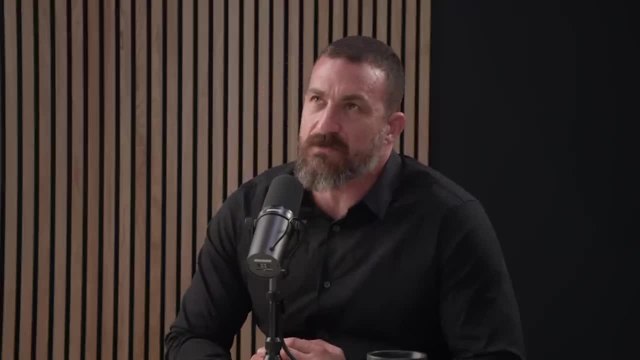 um performance in endurance sports and also just performance for the typical person who's doing some cardiovascular training- hopefully some resistance training also- and just living life. I mean. many more people now, it seems, are vegan or at least avoiding meat, in particular red meat. 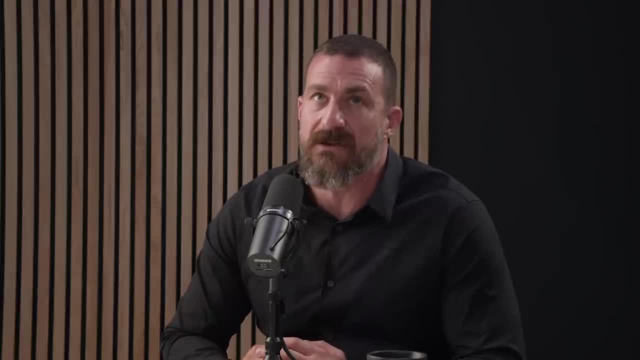 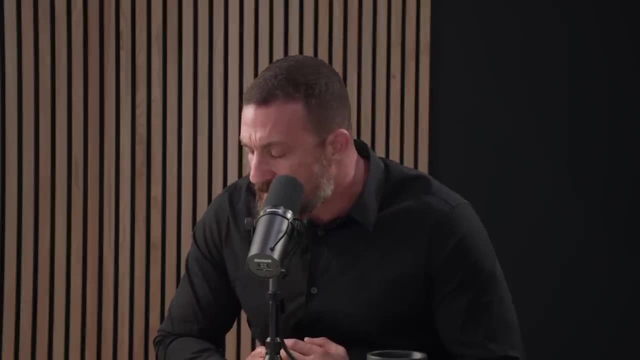 Uh, I'm not one of those people. I limit the amount and I certainly focus on the quality of what I eat, but I do eat red meat, which brings me to a question, Um, about, you know, just generally in terms of food choice. 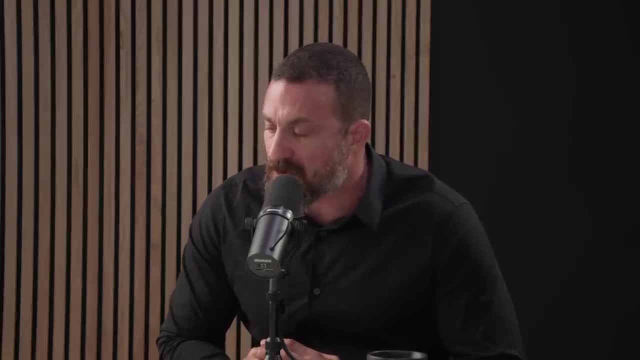 you know I can we come up with a relatively short summary of the following. Tell me if this is um correct or not that most of us should be focused on for for sake of health, health span and lifespan um. 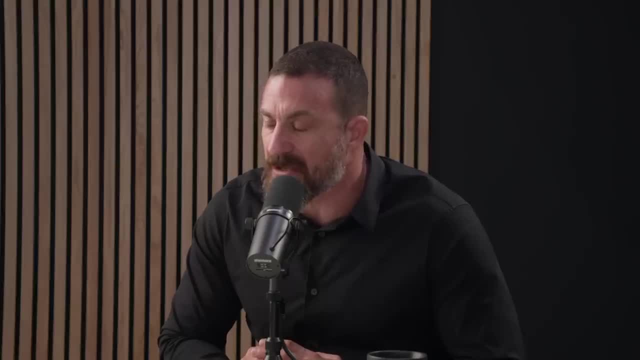 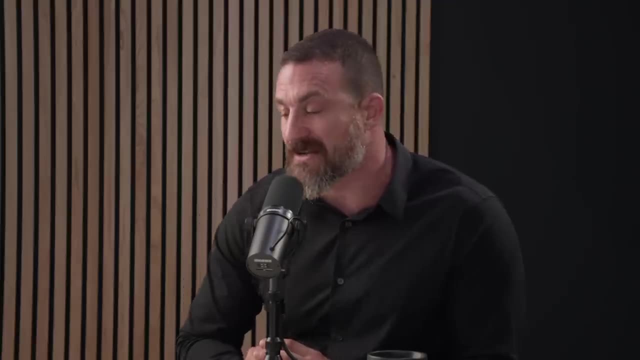 should be focused on ingesting minimally non-processed and minimally processed foods. you know, maybe even cooking our own food. You know, I realize that's heresy now, but I ideally we would do some of that and and really trying to avoid foods that are highly processed and have lots of 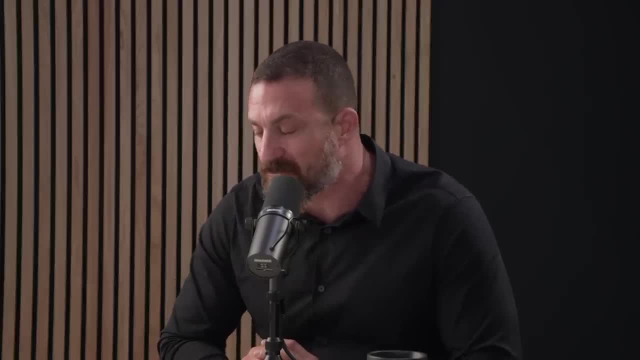 sugar, And I'm using this as a segue to get into a question that I really want your answer to. I've been dying to ask you this, which is if a sugar intake is not actually going up um as much as people think it is. 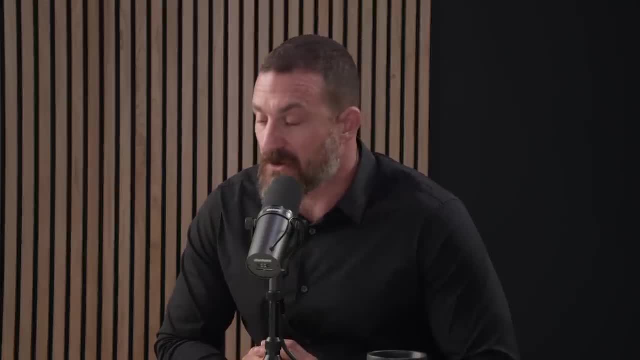 why are people getting so much fatter? Um, so what? what do you think about? um, just a general statement that we should try and eat. What do you think about the fact that we're eating foods that are low to no, minimally to not processed for about 80% of our foods? 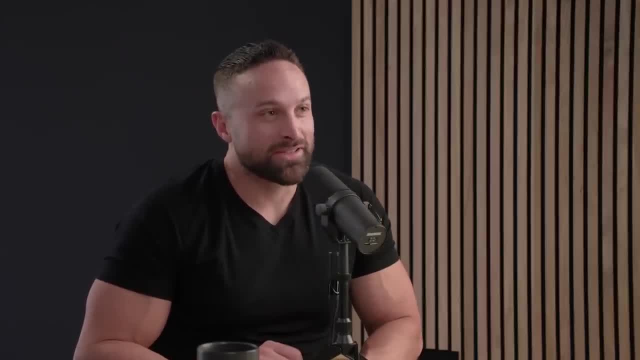 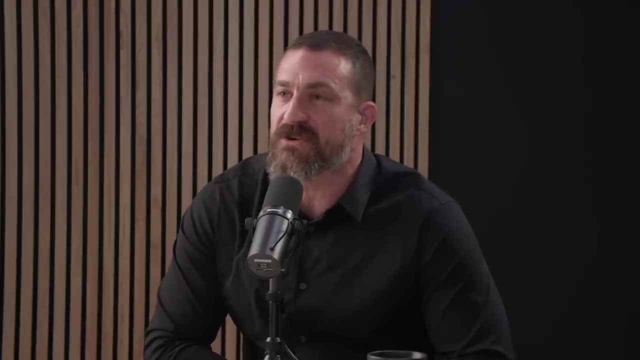 Is that a reasonable number? It's hard to actually get you know completely unprocessed food because almost everything goes through some form of processing, So I'm thinking like anything that wouldn't survive long um on, without refrigerators, Yeah. 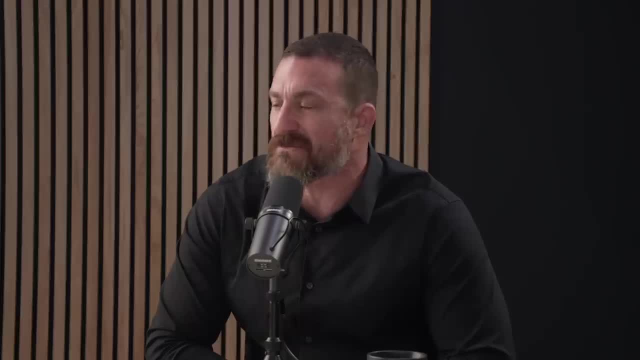 On a shelf like a like an apple or a banana or oatmeal, like ground oats. to me, as long as there isn't a bunch of other stuff in there, would be minimally processed. Um, a steak is not really processed. 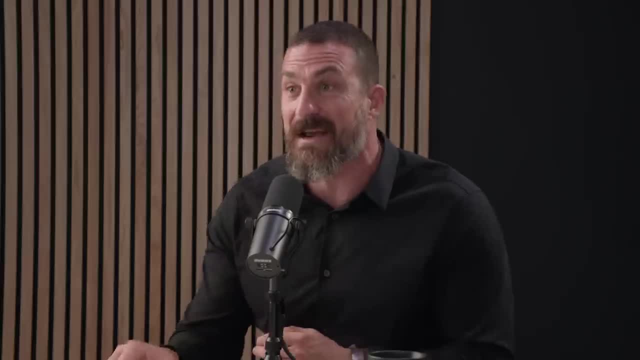 although it's cut off, the, the animal, et cetera. so there's a, there's a few steps in there, but yeah, um, that sort of that's what I mean. Yeah, Yeah, And I and I think everybody kind of gets the gist. 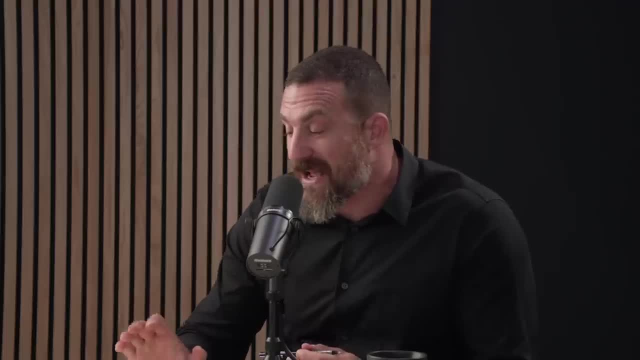 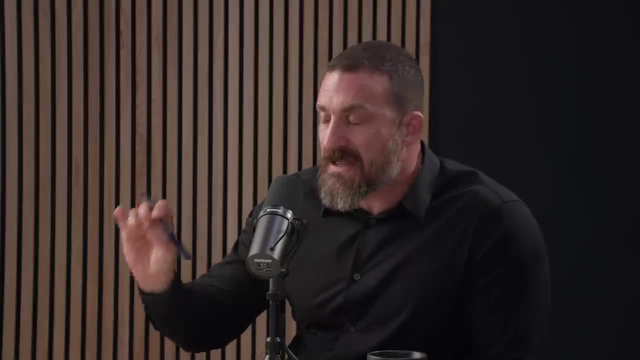 I I'm probably a little bit pedantic when it comes to this stuff. No, this is good. Actually, one of the things I appreciate, appreciate about you is something that I get teased a lot by people close to me, which is the caveats, and the insistence on precision is really important because, especially with online communications these days, 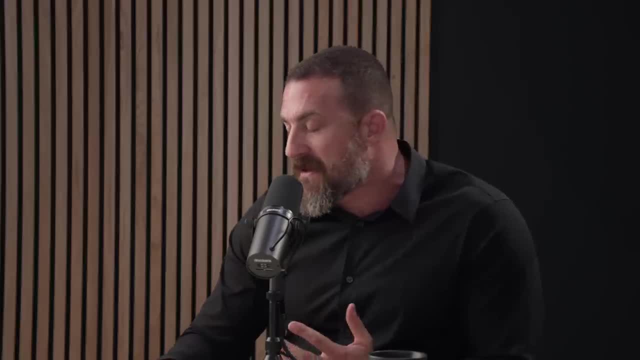 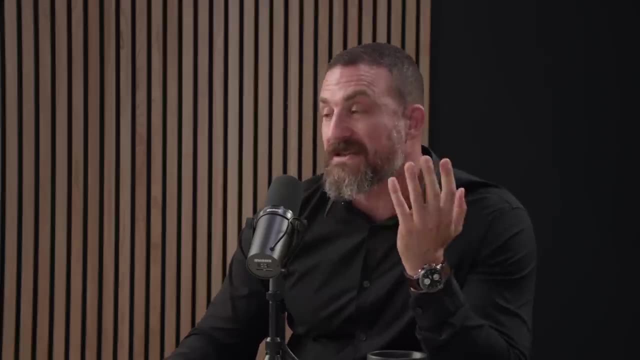 it's like a runaway train. you know people will. you know it's too easy to miss Interpret what you're saying, Very easy to misinterpret, And the misinterpretations are often used to leverage whole new ideas about what is and isn't true. 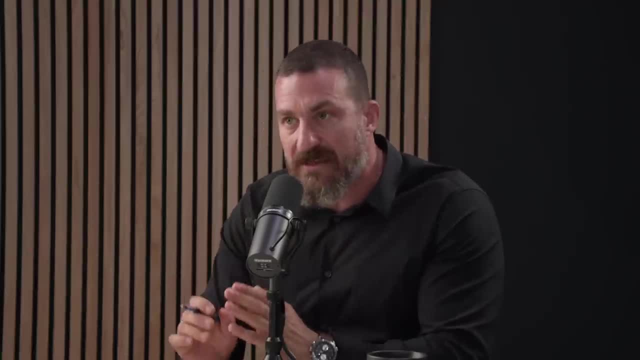 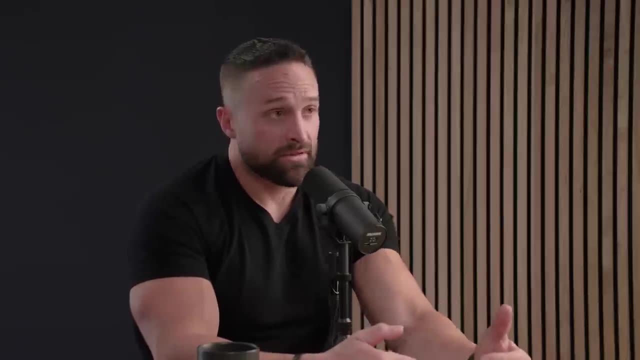 Mostly about what is true, Um. so I really appreciate the nuance and this is what a long form podcast really allows us to do, is is catch every, every curve, Yeah. So I would a hundred percent agree with what you said, that, if you were going to make a broad stroke, that trying to focus on minimally processed foods is very important. 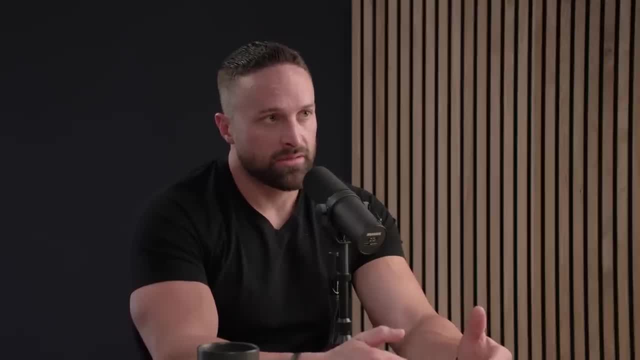 The one caveat I would say is: I think it's important to understand why, because otherwise people can make this weird association that like if I eat any mentally or any processed food it's going to kill me, or like every time I eat it it's like I'm smoking a cigarette and my health 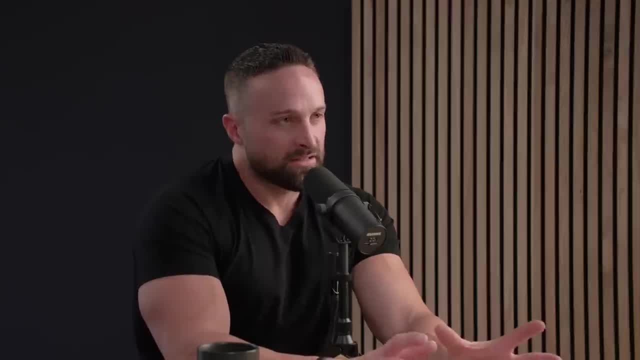 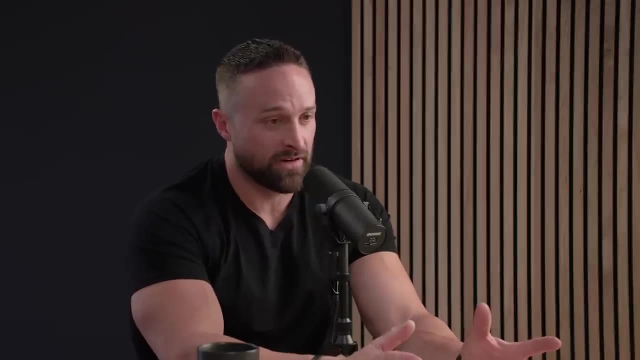 you know, my longevity is declining. based on the studies we have, It's mostly about the energy that processed food just gets people to spontaneously eat more And- and Kevin Hall showed this in his study- that was very- I mean he- he designed some of the most elegant studies in nutrition. 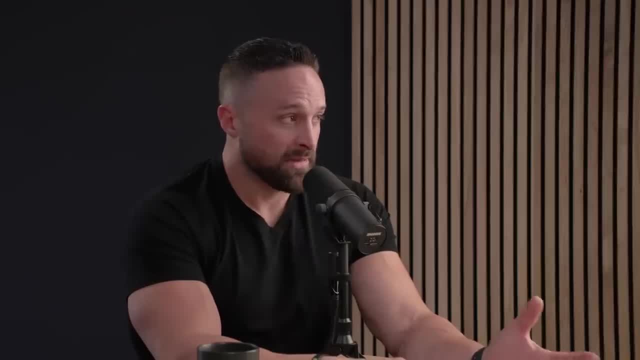 He's great- And they basically took people from a minimally processed food diet and then gave them access to ultra processed foods- Very few instructions, Just eat till you feel satisfied- And they spontaneously increased their calorie intake by 500 calories a day. 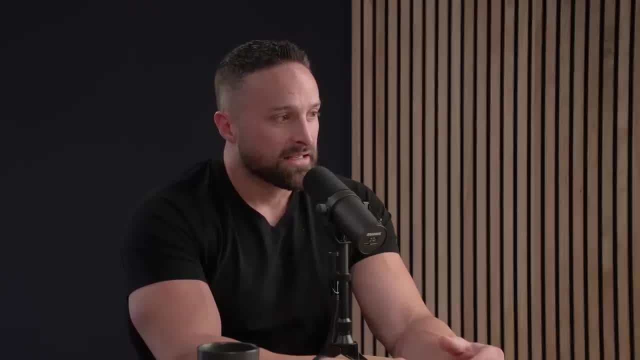 I mean that's, that's massive. So there's some and we quite haven't quite figured it out. You know, people said, well, it's it's car, it's sugar. It doesn't appear to be sugar. 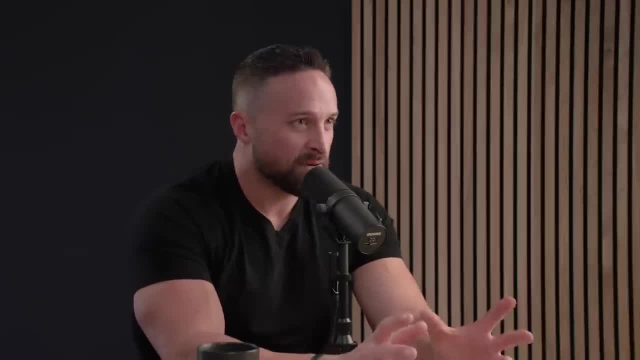 uh, in terms of just an isolation. Uh, well, it's fats. Doesn't appear to be fats in isolation. Well, it's the combination of sugar and fat partly. Well, it's the combination of sugar, fat and salt partly. 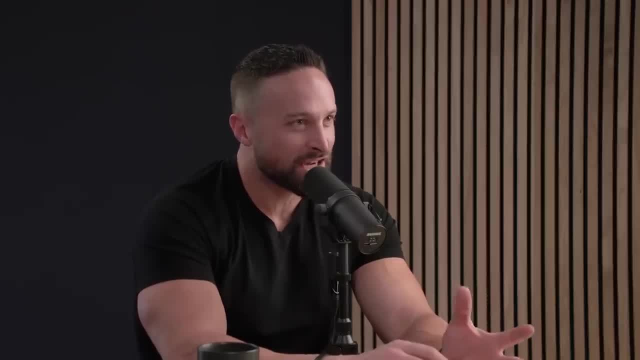 but there's some kind of like overall magic to the texture and the mouthfeel and just the overall palatability of stuff. which is always why I say there's like right and wrong ways to these different diets, Like, for example, like there's a right way to do plant based. 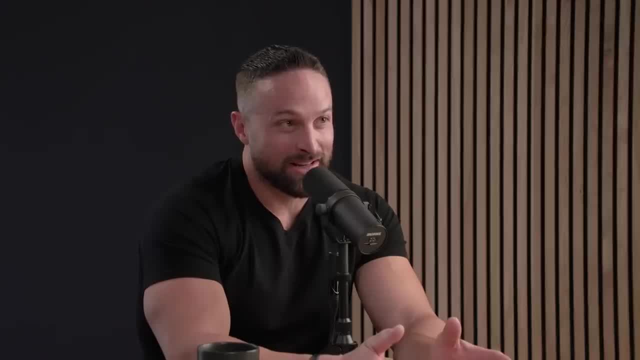 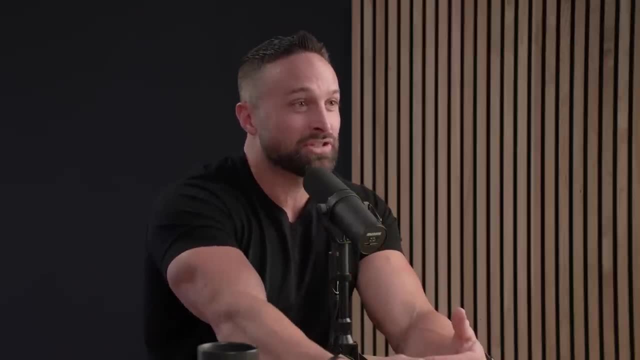 And then there's, you know, like what's in some of these documentaries where they're eating like plant based Mac and cheese. you know, And again, I love a good Mac And cheese, but like that should not form, like that should not be pitched as a healthy diet just because it's plant based. 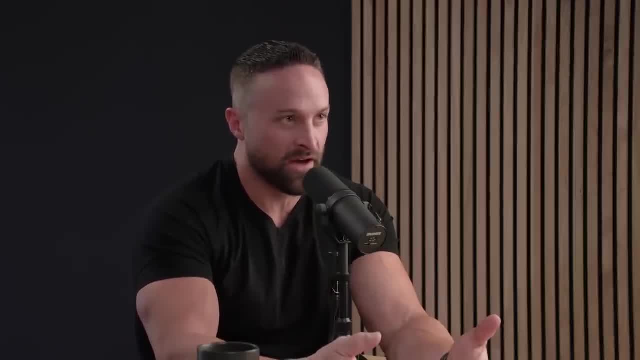 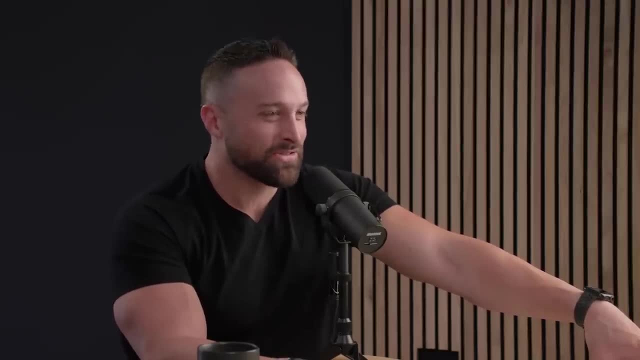 right, Because I mean, you're eating a highly processed food that's very palatable and easy to overeat. Same thing for keto. You've now got like keto ice creams and you've got, you know, keto cookies and all these sorts of things. 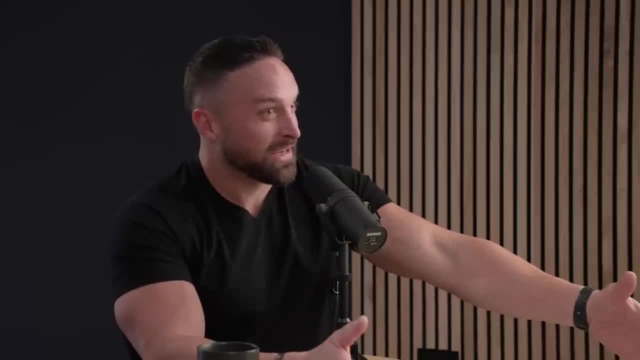 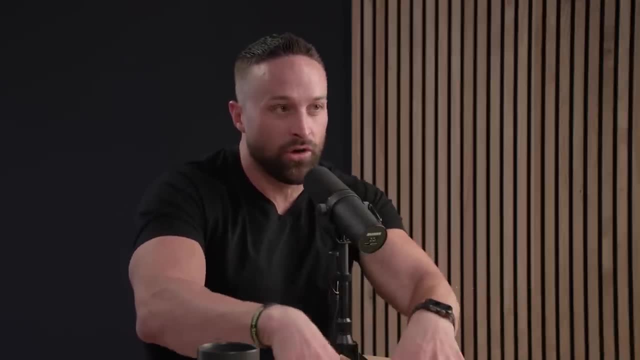 And I'm like, yeah, And if you look at them, they actually have more calories than the normal stuff. And I'm like, yeah, this is completely missing the point here, Like you're actually just taking yourself, Like the whole point of those diets is. 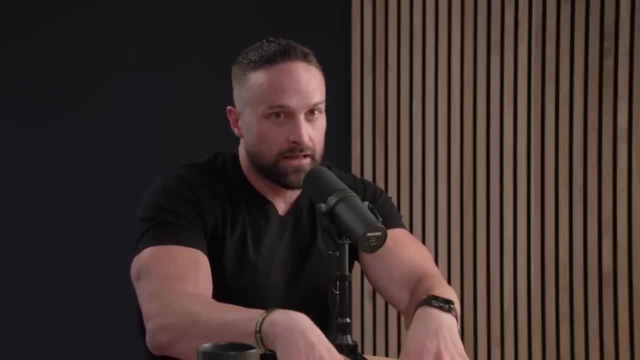 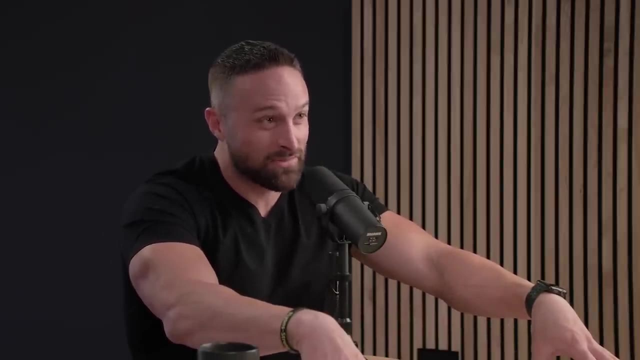 the reason you tend to lose weight is originally like: good luck, you know, 10 years ago, doing a keto diet, eating processed food, right, Like you just couldn't do it. really now you can, but the problem is it's not going to work because you're going to be still consuming too many calories. 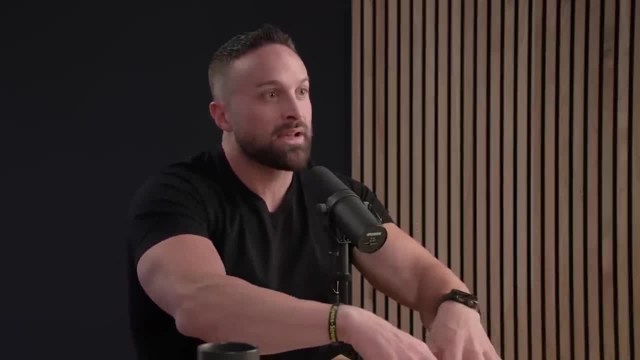 Because, even though it's keto, what are they doing? Well, they're trying to make it more palatable, They're trying to make a better mouth feel, which, I guess, if you're being keto for the sake of being keto, great. 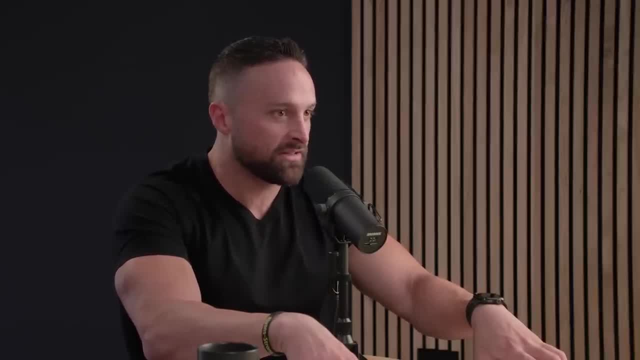 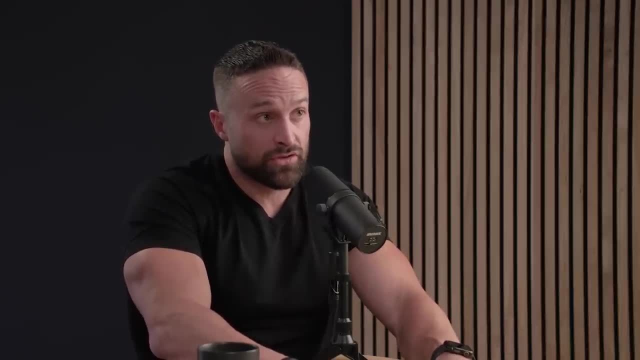 But if there's, if you have hopes of body composition modification, it's going to really negatively impact. So, yes, I think minimizing the amount of processed foods you consume can be important. Now, that being said, it depends on the individual and their goals. 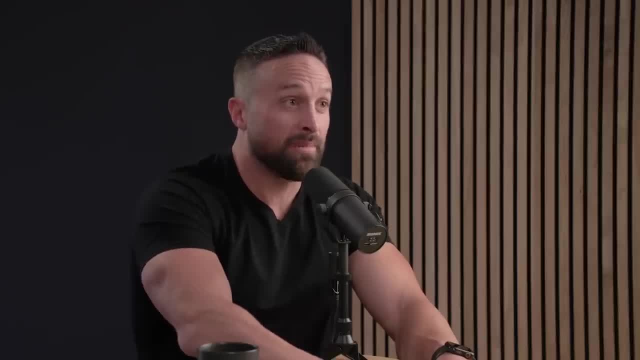 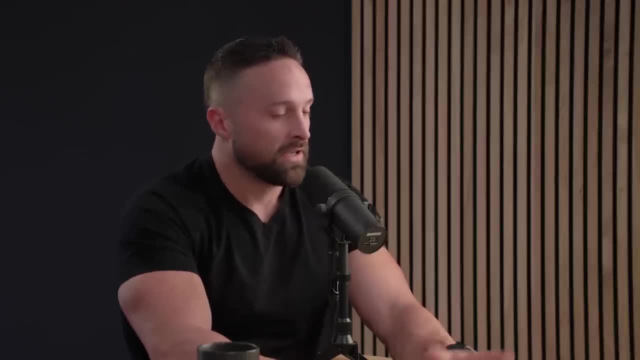 If your goal is to, for example, build muscle or maintain a high body weight for a sport, for example, like an NFL offensive lineman or something of that nature, or if you're. you know, I worked with an NBA team and they were kind of. 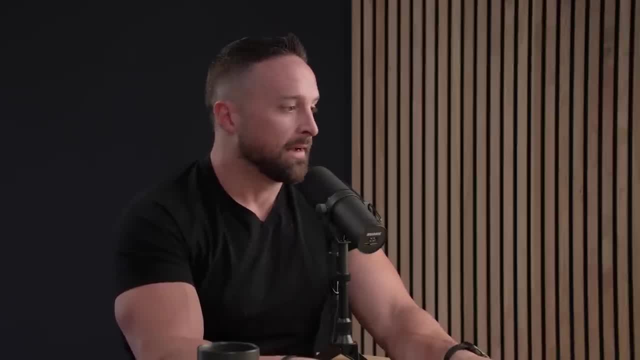 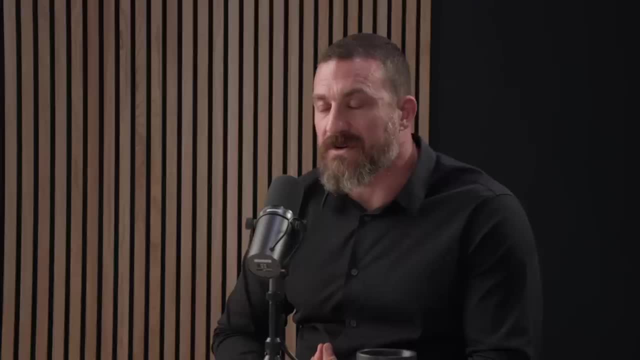 I can't disclose anything but they. they were looking at drafting a certain player and you know like, for them, processed foods may actually be a tool, or teenagers Right, And we all want young people to eat more healthfully, I think, develop great habits. 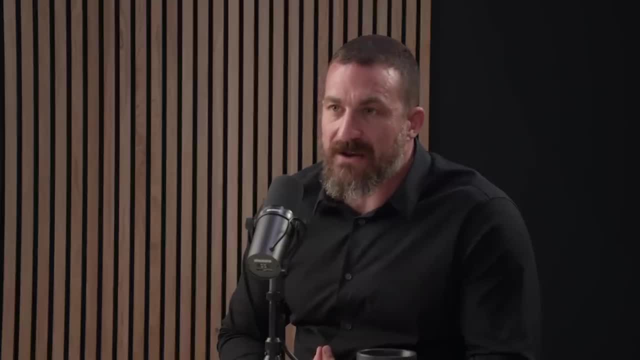 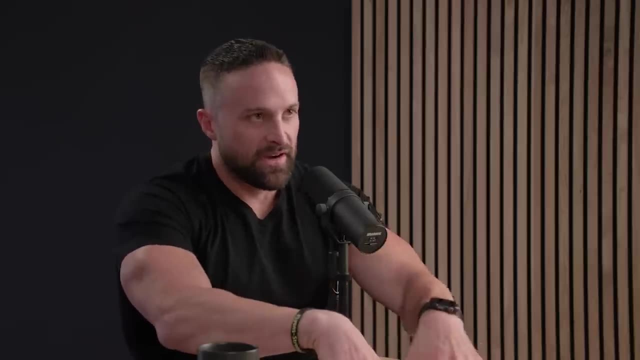 but some of them, their caloric needs are so high, so high that if they were eating what I eat, they're going to dissolve into a you know, they're just waste away. So I I described this again with a financial example. 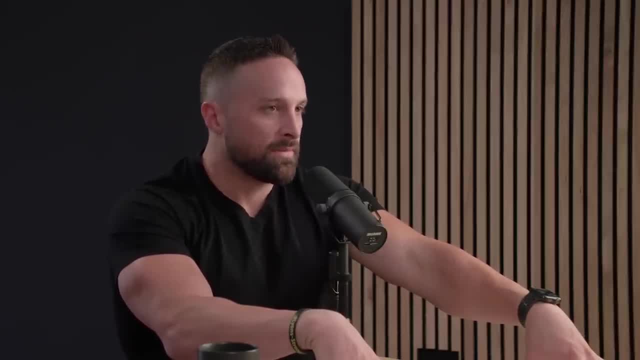 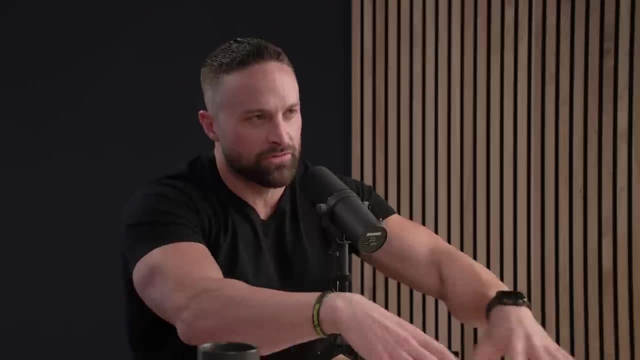 It's like a budget, right? So if I make a million dollars a year, for example, is it okay for me to buy, like, a $100,000 sports car? Let's assume that loans don't exist, right? Is it okay for me to buy a $100,000 sports car if I? 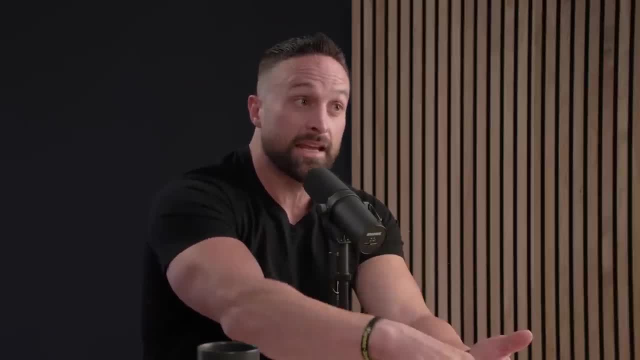 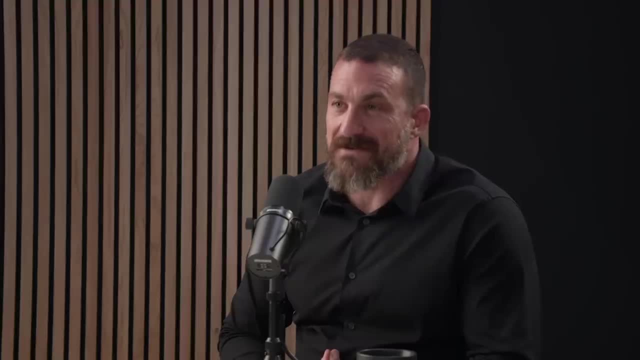 still am able to pay my mortgage and pay my utilities and like take care of my responsibilities, the things I should do. Is it okay if I do that? If it like makes me feel good and it's fun by me, Yeah, it's fine. 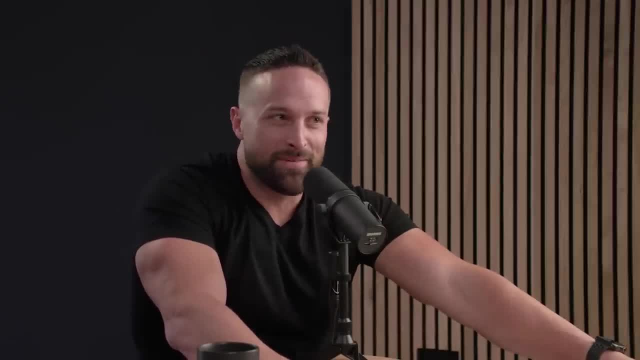 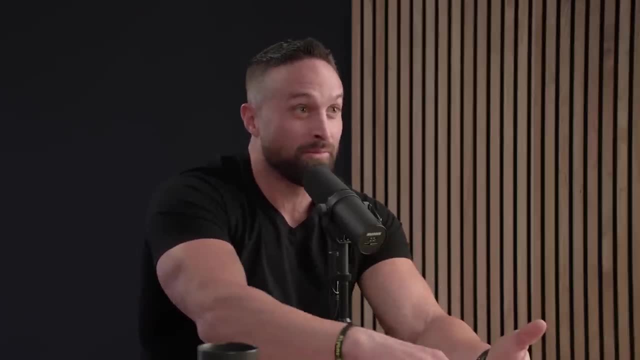 Right, Like it fits in your budget. If my, if I have, if I make you know, 50 grand a year, should I be going out and buying a sports car? Probably not, because I'm not going to be able to pay my. 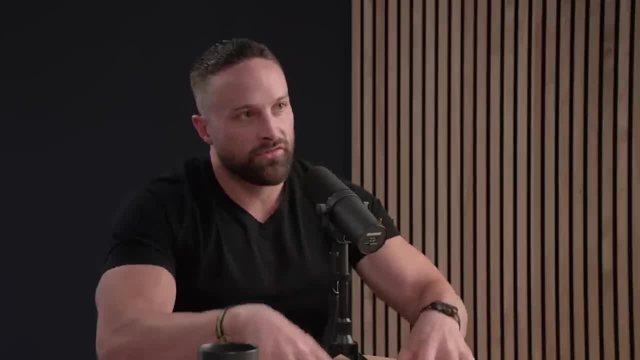 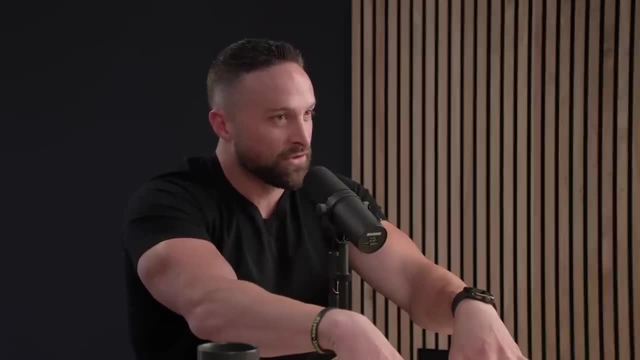 mortgage and all these other responsibilities. So your, your protein, your fiber, your micronutrients, these are your responsibilities, but those become much easier to hit when you have higher calories, right? So, if you're, if you're, you know. eating 4,000 calories a day. for whatever goal you have, you're probably going to have some leftover and, like good luck, eating 4,000 calories from minimally processed foods. You, quite frankly, you'll be miserable Because you're. 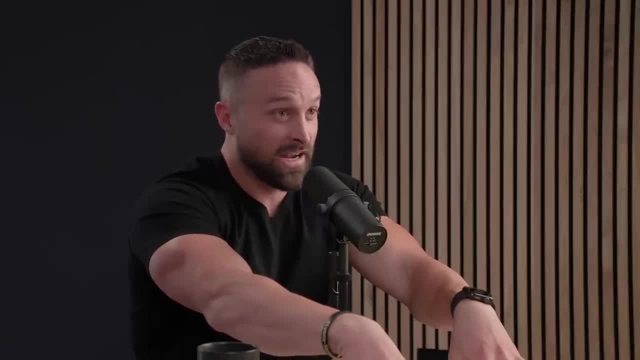 you're going to have such gut fill that you're going to feel like you can't even move, And so again, now it becomes okay. Well, is there something inherent to that food processing? Is there something you know that we can pick out, that we know? 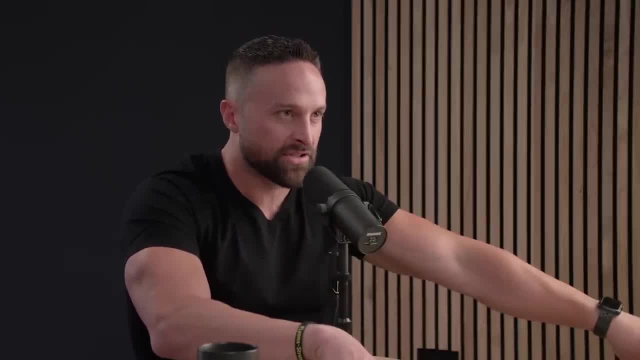 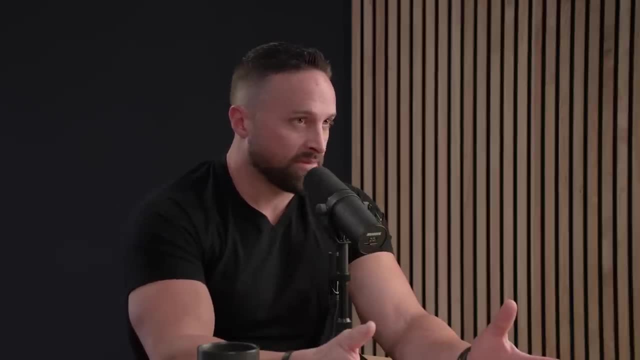 okay. well, this is going to be a negative effect on health, even like body composition stuff aside, And I would say there's not really great evidence of that so far, And a great example of that is sugar. I mean, I actually just wrote a really long article. 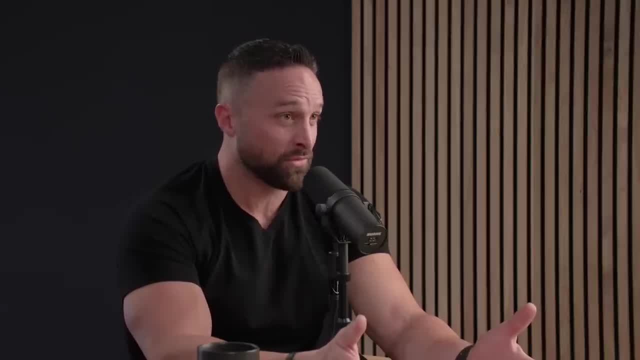 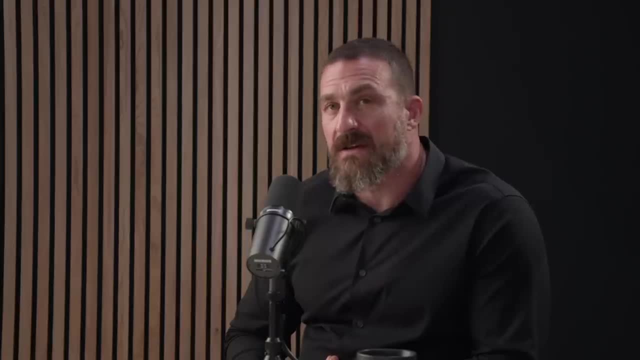 article on my website about why I think sugar was not the root cause of the obesity epidemic. And you kind of mentioned, like sugar intake in the last 20 years has actually gone down a little bit Alcohol intake. Well, if you look on the whole, 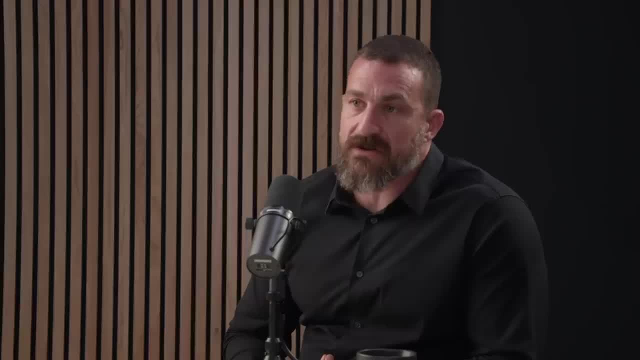 it might've gone up a little bit, but it you know certain in, certainly in the male sector, it's gone way down. drinking used to be- there was a five o'clock, people drinking all day. People were smoking a lot less. 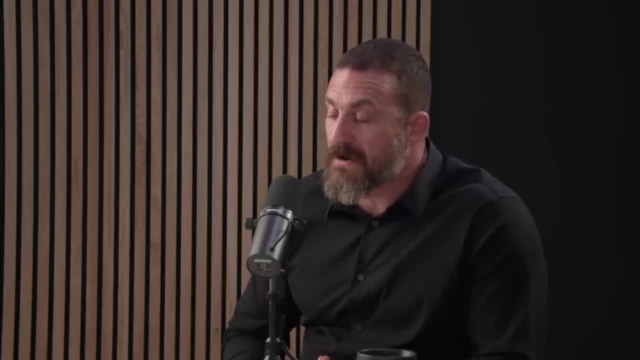 There. I think it's a real puzzle. I'd love to know what your um hypothesis is: Actually be an opposite opposition, because nicotine is actually an appetite suppressant and also increases focus. The problem is it often arrives in a delivery device that can kill you. 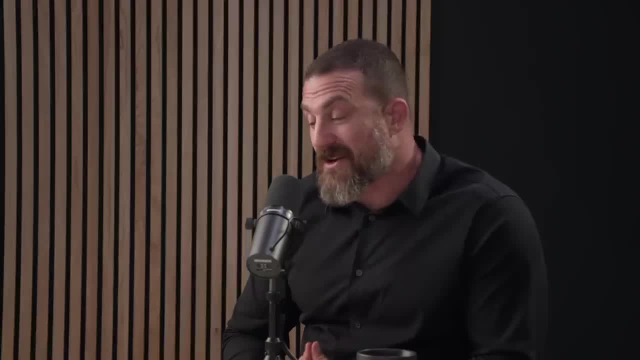 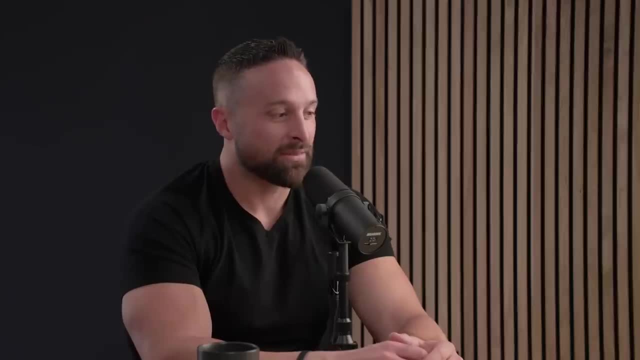 But nicotine itself is a powerful agent. It also can offset age related cognitive decline- not entirely, but it's. it makes the brain work better. I've got a buddy who doesn't like caffeine and he just takes those nicotine pouches and like basically has one in almost all day because he's a 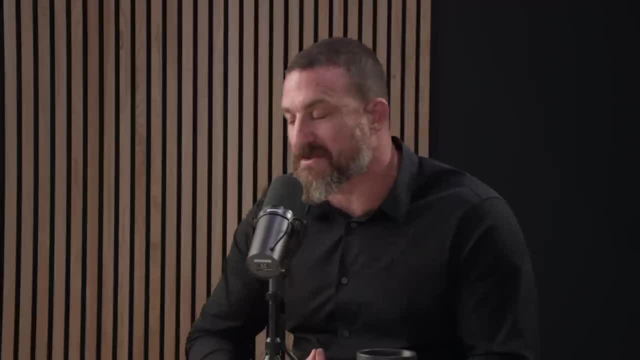 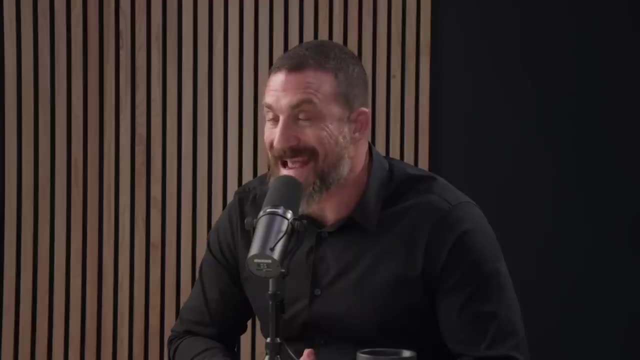 like a. he has a very stressful job and as a high performer you know you have to be careful how you deliver it. But there's a Nobel prize winning neuroscientists that will chew five or six pieces of Nicorette an hour. 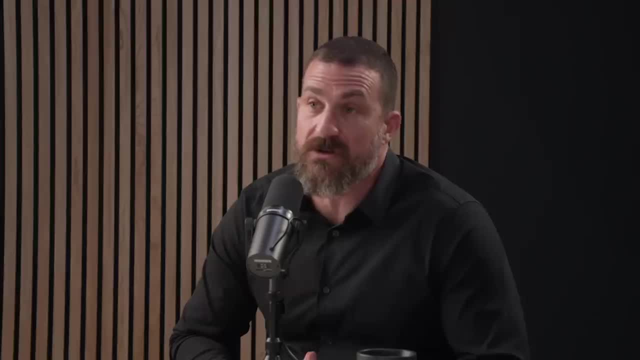 which I do not recommend, And but when he quit smoking he just simply couldn't function as well. And he was the one who pointed me to the literature on offsetting age related cognitive decline, even neuron maintenance, And it's pretty interesting. 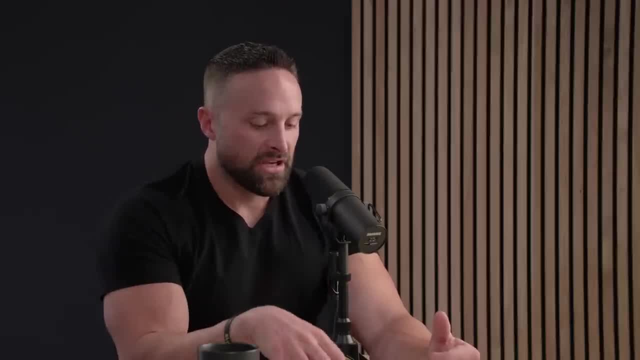 Well, it's a pretty. it's a pretty impressive nootropic, to be honest. Um, so now the first thing to realize is, when we're talking about consumption data, this is based on actual production. Basically, they're assuming that, okay. 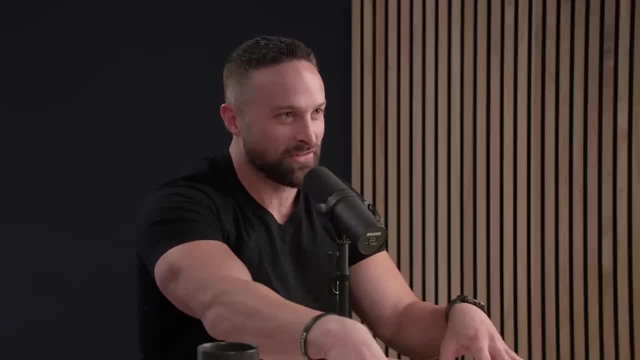 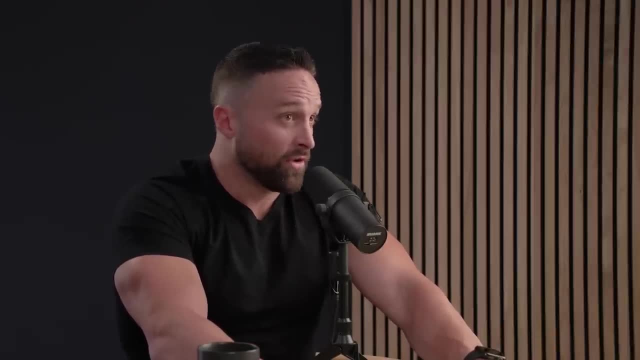 we're producing this amount of these foods, So we can assume the consumption is going to follow that. So it's not a direct measurement, uh, but it has been validated in a few different studies. We know that oil consumption has gone up like that. 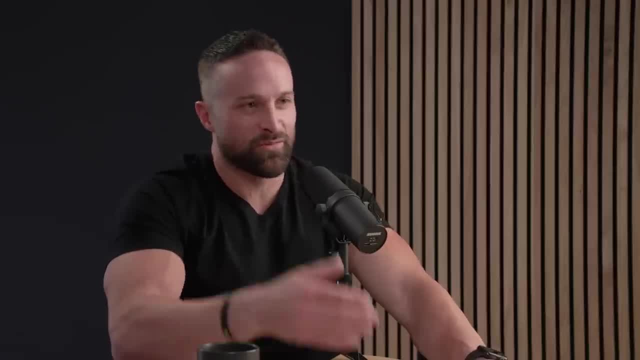 That's, that's, that's, yeah, that's one of the big ones is, and this kind of forms, the crux of like the. the seed oils are, like, the root of the question that I'm going to. they're going to. 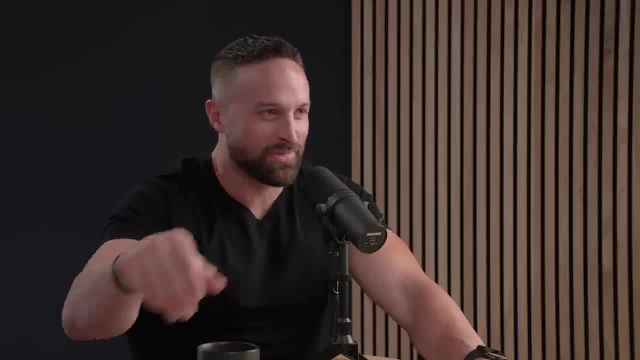 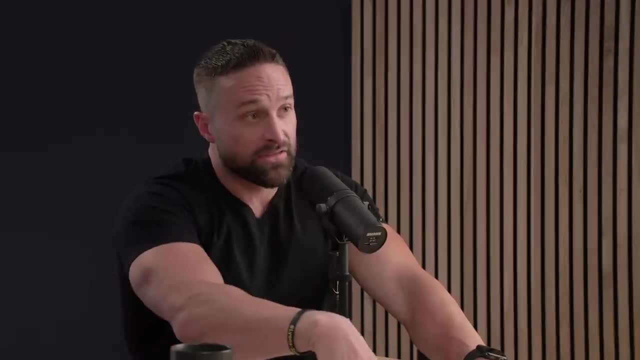 you know, come into your house and kick your dog and, you know, punch your mom and all kinds of stuff. Uh, and I'm happy to address those. But um, so calories have still gone up. Uh, there's. 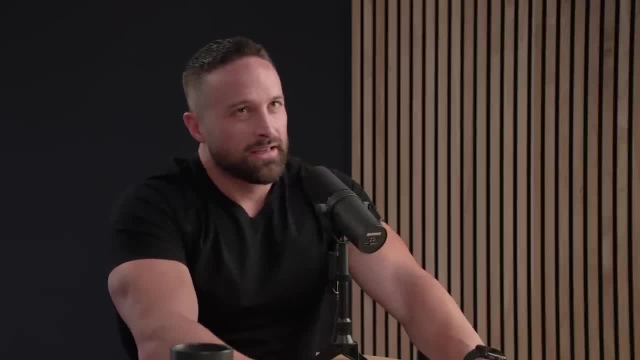 there's some people who claim that they've gone, they've kind of plateaued. I think the data seems to suggest that calorie intake is still increasing. And the other thing to keep in mind is, even if it's plateaued, it's still at a high enough level that obesity is probably going to continue to. 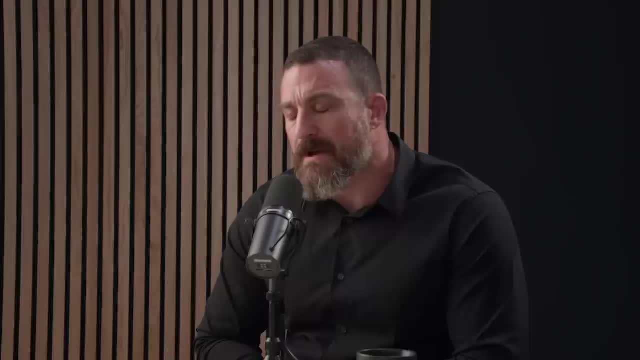 increase up to a point where it'll probably plateau. if calories are plateaued, What about energy output? Um, leaving aside neat, because that sounds highly individual, I mean, people are the people we know are focusing on exercise, but there are a lot of folks out there that don't exercise and 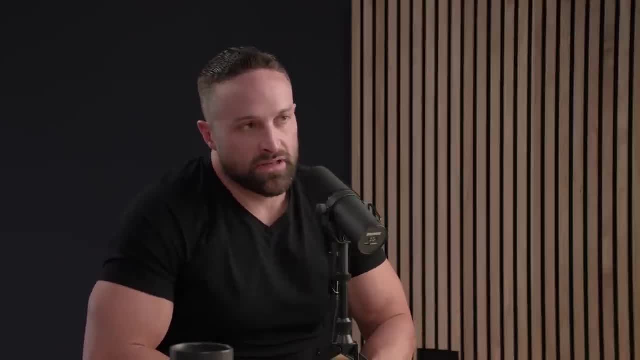 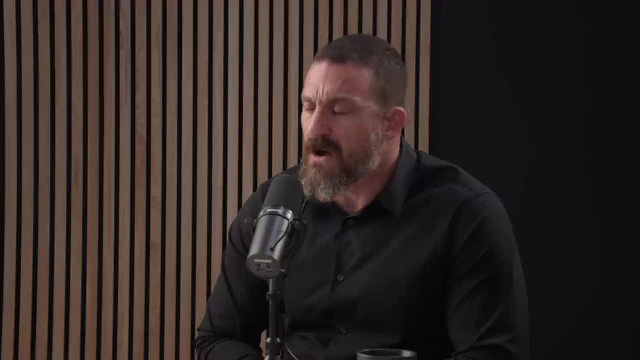 and and energy output has gone down over the years. I mean it's very obvious when you look at how people work now compared to even, you know, 30,, 40 years ago, it's, it's much different: less walking. 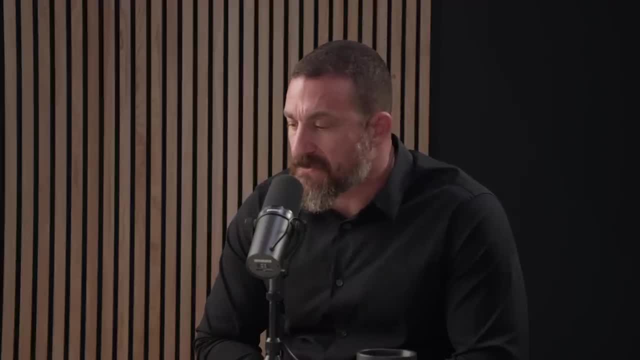 Also, I learned recently that um kids in high school don't take PE class. in many schools We had to suit up and run And suit up And if you didn't bring your change of clothes or you didn't wash them, 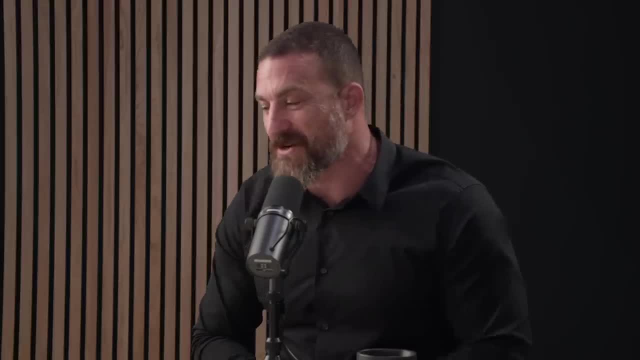 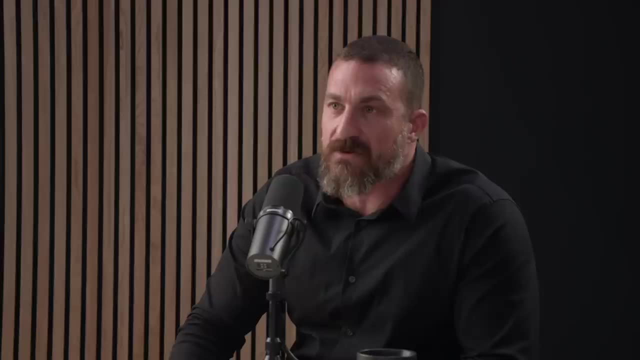 in which case you'd be better off just not wearing. uh, nothing like the smell of a boy's locker room after a weekend, you know, I can still remember it And it's not, um, it's not pleasant, but you had to run and do your pushups with everybody else or play volleyball. 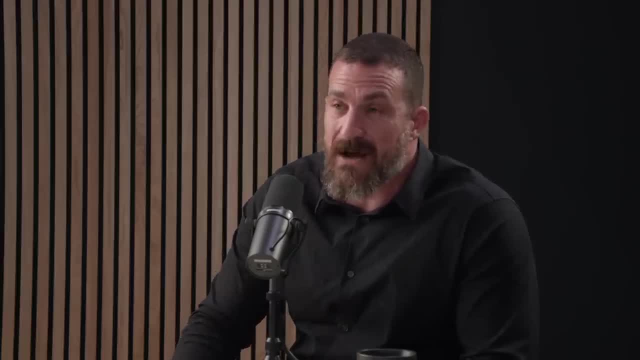 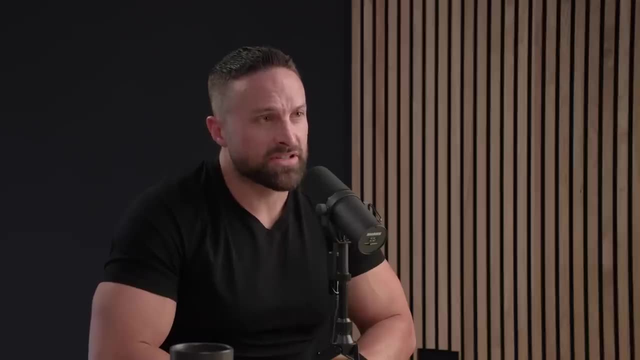 in your in your regular school day clothes, So that I my understanding is that physical education is not part of the basic education any longer. Uh, probably depends on the state, but I know many states have done away with it just because of. 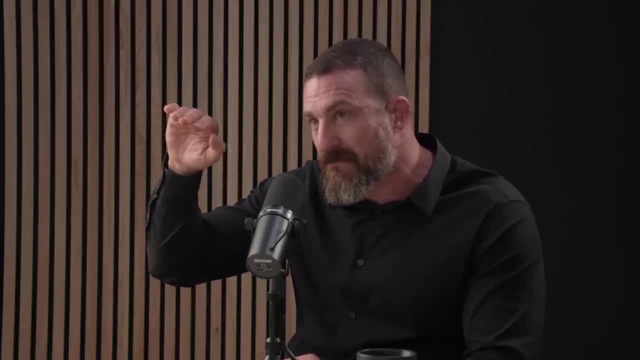 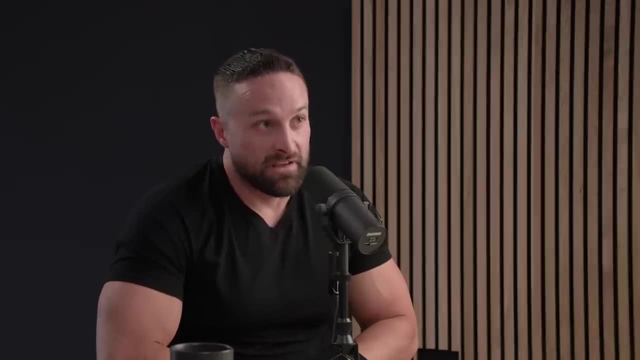 of budget cuts. So activity is going down, Caloric intake is going up, maybe plateauing, maybe plateauing. Is that sufficient to explain the obesity epidemic? Uh, based on what I've seen, I, I, I think it's pretty sufficient. 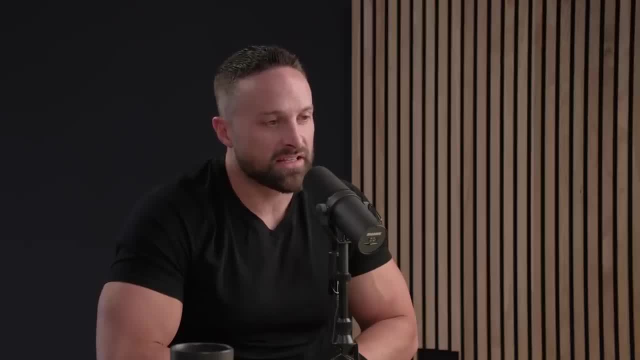 So it might not be that big of a mystery after all. No, I don't think it's a big mystery. I think that, um, people don't like the concept of energy balance, And I think because they insert judgment into it. 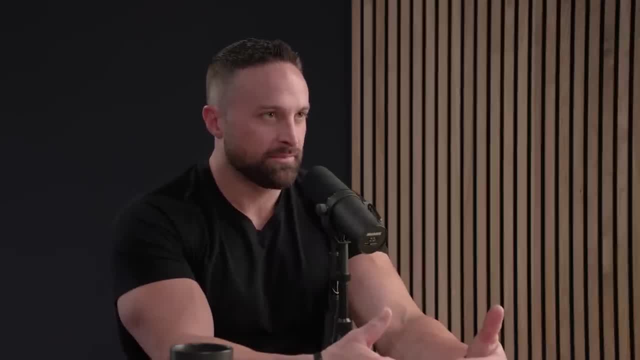 which is okay If you're gaining weight over time. at a fundamental level, it means you are eating. you're consuming more energy than you're expending. People insert the judgment which is: you're lazy, You're a sloth. 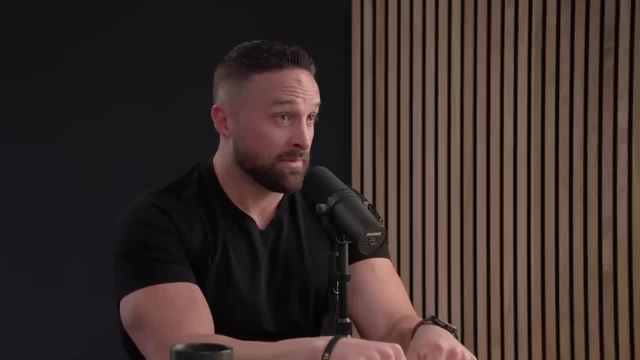 You're, whatever it is, And I think there's a lot of people out there who actually think that I- I actually remember talking to somebody who was like, well, I would never hire an obese person for a job, because it's just obvious that. 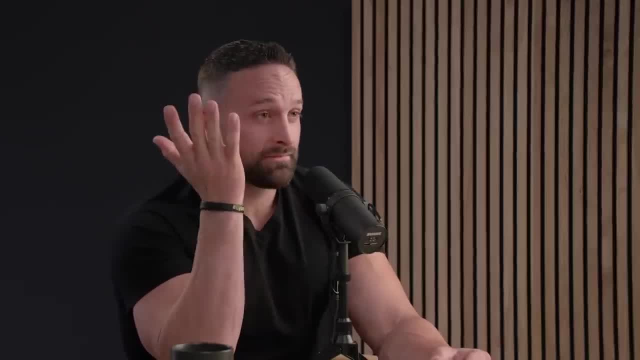 they're lazy And I just remembered going out. Are you serious Like there are plenty of very, very smart, high achieving people who are obese right, Like it's not. this is what happens when you just put people in buckets. 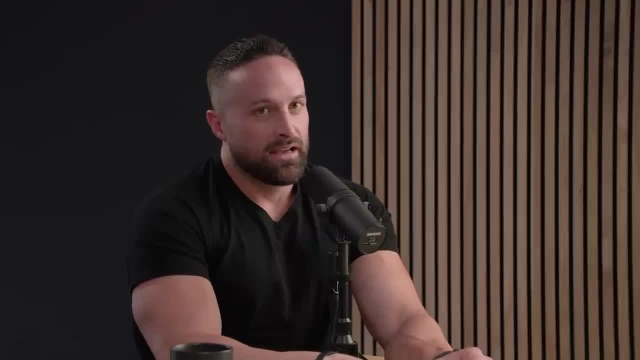 you know like people are much more complicated than this. Yes, there is, there is some personal responsibility, but then when you look through the data and you like take a. there was a study done in obese women where they found that women who were obese were 50% more likely to have had some form of sexual assault trauma in their past. Right, Um, we know that people from lower income areas are more prone to be obese. Um, there's several like people who have a higher ACE score. 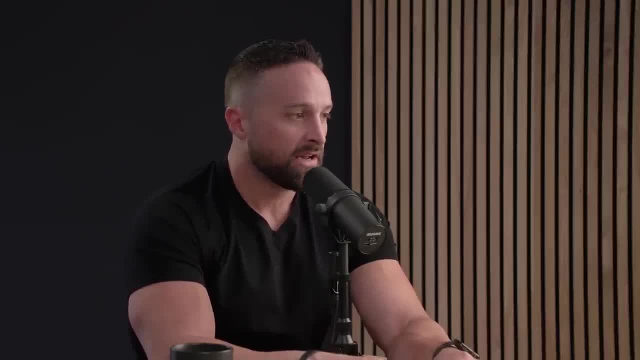 I believe, which is kind of measures like traumatic childhood events. I believe there there was a study showing they're more likely to be obese. So there's, yes, it is an energy imbalance problem, but you know, just saying eat less. 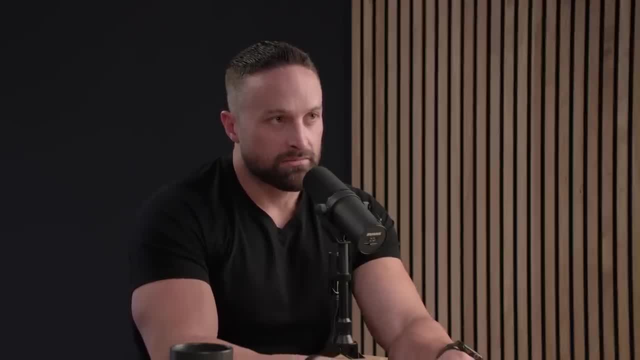 move more. That's like telling broke people: we'll just earn more money than you spend. It's technically right, but it's very unhelpful, right? Well, what is more helpful is to describe and implement the habits and behaviors that will allow them to achieve that. 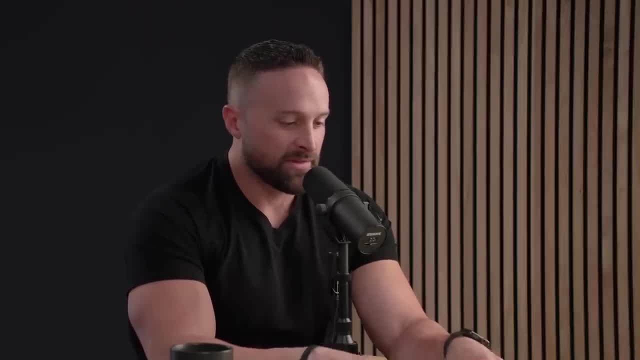 Right. So kind of I realized we kind of got off track a little bit. but circling back to like sugar, circa 2005, I believe that sugar was fattening and bad for your health, independent of any other variable. So independent risk factor. 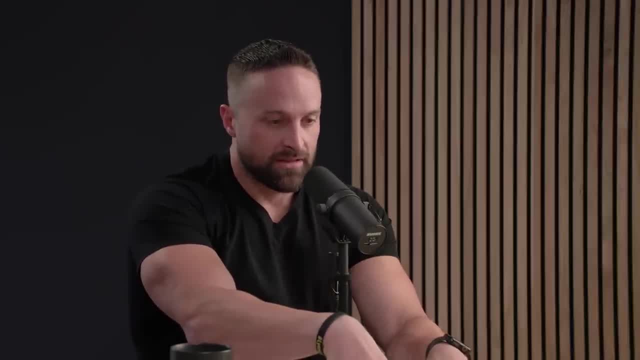 And again I want to be very clear about what independent means. Independent means independent of all of the variables. this thing is bad for your health and body composition. So on its own, independent of whether or not, for instance, it increases hunger and appetite, 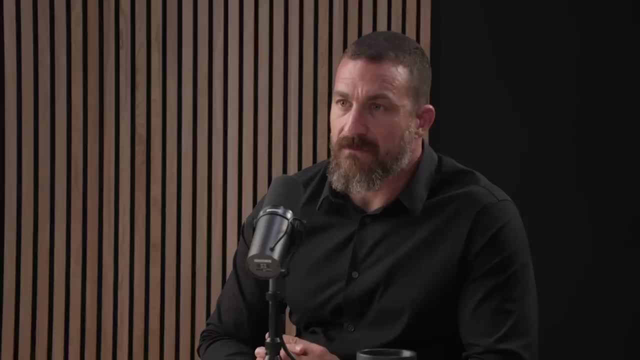 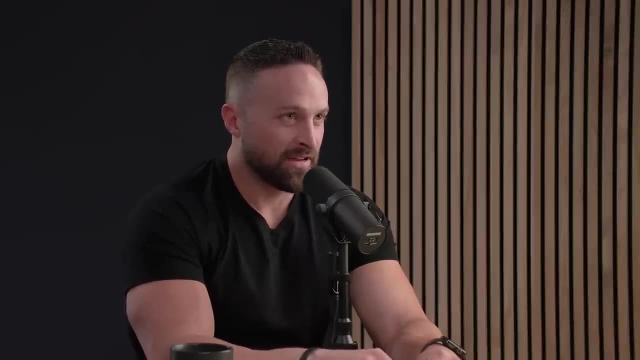 right, Or or caloric intake right. I was at a graduate school mixer and one of the professors there was somebody who had done research on high fructose, corn syrup and fructose specifically as well, And he was talking to another professor and he had done this study in. 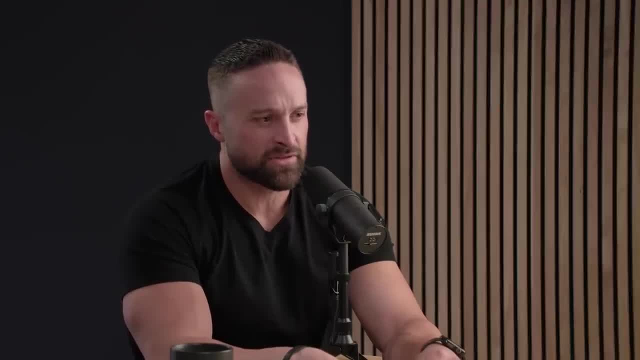 um rodents where he'd fed like a I think it was like 60 or 70% of their calories from fructose, And they saw some really weird things happen in the liver with the novel lipogenesis and all this kind of stuff. 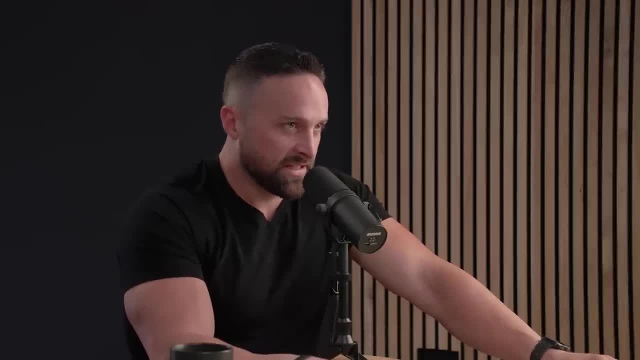 And the other professor is saying to him: yeah, it's pretty obvious that high fructose corn syrup is, you know, fattening. And this professor who had done this research said, yeah, because it's people overeat. And he's like: 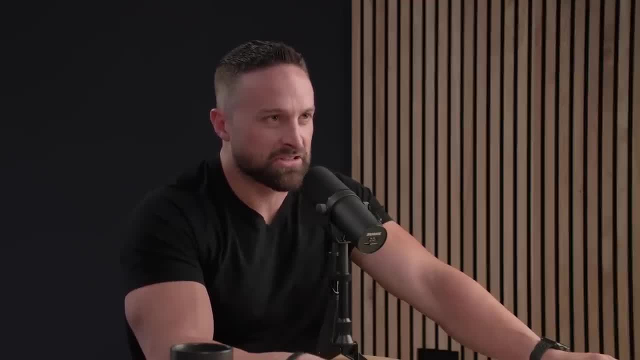 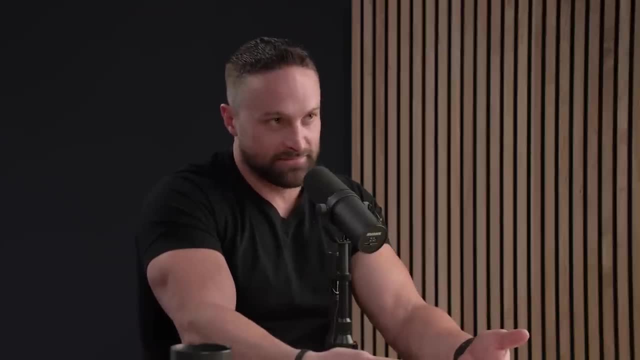 don't you think there's something inherent to it? And he said: no, I think it's just calories, You were eating too many calories. He's like we. we did a proof of concept Looking at you know, could we like try eating 70% of your daily calories from fructose? You actually can't do it. Like high fructose corn syrup is only 55% fructose, So if you ate nothing but high fructose corn syrup, you would still not get to this level that they fed in this study. So that got me kind of like questioning my beliefs about it. 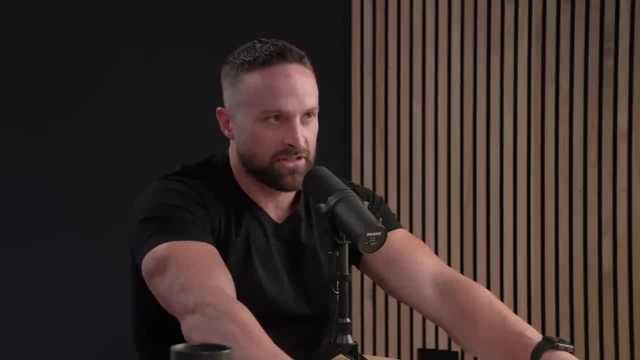 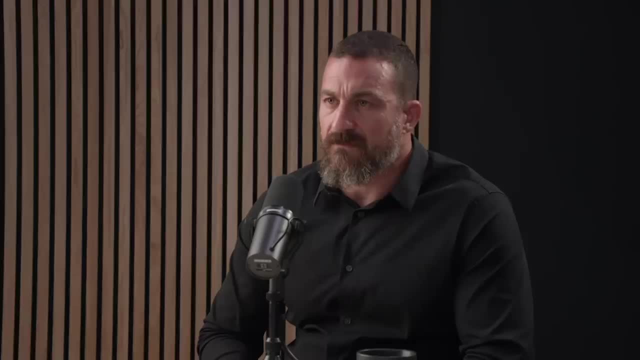 So then I went through and I said, okay, like let's take out the epidemiology. Not that epidemiology is useless, but people who eat more sugar are also likely to eat more calories. So then I looked for the randomized control trials, where they 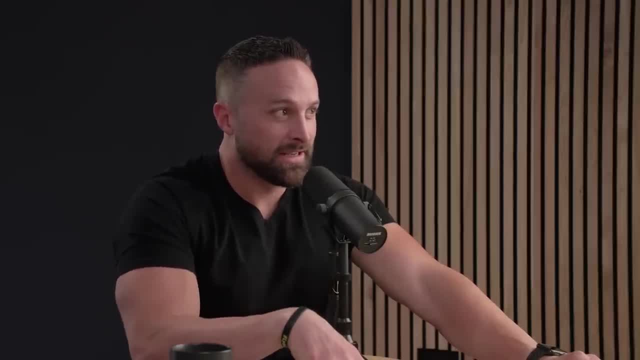 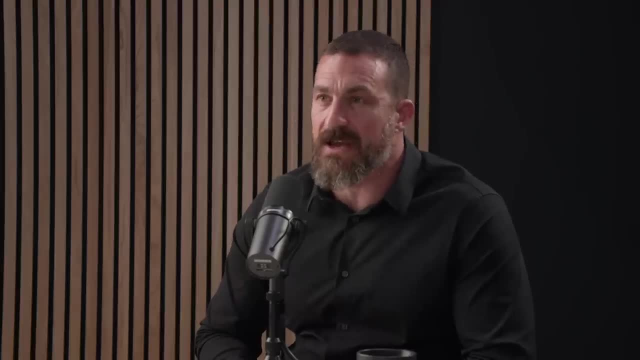 you know, match calories and vary the amount of sugar, And it doesn't seem to make a difference, at least from fat loss or fat gain. But what about health? So, for instance, if somebody- and I know somebody like this- who loves sweets, is thin, 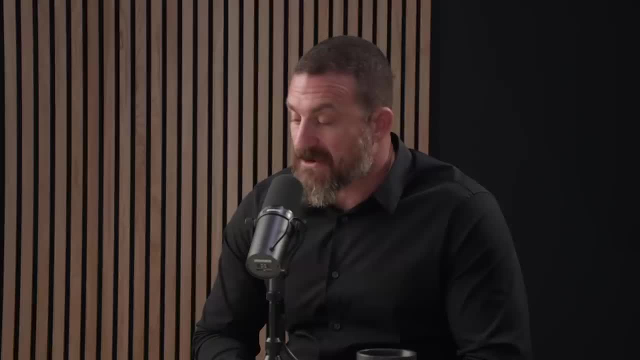 get some exercise, not a ton- But my concern is that a significant fraction of their calories are coming from these sugary foods and therefore they're not getting enough fiber Right, Maybe protein, et cetera. So let's look at epidemiology for a second. 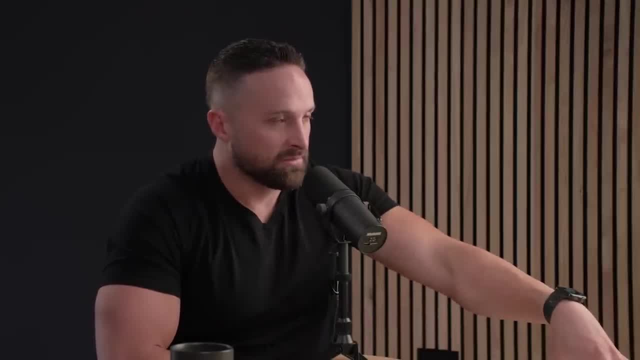 Then I'll address this more directly. When we look at epidemiology, people who eat higher amounts of sugar tend to be more obese. They tend to have worse biomarkers of health. but people who eat fruit, a lot of fruit sugar, don't have those same associations. 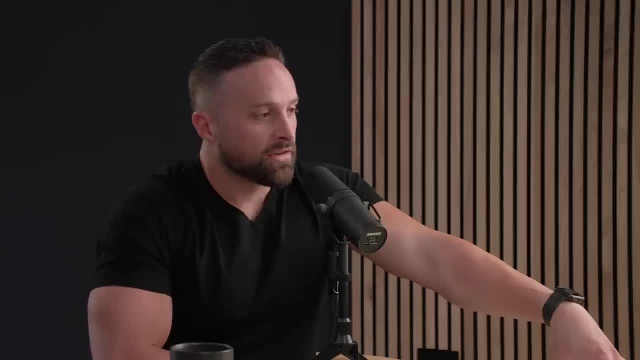 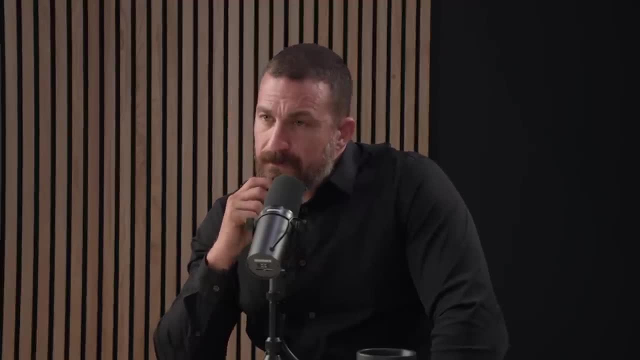 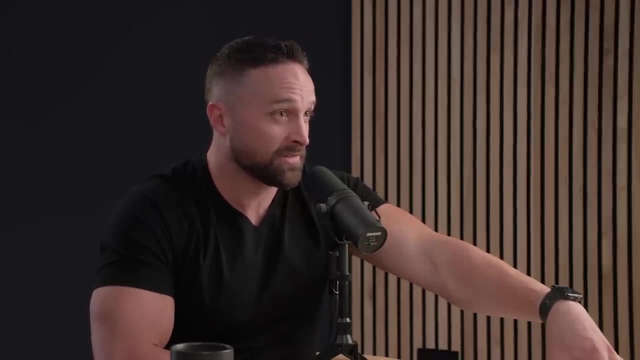 So why is that? Well, because fruit has fiber with it, right? So I started to kind of I believe, based on the data I was looking at, that high sugar intake was not the problem per se. The problem was that high sugary foods typically are very low in fiber. 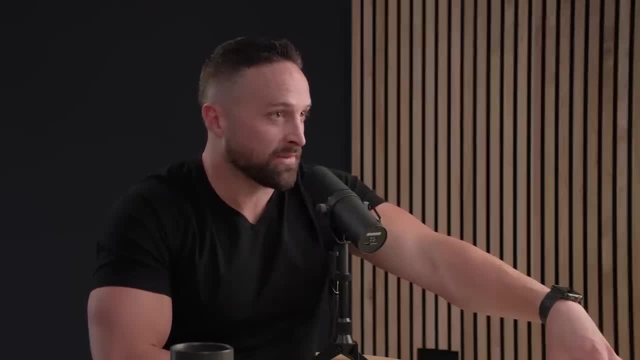 But if you're getting enough fiber, is sugar a problem. So there was a classic study by Surwit in 1997.. I think it's still the best study to this day. looking at this, And I know there's people say well. 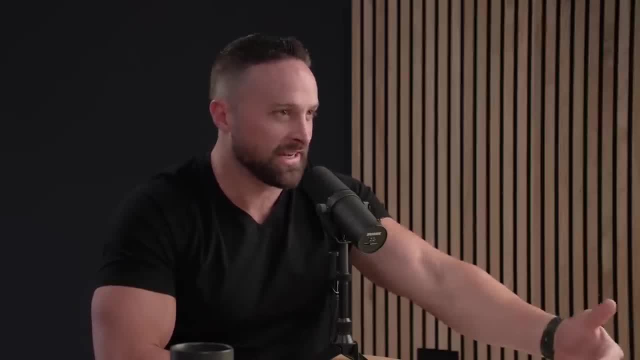 it was done in 1997.. It has no relevance. You know, I know if it's a good study, it's a good study. Some studies are timeless. In fact they have. they're not going to go back and undo the discovery of DNA. 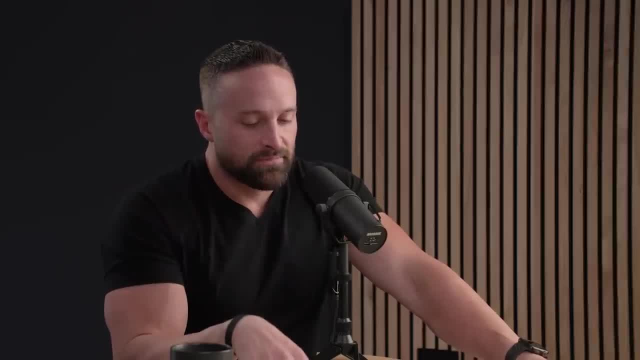 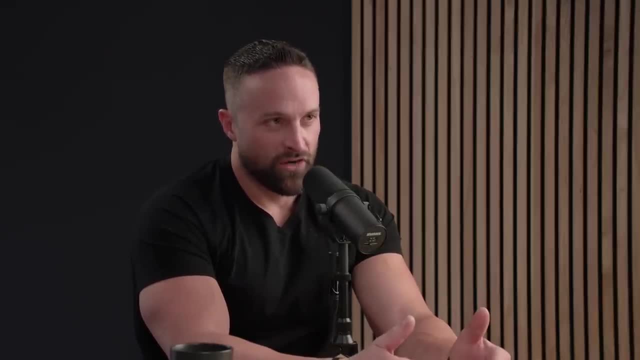 Cause it was, you know, 60 years ago or whatever it is now. So they, they looked at an 1100 calorie diet, So low calorie diet. one group was eating over 110 grams of sugar a day like sucrose. 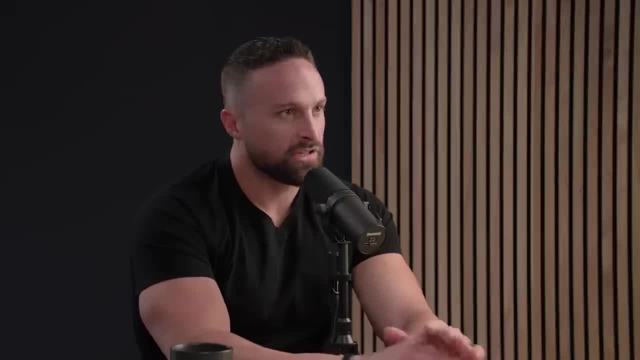 The other group was eating about 10 grams of sugar per day. calories, protein, carbs, fats- all matched right And they provided all the meals to these participants. So very tightly controlled, And it was over six weeks. both groups lost the exact same amount of body fat. 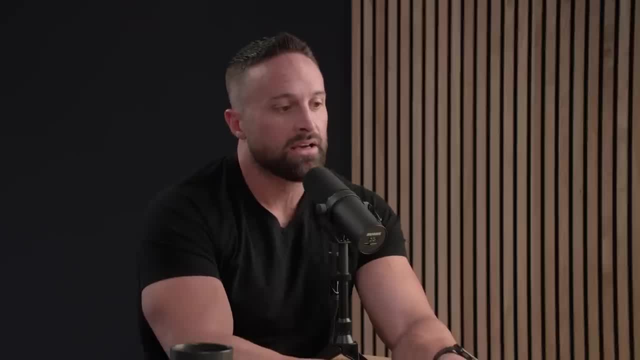 So it doesn't seem to matter for body composition in terms of like sugar per se. Then they also looked at some biomarkers of health like blood lipids and blood sugar and some other things. Again, there was no real differences. The only difference was: so all their biomarkers improved in both groups. The only real difference was a small difference in LDL. So the group eating low sugar had a better improvement slightly in LDL And but that's probably because they were eating more fiber and we know fiber can bind to cholesterol and lower LDL cholesterol. 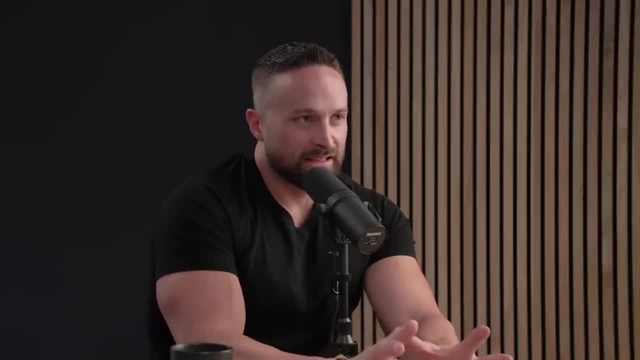 So is now I want to. I want to caveat: this sugar probably doesn't have any like positive health effects. So there's that, right. And? and nutrition is an exchange. If you're eating one thing, you're not eating another thing. 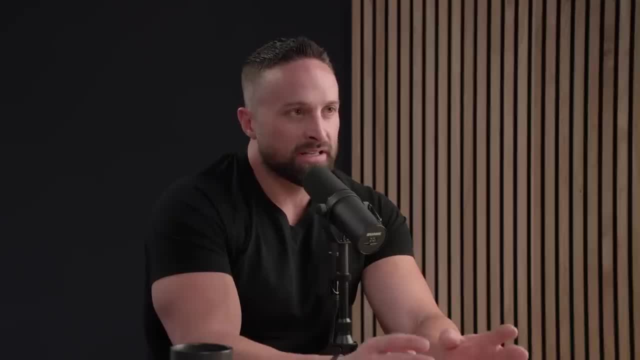 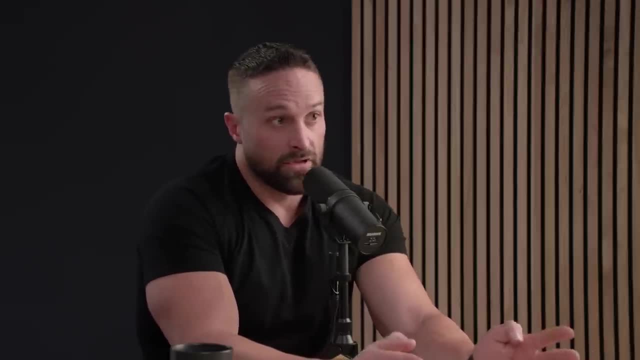 right, So I. but what I would tell people is: focus probably less on sugar, focus more on fiber. So if you're eating 30,, 40,, 50, 60 grams of fiber a day, but your sugar is, you know, 80, 90 grams, I would not be that worried about it, especially if you're controlling calories as well. You know, what I would be worried about is if you're eating, you know, just a decent amount of calories and not getting enough fiber and in. 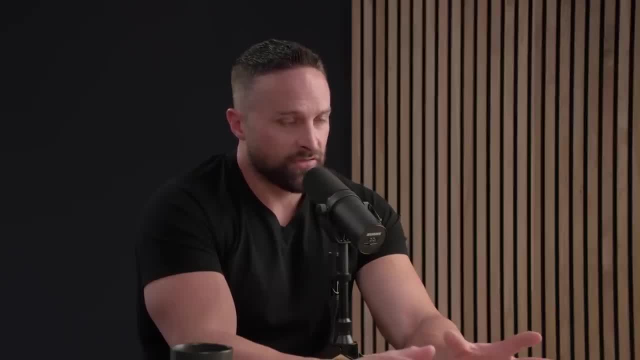 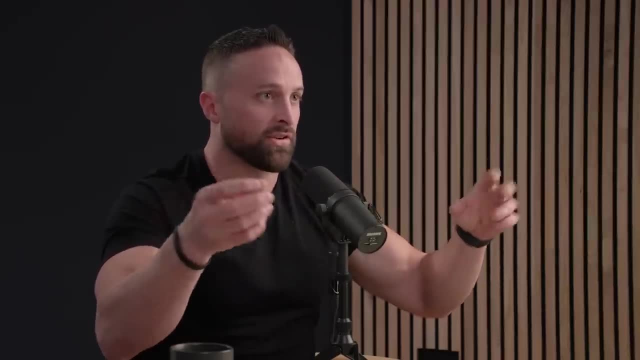 general right And even in studies. there's a few meta-analyses out now looking at ISO energetic exchange of different carbohydrates with sugar carbohydrates, So fructose, and glucose and sucrose. Now why is this important? Well, again. 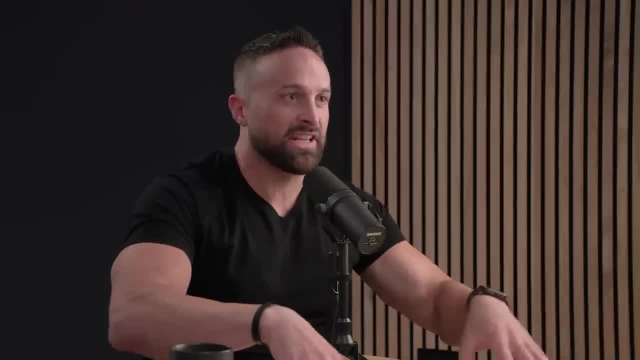 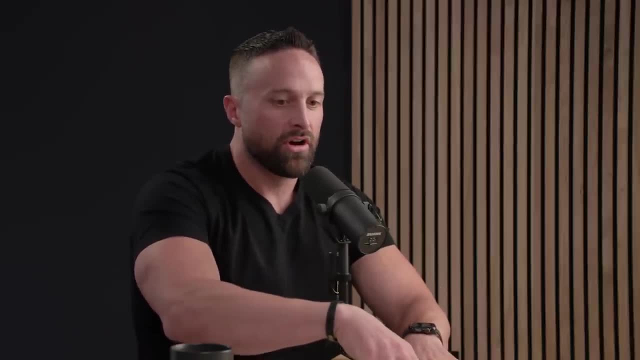 you know if you're not equate. when I say ISO energetic, that means equal in energy, equal in calories. So basically, when they exchange either sucrose or glucose or fructose for other forms of carbohydrate, do they see differences in these markers of health like HPA? 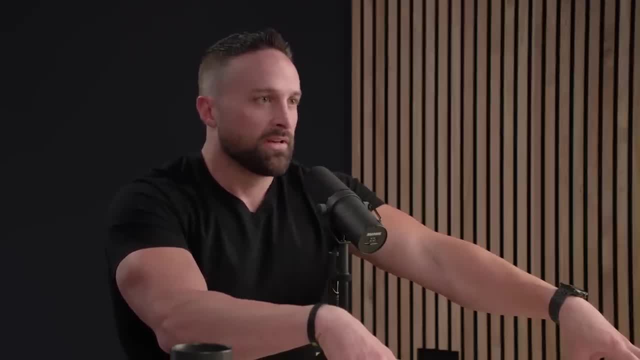 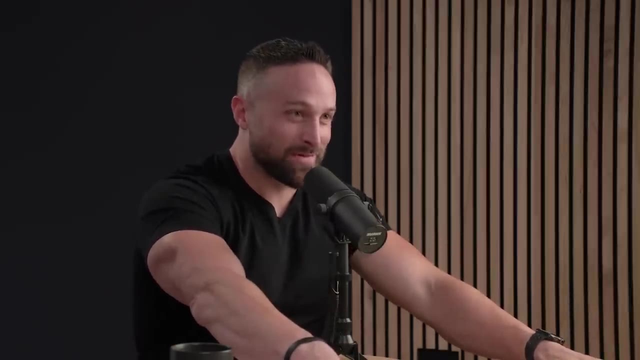 one C, fasting blood glucose, you know, blood lipids, and, with rare exceptions, and I can't remember all the data points exactly, but the take home is doesn't really seem to make a difference. Now, before anybody out there straw man's my argument. 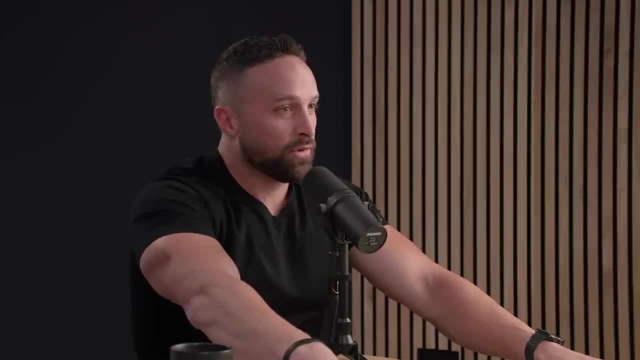 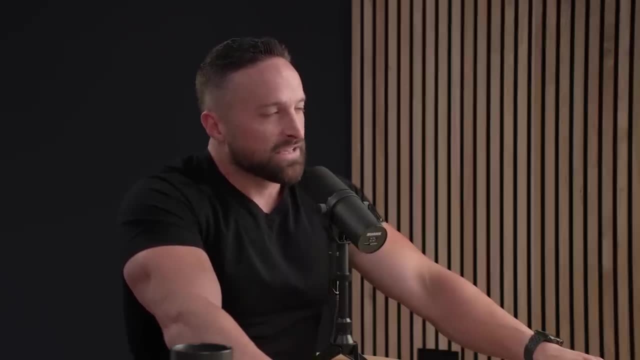 I am not advocating for sugar consumption, but I think it's important for people to not create weird associations in their minds, Because one of the things I've observed, especially in the fitness industry, is when people feel like they can't eat something, like it's one thing. 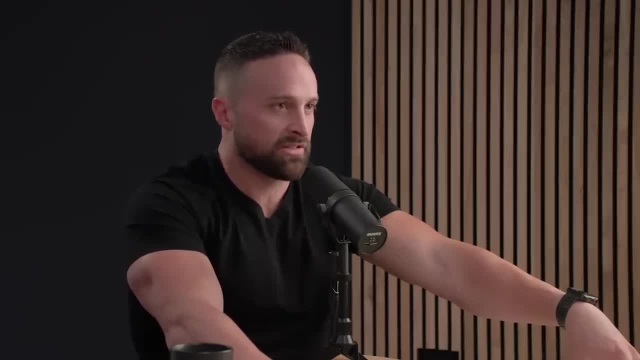 If you say: I am choosing not to eat this just because I'm choosing to. but it's a very different thing when you're purposely restricting because you feel like something is bad. And this- this I mean, you know, the human brain- is in many ways amazing, in many ways. 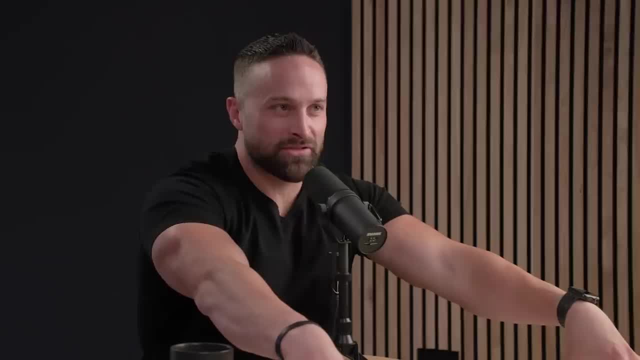 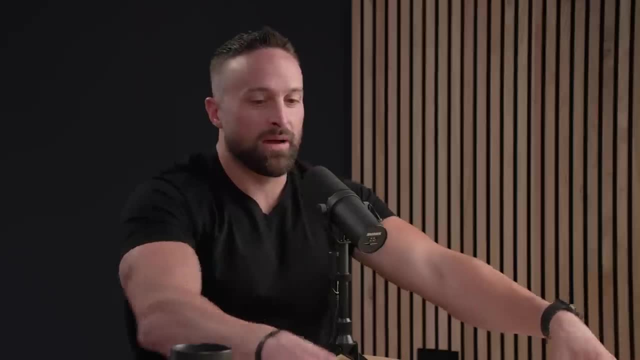 really dumb. Um, so, when you purposely try to restrict something, what tends to happen is you're more prone to binge on it. So people who will try to? well, I'm never going to eat sugar again, or I'm going to try and limit sugar. 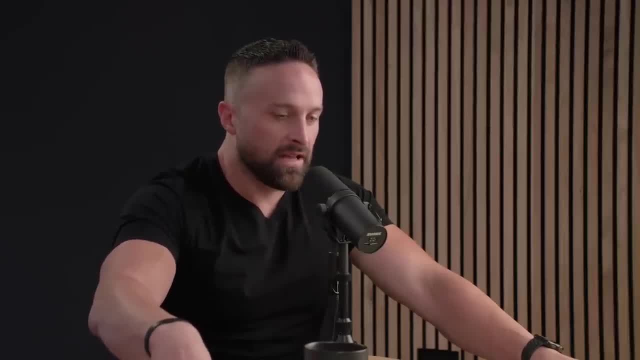 And this isn't the case for everybody, but they have actually shown now in studies- people who are purposely restricting a specific nutrient, they tend to crave more of that nutrient And if they do get exposed to it they're more likely to have what's called a disinhibition reflex. 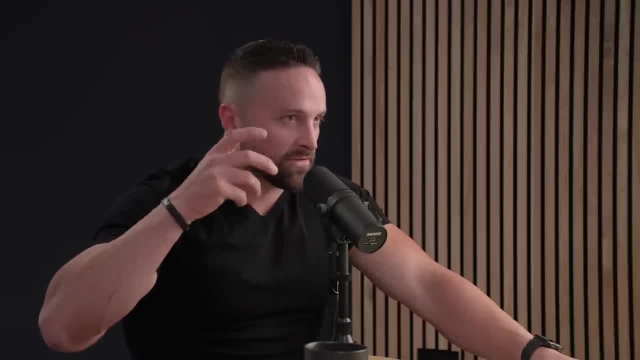 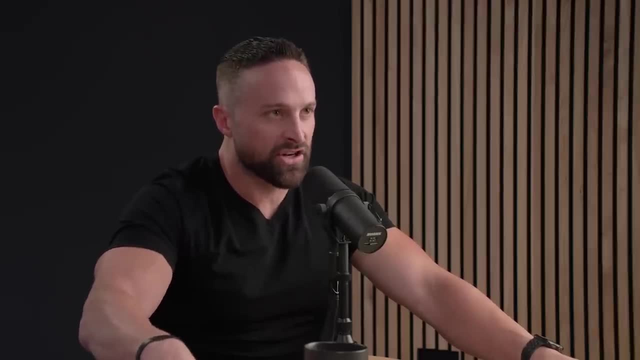 which is basically a binge response because the thinking goes: well, this is bad Any, and there's no context on you know dosage making the poison. This is just bad in general. So if I have it, I've already screwed up. 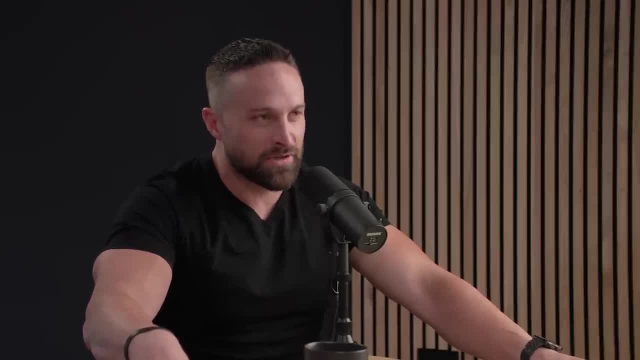 I might as well just have as much as I want, And I like Spencer Nadolsky's comparison. This is: you know, that's like you know getting a flat and then going out and slashing your other three tires because 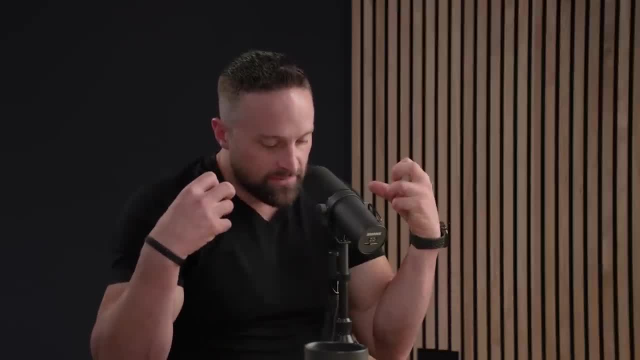 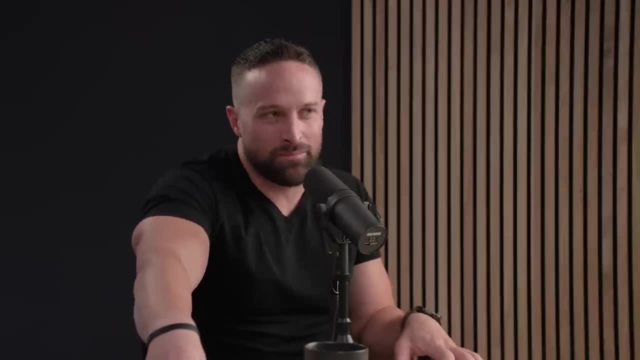 you know you might as well. So I really I try to come from that perspective of I've seen so many people struggle with, you know, maybe not an eating disorder but disordered eating patterns because of these kind of associations they've. 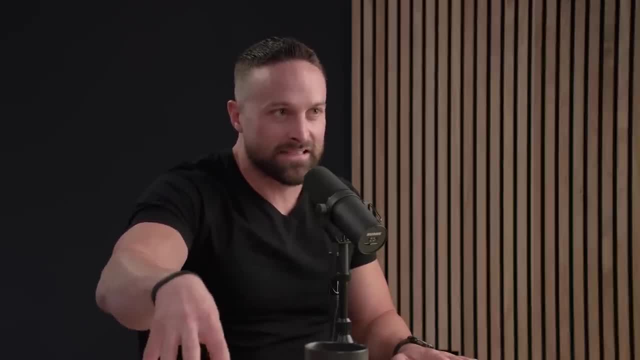 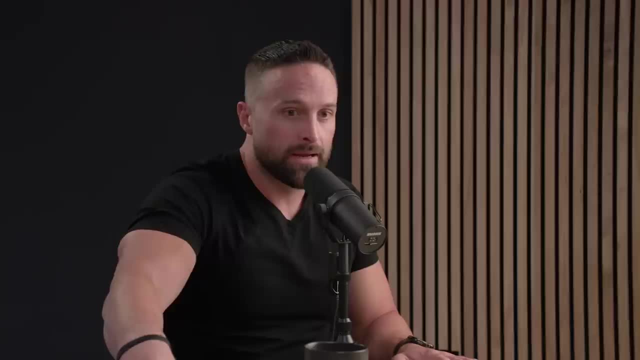 made in their mind, And so that's why I'm so pedantic and a stickler about saying: okay, yes, it's a good idea to eat mentally processed food And try to avoid processed foods, but not because processed foods are bad per se. 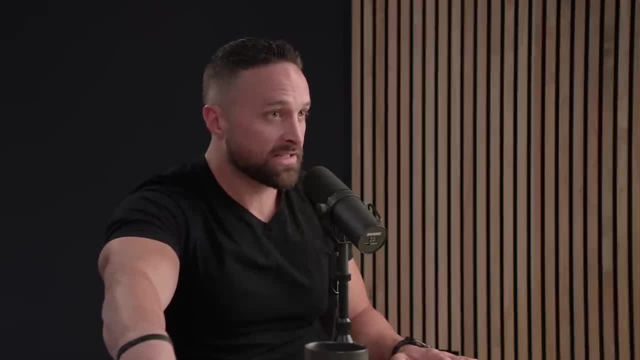 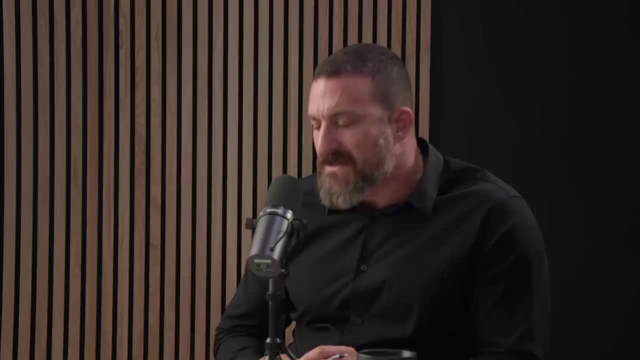 but what the outcome tends to be from a lot of processed food consumption, which is over-consuming calories, And then, therefore, you know, energy toxicity negatively contributing to your health. Yeah, It seems like it again returns to this: the potential for a positive 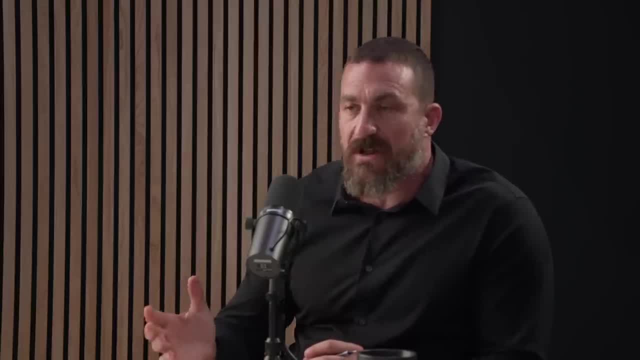 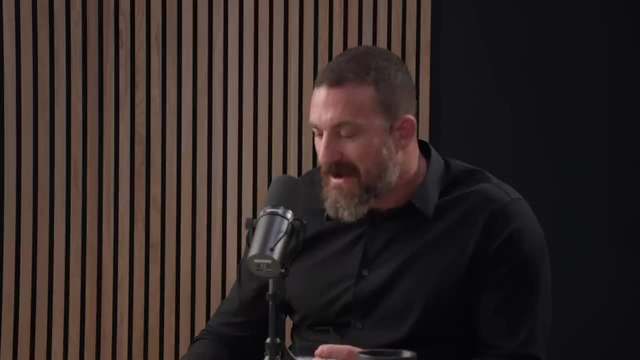 negative or neutral behavioral change and perceptual change of like craving a food all the time that you can't have as as terrible. That's a terrible state to be in And this, I think, is a perfect segue for something that first brought us together. 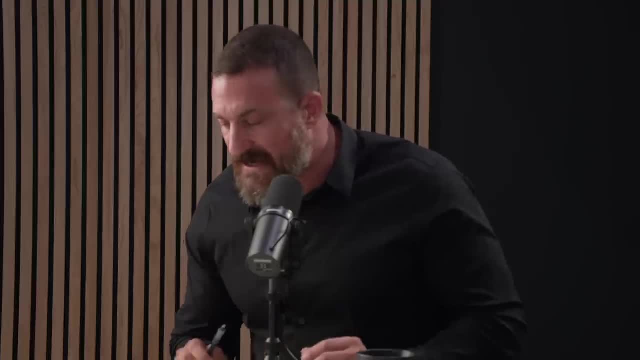 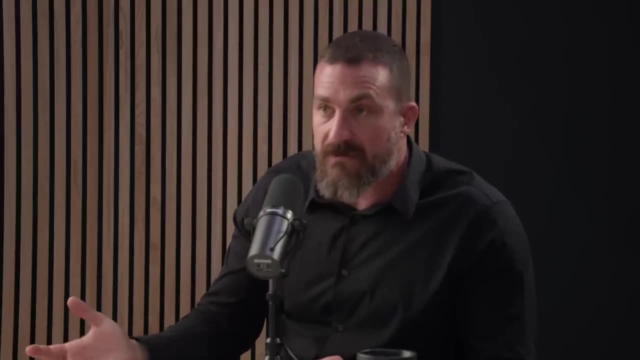 which was you know, which? was this? this thing about artificial sweeteners- And let me, just for the record, be very clear: I have long ingested foods with artificial sweeteners, So I, throughout graduate school, I didn't have the best habits. They're healthier now than they were back then. but I would drink, you know, a diet Coke or two, two per day. I still have the occasional diet Coke. I'm not completely averse to to drink something that has artificial sweetener. 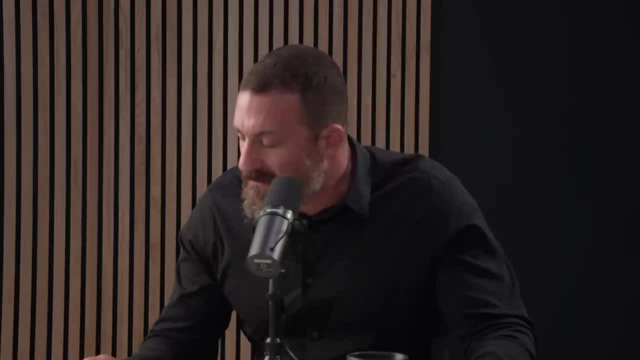 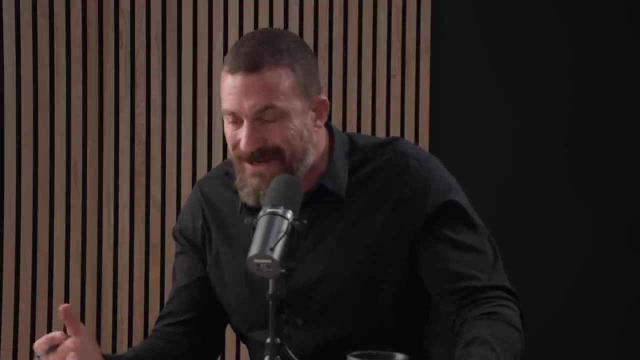 Although I do avoid sucralose for reasons that maybe I can get into a little bit later, but a lot of the things I consume contain Stevia, which is not artificial plant, but it is a plant-based non-caloric sweetener- low caloric sweetener. 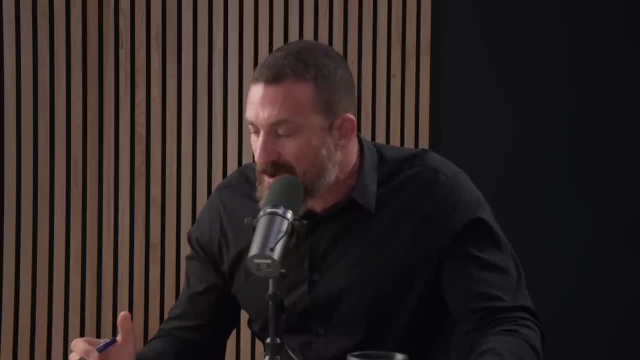 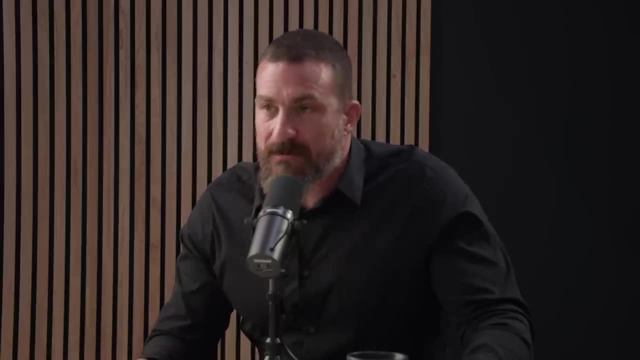 And I don't have a problem with that. I became very interested in artificial sweeteners because you know I'm not a big fan of artificial sweeteners, but I'm a big fan of artificial sweeteners And I think that's one of the reasons why I'm interested in artificial sweeteners- is because of the fact that they have the ability to disrupt the gut microbiome of the animal data. I'm pointing to the idea that they may disrupt the gut microbiome and then disrupt the gut microbiome, as you pointed out, as a very broad statement. 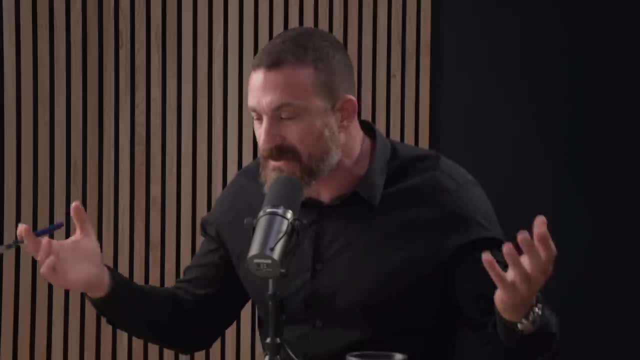 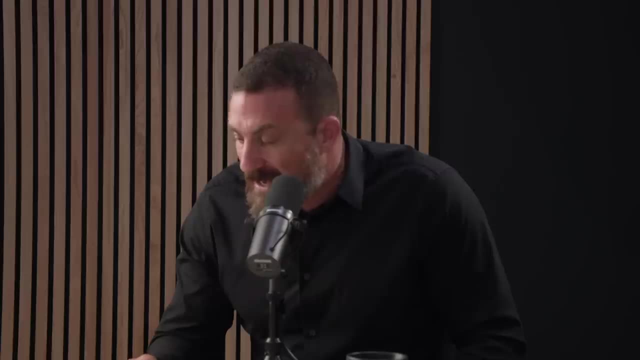 We don't really know the percentage of lactobacillus exobacillus or whatever bacillus, whatever silice illness in there They all seem to end in. illness is ideal And in fact a lot of these companies that are having people send in their stool samples for analysis of the microbiome. 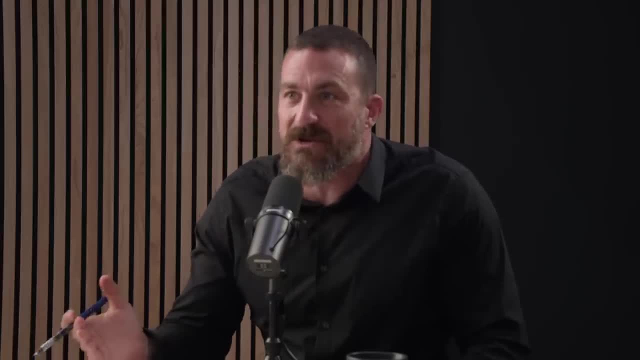 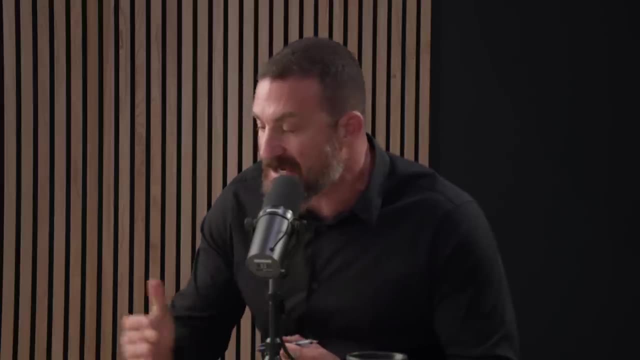 I mean, take note, We don't really know what a healthy microbiome looks like, but we know what an unhealthy microbiome might look like, And it's one that doesn't have a lot of diversity in there. So I was interested in that. 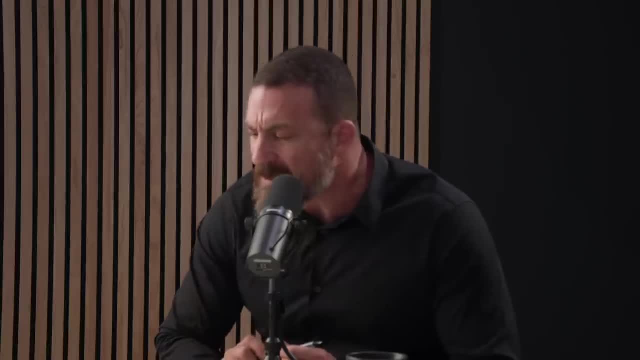 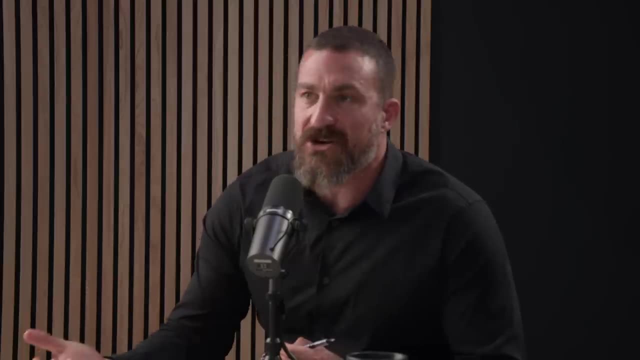 Then there's the recent human study, which we should definitely get into, but I was mostly interested in artificial sweeteners for the reason that there is this food conditioning effect And you see it in animals and you see it in humans- that if you ingest well. 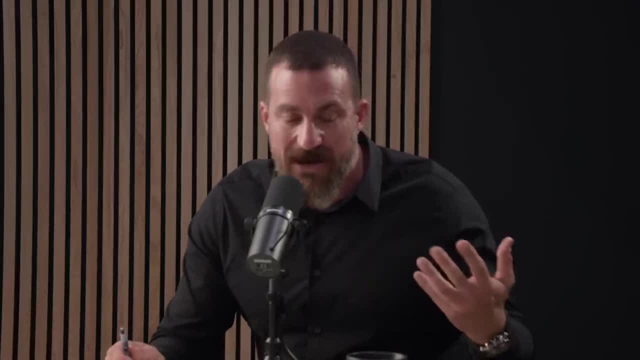 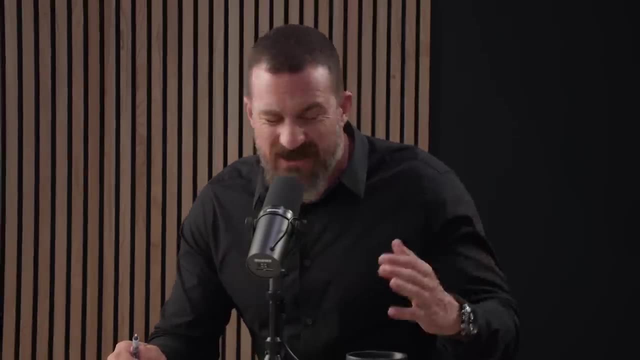 coffee is a really good example. Coffee doesn't actually taste good, folks, even though I like it. But when you taste coffee for the first time, most people think it's bitter And disgusting. most everybody, like 95% of people, will say this: doesn't taste good. 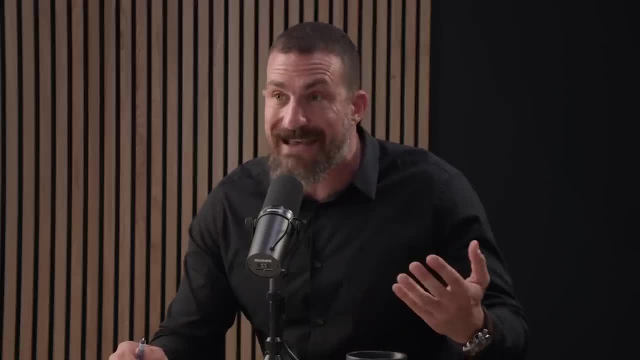 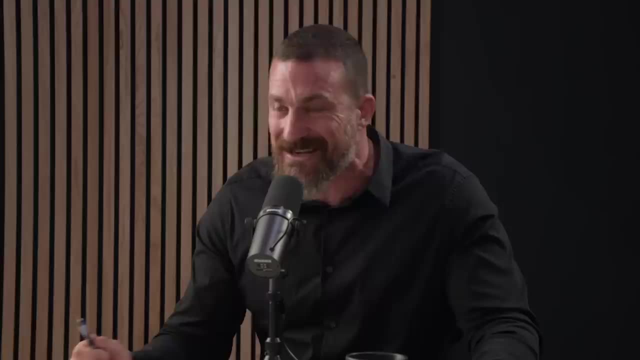 Wine, beer, same thing, Yep. But people learn to associate the state of being caffeinated, which most people like, in order to just feel normal. right, Caffeine is one of the few drugs we ingest just to feel ourselves enough that soon, myself included, really look forward to and enjoy a cup of coffee. 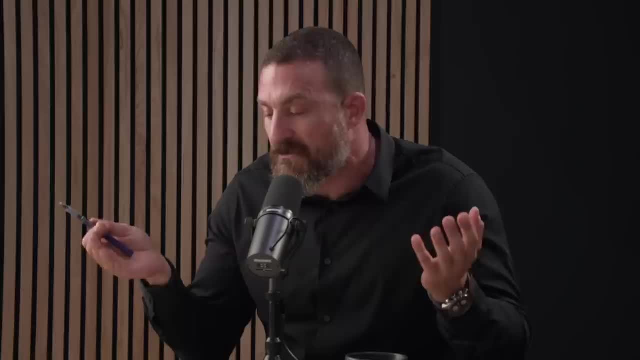 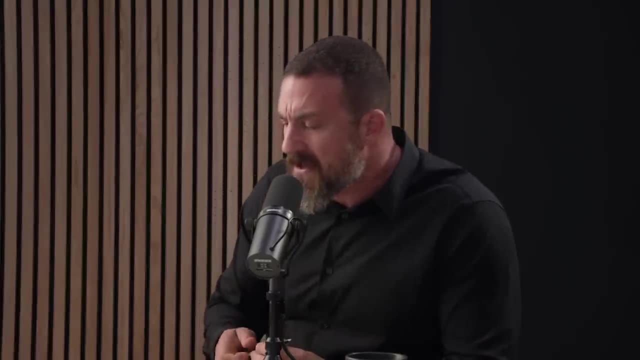 It's so. it's a powerful example, in my opinion, of the food conditioning effect. So it's like a Pavlovian thing: Instead of salivating, you crave right. And it did seem that this study from Dana Small's lab- which admittedly was a small- 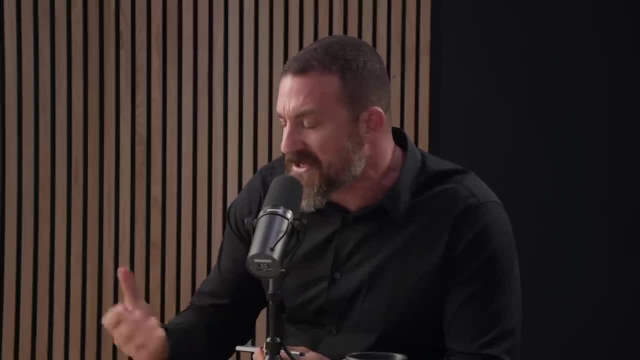 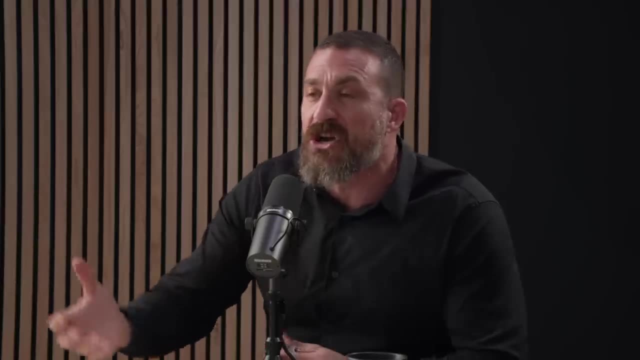 no pun intended. study itself- not very many subjects- showed that if you ingested artificial sweeteners along with food that contained glucose that you could sort of maybe even get a heightened glucose response just from the artificial sweeteners. after a while you and I connected over this study on social media. 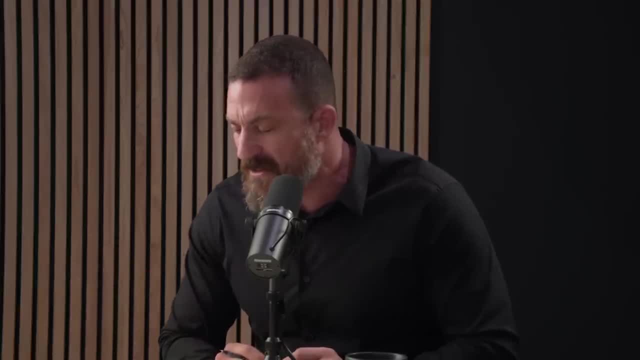 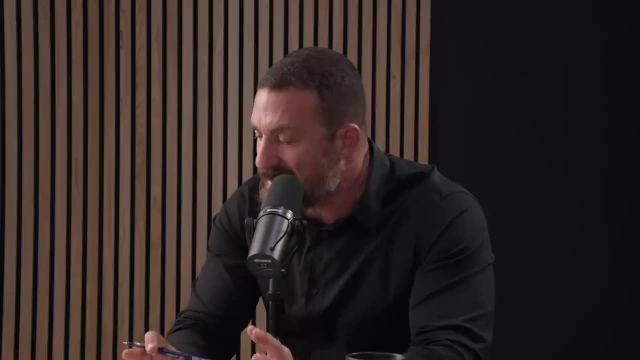 you pointed out that the design of the study wasn't superb. There was, there was co-consumption of glucose, which made it complicated. We can go into that, But the reason I'm spouting off all this context is artificial sweeteners are many things. 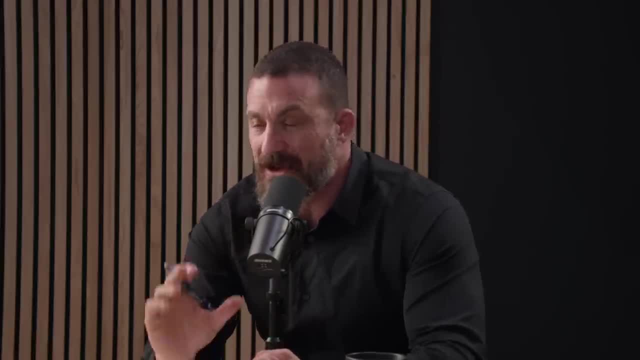 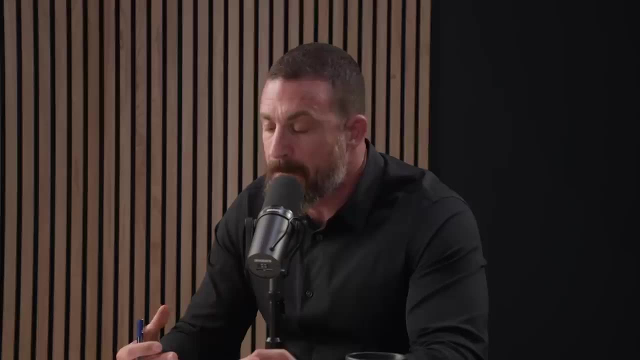 So I'd like to talk about their effects on blood sugar in the acute sense and according to what we might ingest them, with what and how they might be changing blood sugar regulation at the level of brain and or body, And then the gut. microbiome data I think are interesting enough to discuss, and I have changed my view on artificial sweeteners based on what you've taught me. 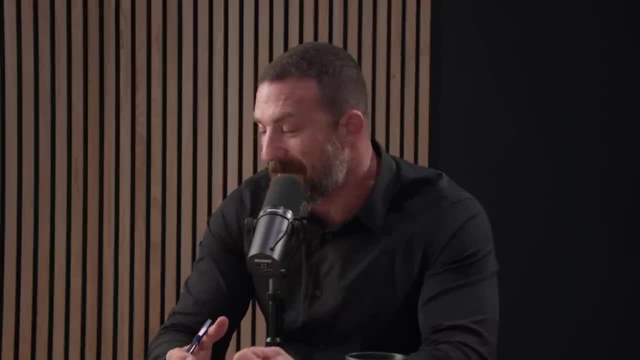 So this is a case where I've completely Changed my view, which is that now I don't- I don't have any problem with them whatsoever, based on the current data, which is not to say that I'm, you know, gulping down a cupfuls of superlose, but I feel okay ingesting some stevia and some aspartame and I'm not too worried about it. 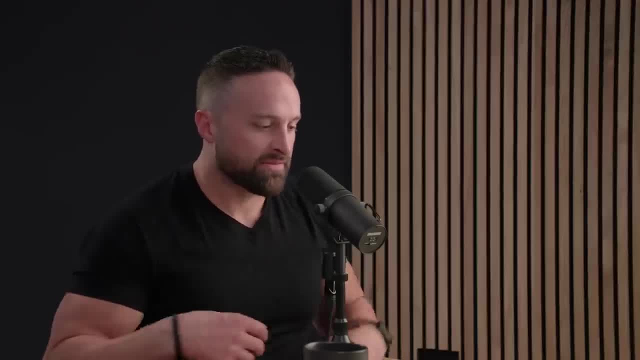 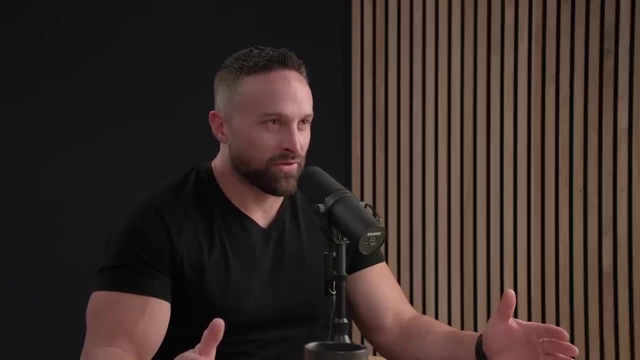 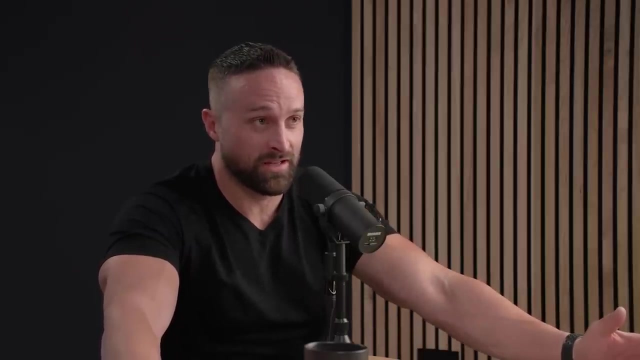 Yeah. So I think, kind of stepping back from a broad view, We have to think about again the hierarchy of importance. Right, And what are you replacing with Right? So There is no situation where it is not a net positive to take somebody who drinks sugar sweetened beverages and have them drink an artificially sweetened beverage like the. in the meta analysis there was actually a recent network meta analysis looking at like, at markers of adiposity. 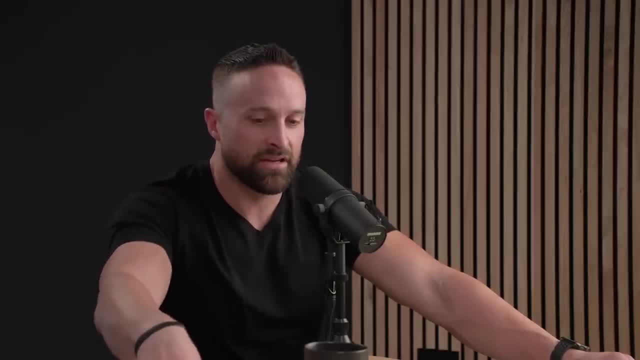 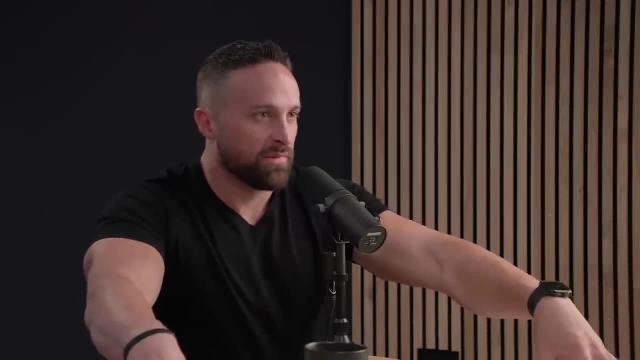 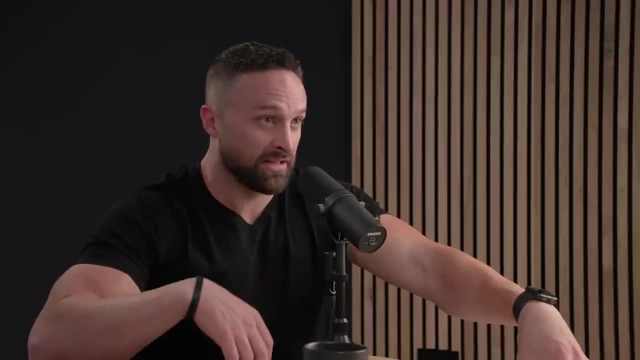 You know HBA1C, a bunch of different health markers, and when you substitute- you know We'll call it- non-nutritive sweeteners, since stevia is- Yeah Yeah, It's not artificial. But so when you substitute NNS for the sugar sweetened beverages, you see improvements in a lot of different things. 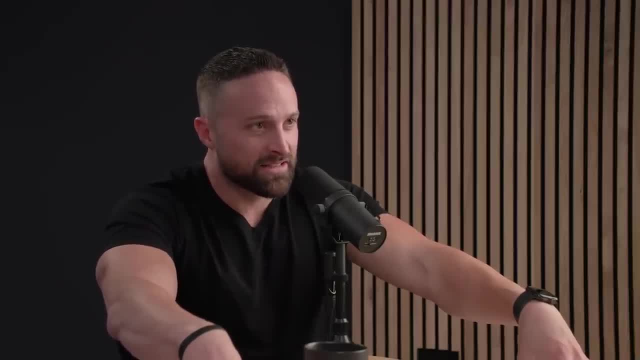 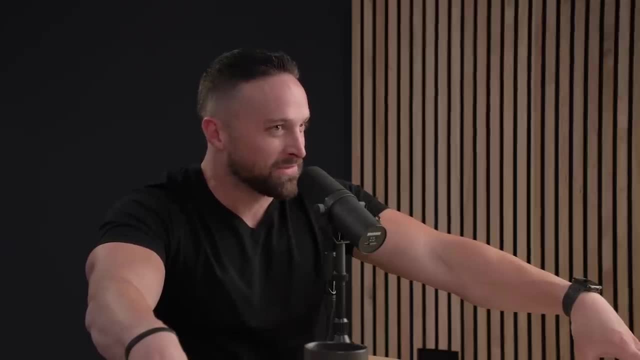 OK, What was really interesting about this network meta analysis was they also looked at water substitution in place of sugar sweetened beverages and the effect wasn't as powerful as- And these are randomized control trials, So artificial sweetener containing beverages are more beneficial. 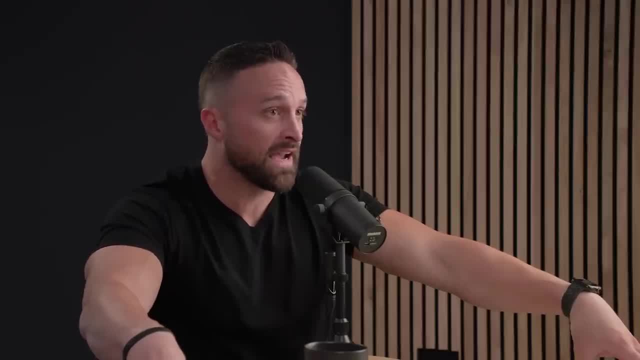 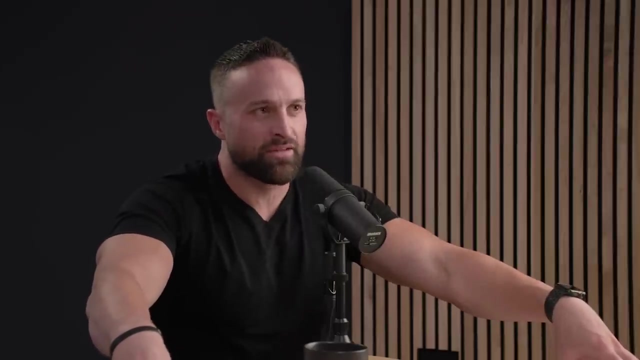 We're better for adiposity, for improving adiposity, And then in the health markers it was kind of a wash water, and water and non-nutritive sweetener beverages performed similar, but they were better than sugar sweetened beverages obviously. So they then based on a network. meta analysis is kind of where you can compare two things that didn't get compared directly. 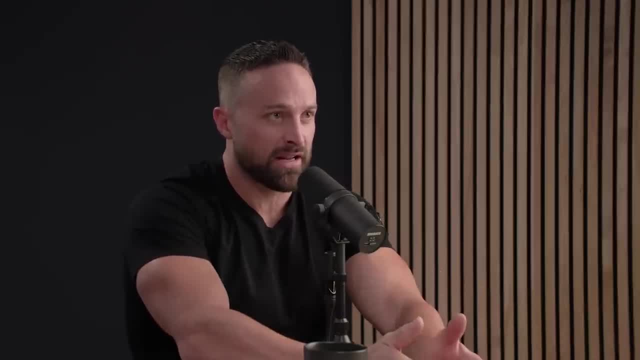 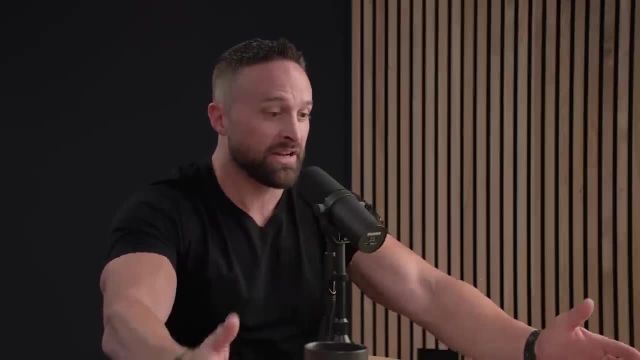 So there's not many studies comparing NNS versus water directly. But if you have a Common comparator- So if you compare A to B and B gets compared to C- you compare A to C based on how they interacted with B. I'm butchering it a little bit, but that's kind of the crux of a network meta analysis. 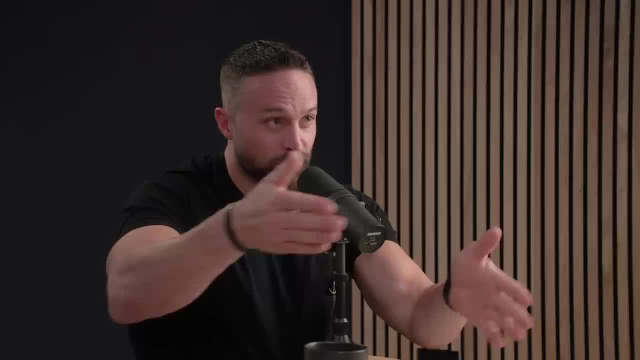 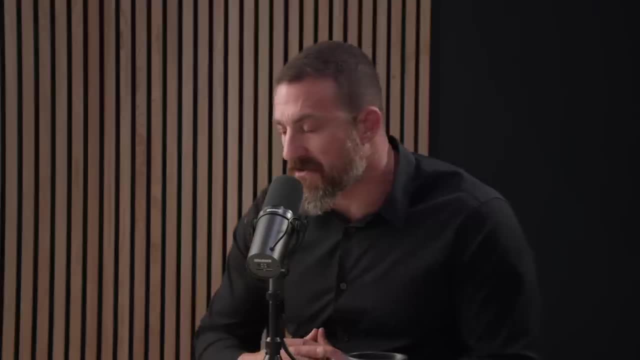 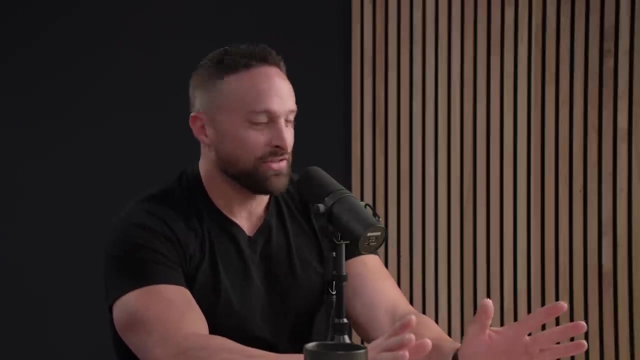 So they looked at NNS versus water and found that actually NNS was slightly better for improving adiposity NNS, of course, being non-nutritive sweeteners, Right. So now again, if you like drinking water and you don't want to. 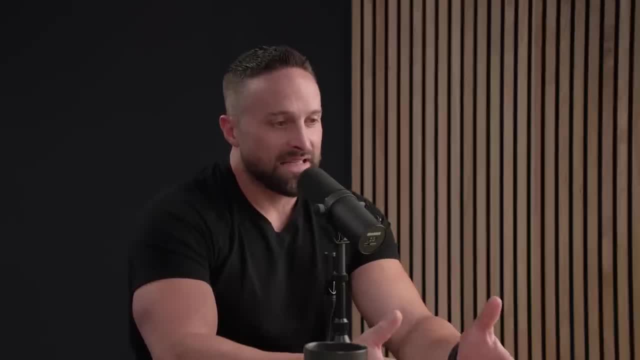 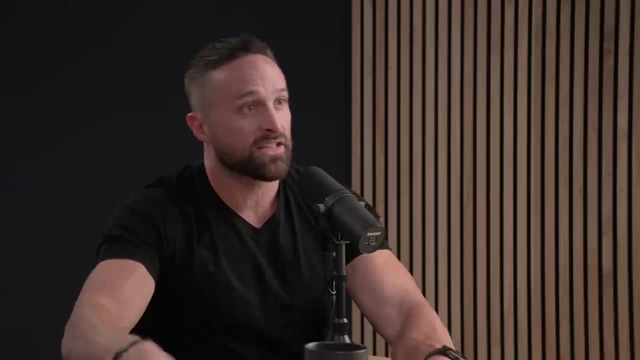 I'm not trying to convince anybody to do that. What that seems to suggest is there is a little bit of an appetite suppressant effect from these artificial sweeteners or non-nutritive sweeteners. Now this gets a little more complicated because if these were people drinking sugar sweetened beverages, maybe they've already developed a sweet taste and try to go to water is too much of a jump for them. 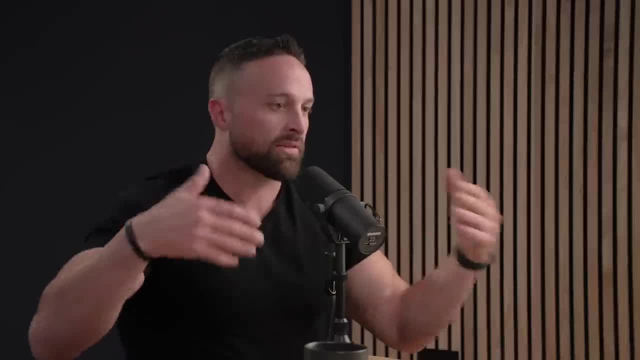 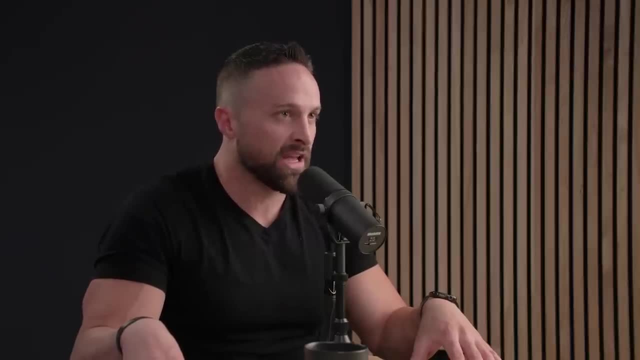 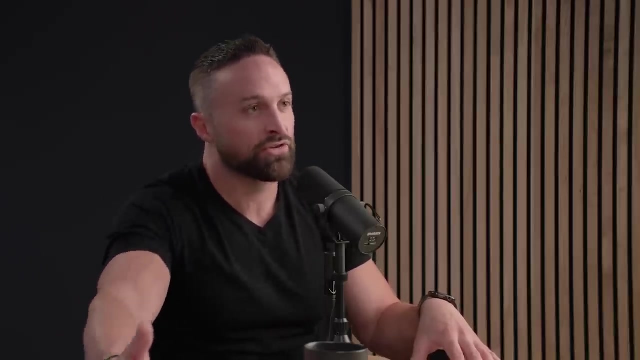 And so going to having something like intermediate is a little bit better, like there's a lot wrapped up in this. But these are the randomized control trials, which are a little bit more tightly controlled, which I I tend to default to a little bit More than I do. the epidemiology, which epidemiology is just so messy because, sure you know, non-nutritive sweetener consumption may be associated with different things. 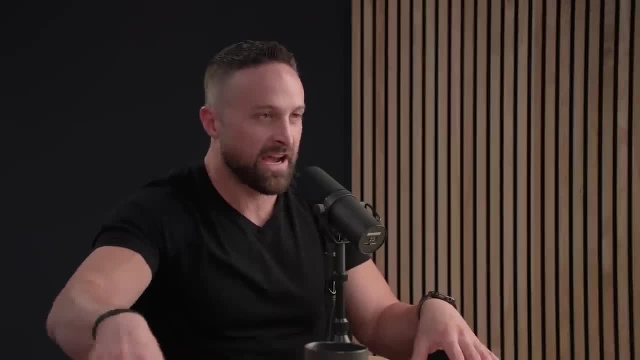 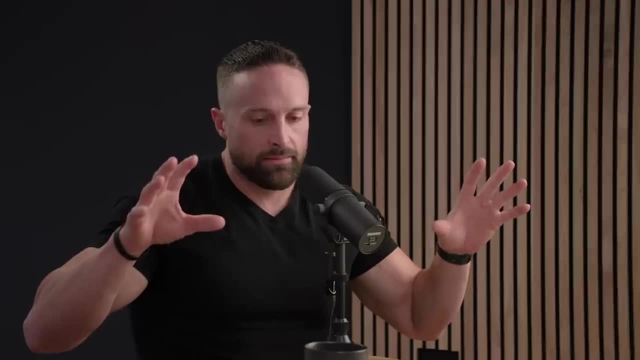 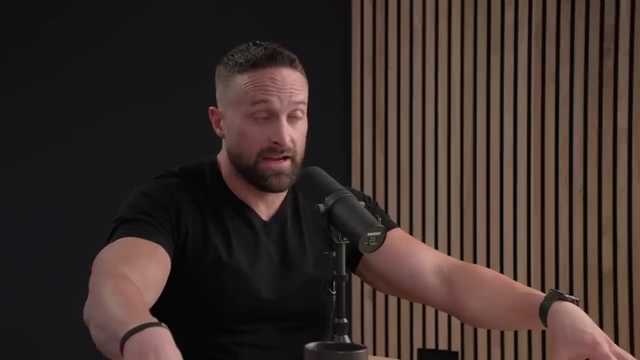 But there's also a whole nother set of lifestyle and habits that are tied up in that, So I tend to hang my hat a little bit more on the randomized control trials. So, understanding that- OK, now, all things being equal- understanding that this is a tool that may help some people. And whenever I post about non-nutritive sweeteners In The comments, there's always one or two or three people who say: all I did was cut out soda and I drank diet soda instead and I lost 50 pounds, or I lost 75 pounds. I even had one percent. I lost 100 pounds. that's the only thing I did. 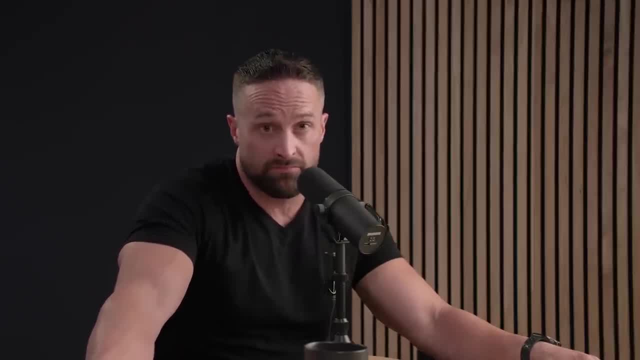 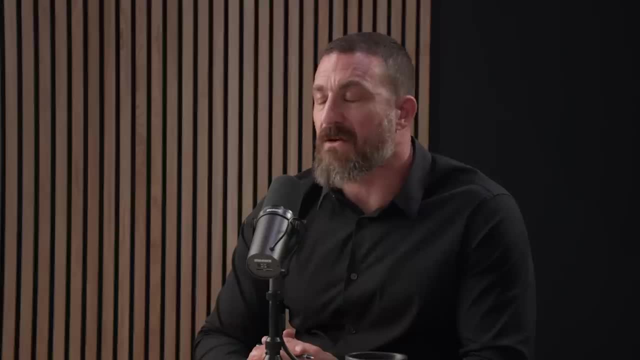 I mean that's a pretty massive lever to pull if you consider somebody who might be having, like I mean, five or six cokes a day. I mean that's you know, we're talking a serious amount of calories. And that also means that by replacing with artificial sweetener containing beverages. 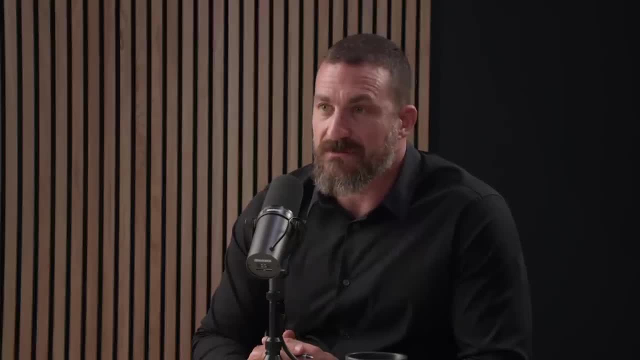 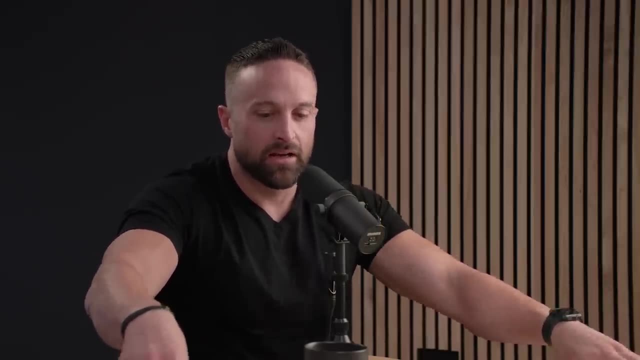 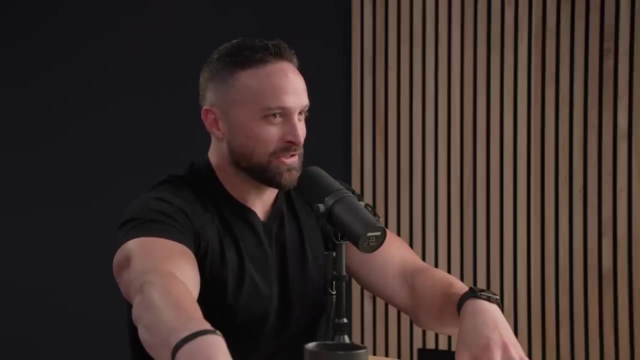 They did not replace the soda With food, Correct. So like let's now, let's talk about right, this is where we can get into the micro analysis. But is that obese person who lost 100 pounds by doing that Do I really care about? maybe a small alteration to their gut microbiome? 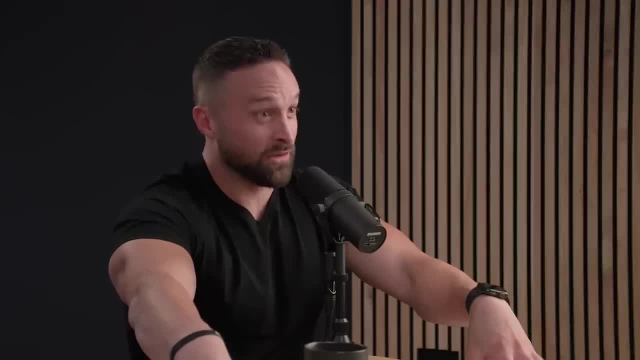 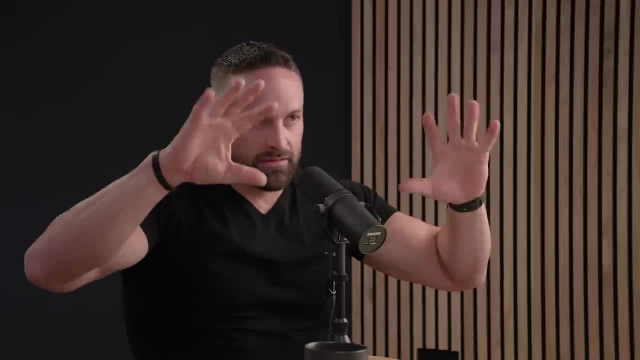 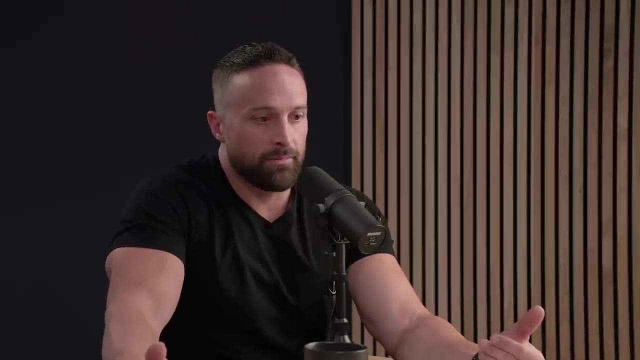 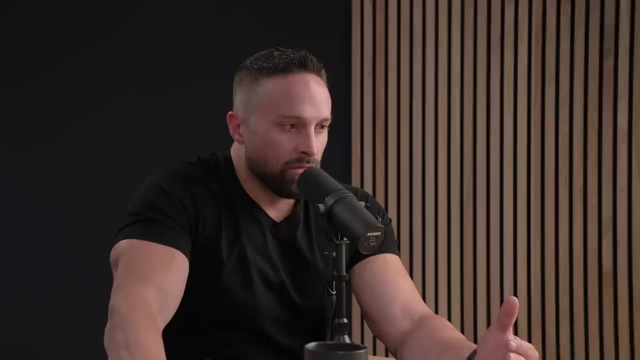 No, because their gut microbiome is actually much more healthy now by them having lost all that excess adipose tissue. So again, the ranking of what I'm worried about, you know, can change Depending On the specific situation. Now let's take somebody like me who's lean and doesn't really have, you know, any health problems that I'm aware of. 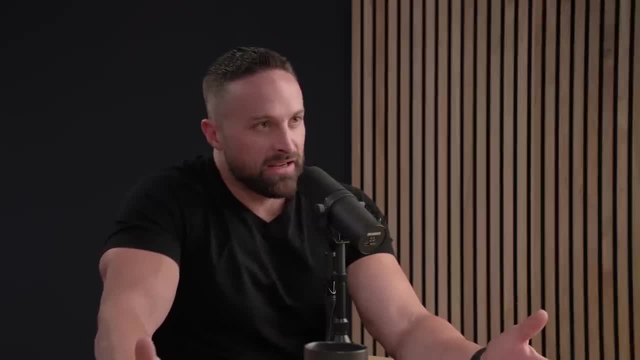 What about artificial sweeteners for me? Well, for me, I kind of got using them because of bodybuilding contest prep, because it was about the only appetite suppressant that worked for me. But do I think that they are healthful? Probably not. Do I think they're unhealthy? 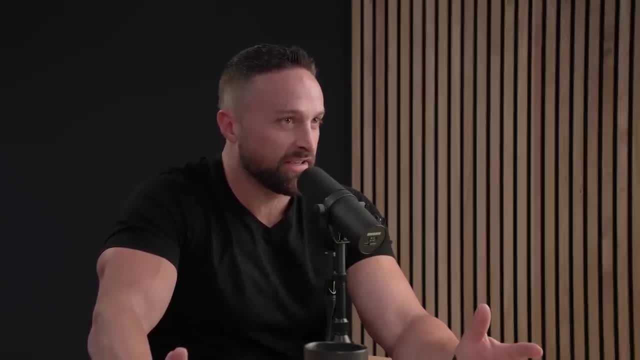 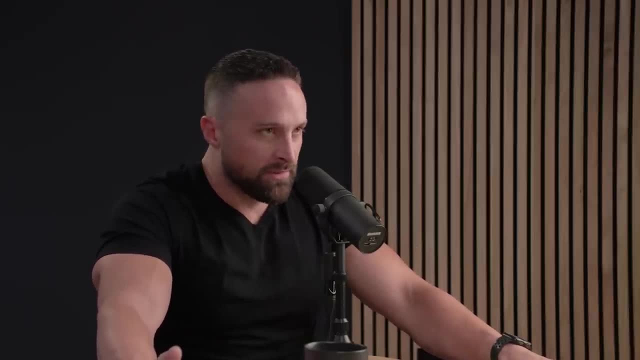 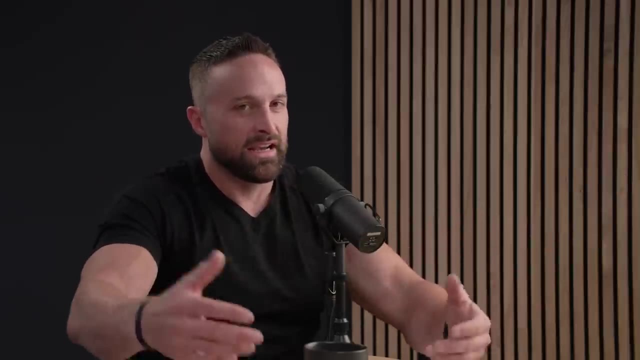 I would say, based on the current data, I don't think that they're unhealthy. Now the information on blood glucose. So there's some of the problems with some of these men analyses or these these reviews is they kind of lump all the non nutritive sweeteners together. 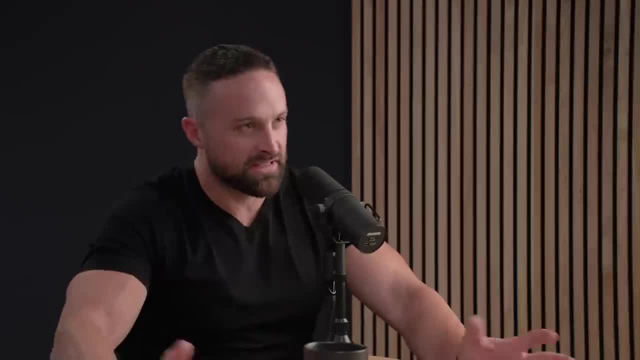 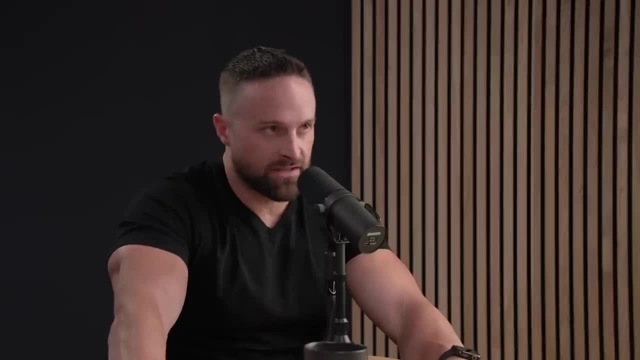 And then they may say: well, there's no effect on this, or there's an effect on this. Well, the problem is is these probably are. These are different molecules and they can interact differently. Aspartame Very clearly seems to have no effect on blood sugar or insulin. 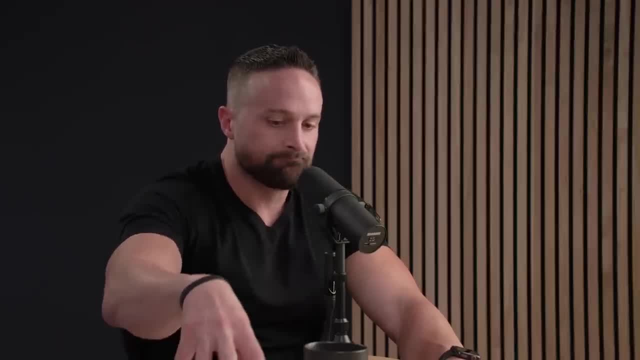 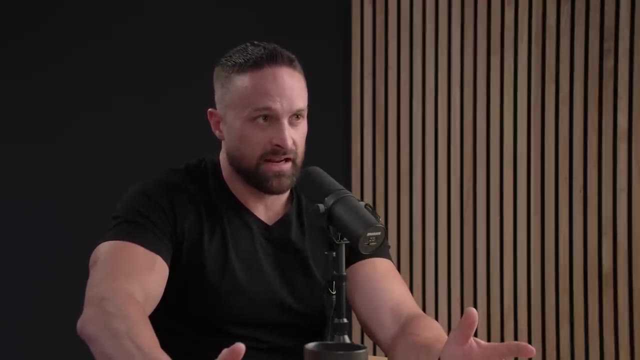 That has been repeatedly shown. Stevia doesn't appear to have much effect. saccharin and sucralose: The jury is kind of mixed. Now. there was the study that we first connected on, which I think their primary outcome measure was actually they were looking at like kind of the sweet taste, like how it affected sweet taste. 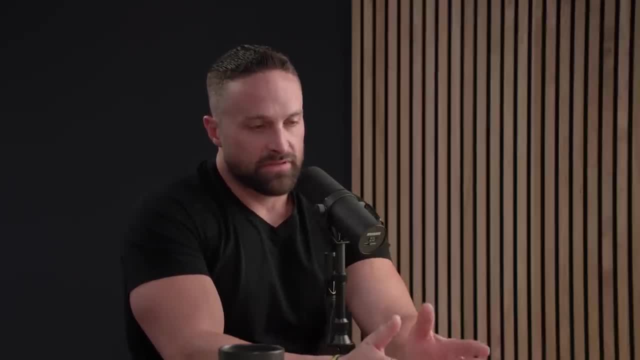 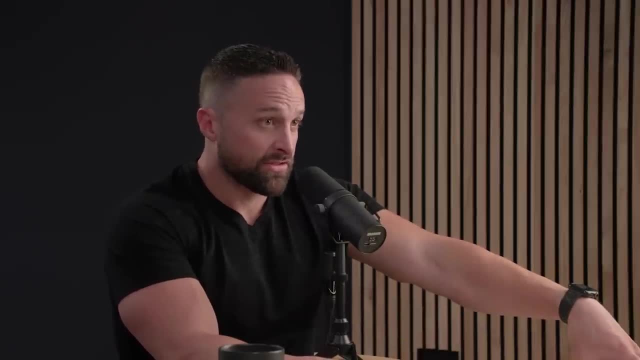 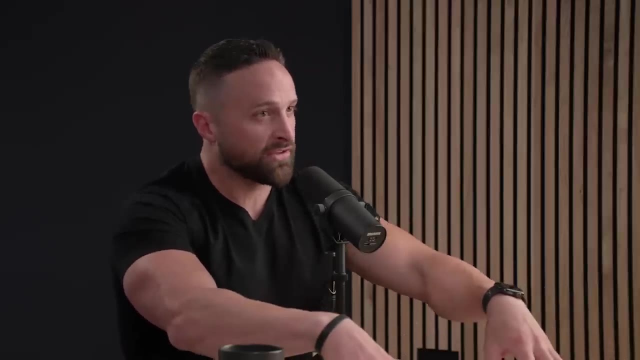 So what they did was: the group that was getting The sucralose was also paired with maltodextrin. The control group was getting sucrose, Which The Is an appropriate way to compare the sweet taste, because maltodextrin is not as sweet as sucrose. 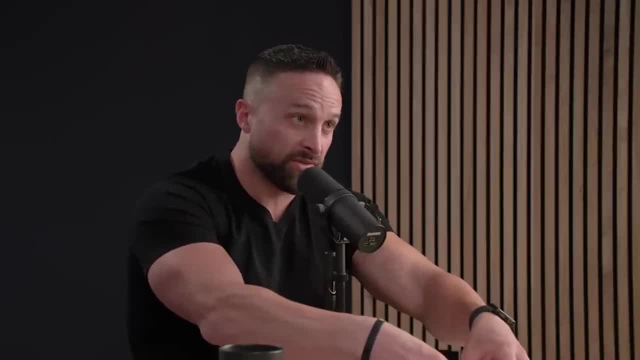 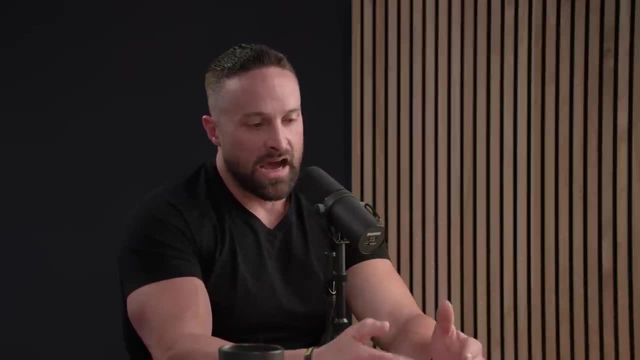 So when you're trying to combine- you know, sucralose, which is already sweet, with another form of carbohydrate, you'd want something less sweet compared to your control. But For the outcome measure of Insulin And blood glucose, Probably not as appropriate, because we know maltodextrin has a much higher glycemic index than sucrose. 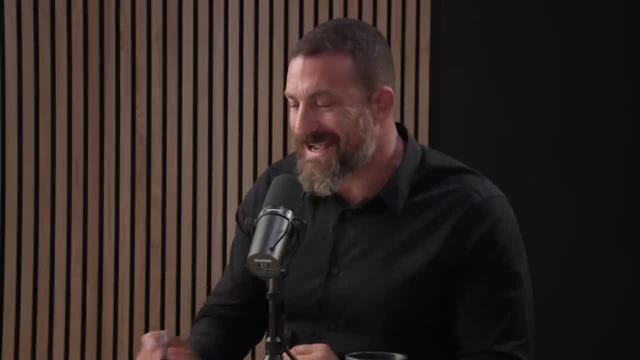 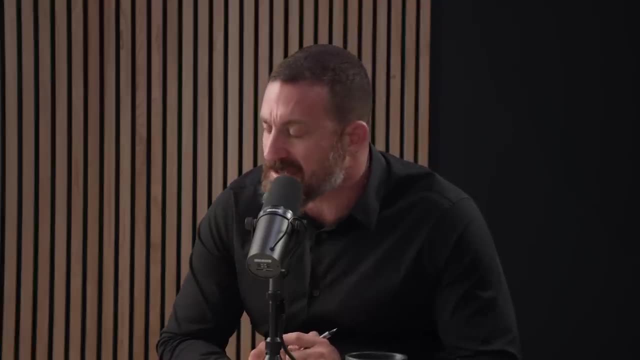 So they they appropriately controlled for For taste, but not for the effect of the sweeteners, And I think that that was a key component And I think, yeah, the part of that study that intrigued me actually was in a talk version of that, because that study drove me to watch a talk that. 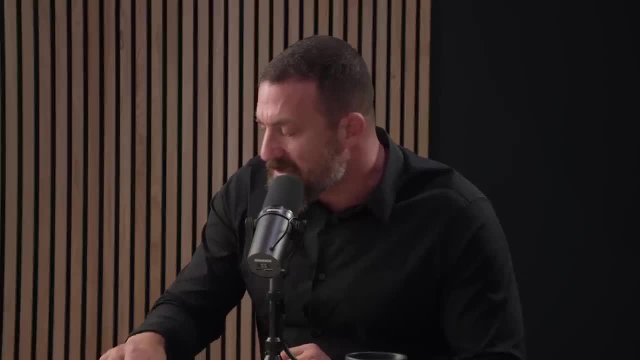 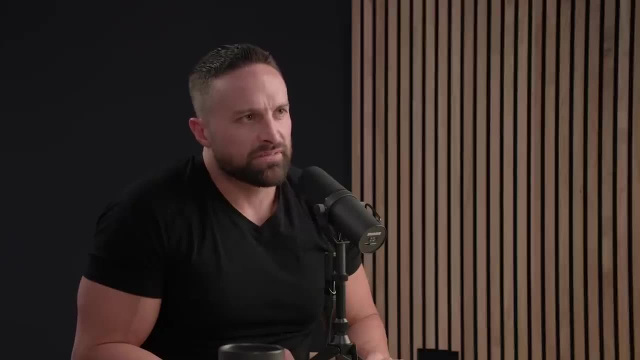 And we'll get Dana small on on the podcast at some point. Hopefully Was that they had. they had kids do this study and they actually had to cease the study because a couple of the kids became pre-diabetic. I mean, it seemed like there was something hazardous about this. was at Yale School of Medicine. 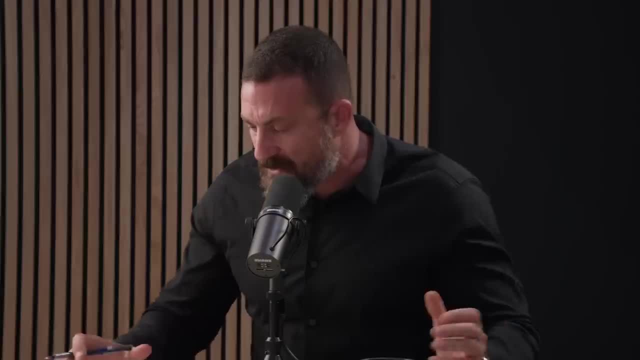 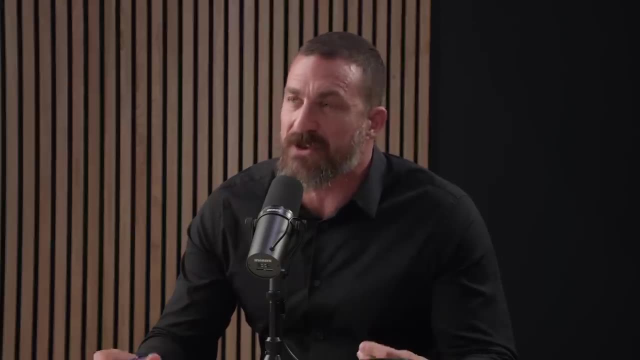 It's a good place. I mean, you know every, you know there's a range everywhere, But it just seemed like there's something about sweet taste that, if taken to the extreme, might be able to impact blood sugar too. This has impacted my sort of behavior. 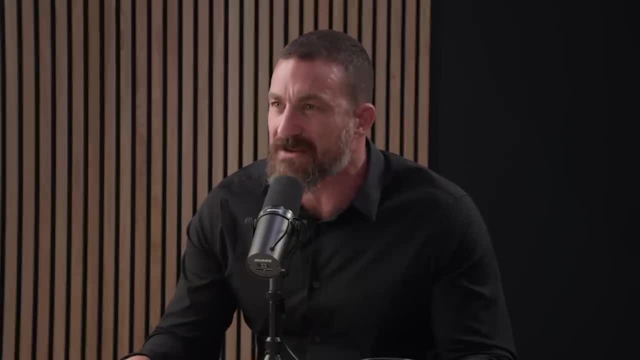 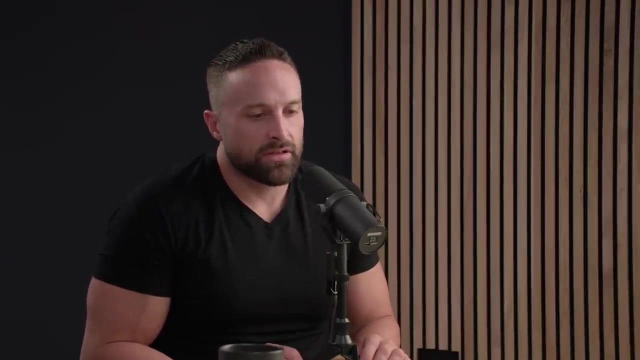 And I trying to. I try to avoid really sweet things unless they're exceptionally delicious or the occasion calls for them, because I do think that it increases my craving for sweet things. Well, it might not be necessarily a craving, but it just programs you. So let's, your taste buds are extremely adaptable. 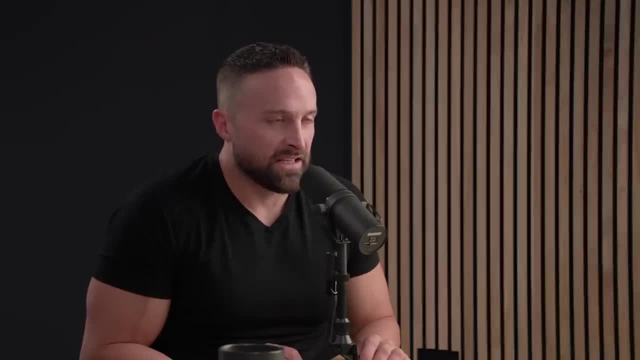 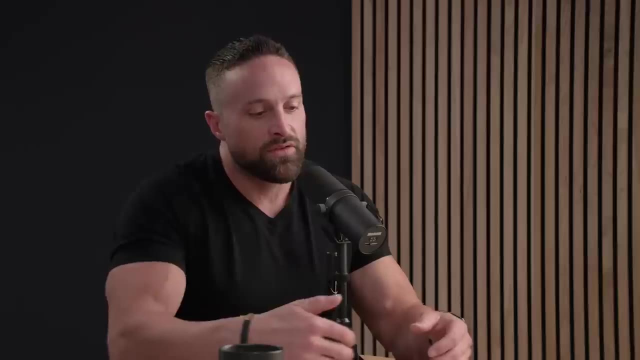 So take, for example, like Indian food. If you bring like Indian people over to America and have them eat some of our food, they think it tastes extremely bland Because they, Because they are used to such spicy food that unless they have a certain level of spice, they hardly even taste it. If you've ever done a high sodium diet and then gone to a low sodium diet, it feels very bland. That's a styrofoam, But you're, you're. over time, your taste buds adjust. So sweet is the same thing. If you're used to eating a lot of sweet, you get kind of desensitized to it. 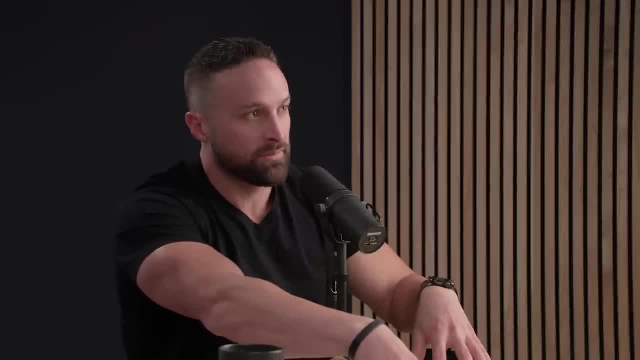 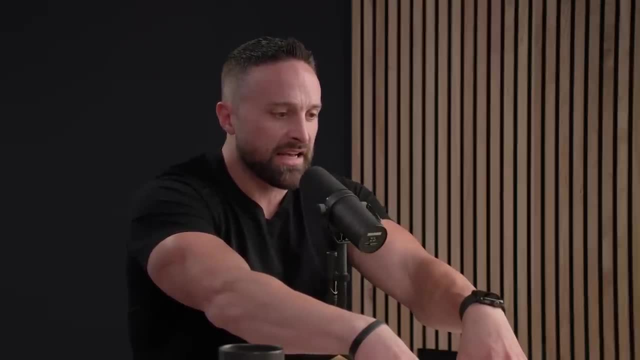 And then if you go to something less sweet, it can kind of taste bland at first. Over time it'll get better. But so I think it's one of those things that again it depends on the situation, right, Like if somebody is obese and they said: well, this is going to help me, you know, eliminate sugar sweetened beverage. 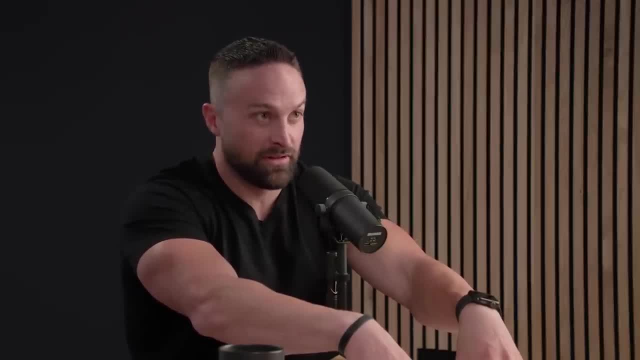 Like why would you want to take that tool away from them? Like that's a great lever to pull. I mean, if somebody can lose literally 100 pounds from just one change in lifestyle, that's not even really that inconvenient of a change. That's. that is powerful. 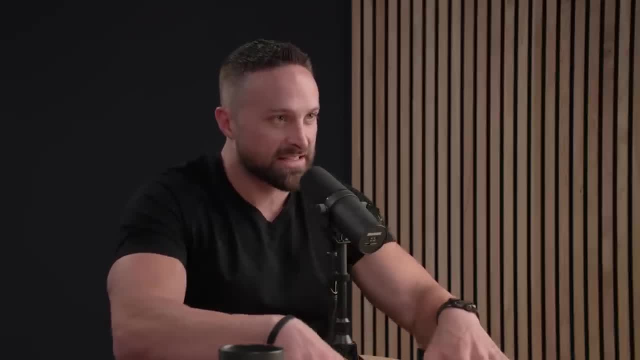 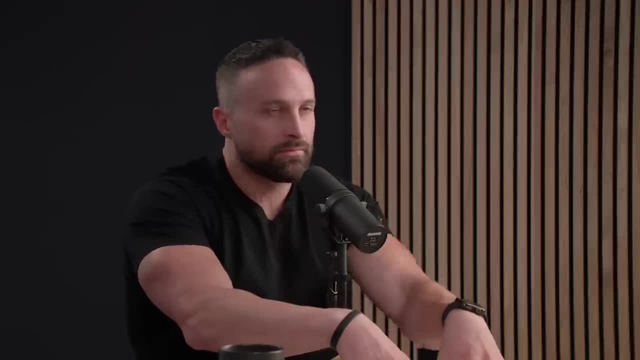 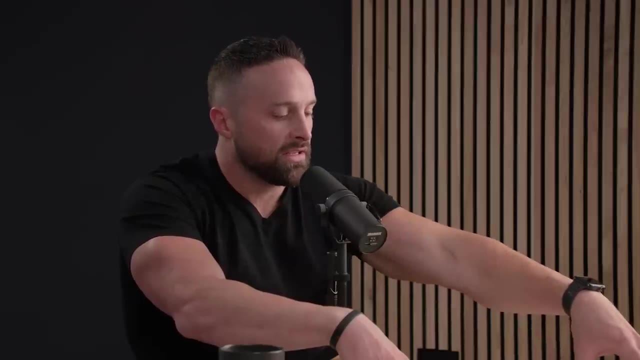 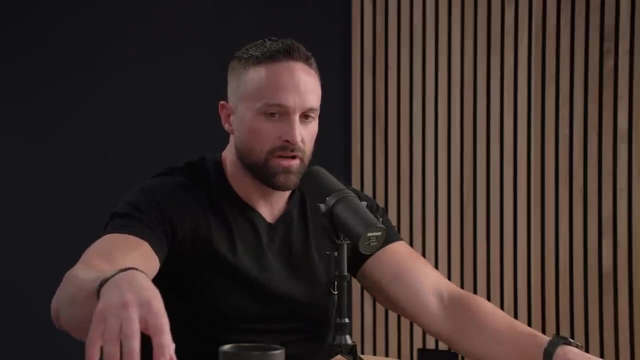 But again, is it the most healthy thing they could do? And I think that's kind of like what tends to get asked. We don't know it. Is it healthier than water? Probably not, maybe as healthy as it, Who knows. Now, the. but I really make all those caveats because you don't want to have people who could use this as a tool. think: well, I can't do this because it's actually bad for me. 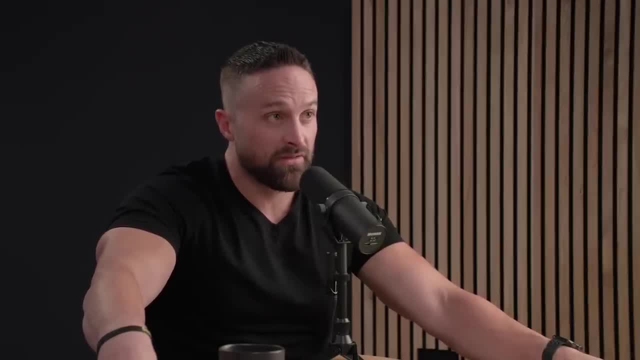 Right, If it helps you lose 50 pounds or 75 pounds, Right Yeah. If it helps you lose 75 pounds, or whatever it is, Trust me, it's not bad for you, Right? Well, it does seem to increase the satiety signals. 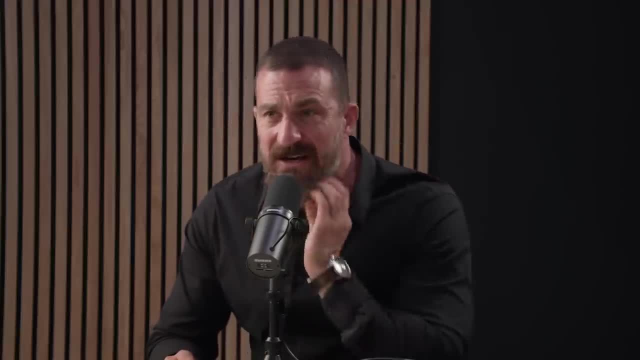 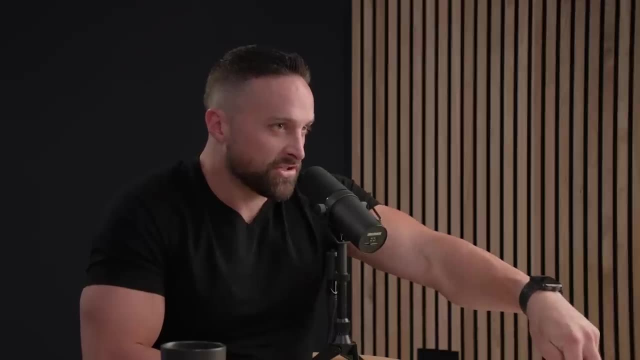 What do you think about the microbiome effects in this recent study? Because the recent study, I think, had some nice features to it And you've done a detailed description of the study. So for those that want that, Is this a two week study. 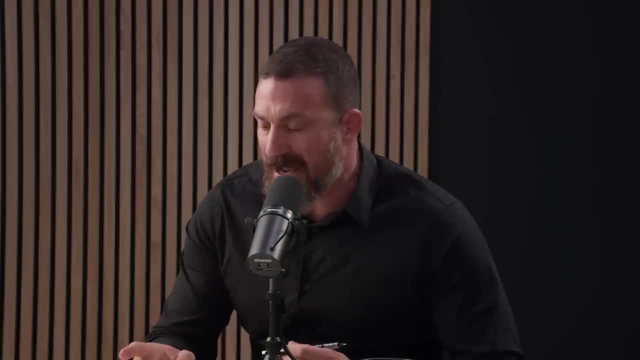 Or the two week study? Yeah, and we will provide a link. You did an excellent video on this on your YouTube channel. that really parses each piece. But they compared the various artificial sweeteners and looked at the glucose response, Looked at microbiome. 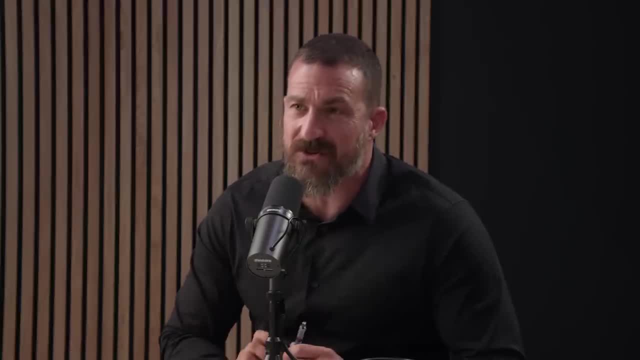 A number of different measures. What was your general take away? And this was in humans, For I think the first time looking at microbiome in humans due to artificial sweeteners. There are a few studies on the microbiome in humans with artificial sweeteners. 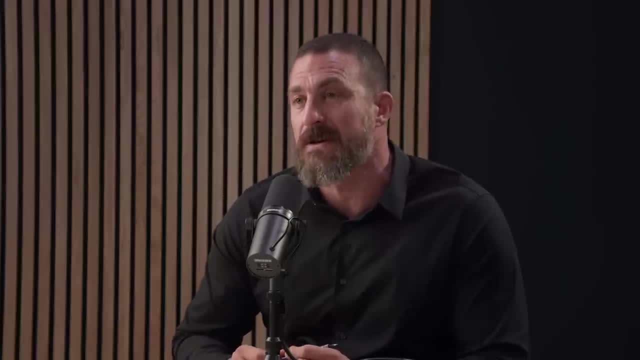 The first two that came out showed pretty much no effect, But they were a little bit shorter in duration, They were like two to four weeks, And again it depends on like what bacteria are getting measured Right, Like there's, you know, many different kinds of bacteria. 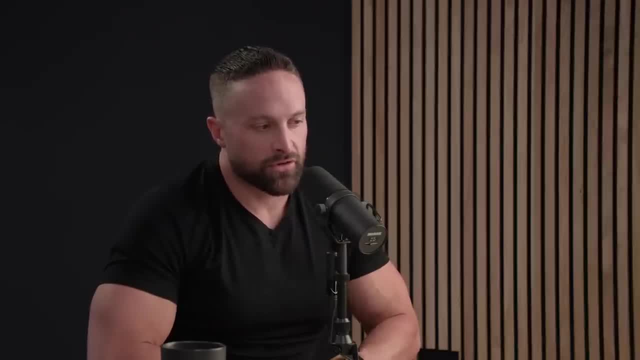 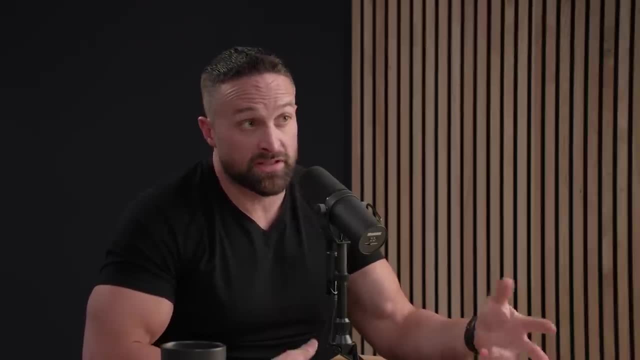 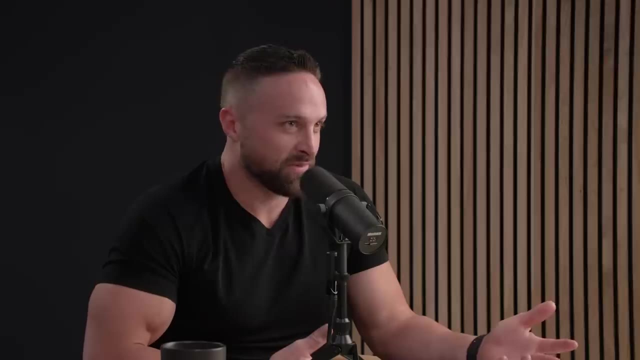 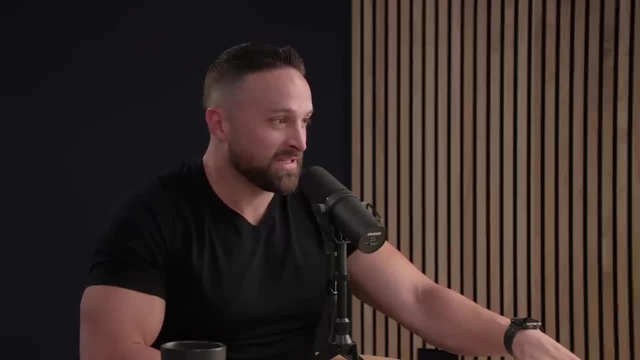 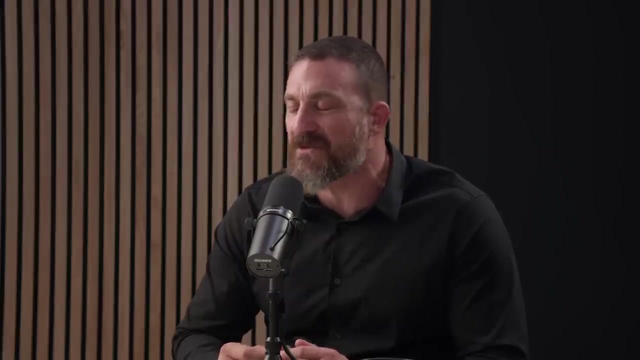 Now what was interesting is when I went into the species that changed. the species that changed the most, compared to control, was a species called- I'm going to butcher the name- but looks like Blaudia coccitis. I think it's called. Yeah, Those that work on the microbiome. it's so difficult to pronounce anything. 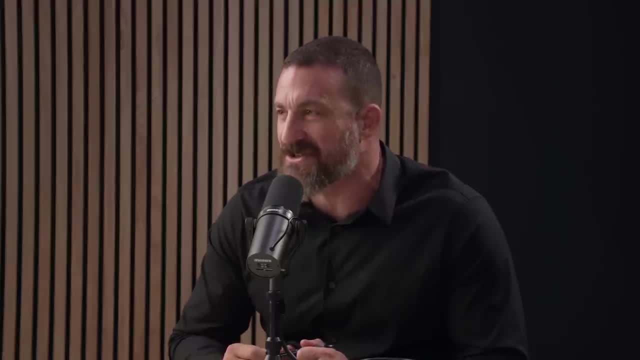 You need a nomenclature committee and you need acronyms. I'm sorry, Just do it. Enough, already You're killing us. We'll call it BC. We'll call it BC. Thank you. We're going to start the nomenclature committee without you if you don't do it soon. 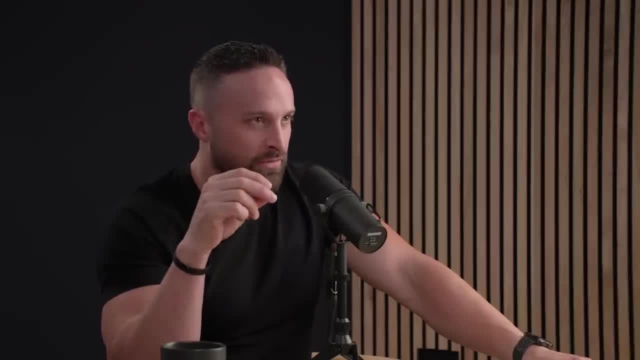 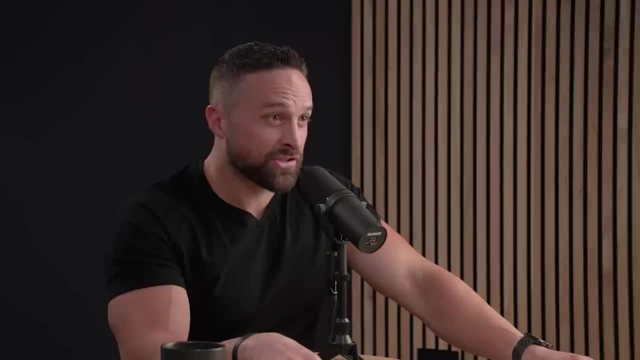 So they noticed that this went up by like three to fourfold, So I kind of went down the rabbit hole on this. So, interestingly, that particular species of bacteria is actually associated with lower adiposity, better insulin sensitivity and people who are obese and children who are. 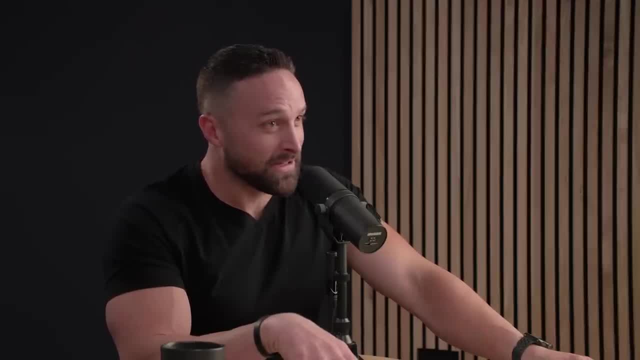 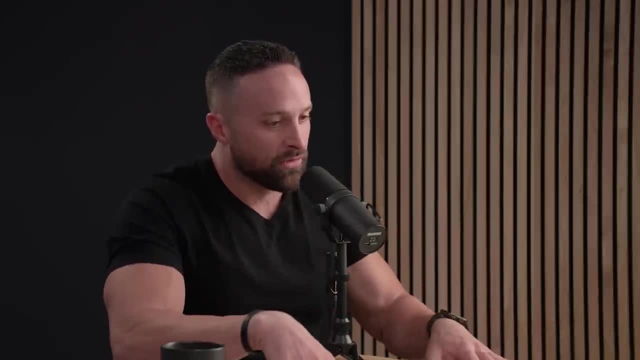 obese tend to have less of it. So I said: well, based on that study, you could actually argue that maybe sucralose actually improved the gut microbiome. Now again, I'm not making that claim because you know we have a hard time understanding. 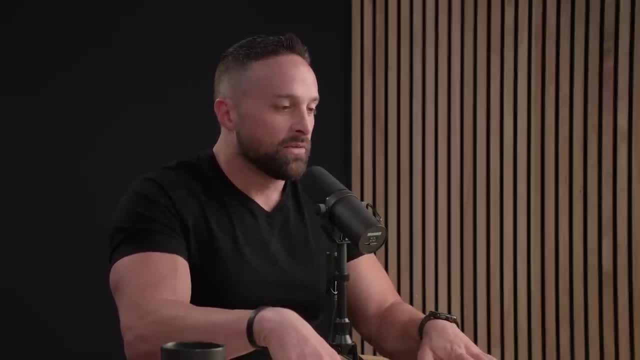 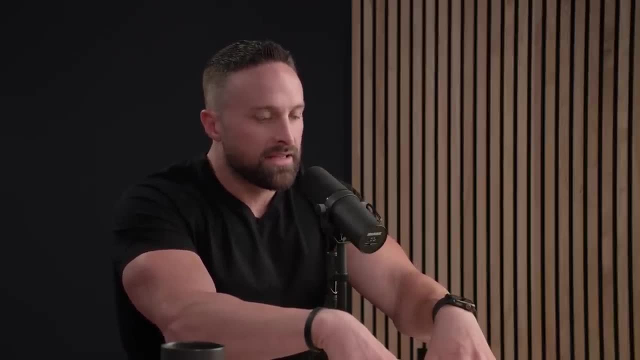 what a healthy microbiome looks like already. What this last study that came out. my biggest take home was. I think it's safe to say that it's not a good study. It's not a good study. Some of these non-nutritive sweeteners are not metabolically inert. 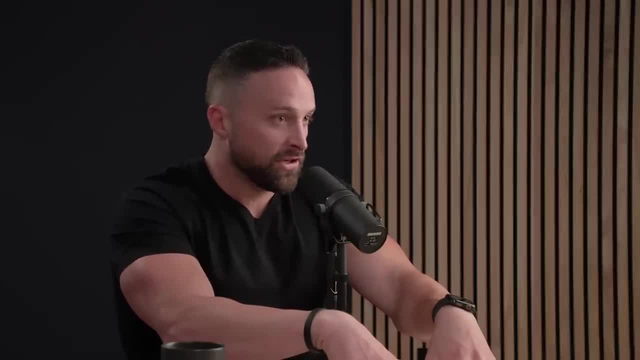 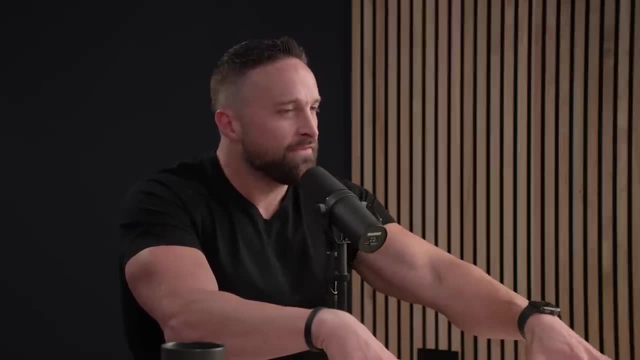 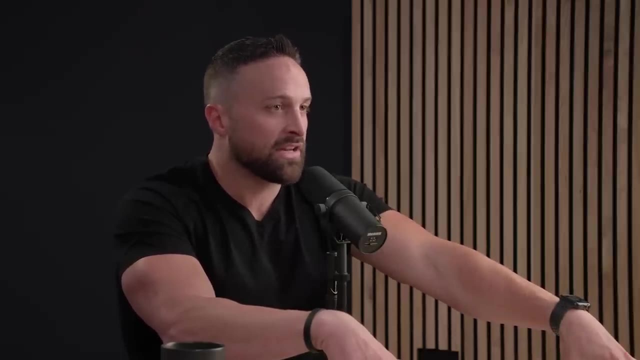 There are some effects. Now are those effects good, bad or neutral? I think has yet to be fully elucidated. Now. I focused more on the blood glucose responses in my analysis. So in that 10-week study they did oral glucose tolerance tests. 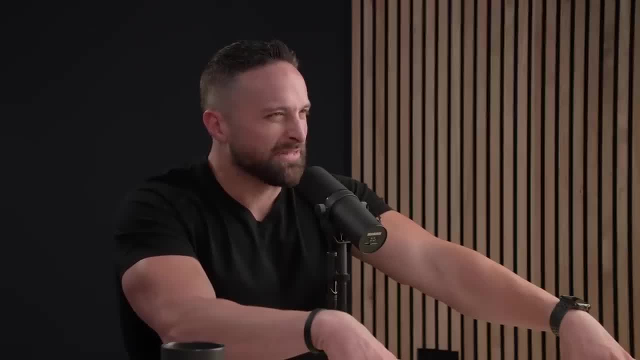 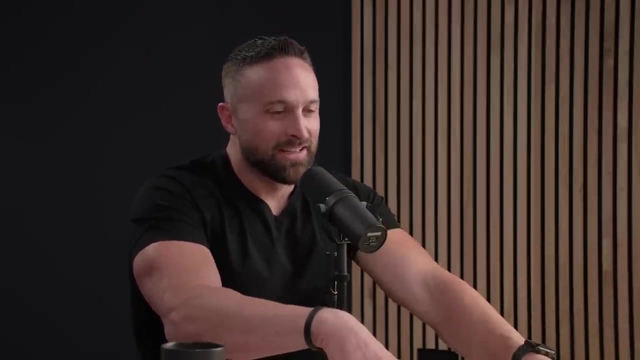 And their conclusion I didn't really feel like fit. They're different. So the conclusion was that- and again I think it was sucralose, that it elevated blood glucose, And this is where statistics can get kind of tricky. So my take home was the area under the curve, the incremental area under the curve, which 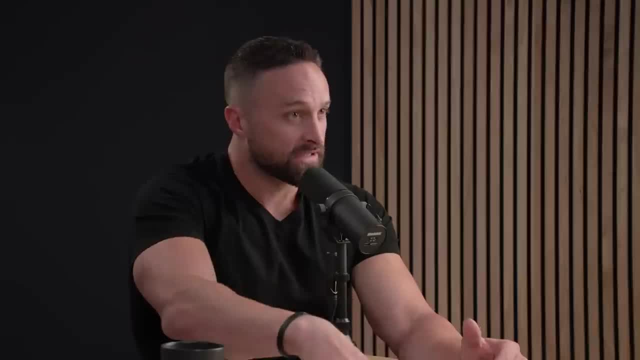 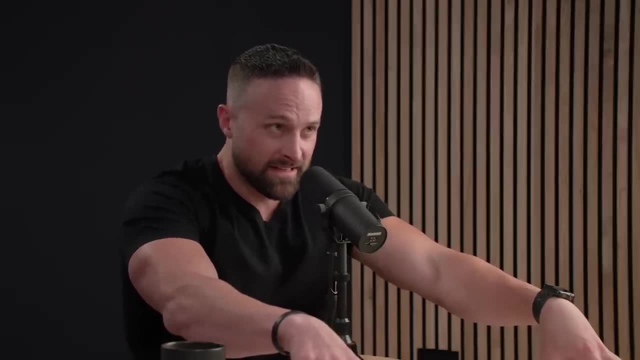 is looking at. basically the entire glucose response was not different between the control and the sucralose group. To me that's the biggest take home. There was one time point at the end of the study In the sucralose group, the 30-minute time point. that was statistically significantly. 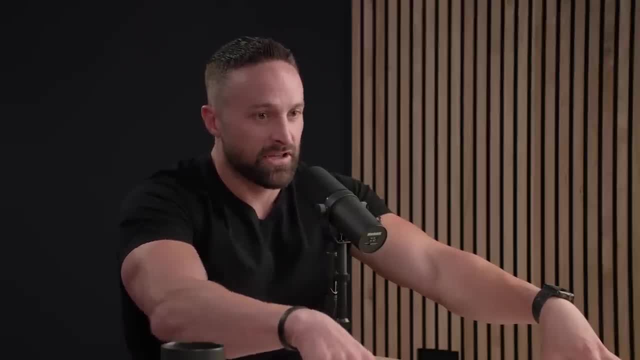 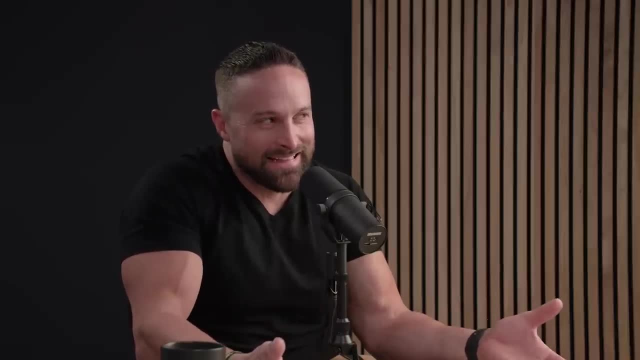 higher blood glucose than the control group. It's kind of one of those things where I go: OK, it was one time point, It's statistically significant. But even then we've seen things be statistically significant that end up being data artifacts because they're not reproduced. 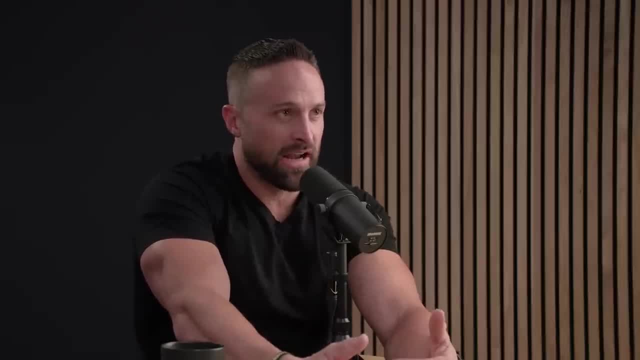 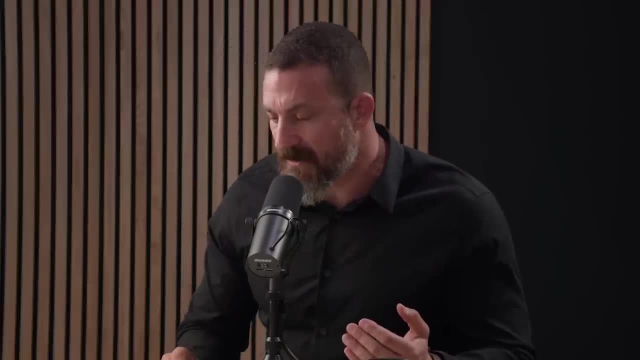 So I'm not saying that's what's happening here, But again, the overall area under the curve was not different. So to me that was the biggest take home. And papers- Papers we should probably mention- are published because of effects generally. 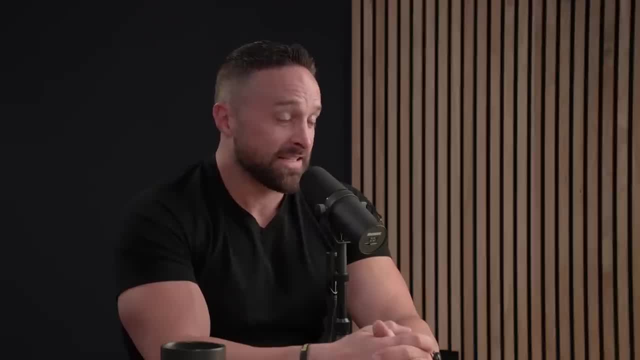 Lack of effect harder to publish Null hypothesis doesn't? it's actually really unfortunate, because a null hypothesis is just as useful data as the non-null hypothesis. But you're right, There is a very strong publication bias towards showing an effect versus not. 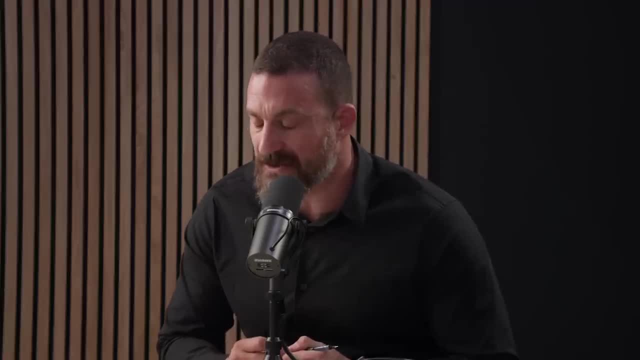 Yeah, unless you can flip a field on its head entirely by showing something did not happen, And typically The positive result out, does the negative result in positive meaning you see a result. And then of course, it's one study And I think that, as you talked about earlier the center of mass of data in a given field, 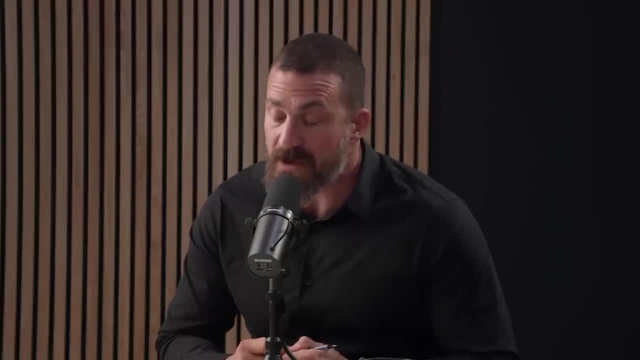 are probably the best basis for what we should do in terms of, And so I'm not changing my behavior around the intake of artificial sweeteners. I personally am still going to consume stevia and aspartame in relatively small amounts, Yeah, But now I'm thinking: well, OK, if something contains sucralose, I don't have to. perhaps 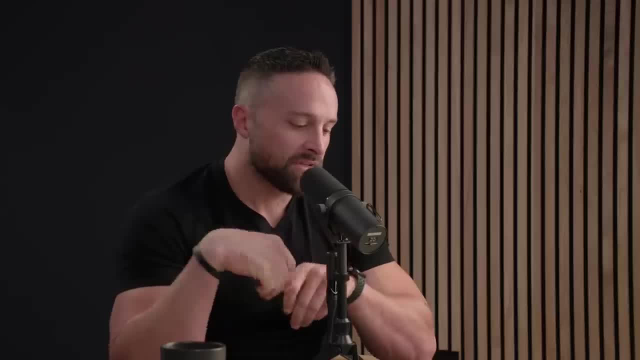 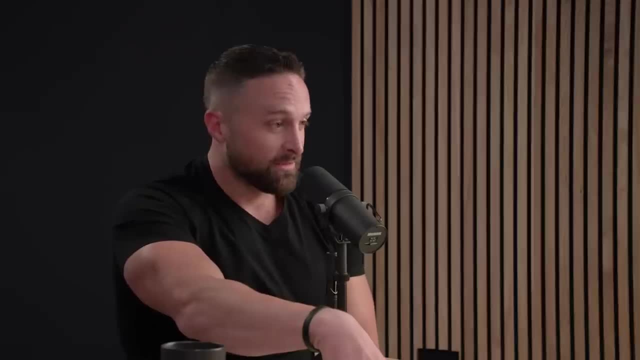 actively avoid it, whereas before I was I was actively avoiding it. So the new study I thought was, very elegantly, very involved. I mean, be quite frank, some of the animal stuff they did was extremely impressive. So there was actually two arms to the study. 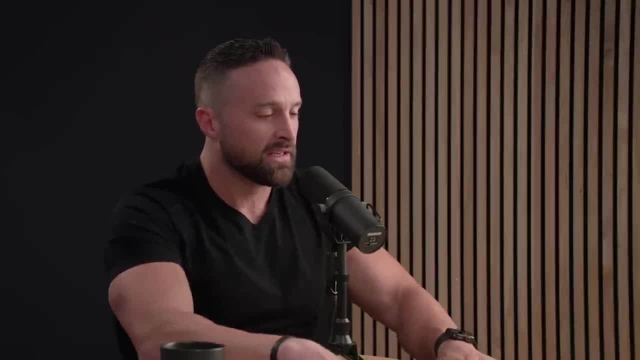 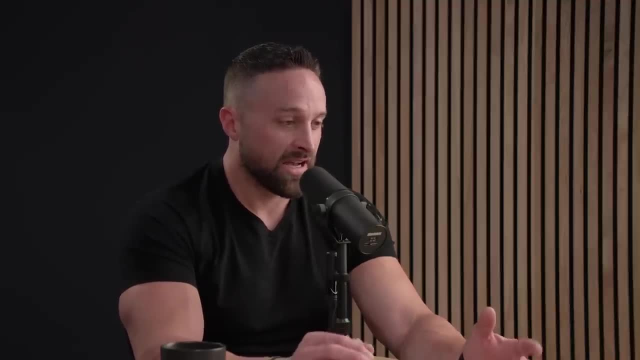 One was a human arm, one was the animal arm. I focused much more on the human side of it. So basically, this was a two week study And the really unique aspect of this, which I think is both a strength and a weakness- 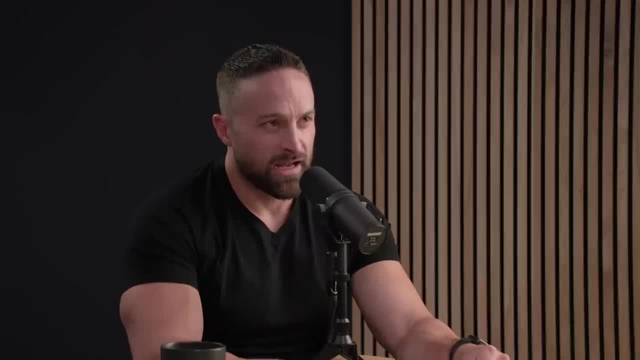 they had almost 1400 people apply for this study and they only had 120, I think that actually went into it because they did a very detailed food analysis of these folks. All these people said that they avoided artificial sweeteners or didn't consume them. 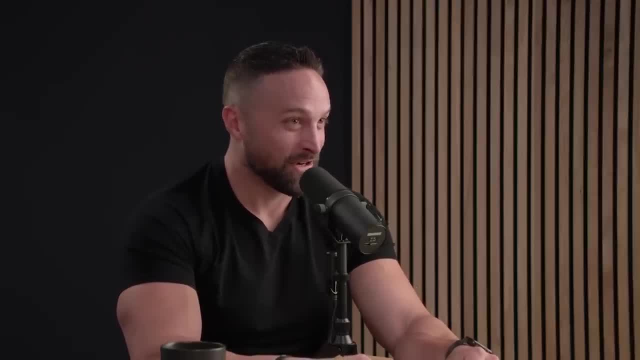 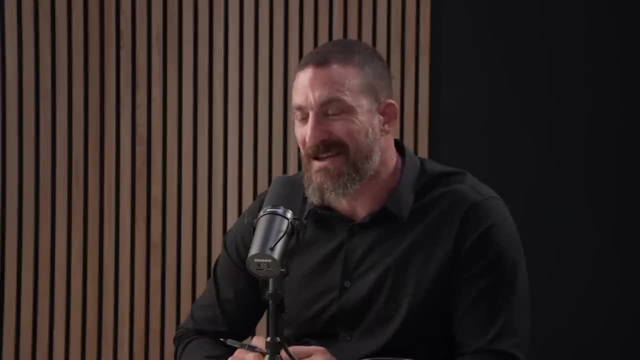 And I think people don't realize how ubiquitous sweeteners are. Prior to the study, these people were like it was like jury select And they had never- it's like not ever- hearing of the plaintiff and the defendant. These are these mutant people who have never had an artificial sweetener. 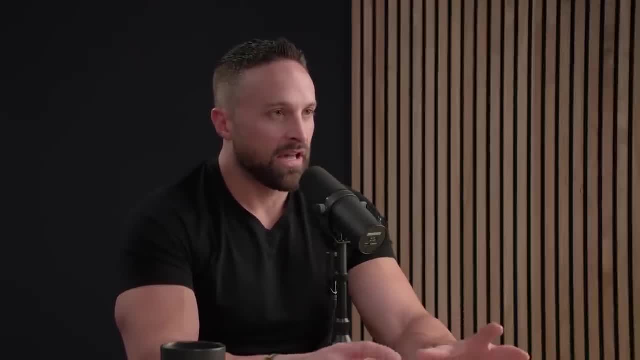 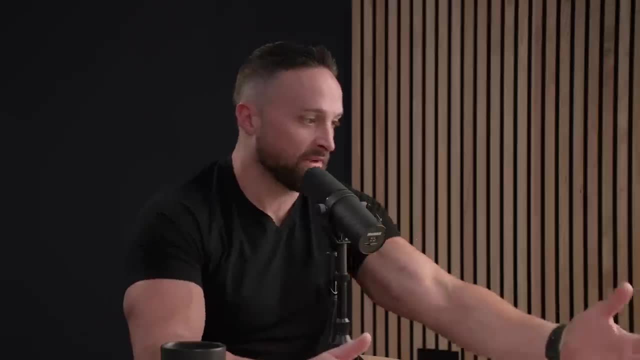 Right. So the strength is now you don't have a lot of like pre-existing, you know effects that may be clouding what would actually happen when you add it in, Like, for example, if you have people who are already consuming artificial sweeteners. 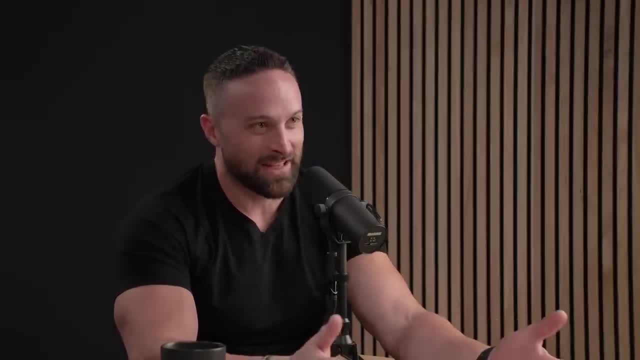 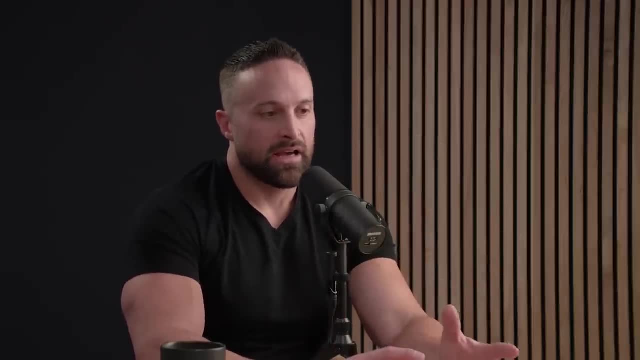 and then you have them consume artificial sweeteners. the likelihood things are going to change is pretty low, Right? So I think that that's a strength. It's also a weakness, And I want to be really careful, because I think people took my words a little bit too. far, which means I probably didn't do a good job of being nuanced enough. There is the possibility for a placebo effect here. So to me, if somebody has gone through that much painstaking care to avoid artificial sweeteners, it's likely they have a preconceived notion that those are bad for you. 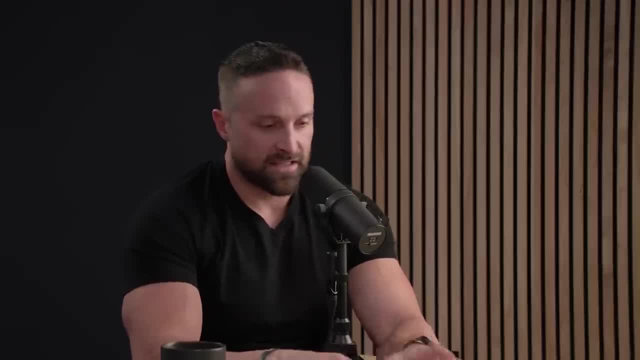 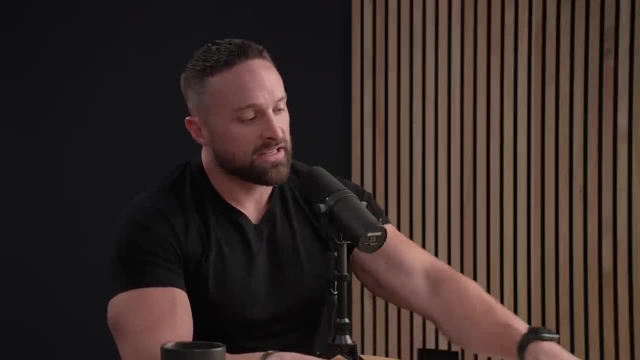 Like to, because they're difficult to avoid. Um, yes, it's possible, if they're eating a very minimally processed diet, that they're just not exposed to them, And that's very true as well. Uh, but the other thing that the researchers acknowledged was they weren't able to blind. 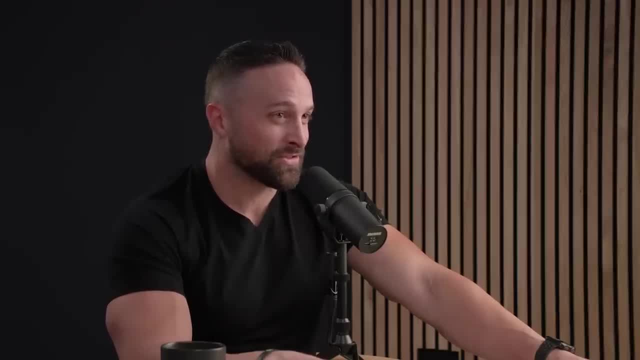 the study because if you've never had an artificial sweetener before- you're only used to like regular sugar- and you have an artificial sweetener, you know you taste it. you know um, it's still sweet, but it's not the same sweet. And there's an interesting effect there where a lot of people don't like the taste of aspartame the first time. Yeah, I actually quit drinking diet soda for a while, thinking I should, And then and had one. it tasted really. I can only describe it as kind of artificial chemical. 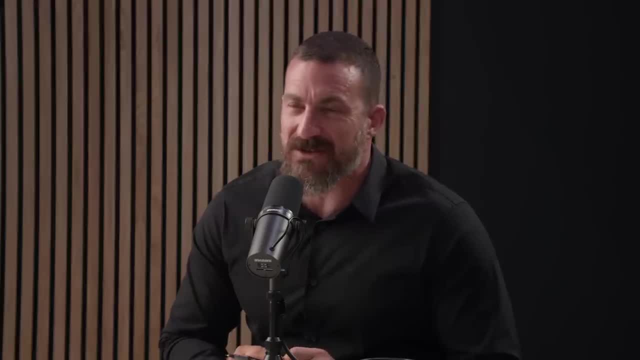 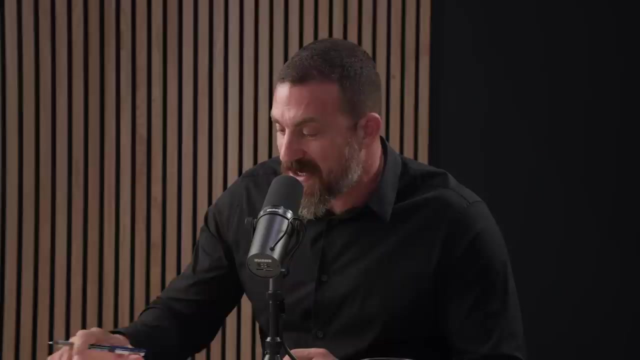 and then pretty soon tasted great again, Yep. And so there is some attenuation there, and whether or not that's central meaning within the brain or peripheral, I don't know, but very interesting. Well, I I see you as playing a critical role in defining what is and what isn't, what still. 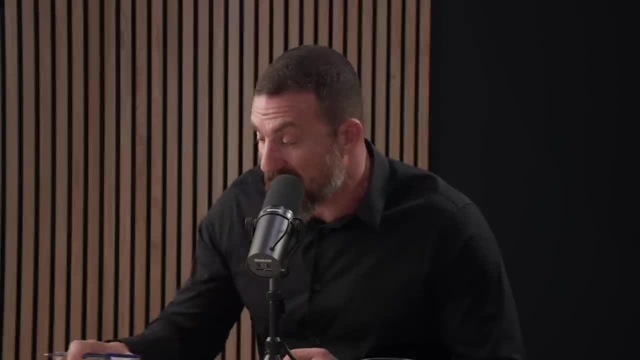 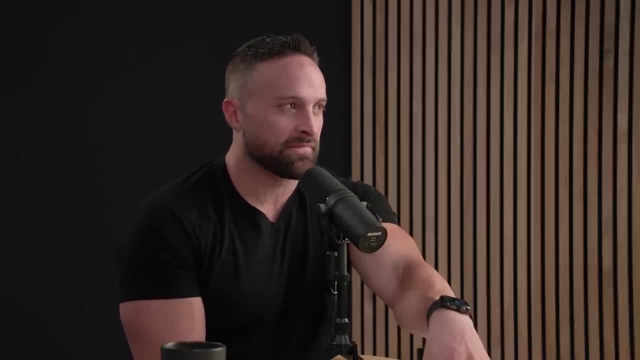 needs to be determined. um, in terms of this landscape and the entire landscape, really, of nutrition, And that study did change my opinion In terms of, okay, I, I, I think we can clearly say now that, like, these aren't, these aren't. 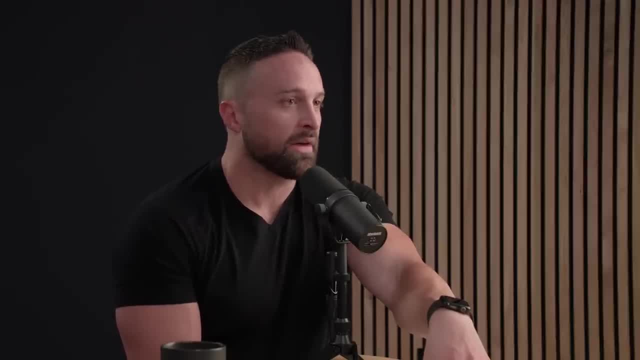 neutral or sorry that they're not inert, right Like that. that was the thought process before. it was well, they're not digested or whatnot, So they they must be an inert. that doesn't appear to be the case. 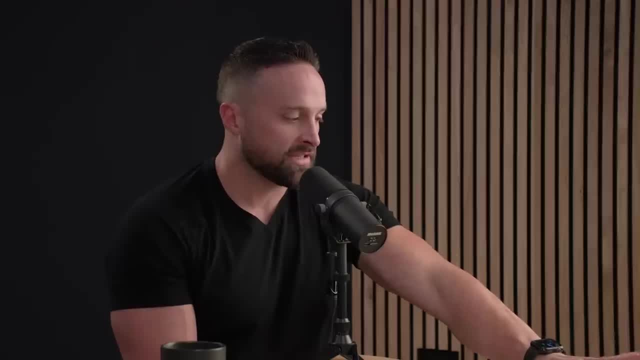 Um, but again, like when we look at the, the blood glucose data there's and I'm not saying this is what happened. I want to be very clear: not saying this is what happened, I'm saying it's possible. 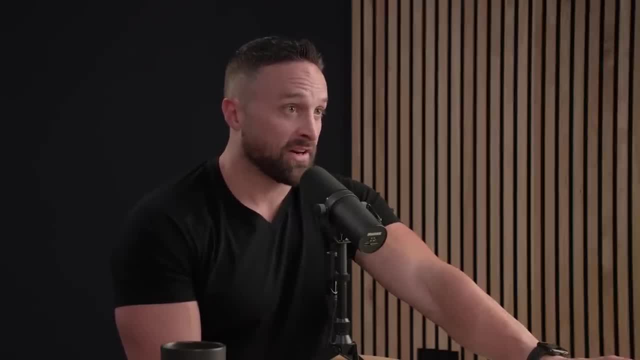 This happened, And so this is why we need more studies to verify if these people had a preconceived notion that artificial sweeteners were bad for them. it's possible, knowing they're ingesting artificial sweeteners, that they could have had a a blood glucose response. 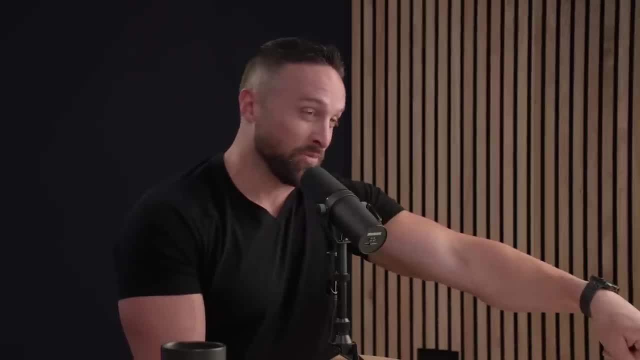 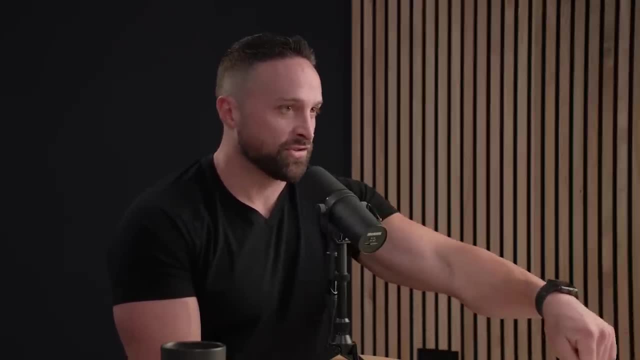 Now the my pushback on my own point there would be, then we should have expected to see it in all the art and all the non-nutritive sweeteners, which they didn't. It was just in sucralose and saccharin. 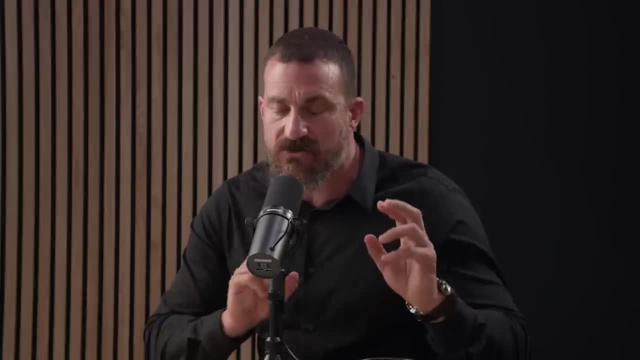 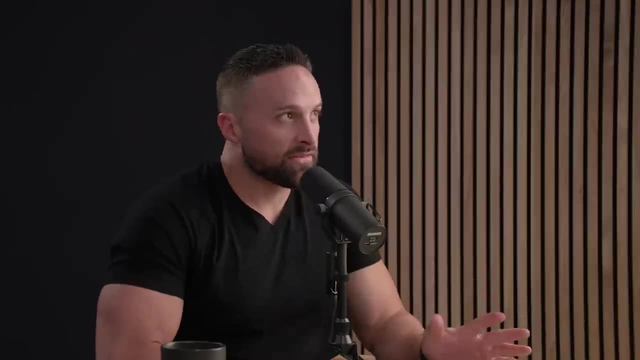 It was kind of a graded effect where sucralose and saccharin showed the most dramatic change. Um, and stevia and a few of the others did not, And the other. the other issue I took with it- maybe it's a ticky tack thing- was their. 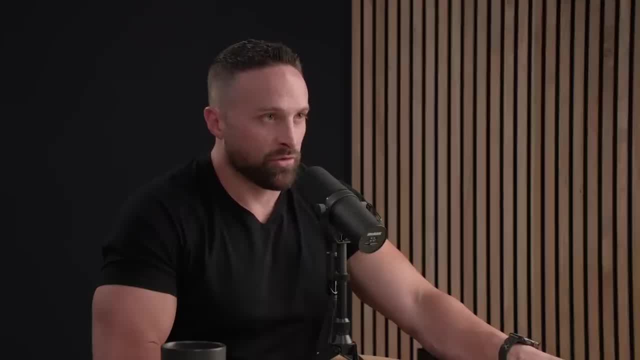 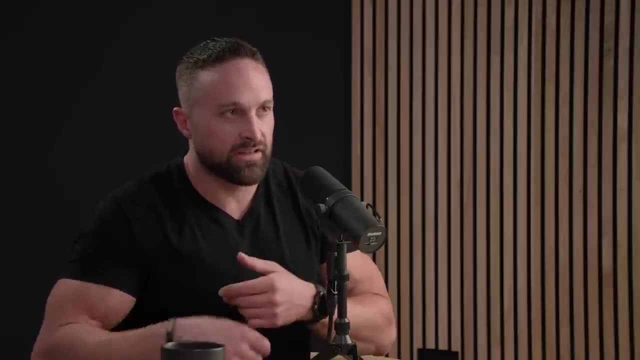 primary outcome measure was uh, blood glucose- of the oral glucose tolerance test, but they had people administer their own oral glucose tolerance tests which basically they gave them. they said, okay, drink this drink. And they were wearing continuous glucose monitors, which should have been fine. 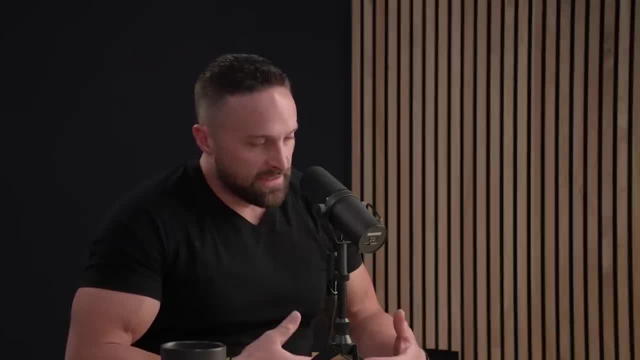 Um, but again to me, and I'm I'm being ticky tacky And again, I know all studies, Studies are limited by funding. So I think, overall, this was a great study, but I would have liked to seen them, uh, you. 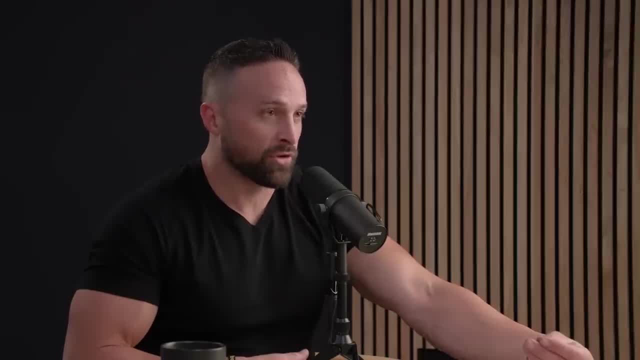 know, monitor the, the um oral glucose tolerance test, to administer it before or after. you want to know that they didn't ingest this or didn't ingest that. Yeah, Those those two things, But the other one of the caveat is it was a two week study, right. 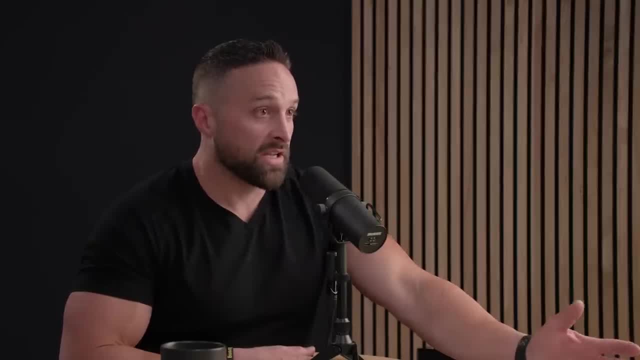 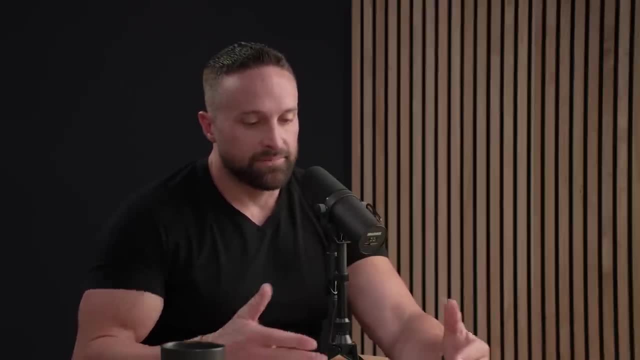 So we've got to be really careful how much we interpret in this, because it's also possible that this is a transient effect, right, And maybe it goes away over time. We don't know, But again, I think it's. we can clearly say it's not inert, right. 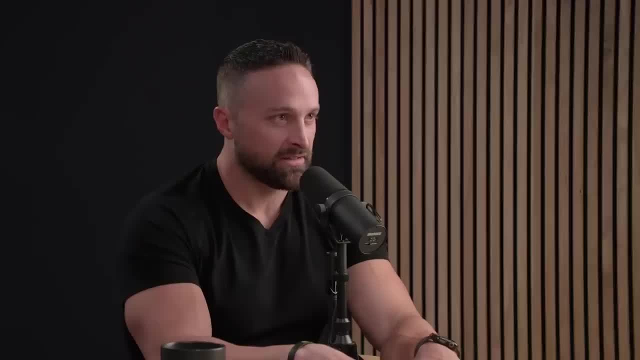 Now how much emphasis we put on that, on a two week study, I, I'm, I still will say: okay, maybe, if you're worried, don't consume sucralose, right, But if you're, you know, a hundred pounds overweight and you want to use some sucralose, 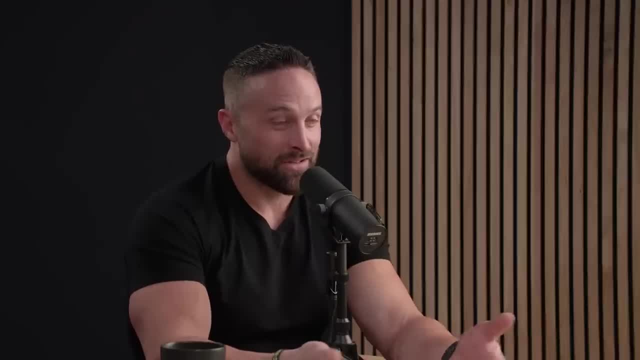 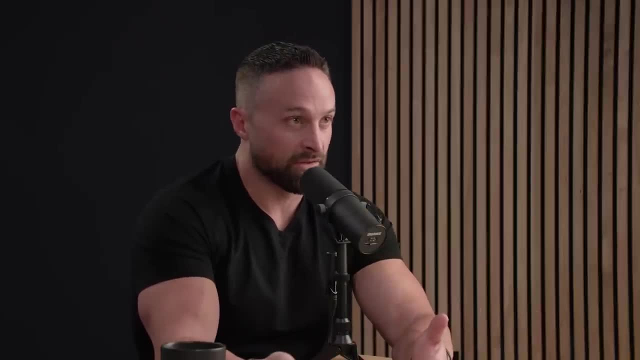 as a replacement To help you lose weight, I would say: don't let this study deter you from doing that, because the net effect is still going to be more positive than you not losing the weight right. So if it's a tool that helps you, fine, but I do hold open the idea that well there. 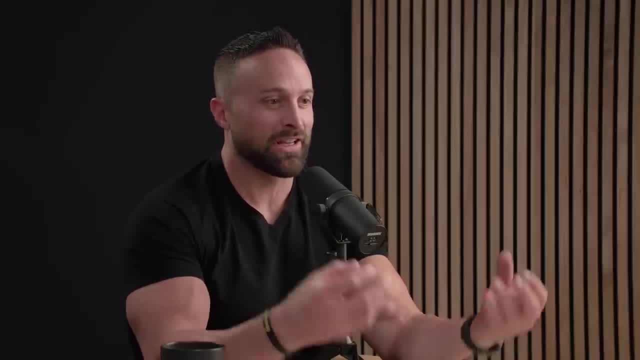 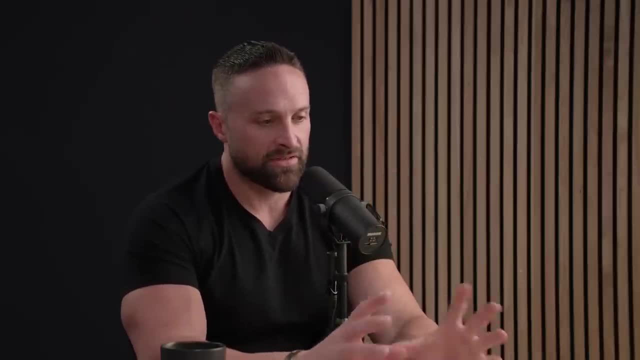 could be negative effects from it as well. But again we're we're looking at like: what's the what is the overall outcome, right? And then when I looked at um, they examined like some of the different things that were. 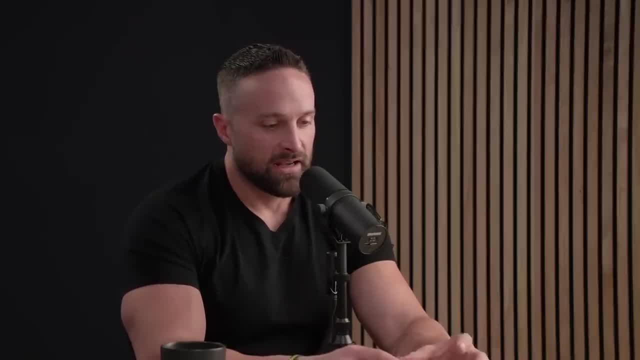 increased with these different, uh, sweeteners- And again, this word gets messy, because one of the things I saw was a big increase in butyrate production from the change in the gut microbiome, presumably. Well, as we discussed earlier, butyrate is actually associated with like positive outcomes. 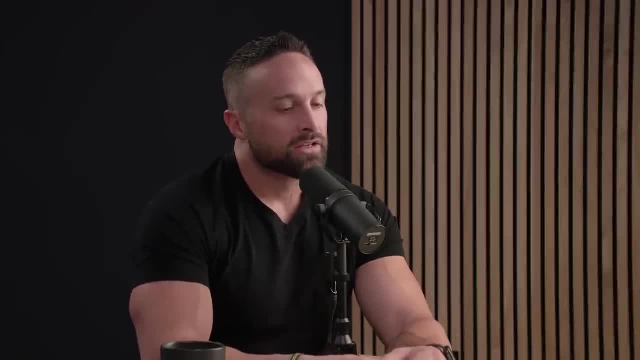 in terms of insulin sensitivity, inflammation and some other things. So I just I want to be real cautious before people say, well, there's a change in the microbiome, It must be a bad change. We don't know. it's possible. 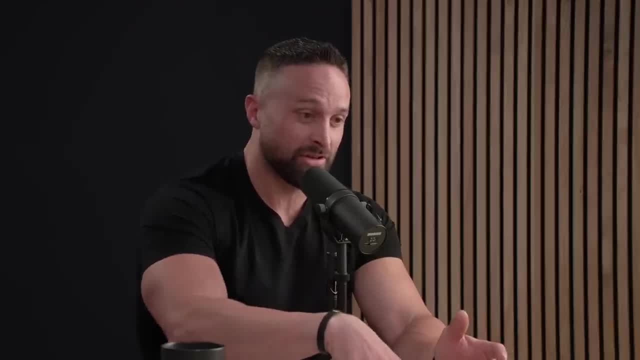 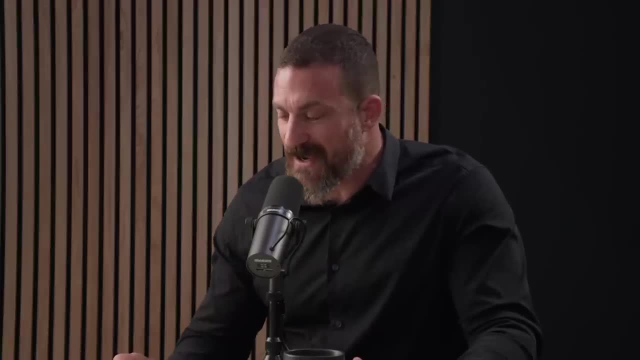 And again, if we have, you know, 10 more studies come out and start to show this, then I will start to shift my My personal opinion of artificial sweeteners. So, in anticipation of sitting down today, I did solicit uh for questions on social. 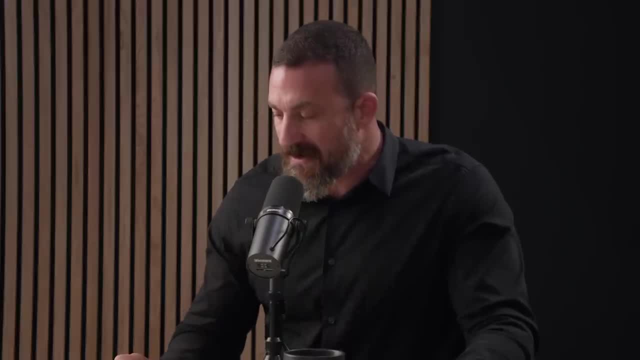 media And one of the questions that got a lot of upvotes, uh likes if, if you will- was it one that I think raises interesting questions about short-term and long-term health, And it's the following: I think it's a common scenario: 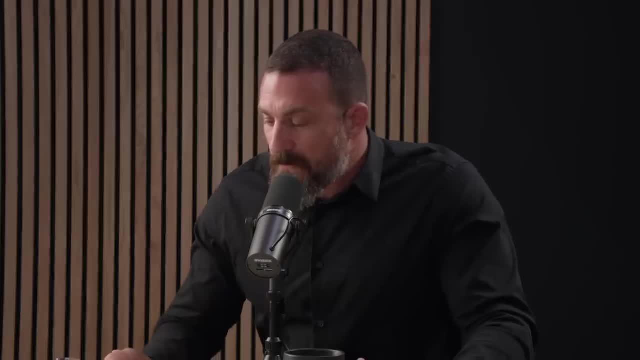 A number of people want to know what is the healthiest way to approach a kind of a healthy, kind of rapid weight loss. And here what I think is happening is somebody has an event coming up or they're just tired of being- uh, the weight they are carrying, the amount of adipose tissue they are. 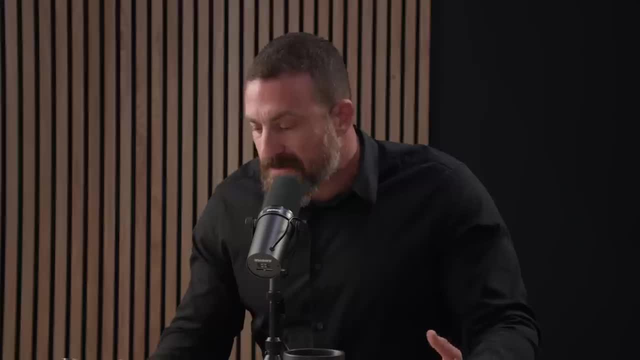 And they wanted to know whether or not it is safe to, for instance, lose three pounds a week for a few weeks in anticipation of a wedding or some other event, and whether or not straight caloric restriction and increasing activity uh is the best way to approach. 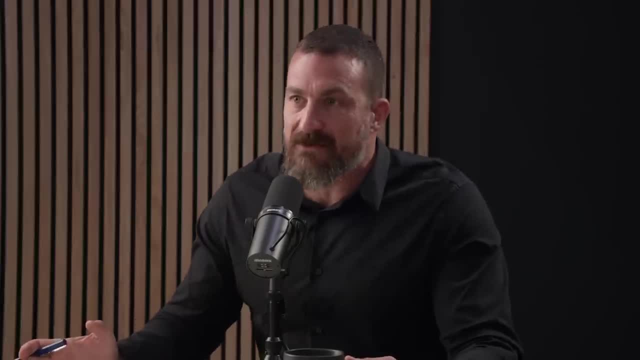 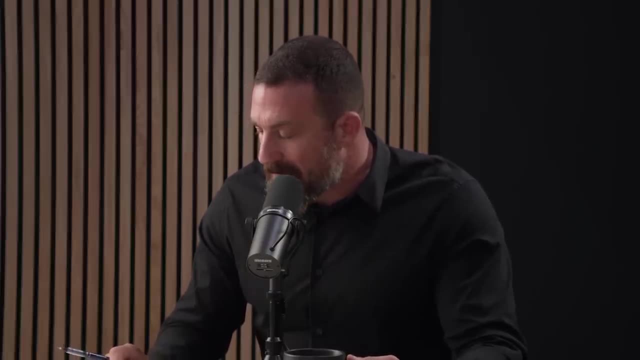 that, Um, with the understanding that they may gain back a little afterwards, they might make. I think, ideally they'd like to maintain it afterwards. But what do you think of that sort of approach? Uh, you know, cutting caloric intake in half, for instance, and then doubling, and also doubling. your physical output. So it's interesting- because the you might be surprised by what I'm going to say, which is the research data actually tends to suggest that people who are like obese, who lose a lot more weight Early, are more likely to keep it off, which seems a little bit kind of contradictory. 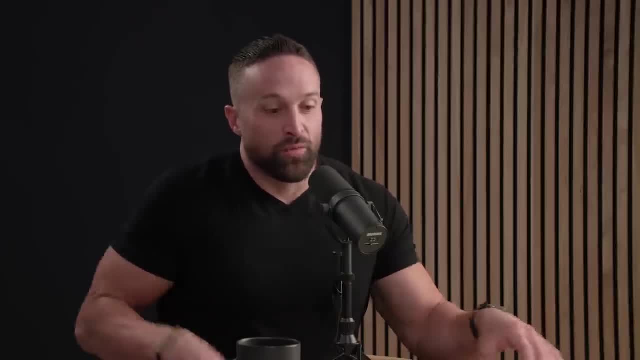 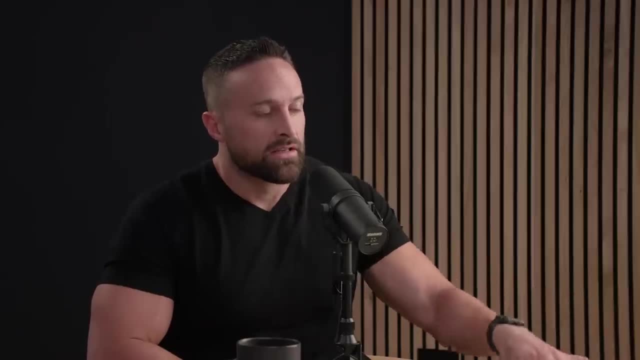 right, Like well, that doesn't seem very sustainable. but again you're, you're weighing, competing things. So there's sustainability aspect. but then there's also like buy-in is huge for sustainability, right. So for a lot of overweight or obese people if they start a diet and they don't see something. 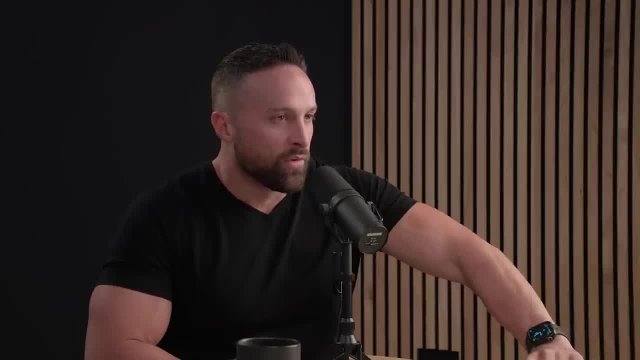 quickly. they kind of bail on it because it's you know it's not working, Whereas if they see some rapid results pretty quickly, they buy in even harder Right. And so I think the the conversation, especially for if there's any coaches or trainers out. 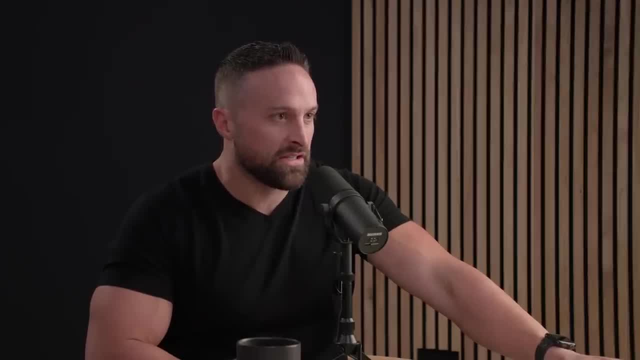 there is just presenting that as the they're. you know, one of my favorite lines is: there are no solutions, There's only trade-offs. I think Thomas Sowell said that. So you're, you're having a trade-off here. 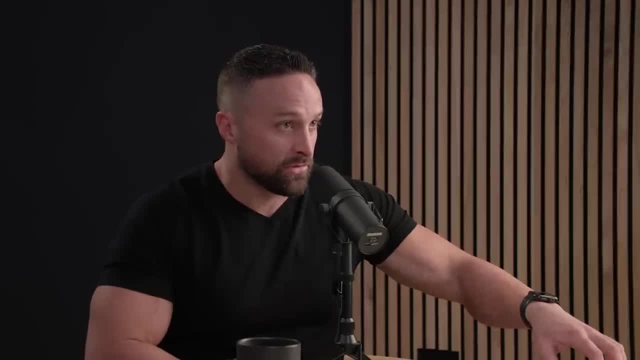 It is. yes, you're going to lose fat faster. You might lose lean mass a little bit faster too, which can be a problem. But I will say: the more adipose tissue you have, the more aggressively you can diet without negative. consequences. Somebody like me. doing a really aggressive diet is not going to be good for my lean mass. One: I have a higher lean mass than normal. Two, I have a lower body fat than normal. As your body fat goes down, the percentage of weight loss from lean mass goes up. So people who are very obese, because they have so much adipose tissue to pull from, there's very little reason for the body to catabolize lean tissue. Now, that being said, if you go on a people misinterpret like they're like well, I. got an in-body done and or a DEXA done and I've lost, you know, two pounds of lean mass and they've, you know they've lost 20 pounds overall. Well, keep in mind, adipose tissue itself is 13% lean mass. So there's actually, like you know, protein component, to like the structural component of the adipose tissue, And it does have some water. So it's about 87% lipid, but the other part is lean. So at minimum you should expect a 13% reduction in lean mass when you diet. And then when you consider like you lose body water overall, which is registers as lean mass, and you lose your splint, neck tissues can shrink a little bit, So it's normal to lose. you know, for the average person to lose like 25 or 30% of the. 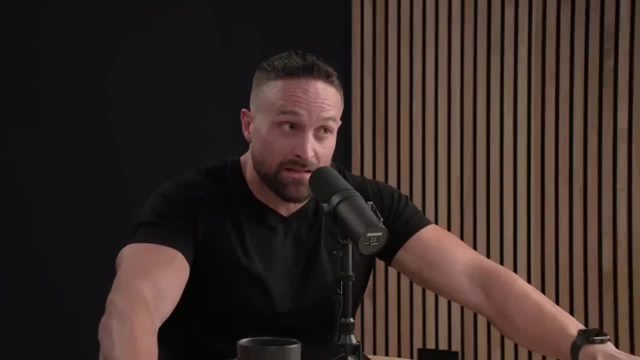 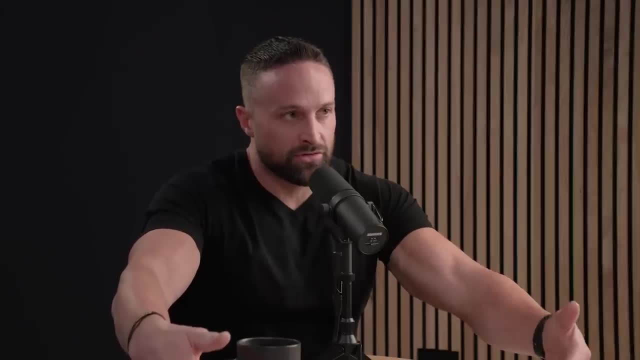 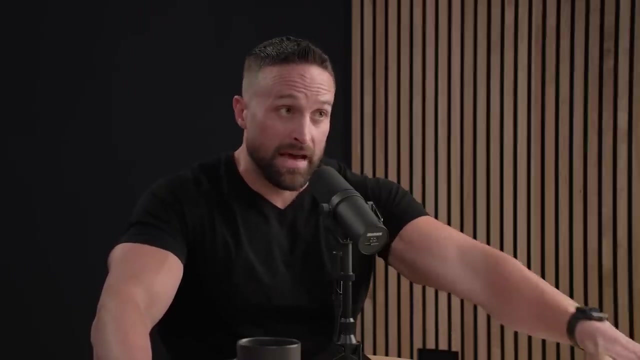 weight that they lose from lean mass. But that doesn't mean skeletal muscle tissue. And again, the the more adipose you have, the more aggressively you can approach the diet without really negative long-term consequences to lean mass or your overall health. but balance. 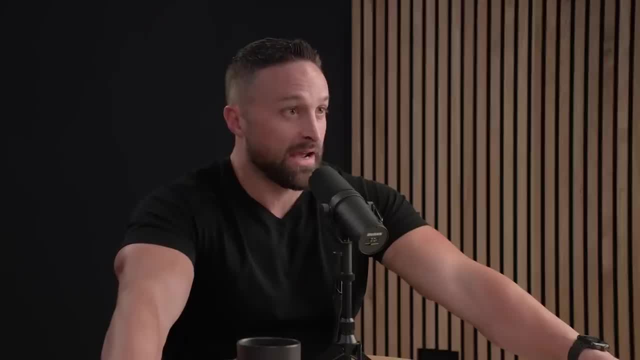 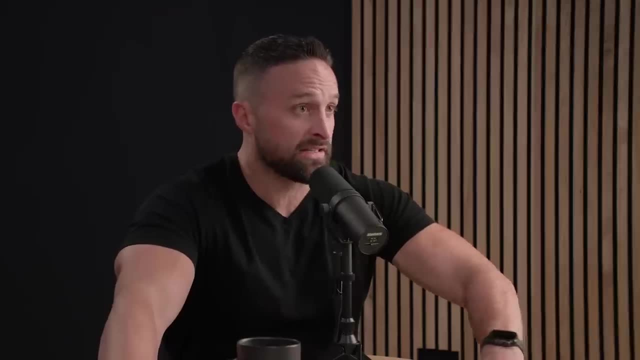 that with: okay. if I'm going to do this, I need to understand that I'm not going to be dieting this way forever. I'm doing this to give myself a boost at the beginning, And I have to be okay at some point with transitioning to something that's a little. 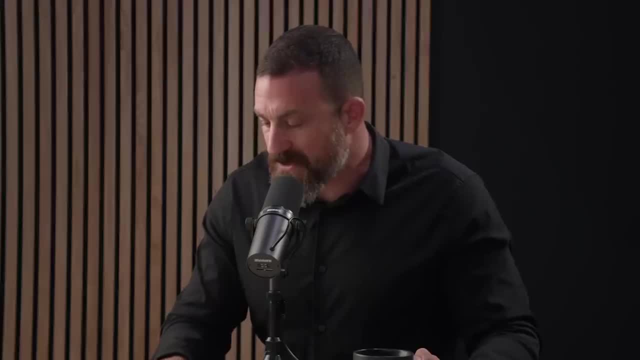 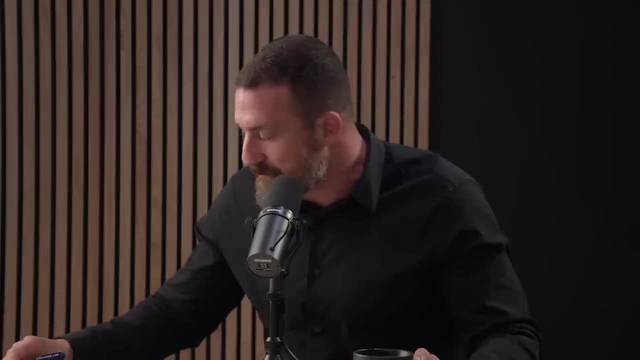 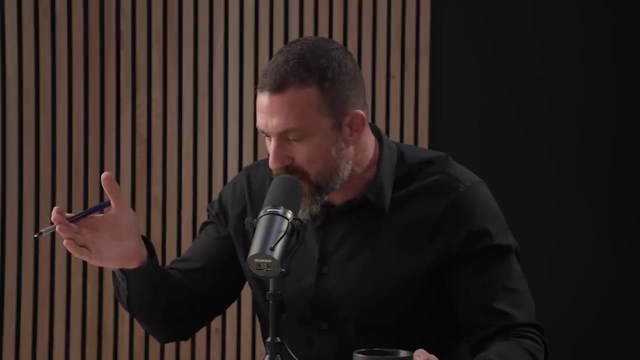 bit more sustainable. Based on what you just said. it reminds me of the- uh, satiety signal effect of exercise. You mentioned earlier that exercising can improve, um, our sense of when we've had enough to eat. I just want to briefly mention that when Allie Crum was on the podcast, she mentioned that 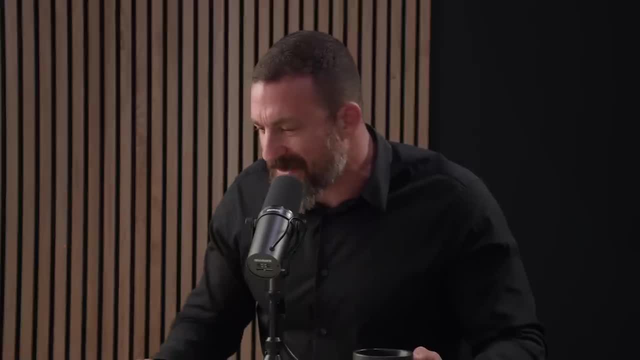 they'd been doing a study that I I have to pair you to and have a hear the conversation as a fly on the wall, because what she was telling me was that if people believe that a food is nutritious for them, then eating less of it uh registers. 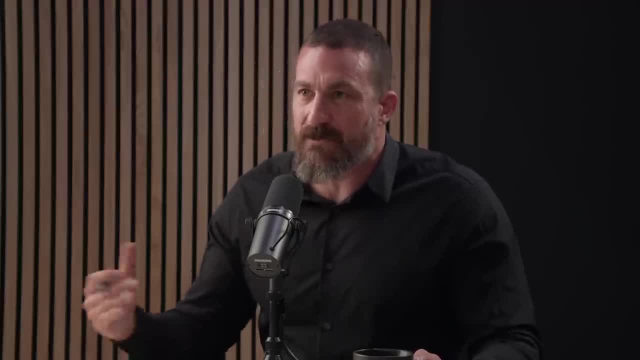 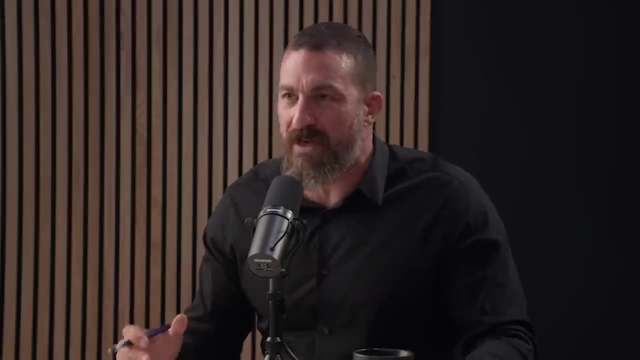 As more satiating, Whereas if people view dieting as a deprivation system, you know like, oh you know, dieting is hard and the food sucks and it's terrible, Well then they crave all sorts of other things, Whereas they could. they actually observe in their studies, where people report reduced 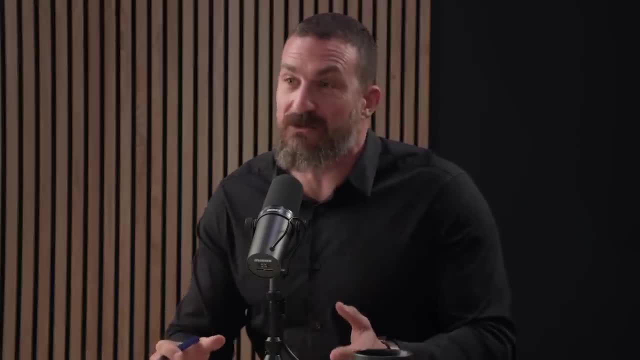 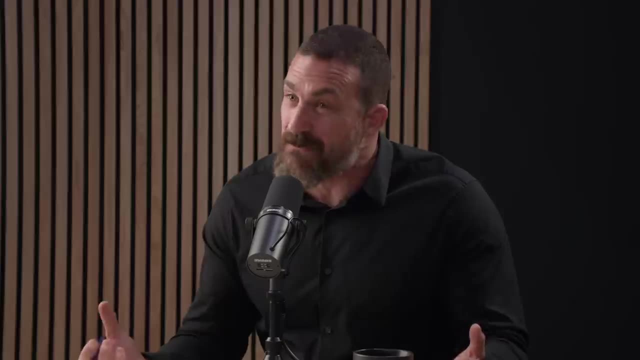 craving. If they are told, for instance, a chicken breast and broccoli and some olive oil and rice is actually quite nourishing, It's actually really good for you, Then people eat that and they feel like they've actually eaten more. The satiety signaling goes up. 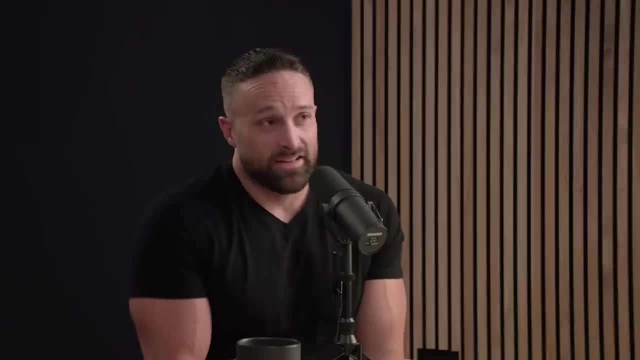 So it's just a just a point that Allie made. uh, those aren't. my data is so impressive because even the rate at which you eat and right down to the size of the plate and the color of the plate, like the contrast in color, they, they see. I can't remember exactly. 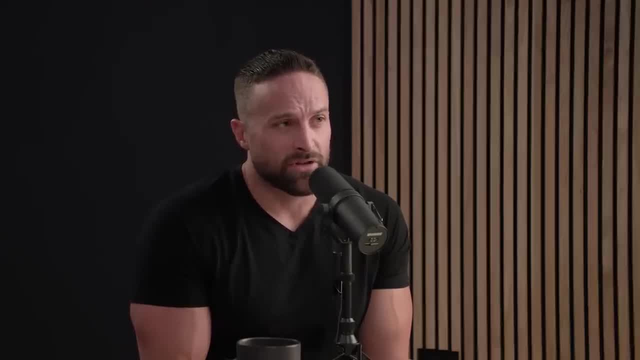 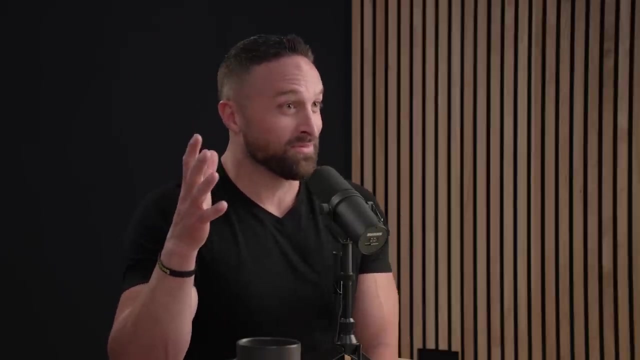 I think it's. if the plate is a similar color to the food, I think people eat more, Whereas if it's a bigger contrast, they eat less. So even like, plate color can make a difference on how much you eat. So again, human brain, very amazing, but also very dumb in some ways. 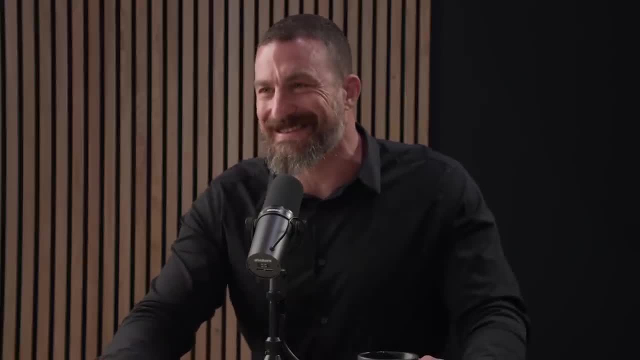 Right, Like not an optimized algorithm. I always, I always joke with people. I'm like just look at how stupid humans are. You put some water in front of them, like you know the ocean. they're like, oh yeah. 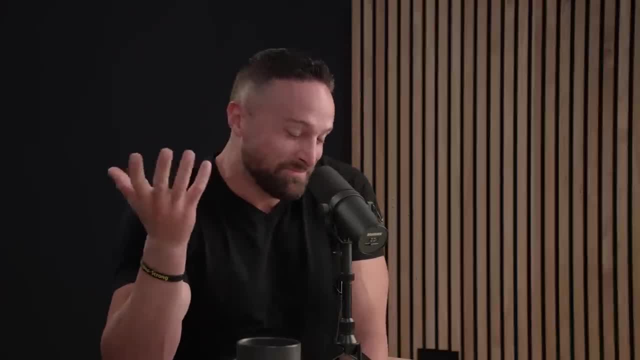 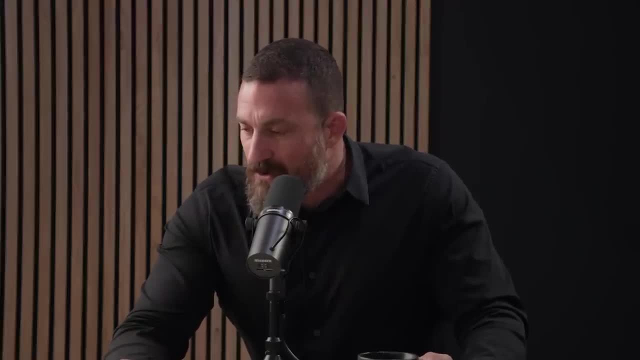 I'll pay 10 times more for this, you know Like, but it's just we're kind of wired that way. The um the reward signaling pathways in the brain run one chemical, mainly dopamine. There are others, Of course, but and very few algorithms. 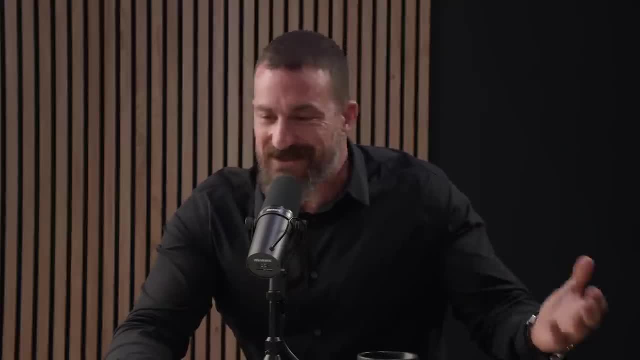 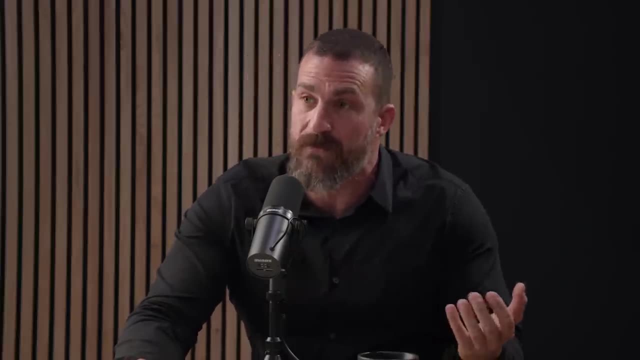 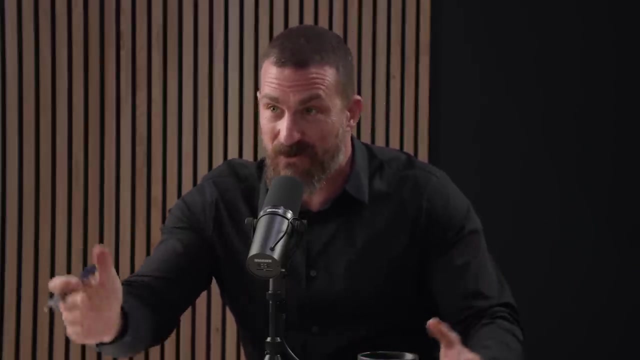 It's sort of like a intermittent reinforcement is one random reinforcement, but in the end that there aren't many algorithms and we, we are probably not optimized, certainly not optimized for our own health, because people will eat themselves to death, drug themselves to death, et cetera, simply because something felt good at one point. it's. it proves your. 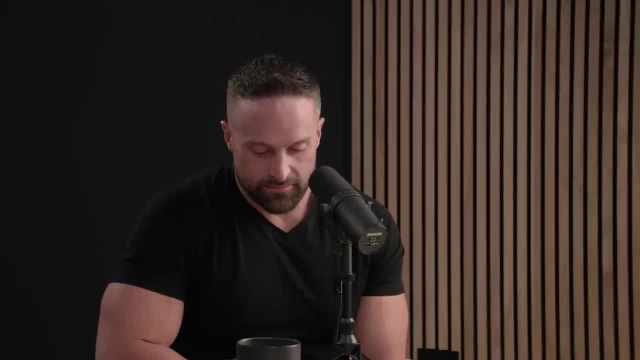 point. One of the things I tell people- I said this on um Andy for solace podcast- was, interestingly, the dichotomy of life. Yeah, He said, if you do what's easy in the short term, your life will be hard. 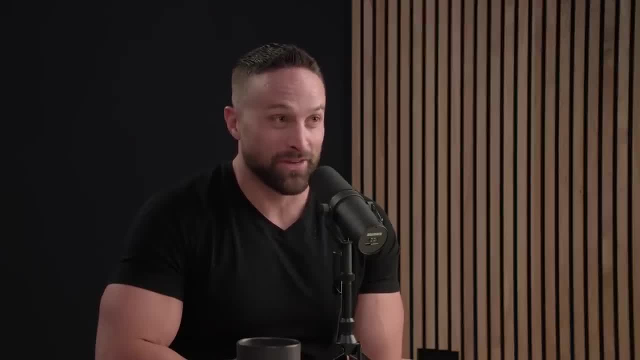 If you do what's hard in the short term, your life will get easier. It's very strange, And actually Ethan Suplee had a great example of this when he was over 500 pounds. he said the amount of work I had to do to construct my life that I could just live was so much. 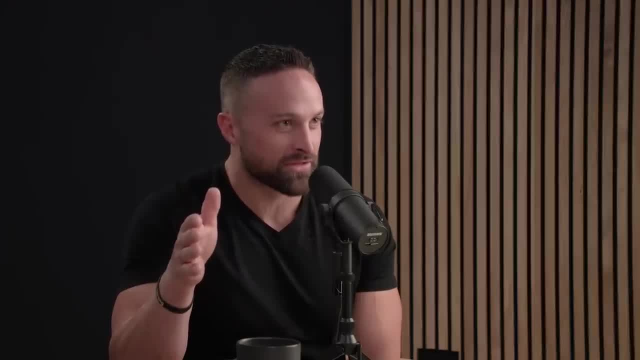 more work than just going to the gym for a couple hours a day. He's like. the gym work is hard, He's like, but when I look back, how much work I had to do to sustain that lifestyle versus just going to the gym and 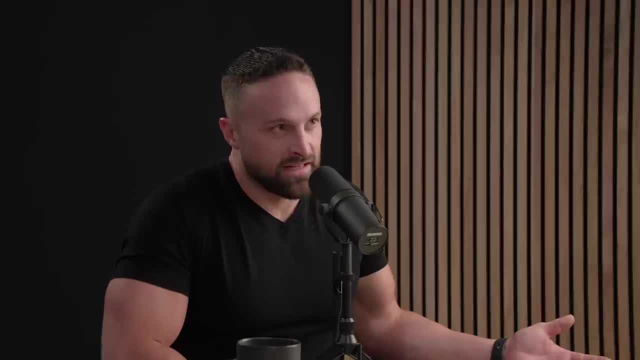 like you know, restricting calories he's like to maintain the lifestyle of being 500 pounds was infinitely more difficult than what I do now, And so again, again, a great example: short-term, hard, going to the gym, calorie restriction. 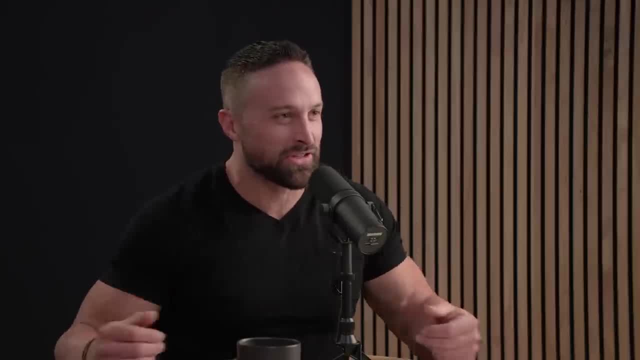 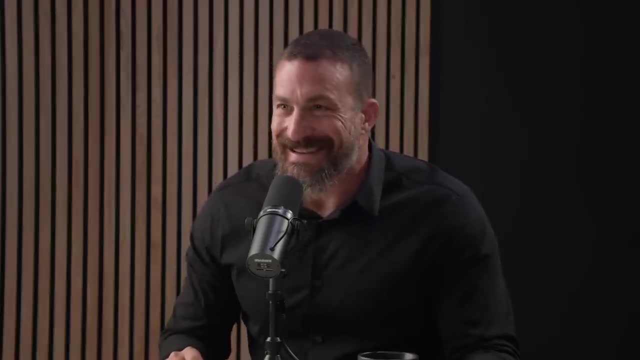 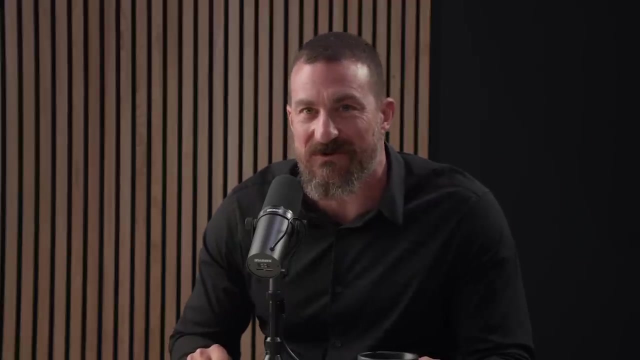 long-term life's easier. Just really interesting dichotomy. I think about a lot And I can't be restated often enough. And I think about a lot Seed oils. People want to ask about seed oils And for those of you that are listening who are wondering why, we're sort of chuckling. 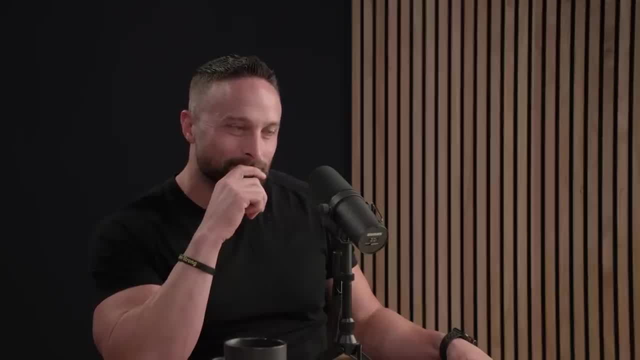 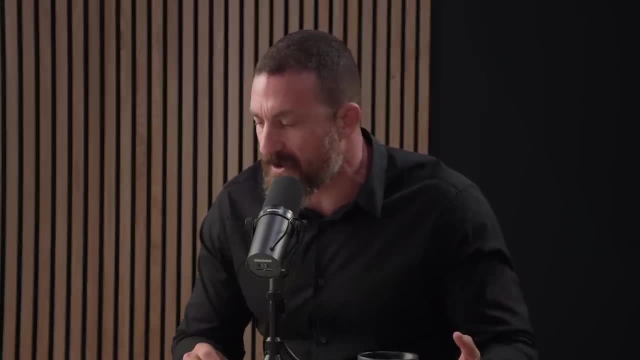 already. she mentioned that, both in the Twitter sphere and Instagram and online, that there's these very polarized views that probably aren't worth focusing on for too long, But there are a number of folks out there who are arguing that seed oils are the source. 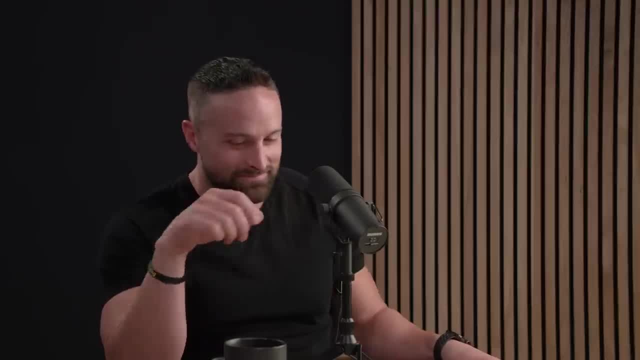 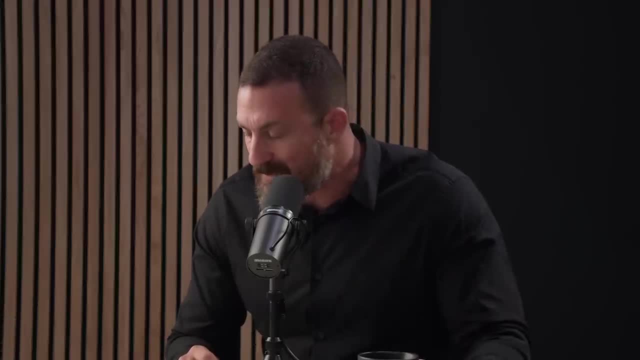 of all. you know, the obesity, epidemic, inflammation, et cetera, Illuminati, Everything. And then there are those that would argue just the opposite, that, you know, meat is the source of all problems, et cetera. 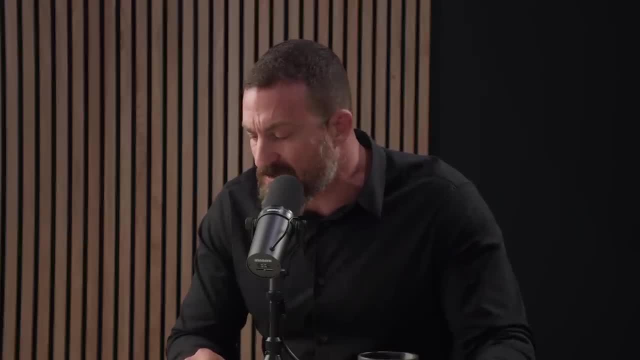 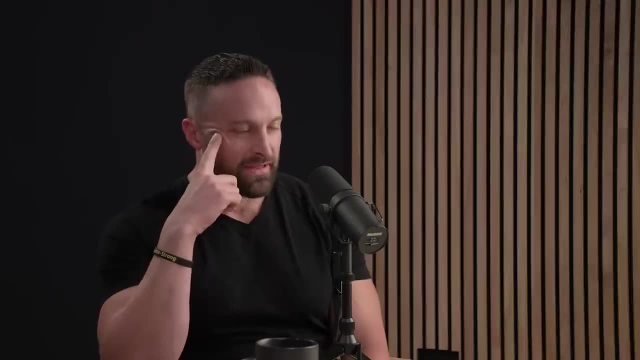 And I think we've- thanks to your nuance and expertise- we've hopefully appropriately framed things- that it's never that black and white. It's simply not Rarely. Rarely. I love olive oil. I realize that doesn't fit exactly into the seed oil category. 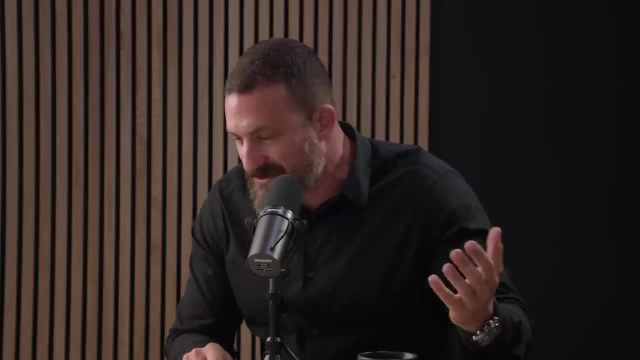 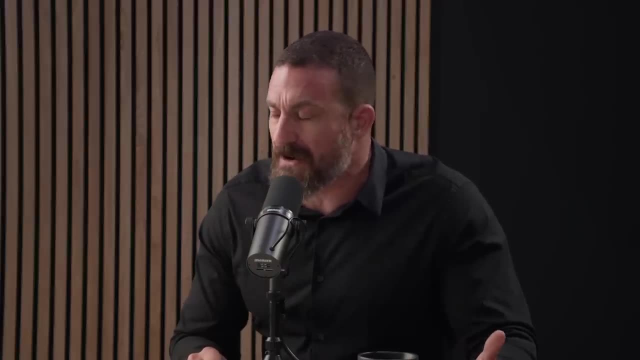 I love olive oil. I use it in moderation. I do also consume some butter in moderation. But are there any data on seed oils? And here a good example, I think would be like canola oil, which comes from the rape seed that literally was renamed canola oil, because rape seed oil is not good marketing. 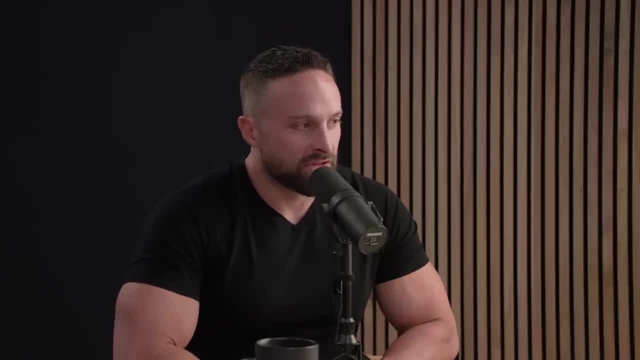 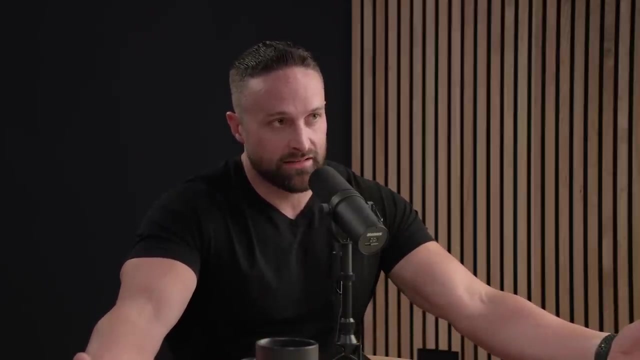 No, no, exactly. So the first thing I'll say is seed oils have negatively contributed to our overall health because people in the last, you know, 20,, 30 years, What they have tended to add into their diet, that has increased the overall calorie load. 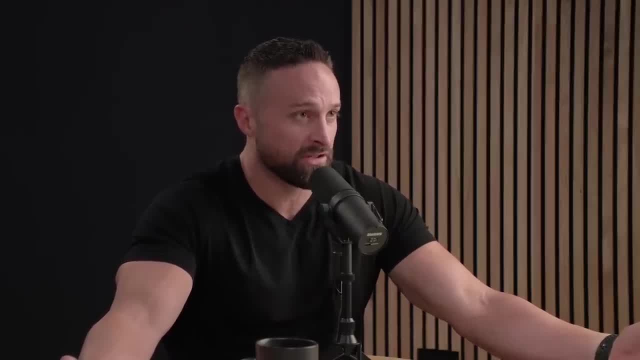 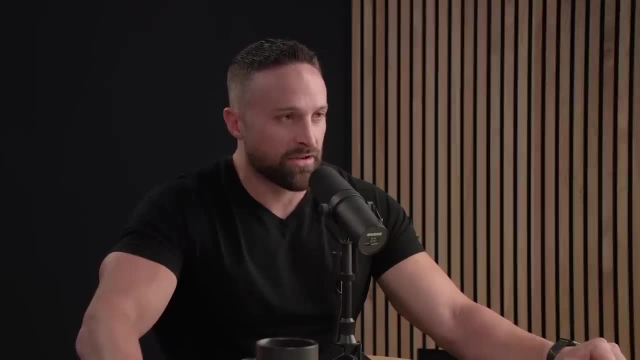 is oil like these, various, mostly from seed oils, But when we look at like one-to-one replacement with other fats. and so I, if you look at the epidemiology- yeah, you can find some epidemiology showing people who consume more. 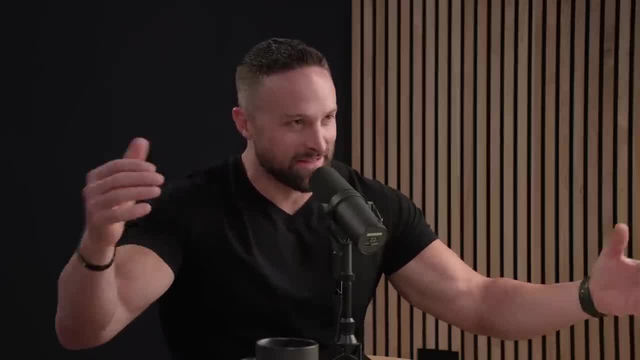 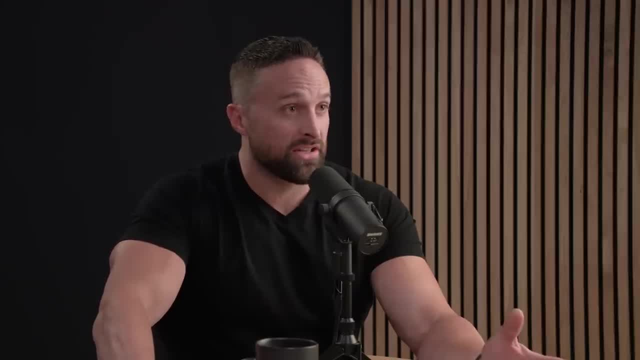 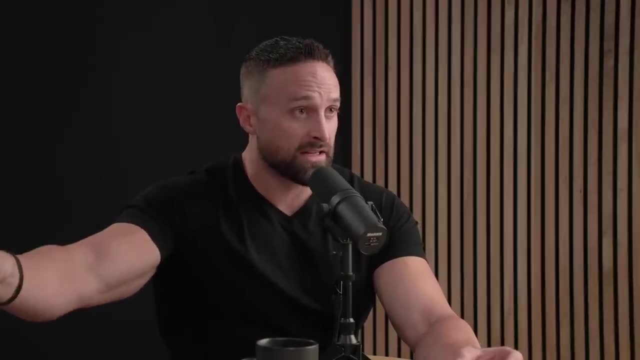 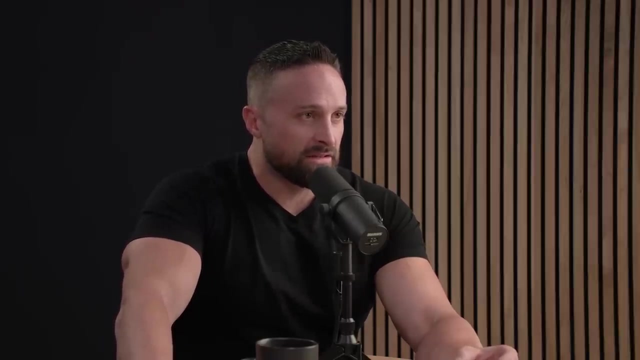 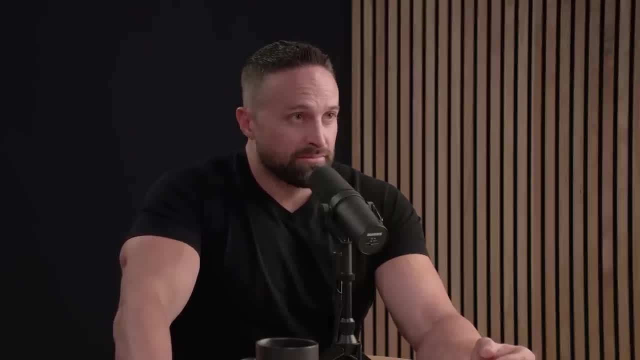 So that's a plausible mechanism. So, as always, I defer to the human randomized control trials, and so what you tend to find is when you substitute polyunsaturated fats or, sorry, when you substitute saturated fats for polyunsaturated fats, it's either neutral or 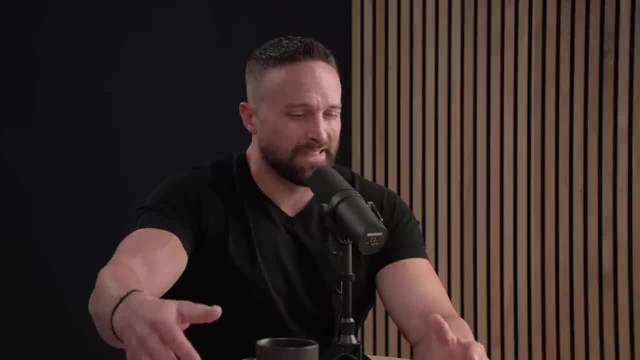 positive in terms of the effects on like inflammation is basically neutral. there there's some studies that show a positive effect of doing uh, polyunsaturated fats, but it probably depends on the individual polyunsaturated fat, and that's the other thing i don't really is difficult. 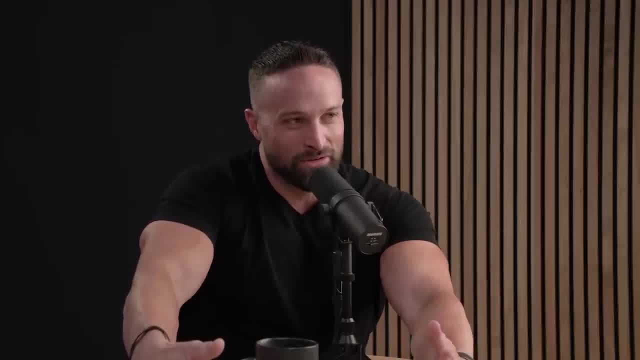 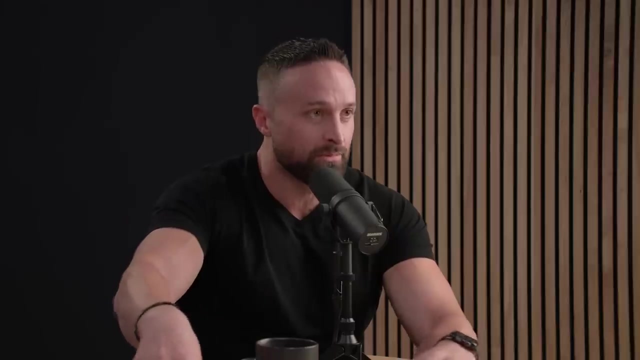 because you're categorizing, like everything in this one bucket and there are some differences between individual fatty acids. even with saturated fat, like, for example, uh, stearic acid doesn't tend to raise ldl cholesterol, whereas, you know, saturated fat as a whole tends to raise ldl cholesterol, but there are some saturated fats that don't. so again, it's. 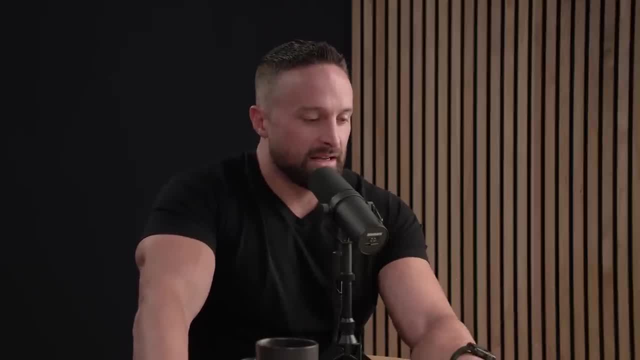 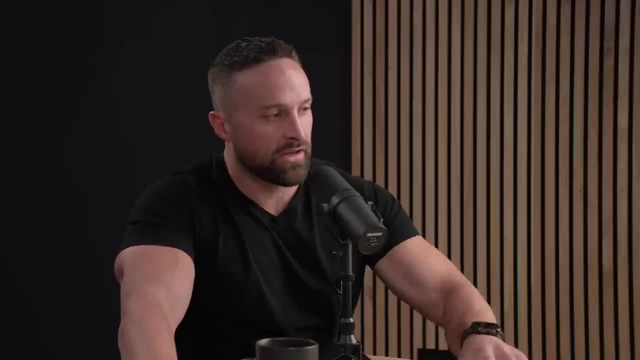 it's like we're putting things in buckets and it's a little more nuanced than that. then if you look at um, like the effects of um, you know polyunsaturated fats on markers of cardiovascular disease again tends to either be a neutral or positive effect when you substitute. 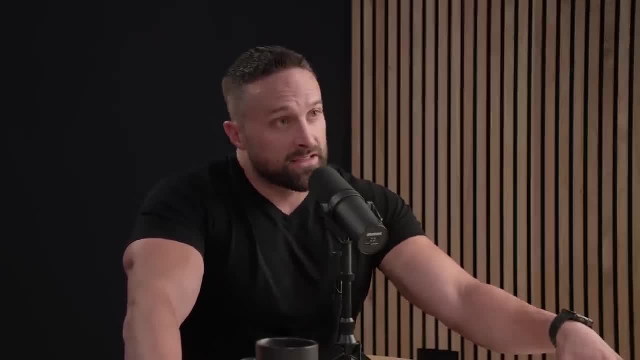 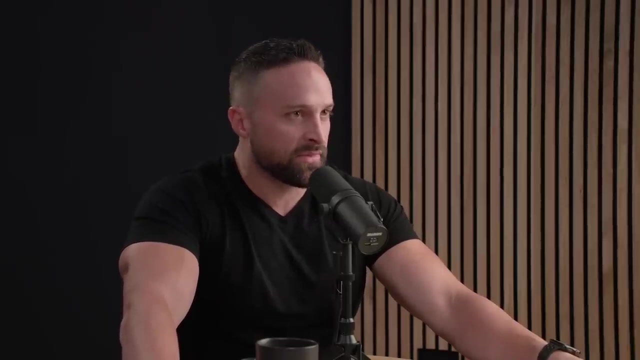 saturated fat for polyunsaturated fat. now, if you want to get into like monounsaturated versus polyunsaturated, there's some. there's quite a bit of disagreement between the studies. what i would say, based on the human randomized control trials, is that you're probably better off consuming monounsaturated and polyunsaturated in place of saturated fat. 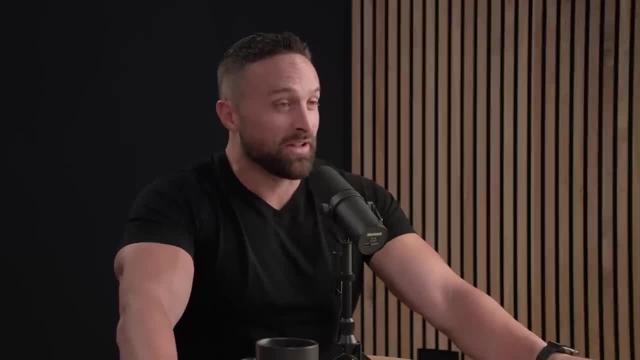 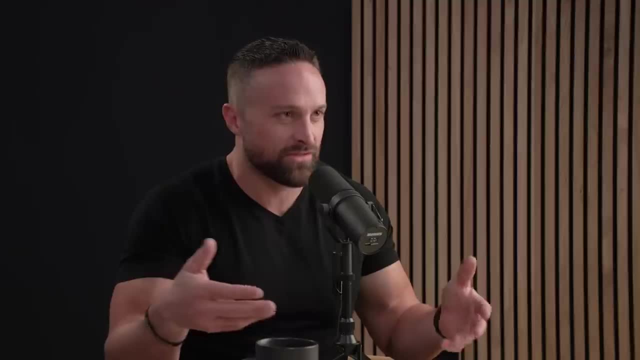 but again, if the idea is, well, that means poly is unsaturated, or good for me. so i'm just going to dump a bunch of oil on everything and now you're upping your calories. well, that's that's. that's a negative. now right, because you have to deal with the bigger problem of overall. 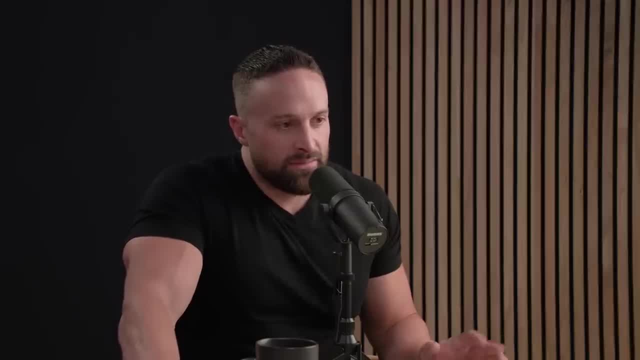 energy toxicity. so i'm not somebody who likes to demonize individual nutrients. i just haven't seen really compelling evidence that seed oils are the root cause of the problems that are being suggested, and i think this is a good example of kind of like. whenever there's a something that pops up in the fitness industry, there's always like the opposite. 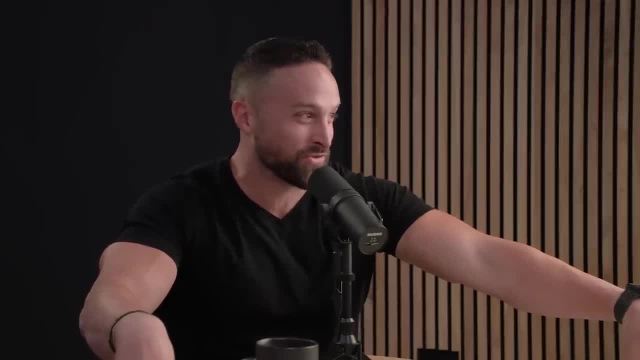 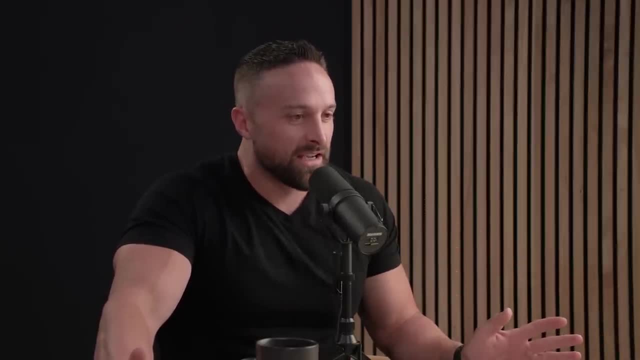 thing that pops up and it's like the reactionary- you know extreme reaction to whatever this thing was over here. i think that's what we're seeing with some of the the seed oil stuff is it's it's mostly people who are trying to kind of expose the virtues of saturated fat. 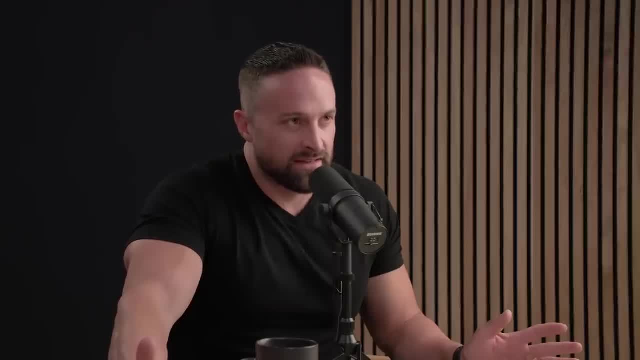 and listen. i think it's fine to consume some saturated fat but again, you know, i think limiting it to, you know, seven to ten percent of your daily calorie intake is probably wise. again, based on the the all the consensus of the evidence i've seen, and so once, 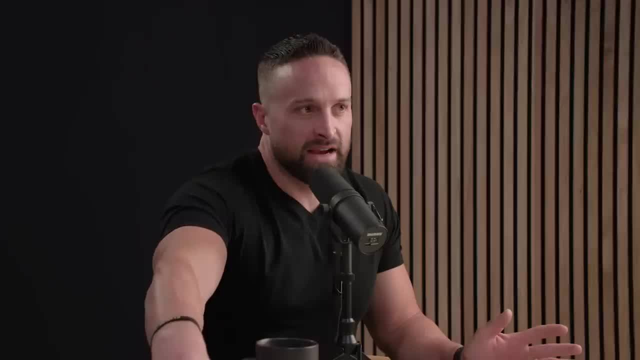 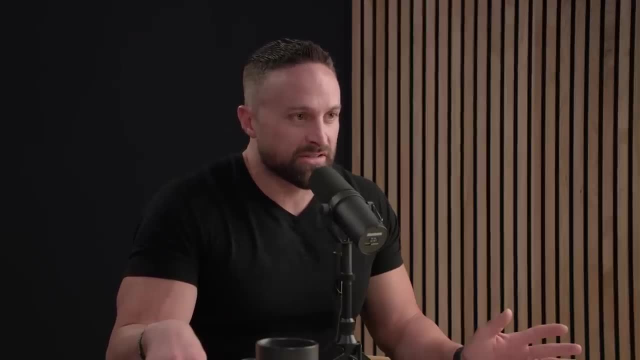 again like we're struggling with this. okay, we've got this epidemiology and these mechanisms that sound good, but then what actually happens when we we do some human randomized control trials, and and. again we have these two different types of data that are being used: that and, and and are 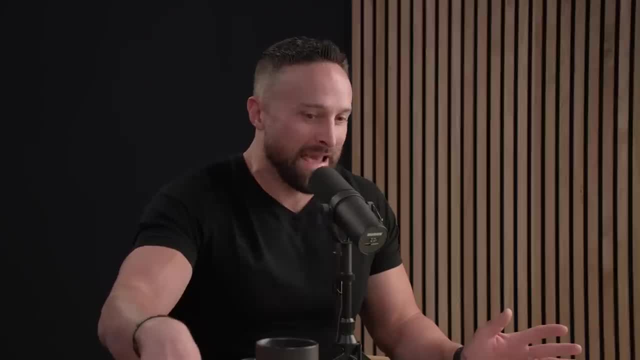 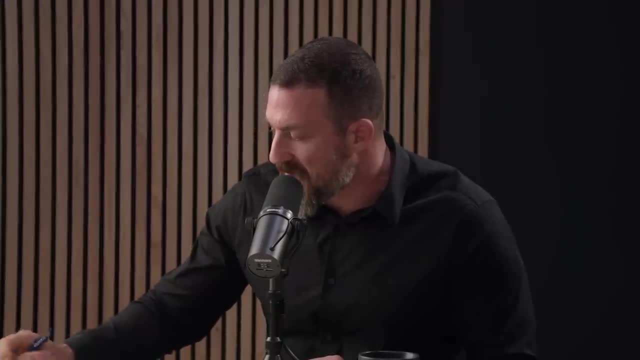 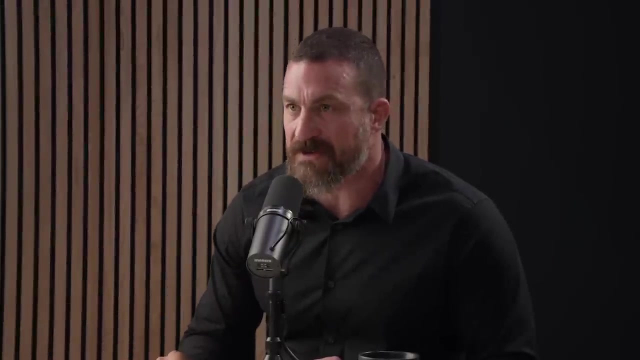 extremely important to understand and i think there's a lot of evidence to suggest that seed oils are independently bad for you, independent of the calories they contain. you said the words overall energy toxicity and i just want to highlight that i think that's a fabulous term. i don't. i don't think enough people think about that because they, they are primed or we are all. 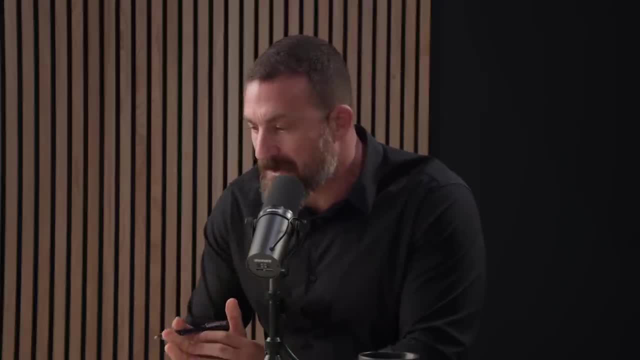 primed to think, okay, seed oils might be bad, or artificial sweeteners might be bad, or this might represent something good or bad, without taking into account overall energy toxicity of the toxicity of over consuming calories, energy. And thank you for pointing out that most of the 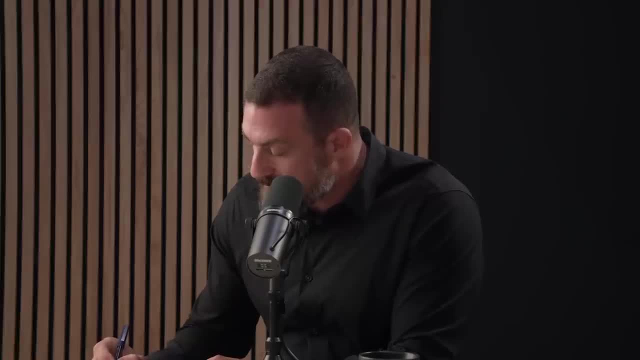 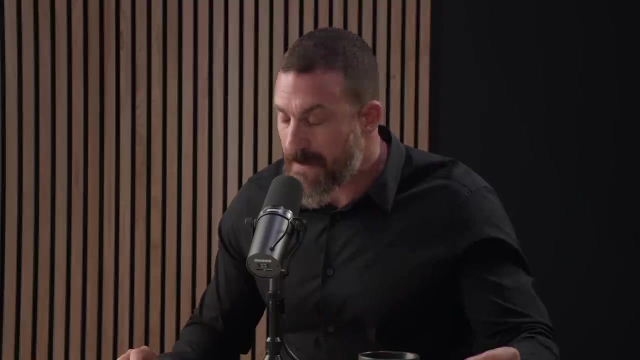 data point to the fact that saturated fat should make up about no more than seven to 10% of total daily caloric intake. Is there a lower end threshold? that can be problematic. For instance, I've noticed that my blood profiles, especially in terms of hormones, improve when I'm getting 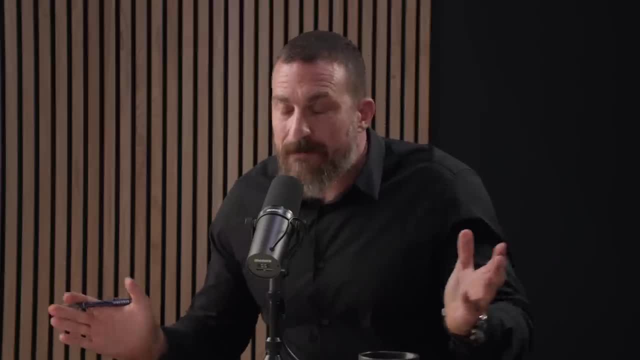 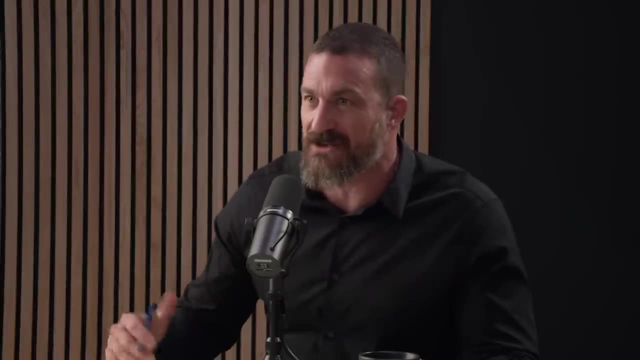 sufficient saturated fat. Maybe I'm a mutant, but years ago, because I'm a product of growing up in the nineties, I tried a low fat diet. I it certainly crushed my androgen levels. I started adding some butter back in and I was right back in the, in the, in the sweet zone where I wanted. to be. So you know, seven to 10% of totally daily caloric intake is, I'm guessing is probably about what I do now. I'll have to check. but is there, is there a danger to going too low in saturated fats? 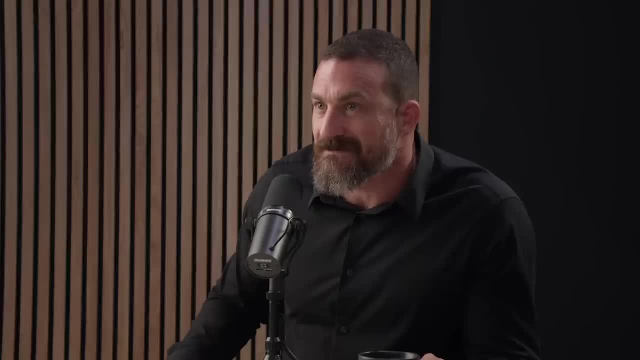 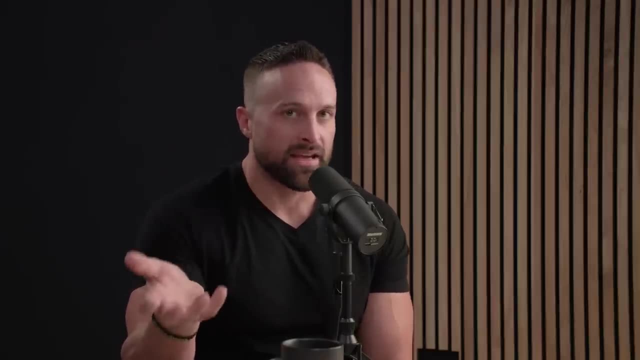 So again, no solutions, only trade-offs. right, What maximizes out testosterone might not be the best thing for longevity, right And and vice versa. Now, I'm not, I'm not making that claim specifically, but I think it's important to understand this, that I think we all have this. 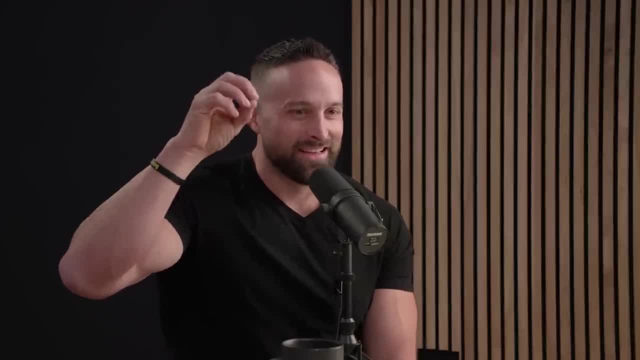 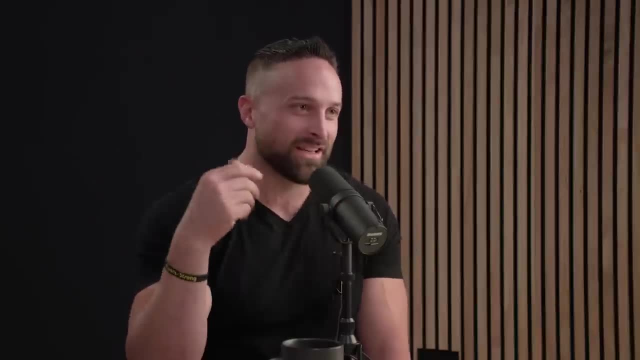 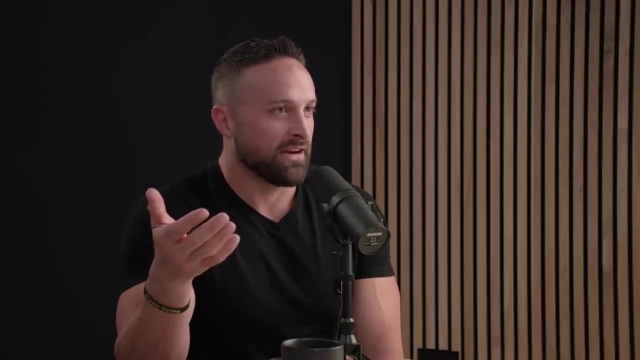 idea that there's this one iconic diet out there that is going to be the best diet for building muscle and burning fat and preventing cancer and heart disease. And the reality is like there's overall healthy dietary Patterns that we see that are good for those things, But when we get down into the weeds, 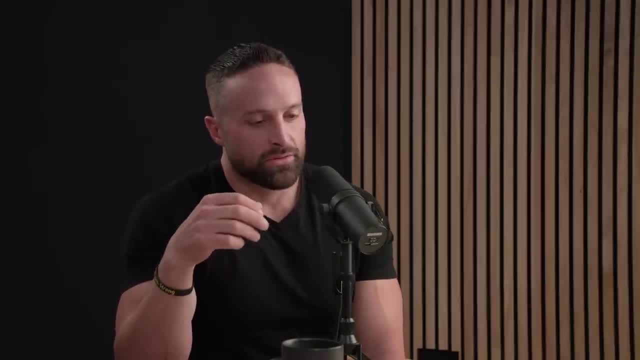 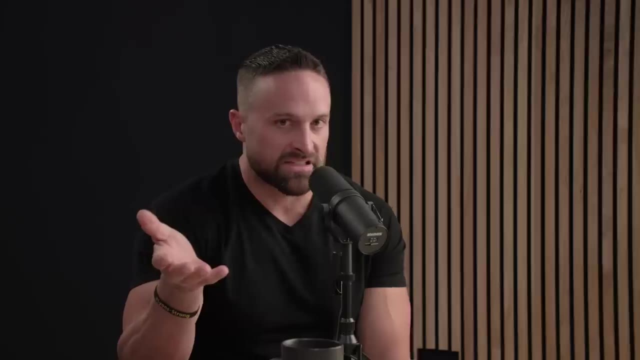 there's probably some push and pull here as well, right? So when it comes to saturated fat, there is some evidence that if you're too low on it, that yes, you can have a reduction in testosterone. Now, is that reduction in testosterone? let's say, 15,, 20%, whatever it may be. 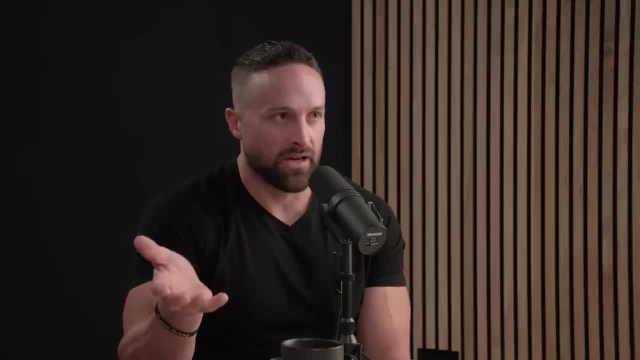 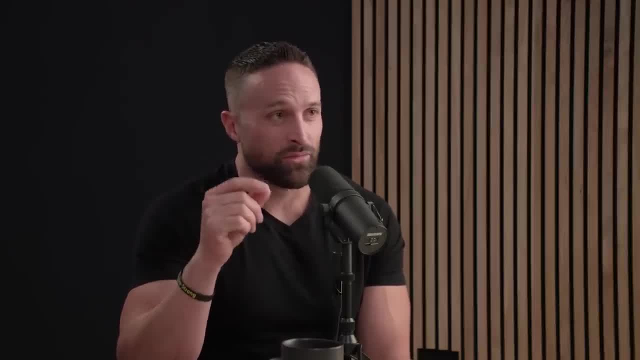 that's never been shown. Interestingly- I just remembered this- There was one study that was comparing polyunsaturated fat versus saturated fat And they equated total fat And one of the really interesting things was the group getting the polyunsaturated fat had more lean mass at the 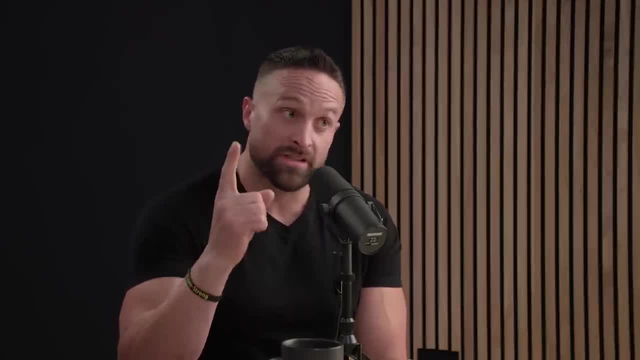 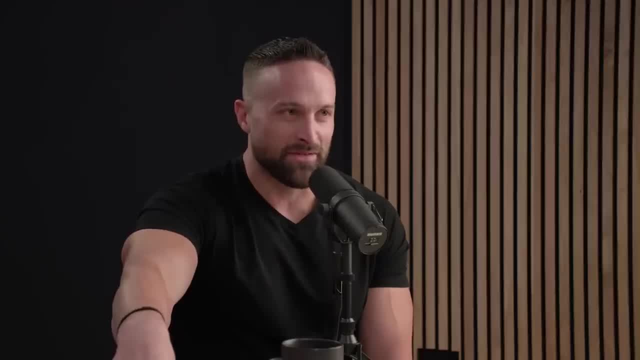 is a situation where I say I would like to find out what the mechanism of that is, because this could just be random. But if that gets shown over and over, what I might say is: okay, well, what's the? what are we if polyunsaturated are somehow increasing lean? 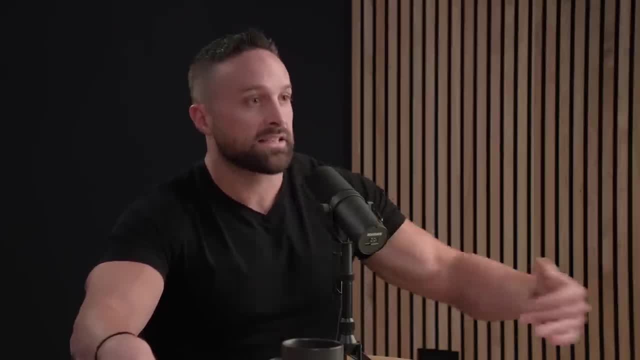 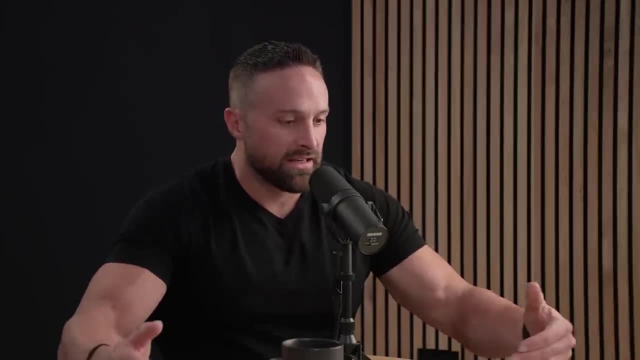 mass compared to saturated fat. who cares what happens with testosterone, unless that reduction in testosterone is causing some kind of impotence for your life, right? So all that to say. I don't really know. And, by the way, that's something for those watching and 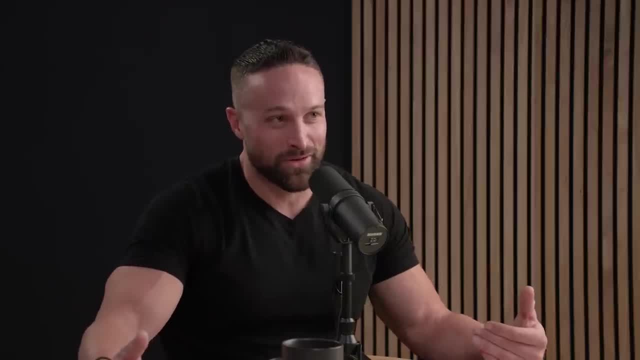 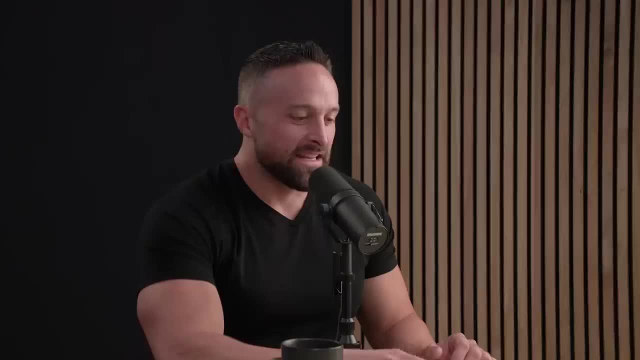 listening real experts. every once in a while, you should hear them say the following words. I don't know Exactly, My graduate advisor was exceptional at that and she was brilliant right. And then, in terms of, like cholesterol synthesis, you really need a very, very small. amount of saturated fat for LDL cholesterol synthesis Your liver can synthesize, like the amount of LDL cholesterol or cholesterol that your body needs to be able to synthesize It requires is so small in terms of, like, just living and being healthy. So I don't think you. 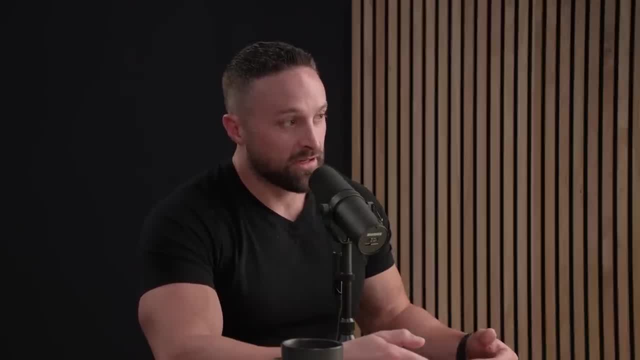 need to worry about that And from a cardiovascular disease standpoint, there is some evidence that even taking people who have, like quote unquote- low LDL of, like you know, 80 or 90, and taking them down to like 30 or 40, that there is still a benefit for the risk of cardiovascular disease. 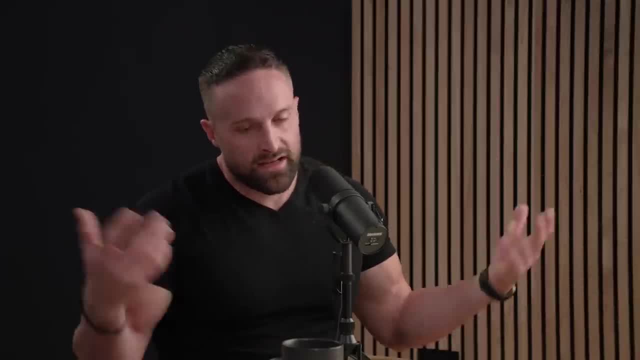 So again, you're weighing these two buckets right. So what I say? you know, if you're doing 70 to 10 percent from saturated fat, you're going to have a lot of LDL cholesterol synthesis. If you're doing 70 to 10 percent from saturated fat, you're probably fine. 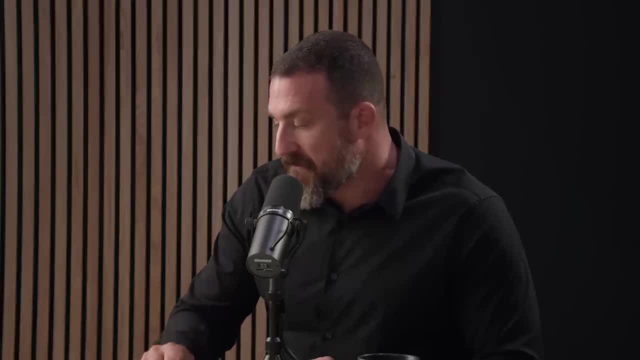 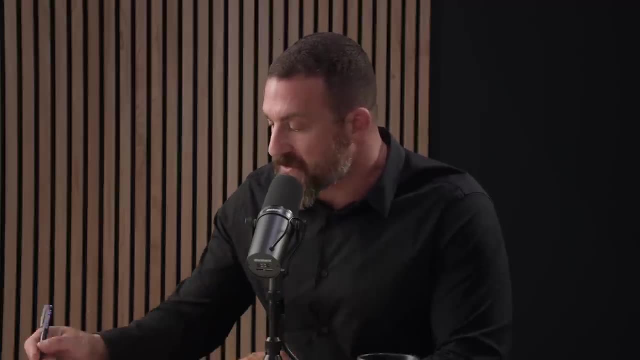 I received a lot of questions about whether or not there are female-specific diet and exercise protocols, And I realize this is a vast landscape, but some of those questions related to menopause and premenopause and some related to the menstrual cycle, most related to variations across the. 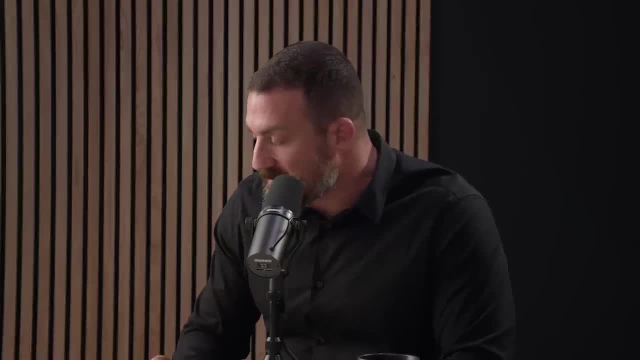 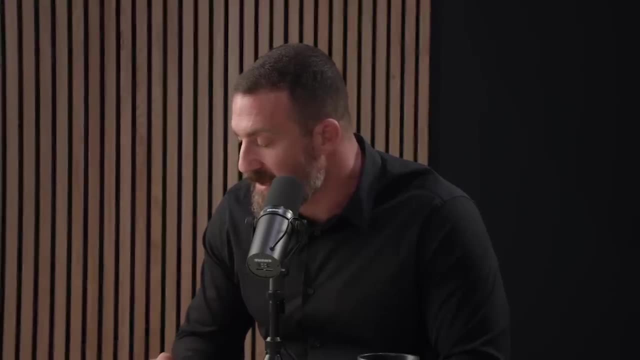 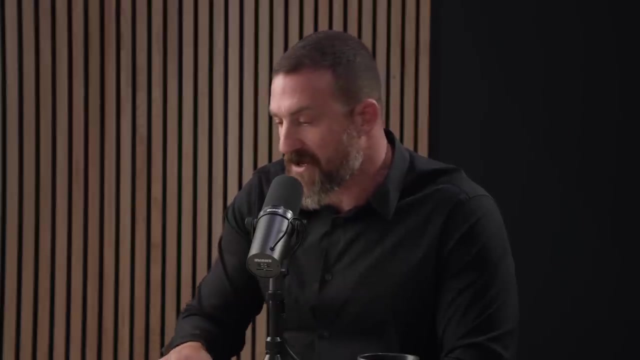 menstrual cycle In terms of, let's just say, diet maintenance or subcaloric diet. are there any things that you've observed? We'll talk a little bit later about this wonderful app that you've produced, this Carbon app, which helps people manage their energy intake, and a number of 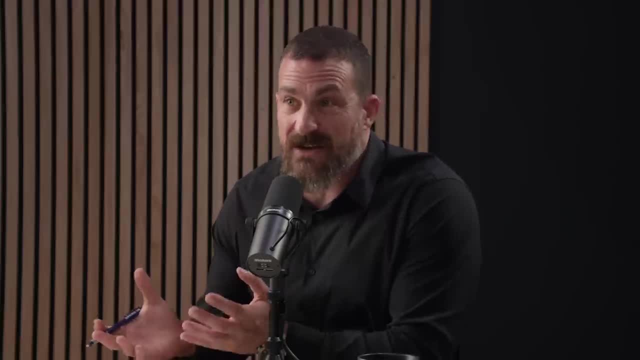 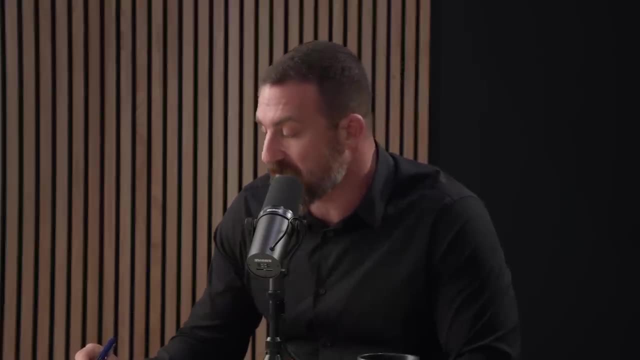 other things. And so there you have a sort of a database or at least an experience base. And then I'm guessing there are probably also studies exploring male versus female differences in terms of adherence and what sorts of diets work. Are there any general themes that one can extract? 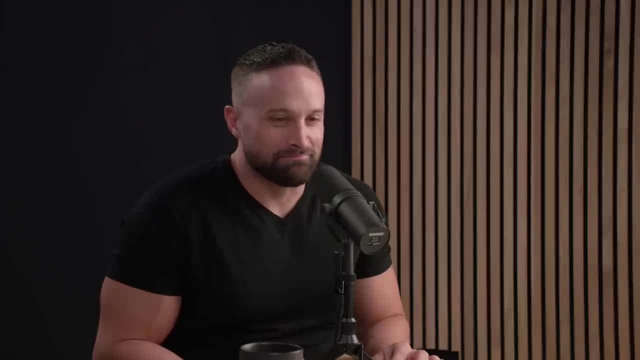 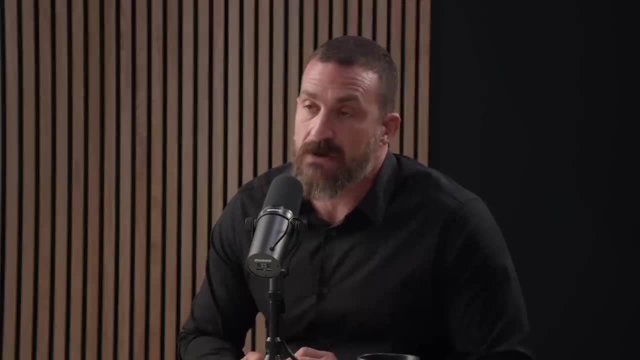 from that, This is going to be a really unpopular segment. for the women, It doesn't seem to make a big difference. Well, actually, they may be relieved to hear that, because it would make sorting through the information space- and certainly the information we've covered in this podcast up until now- simpler. It means that everything isn't different. 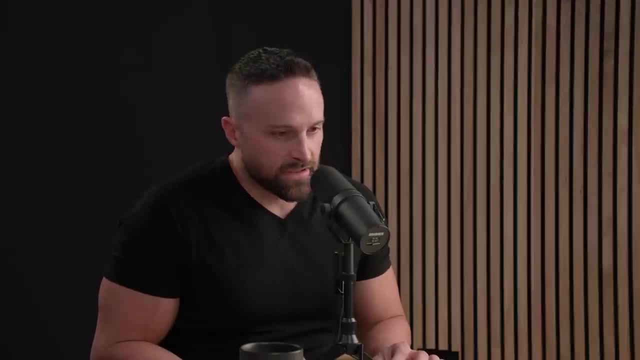 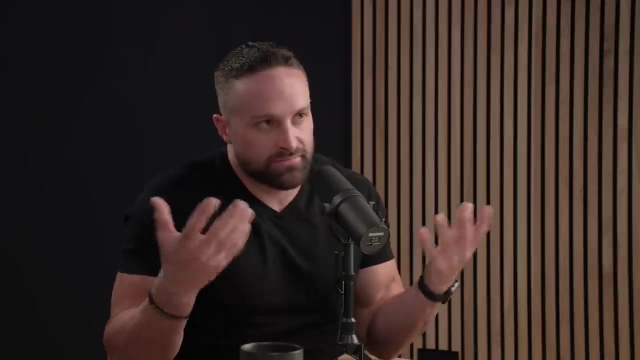 for them. Yeah, So if you look at the male versus female studies relation to diet, they seem to respond to some similar way, like similar calorie deficit seems to produce similar results. If you do low carb, high carb, regardless it seems to. 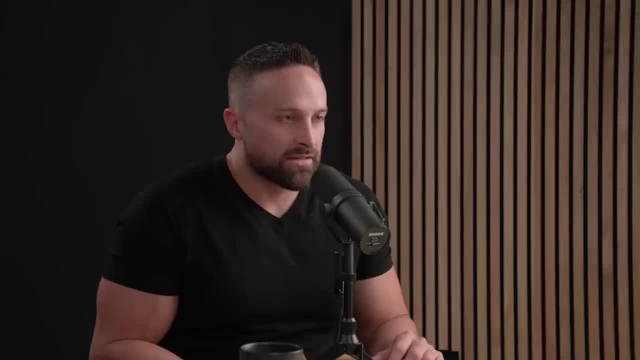 boil down to the same principles. Now, training wise. we do know that female, like the muscle fibers, adapt a little bit differently to training. but without getting too far into the weeds, it doesn't really change the way you should train, Because for the most part, building muscle, 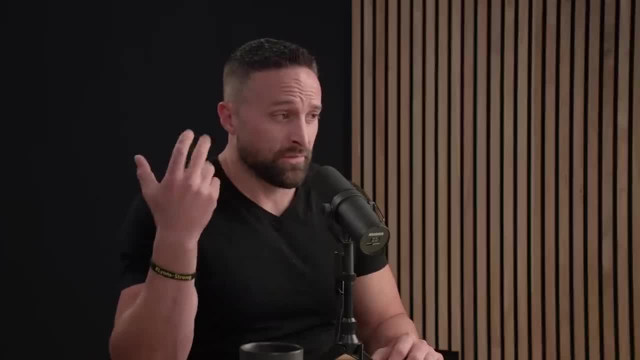 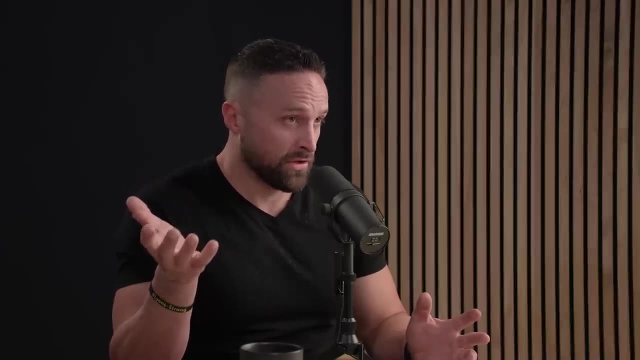 there's a lot of different ways to build muscle, So we know that like light loads up to maybe like 30 reps- as long as it's taken close to failure- have basically the same effect on your building muscle, at least in the short term, as heavy loads for low reps. It's mostly about taking the muscle close to fatigue or failure. right, You don't have to go to failure, but getting close- within a few reps- If you're between one rep and 30 reps if you're getting close to failure- seem to produce similar results. So again, great, You can pick with whichever form. 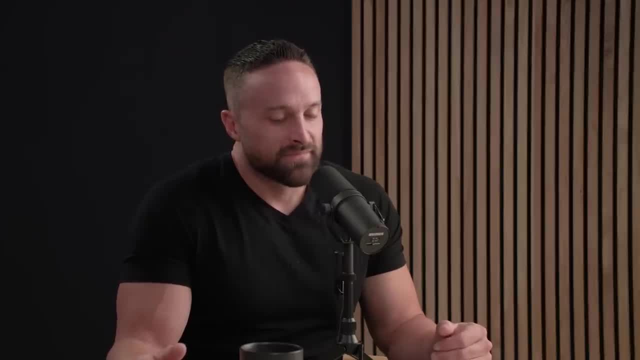 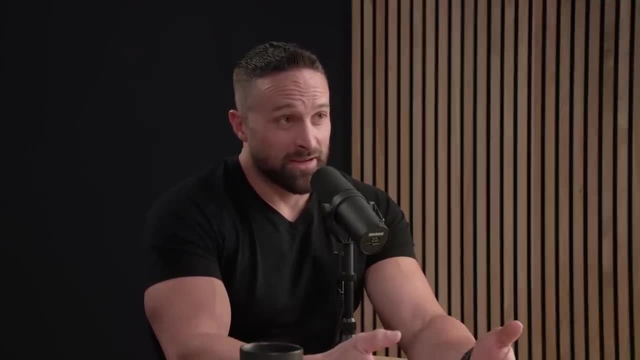 of discomfort you prefer, right Um, when it comes to female specific training- again, females actually- this is one thing that a lot of people don't know- They actually put on a similar amount of lean mass as a percentage of their starting lean. 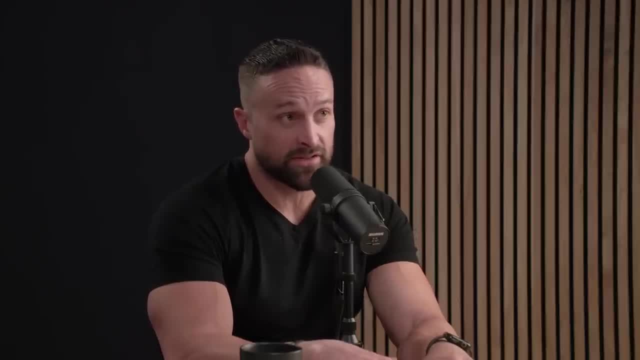 mass as men. In fact, there's no statistically significant difference in the amount of lean mass they put on. Now. the absolute amount of lean mass that's added will be greater for men because they started with a greater amount of lean mass, But the relative increase in lean mass 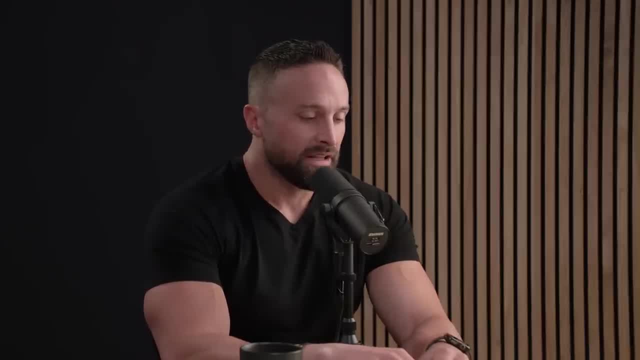 is pretty much the same from similar training. Now, uh, females, there's some differences in like fiber types. Females tend to be a little bit less fatigable than than men. They can. they can go a little bit harder, a little bit longer, And 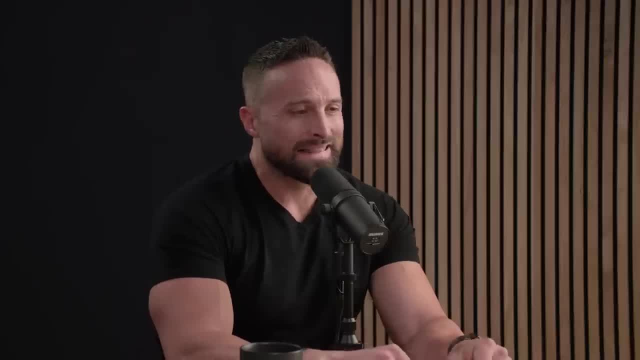 there's also some evidence that they recover a little bit better, but that also could be simply due to the fact that they're not able to use as heavy of loads to to induce hypertrophy. So I kind of have this theory that, while you know, as a percentage of your one rep max. 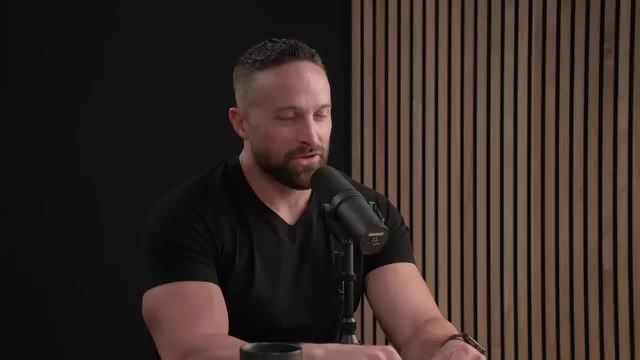 you can program things. I think absolute load matters When you look at like the most elite power lifters- the super heavyweights aren't squatting three or four times a week because you know they're squatting eight 900 pounds. I think that there's an overall recovery. 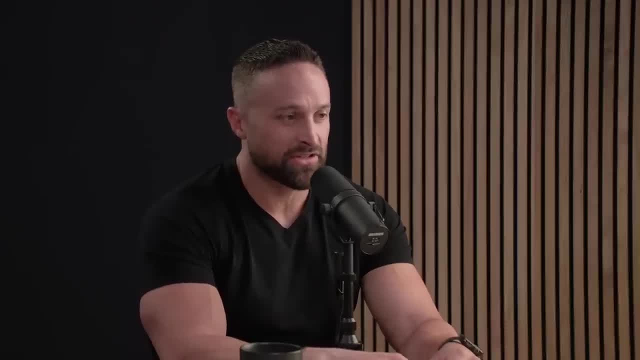 effect there. Again, I have no data to back this up. This is just my, my observation. But when you get into the lighter weight classes- and this goes for men too- you do see quite a few people who do you know many training sessions at. 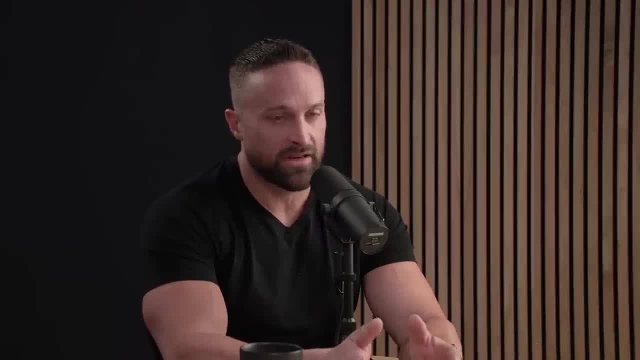 high RPEs and seem to be able to recover from that. So I do think the absolute load makes a difference. Now, when it comes to like menstrual cycle, this is one of those things where I kind of tell people: you know, do what you prefer. So there's some people who have said you should. 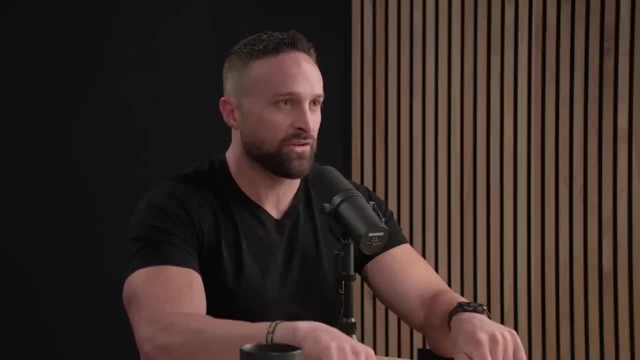 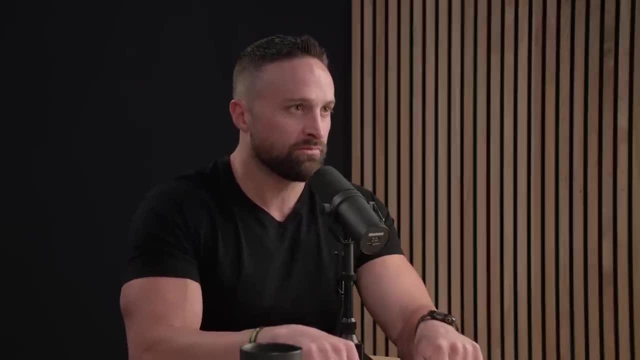 program you should like kind of schedule your training around your menstrual cycle, which is whenever you're going through your menstrual cycle. you know, reduce the intensity, reduce the volume, because you're you know you're not going to feel as good, You're not. 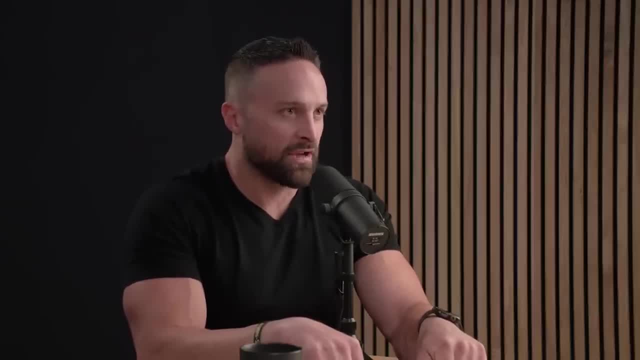 going to train as well. What I would say is: just auto-regulate that if you go in and you're on your period, but you you feel good and you're doing well that day, then I don't think you necessarily need to back it off. And there there was one study that kind of supported that notion. But 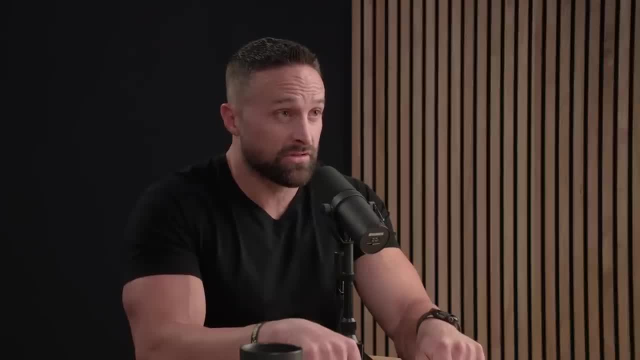 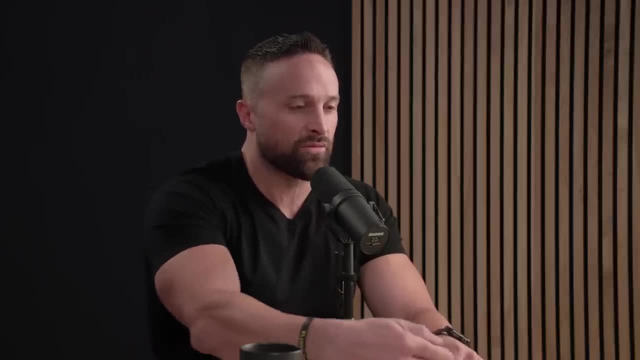 if you go in and you feel terrible and you know you feel like you could use, you know, a reduction in intensity and volume, then it's totally fine to auto-regulate that. And when I say auto-regulation, auto-regulation means you are regulating the individual training session. 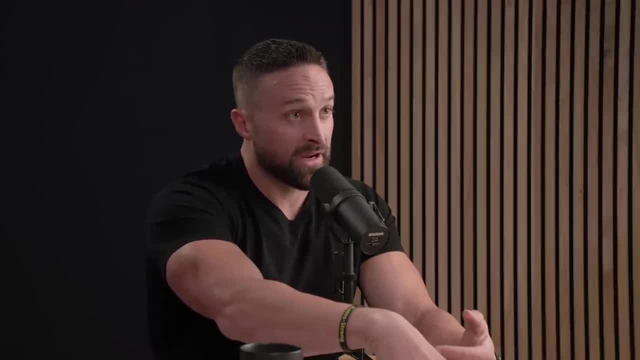 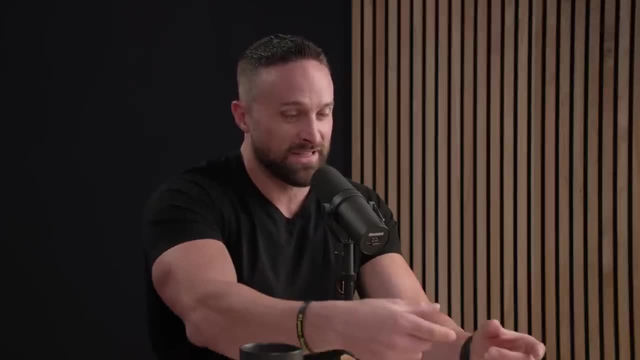 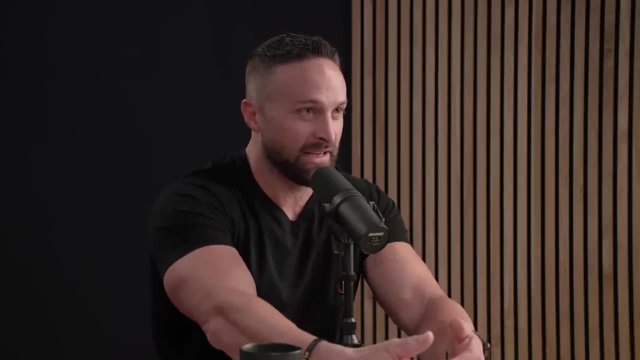 based on your performance. So I auto-regulate in so far as, like I'm a, I'm a super nerd, So I have a velocity device so I can actually attach to the bar and see how fast the load moves And I know at various different, like warmup weights, what velocities I should be hitting. So if I hit my 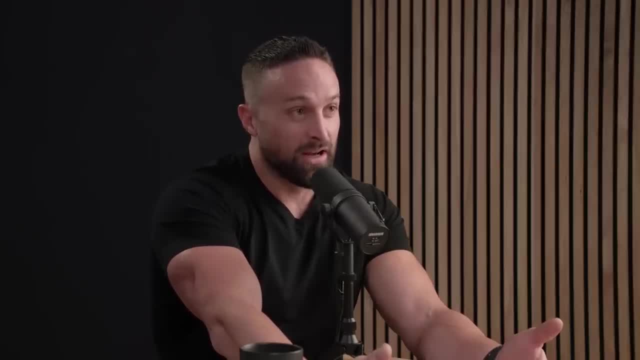 last warmup and my velocity is about 10% higher than usual. I can be pretty confident that that's going to be a good day for me. If it's lower than I, can back it off a little bit, In fact, at worlds. 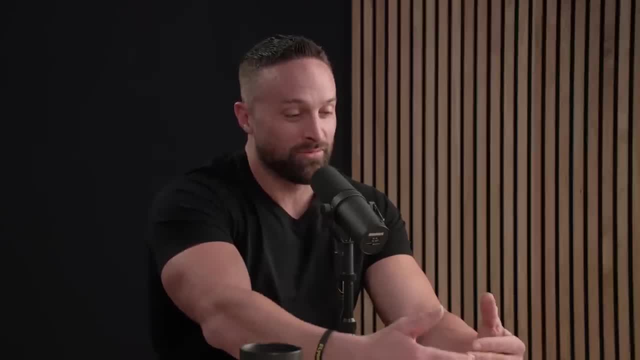 when I hit my last deadlift, it was 30%. my last, my last deadlift warmup- it was 30% faster than I usually hit in the gym And I turned and looked at my coach and I said, yeah, we're going to get. 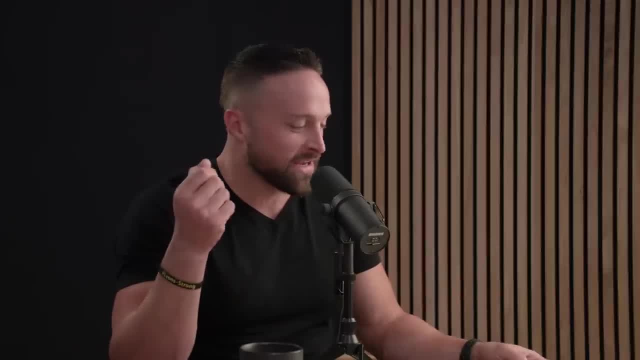 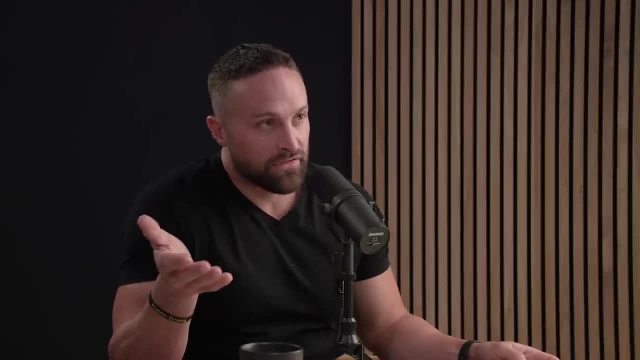 this today. So there's various forms of ways to auto-regulate. but again, women, if you're on your period but you feel good, I don't think there's any reason you need to back off. But if you're not feeling good, then it's totally appropriate to back off. 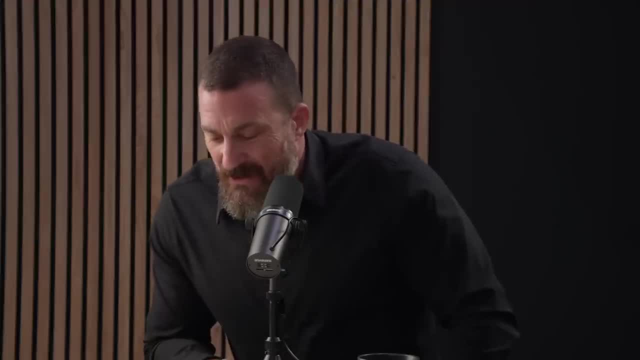 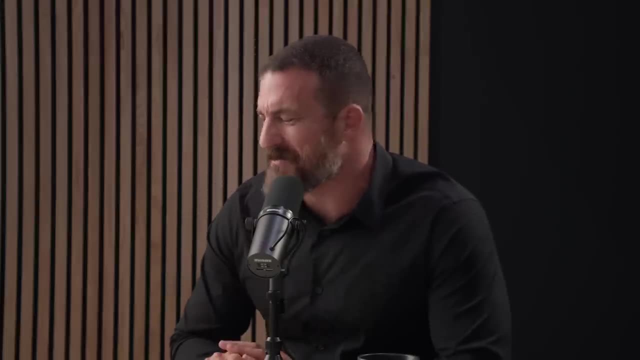 Raw versus cooked foods. People wanted to know whether or not, for instance, you know, eating a raw apple versus I don't know, does anyone cook apples? I guess people used to bake and they were baked. apples was a dessert When I was a kid. it was kind of the. 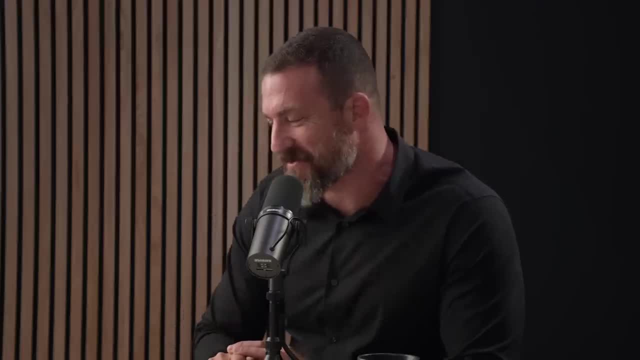 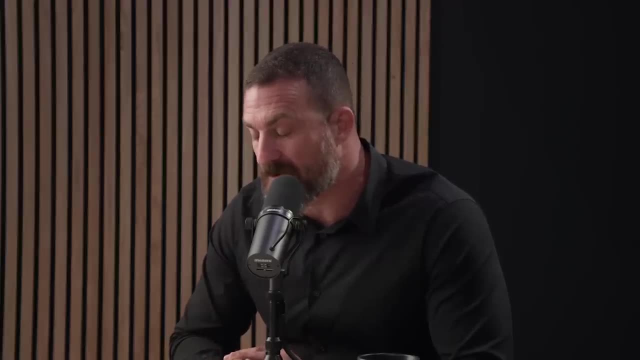 letdown dessert. Sorry, mom, It was kind of like not awesome unless it had a scoop of ice cream in it, And even then maybe not awesome. but anyway, raw versus cooked. Obviously, if you burn a piece of meat to the point where it's pure charcoal, that's too much, And if you eat there is a small. 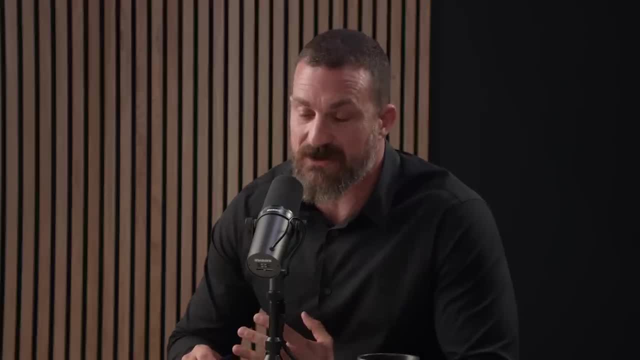 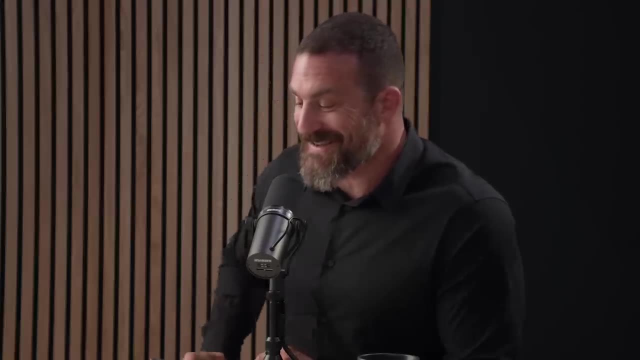 movement surrounding eating raw meats. That's not something I particularly enjoy. frankly, Sushi is the only raw food I personally ingest And I'm very- I am- very- careful about the sourcing- frankly, Reputable places. Is there anything you know real about this in terms of 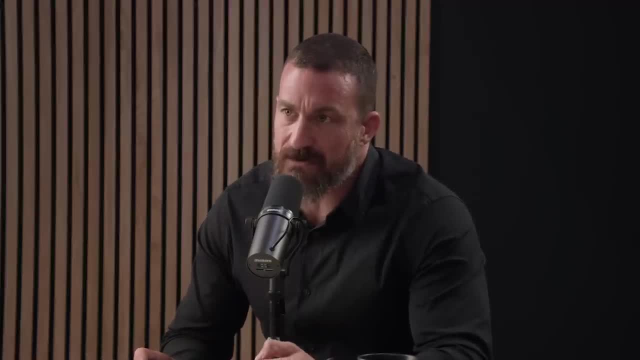 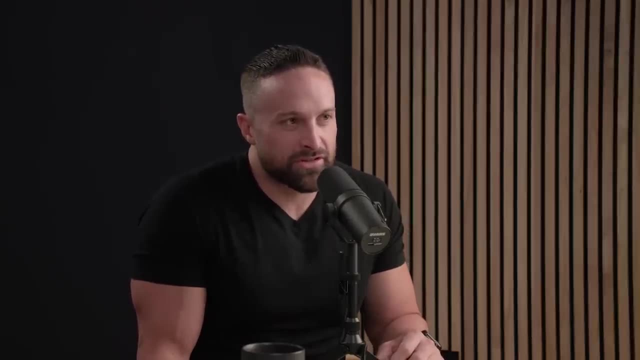 being able to extract the amino acids, vitamins and minerals from the food raw versus cooked. It just looks cool for Instagram. So when you cook foods, they actually tend to become. in terms of protein containing foods, they tend to become more digestible, not less. 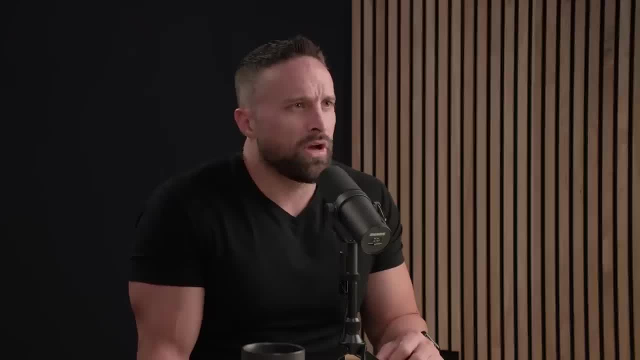 Eggs are this way, Meats are this way. People say: well, you know, when you heat protein, you denature it. And I think they hear that word denature and they think destroy. And that is not what denature means. So proteins fold up into 3D. 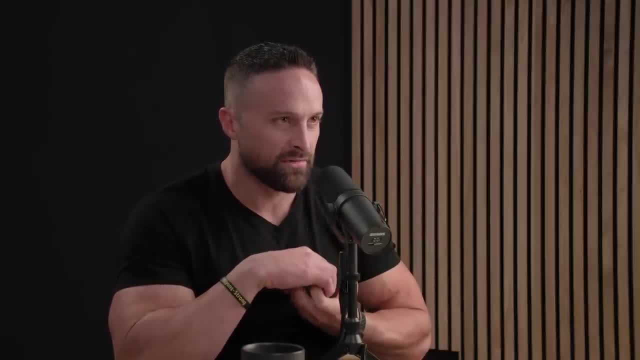 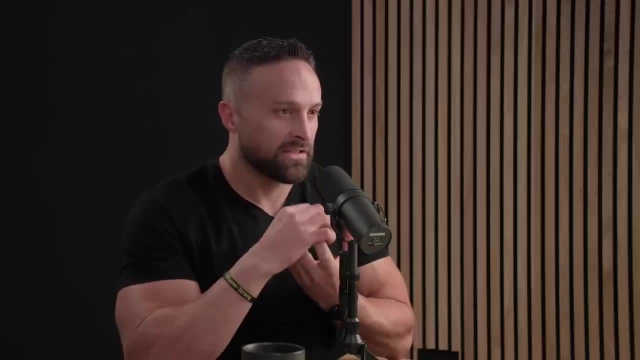 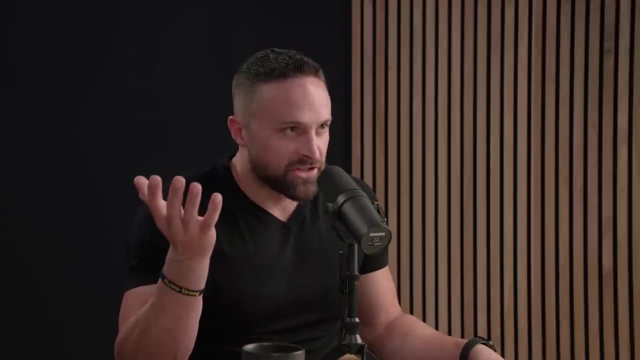 dimensional structures- You know this, of course- based on their amino acid sequence and their specific energies of those amino acids. When you heat protein or add acid, it starts to unfold that protein structure. That happens during digestion anyway. So I always chuckle when, like the like, I've seen some. 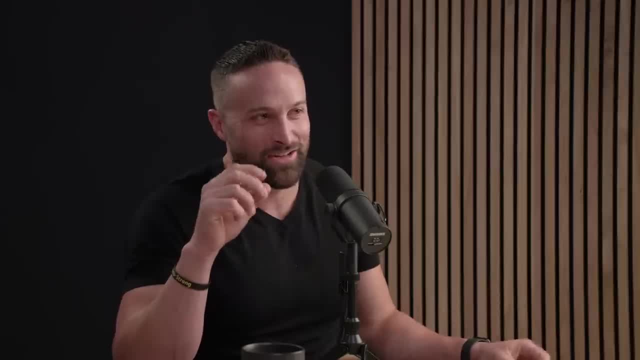 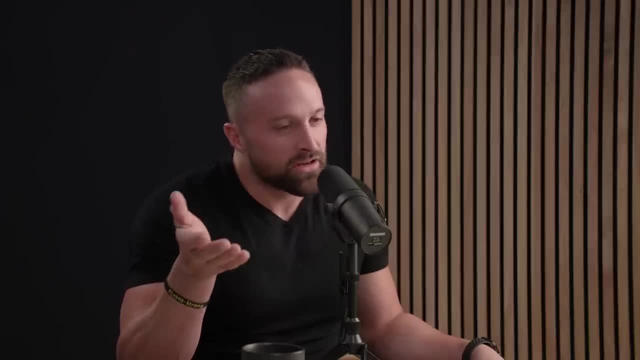 companies come out with way that you can cook with, right, That's not going to destroy the amino acids, And I'm like: so you mean like regular way, right? So yeah, cooking, typically cooking actually makes amino acids more bioavailable, not less. Now I would stay away from charring your. 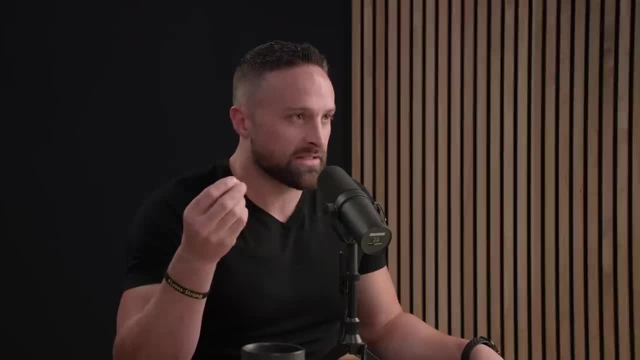 meat because there is some evidence that charring creates polyaromatic hydrocarbons Which, at least in animals, when they give those they, appear to be carcinogenic. So if you do charring meat by accident, I would just cut off the charred portions And then you should be fine. 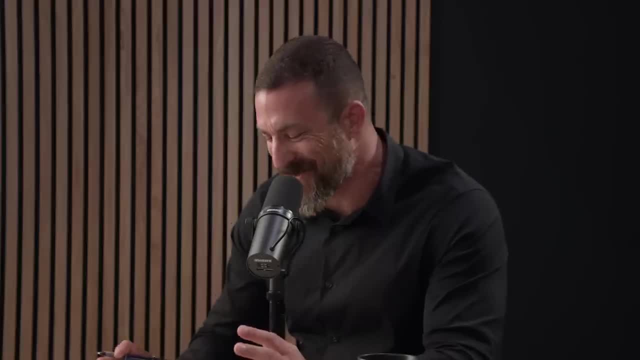 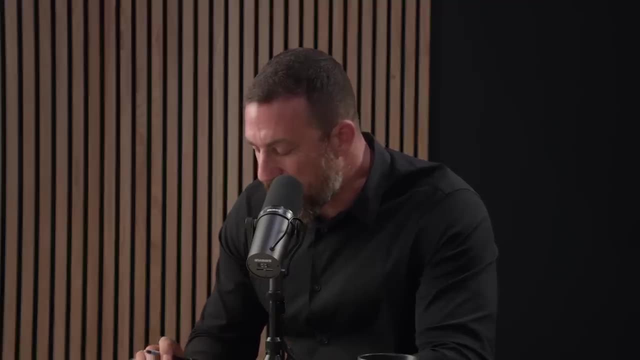 The char is delicious- Not not, if it's charred too much, but there is something about a charred crust on a meat. My dad's Argentine and I would like a good barbecue. What about people referred to them in their questions as carb blockers, but I think what they're referring to are things like: 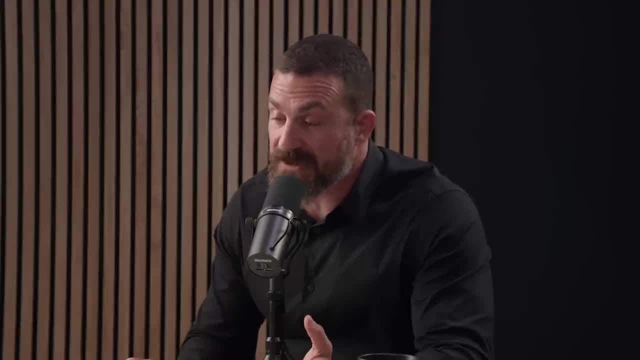 berberine and some of the glucose scavengers. And one glucose scavenger I'd love for you to comment on is this assertion that taking a brisk walk after a meal, or maybe even a slow walk after a meal- some movement- can help downshift the 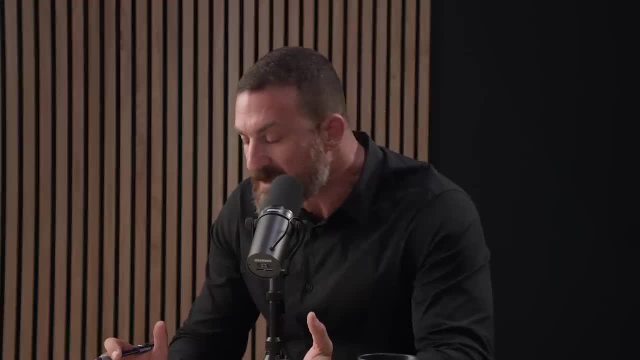 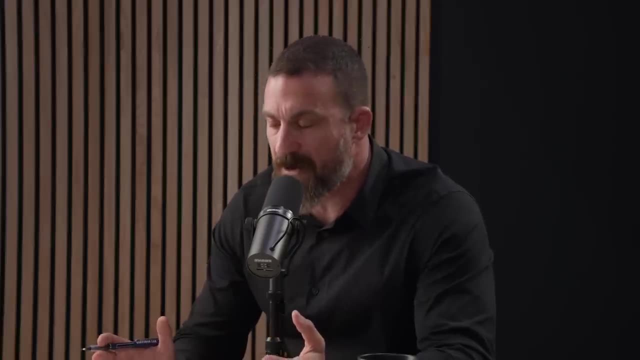 amount of circulating glucose in some way. I've heard that not a lot of people, but some are starting to pay attention to this idea of taking things like berberine or even metformin can scavenge glucose. I personally can't take berberine. If I take it, I get massive headaches. 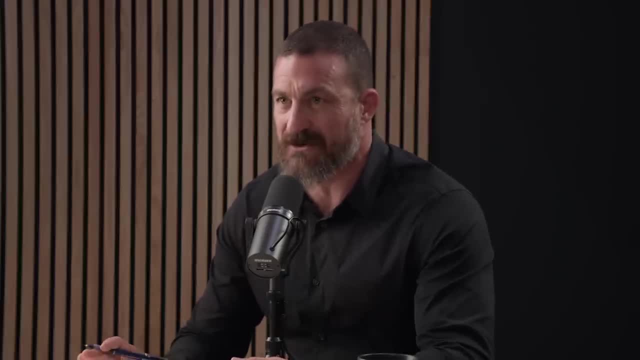 unless I've ingested tons of sugar, Dr, So I just don't mess around with it, But I I know there are a number of people out there that want to know whether or not these glucose scavengers can be useful. I think that is really majoring in the minors, If I'm being honest, as far as like the carb blockers. 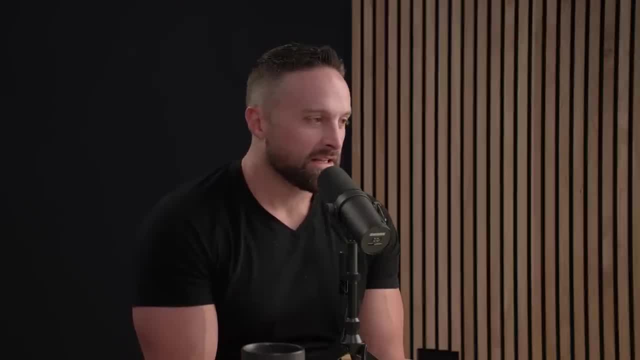 there's like some white kidney bean extract and those sorts of things. They can. they do block the digestion of carbohydrates, some. So when I say block, that's those watching or listening. metabolism is typically not on and off. Dr, Yeah, Dr Okay. So when we say things like block or attenuate or inhibit, typically we're, we're not. 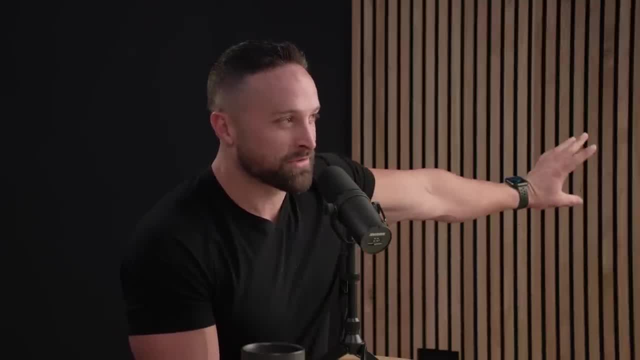 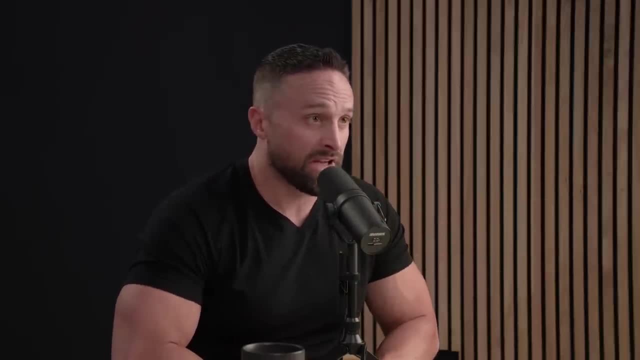 talking about just a switch on the wall that you press it and everything turns off. We're talking about a dimmer switch. Okay, Like so you. it just changes the emphasis. But these carb blockers can reduce the absorption of carbohydrate. Now they don't seem to cause weight loss when, when you just do it a normal diet. Now, why is that? Well, all it does is, once those, those, those, those carbohydrates get to the um large intestine and your bacteria get ahold of them, they start fermenting them to volatile fatty acids which could reabsorb into your liver. So you don't get. 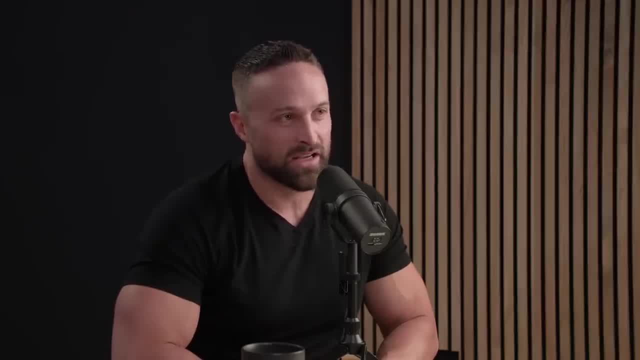 the increase in blood glucose, but you still get almost all the calories from it because it's just in a different form. So you know if carb blockers, if they actually worked really well- I mean, if you block something from being absorbed, your GI typically does not just. 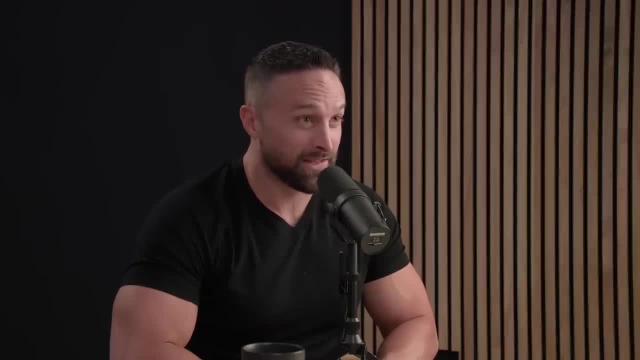 let undigested material sit in there, You get diarrhea. I mean that would be the outcome, Dr. Yeah, It's also how I like debunked the whole. like 30 grams of protein at a meal You can't absorb. 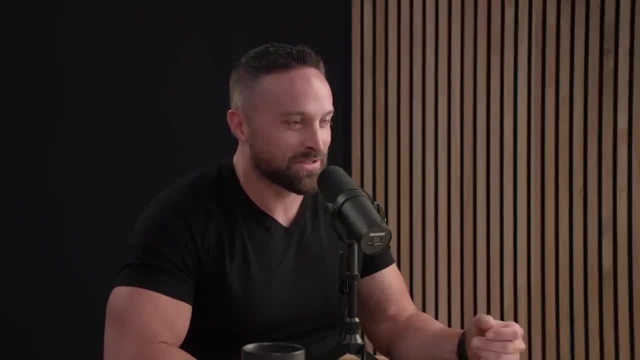 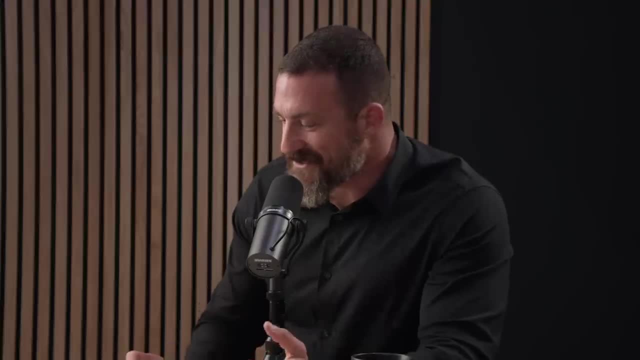 any more than that. I'm like if that was the case- like when you ate a steak, like you would just start having diarrhea every time you went over that 30 gram threshold, Right, Dr. I remember during college, So this would be early nineties- There was the 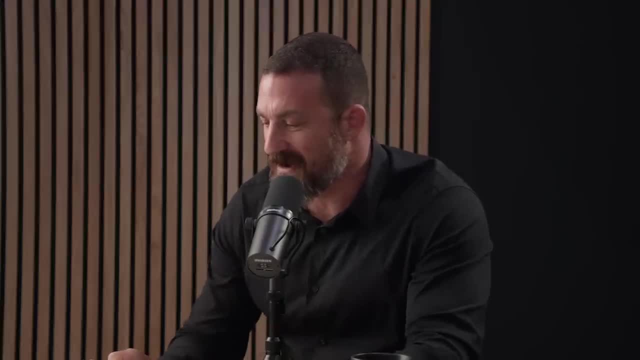 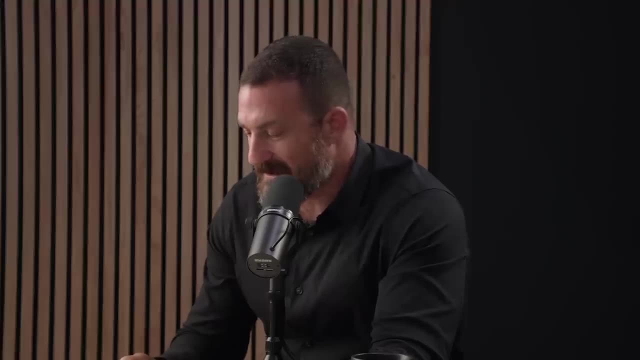 Olestra craze. this idea of of putting in non-digestible um thing into things like potato chips so that it would um clear through, uh, the the GI tract faster not absorb as many calories Dr It does raise. this went nowhere. obviously, um, you don't hear about this. 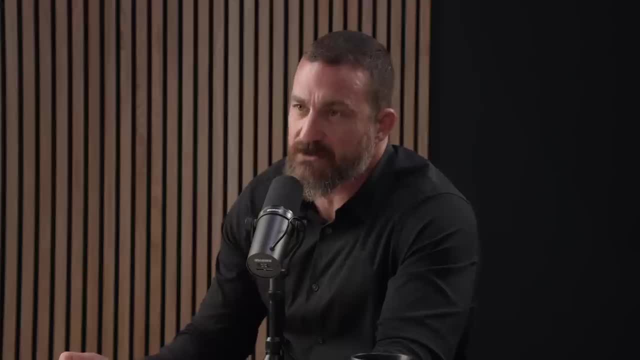 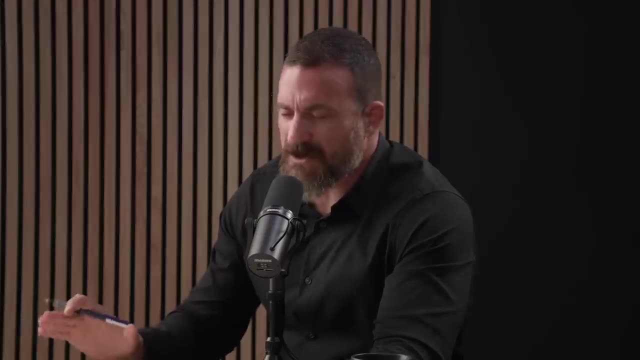 anymore, but it does raise an interesting question related to energy balance, which is gastric emptying time, Um, and obviously in in the landscape of eating disorders, in particular anorexia, abusive lack use and abusive um laxatives is a way in which people 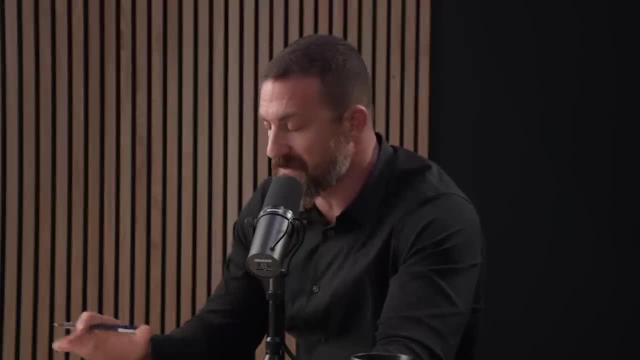 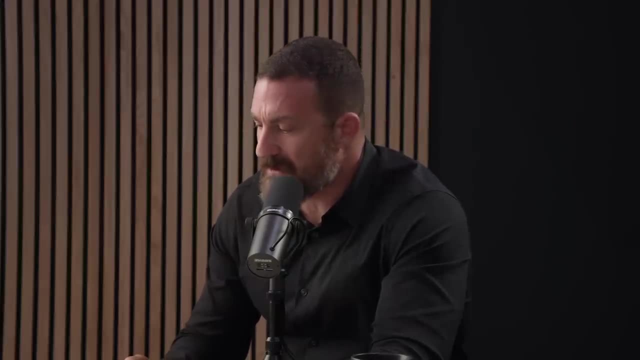 will, uh, in an unhealthy way. uh, try and control their weight, And there's a lot of problems with that approach. But, um, what about gastric emptying time? Is this one way that people could um control their energy balance in a healthy way And um 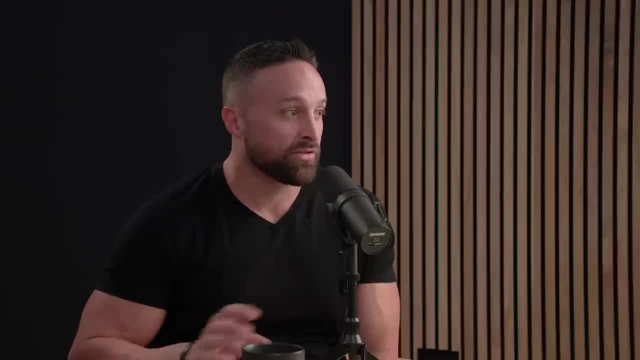 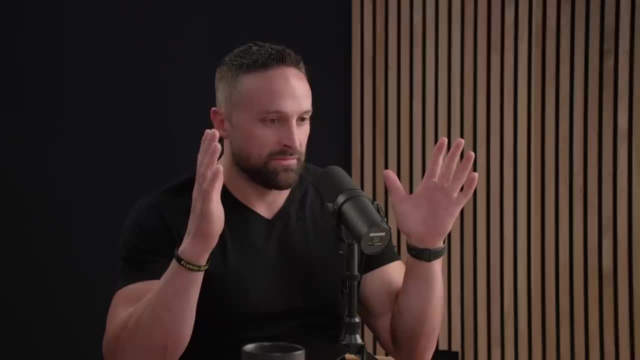 where does fiber come into play, Dr Uh, fiber tends to improve GI transit time because it adds bulk. So you know your, your GI system is basically a tube and it has peristalsis, which is wave-like contractions that moves the food down through the tube. Well, 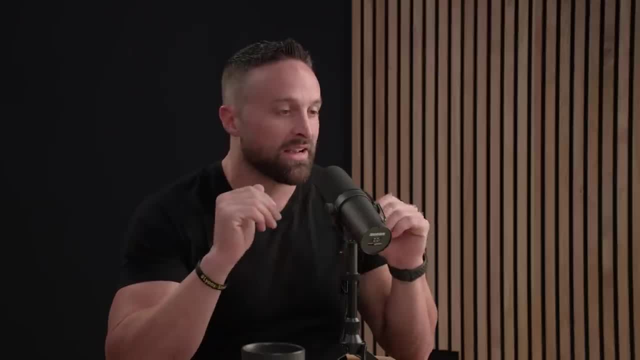 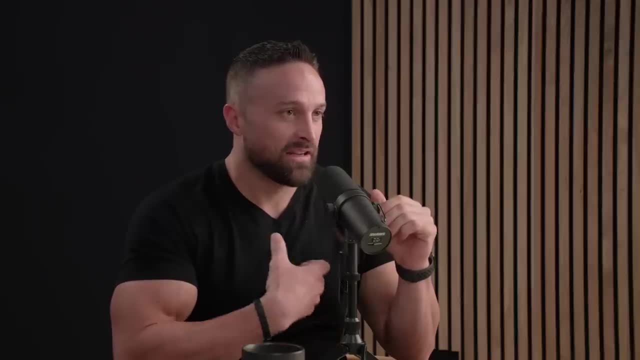 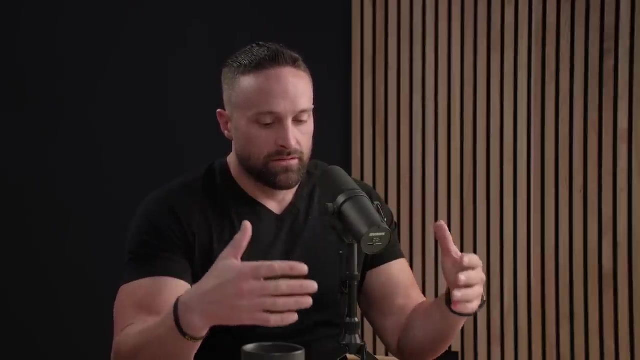 if you have more bulk to the food, like with fiber, you can move it through a little bit better. Now, in the gastric, the stomach specifically, fiber tends to delay gastric emptying and slow it a bit. um, probably because it congeals a little bit. Um, now this kind of gets into like the glycemic index. 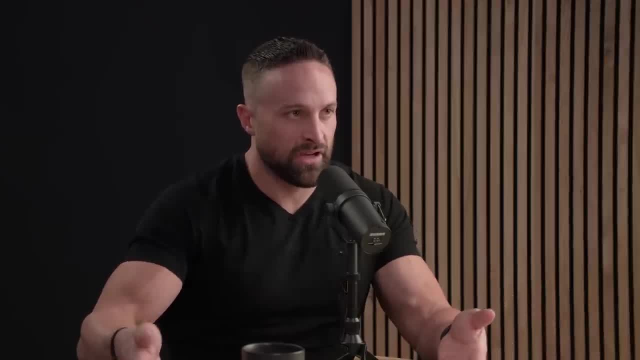 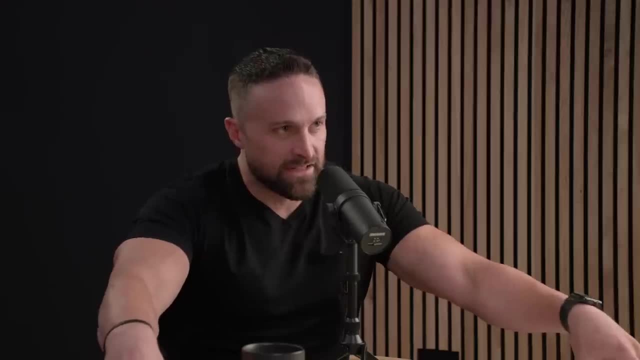 argument right, Like if you do- if you do like low GI foods- you'll have a slower release of glucose. Um, it's a slower gastric emptying time. Does that affect energy balance? And so there are quite a few studies looking at like low GI versus low GI, Dr. Uh yeah. 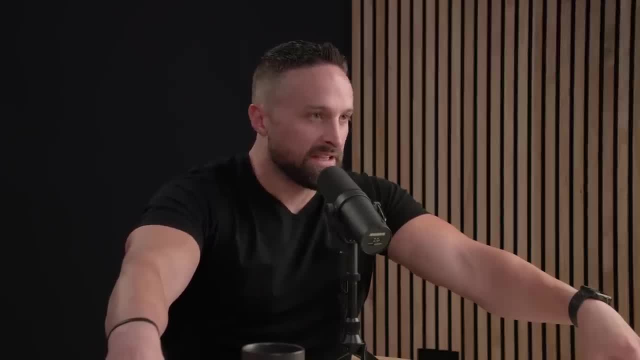 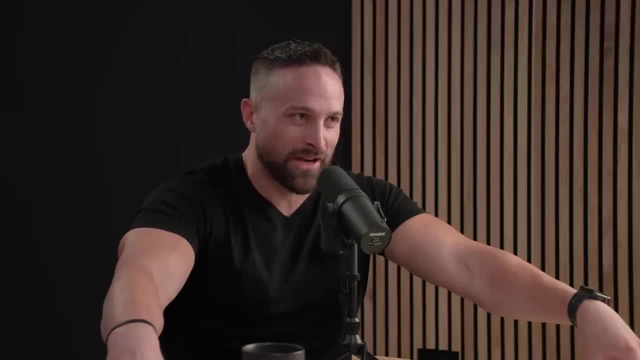 low GI tends to outperform high GI, but when they control calories there's no difference, And so what that tends to, what I think that suggests, is low GI foods just by their nature tend to be higher in fiber, And so I think it it just kind of comes back to the fiber issue. 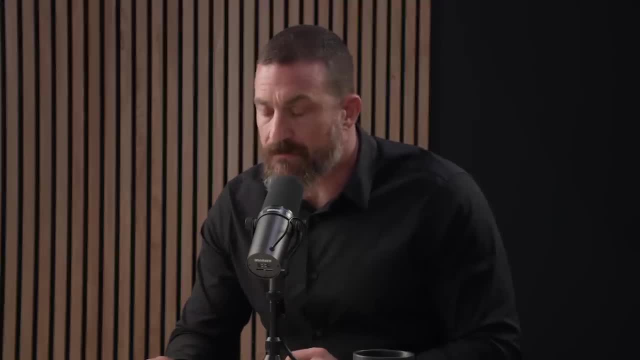 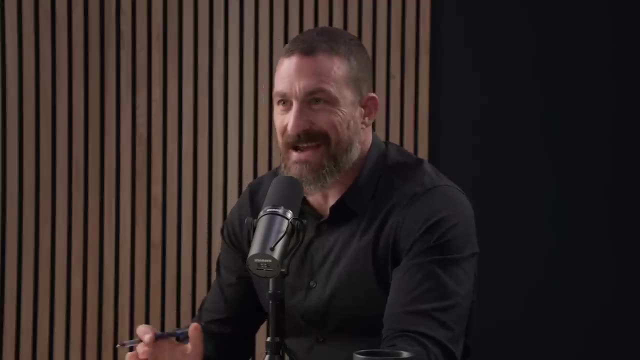 Dr Got it. I'd like to ask you about supplements for a moment. Um, it's an enormous landscape, but I believe there are a few things that you believe in meaning. they exist and and there are decent data to support their use. maybe even some anecdotal data based on your own. 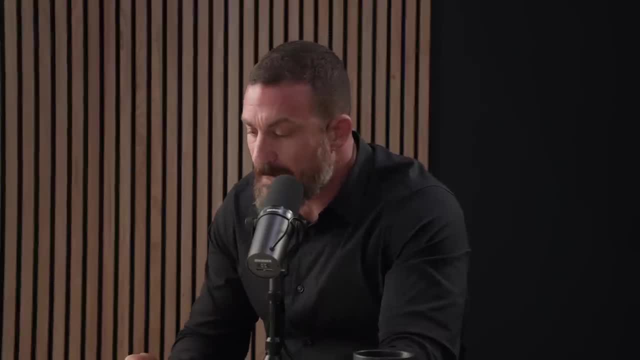 experience. As long as we highlight it as such, it could be interesting. I've heard you talk about two in particular, uh, one that I'm very familiar with, which is creatine monohydrate- If you could um share your thoughts on that, not just for muscle building, but maybe any other purposes. 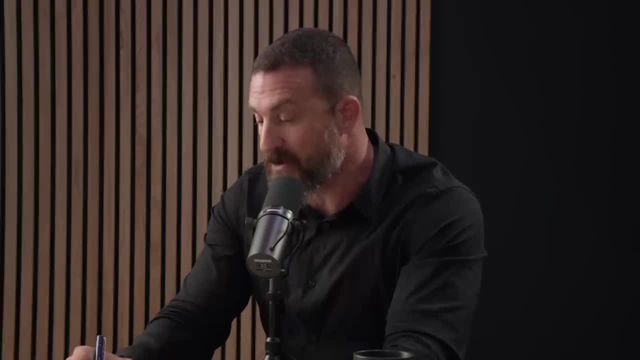 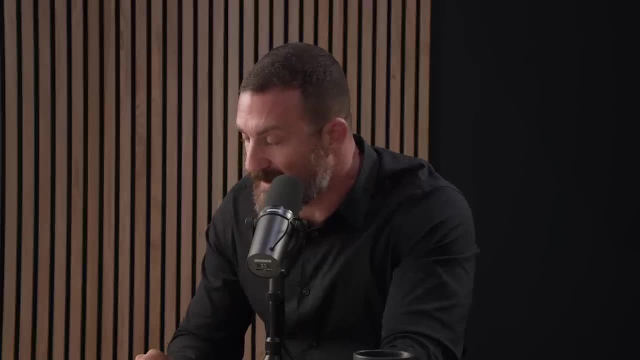 for it. Um, and then the other one is one that- um, frankly, I'm learning more about all the time now thanks to your prompt, which is Redolia Rosea- I think I pronounced that correctly- And um, and why that might be interesting or of use to people. 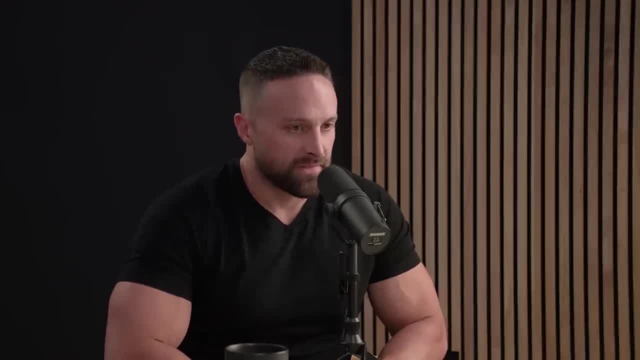 Dr. Yeah, So, touching on creatine, it is the most tested, safe and effective sports supplement we have. I mean, it's just, there are thousands of studies on creatine monohydrate now, And I would, I would say very clearly too: um, if you're using any other form, 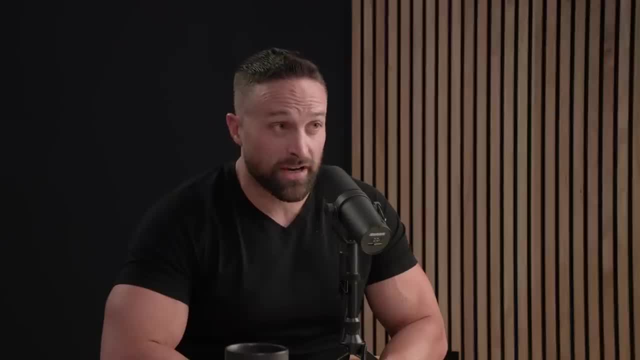 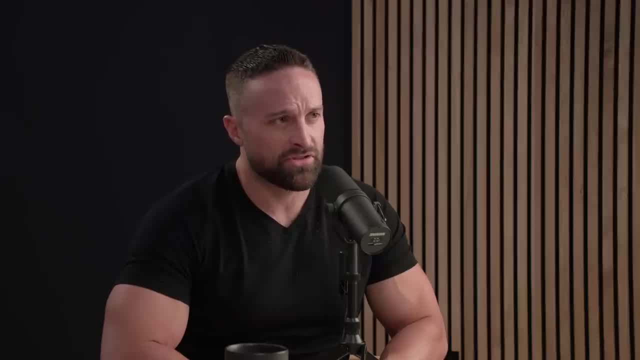 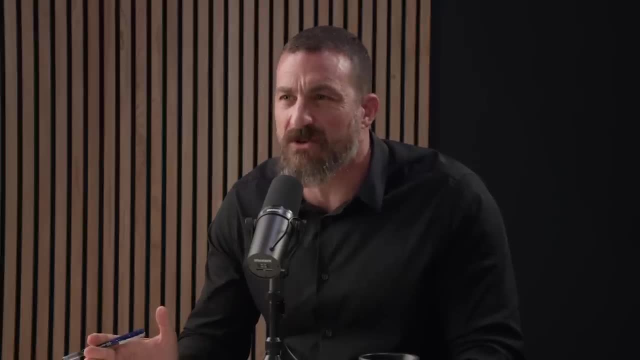 it's. it's apparently it's a little more soluble Um. the claim is that you need less um, but there's only a couple of studies on it and it's more expensive. Dr And creatine monohydrate is not particularly expensive, I realize. 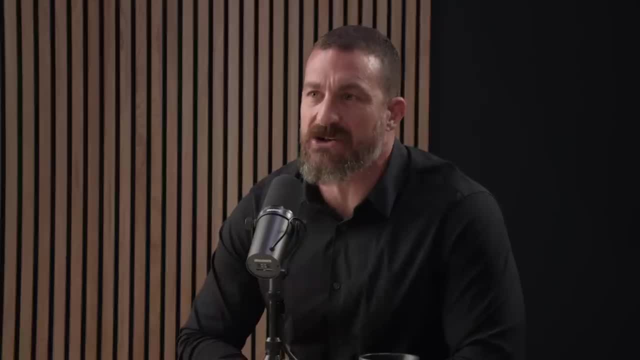 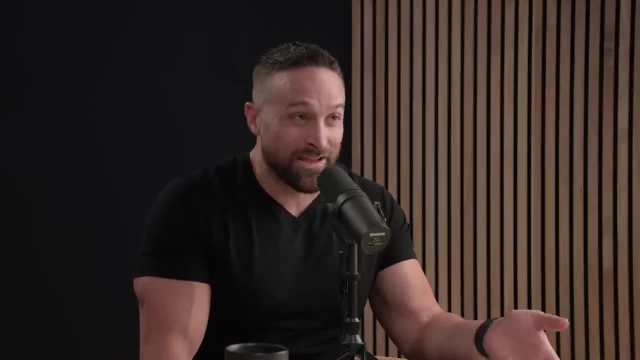 people have different budgets, but it's not. it doesn't land in the. it's not a budget breaker, Dr. Yeah, It's gotten more expensive because of COVID and supply chain issues. Even the there's forms of creatine that appear to be as good like hydrochloride. 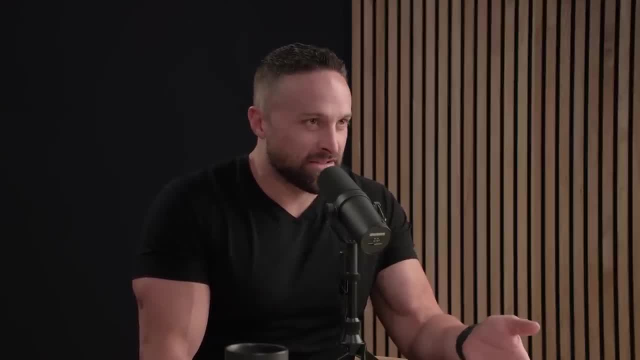 but it's more expensive. And then things like creatine ethyl ester has been shown to be worse than creatine monohydrate. uh, buffered creatine is as good or worse and it's much more expensive. So I tell people: just take creatine monohydrate. It is tried and true. It's been shown to. 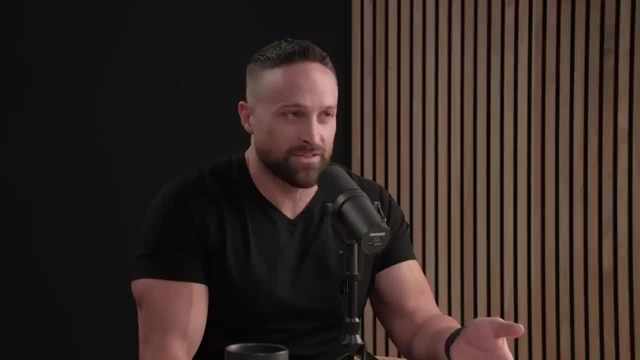 saturate the muscle cells 100% with phosphocreatine, and that's what you want. So creatine uh works through a few different methodologies: one through increasing phosphocreatine content, which helps improve exercise performance. Um, it also appears to improve in cover. It appears to improve recovery. 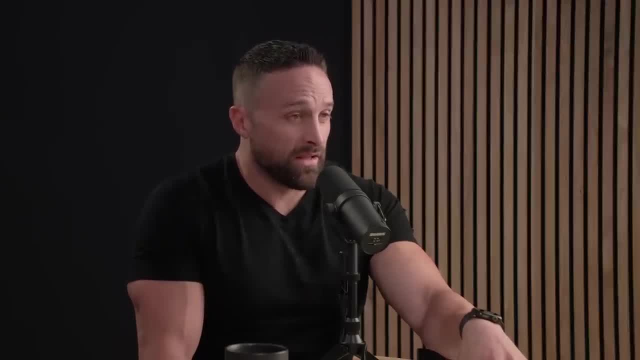 and it increases lean mass, A lot of which is through bringing water into the muscle cells. but that is I mean. muscle cells are mostly water. So when people say, well, it's just water, that's what muscle cells mostly are, Um and uh. it also increases strength and some other. 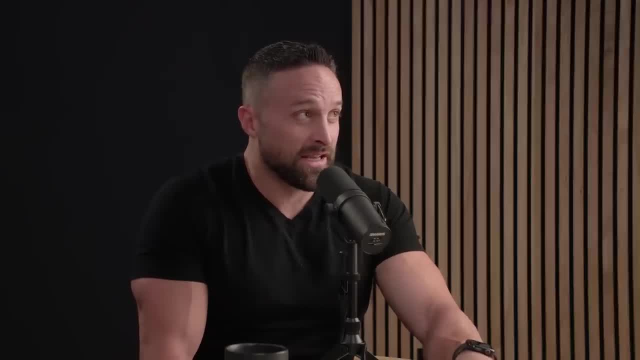 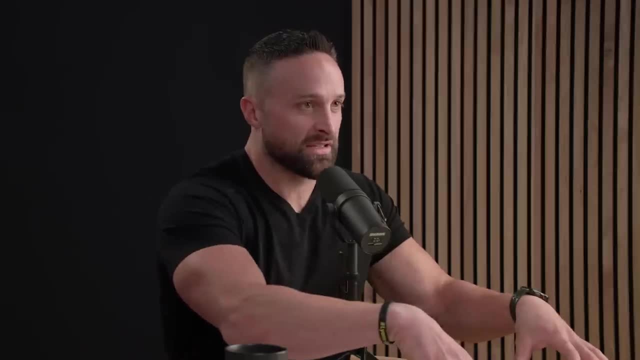 metrics. Now it also has been shown in studies that people tend to get a decrease in body fat percentage. Now, that's probably because they're getting an increase in lean mass, And so the increase in body fat percentage. but there are a few studies to show a decrease in fat mass as well. 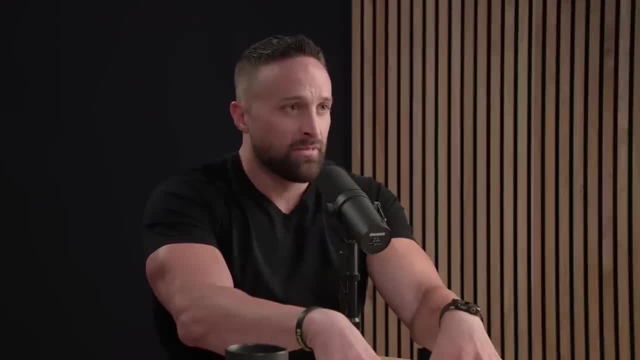 I don't think that creatine is a fat burner. I think that people were able to train harder, build more lean tissue, And so that's probably having an effect on fat mass. Then they've actually shown more recently some cognitive benefits to creatine, which I find. 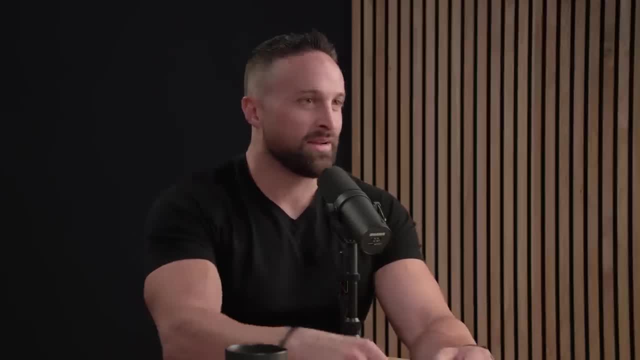 really interesting as well. but the only knock on creatine that anybody's been able to come up with, because they've they've debunked the kidney stuff, They've debunked the liver study. There's no evidence that it harms healthy kidney, kidney or liver. uh is. 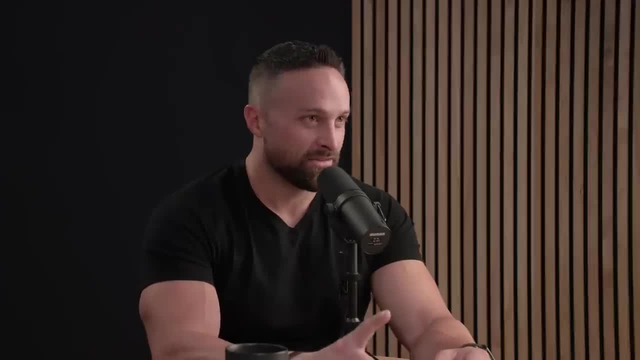 hair loss. So what about hair loss? Cause there was one study in 2009 that showed the creatine increased DHT. Um, but they didn't really show an effect on any other sex hormone. So it's kind of strange. Like you would think, if there was an increase in DHT there would be like something. 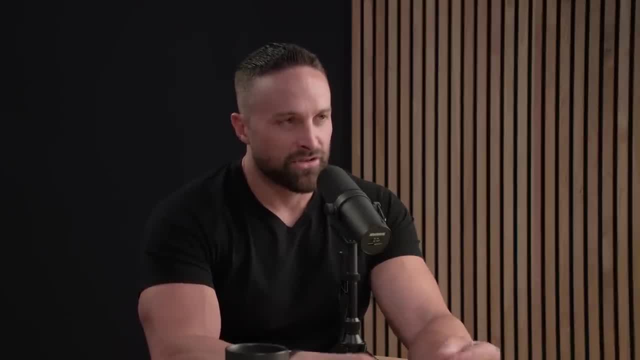 else that changes as well. Um, and it's only one study and, again, didn't directly measure hair loss, measured DHT, which we know is involved in the loss of the follicle, the follicle. So what I would say is that I am not convinced. it's only one study. 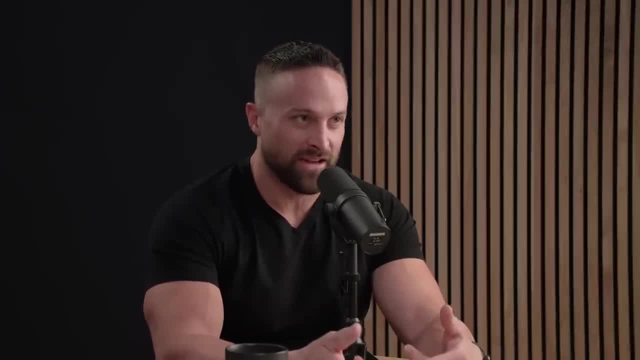 never been replicated, to my knowledge, And it was looking at a mechanism rather than an outcome. So, uh, if you, if you're somebody who's prone to hair loss and you want to avoid creatine because of that, I understand, but for most people, I don't think it's a, I don't think it's something. to worry about? Do you emphasize the classic loading of creatine, taking it a bunch of times per day and then backing off, or just taking it consistently at the I think five grams per day, Yeah Is kind of the typical um dose. That people take. So again, no solutions, only trade-offs. Um, you can load it and you will saturate your phosphocreatine. phosphocreatine stores faster, like usually within a week, Uh. if you just take five grams per day, it'll take two, three, four weeks, Uh, but you will get to the same place. 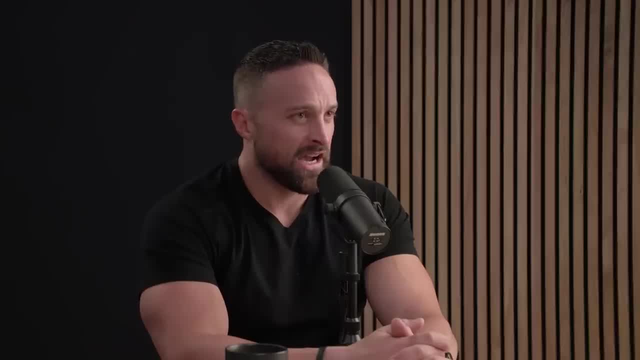 and you're probably going to have a much lower risk of GI issues. Some people, creatine can be a gut irritant. Um, if it is for some folks, I would recommend splitting it into multiple doses, So maybe like multiple two, one or two gram doses per day. 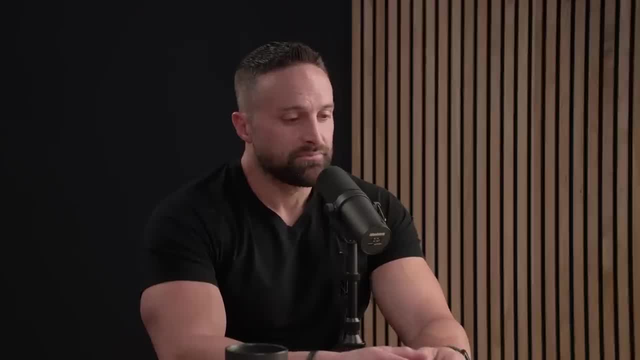 and definitely don't load it If you're somebody who has GI issues from it. as far as uh rhodiola rosea, the research is still in its infancy. I was just reading a new systematic review that kind of concluded that we need more high quality research, but the research that is. 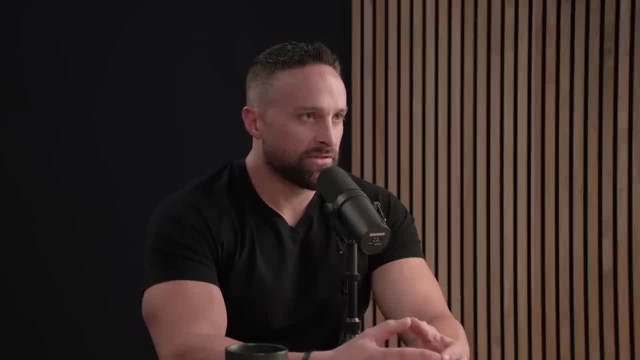 out there seems to suggest that not only does it reduce physical fatigue, but it also reduces the perception of fatigue and may also enhance, uh, memory and cognition as well, And it's referred to as an adaptogen, So I really like it. Um, my anecdotal experience is when I combine that with caffeine. it tends to kind of smooth out the effects of caffeine. It's a more pleasant experience And there's also some evidence that if you're like coming off caffeine then it can reduce the- uh, the negative side effects to caffeine. In the last few years or so there's a lot of eye. to caffeine withdrawal, which, by the way, i didn't really believe in that until i actually did a cold turkey. uh, so before i meet, i will cut out caffeine for seven days, because you can basically reset your caffeine tolerance in seven days and like two days in. i mean, i'm groggy, i've got the headaches. usually i'll get like body aches that come up, because caffeine is actually a mild analgesic, um and yeah, so it's very interesting to see, but i slept like a baby, i'll tell you that i. and then you took caffeine prior to to your event. to the meat, yeah, you really want the maximum punch. 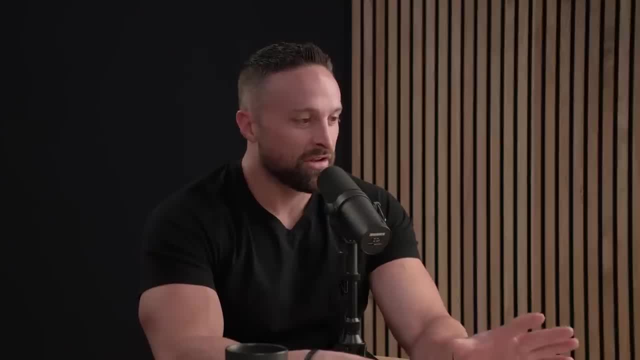 from it. yeah, that's why you do that. yeah, and, like i said, uh, rhodiola tends to. it doesn't eliminate those, those negative effects, but they tend to. it tends to dampen them a little bit. so i really like it again. would like to see more research on it, but there's a lot more stuff. 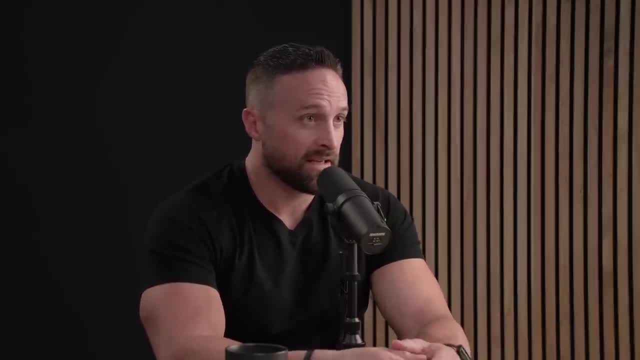 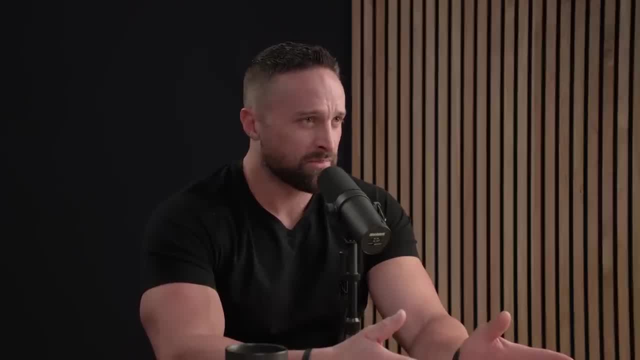 shown increases in lean mass, and they've shown increases in lean mass. i don't think the increase in testosterone uh explains the increase in lean mass. it's just not a big enough increase. could it be the decrease in cortisol people have talked about possible? it does decrease uh, stress, stress. 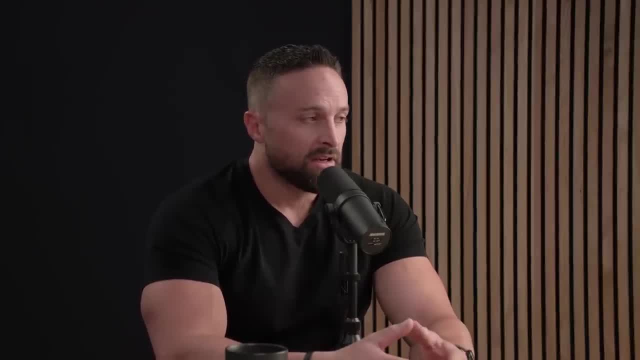 hormones. it also has been shown to help with sleep, um, but i would like to see more research looking at mechanistically how it's increasing lean mass before i kind of say conclusively that this is, you know, the next creatine. there's more research that needs to come out, and then there's some other. 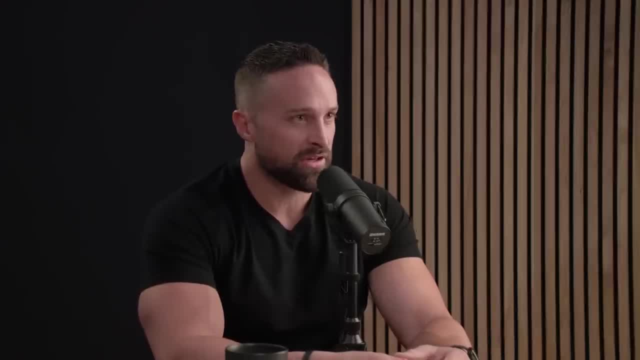 things that that have an effect. um, you know, there's some other things that that have an effect. um, you know, citrulline malate there's. there was a new meta-analysis that showed that citrulline malate can reduce fatigue and increase, i think, time to fatigue, and it may actually have some small 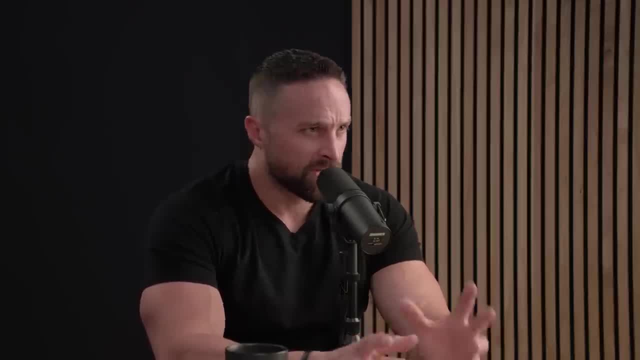 recovery benefits as well. um, different forms of carnity carnitine can actually have recovery benefits and actually interesting- um, i think it's carnitine tartrate actually has been shown. uh, volick published a study that actually showed that it increased androgen receptor. 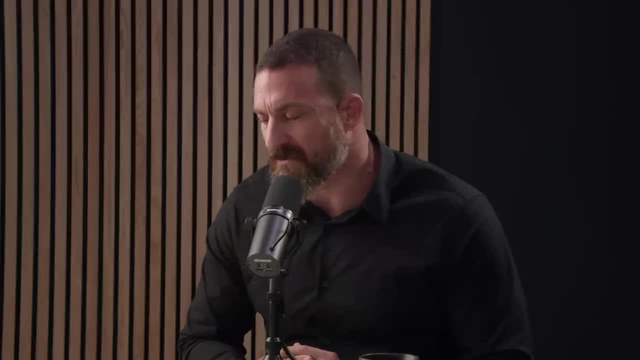 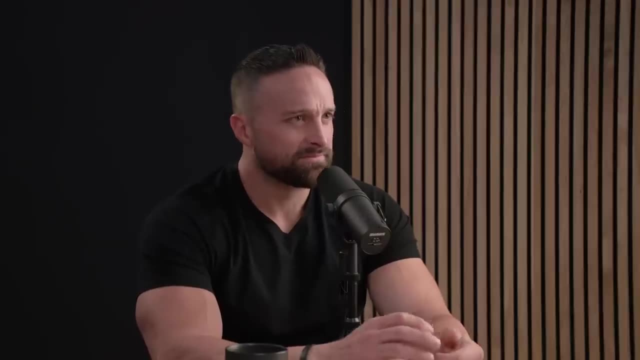 density in muscle cells. that's interesting. now l-carnitine and its other forms- that are pretty. i think there's good evidence that they can improve um sperm and egg health for people who are looking to conceive- interesting, yeah, they're um surprising number of studies on. 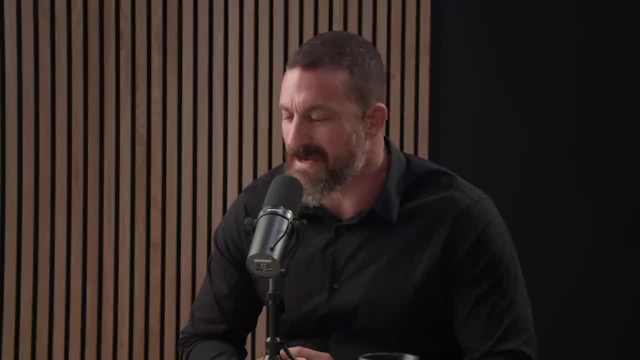 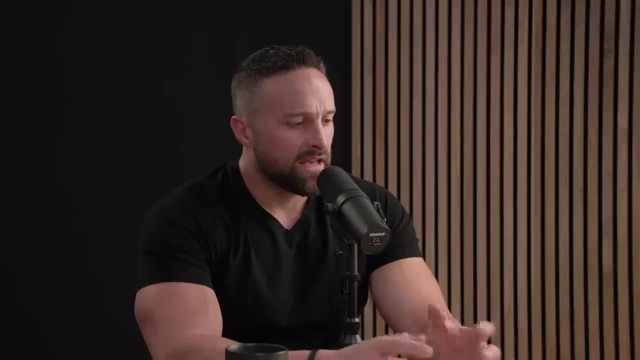 this in humans. um, but yeah, androgen receptor density and that's from oral l-carnitine. people are taking capsules, not injecting directly into a muscle. yeah, and then you've got things like: obviously, like the other most effective supplement out there is probably caffeine. i mean like, if you look at the research studies, caffeine produces very consistently. 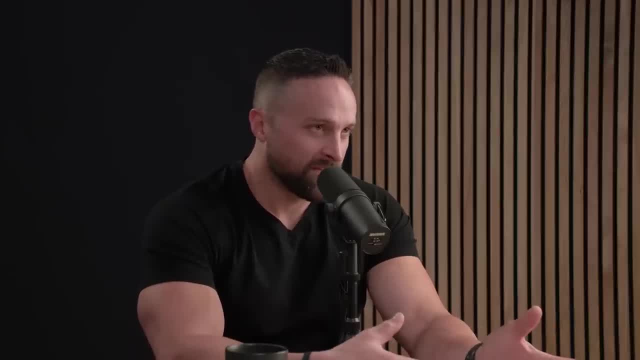 improvements in performance. um, so that's another one. some people don't like the effect of caffeine. that's okay, but i wouldn't know because i've never come off it. yeah, exactly, exactly. well, interestingly, they do show that the effect appears to be consistent, that that, even if you're a 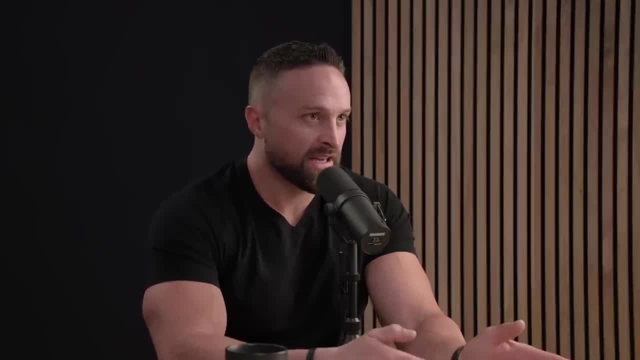 habitual caffeine user. you do still get a benefit every time you take it, but, like you said, you're just used to it, you know um, so you know there's those things. you then you've got like things like beta alanine, which for it's in our it's in our pre-workout, probably not super helpful for. 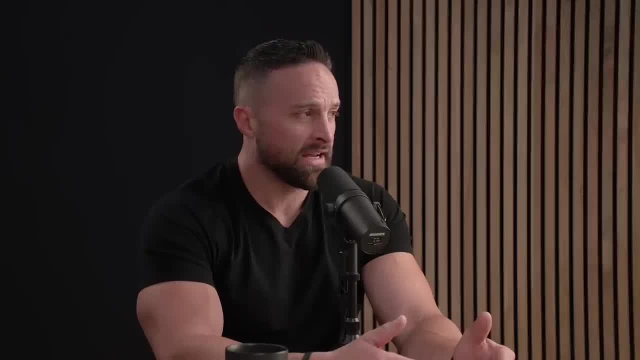 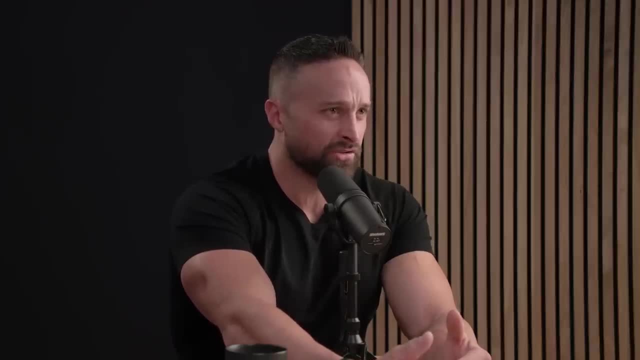 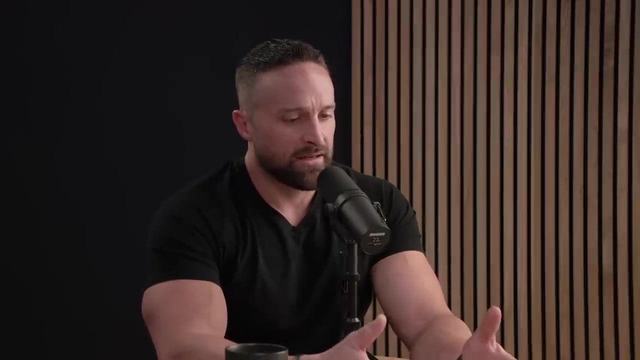 most people for resistance training. it does seem to have some uh benefits for like high intensity, like if you get out you know more than like 45 seconds or 60 seconds of like really hard training. it does appear to help with delaying fatigue for that um, and then you've got things like uh, betaine. 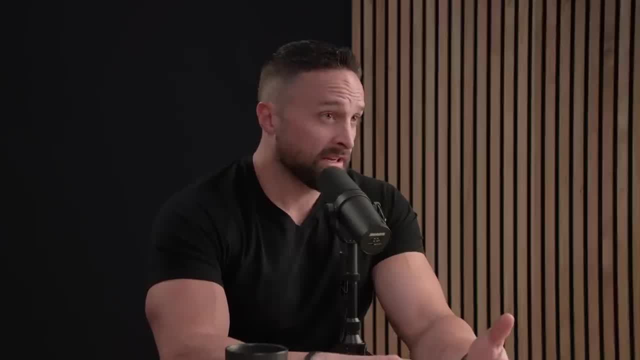 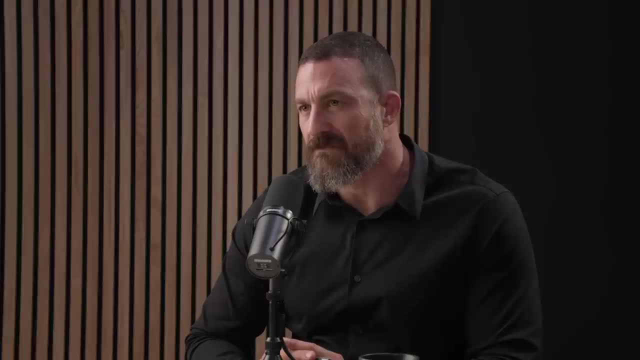 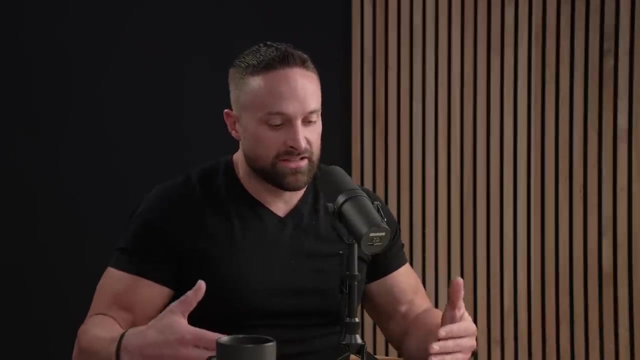 or also called trimethylglycine, which there's some evidence it can improve lean mass. um, there's some evidence that it can um improve power output. so there's a few things out there, but you know, most of the stuff is not very good. so you know, i i think that that's you. 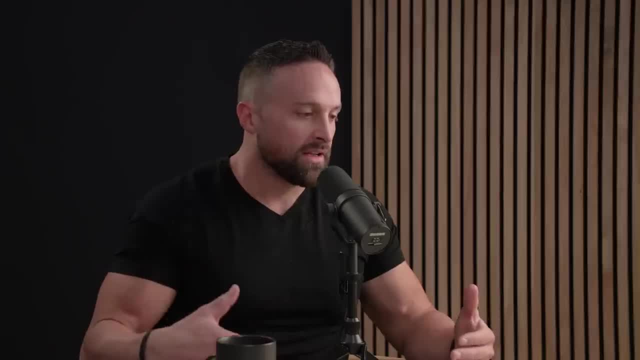 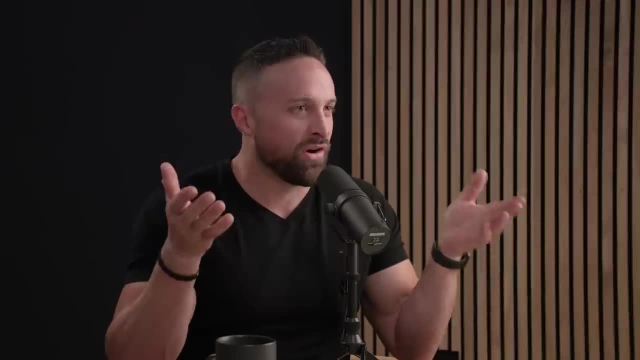 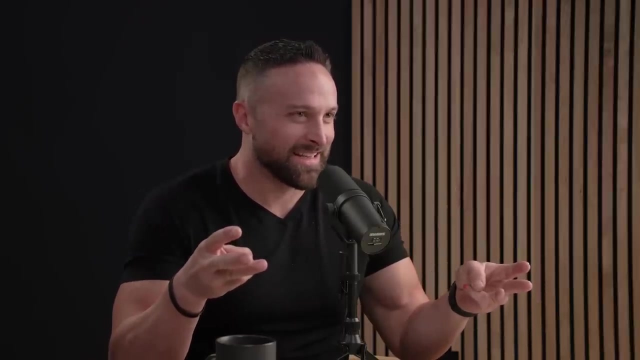 know those kinds of supplements you know, very useful, uh, but again, i would never tell people they need supplements like again, even like something like creatine is going to be a very small effect compared to like proper nutrition, recovery and hard training. you know, uh, one of the things i i was i was talking with ben bruno the other day and uh, i said you know. 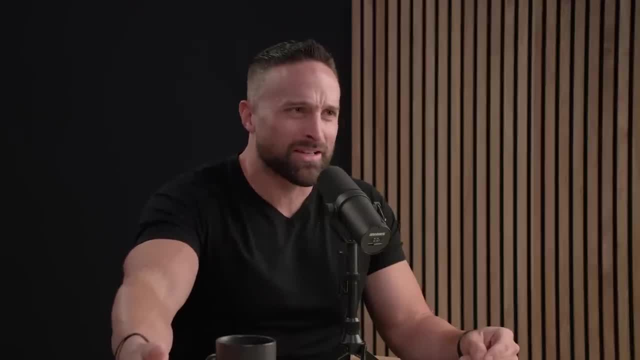 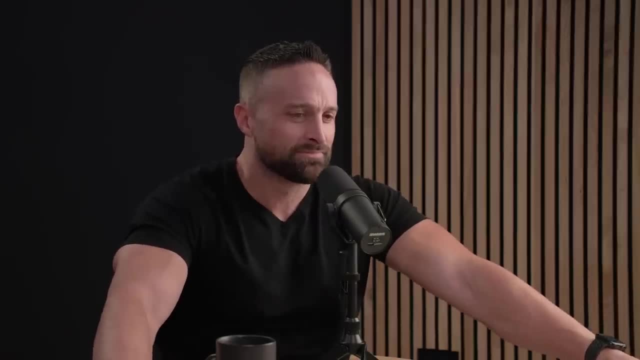 like some people will ask me: like how does this person make progress? because you know their programming is, you know it's not evidence-based. or or you know this guy, how's he like he's? his exercises are dumb. and i'll say, yeah, but they train really hard for 20 years, like you know. 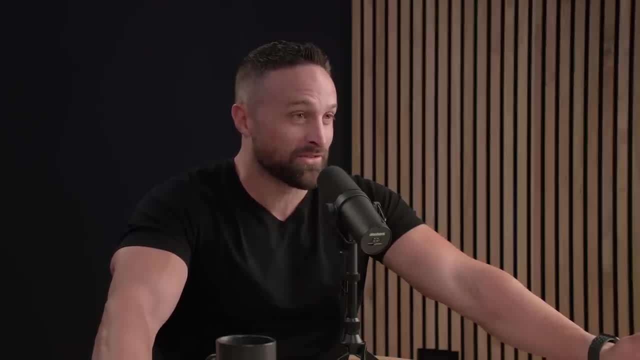 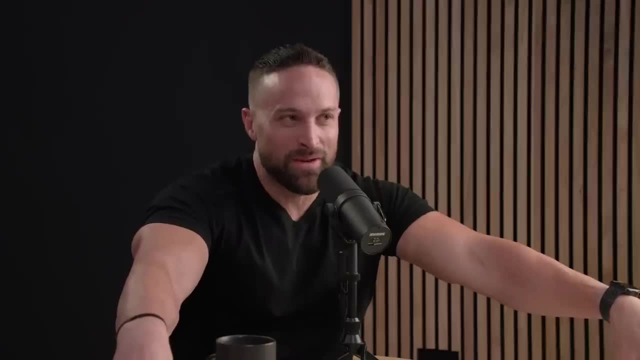 one commonality you see between like really successful athletes or bodybuilders is they train really hard, and one of the things i have observed is the more into the weeds people tend to get- and again this is just my own anecdote and observation- the more in the 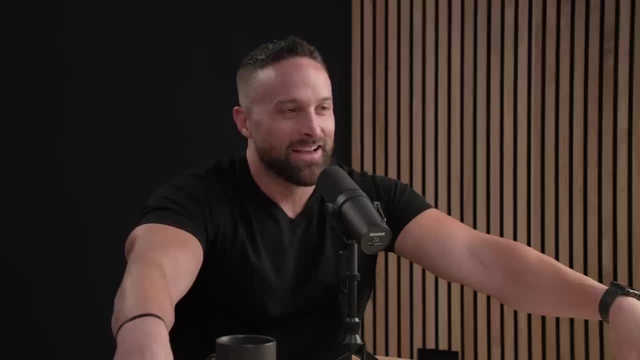 weeds they tend to get the less hard i see them train and so one of the things i really like that mike israel said, who's got a phd and is a bodybuilder himself. he said you can't out science hard training. that if you're looking to build muscle and you're looking to improve your body, 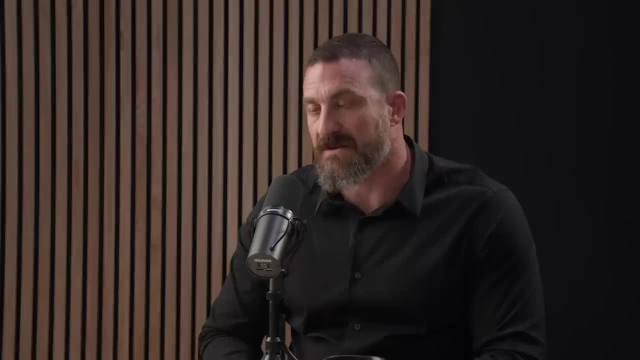 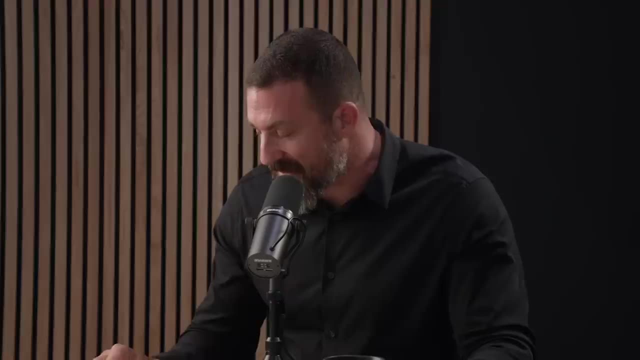 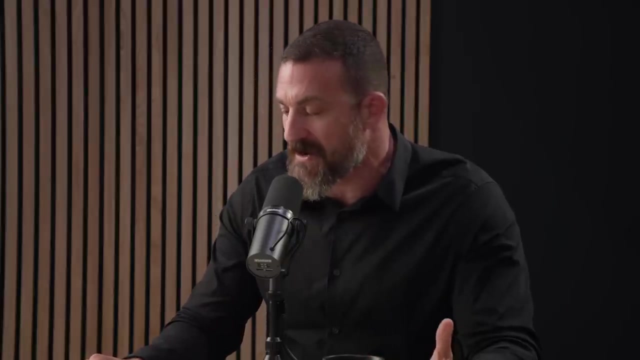 composition. the main thing is just doing the work over time and the hard work, and i would add to that- and this is true- academic endeavors, um too, of course. i think i hope you'll agree absolutely, which is that, yeah, you know. the other thing is, given the mental side. earlier we were talking about how satiety signals 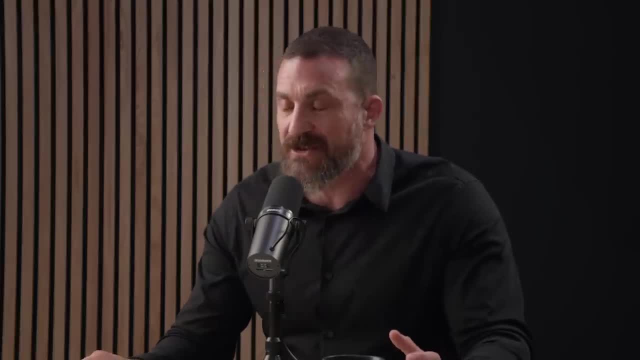 in the brain and what you think about foods can be relevant: learning to really enjoy training hard, in addition to learning to really enjoy eating well, not just for the effects that it has on body competition composition- excuse me those two, of course- but just learning to really enjoy the. 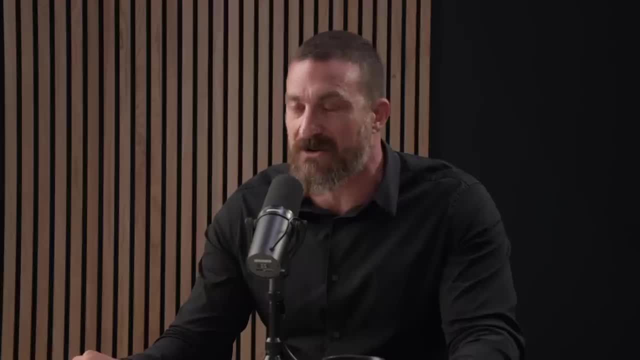 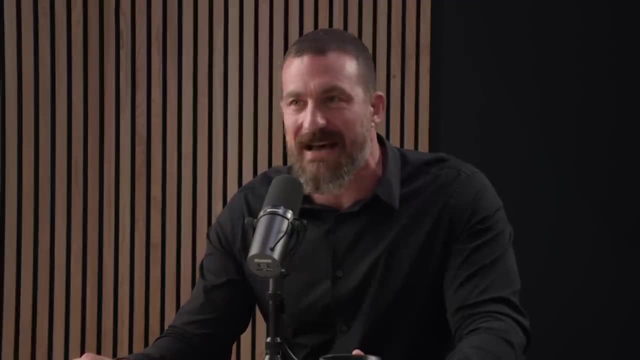 process of training hard and a really hard workout, or a really hard um paper that you have to sort through, or really digging through a book. that's challenging learning to really enjoy. that, i think is is a. if there is a power tool out there, it's. it's the psychological end and i think a lot of that is. 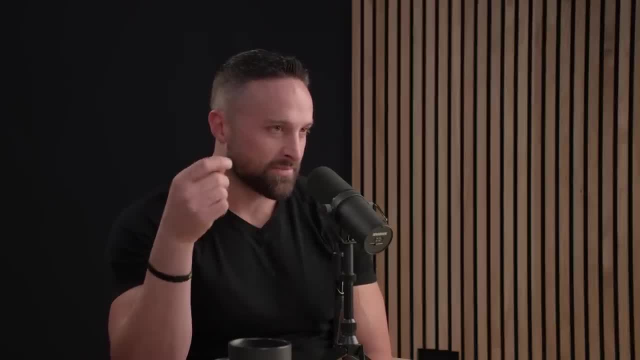 getting the confidence of doing something hard, that there's a payoff at the end. you know, and a lot of people i get asked a lot in my q and a's- how do i get more confident? how do i become more confident? i'll tell people you have to do, you do sobre vale, and then, to answer to one, that's what you do. so think about that, though. 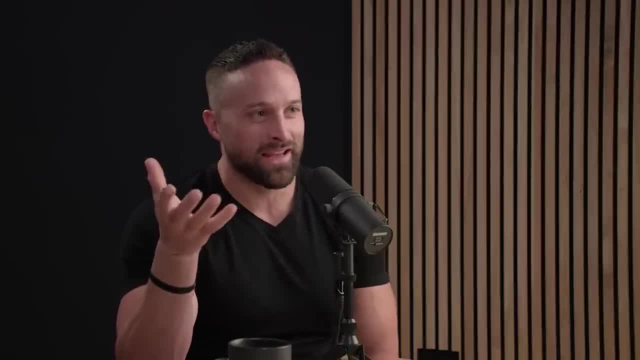 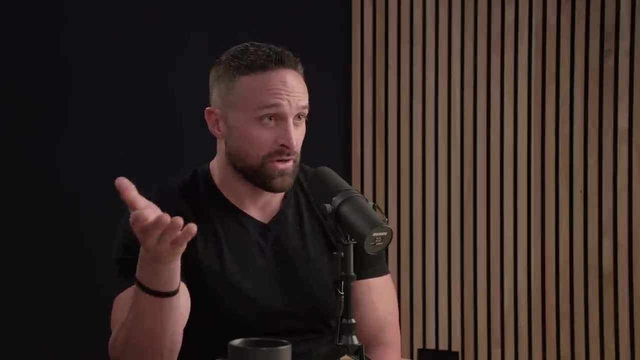 you have. there's no hack, You can't read about it. You got to get in the arena, And I don't mean like compete in sports, necessarily, but like doing a PhD or doing something, just something hard, where you're putting yourself out there and you're saying: this is my goal and I'm going to go for. 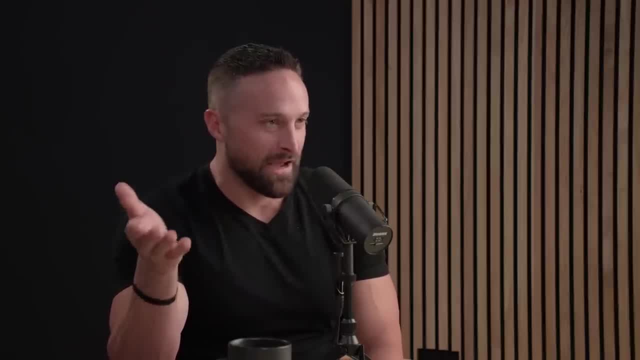 it. You just learn so much by doing that about yourself. Um, and so just what you said, I will reframe things in my mind when bad things happen. from it's not to say I never get stressed out because I do, And it's not to say that I never get down because I do, because I'm a human. 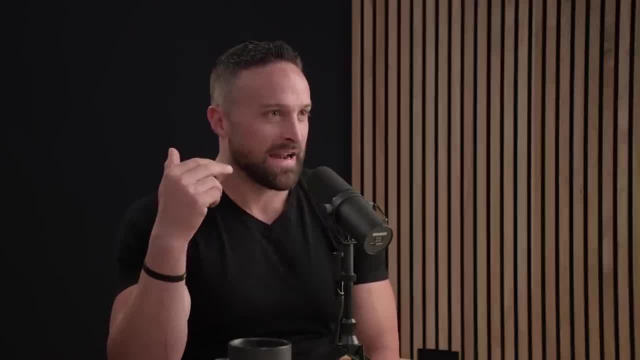 But when something bad happens, I should post about this in my store today. When something bad happens, I very rarely anymore do I go. woe is me. Why did this happen to me? Because you're in the universe, random bad things are going to happen. So instead I say: you know if I'm not. 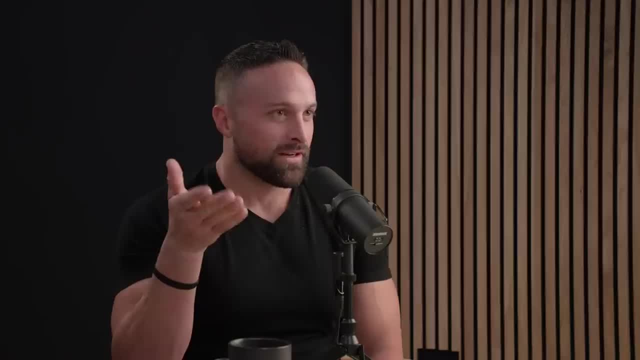 dead. instead I say, well, what an exciting opportunity to overcome an obstacle. And I bet because, in the experience of my life, the biggest lessons and the best things in my life have actually come out of the most challenging, worst things that have happened. And so again, 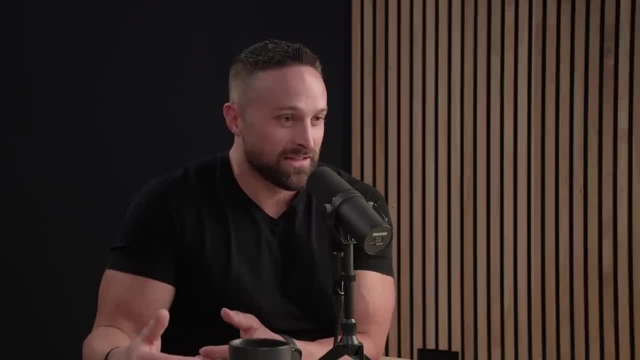 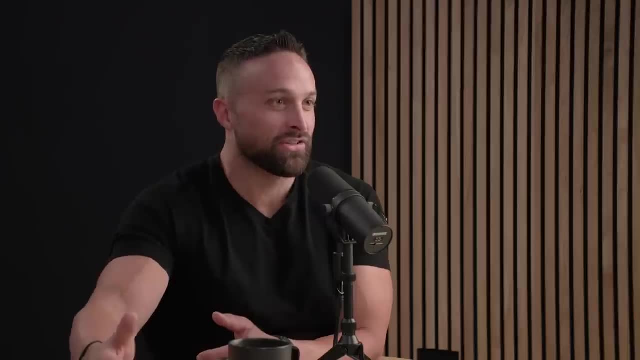 this is. I would never have been able to do these sorts of things if I hadn't taken up weightlifting, because weightlifting taught me so much about perseverance, delayed gratification, overcoming obstacles, And that's why I love it even to this day, And I'll still get butterflies when I go in. 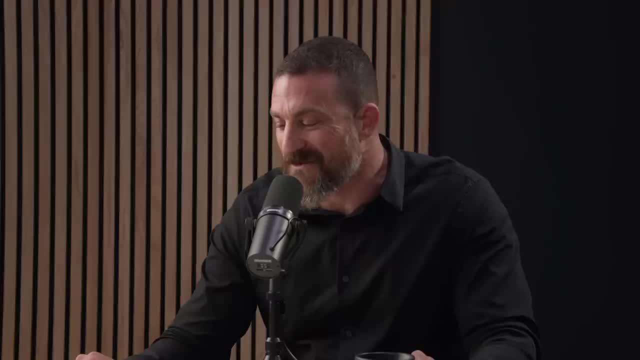 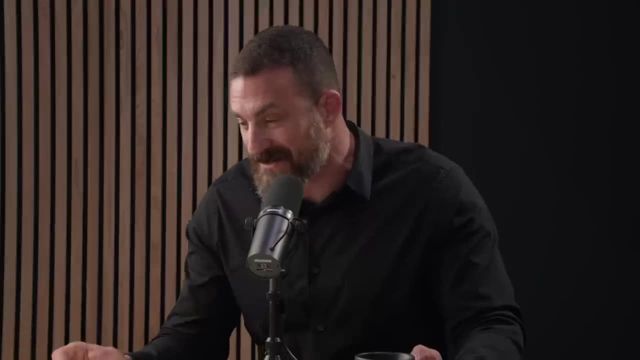 for a squat session, even though I've been doing it for 23 years. That's wonderful. Well, it's clear that you embrace hard things And I for people listening to this. obviously it doesn't have to be weightlifting, you know picking hard things. 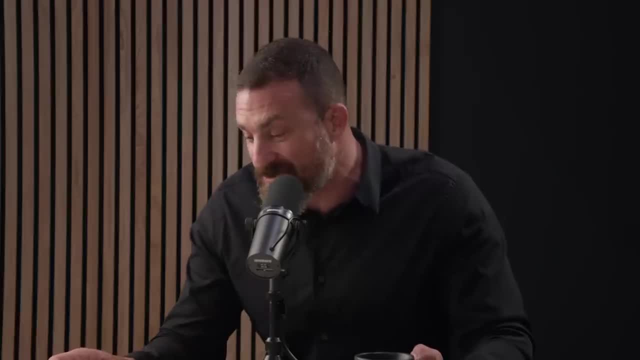 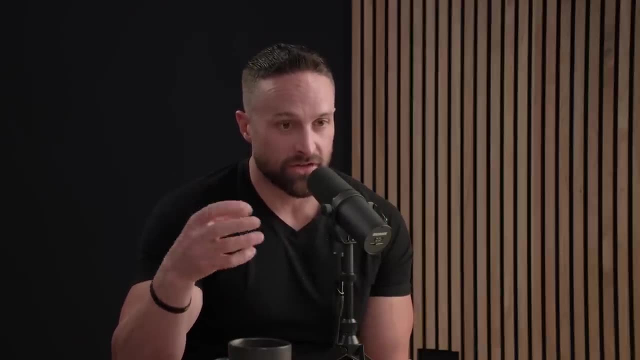 learning an instrument, learning a language Challenge is is a is an absolute builder And they've actually shown, like those sorts of things, like when you challenge yourself and also mentally, that I think there was a new study that came out basically showing a reduction in the 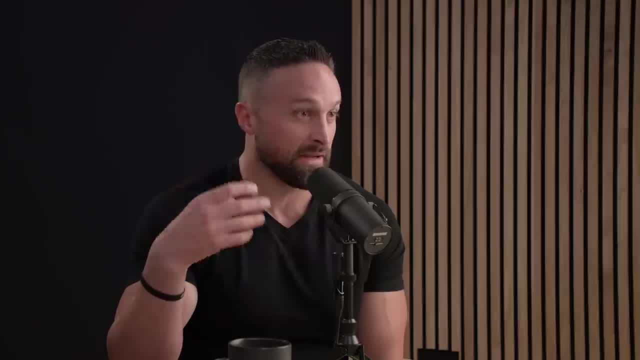 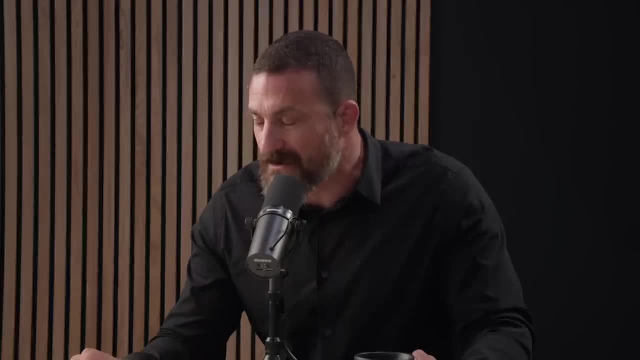 risk of Alzheimer's and other age related cognitive decline. I mean basically like use it or lose it. Right, Yeah, The, the, the will, the desire and the will, um, to persevere no doubt translates to this thing that we we call the will to live. right, It's, it's related. 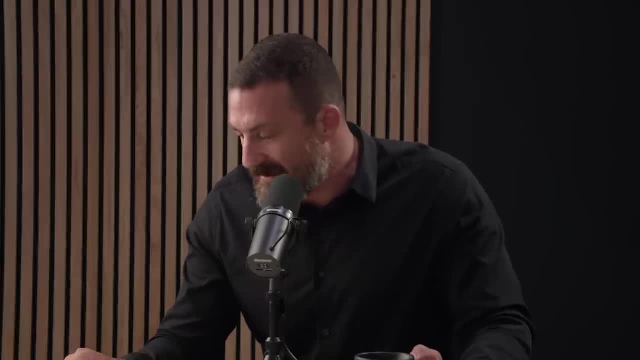 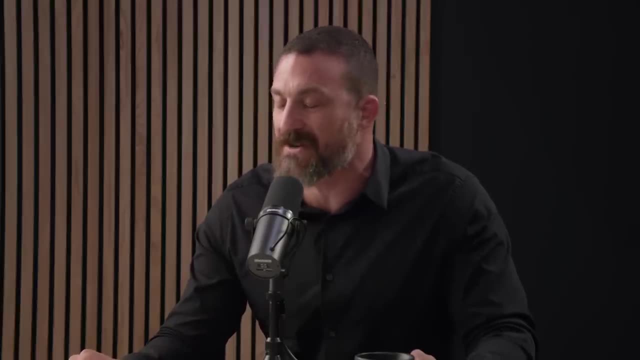 to the will to live Well. I think that what you just said, you know, beautifully embodies what most people are aspiring to, which is to. I think most people actually want to do hard things. They don't just want to have the results. I think that most people deep down. 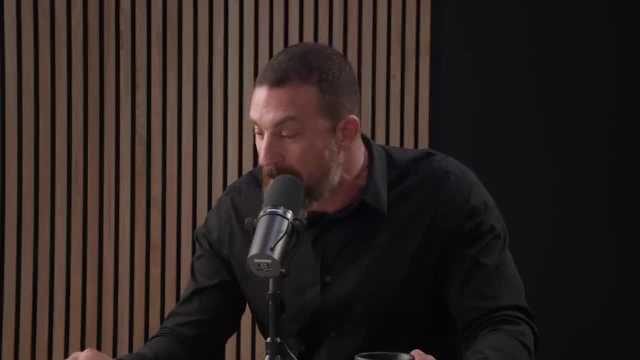 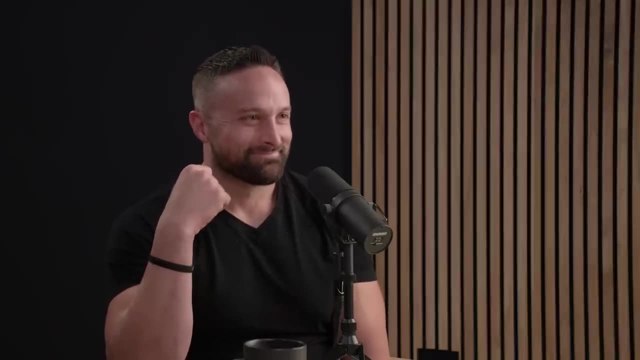 have some understanding that their reward system works that way. I must say this conversation for me has been tremendously rewarding. First of all, it allowed me to meet you in person for the first time, which I've really enjoyed. I'm certain this won't be our last interaction on this podcast and 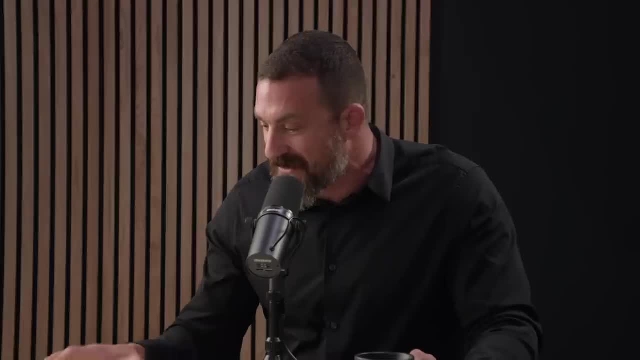 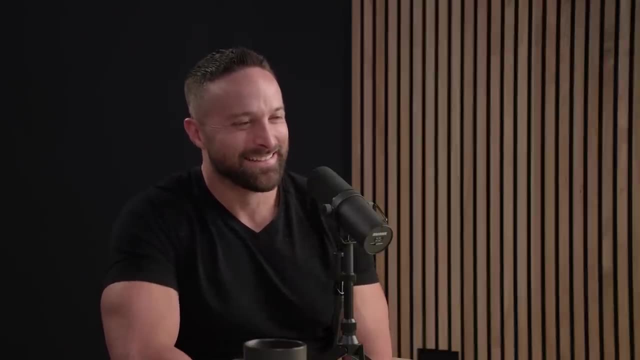 elsewhere. Uh, also, the amount of knowledge that you contain inside you is is astonishing, And there's a lot of stuff rattling around. Well, and, and we all benefit because your ability to pull from the mechanistic side- again, I think in not. 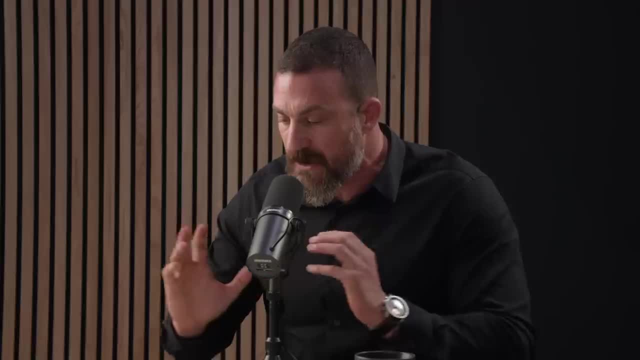 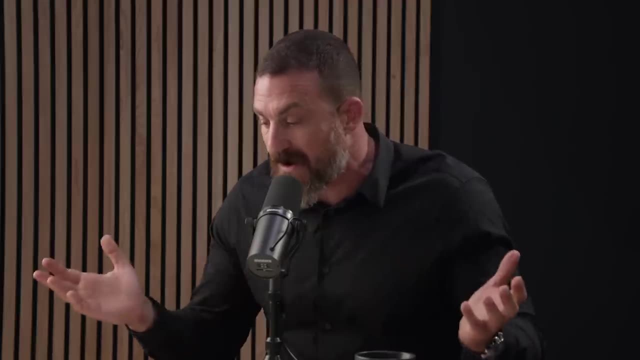 limited to but relate to your background in biochemistry, all the way through to the um, the impact in humans, animal studies, being able to understand where those sit relative to one another. And then you're obviously a practitioner of- uh, you practice what you preach and what you. 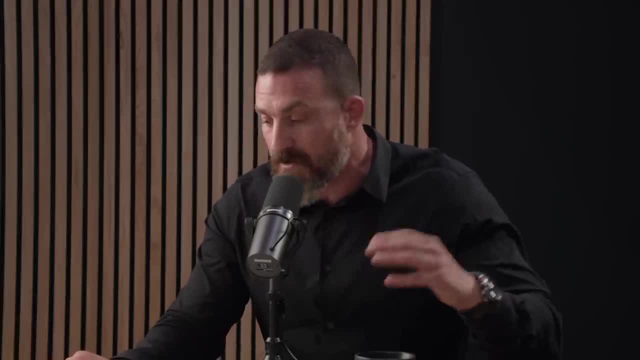 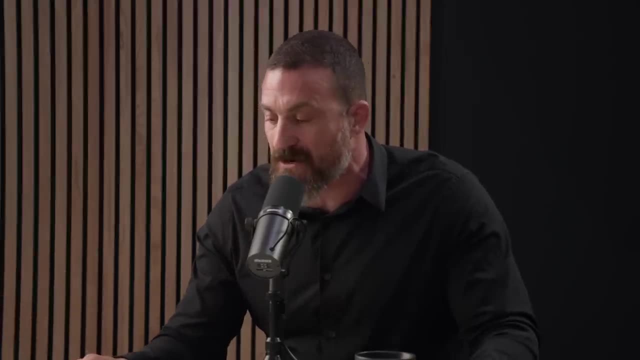 talk about pertains to men, to women, younger people, older people, people who are vegan, keto, carnivore. you really are able to net a tremendous number of ideas while staying really nuanced and data-driven, And so I just want to thank you for that. 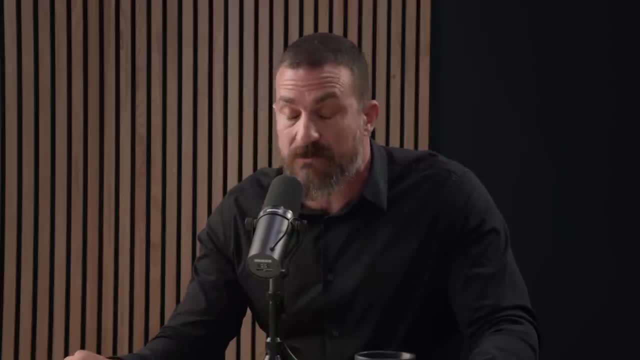 I want to say, for myself and on behalf of the listeners, really appreciate you coming in here today and and sharing with us your knowledge. We will absolutely point people in the direction of um, where they can learn more about you, And um, one of the places, uh, that I want, I definitely. 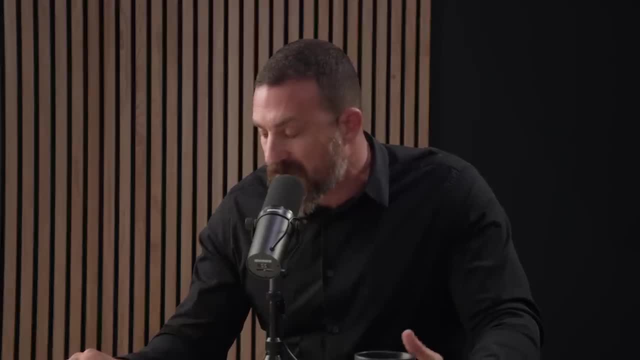 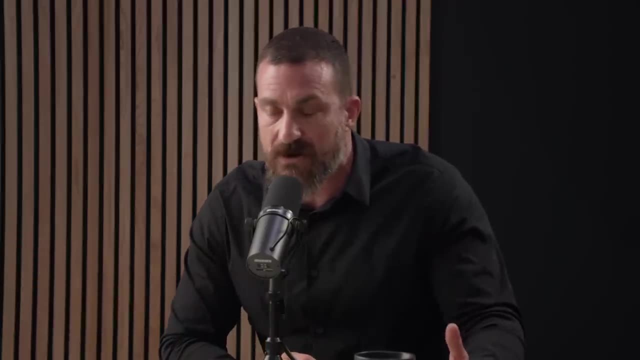 want to mention before we we part, however, is um, this carbon app, And I should just mention I'm not, this isn't a paid promotion or anything of that sort. Actually, one of our podcast team members is has been using carbon for a long time. This is an app that you devised, which 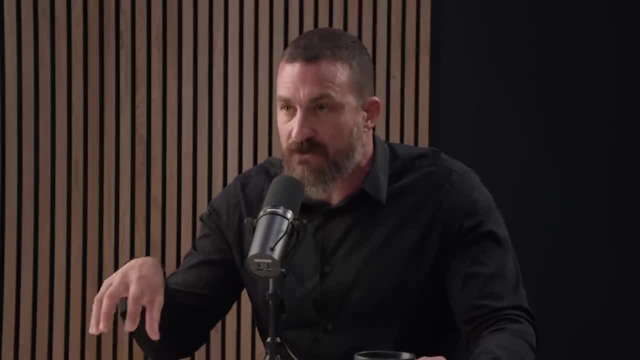 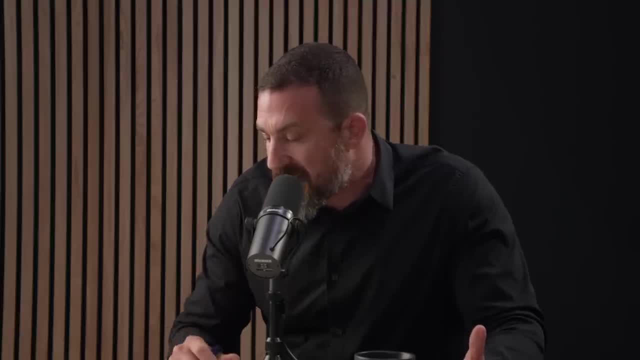 conclude, um, without necessarily telling us everything that's in the carbon app, I'd love to know what are the major things that it does and is good for. and then, what were some of the key things that you wanted to make sure were in there when you built it? Like what? what's the sort of 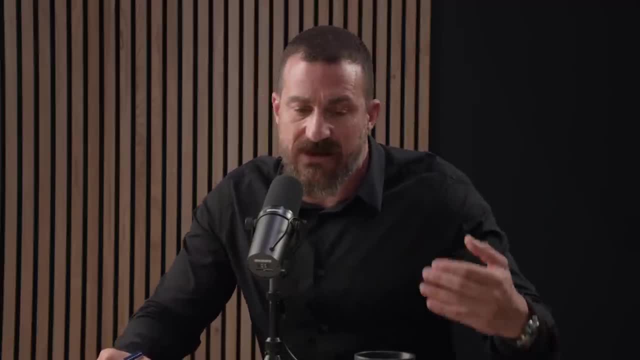 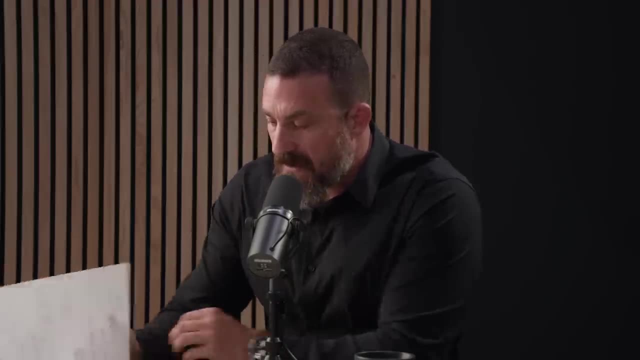 backbone behind it, Cause I think there are a lot of um food counting, calorie counting, exercise apps out there. Um, everyone I've talked to that uses carbon, um including, uh, our mutual friends cigar and Getty. this member of my podcast, et cetera, raves about it. So what is? 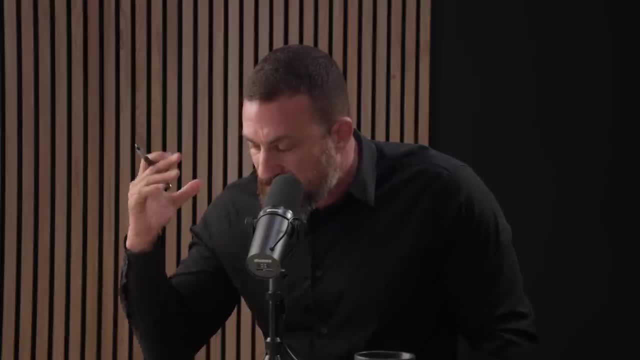 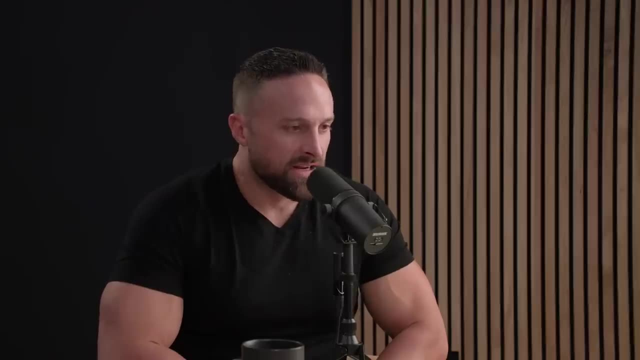 carbon and and what does it do And what was your mindset in building it? What did you really want to see there that you didn't see elsewhere? So those listening may not know, but I really I started online coaching people for nutrition back in 2005.. And that was the the vast majority. 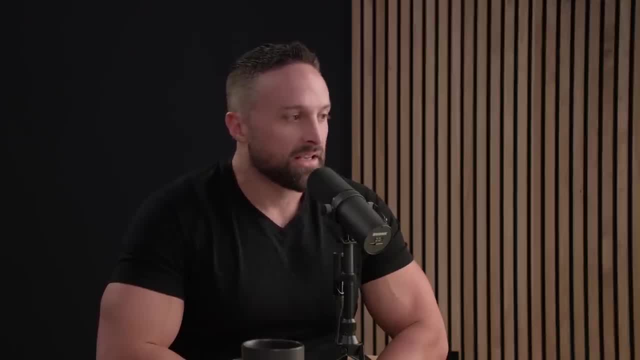 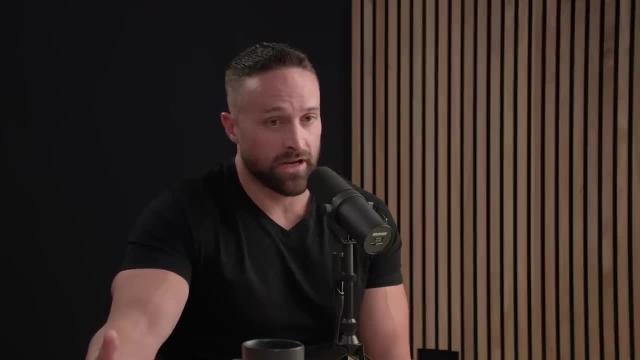 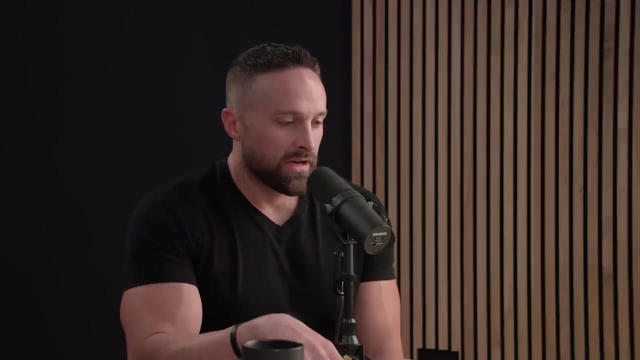 of my business all the way up until like 2017.. And I had a lot of success with that where- whether whether it be just average folks looking to lose weight or build muscle and right up to elite level- uh, competitors in physique sport. So I kind of had this idea, like I don't want to say I had 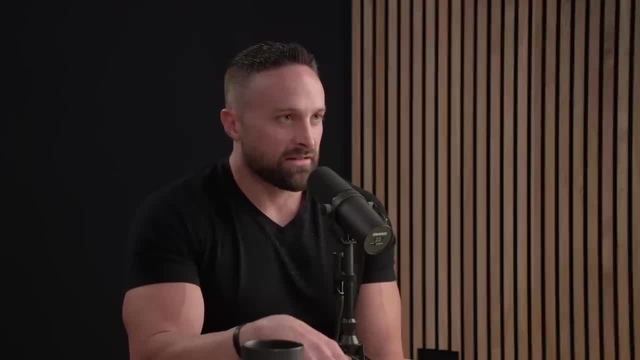 the idea. A few people had the idea: What if we could take what I do in coaching and try to automate as much of that as possible? And I think that's. I think that's a really good idea Because you know, by the time I was becoming a really popular coach, I mean I was expensive. You. 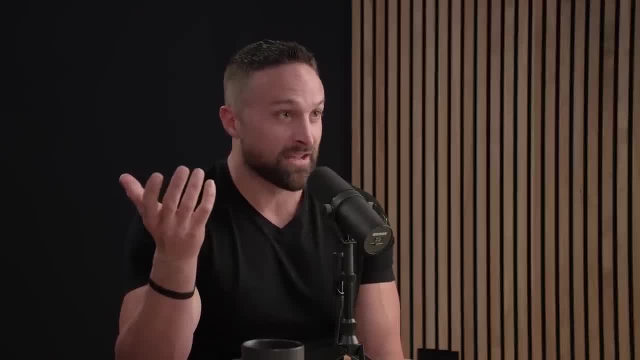 know you were looking at, like you know me charging. I got to the point where I was charging about a thousand dollars a month for coaching Right, And not all. most people cannot afford that And I would like to not just coach rich people. You know what I mean. Uh, I would like 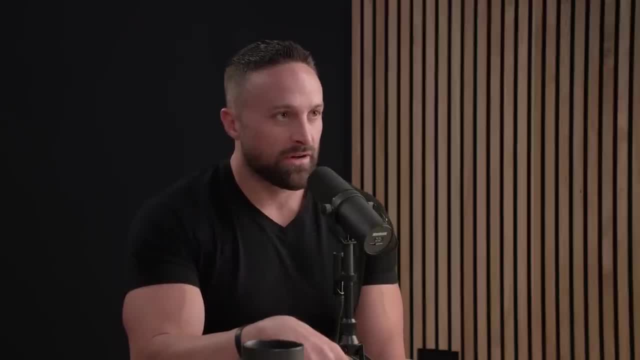 to be able to help other people, So the idea was to create an app that could do some of this stuff. Now, there's always a place for human interaction, but for people who who can afford that, our app is basically 10 bucks a month, And basically what we wanted to do was 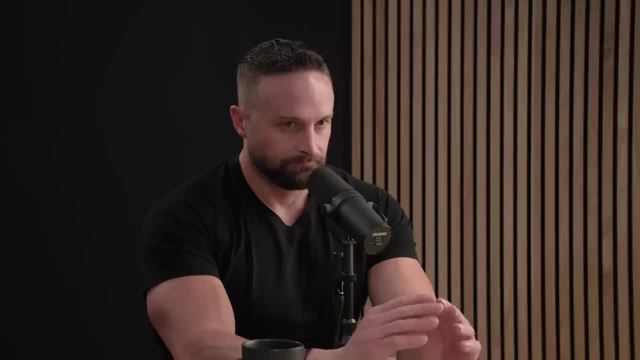 set up an app where. think about if you went to a nutrition coach. what would they do? They would probably ask you some questions about your goals. uh, take some anthropometrics, um, and then they would use like that information, maybe dietary preference, And they'd use that information to. 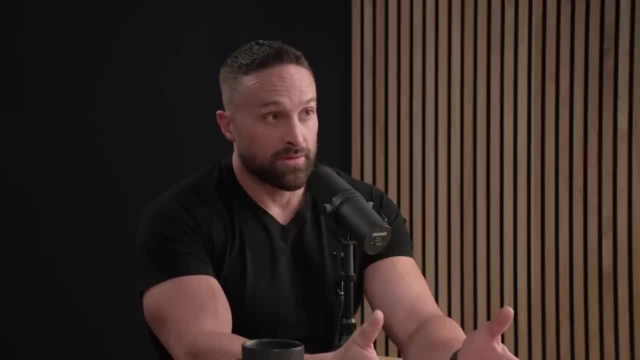 kind of formulate a baseline plan. That's what carbon does. So we ask you- I think there's eight questions in the signup flow- about like your activity, um your exercise, uh your lifestyle, uh your body weight, um your body fat percentage, And if you don't know it, we help you calculate it. 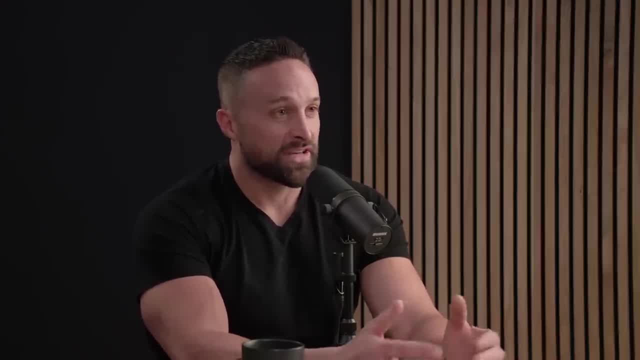 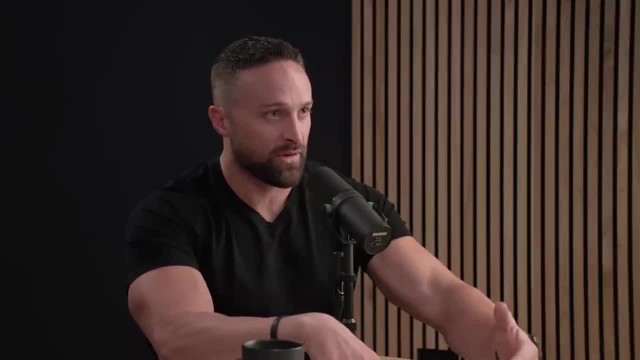 It's not perfect, but it's better than nothing. Um, and then your dietary preferences, And we use that to come up with kind of your baseline. and your baseline will be: you know your calories, your protein, your carbohydrates and fats. And what's different about our app? because, like apps, 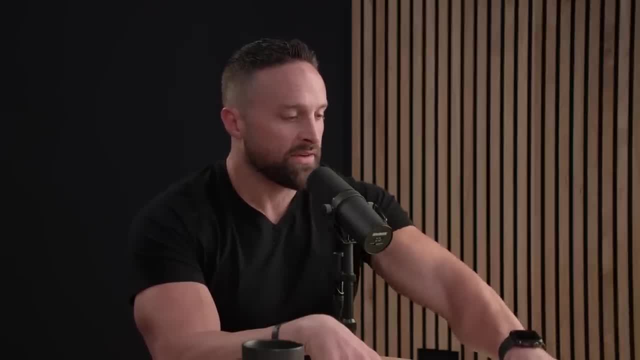 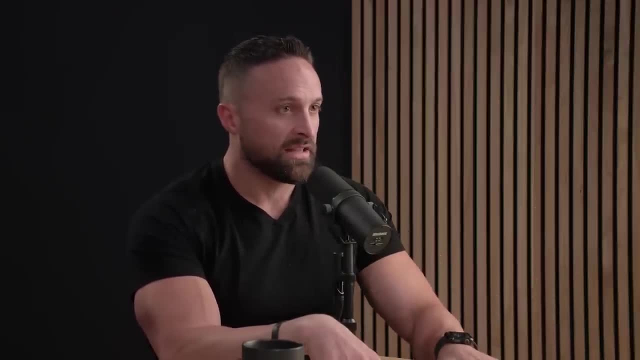 like: uh, you know my fitness power. whatever, we'll do that as well. Uh, what's different about ours is you? we encourage people to log their weight daily for the reasons that we talked about earlier. Um, and then you can also track your food in the app And, honestly, 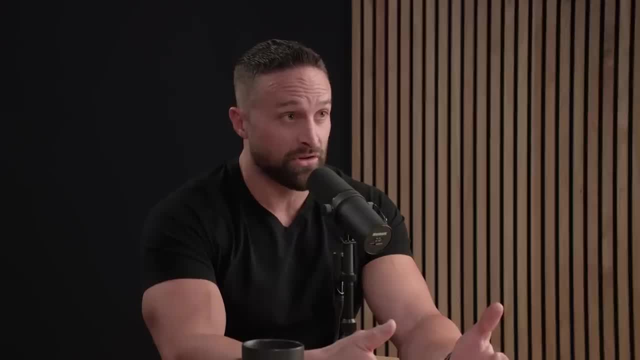 I think our food tracker is actually like way easier to use than most of them out there are are. what we typically get great rave reviews about is how user-friendly our interface is, that it makes intuitive sense, And so you track your food. try to hit these, these macros that you're. 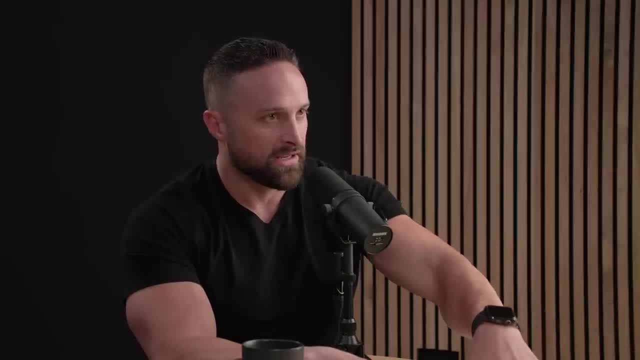 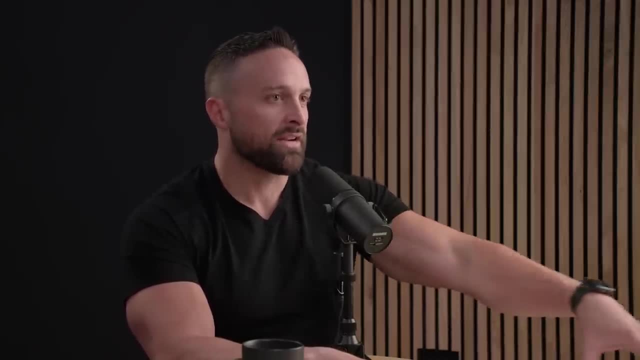 prescribed and Each week you will be prompted to check in with the coach on your check-in day And then you you put in some information and then, based on how you're progressing, the app will adjust or not adjust based on how you're progressing. So, for example, if you're hitting a weight loss plateau, 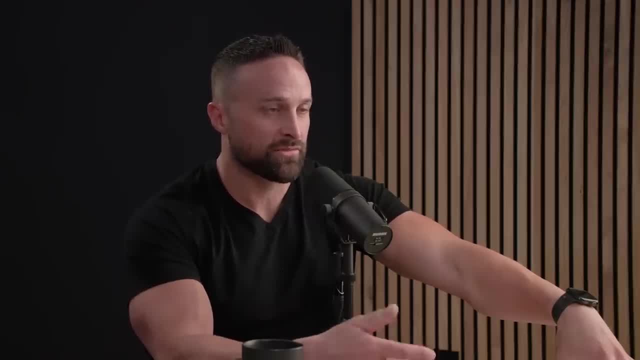 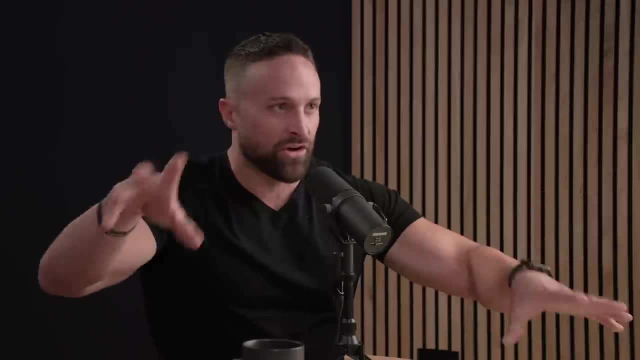 it will sense that and it will, you know, reduce your calories. or or, if you're trying to gain weight and you're, you know, hit a plateau, it'll increase your calories. And there's a lot of, you know, backend algorithm stuff. 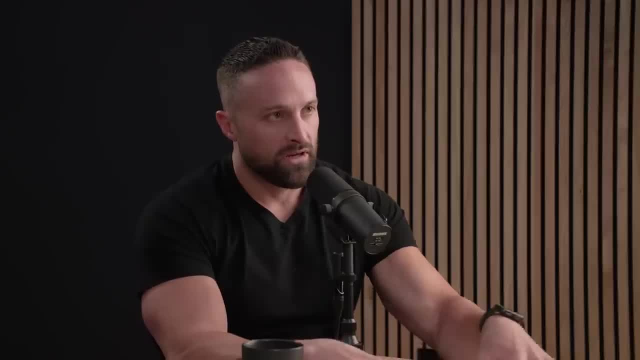 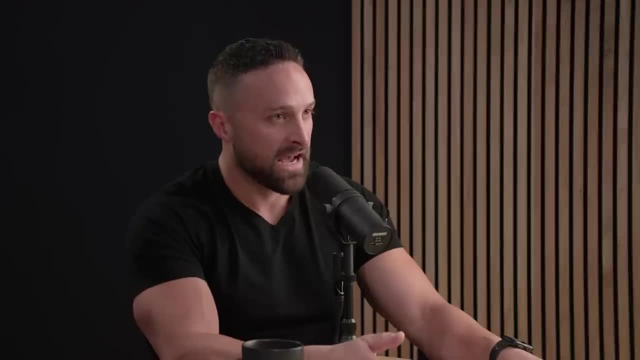 That. that takes care of this, but the fundamental crux of the app is we. we try to determine your total daily energy expenditure, because that's gonna tell us the first big thing we need to know, which is how many calories do you need to be eating for your goal, Right? So? 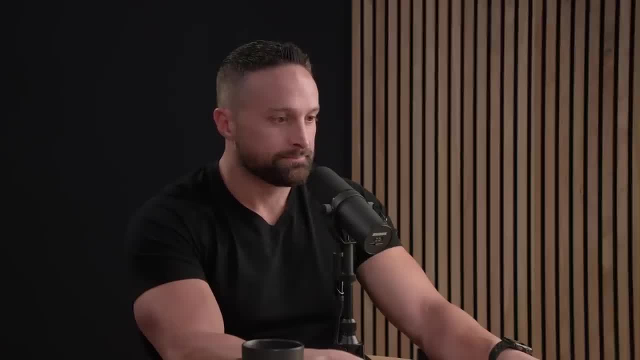 On the front end, we, we basically um, do our best guess based on your anthropometrics. not gonna be perfect, but it'll get us in the ballpark. And if you do know- like some people already know well, I know what I maintain my body weight on. There's 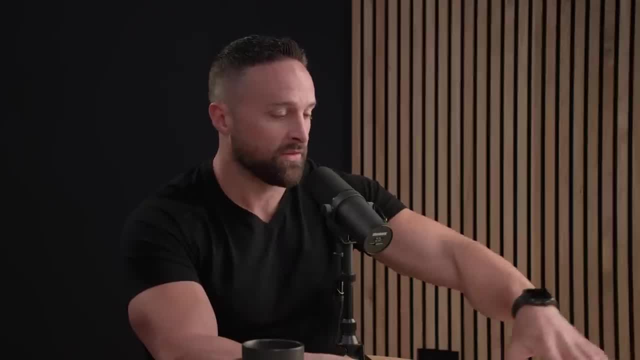 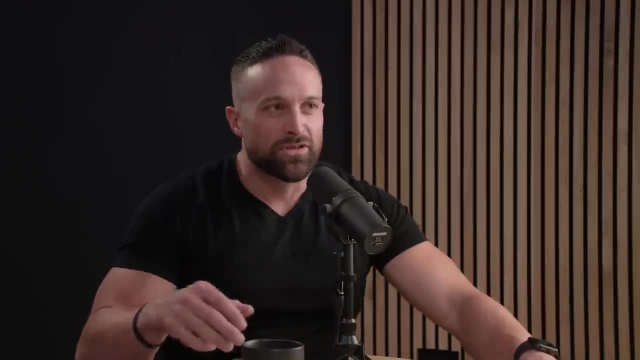 a spot where you can manually enter that during the signup flow, So that's helpful for people who are super nerds like me. Um, but then if you're just, people will ask: well, do you, do you take Apple watch data, Do you take this, Do you take that? And no, for the reasons we talked about. 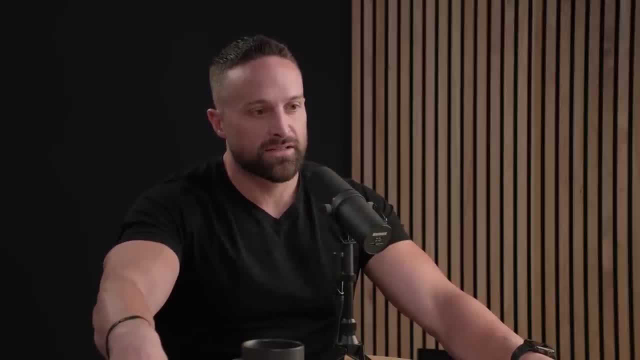 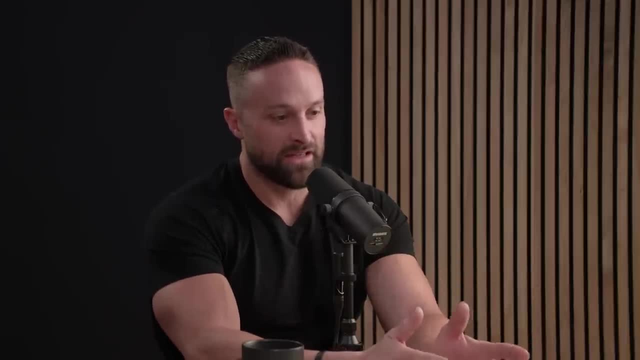 that it overestimates energy expenditure. What our app does is- it's an algebra equation: If you, because your body weight, your, your maintenance calories, is your total daily energy expenditure, your average calories that you eat to maintain Your body weight will be the same as your total daily energy expenditure. 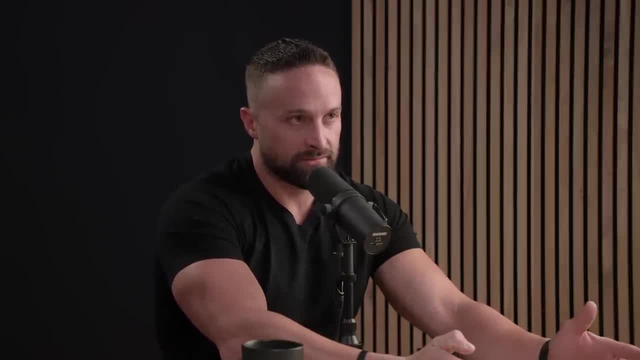 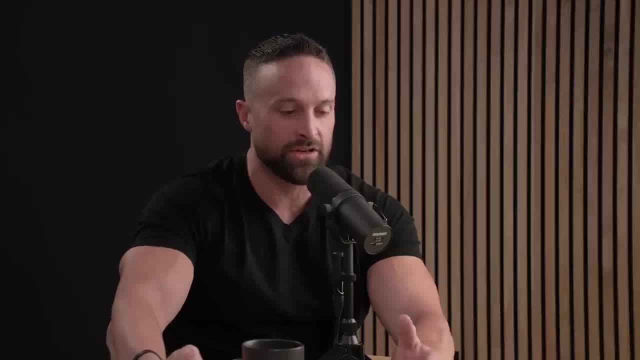 So if we know how body weight is changing and we know how many calories the person's consuming, we can actually solve for what energy expenditure is Right And you can see in the app that will. uh, there's a kind of a a maintenance calorie tracker or energy expenditure tracker, And typically after about three to four weeks. even if the app was off at first, it will have you pretty darn close because, like, let's say, somebody um comes on and they, their goal is to lose, you know, a pound and a half a. 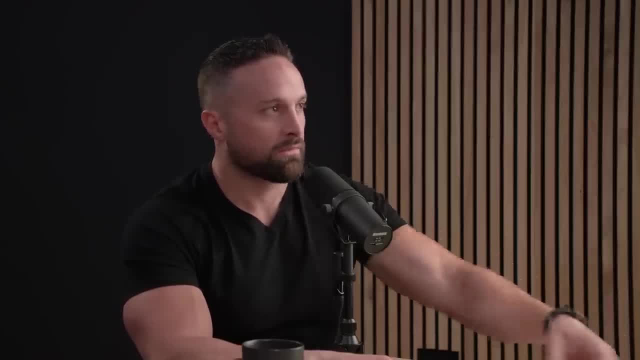 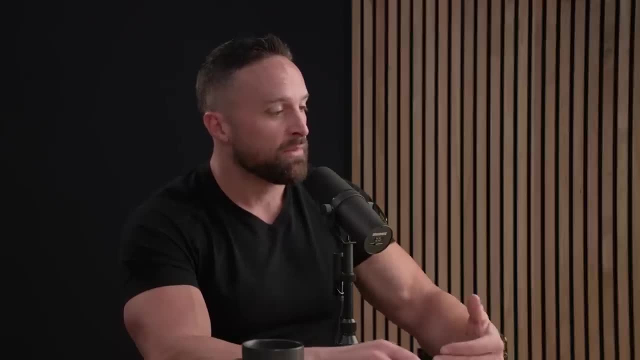 week or something like that, And the first week they lose three pounds. Now the app actually accounts for the fact that you can lose more water weight the first week, So they probably wouldn't get an adjustment. but let's say, the next week they lose three pounds, The app will. 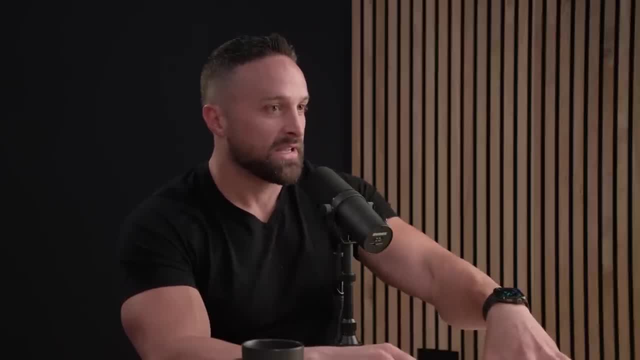 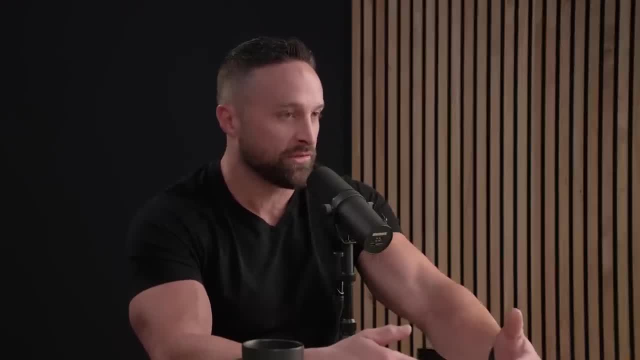 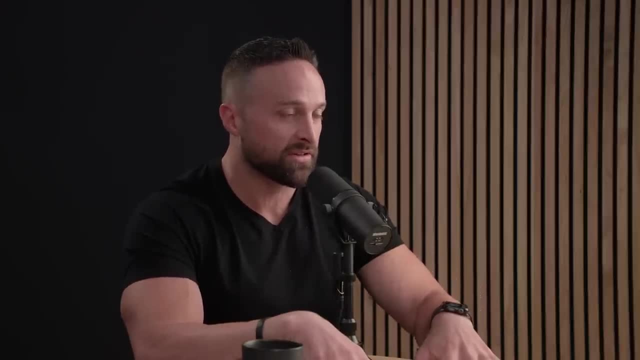 Based on the amount of weight they're losing. And the same thing goes in reverse: If they're not losing the amount of weight that they're supposed to, uh, it will lower them based on the fact that it may have overestimated their energy expenditure. But um, that's the first. 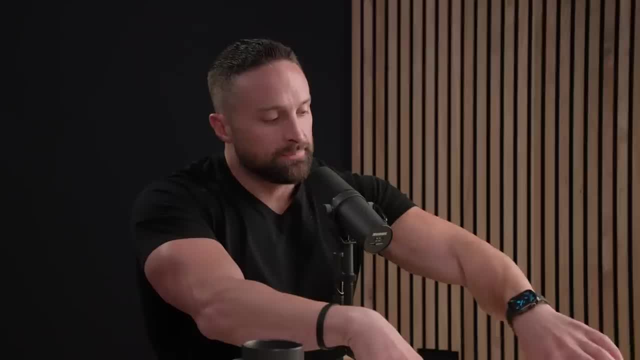 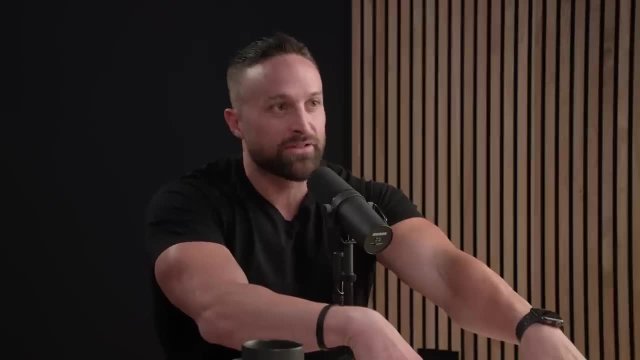 crux of it is tracking that energy expenditure And then the next thing is protein. So when the the backend algorithm stuff is happening, calories are set first based on your energy expenditure and your goal. So, for example, if you have an, if you're on an aggressive diet. um, your calories are going to be lower, even if your energy expenditure might be a little bit high. Um, just because if you're trying to lose two pounds a week, I mean you're going to be in a pretty aggressive calorie deficit. So it's going to set the calories first, Then it will set. 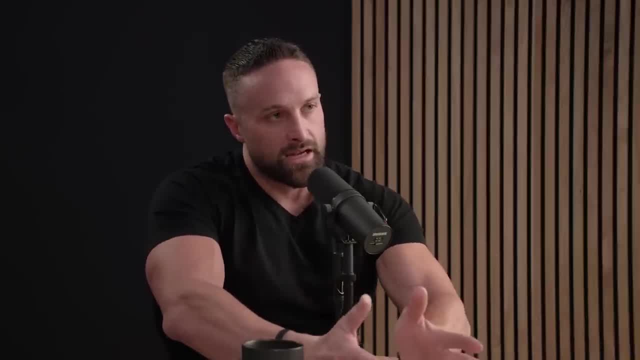 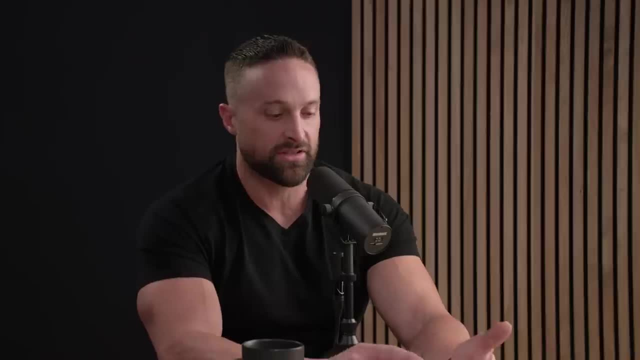 protein based on your lean body mass. Then the calories that are left over will be allotted to carbohydrate and fat, depending on your dietary preference, And we have a few different dietary preferences. There's balanced, which is um about 50, 50 to. 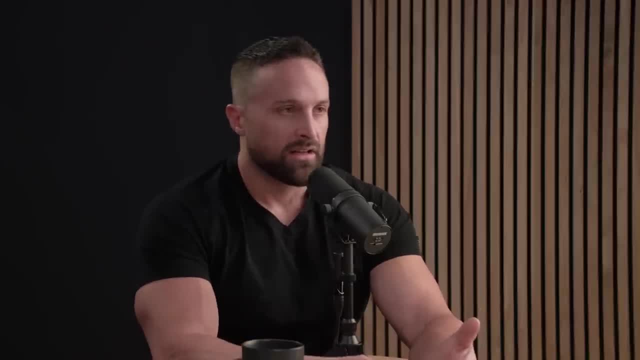 60,, 40 carbohydrate to fat of the remaining calories. Then you have low fat, which is obviously a higher ratio of carbohydrate. You have low carb. You have a ketogenic diet, which is very, very low carb, And then there's also a plant-based option. 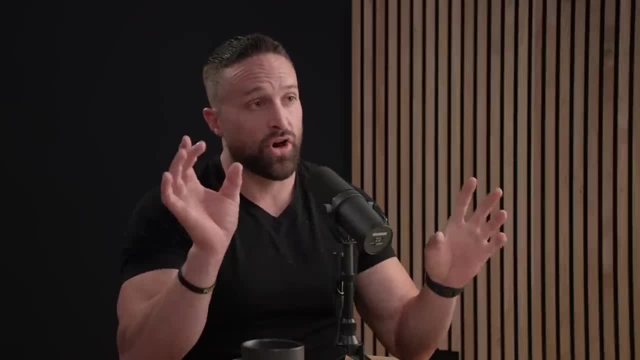 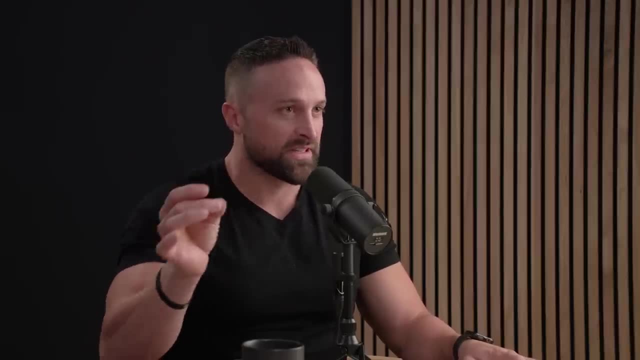 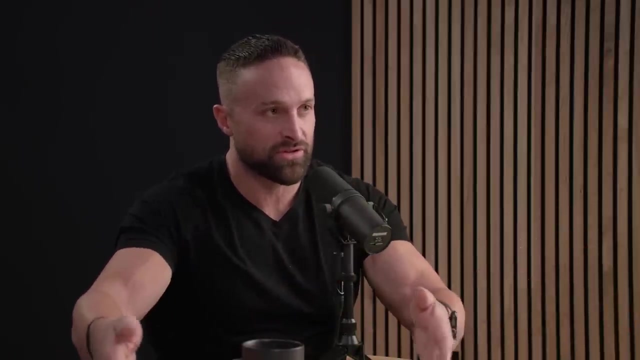 And within each of those options still, you can go in and actually shimmy the macros a little bit within a certain range so that you can kind of dial in what your specific dietary preferences. because, again, if we go back to what is going to produce the best long-term results, it's whatever the person can adhere to. 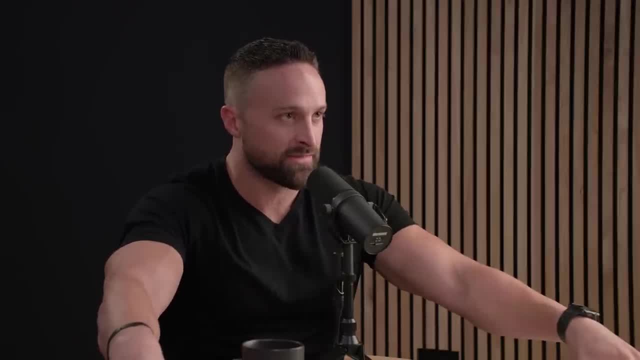 So we really try to start with the concept of adherence by allowing people to have the dietary preference that they want. And there's some other apps out there that are good- apps Like um, for example. we get asked a lot: what's the difference between our app? and? 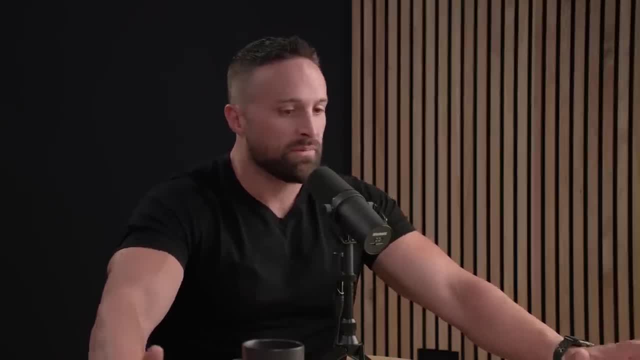 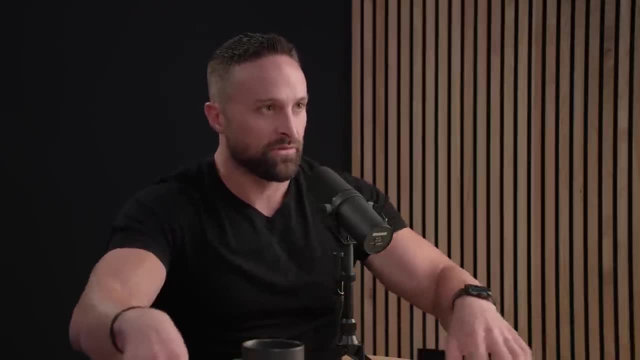 the Renaissance periodization app And they have a great app, Um, but theirs is kind of more rigid and it'll say: you know, you're going to eat this many meals and you're going to have these foods at these times. So we're kind of the opposite. We want to give you maximum. 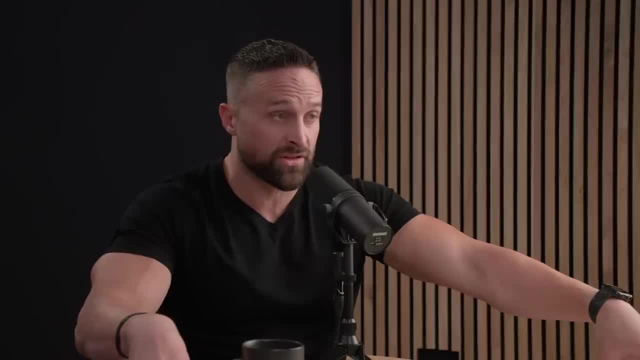 maximum flexibility. Now, for some people they would prefer the rigid structure at first, Um, but we find that for most people, giving them more flexibility, uh, typically improves adherence over the long run. So that's kind of how the app works. And again, like there's, 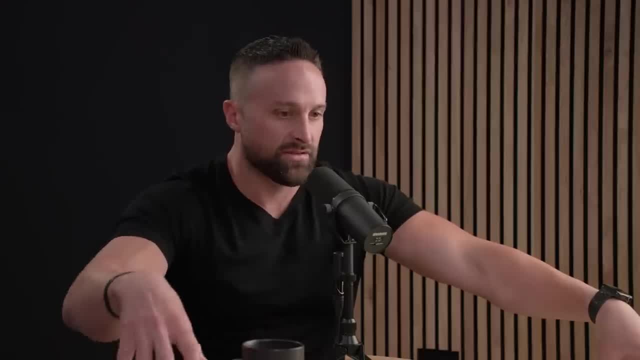 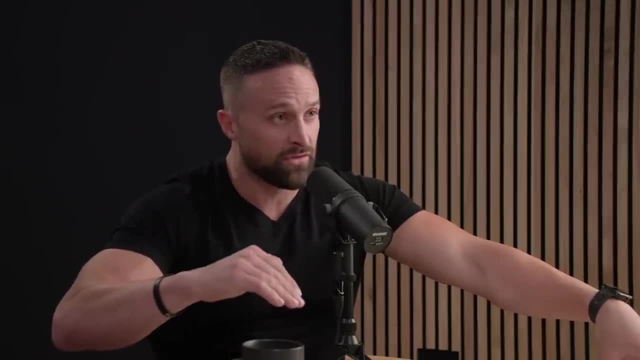 multiple different goals. It's not just a weight loss app. There's a maintenance, there's a muscle building, Um, so you've got all kinds of different goals that can be accommodated, different rates of each of those goals, And I mean I've used the app for 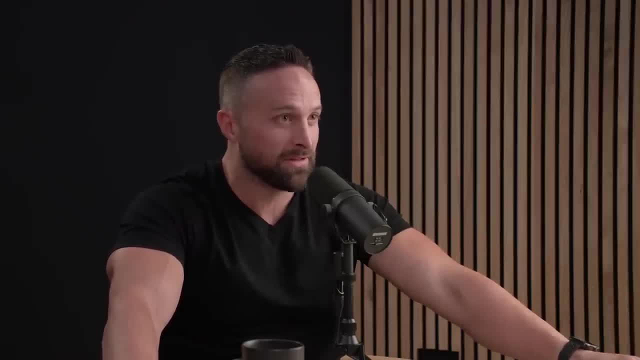 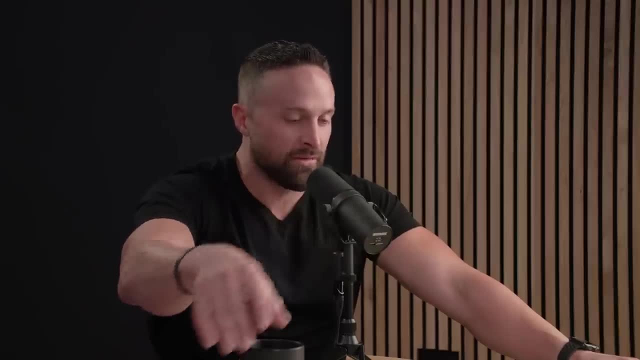 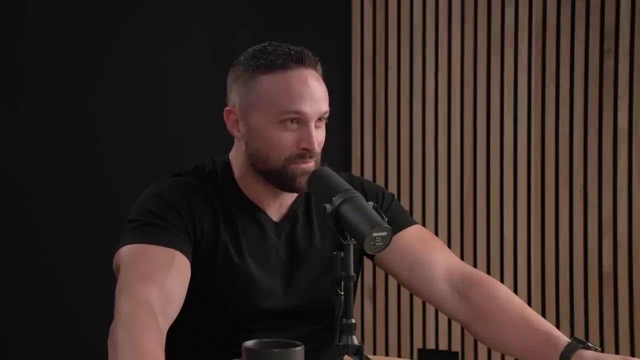 over three years now to do my body weight. And I mean like when I say that it's dialed me in because I'm I'm very regimented with, you know, logging and and and logging my weight. So what I targeted to weigh in at worlds, I got down to the 0.1 kilogram, So it was pretty cool. 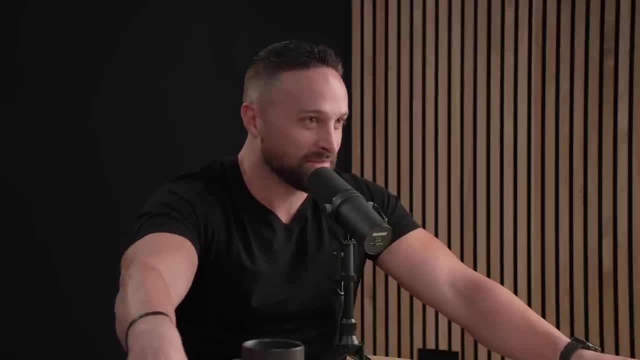 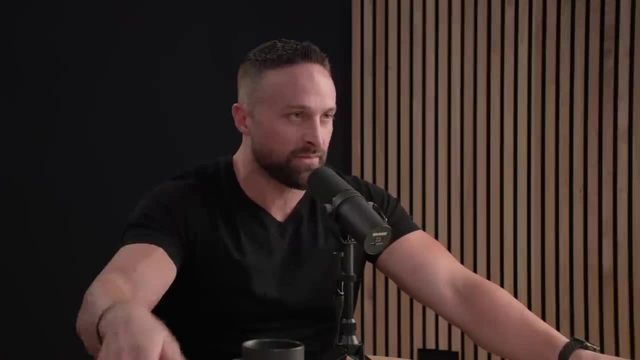 to be able to, like, use a tool that I helped develop to actually coach me. So it's a great tool. Um, you know, we, we, we did some statistics. we polled 2,500 members And, uh, one of the questions we asked is: 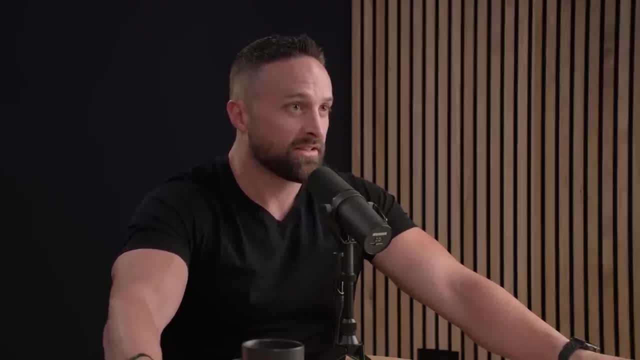 would you recommend this to a friend? And 91% said yes. So we, we on our average. I think our average retention is like seven months, which, for an app that costs $10 a month is is really great. So 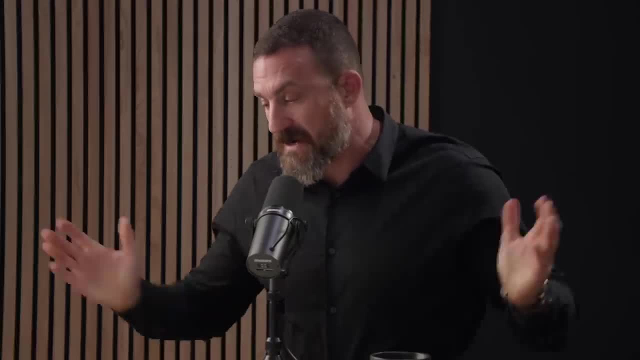 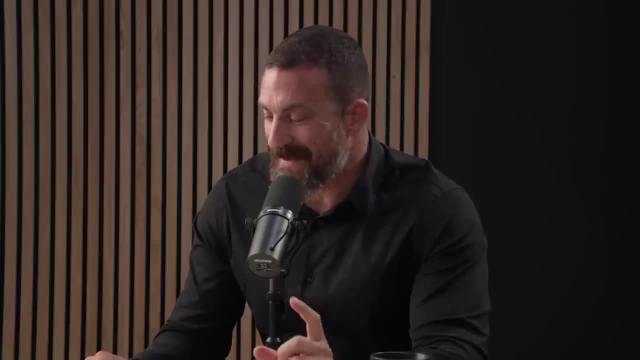 yeah, as I mentioned, a number of people I know use it. this is not a paid promotion, I um, but I think people need guidance and tools, And what we know about the human brain is that winging it can work, but that, uh, the brain. 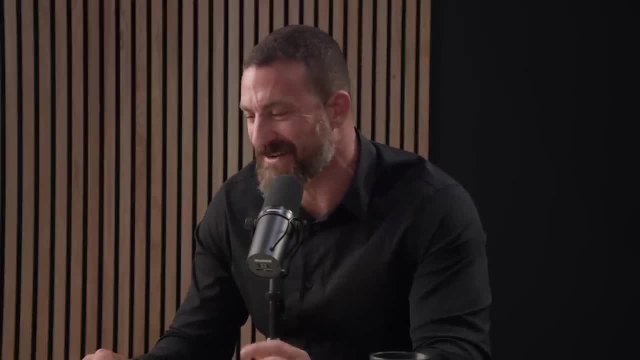 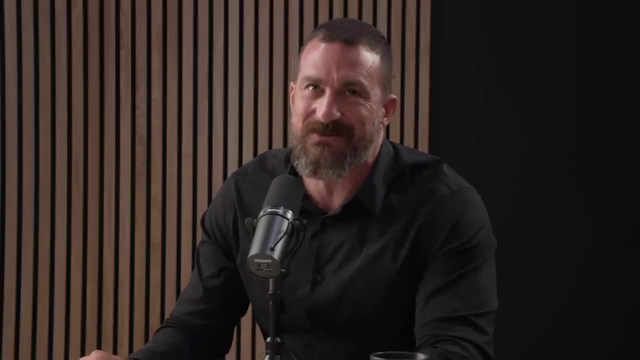 um, will cheat itself often. Um, what's? there's a Feynman quote about this and I'll get it wrong And always bad to try and quote Feynman, uh, anyway, cuz he said it so much better, but that we are the easiest. uh, you know, it's easy to fool ourselves. basically is what he was. 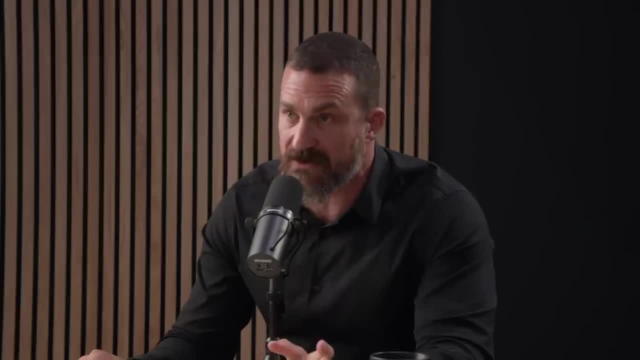 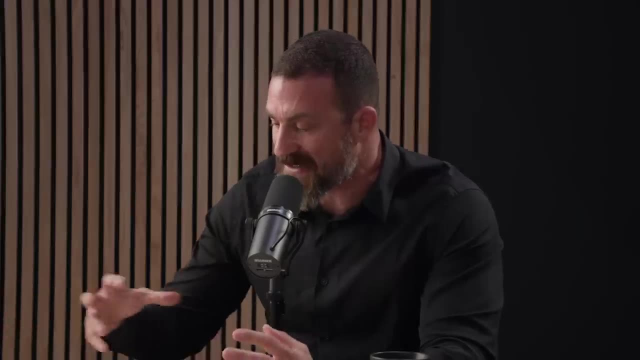 saying Easiest to fool ourselves. Absolutely. Um sounds great. We will put a link to it so that people can um check it out. Uh, again, uh, it sounds like a, a wonderful tool and and a tool that nets a lot of the, the principles that sit as um major themes for weight loss. 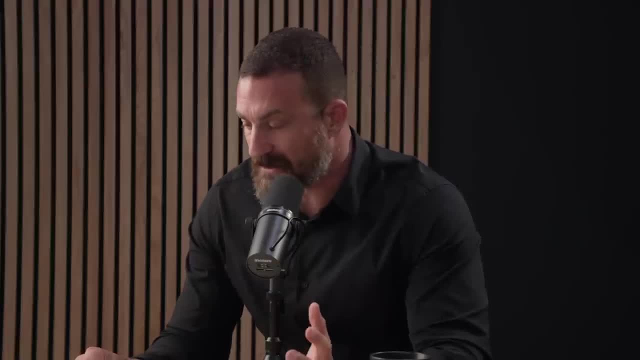 weight gain- I would assume uh directed, uh lean muscle, uh lean tissue gain is what most people are after- and weight maintenance, because a number of people would like to just maintain. Listen, I really appreciate your time and all that you're doing. Um, certainly your time and energy. 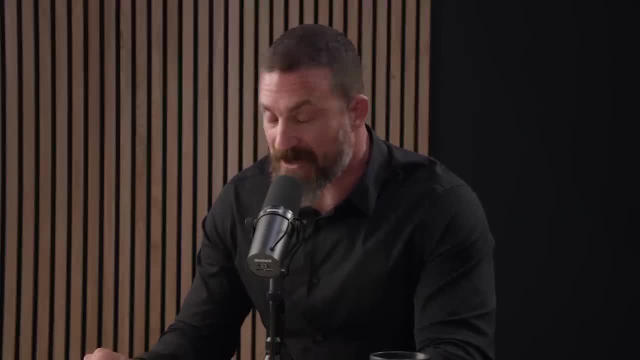 and knowledge today, but also what you're doing on the various social media channels, And and just the fact that somebody from the depths of academia, um is out there sharing so much knowledge across so many domains. Um, you're a gem in this landscape of of nutrition and one that people really um need to hear from. 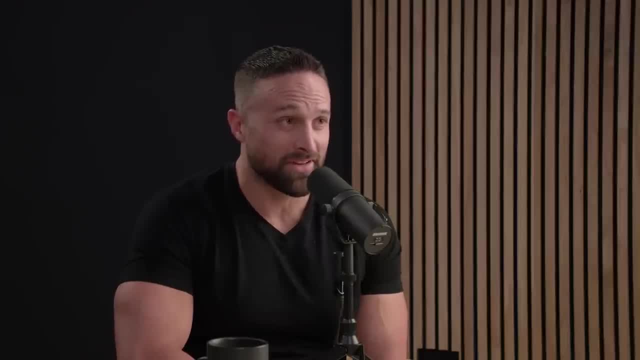 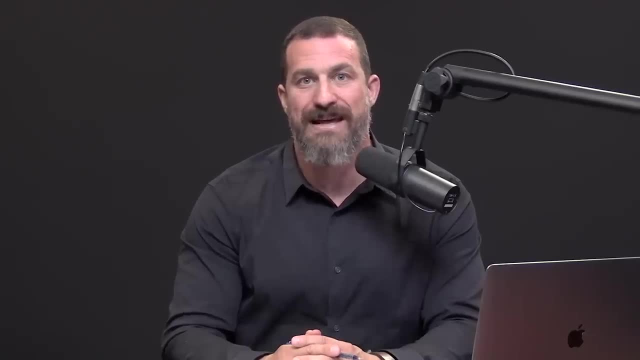 So thank you so much for your time. Thank you, I appreciate the opportunity. I really enjoyed it. We'll do it again. Thank you for joining me today for my discussion with Dr Lane Norton. I hope you found it to be as interesting and informative and actionable as I did. If you're learning from enter and join this. 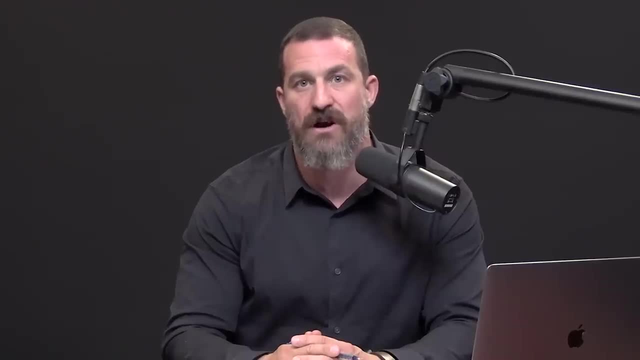 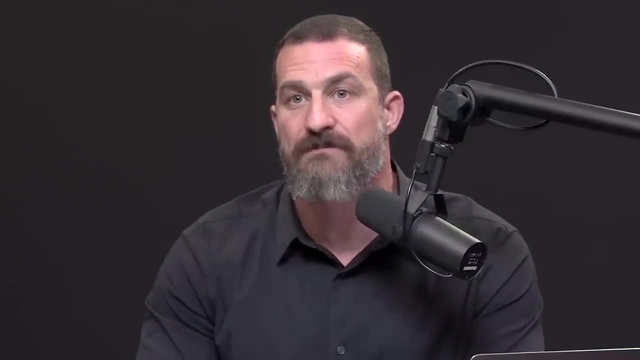 podcast. please subscribe to our YouTube channel. That's a terrific, zero cost way to support us. In addition, please subscribe to the podcast Podcast on Spotify and Apple, and on both Spotify and Apple, you can leave us up to a five-star review If you have questions or suggestions about topics and guests you'd like me to include. 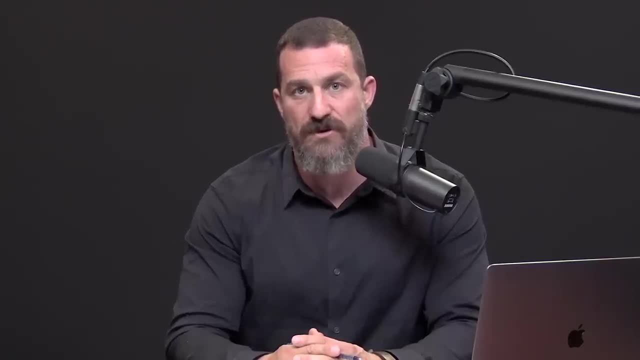 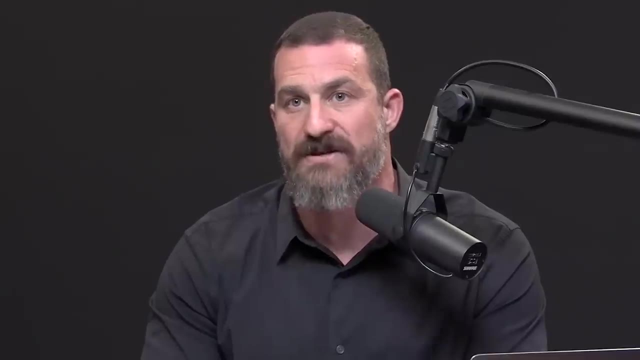 on the Huberman lab podcast. please put those in the comment section on YouTube. I do read all the comments. In addition, please check out the sponsors mentioned at the beginning of today's episode. That's the best way to support this podcast. during today's episode And on many 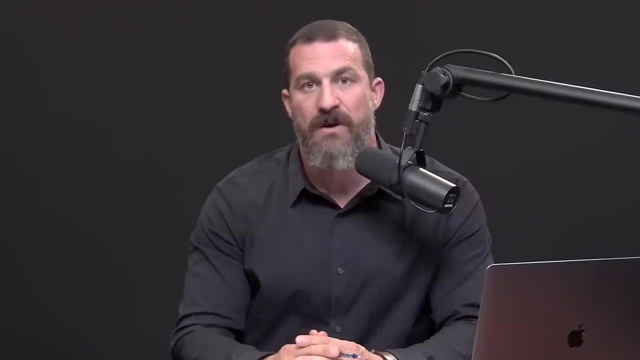 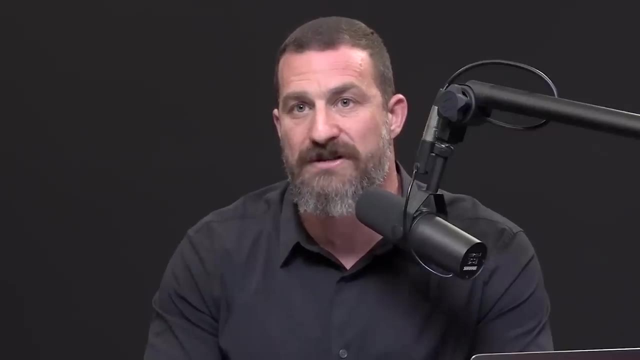 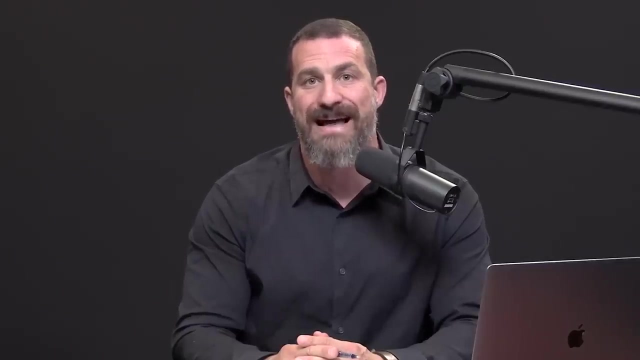 previous episodes of the Huberman lab podcast, we discussed supplements. while supplements aren't necessary for everybody, Many people derive tremendous benefit from them. So if you're interested in learning more about the Huberman lab podcast, please go to live momentouscom slash. 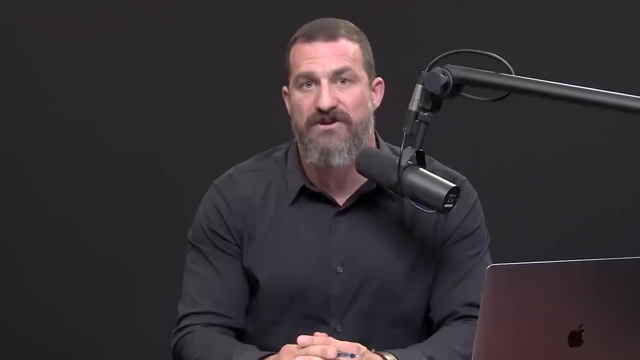 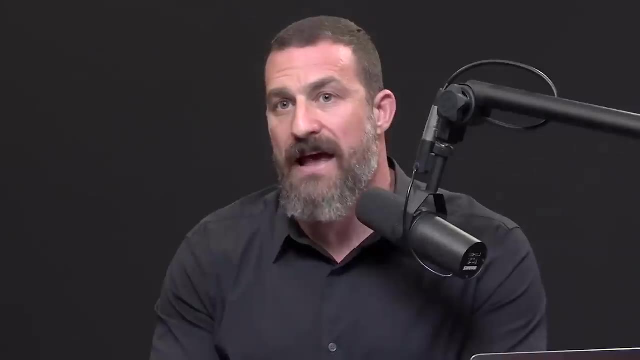 Huberman We partnered with momentous because they are extremely high quality, They ship internationally and they formulated supplements in the precise ways that are discussed as optimal to take for various outcomes here on the Huberman lab podcast. The Huberman lab also has a zero cost. 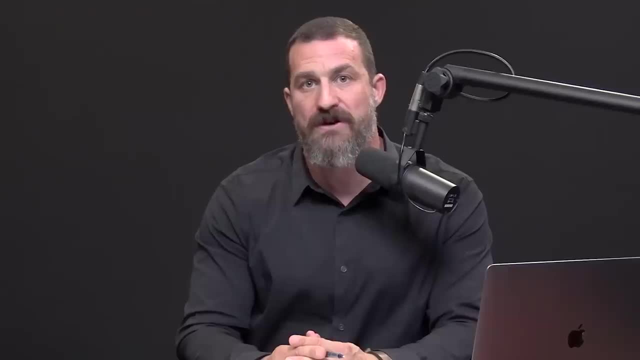 newsletter that you can access. It includes summaries of podcasts, episodes, as well as summaries of various protocols for mental health, physical health and performance. You can sign up for the newsletter by going to Huberman labcom, going to the menu and look for the neural network newsletter signup. You just provide your email. 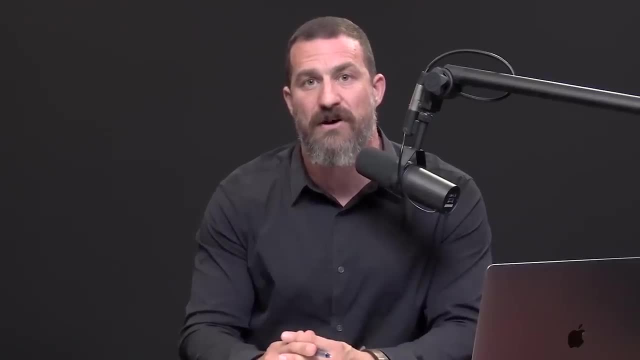 And I assure you we do not share your email with anybody. And again, it's completely zero cost. Again, go to Huberman labcom and sign up for the neural network newsletter. And if you're not already following us on social media, we are: Huberman lab on Instagram. Huberman lab on 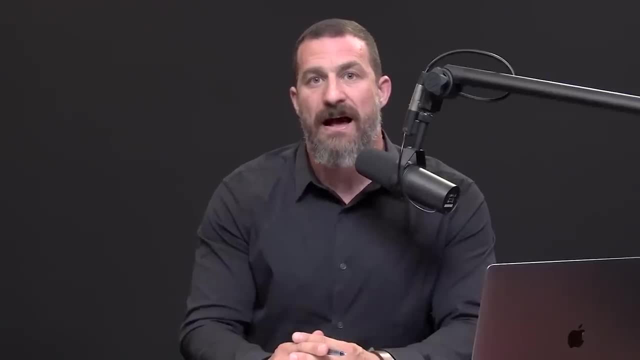 Twitter and Huberman lab on Facebook And at all of those sites, provide science and science related tools for mental health, physical health and performance, Some of which overlap with information covered on the Huberman lab podcast, but often which is distinct from information covered on the Huberman lab podcast. So, again, 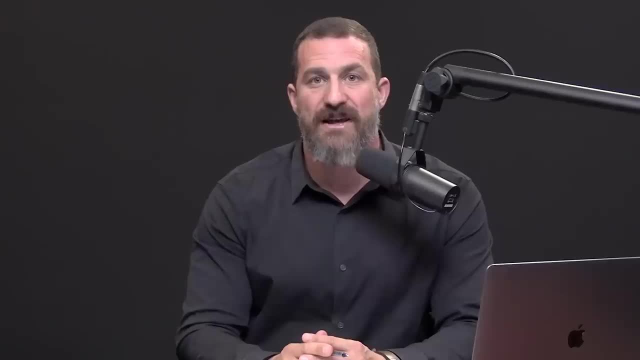 that's Huberman lab on Instagram, Twitter and Facebook. Thank you once again for joining me for today's discussion with Dr Lane Norton, If you are interested in some of the resources that he and I discussed, including his carbon app, as well as other resources that he provides. 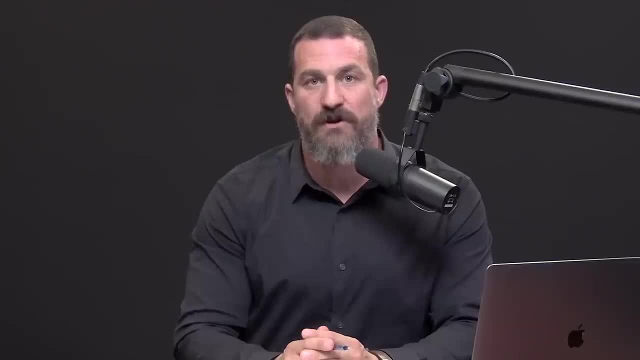 please go to the links in the show note captions and, last but certainly not least, thank you for your interest in science. 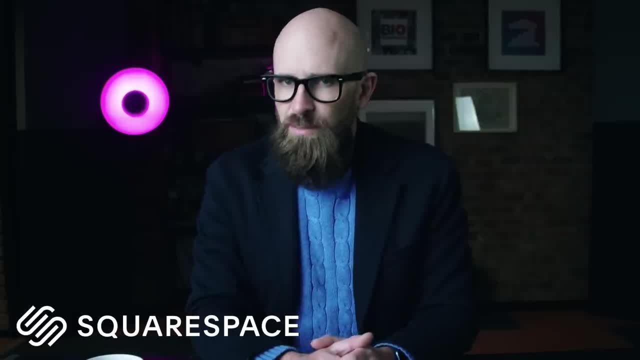 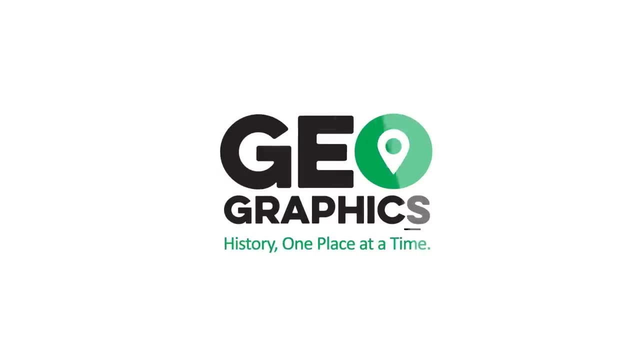 Today's episode is brought to you by Squarespace, the tool to use to make a website for your brand or business. More about them in just a bit. There was a time when Earth came perilously close to losing all life upon it. This mass 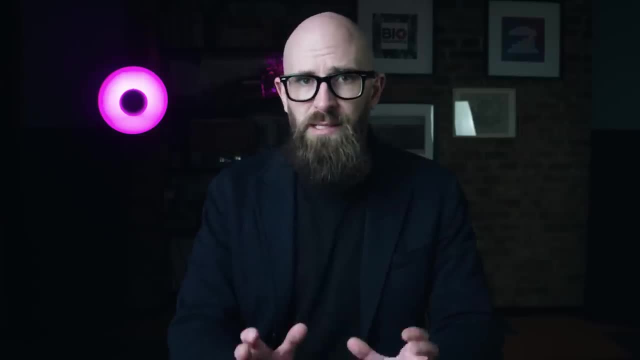 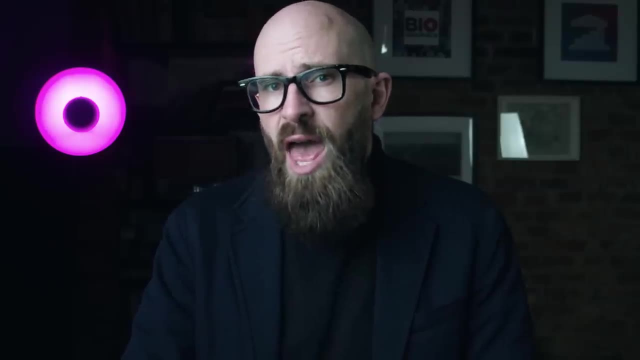 Yet we can understand what happened. despite the utterly vast expanse of time involved, The array of animals wiped out in massive numbers can seem tangible when we contemplate their fossilized skeletons and imagine how they must have looked roaming their ancient world. Some of those peculiar beasts looked nothing like us. Thankfully, so were our ancestors.